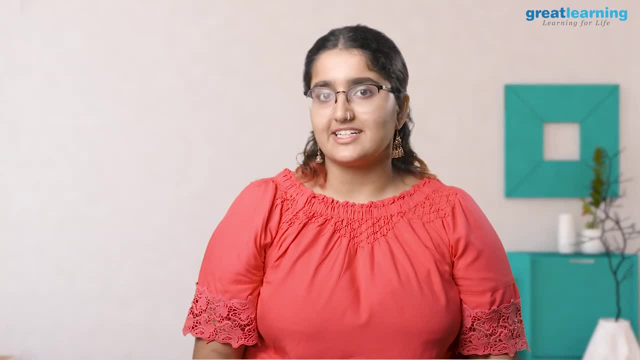 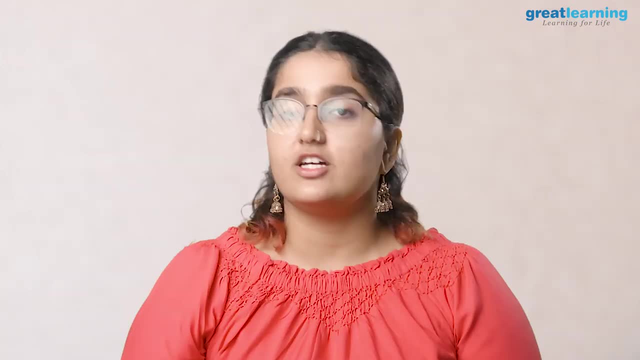 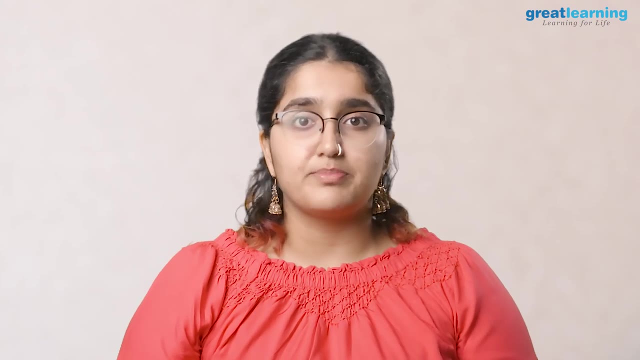 growing startups are always in search of big data experts. Now, before we start off with the session, I'd like to inform you that we will be coming up with a series of high quality tutorials on computer vision, cybersecurity, cloud computing and so much more. So don't forget to. 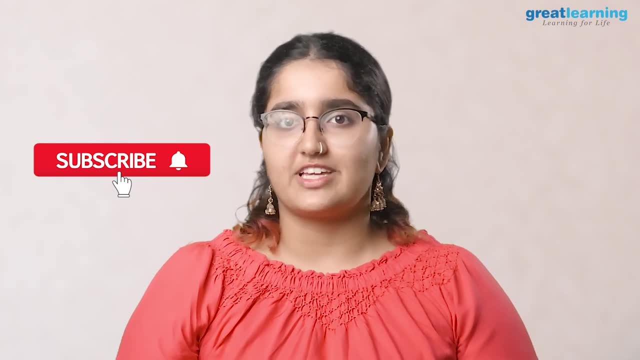 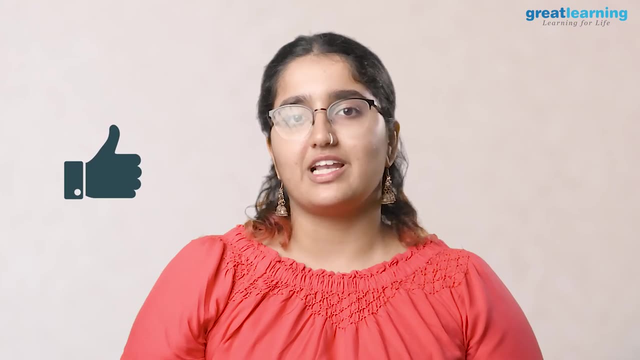 subscribe to our channel and hit the bell icon so you get a notification when we upload new videos. If you like this tutorial, don't forget to click on the thumbs up and comment down below what you'd like to see next. Now let's go through what you will learn today. First, we will discuss what 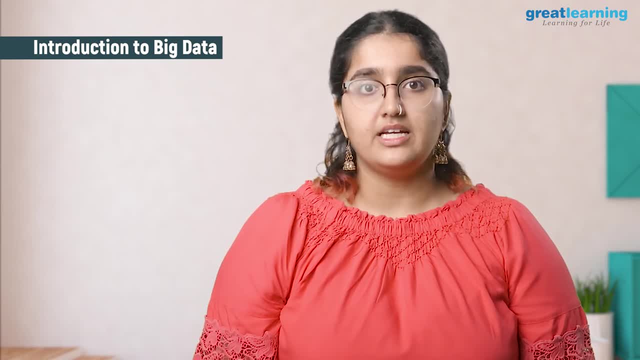 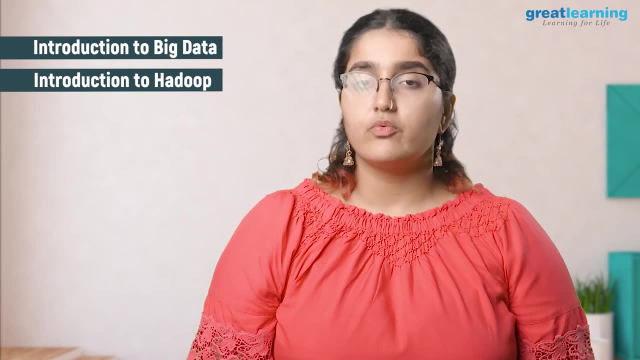 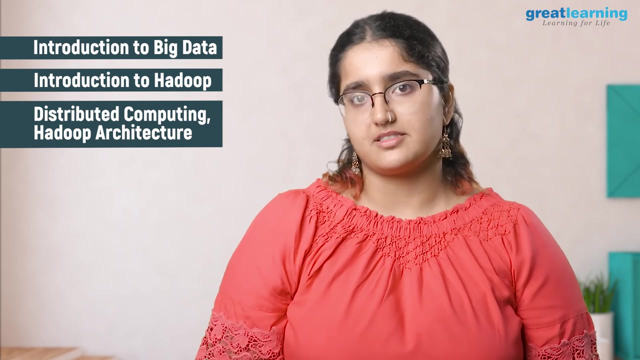 exactly big data is and some processes associated with it in traditional data analysis. Then we'll get introduced to Hadoop and understand it a little better. We'll move on to distributed computing and Hadoop architecture and learn how we can store a file on Hadoop distributed file systems. 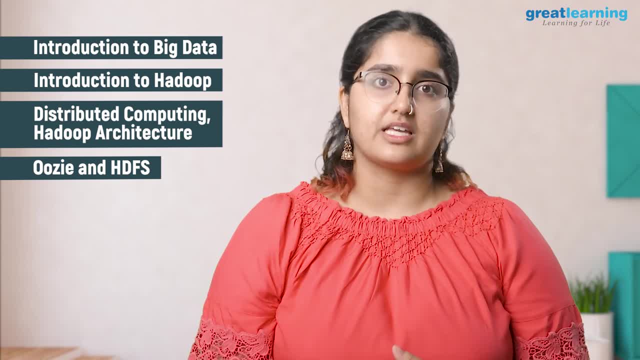 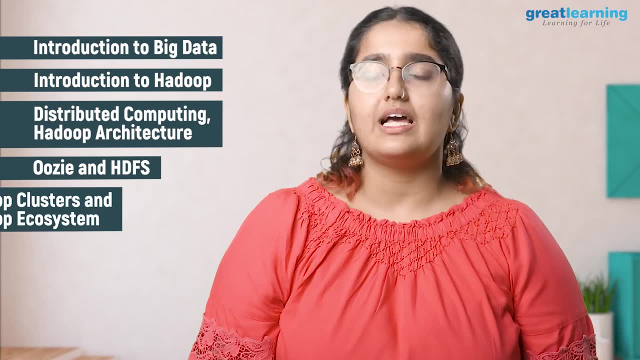 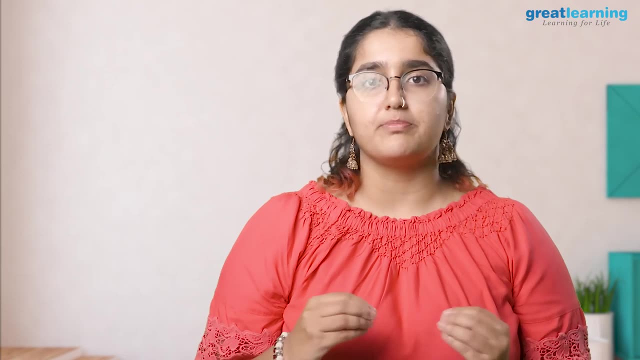 An introduction to Uzi and HDFS processing will get you right on track to understand how you can really utilize Hadoop for your data. Then we'll help you comprehend Hadoop clusters and how Hadoop ecosystem is built. We'll also delve into MapReduce what it is and an example to help you understand. 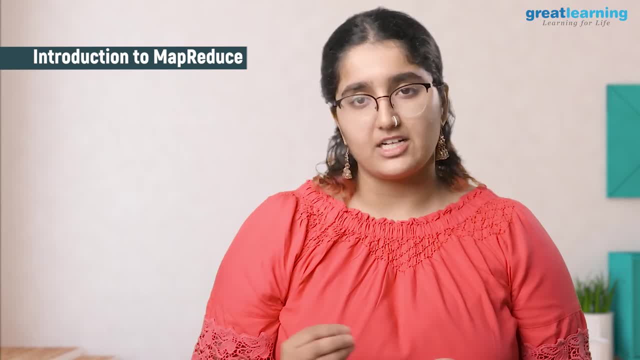 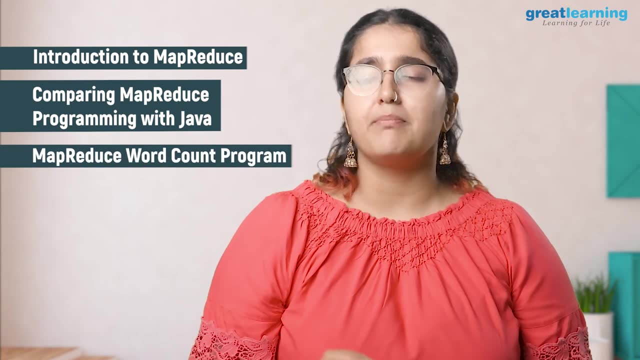 better To get some good insights and context. we will then compare MapReduce programming with Java. Next we'll dive into Hadoop, dive in to try a MapReduce word count, program Code and all, And to tie it all up, we'll discuss. 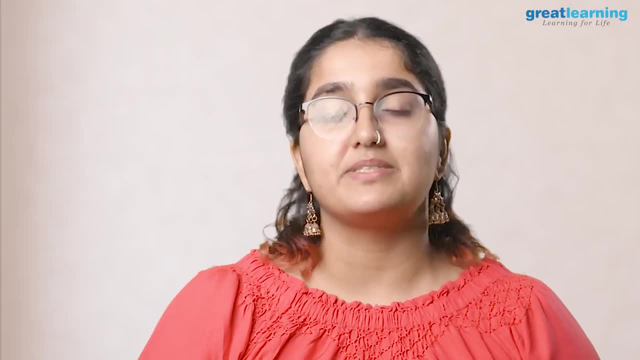 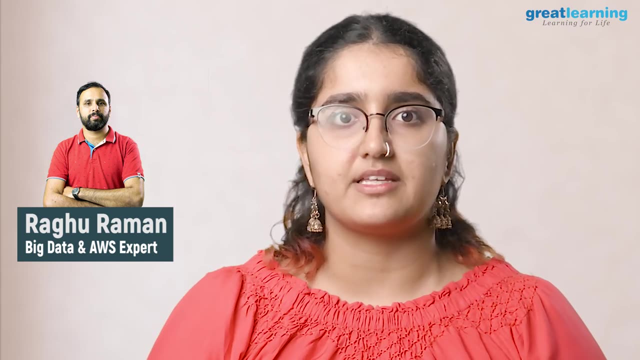 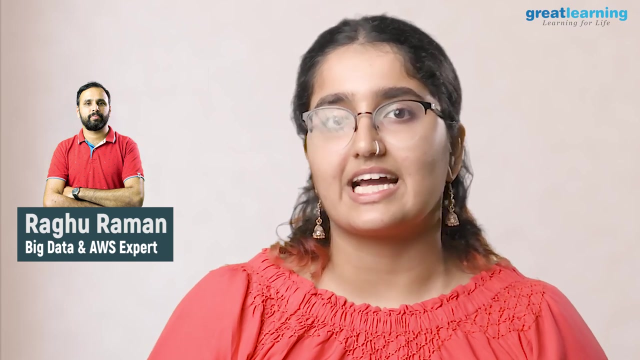 the aspects of Apache Hadoop Yarn. This course will be taught by Mr Raghu Raman. Mr Raghu Raman is a big data and AWS expert with over a decade of training and consulting experience in AWS and Apache Hadoop ecosystem. He has an impressive resume, having worked with global customers like 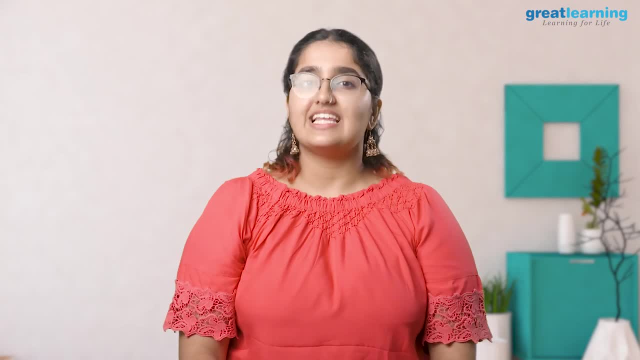 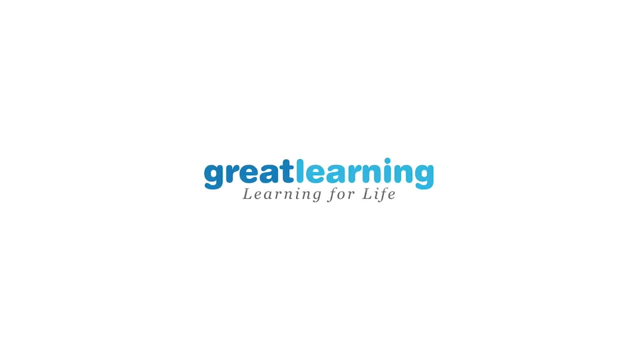 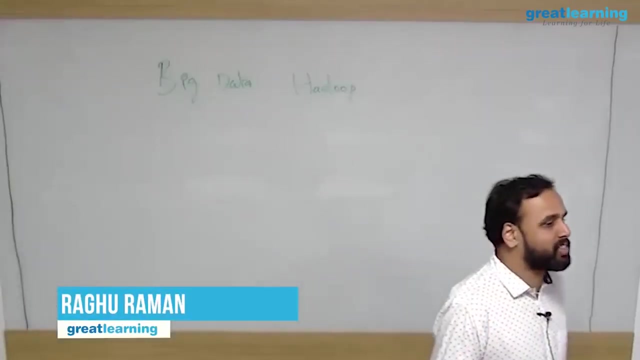 IBM, Capgemini and Wipro. With that, let's get into this amazing Hadoop course. It's time for some great learning. So who can tell me what is big data? So that is the first question: Who can tell? 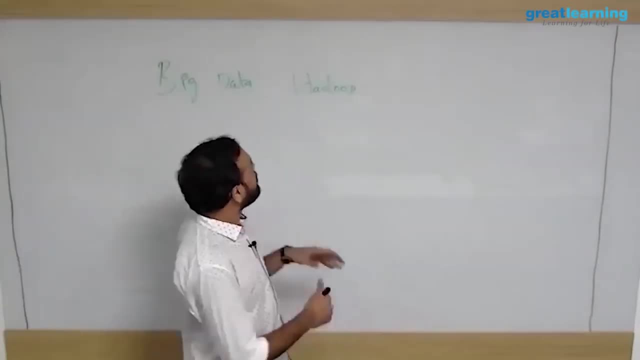 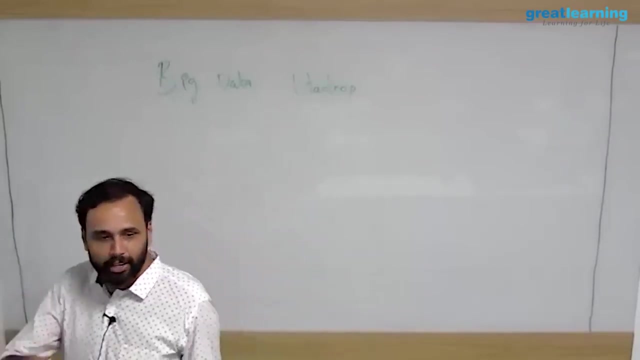 me: what do you mean by big data? Have you heard this term anywhere before? The definition of big data? if you Google, you will get First thing. you can just go to Google and say what is big data? You will get tons of articles, PDFs and presentations. You will get tons of articles. 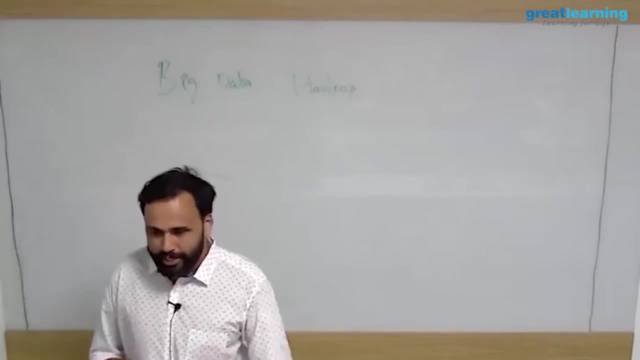 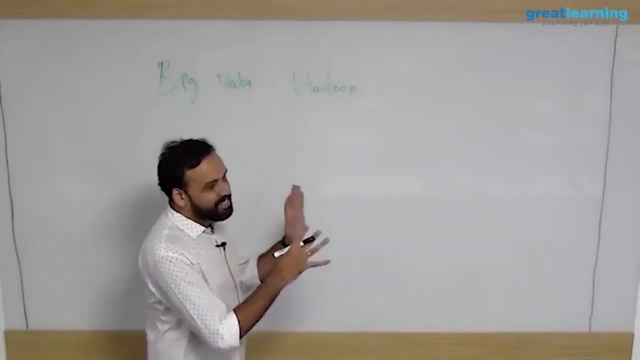 PDFs and presentations. That is not what I'm going to teach you. Let's take a practical use case, right? Let's take a practical use case and try to understand how big data actually makes sense, right? First of all, big data is related to IT, So you need some level of IT knowledge to 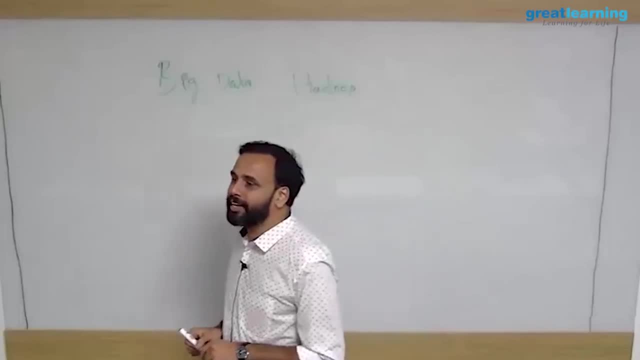 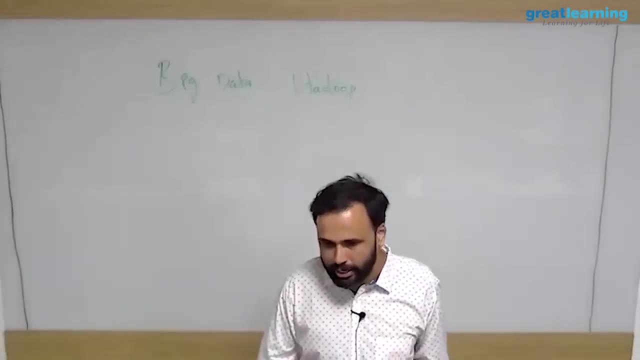 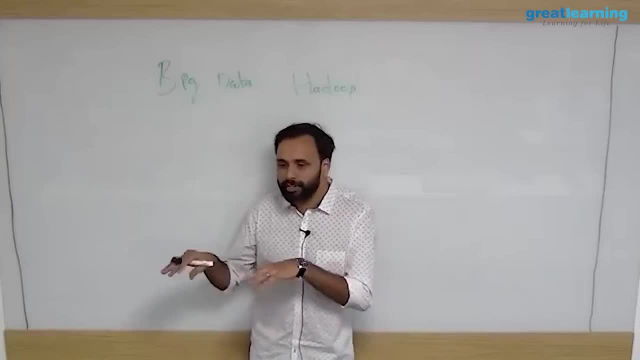 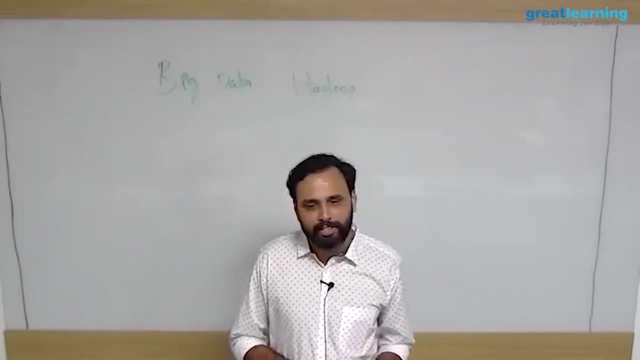 a company in Bangalore and we had created an application And I was working with a sales application. So basically what we do: if you install this application, there was a retail company. the customers will input all their sales data in that. So they will say that today. 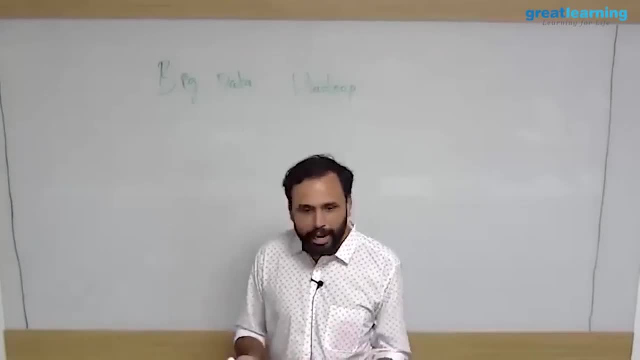 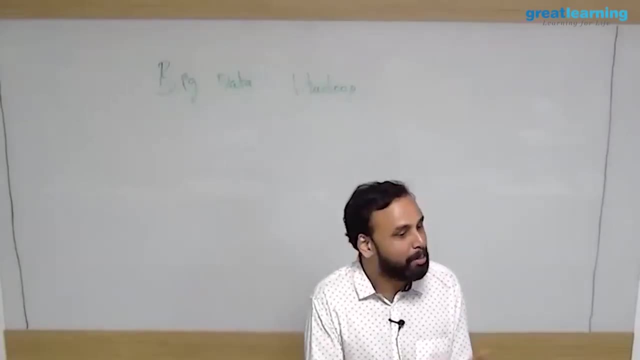 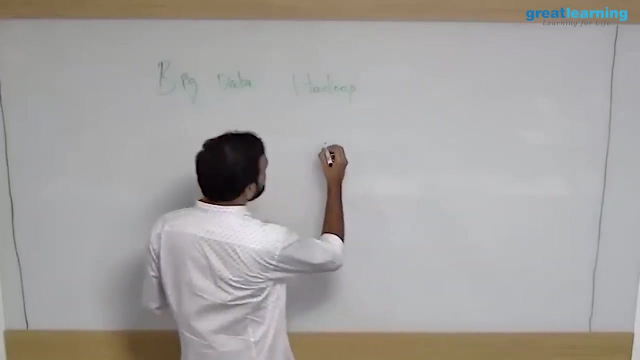 this much quantity item sold, sold and sold and sold, And this application will capture all the data, okay, and store it. Now, that was a very simple world. We did not have mobile phones, we did not have Facebook, WhatsApp, nothing was there 2005,, right, And we were using an RDBMS system to 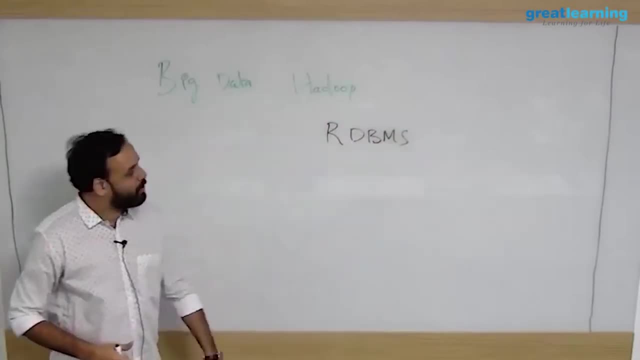 store this. You know what is an RDBMS. So RDBMS is what we were using to traditionally store the data, right, And what is an RDBMS system? It has a row column format. you have a table, you insert. 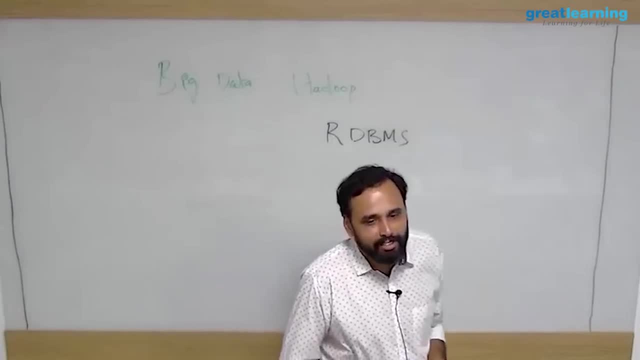 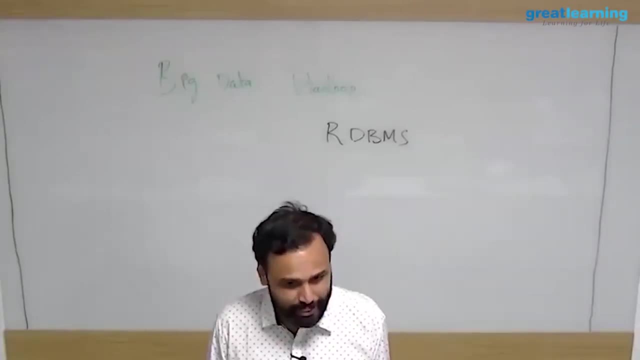 the data. Now, if somebody is teaching you RDBMS, they will say that: well, RDBMS is great, it can store everything, you know that's all fine, But unless your data starts increasing, right. So originally RDBMS can store everything. I don't have any. I'm not against RDBMS, but I don't have. 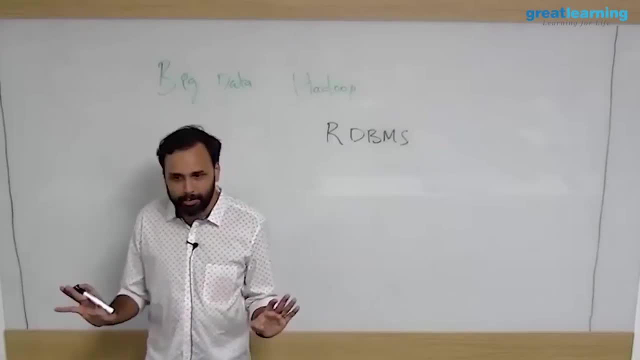 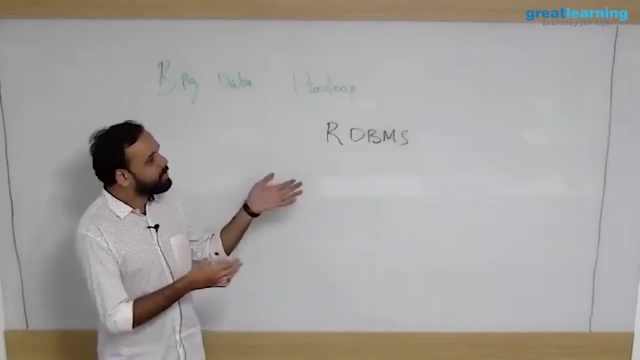 RDBMS or something, Even for transactional management. we use RDBMS, there is no doubt about it. MySQL Oracle- we were using MySQL actually. So whatever the customer is inserting, this MySQL will capture it. End of the year. you do some processing, you will understand how many. 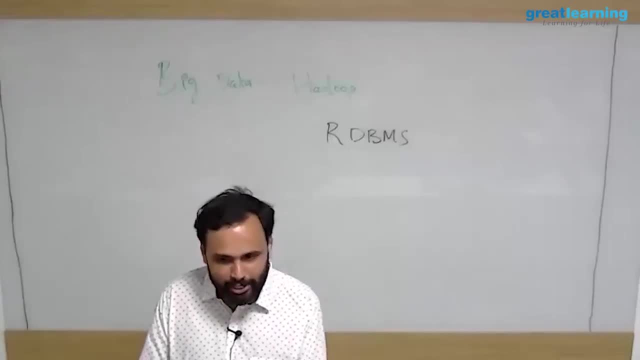 items were sold. Everybody is happy, happy. This is what was happening in 2005.. Fast forward to 2011.. I am working with ICICI Bank. ICICI Bank want to migrate to big data platform, So what is the problem with ICICI Bank? right? 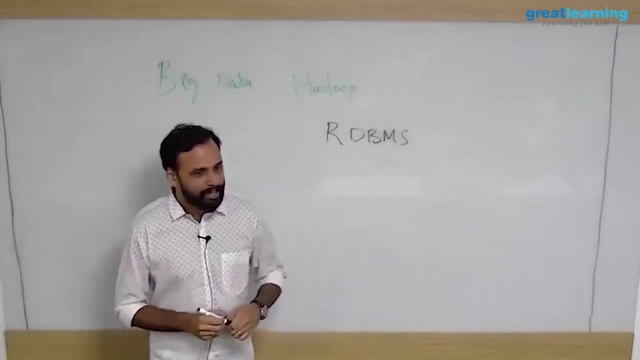 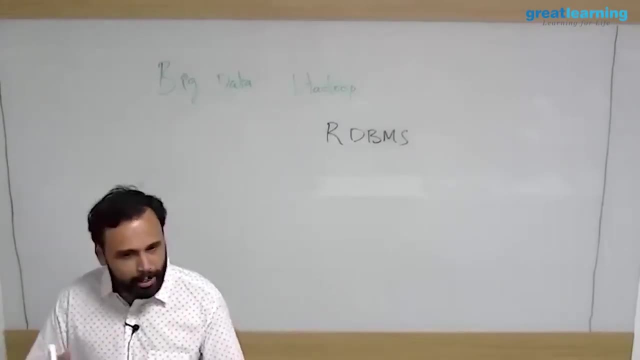 So that is the question Why ICICI Bank want to go to big data right Now. this example will also help you to understand the IT world right. So for people who are not coming from the IT background, they might need to understand how things are working right. So we went to ICICI Bank, we spoke. 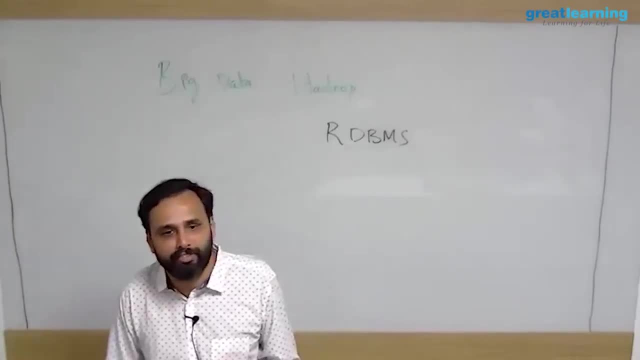 with them. we said: hey, what do you want? They said: you know what? we are facing? a lot of problems. We want to go to big data. We want to go to Hadoop. We'll see what is Hadoop later. 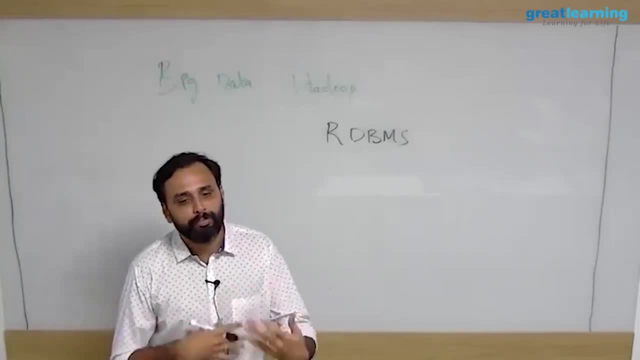 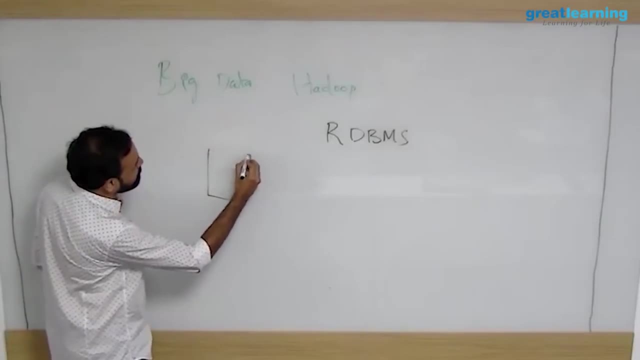 So we asked: what is a big deal? What is your problem? What are the problems which they were facing? One of the problems is that if you look at this RDBMS system- right, Your typical RDBMS system- What is RDBMS system doing? They will store the 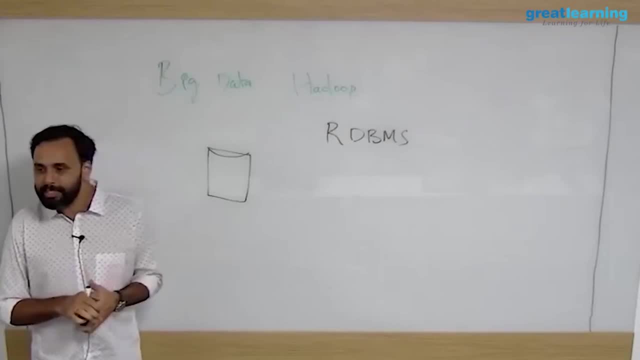 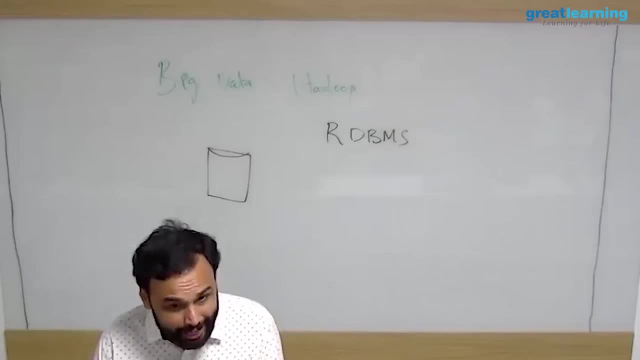 data in the form of a table. right Now, if your table size is very, very small, it's not a big deal. Even if you look at MySQL or if you go to Enterprise Scale Oracle and all you know, they can store gigabytes and sometimes up to terabytes of data. 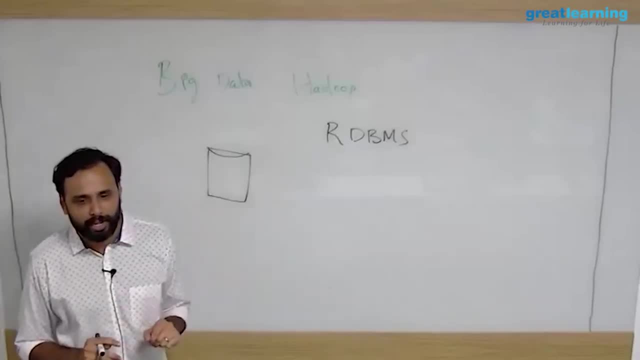 This size becomes big. So let's say I ask you: okay, you have to store the data in Oracle. The data is keep on increasing every week. You are not ready to migrate anywhere Oracle- if you talk only about Oracle, they have storage separate and DBMS engine separate In Oracle. 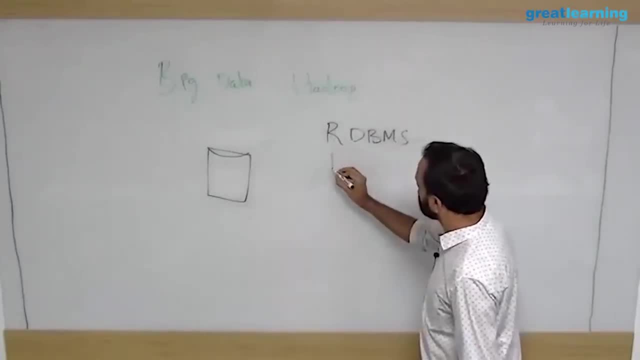 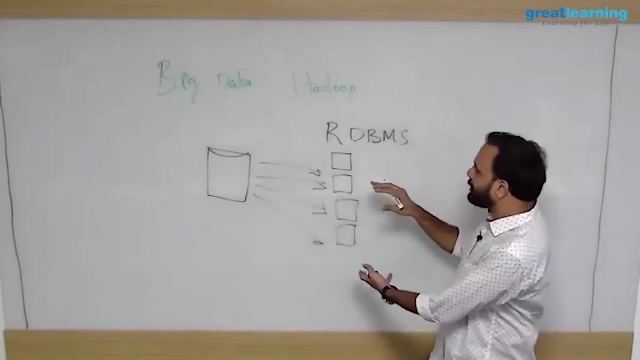 what I can do. I can purchase Oracle and I can add storage boxes as many as I want, You know. so these boxes will be in the network, So my database engine will be connecting to them and storing the data, whatever data I'm giving. So you can argue saying that I can. 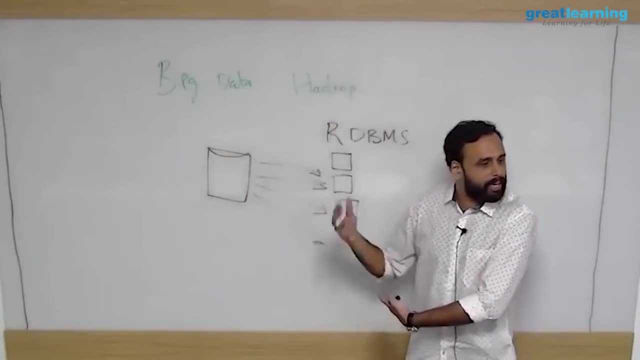 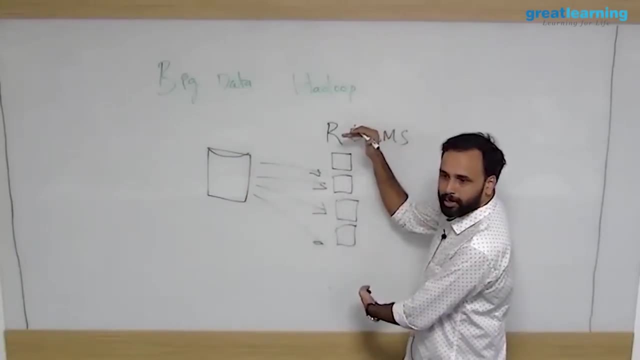 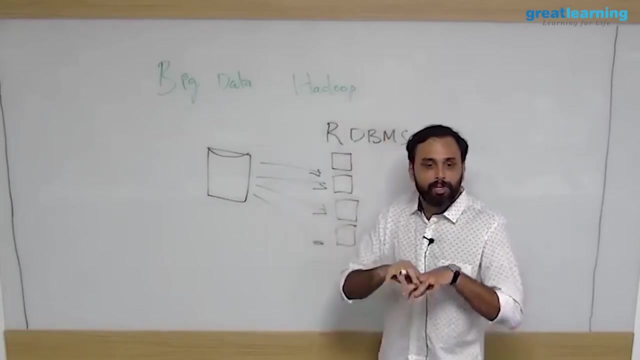 increase the storage capacity and then Oracle can store as much data as you want. There is no doubt about it, right, But there is also a limitation for the storage One problem. Second problem is that as this box increases, the storage in Oracle increases, you have to divide your data, So you 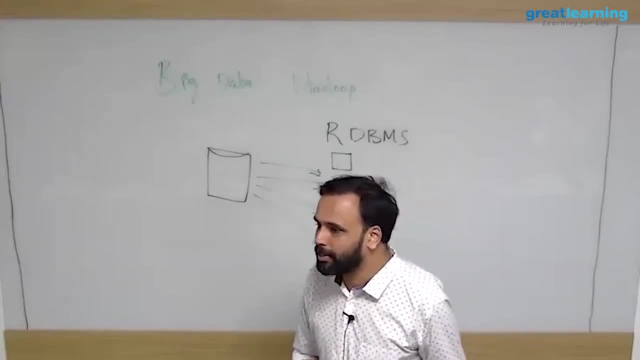 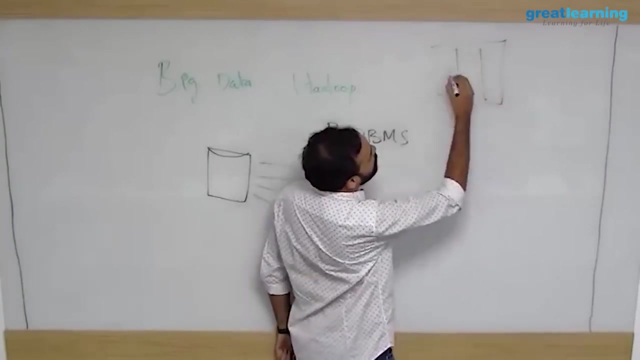 are selling iPhone, Let's say you're working with Apple, right? So one of the example is that if you are creating tables to store iPhone data, typically, if you look at the schema and all what we will do is that there will be one table- okay, there'll be one table wherein you will be having properties. 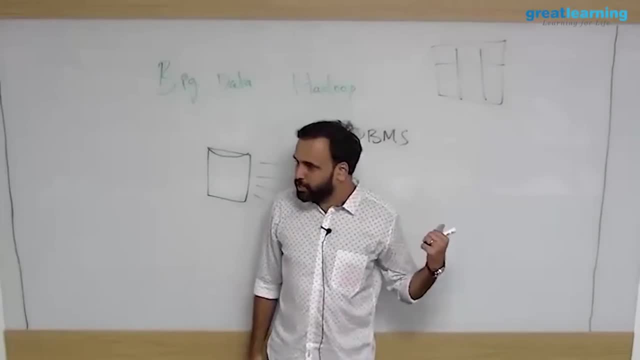 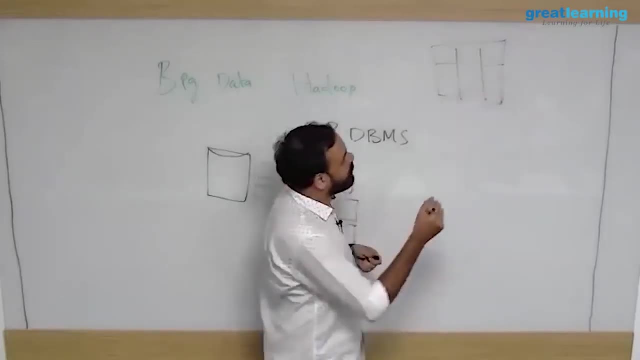 like you know how many items were purchased, at what rate they were purchased, how many people bought, so on and so forth. So this will be your items table. So in the items table you will have all the data related to the iPhones you were selling, right? 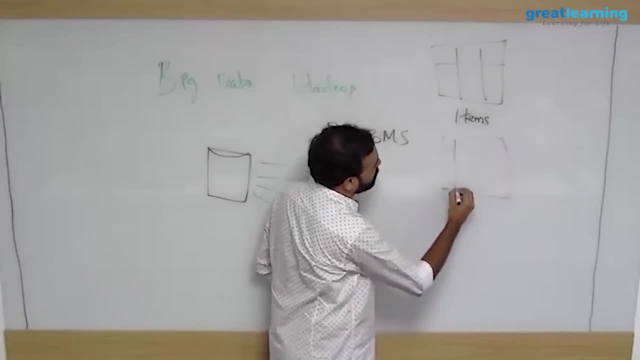 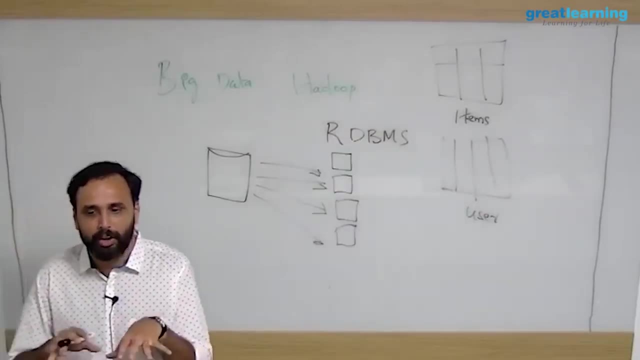 You will also have another table where there will be the user data. You will also have the user data. You know what is normalization In RDBMA systems. in order to avoid duplication of data, what we do is that we normalize the data. 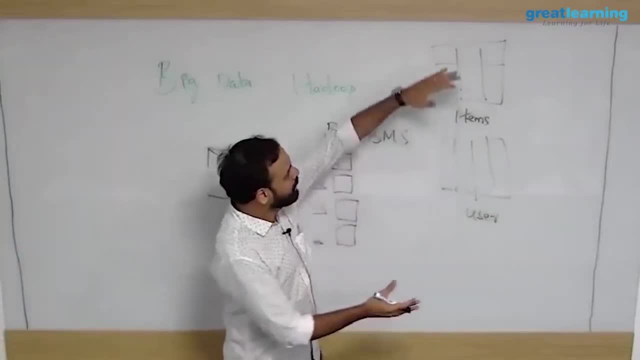 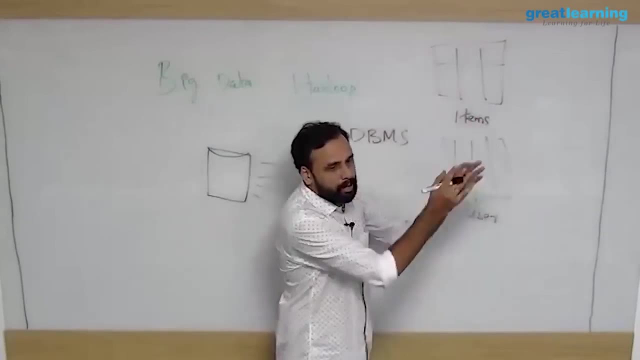 We always keep the data in different, different tables, So if I want to get both the data from this, I have to do something called a join query. I fire a join query and all the data from here will come and join and produce me the 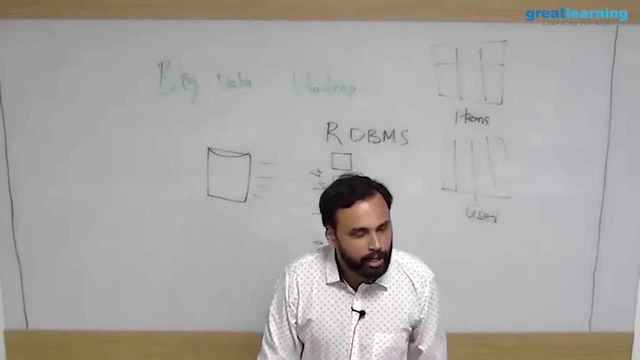 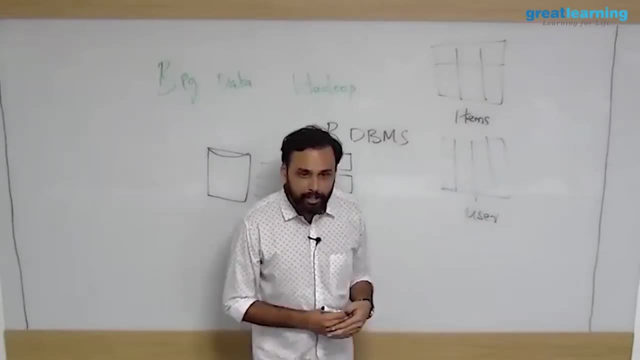 output. This is good if you are having small amount of data. What if you have terabytes of data here and here? My join query will fail or the join query has to wait Now. another point that people say is that if your RDBMS is becoming bigger and bigger, 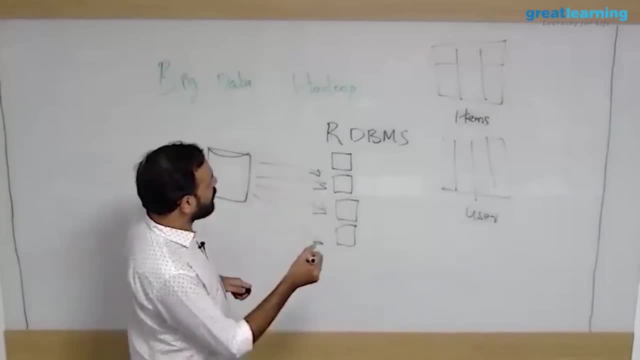 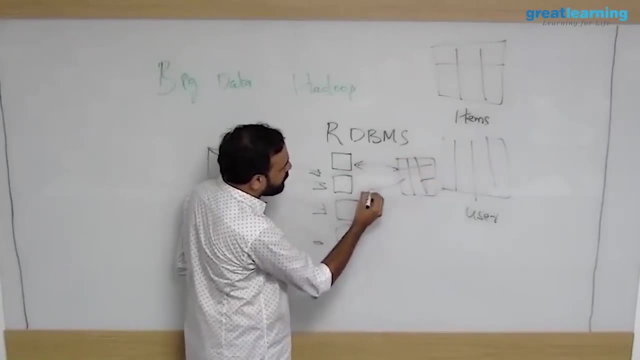 why don't you partition your data? That is possible. I can have like four boxes my one table. if this is my table, it can be logically partitioned and kept on four machines. if it is becoming bigger and bigger, This is possible. 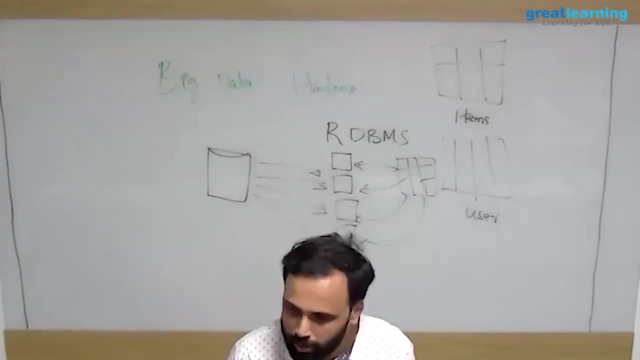 There is something called logical partitioning. Look at the iPhone data. I can say all the data where people from India are buying the iPhone go to this machine. that's called logical partitioning based on the country column. So here I have all the India data where people are buying iPhone. 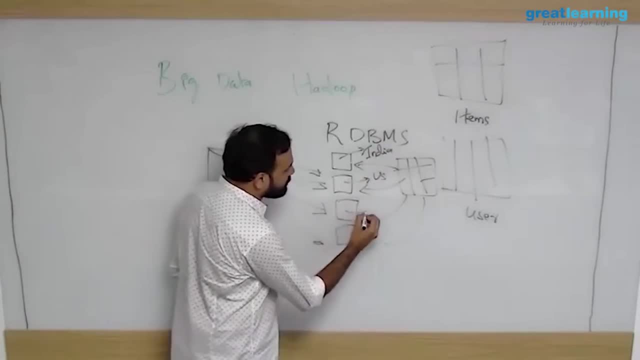 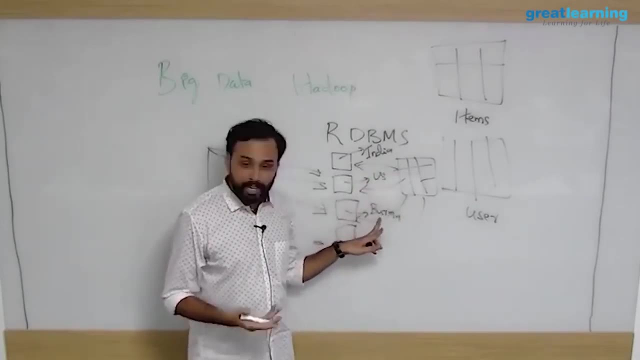 Here I have the US data where people are buying the iPhone. But the problem is, here I'll have the Burma data also. India data will be, let's say, two terabyte. China data will be three terabyte. This will be KBs actually. 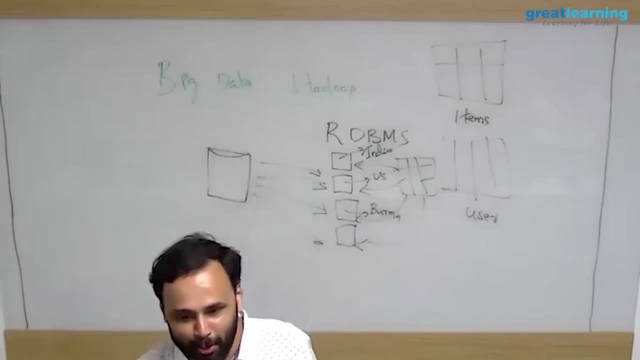 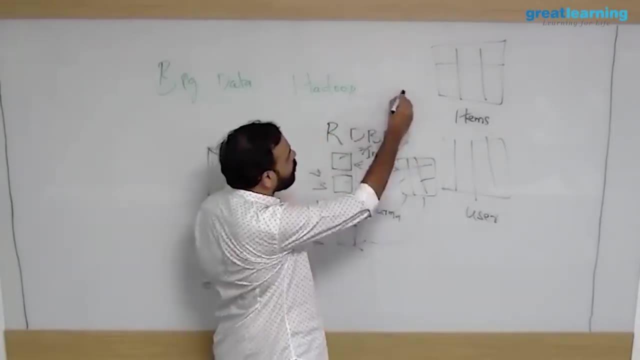 Because in Burma I don't think a lot of people are actually buying iPhone- probably Right, Exactly. So the problem is that if a table is becoming so big, I can cluster it. I can take four machines in my RDBMS or data warehousing architecture and I can say partition. 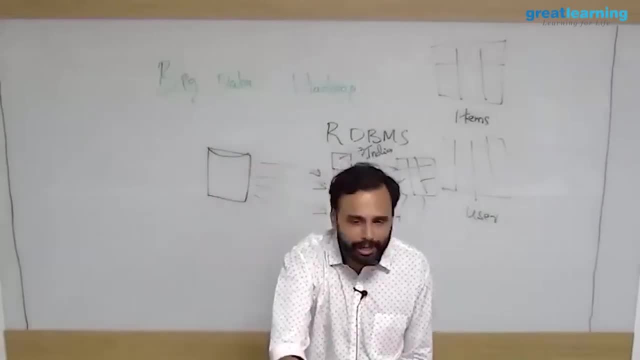 the data, Because if a table is so big, if I fire a query, the query will take a lot of time. So what I do? I say that, okay, don't store the full table, divide the table or partition the table. 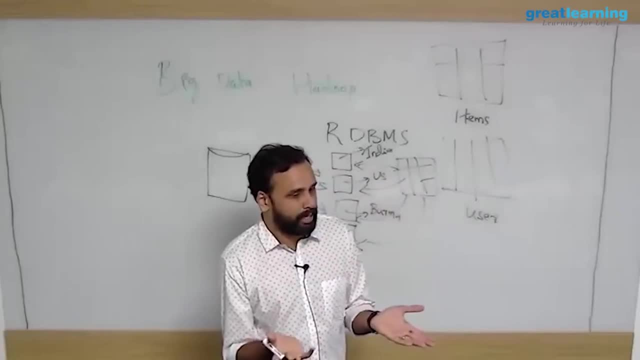 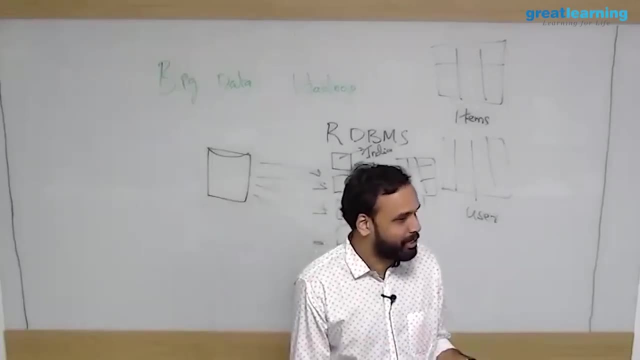 To partition. So I have to say that you have to use some logic for partitioning. I cannot physically divide the data. That's not possible in RDBMS. I cannot say that. take a table and cut it into four Doesn't work. 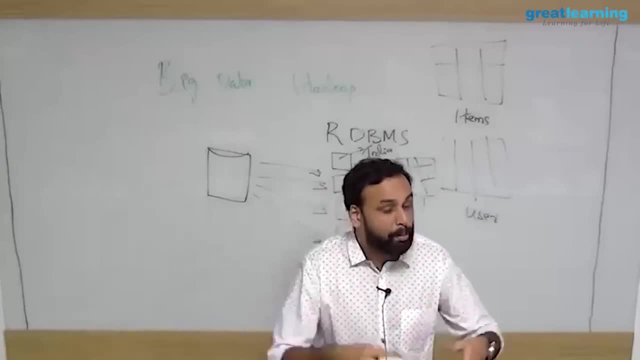 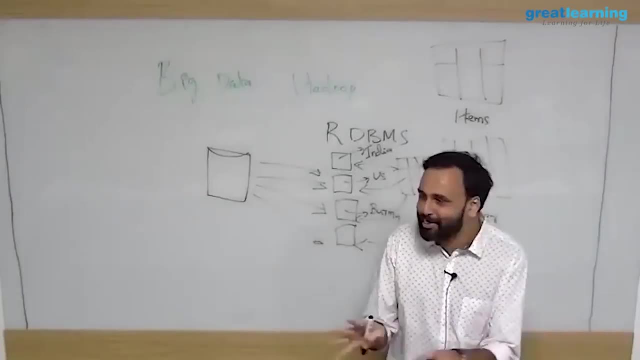 So I have to logically partition. So I have to say that there is a country column. How many countries are there in the world? Maximum: 155.. Right, I'm not much of a geography person, but I think somewhere around 155. 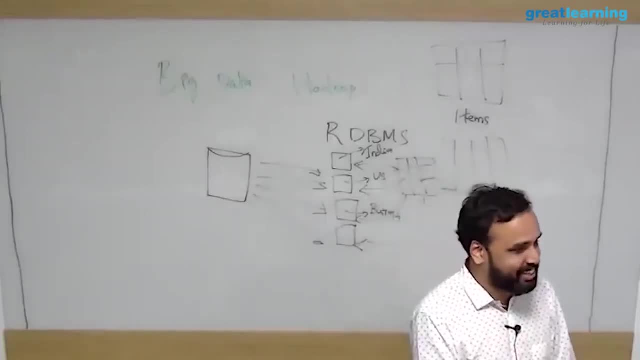 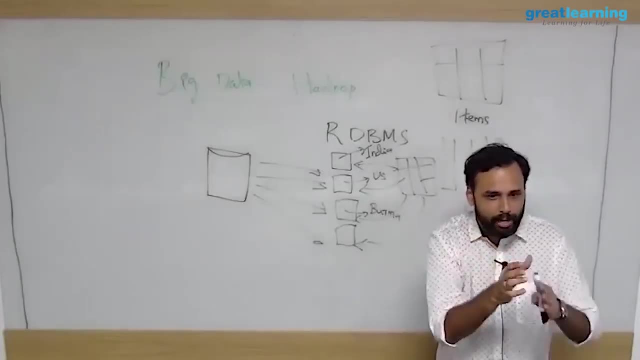 Right, But at least people who buy iPhone, 155 countries are there. So I will say: take the country column, So everybody who is buying an iPhone will have a country column. So, based on the country column, it will partition your data. 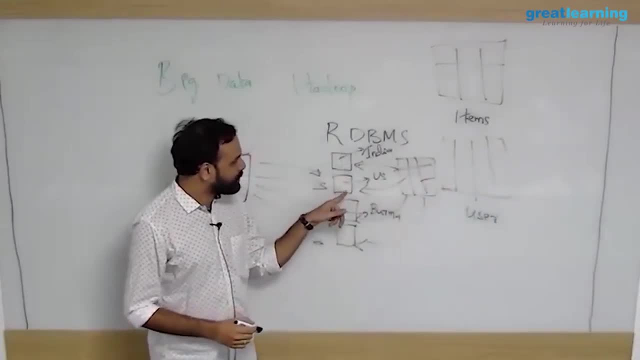 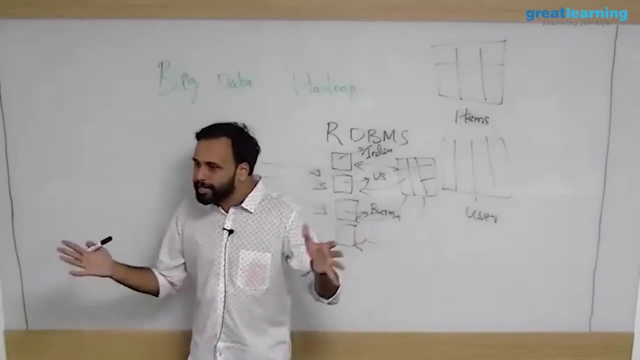 Right Now I have four boxes. This box has India data, US data, Burma data and something data Again. same story if you're running the join query, this box has to process all the India data for join query. This box will complete very fast. 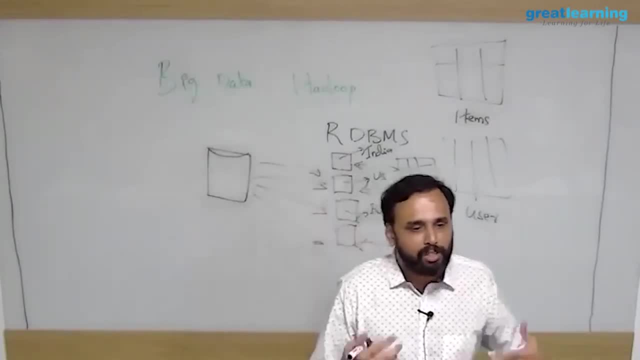 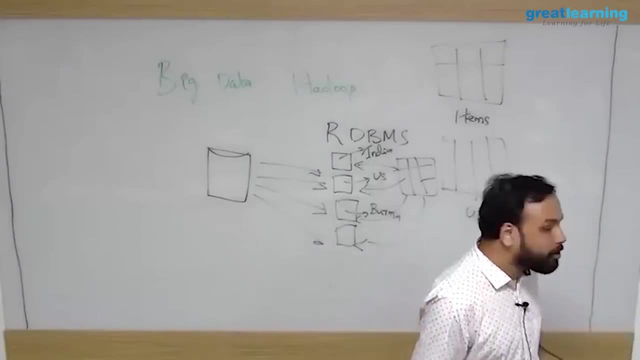 This guy has to wait, So again you're. so the problem is that traditionally, people were using RDBMS systems and data warehouses to store the data. Now what is the drawback? One of the drawback is that as the size of the data increases, your processing will become. 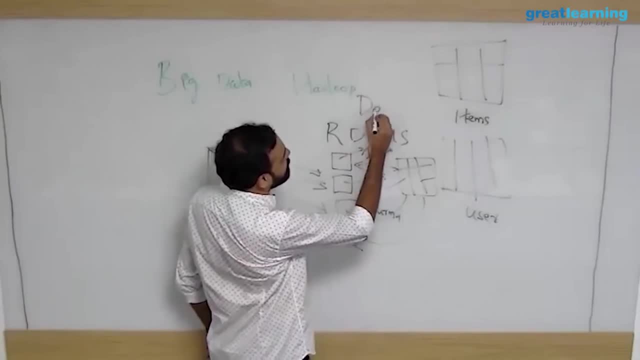 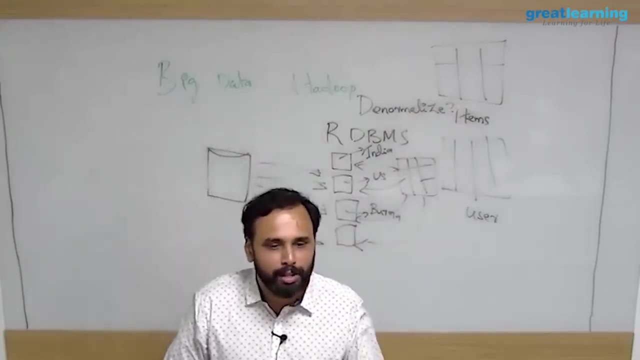 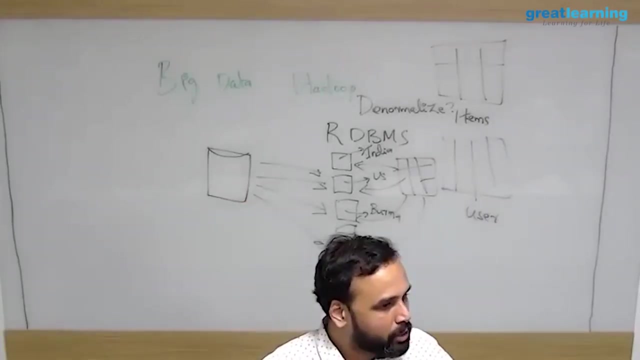 very, very slow. Why don't you denormalize the data? Why don't you denormalize the data? For example, all the transaction data, user data, everything I'll keep in one table. Is that possible? I can't do. 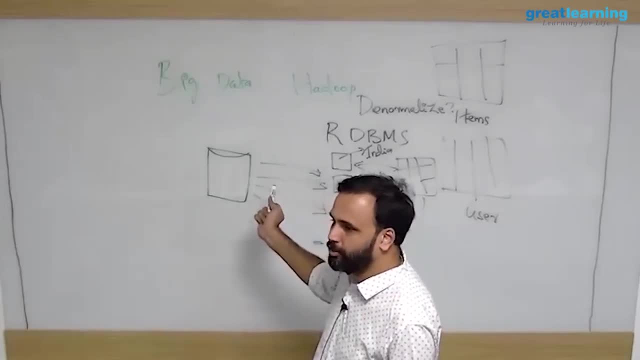 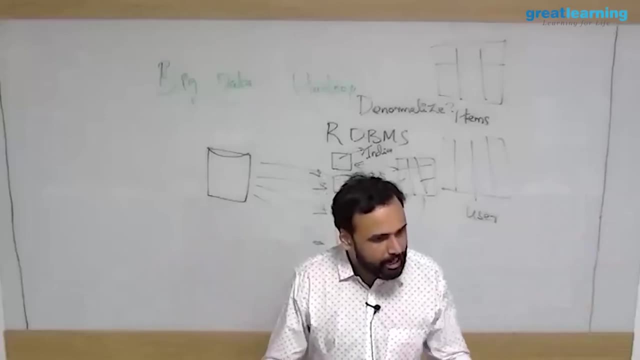 So that is the reason they don't provide the denormalized solutions. If you look at RDBMS systems, they will always say: normalize your data Right So that it will be represented in different, different tables, And whenever you need the answer, you do a join and you get the result. 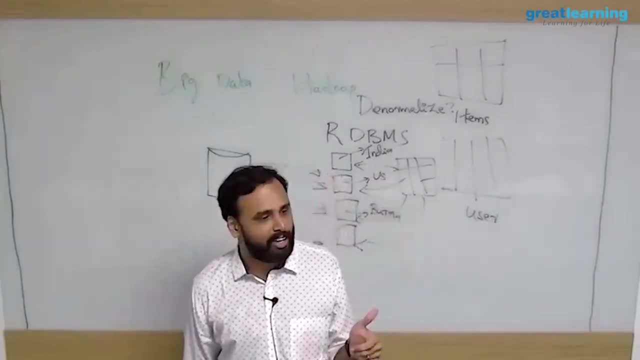 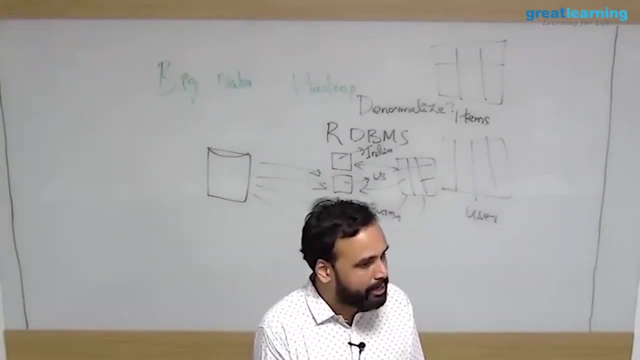 Second drawback: This is only structured data, meaning anything which you can represent in raw column. I can dump here like an Excel sheet data, right? Can I dump images and audio files in this table, Yes or no? Can we store unstructured data in RDBMS? 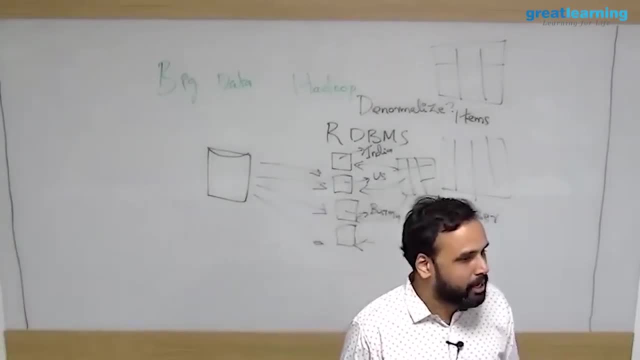 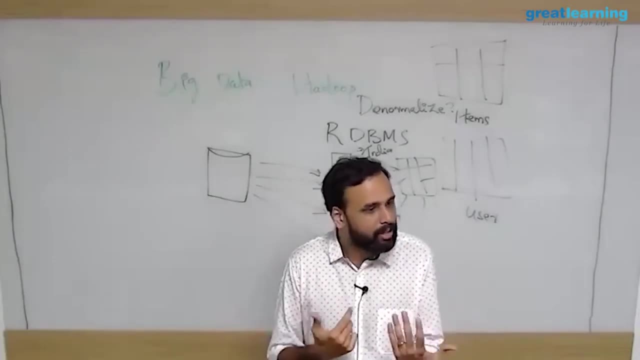 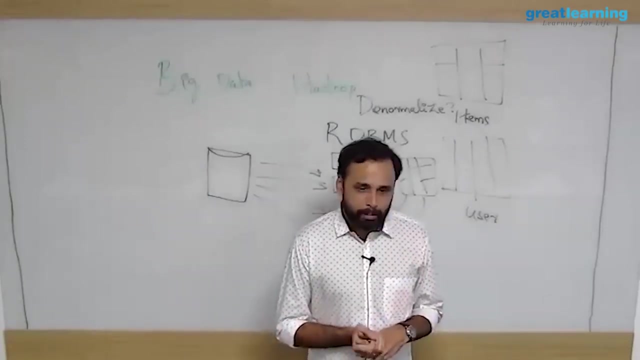 Yes, you can. There is clob, blob and all objects, right. But can it process unstructured data? Not possible. So size of the data increases. It cannot cop up with processing One of the problem right? Second problem is the schema, meaning anything which you can represent in a row, column format. 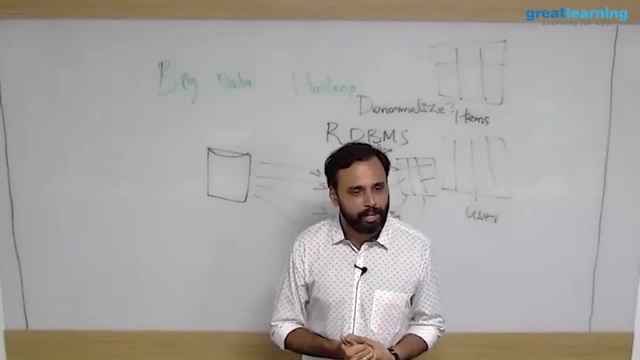 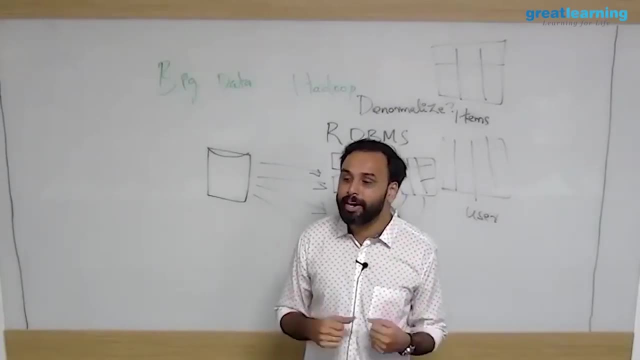 I can dump in an RDBMS Anything apart from that. I have to figure out a solution. So what is the actual solution? if I have to store images and retrieve them in real time, How does Flipkart stores the data? I was working with Flipkart for some time. 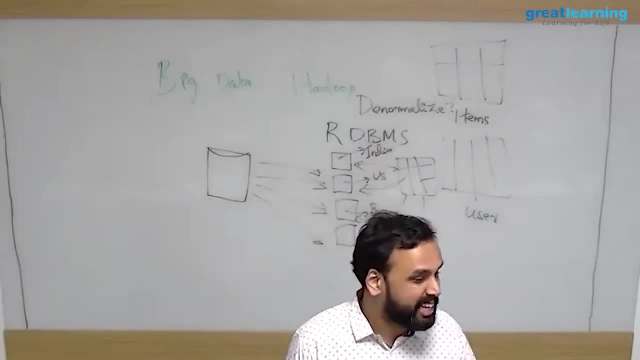 Flipkart has around 10 million products. Each product has 10 images. That is, 1 billion images. So when you click on an iPhone X picture on Flipkart, Flipkart will say that come after 10 minutes or immediately display. Have you ever thought how it is happening? 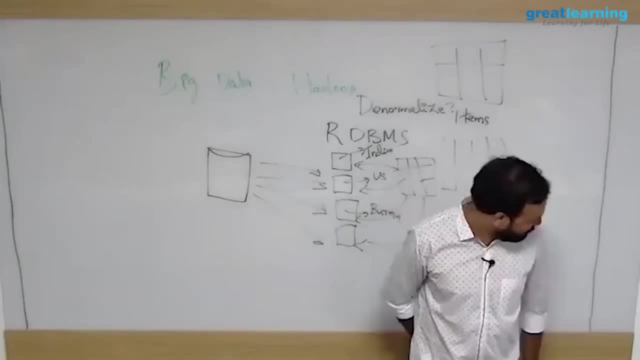 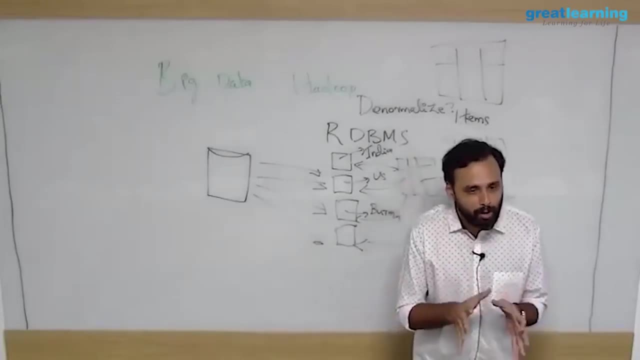 How it is happening, right? So do you think they are dumping in an RDBMS and picking it from there? 1 billion images. There is a whole arena of databases called NoSQL. If you have heard about MongoDB, Cassandra, Hspace, Neo4j, Voldemort, these are all popular vendors. 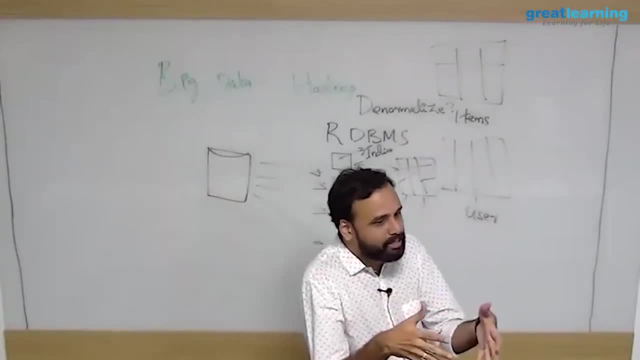 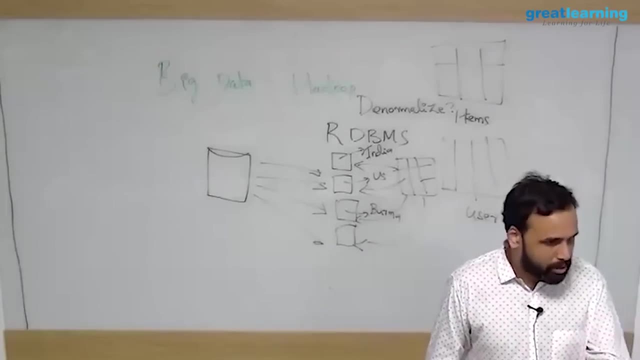 So what is NoSQL? It is a database of NoSQL databases. So NoSQL databases will help you to store and retrieve unstructured data at any speed you want. So what Amazon- Amazoncom- actually does? Amazon has something called DynamoDB. 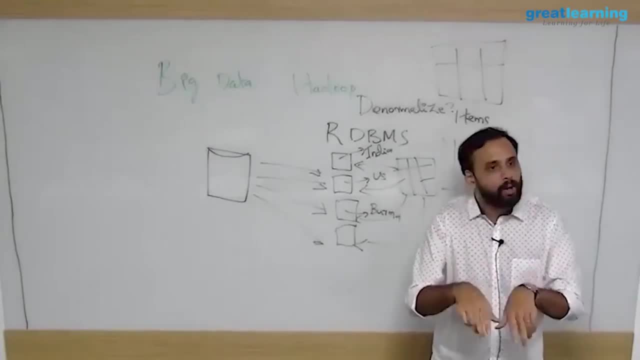 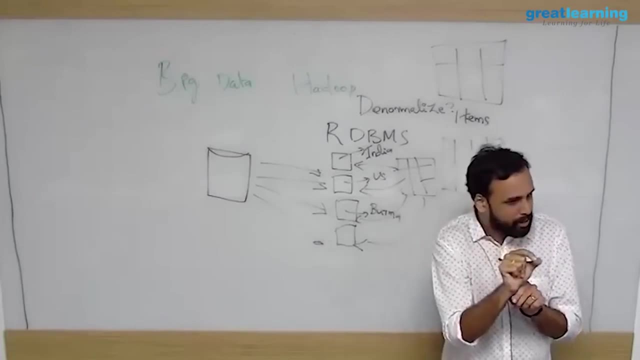 DynamoDB is a NoSQL database, So in DynamoDB I don't have a row column, I have key value pairs. So what they do, the key will be the product name. Say, you are clicking on iPhone X, iPhone X is the key. 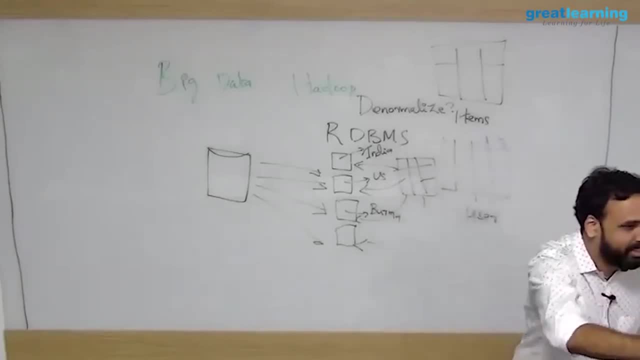 The value will be all the data you have. So the moment you click Boom, your page is there. So NoSQL databases are really faster. Also, it helps you to store unstructured data. How are you booking a cab using Ola? 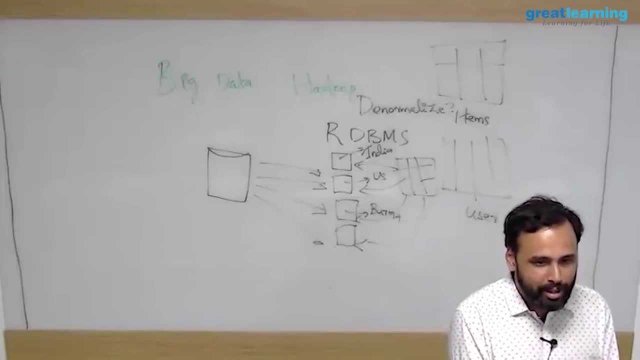 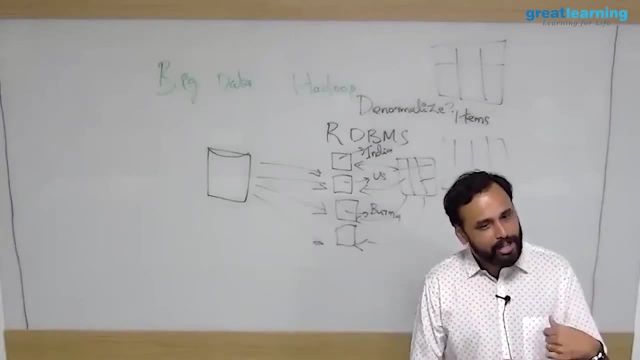 If I try to get a cab using Ola, I open up Ola. How many customers Ola has? Millions in India And all of them are booking at the same time, right? Do you think all your requests are taken by an RDBMS and searched in the table and give? 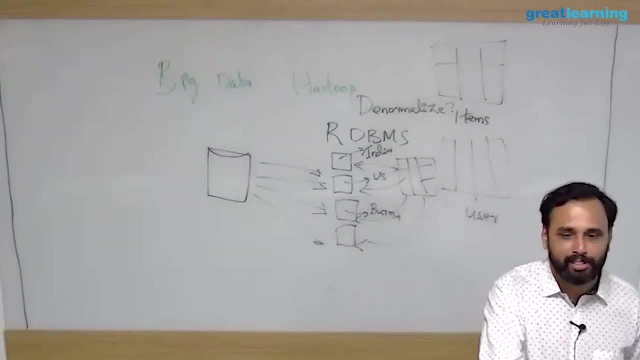 you a cab? Does it work? Can an RDBMS system handle 30 million- 40 million? No, It can handle 30 million- 40 million concurrent sessions on this amount of data calculating route. MongoDB NoSQL database. 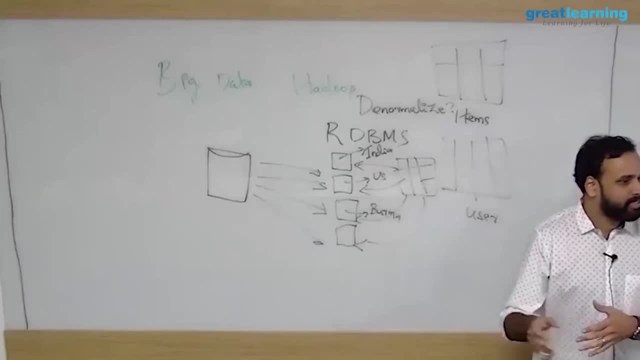 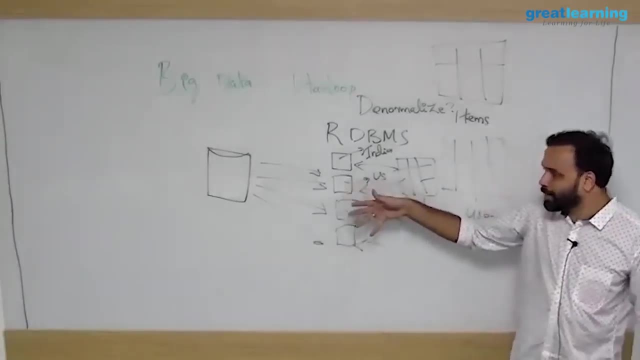 Ola runs on MongoDB. I was working with Ola for one of their design problems, actually, So I didn't design anything, but they told me that they are using MongoDB. So the second drawback of your RDBMS is scalability. is there? 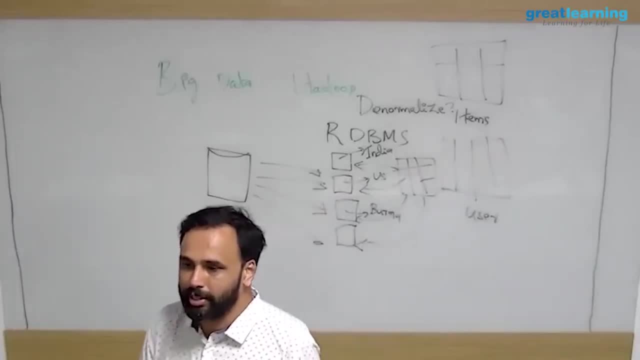 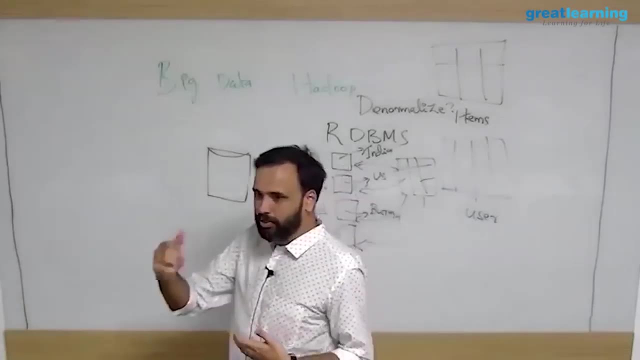 Third is price. Price is a problem, right? I mean, obviously, if you calculate the cost, if you look at Oracle and all they are very, very costly. Solutionри storing the data or an RDBMS, and retrieving is not good for the modern day. 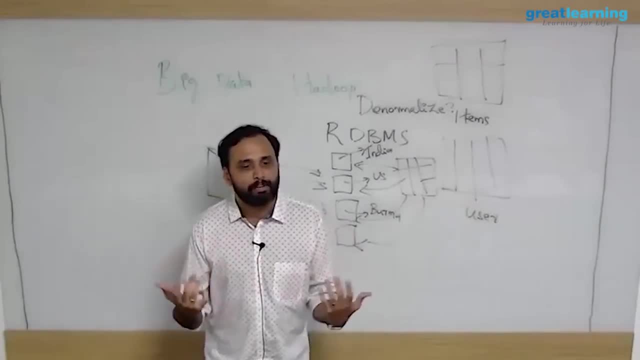 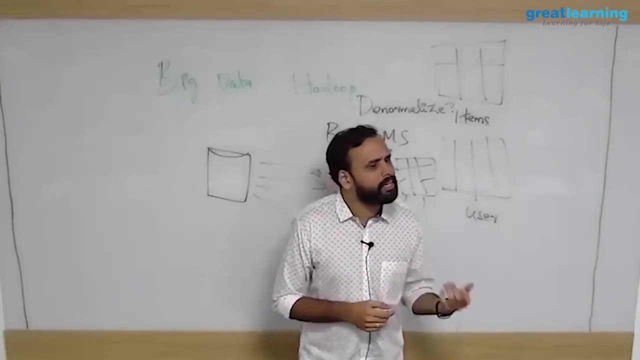 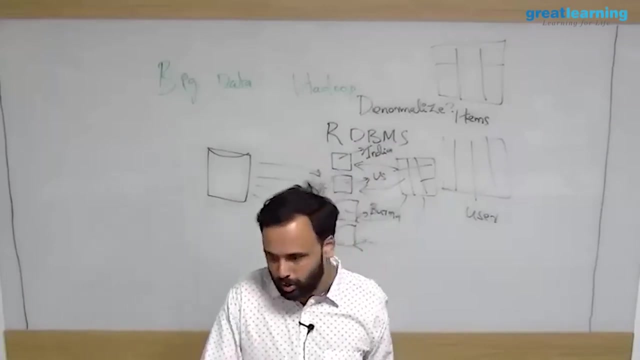 In the modern day, what is happening is that every company want to collect and analyze the data, Be it banking industry, e-commerce industry or any industry that you want. they want to collect and analyze the data. So, to give you an example, if you visit Amazoncom or a Flipkartcom, what is happening? 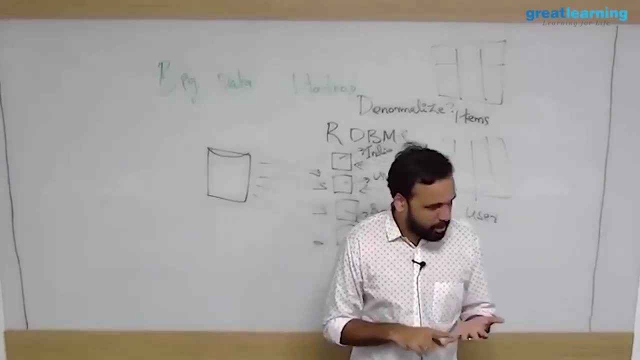 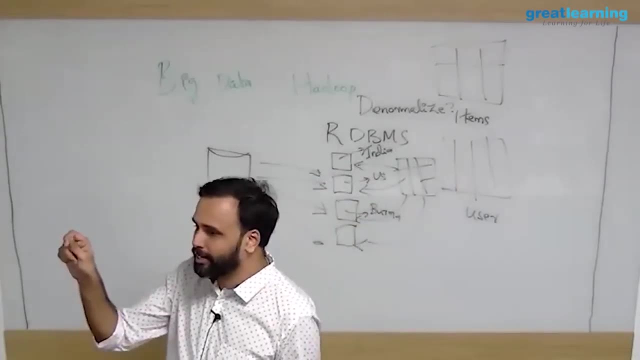 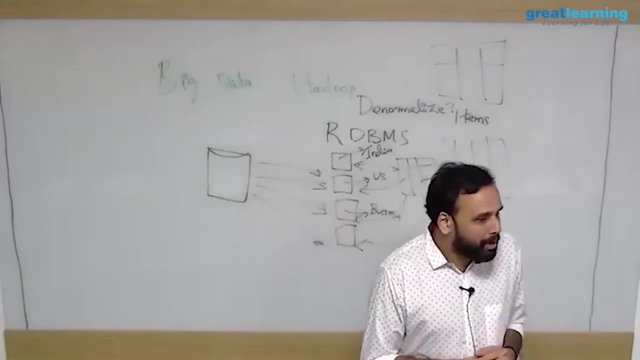 They start tracking from automation. Things are changing: which ip address you are visiting the website, how long you are clicking on a page, which items you are adding to cart, which images you are clicking, which offers you are clicking. all this data is analyzed to understand how a customer will behave. that is how they do marketing right, so the more 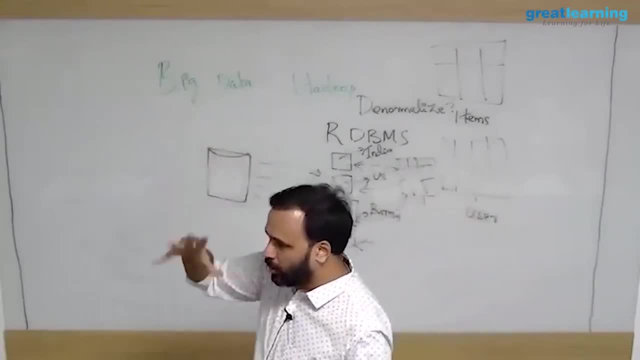 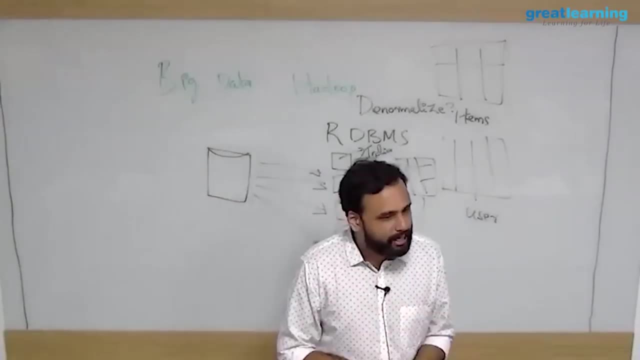 you start visiting the e-commerce companies, you start seeing recommendations and all the more, the more you visit amazon, they will start recommending products to you, asking you to buy. so they have to collect all this data. so when i was working with flipkart, flipkart said that. 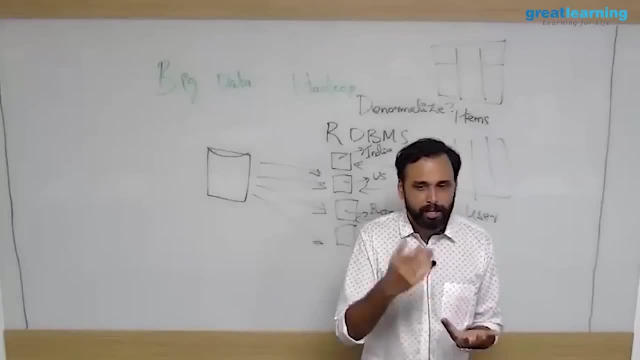 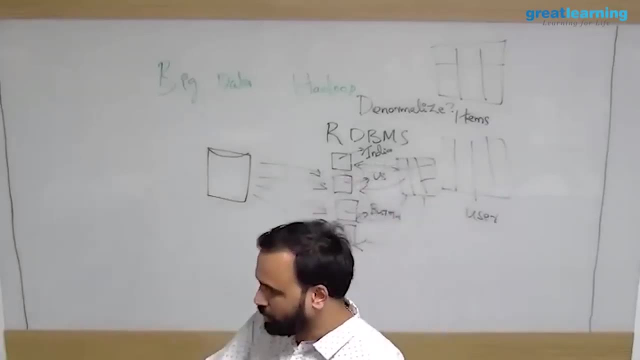 they collect data from the apps that you are using, from the website that you are having, even from social media. flipkart is very active in social media like facebook, twitter, all these places they are active. so if anybody tweets about flipkart or visit their facebook page, all this data is. 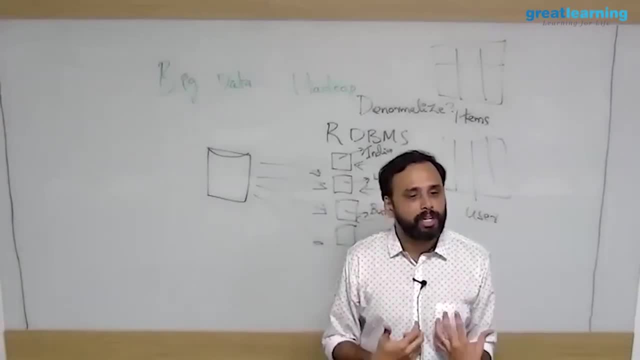 being collected now. this, though, so this is actually called a big data. so the technical definition of big data is: you know, like you know your baking, where are you eating breakfasts, etc. etc. you know like you add flavors based stuff, like you are adding onions or something, and, being uh uh left say: according to you, do something like that, Aqualito, lick it off, do some shale, and that is possible. 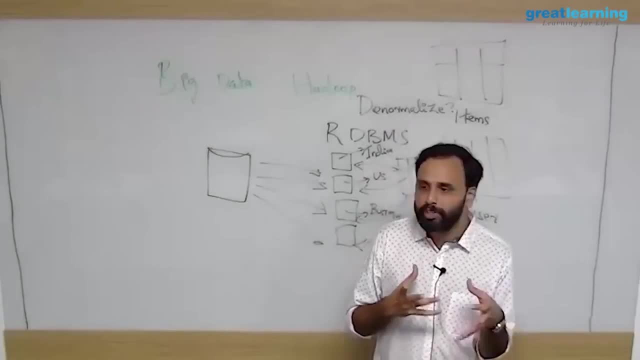 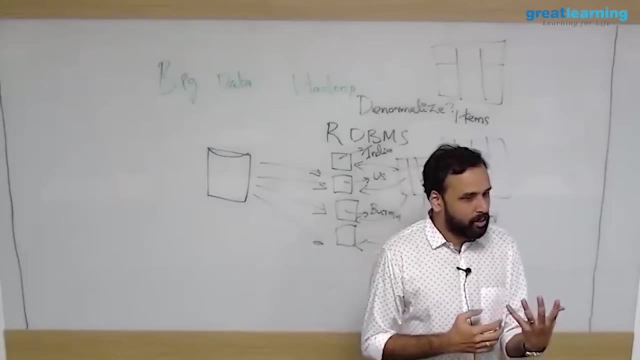 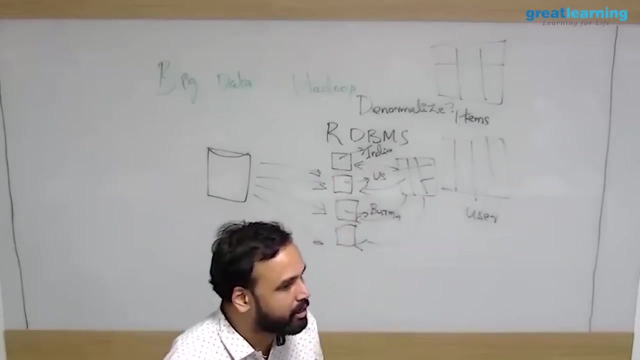 is this huge amount of data which you cannot process using your traditional methods. that is called big data, right? so why that is of interest to us. we are going to figure out how to store this data- huge amount of data, right- and how to process this data. when I say no sequel databases are there, it does not. 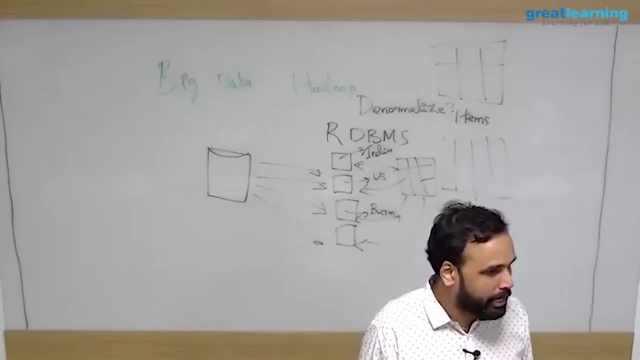 mean your RDBMS is gone. so many people ask this question. okay, RDBMS is the only solution for transaction management. so, even if you're buying something from Flipkart, who will complete your transaction? or AQIL, probably, or any transactional system for transactional management? and why is that? because 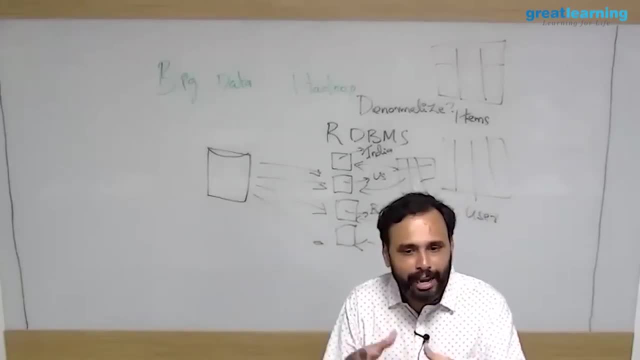 RDBMS systems are the only ones which can ensure the ACID properties right, if a transaction goes or not goes. you bought something from Flipkart. tomorrow Flipkart cannot come back to it and say that I don't really think. I don't know whether the transaction happened or not. probably you've got the 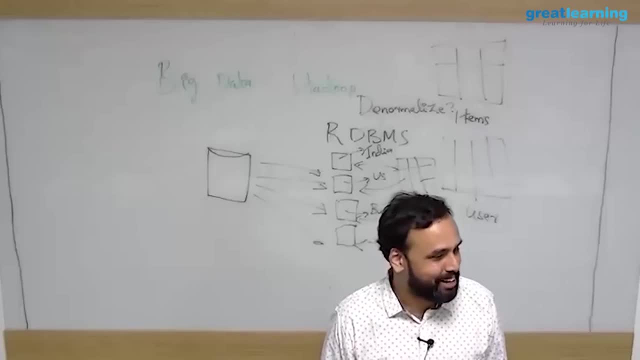 management or not. it is up to you to decide that this is what we want. now we are going to read this question. Thanks for watching. It's not possible, right? Then you will start complaining again, Flipkart, right? So Flipkart comes to you and say that you know what? 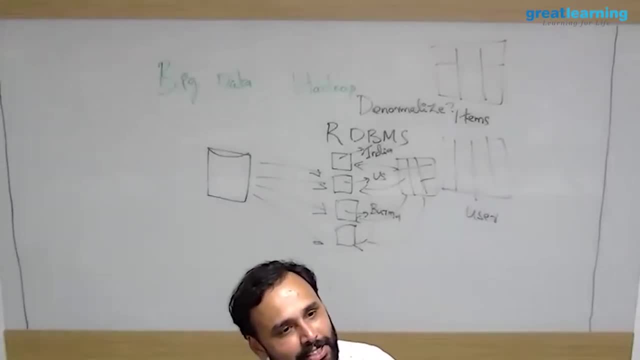 We are using Cassandra. As per Cassandra, your transaction is we don't know. We'll come back in another one week. Is that possible? No, So, transaction management- very good question- is still handled by RDBM Polyglot persistence. 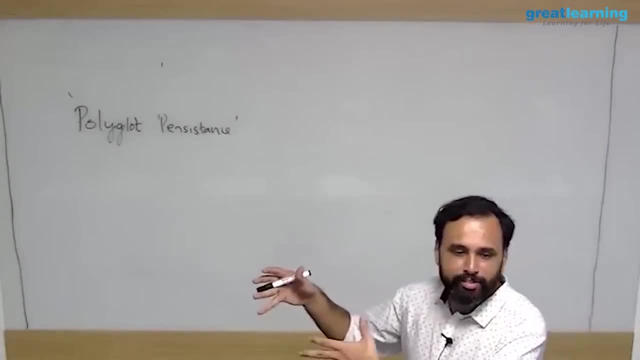 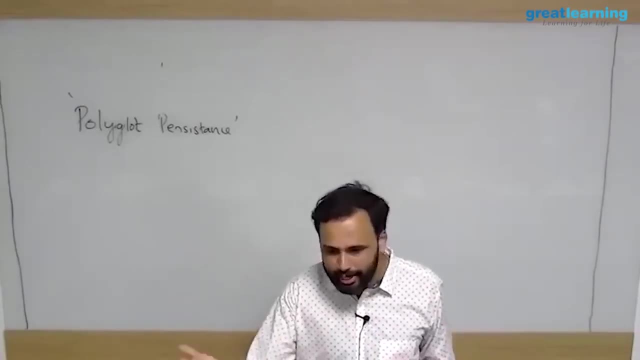 In the world of big data, there is a separate category of systems called NoSQL databases, And they are databases. So what is a database? It is real-time queries, right, And in that area we have MongoDB, Cassandra, Hspace. 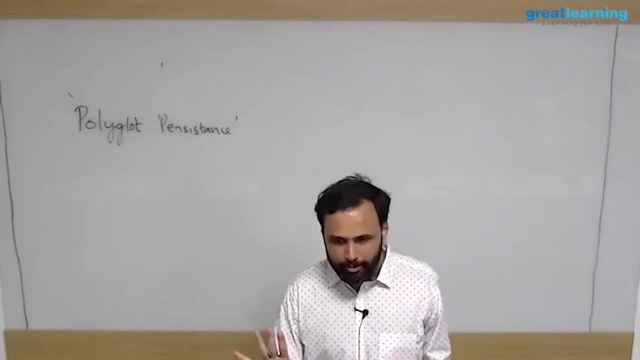 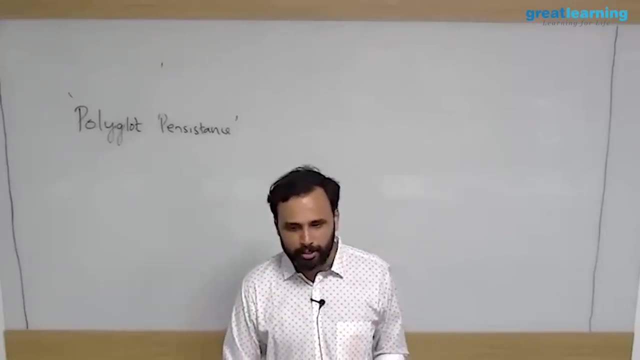 and these guys. Now, these guys are used in real-time. if you want to fetch the data, Say, for example, you are opening an e-commerce website, Probably it is given by a NoSQL database, right? Or millions of people are booking flights. 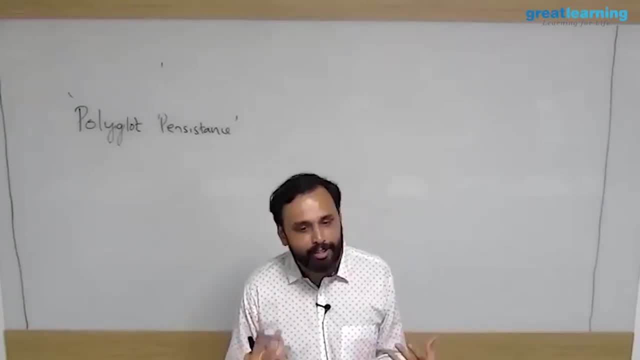 through cleartripcom And cleartrip has to identify how many people are booking in a particular route so that you can give a better offer. This is probably done by reading real-time data from a NoSQL system. Our area is not NoSQL. 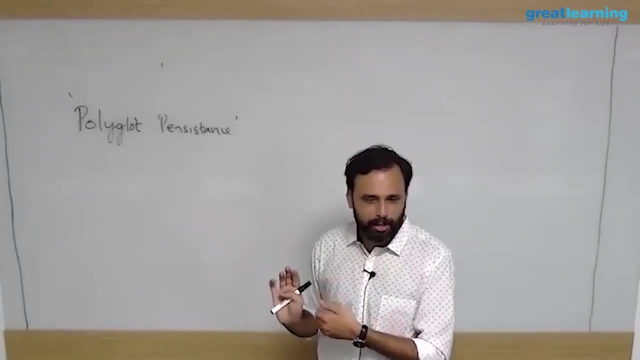 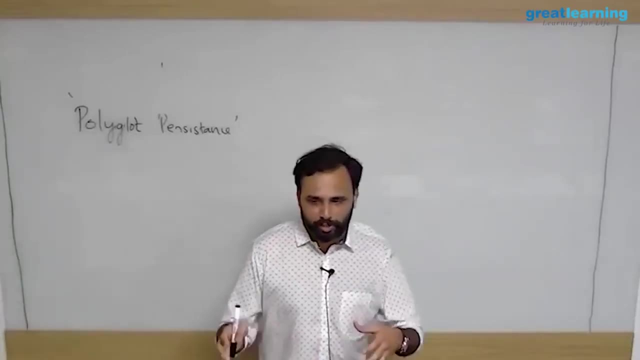 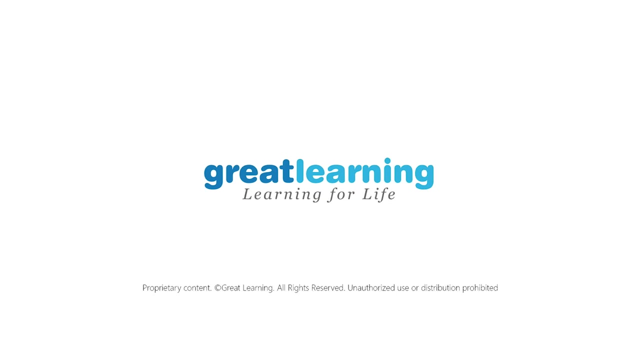 NoSQL is a DB. actually It's a database. Our area is not NoSQL. We will come to Hadoop right Now. so this is the technical term for coexistence of DBs and NoSQL and all Now. there is a very important term. 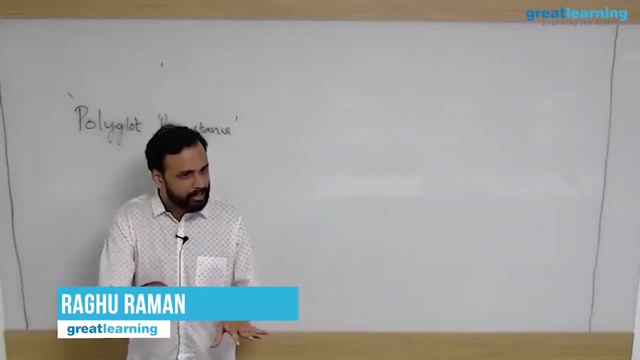 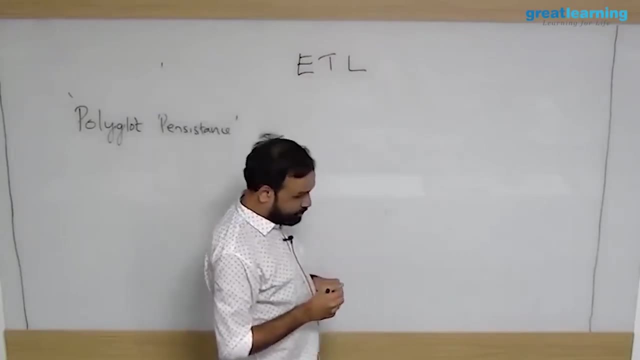 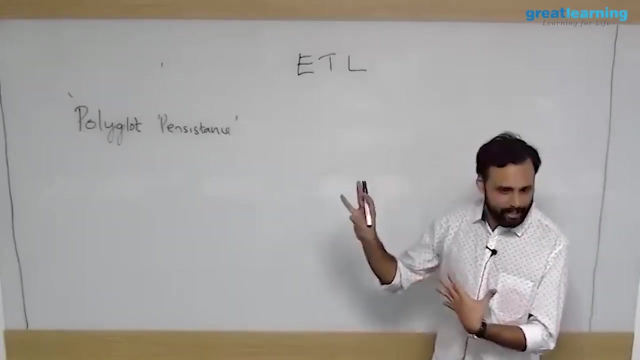 even though it is not directly related to your syllabus, but I think it makes a lot of sense. How many of you are aware of this term? So ETL stands for extract, transform and load. So what is the idea here? is that see? 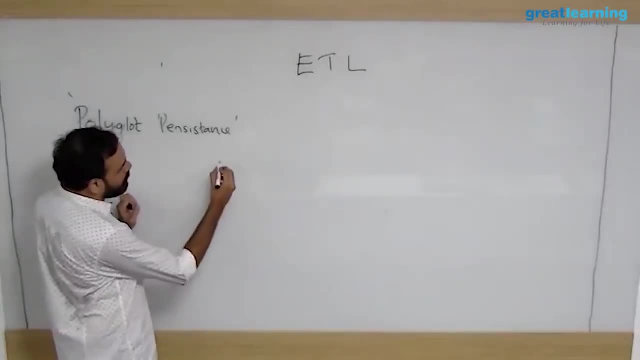 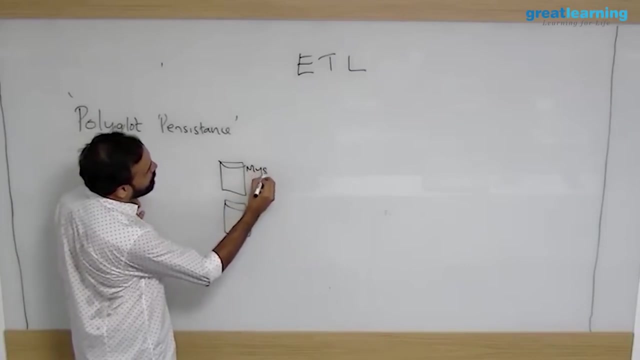 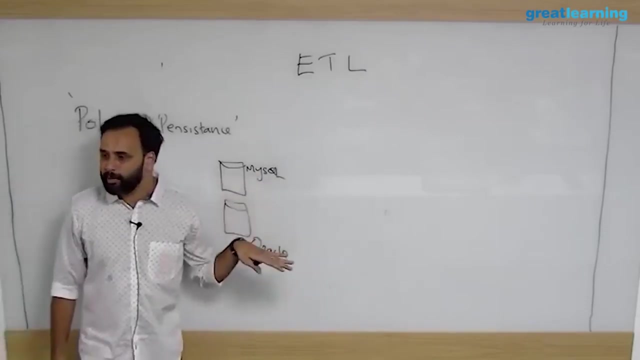 if I'm working with a company right, the company will have RDBMS systems right. So these are all RDBMS systems. So probably this guy is using MySQL and he's also using Oracle right. A lot of RDBMS systems are being used by a company right. 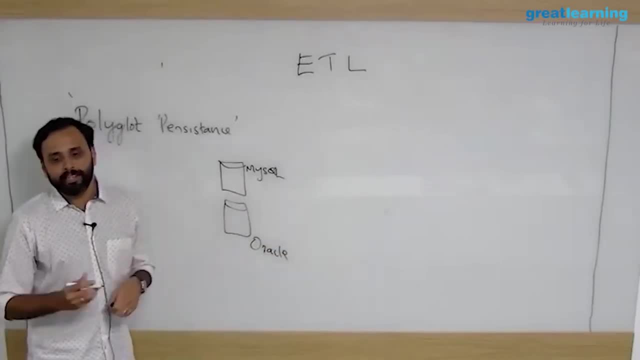 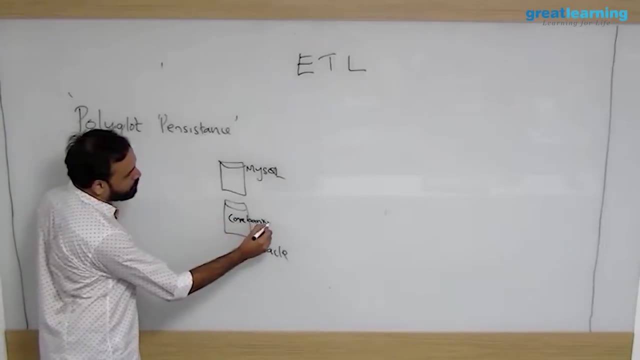 Now, these are all serving the customers. So if you take the example of ICICI Bank, all their core banking data is in Oracle. All their core banking data is in Oracle. So if you are making an online transaction, the data it's Oracle. 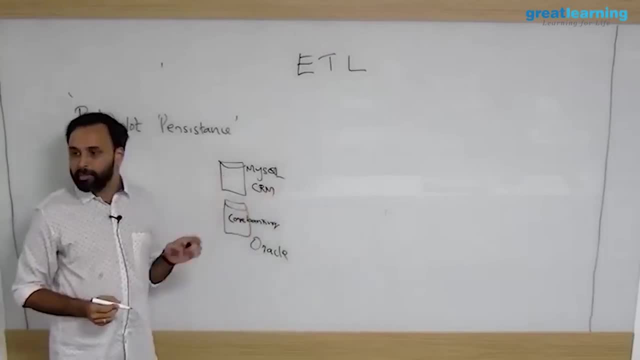 All their CRM data is in MySQL. What do you mean by CRM, Customer relationship, right, Your name, address, blah, blah, blah. So they have these two types of data. Now is this the only type of data that they have? 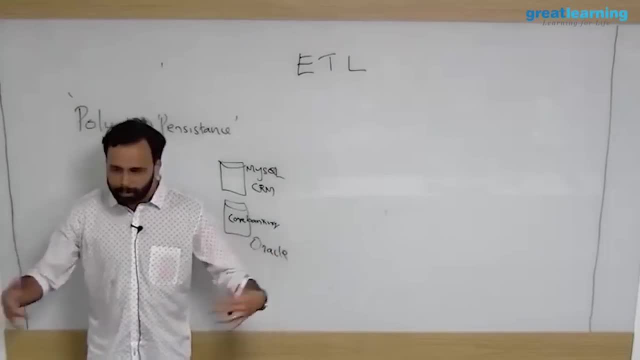 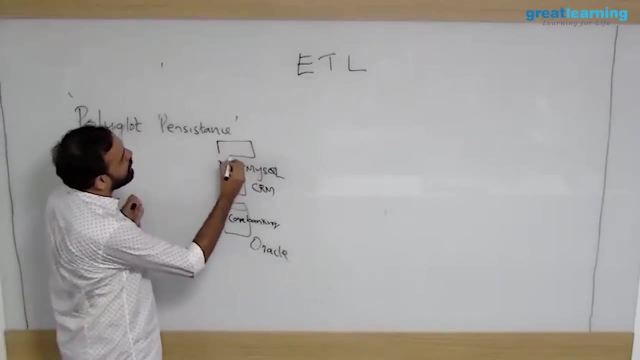 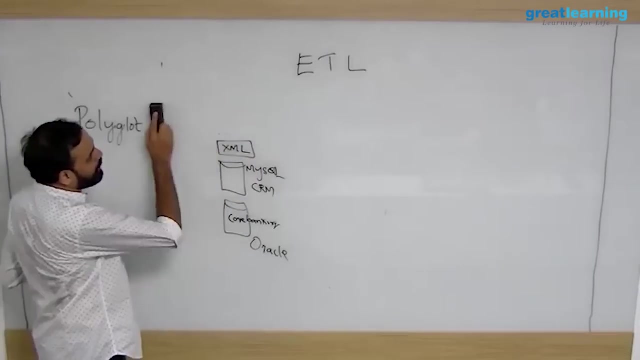 No, ICICI Bank had also acquired a lot of other companies when we were working with them, So their subsidiary companies were giving them data in the form of XML files- XML right Now. ICICI Bank also had a Facebook page, from where they were getting around 10,000 people visiting. 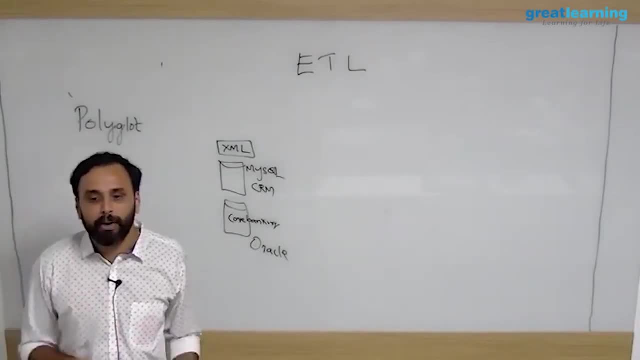 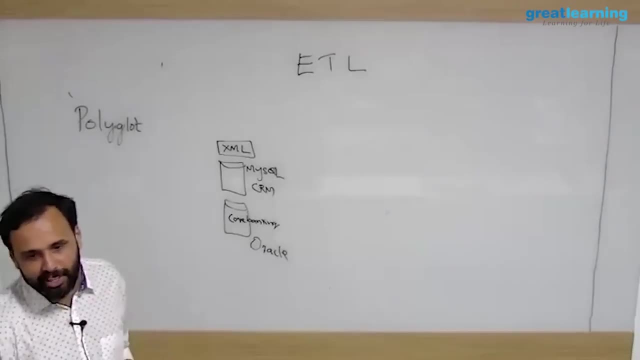 every day that Facebook page And they used to click on some item. So they have to do this cross-selling up-selling. If a user goes to Facebook page and say that I really like your lawn, take more lawn right. 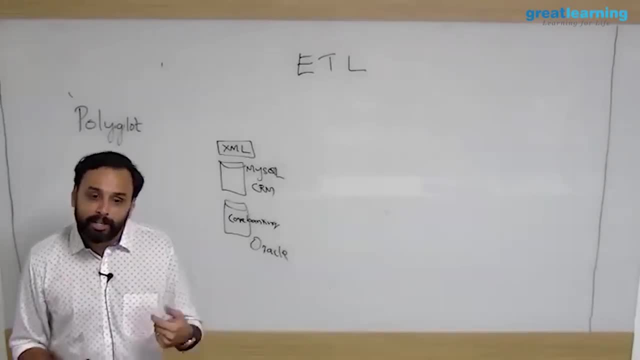 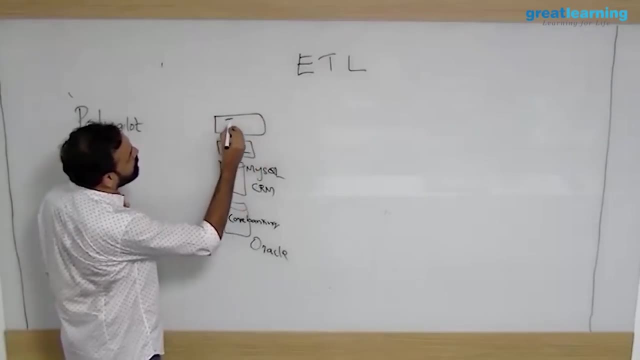 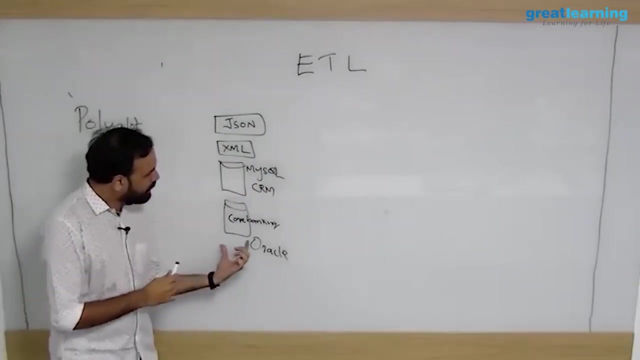 So that is your cross-selling and up-selling right. So what they do? they collect all this data from social media That comes in the format of what? JSON JavaScript Object Notation, JSON key value pairs, basically. So this is where their core banking data. 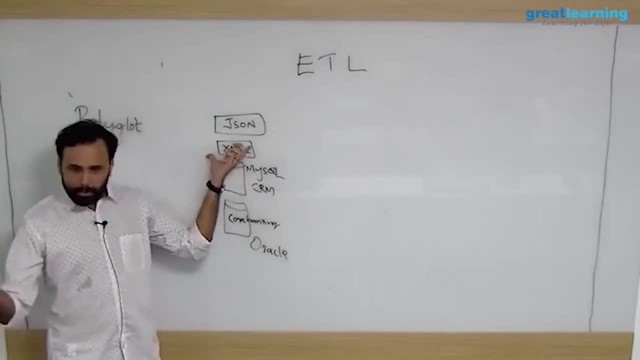 this is where their CRM data, this is from their partner companies. this is from the social media data they are getting This one, the social media data, they want to do analytics. So every day, 10,000 people are visiting their web page. 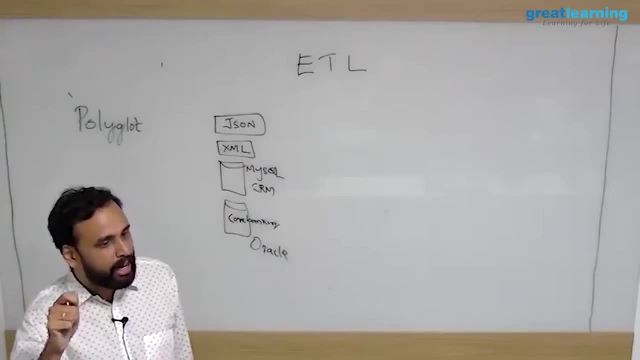 They want to know a person clicked on, let's say, a lawn offer, and how much time he stayed on the page and what age group he belongs to, so that they can recommend products, recommendations, actually A lot of recommendations. So social media data was being used. 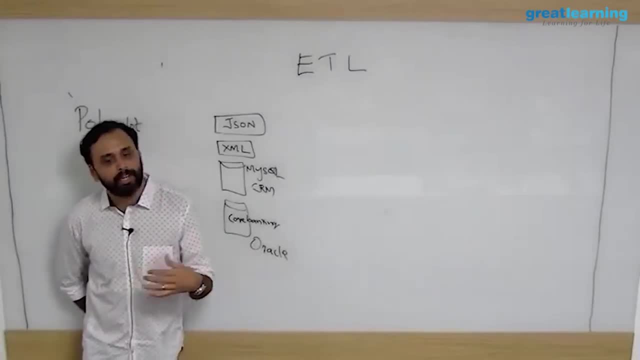 They did not reveal all the things that they are doing because that were internal, But basically, using the social media data, they were doing recommendations. So they will download all this data. So if a customer is clicking on the Facebook page, they will get the access of this guy. 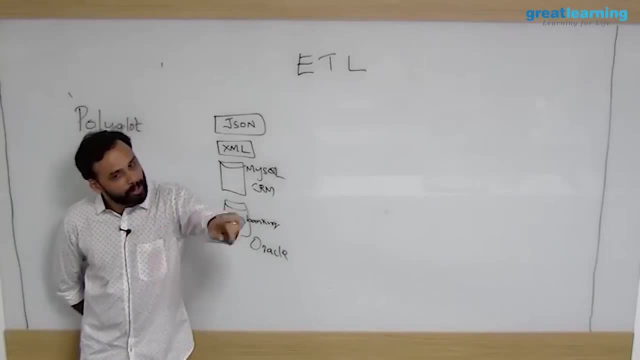 If you are clicking on ICICI Bank's Facebook page, they will know your age, your occupation, everything you shared in Facebook That is by default given to them. In most of the cases You can restrict the information, But most of the public customers- they will share this. 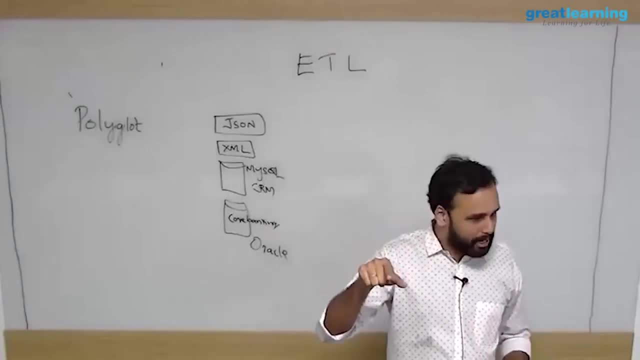 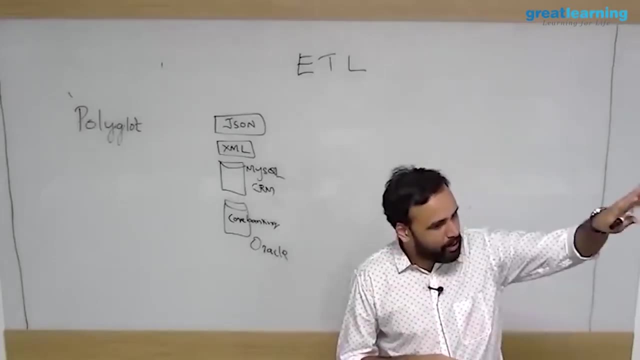 So by downloading this data today, they will understand. 10,000 people clicked And out of them, 5,000 were youngsters And they clicked on this lawn. That means the trend is towards a particular bike lawn. If we give an offer on a bike lawn, 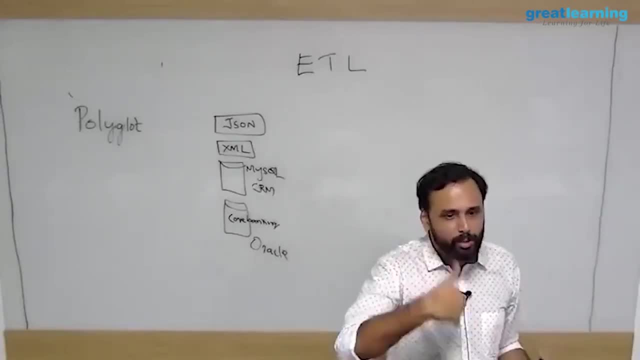 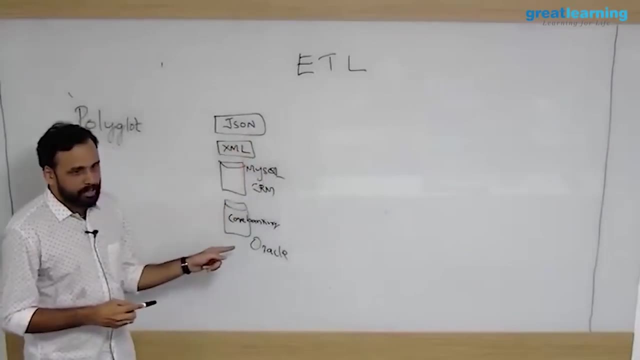 youngsters may actually buy it. So this is analytics, right. So all the social media data they can use in multiple ways actually. So this was getting in the JSON format actually, And this type of data was there. They also were collecting their customer care log files. 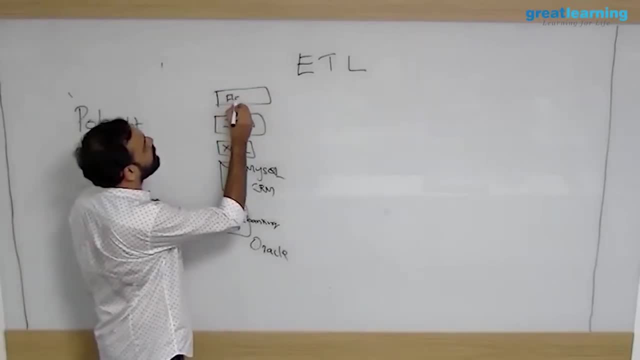 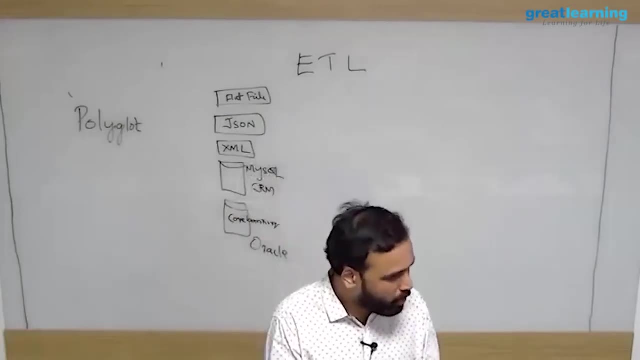 So that is again flat file. It was coming in a format of flat file. Flat file means text file, So customer care log actually means the chat logs that they were having, also the call logs. They don't get the actual call, but how long the call happened. 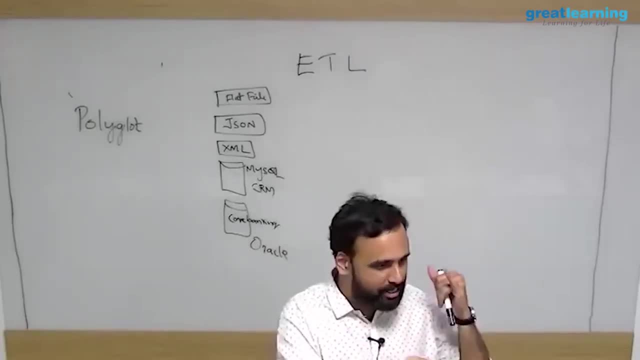 and what you pressed. So when you call customer care, you press right, This, this, this, That is actually captured. And then they want to figure out how many people called on what category, how much time they spent right. 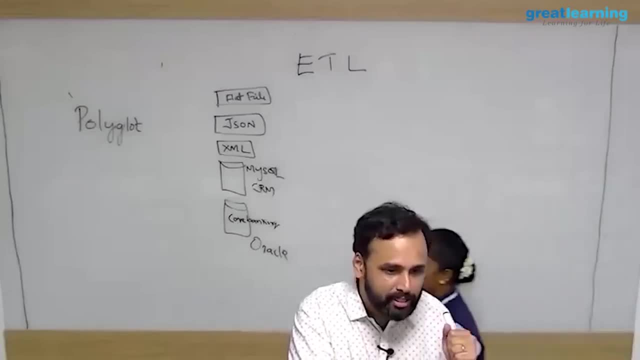 So if you have clicked on a Complaint button and you talk for one hour, chances are very high you are a bad customer, right? I mean one hour. you're scolding, probably right, So they want to figure it out, right. 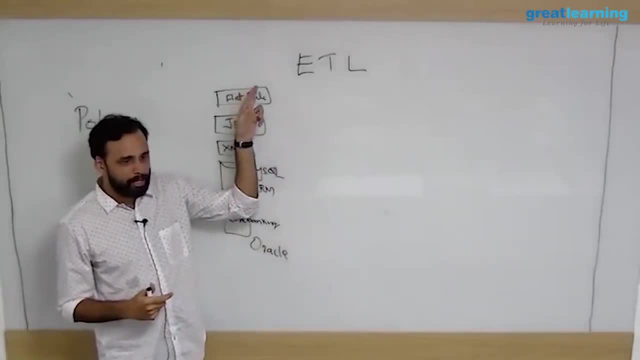 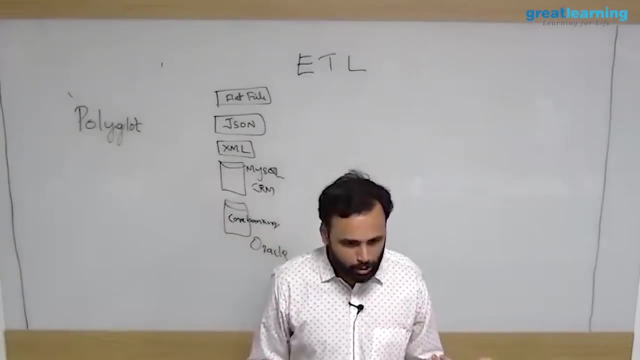 So that is the call record that was coming in flat file, this format right, And at that point in time ICICI Bank also wanted to offer a solution. So previously what they used to do- their agents- were there, people who 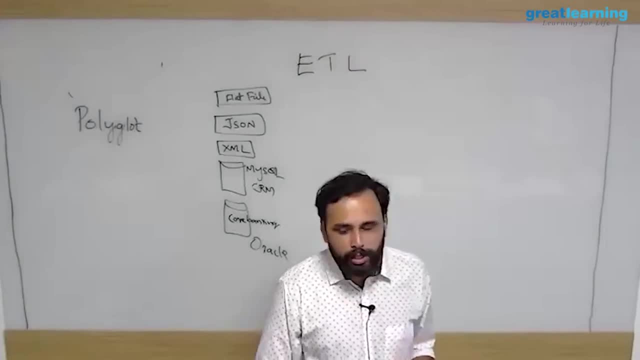 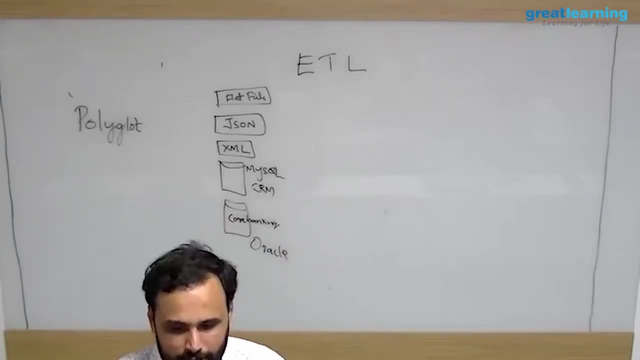 Go to your house and make you buy lawn and all. So they used to go to every place. So this agent will get a list and he will go to that place And he will go to your house and say that sir, please take a car loan. 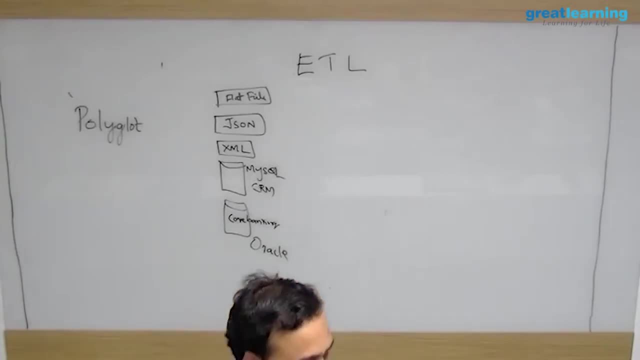 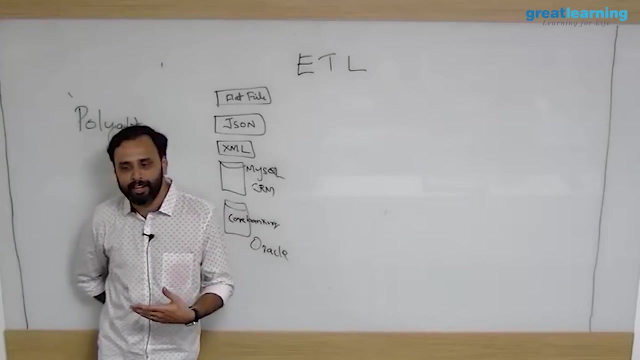 He will say no, he will say bye, He will get money, He is getting salary right. So this technique was not working, Because if I get a list, okay, One customer will be in, one guy will be in OMR. 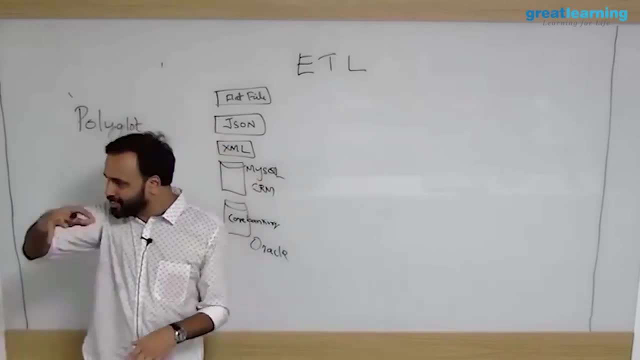 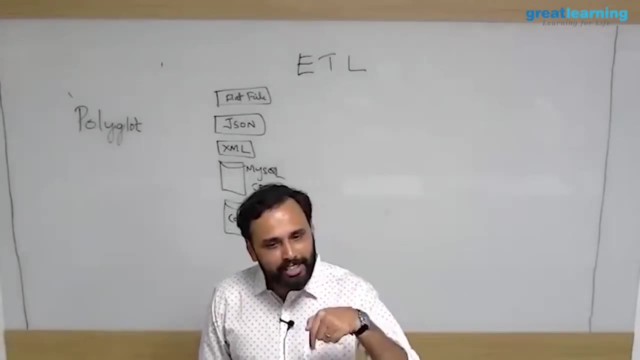 another guy will be in some other remote place in Chennai. So by the time he travels from here to there, from here to that place, day will be over. So he is able to cover only two customers. So what ICICI Bank had in mind? they will track his location. 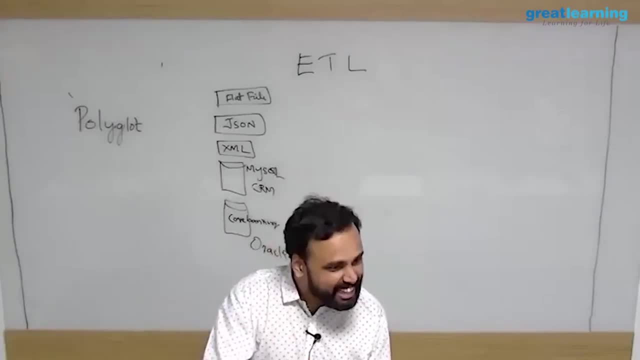 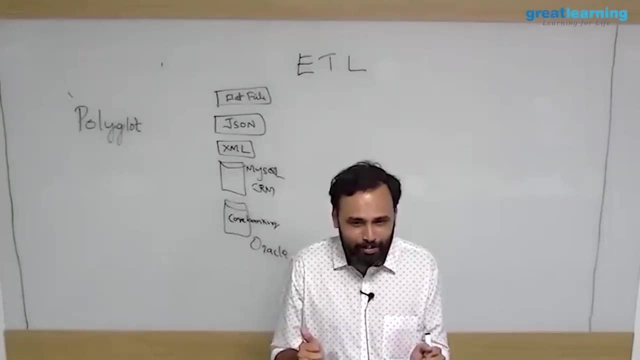 He has a device, okay, And give him customers in real time. So if he's in Kannan-Javadi he'll get all the customers nearby him. So this guy has to go right. He cannot say I can't go. 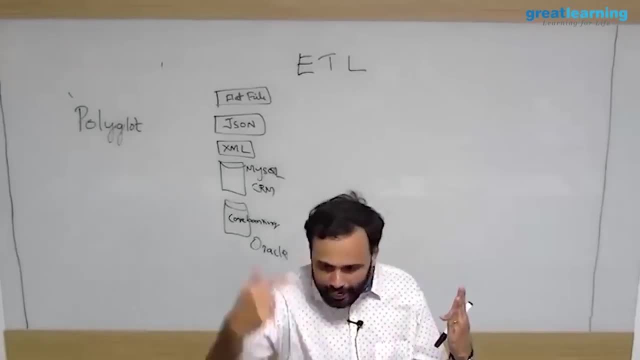 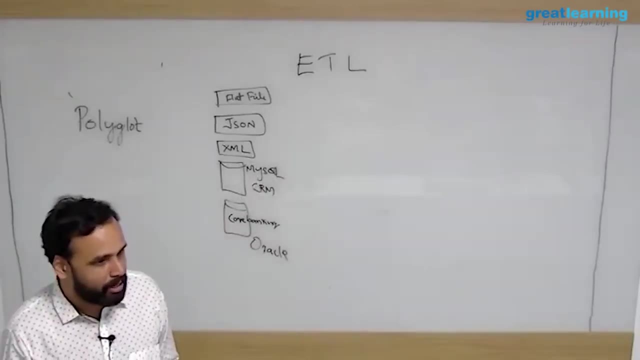 So he will. the customer application- it was a tablet- will track this guy And wherever this guy goes, the nearby customers will be provided to him So he can cover more customers right, And this has a lot of impact Because why it was practical. 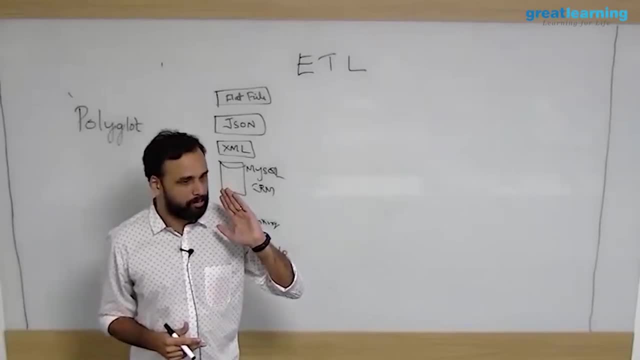 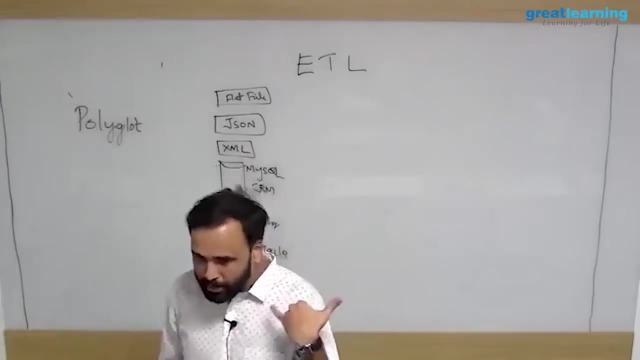 Because sometimes the customers will call and say that please come, I'll give you a loan. So what you do From here, you might travel to Paris, right, And because the customer called right, So you go to Paris and meet the customer. 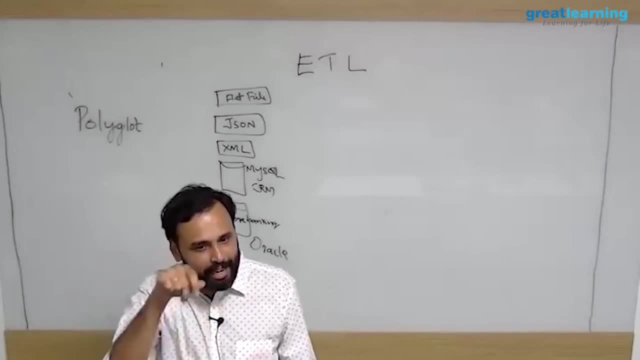 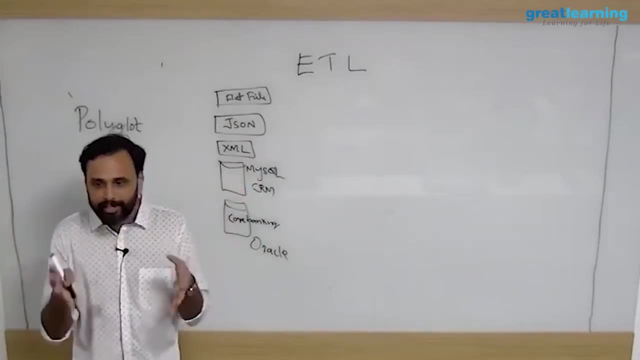 Now you don't know how many customers are around Paris That this application will track and send it to you. So these guys were collecting that data also from all the tabs, And that was. There was quite some big amount of data they were collecting. 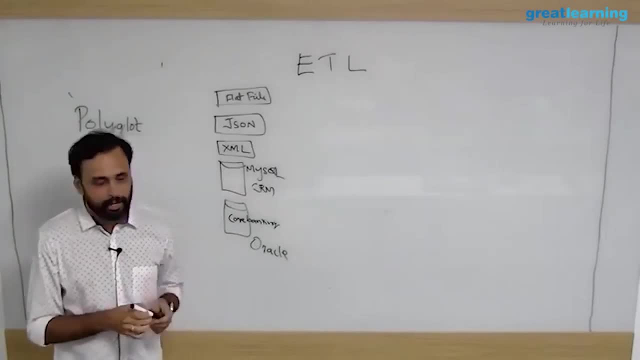 So how many customers they met and whether they closed it or not closed. OK, That was coming in, I think, some other format, So some format I write. I forgot actually how it was coming. So this is the whole data. they have right. 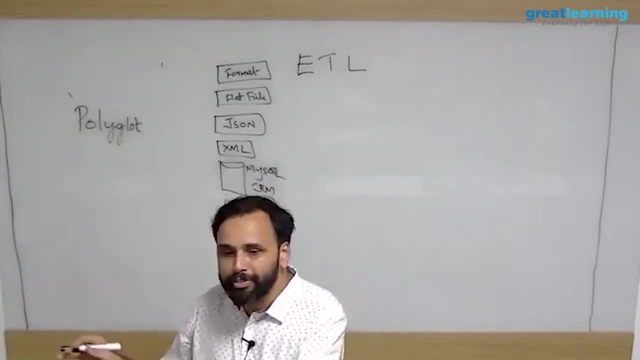 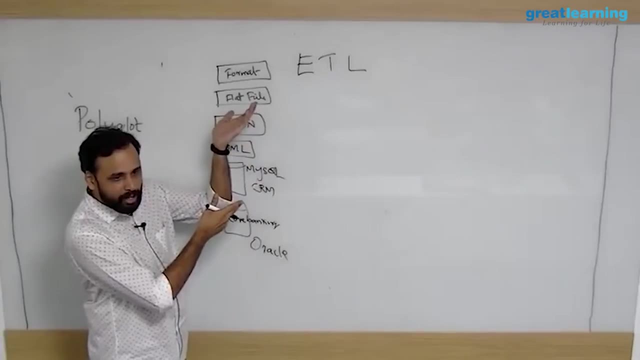 And some more data was there, And this data is lying on different, different systems. It's not in one place. The core banking data is in Oracle. Some other data is in some other place, right, And if you want to analyze this data, right. 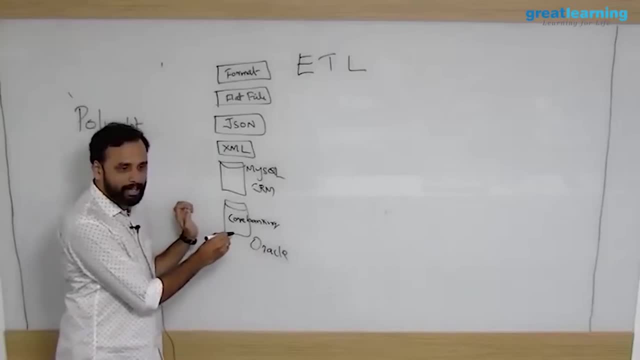 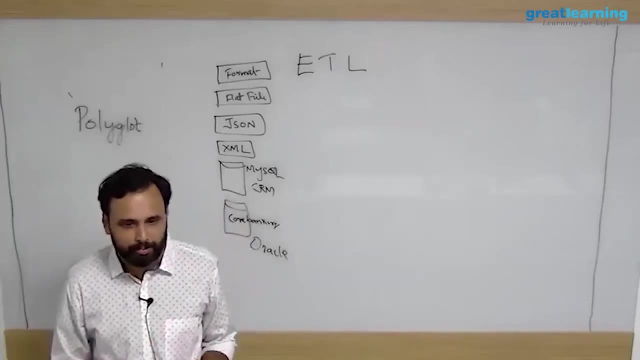 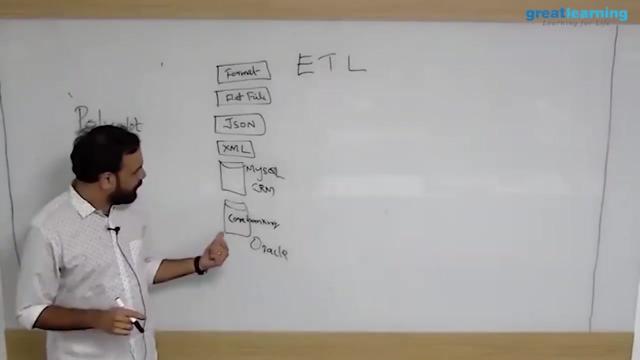 If you want to analyze this data. one thing is that I cannot go to Oracle and say that I want to analyze your data. Why? Because this Oracle DB is already busy serving customers. Correct, This Oracle DB is the core banking database. So if you are making a transaction, 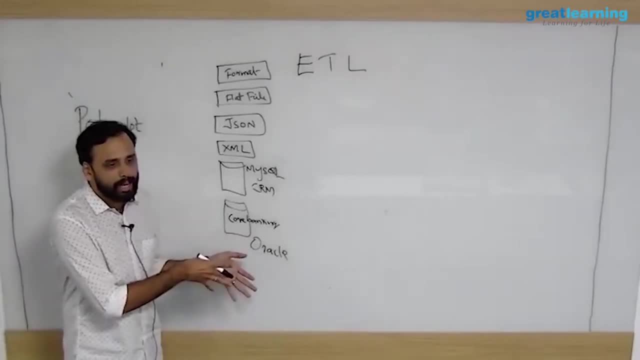 Oracle is handling that right. So I cannot go to Oracle and say that let me run some analytics on your data. Doesn't work that way, Because then Oracle will slow down. I can't do that, So I have to take on the data. 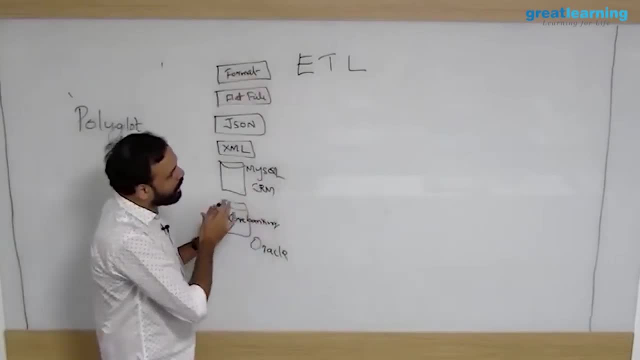 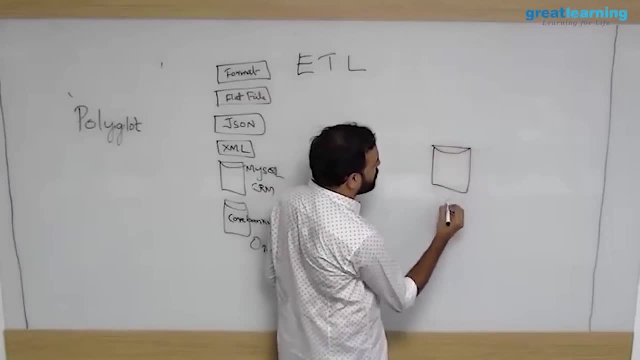 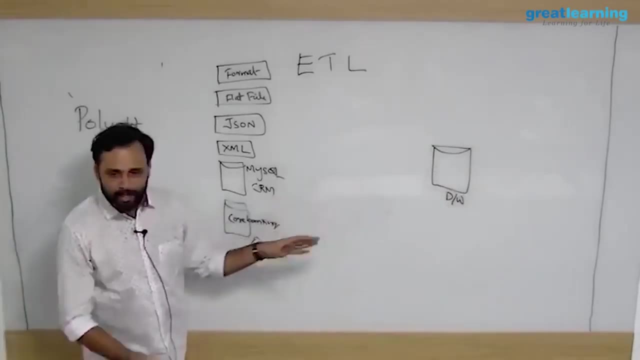 So that is what is you call as your data warehouse, right, That is called a. how many of you know what is a data warehouse? So a data warehouse is nothing but a database. only in one way: It understands the language of SQL. 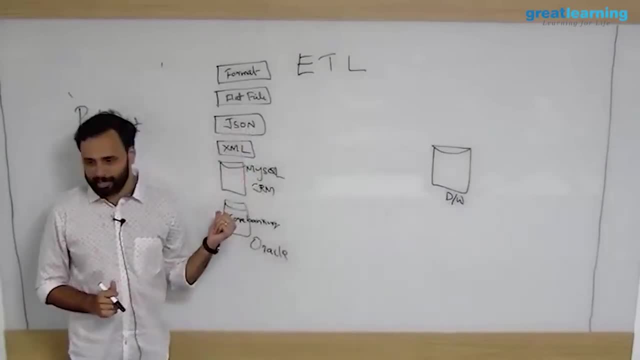 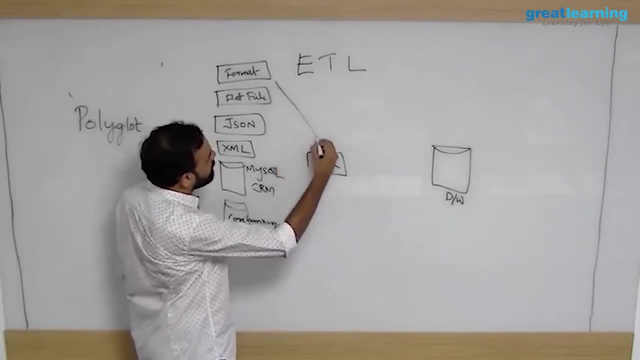 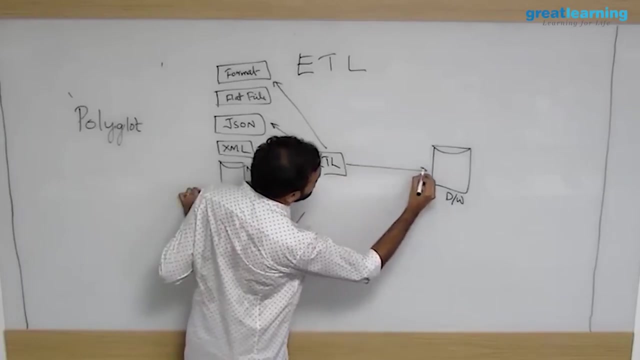 But the major difference is that it is not facing the customer, So you will do something called ETL. OK, So there are ETL tools. So there are ETL tools Which can get the data from all these places, right, And this guy will dump it into a data warehouse, right? 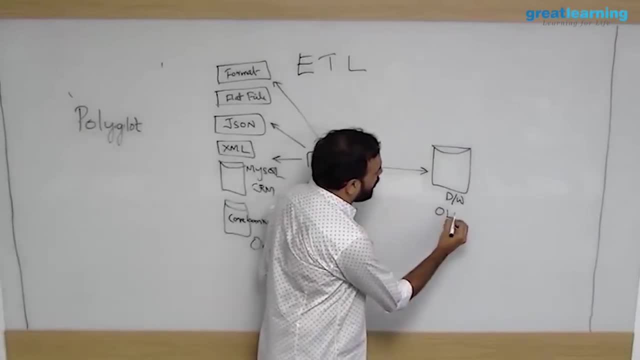 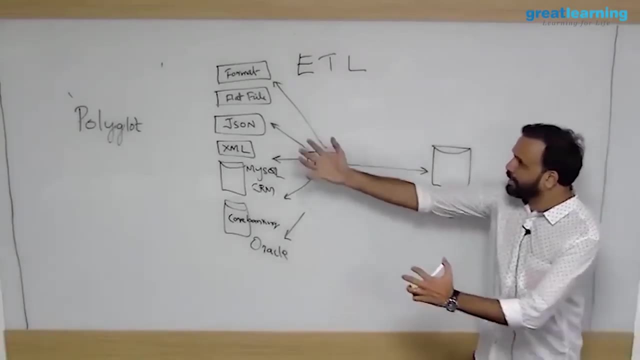 So data warehouse is also called as your OLAP, online analytical platform, so on and so forth. And what is the purpose of this guy? So this guy will have all the data from here, OK, And you can transform the data as well. 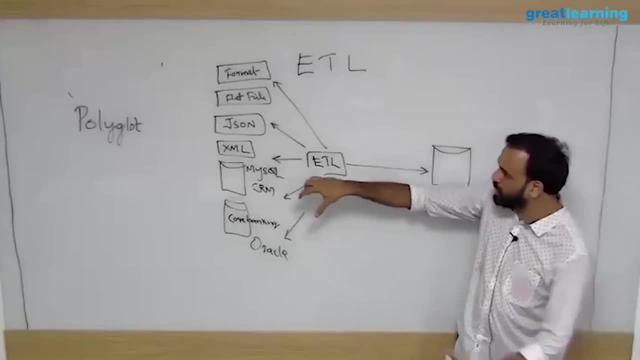 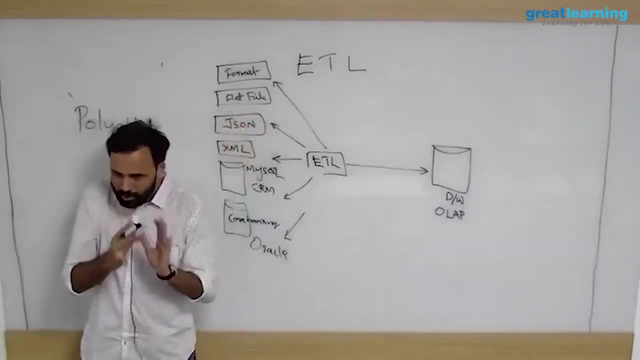 So that is why it is called ETL: extract, transform and load. You don't just take the data, You take the data and dump it here. then it is useless, right? I can read the data from a flat file and give some structure and then dump it here, like. 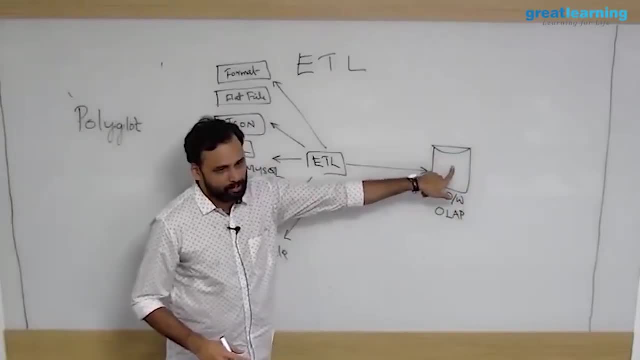 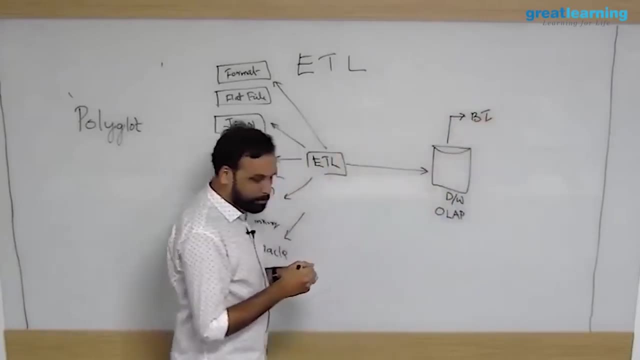 a proper table format. So now all my data is here from this right And I can run business intelligence here: BI tools Tableau, right. If you have heard about MicroStrategy Tableau, what I can do- I can connect a visualization. 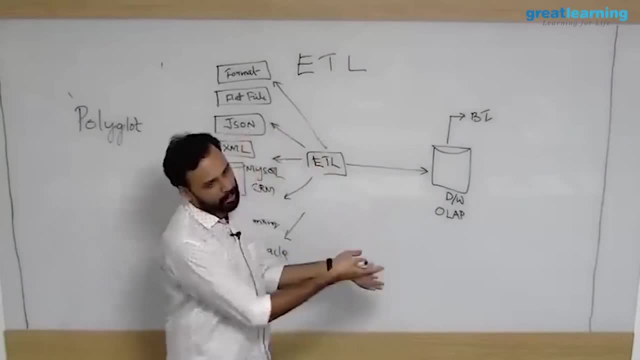 tool here and it will show me in charts and diagrams what is happening. I mean, this is traditional data, This is traditional enterprise architecture. This is how people used to work forever. I mean, every company you go, this will be there by default. 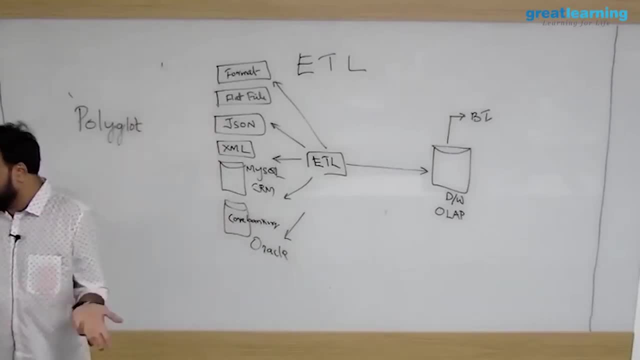 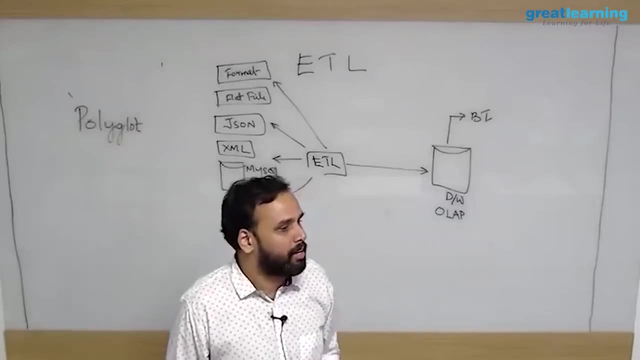 They will have these disparate discrete data sources and ETL tools. So if you have heard about Informatica, Informatica is one of the biggest ETL tool: Informatica, Talent, Pentaho, BI, SSIS. So these are all ETL tools. 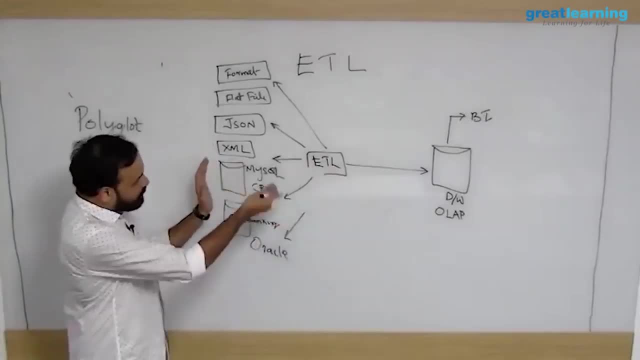 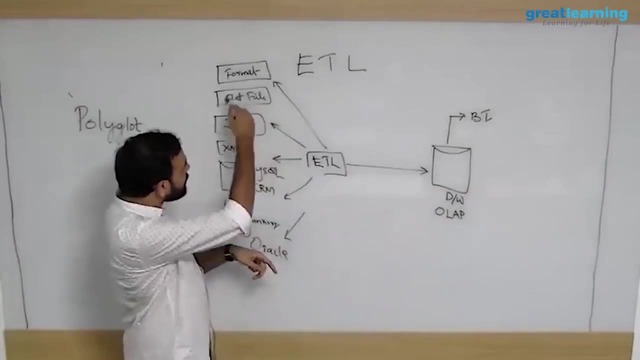 So these tools, what they do, They will connect, They will connect with here and take all the data and apply some schema and push it to a data warehouse. Now the data will be here. So now all the data is in one place. 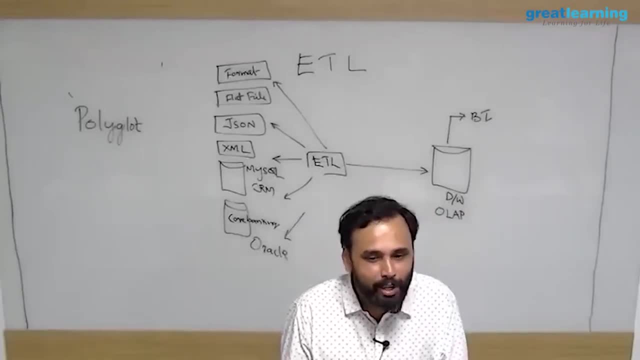 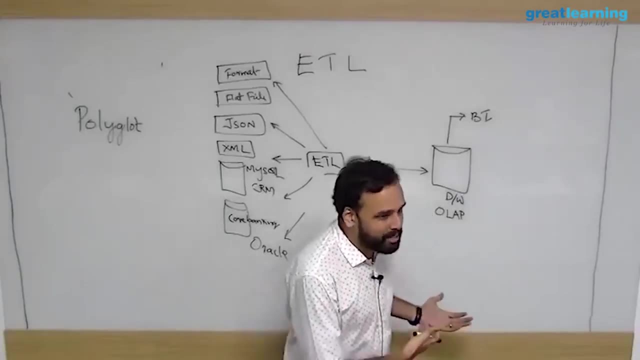 So Chandra Kuchar may not know SQL, right? You can't expect that, right? If you're a CEO of the company, I can't ask you: do you know Java? I'll be fired next moment, right, So? but the CEO want to know what is happening, right? 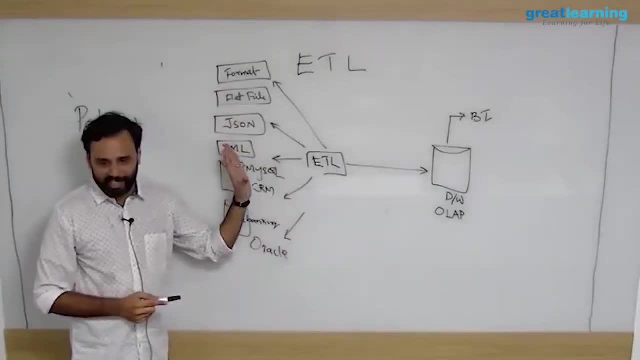 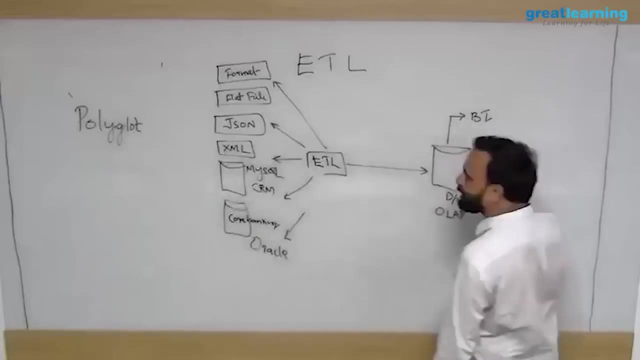 By getting all this data only you will understand what's happening in the company. But you don't have time to sit and learn all this language or anything. So if I'm Chandra Kuchar, I'll go here, I'll connect my Tableau and I'll ask my Tableau. 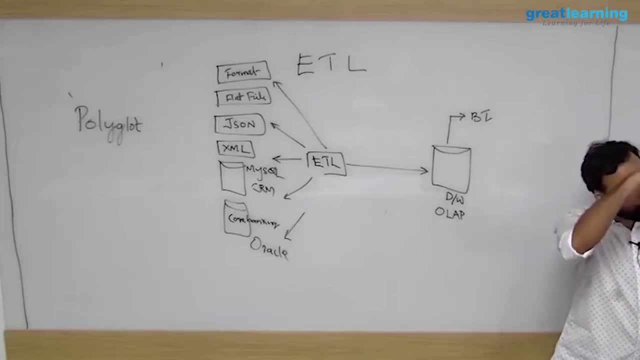 show me the last month's transaction, this quarter, this product, this area. show me. it will show a nice bar chart Now why this is very, very important. If you make any mistake in any of this, this entire stuff will be changed, right. 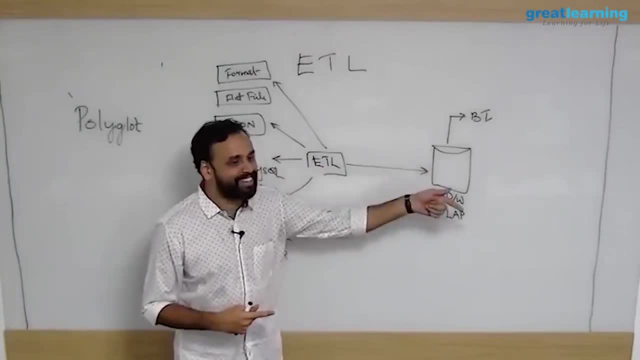 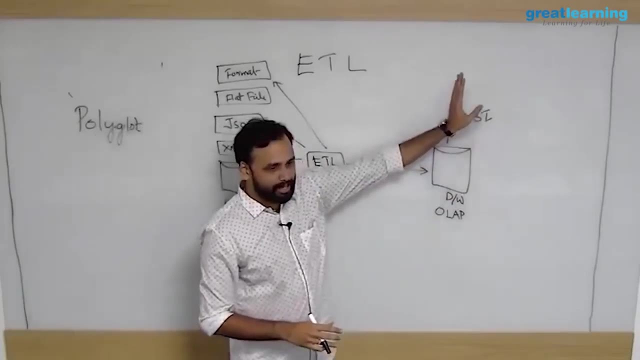 And what she sees will be different. right, She has no idea how this is happening, right? Only you know how this is happening. So your ETL tools should run proper. The data should be captured, Dumped here and then analyzed. 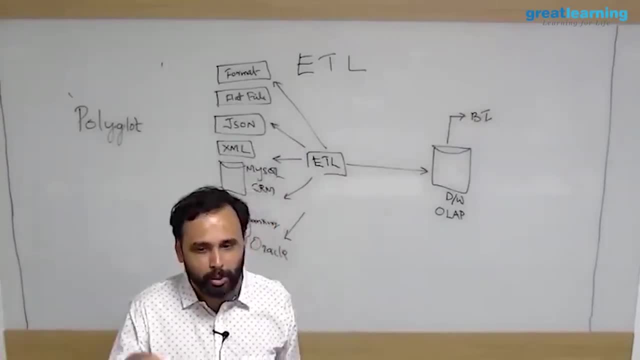 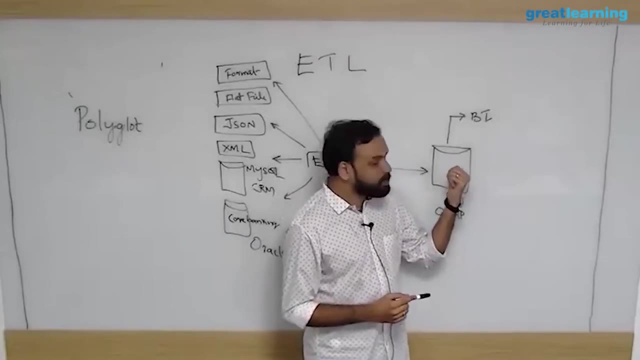 So for CEOs and CTOs. they use visualization tools to connect with a data warehouse, then analyze the data. So all the data is inside this data warehouse, right, And this is not accessible by public. Public has no access to this. 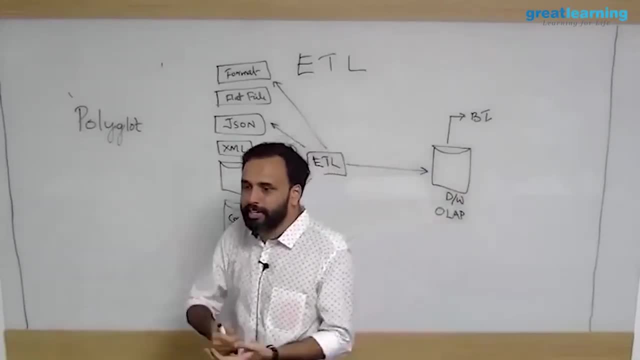 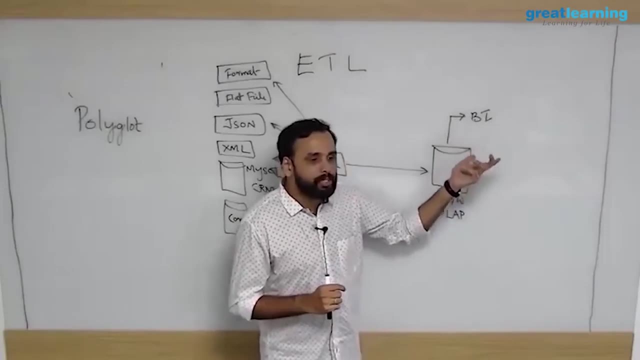 Only internal company has access, like maybe CEOs of ICICI bank. they can go here and visualize the data from here. Others, public, does not have any access to here, right, And then they visualize the data. They make a decision. They do not make a decision, that is up to them. 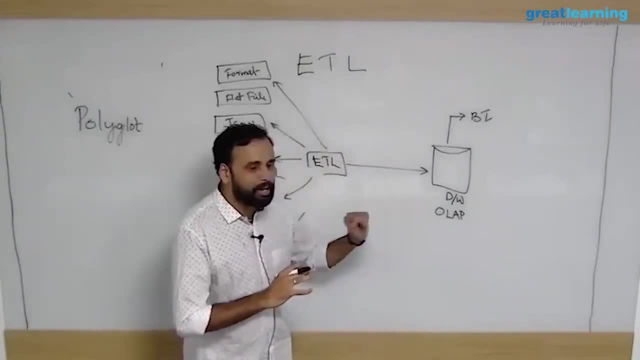 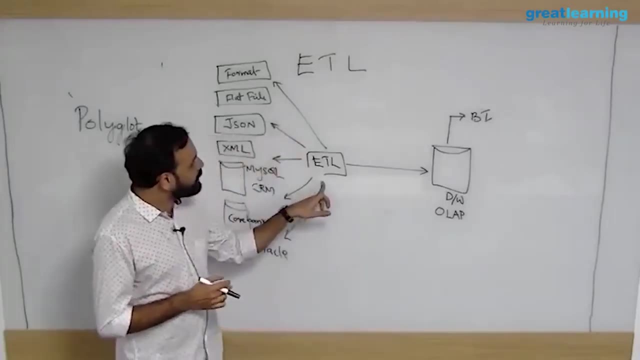 In the whole setup. there is no Hadoop so far, And this is how ICICI bank was running so far. Now, what were the challenges they faced? One of the challenges was that this ETL tool- okay, I don't know how many of you have run. 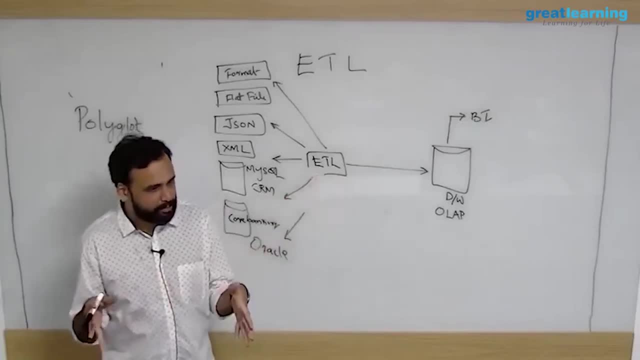 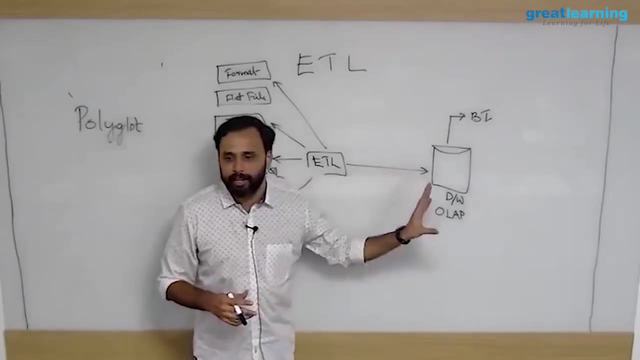 on ETL tools. okay, They typically run on a single machine, So there is a limit as to how much this guy can pull to a data warehouse, How much amount of data this guy can pull from here to a data warehouse. there is a 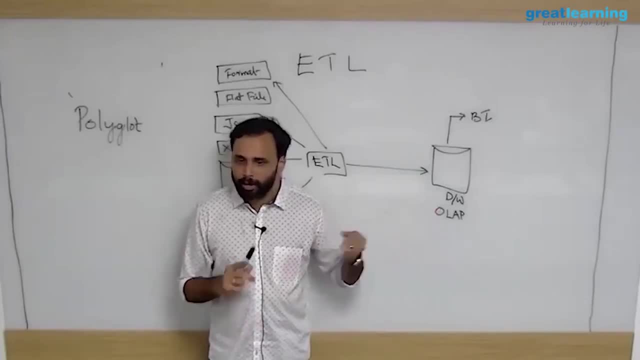 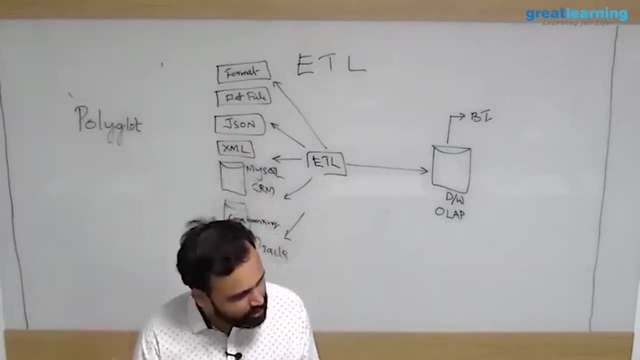 limitation. You can't have terabytes of data being pulled. Okay, Point number one. Point number two: none of this is real time. I go to Tanishq store. Tanishq is a jewelry stuff. I go to a Tanishq store. 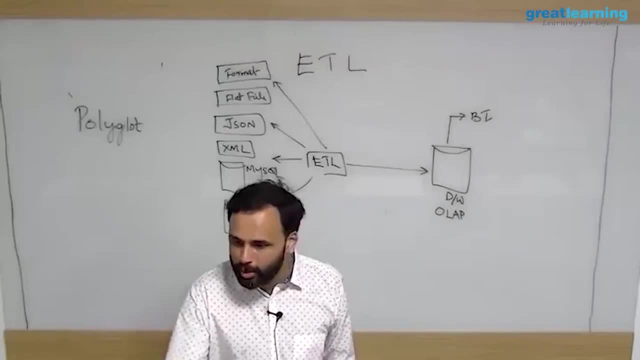 I buy something from there for 20,000 rupees, I use ICICI credit card. I should immediately get a message saying that again you shopped 20% discount. That is real time, because all these are separate data and these ETL jobs run at the night. 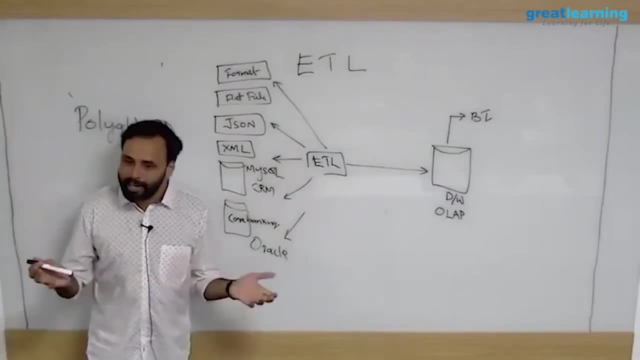 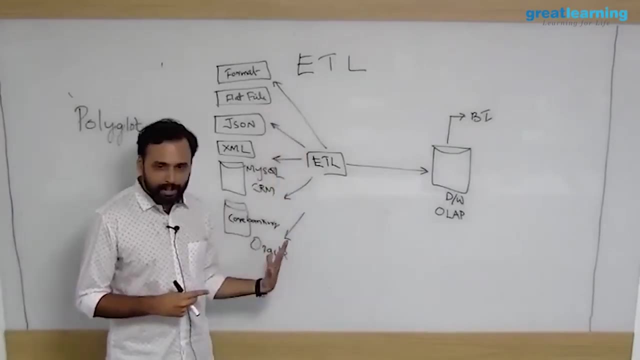 So today morning, if I'm shopping tomorrow, I'll get the message 20% off Anytime I'm out of Tanishq shop. I may not use it at all. So ICICI bank's first problem was that, since the data was increasing, they were not able. 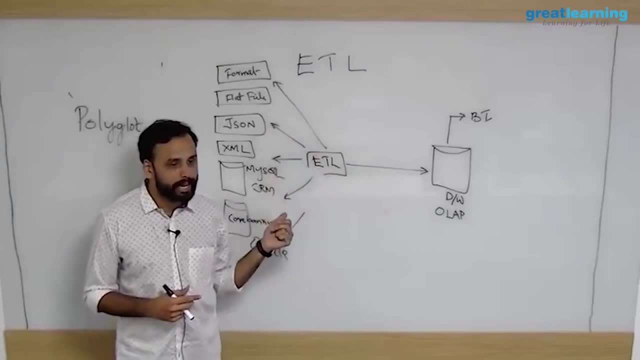 to run ETL properly. Second problem: none of this is real time. They wanted to push customized offers. Their requirement was that whenever any transaction is made, they want to capture it, analyze it and, based on that, they have to recommend something to the user using credit card or 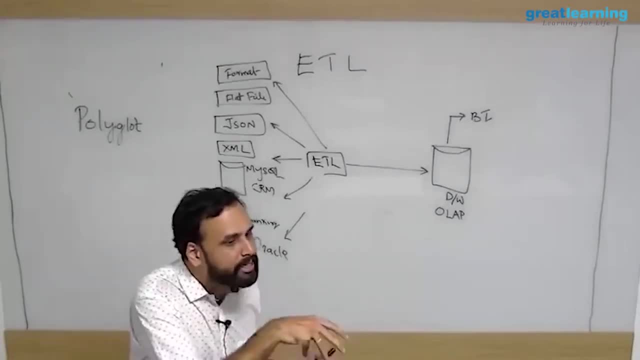 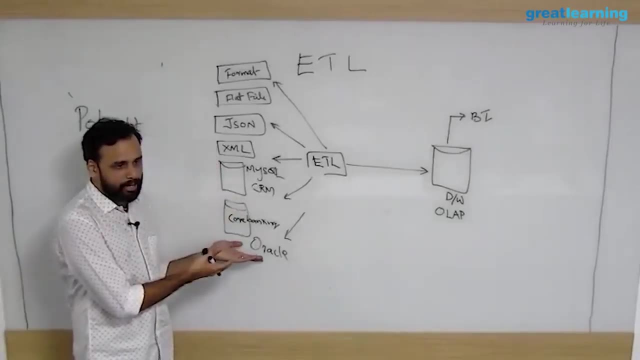 debit card, or even you're clicking on some link, Immediately, something should happen. Now that is not so easy, right, Because your data might be somewhere in here, Oracle and I cannot track each and every transaction here because this is my transactional DB. 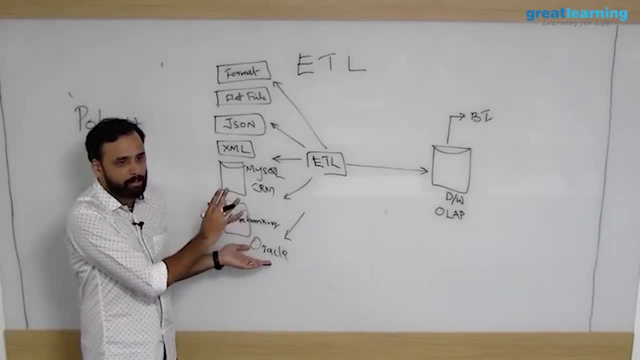 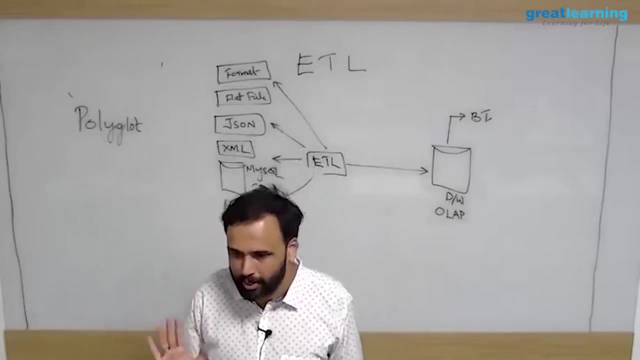 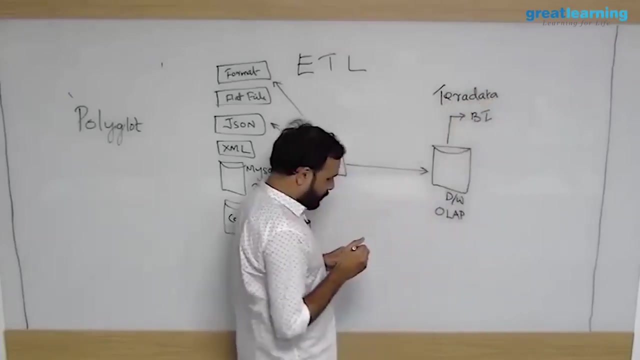 I can't say that track each and everything from here, right, That's not possible. Third problem: this data warehouse. This data warehouse is a very costly affair. I have worked with a company called Teradata. They are the leader in data warehousing market. 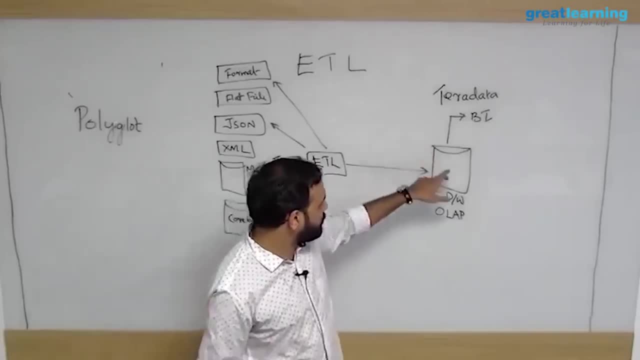 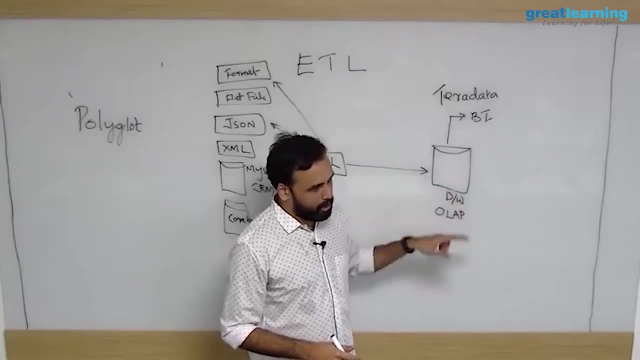 I had a US client. they were using a product called Teradata for data warehouse. They were paying around $5 million every year only for this setup. Now it is good, You can analyze the data and all that's okay, but you're paying a lot of money actually. 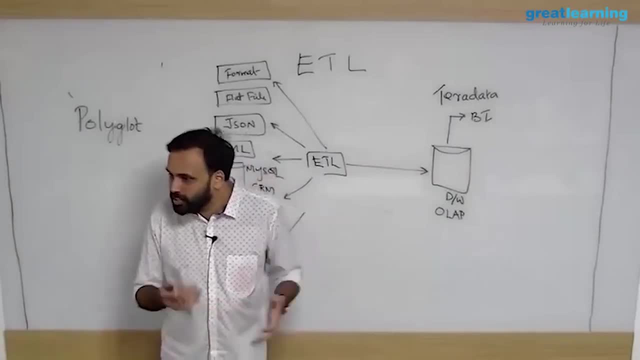 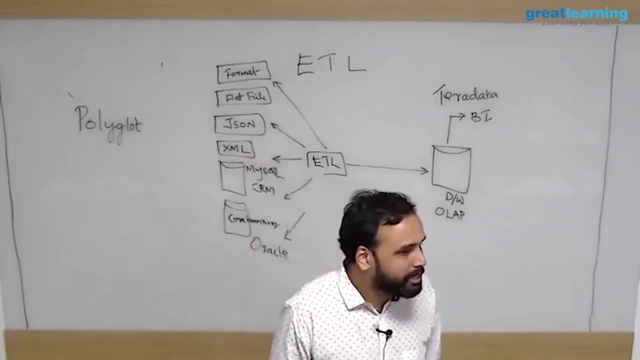 So data warehousing is actually a very costly affair. It's not so cheap if you want to implement. but companies like ICICI bank, they must use it right So they can't say that we will not use it. So they wanted a cheaper solution. 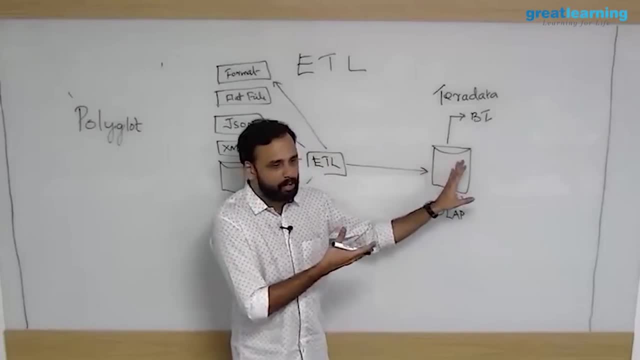 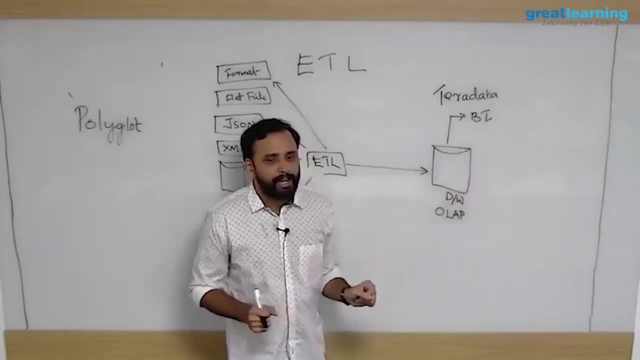 So they wanted a cheaper solution. They don't want all their data in this data warehouse. They want an alternate solution. should be real time, cheaper, scalable, right And anything they want to integrate. any type of data that comes they wanted to integrate. 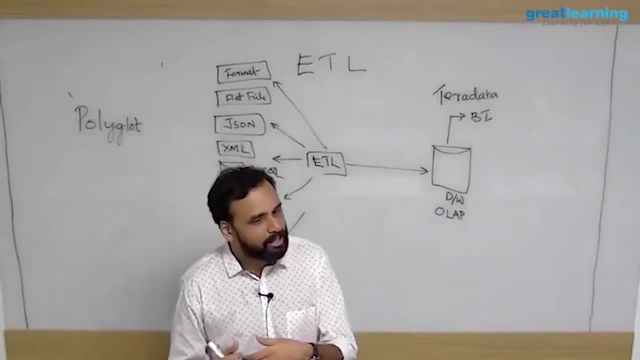 And that is how they came to us and asked us: like can we migrate to some big data solution? And we recommended Hadoop, and then the migration took a lot of time. That is a different case altogether. There is something called MPP. 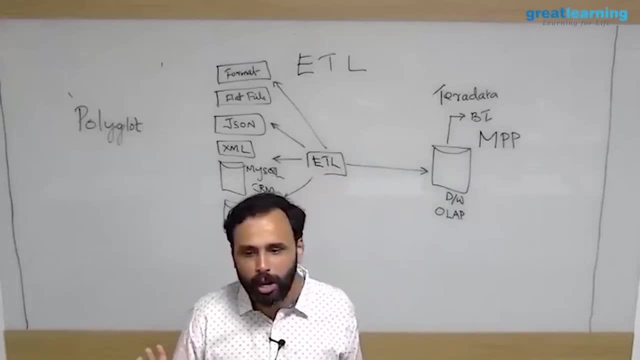 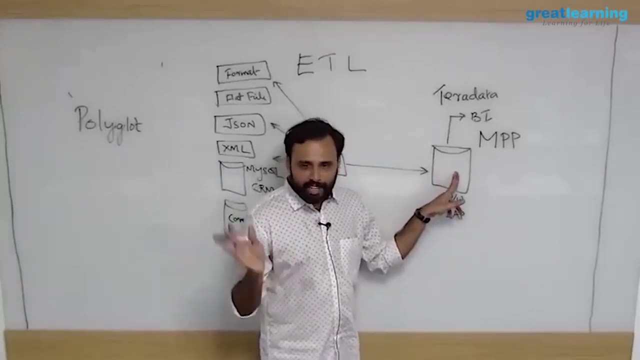 MPP means Massive Parallel Processing. So a lot of people came saying that. So these systems are actually Teradata and all are really faster- actually I mean not like RDBMS, but they're faster. So a lot of people came up and said that, okay, if your data warehouse is very slow. 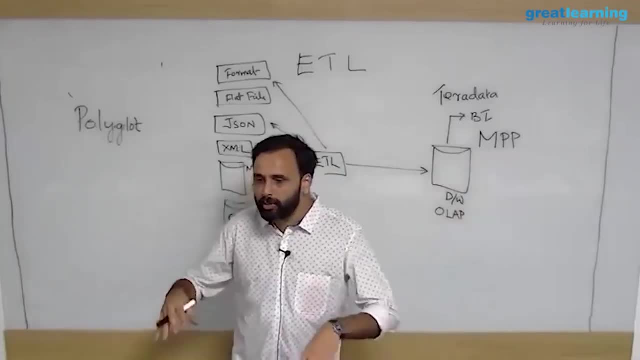 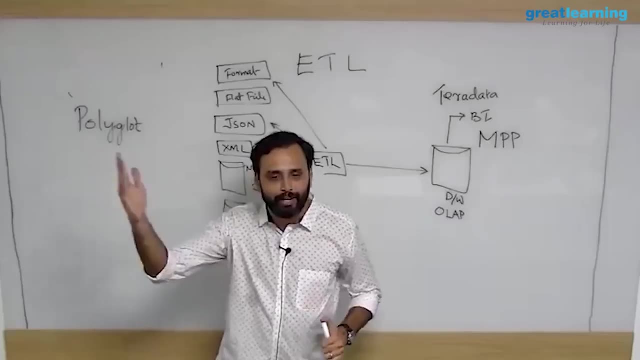 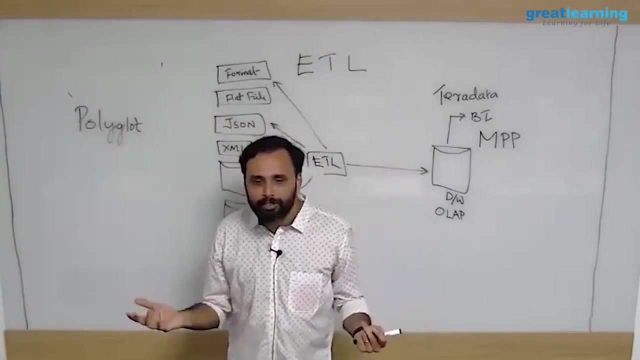 why don't you do parallel processing? You install it on four or five machines and you can do parallel processing. That is possible, but still the same problem exists. You cannot physically divide your tables. Only logical division is possible. Like I said, country-based, you can divide, or month-based you can divide. 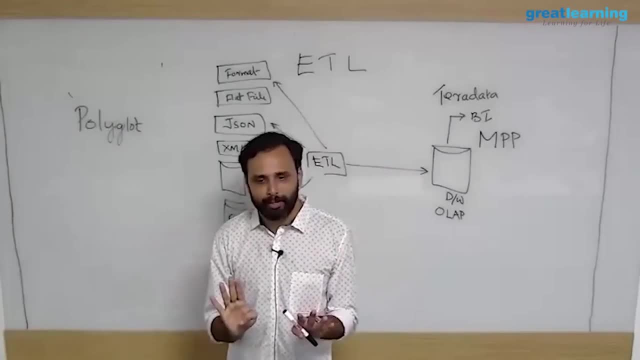 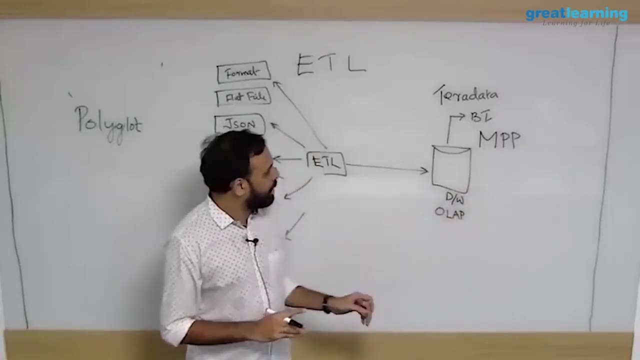 End of the day, if you want to do a join operation or something, same questions will happen, So I can never propose this as a real-time solution. That is my crux of what I'm trying to tell you, And this is how even ICICI bank was running, and cost was another problem. 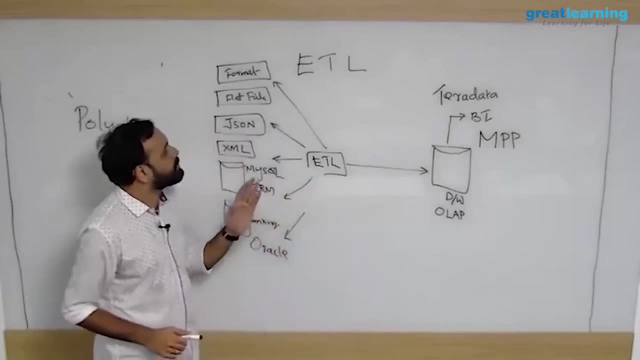 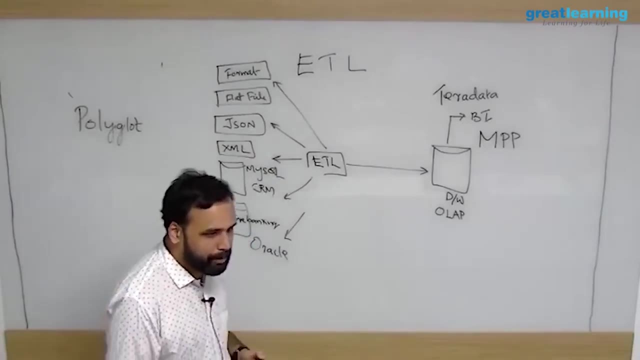 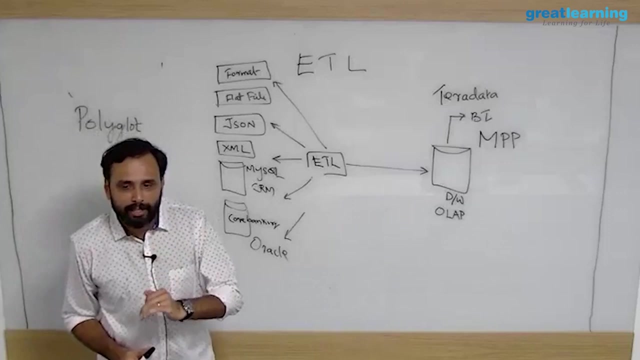 They had a lot of cost involved. So, and obviously, since they wanted to collect a lot of unstructured data, they wanted to go to a better solution. Okay, So Hadoop came into the picture. So now the point is that now let's discuss a little bit about Hadoop. 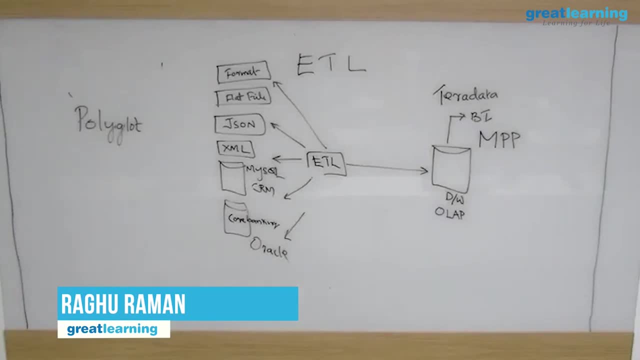 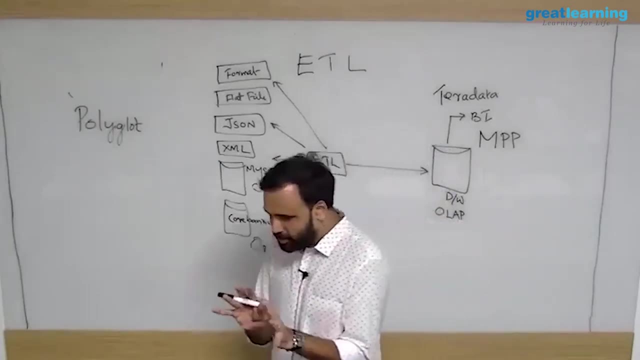 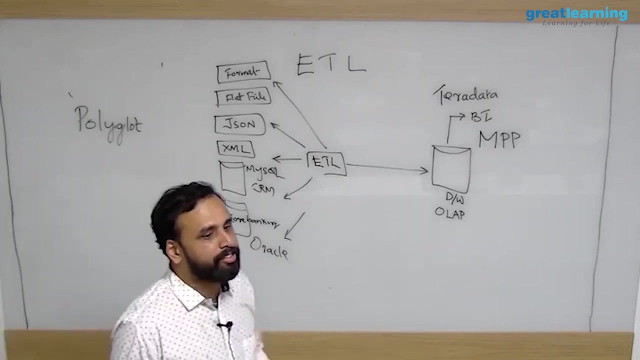 So what I thought is like today: probably we can cover the architecture and a little bit of theory, And then you have MapReduce. Now there is a catch here. MapReduce is the default programming framework on top of Hadoop, So if anybody wants to analyze the data, 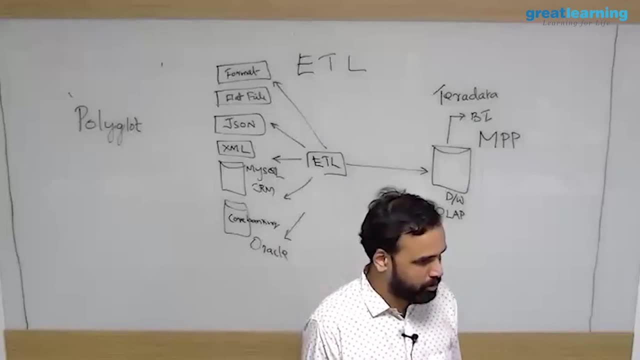 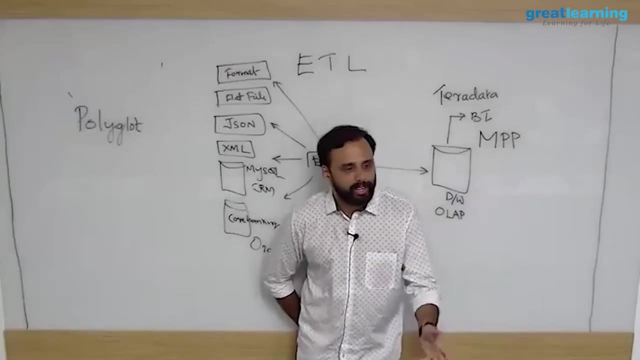 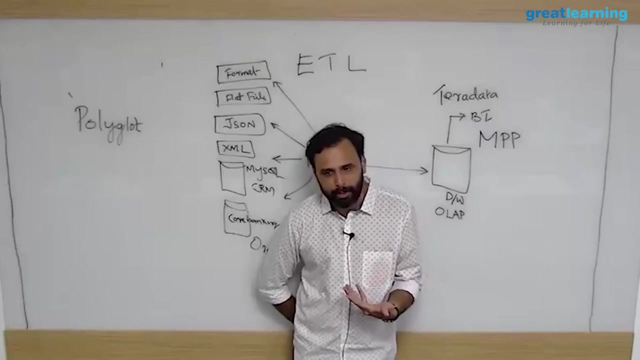 On top of Hadoop they use something called MapReduce, Point number one. Now, MapReduce came long back, Okay, And today there are a lot of ways to analyze the data, not only MapReduce. Now, as per your syllabus, the curriculum says: teach MapReduce and then some concepts in. 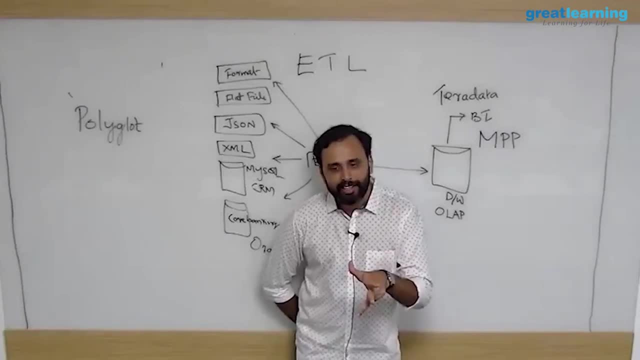 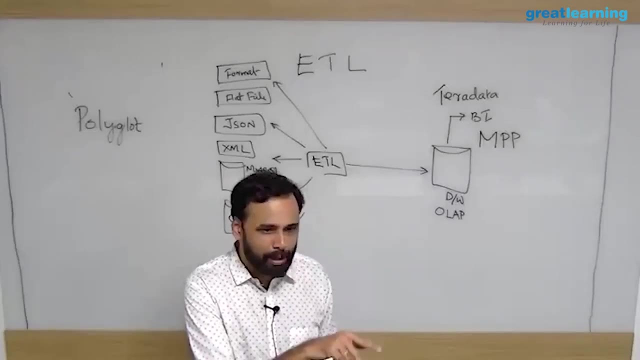 MapReduce And I will be doing that. But one other thing is that if you want to learn MapReduce, ideally you should be an expert in Java, Because MapReduce programs are written in Java. Okay, Or any other programming language. 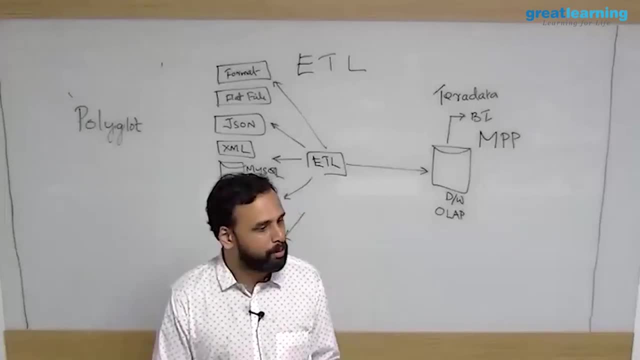 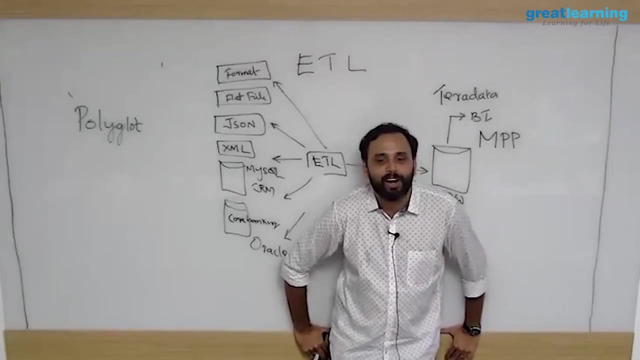 You can write in Python and other things, But natively people write MapReduce programs in Java. Now I know that not all of you are familiar with Java and comfortable with Java, So if I talk a lot about Java it may not make much sense out of you. 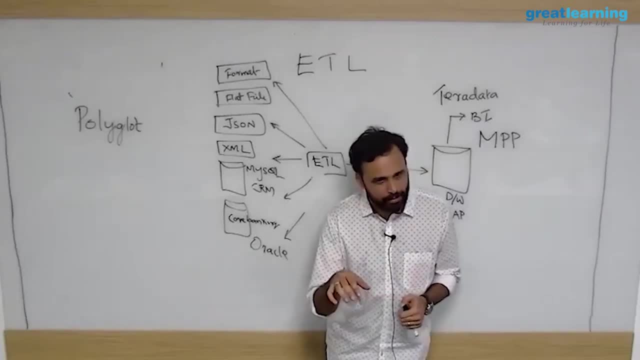 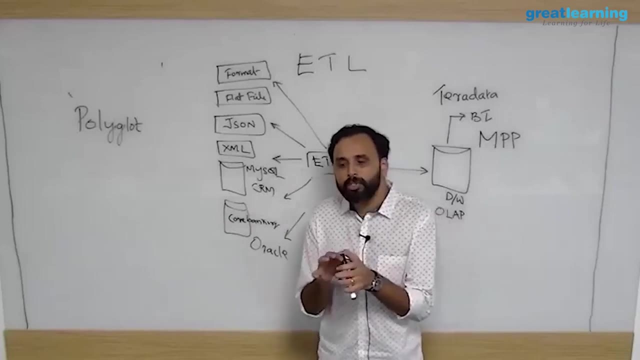 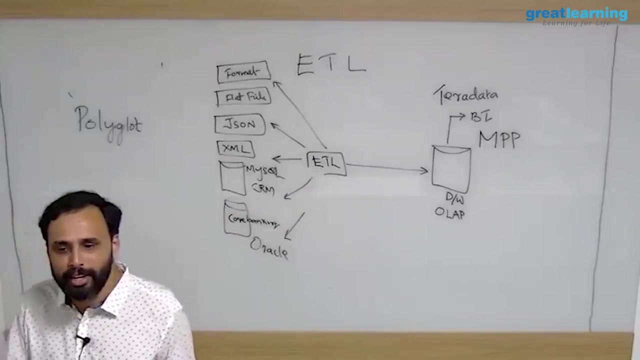 But then why you are learning MapReduce is to help you in Spark. So next you will be learning something called Spark. right, 16 hours of Spark content will be there. Spark also uses similar concepts as MapReduce. So, even if, even though you're not able to understand each and every line of code, that 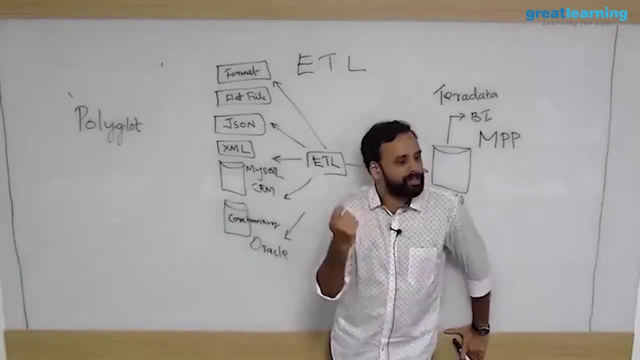 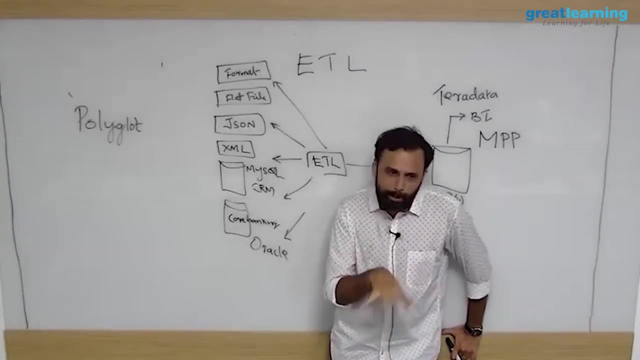 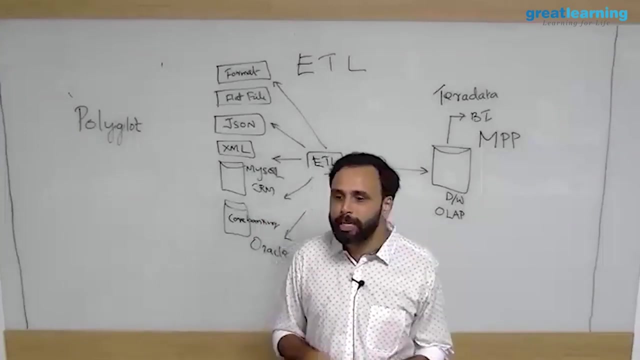 I'm writing, that's okay, But you need to understand the logic, how it is working, Because Java programs not everybody will be able to follow and understand and debug, So that is not expected also from you. But if we discuss MapReduce, I write a MapReduce program and we run a MapReduce program. you. 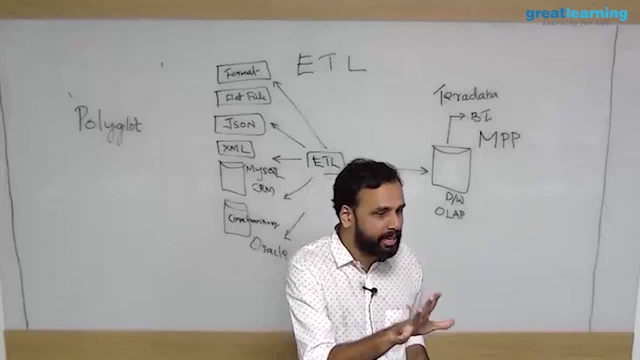 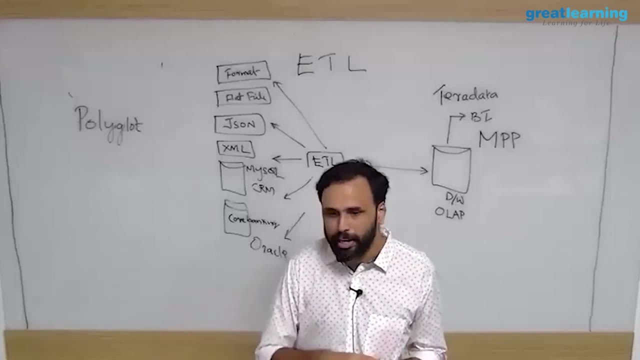 should be able to understand what is happening inside that right logically, not like syntax. wise, line by line, wise right. So once we complete Hadoop architecture- like tomorrow I will be discussing MapReduce theory- and MapReduce programs will be running. 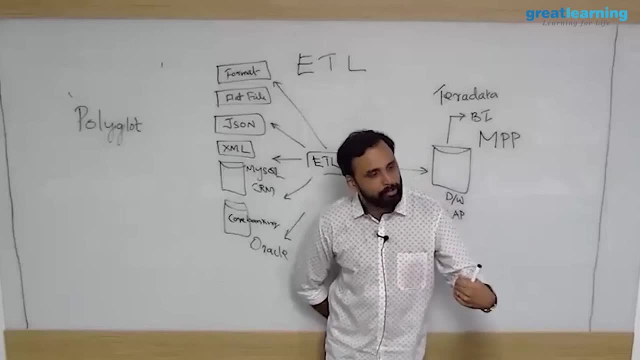 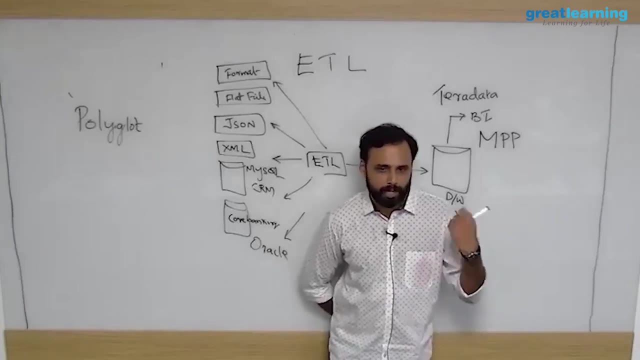 And then in the next eight hour syllabus we will be completing bit of MapReduce and going to something called Hive, Apache, Hive. So Hive is your data warehouse in Hadoop, So that is more of SQL side. So you can understand that point. 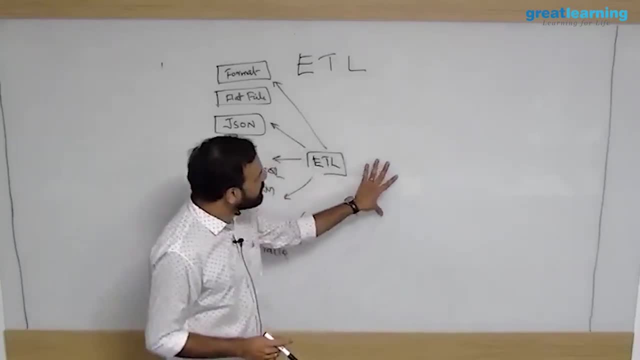 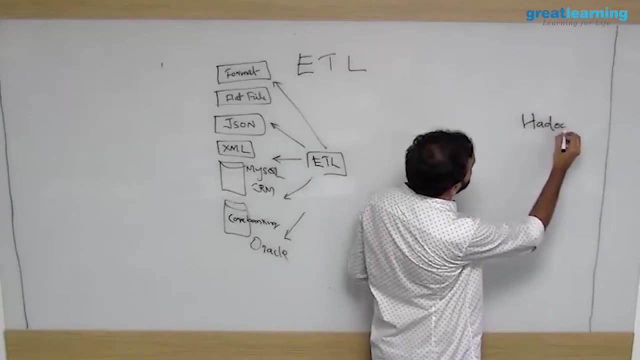 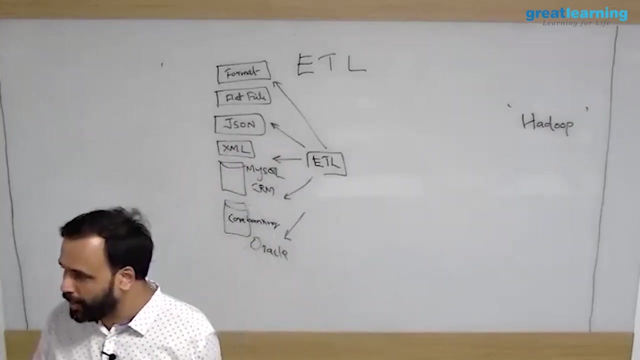 So now, speaking of Hadoop, our architecture is here still, I just changed a little bit. Okay, I'll just write it here. The question is when all this happened? right? So a lot of people. so I handled a lot of trainings in Hadoop and Spark. 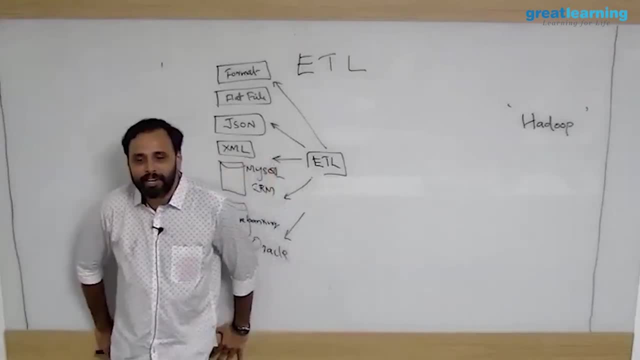 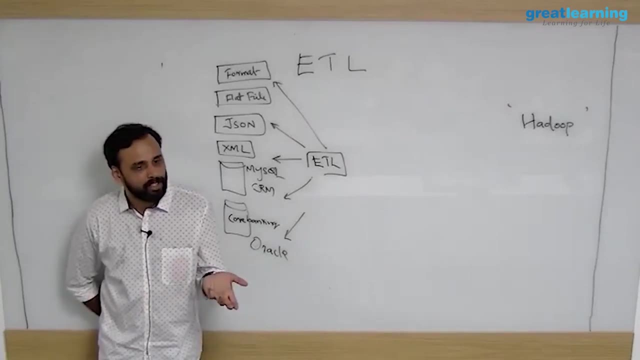 So a lot of people asked me that. okay, so we are learning a completely new technology called Hadoop, And I will say that you are wrong, because Hadoop came in 2005.. So almost 13 years now, So it's almost like very old. 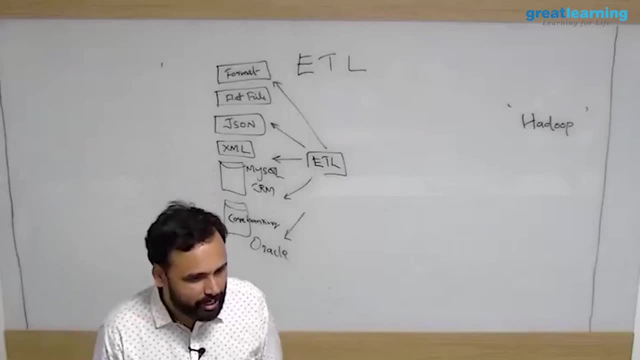 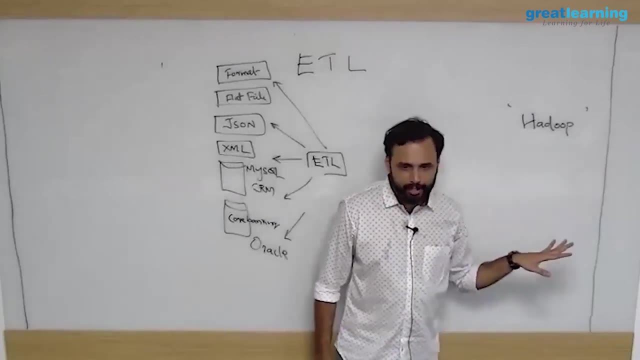 But for people it is still very old, But for people it is still very new for those who do not understand Hadoop. So in 2005,, this framework called Hadoop was created a long back right, And there were two guys called Doug Cutting and Mike Caffrilla who created this framework. 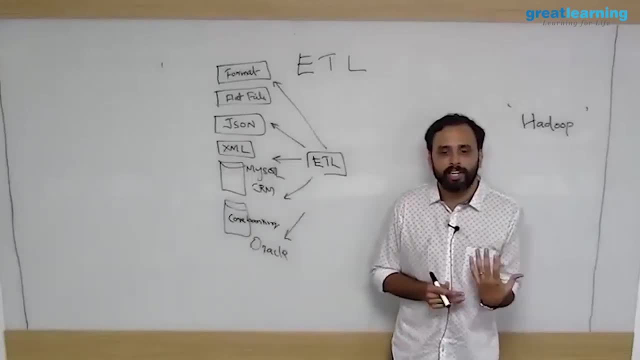 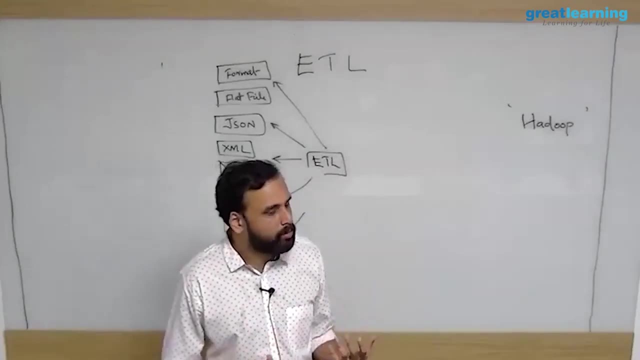 They took the original idea from Google. So Google was already doing a lot of distributed computing And Google was dealing with a lot of big data right. So they published a couple of white papers And this- Doug Cutting and Mike Caffrilla- they took the idea from Google and then created 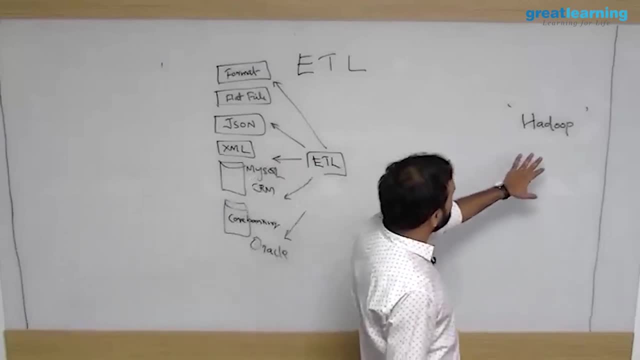 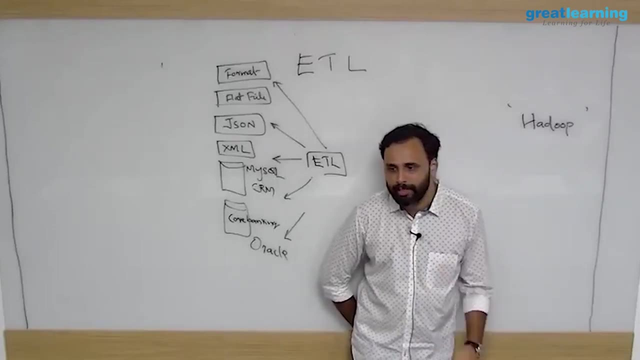 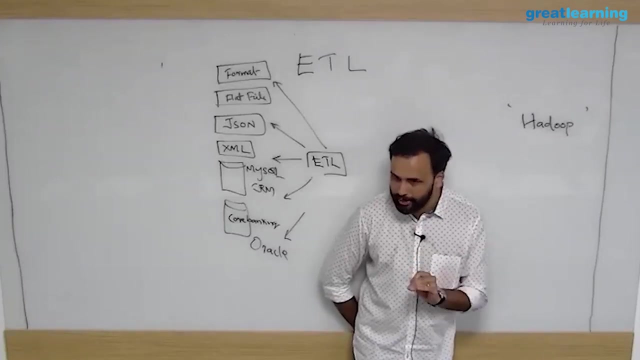 a framework called Hadoop, And later they gave it to Apache as an open source project. So Hadoop is an open source project actually, which means it is with Apache. right now. You can download it for free, install it for free. you don't have to pay any money. 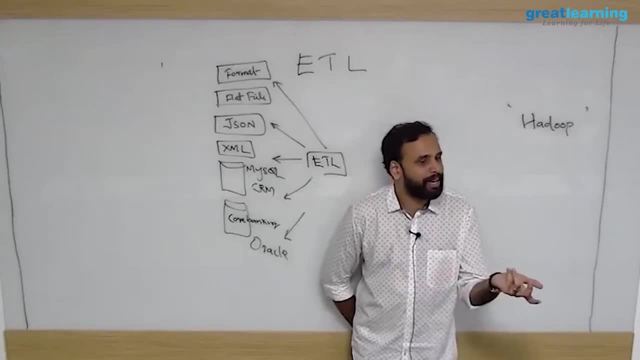 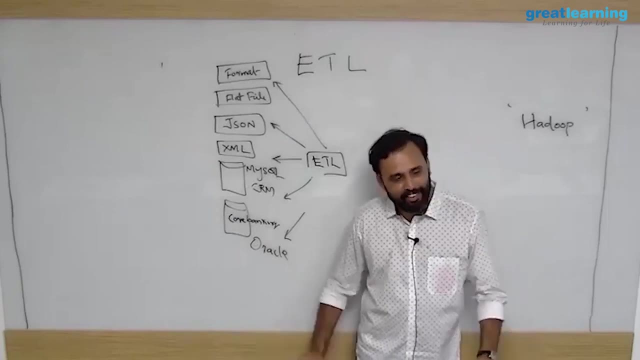 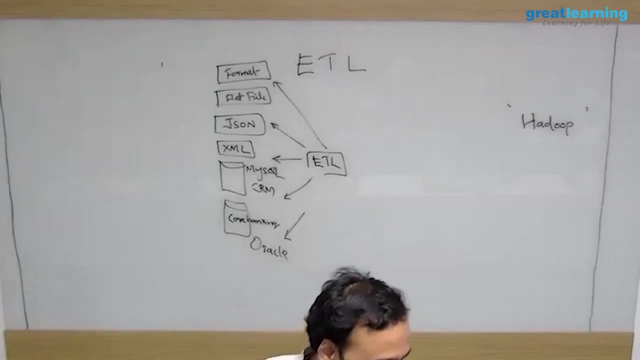 But if something is really free, you have drawbacks also, right, Correct. For example, you have Android phones. I have an iPhone, I used to use Android phones, but you know the difference, right, The difference is not show off. That is not the difference. The real difference is that Android phone might get a lot of bugs which may not come in an Apple phone. If you have used both, you will understand. The problem is Android is open source right And open source means every company will modify according to the requirement. as Samsung phone. 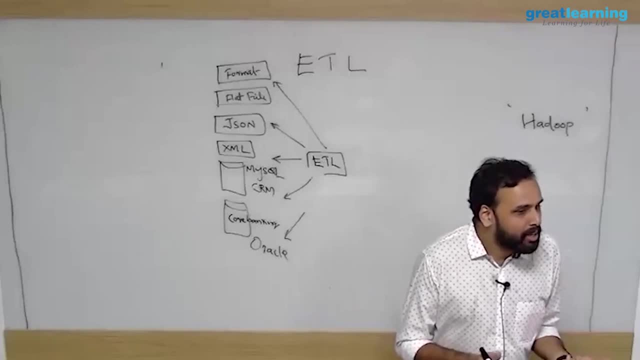 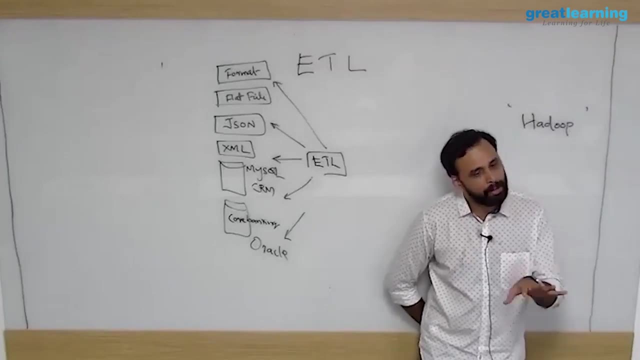 they will have their own Android right. So accordingly, a lot of bugs may come. The platform may not be so stable as it is. If it is an Apple phone, only Apple produces it right, And if there is a bug, also if I call Apple or somebody called Apple, they will fix it. 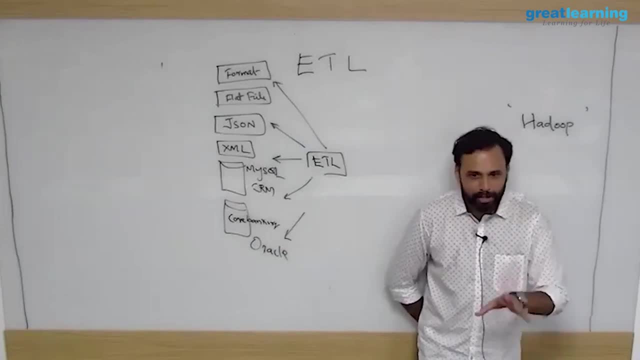 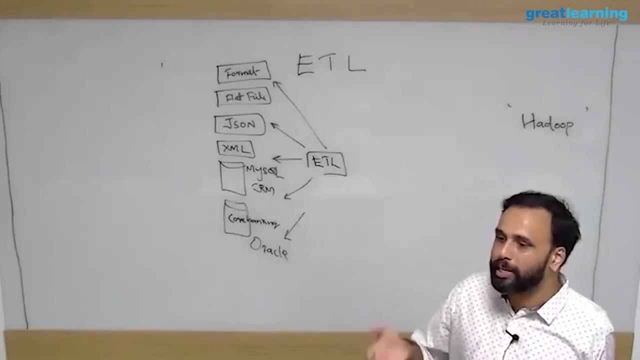 Because there is only one version of it available And they know what bugs may come, may not come. So the same story here. originally it was Apache Hadoop And even still you can go to the Apache website and download Hadoop. 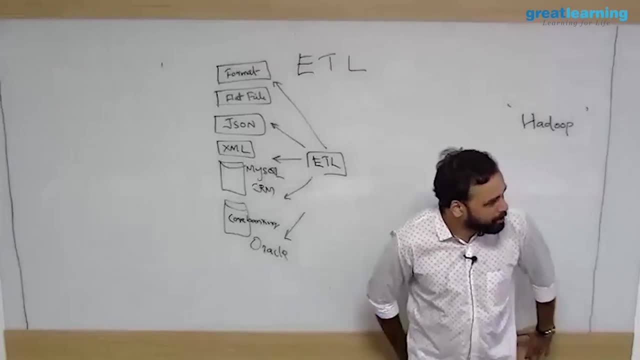 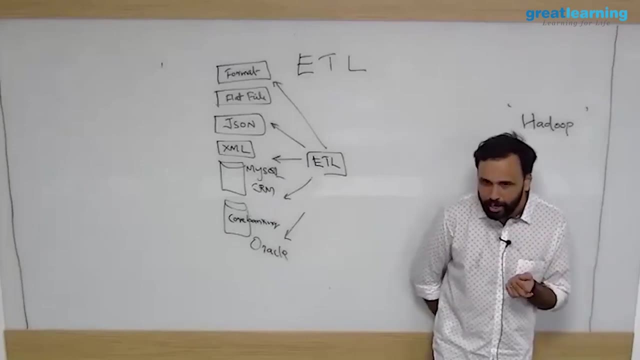 But soon people realize that if they are using Apache, Hadoop, it is open source. But if something does not work, something crashes, nobody is there to fix it Because it is open source And accordingly a company called Cloudera came. 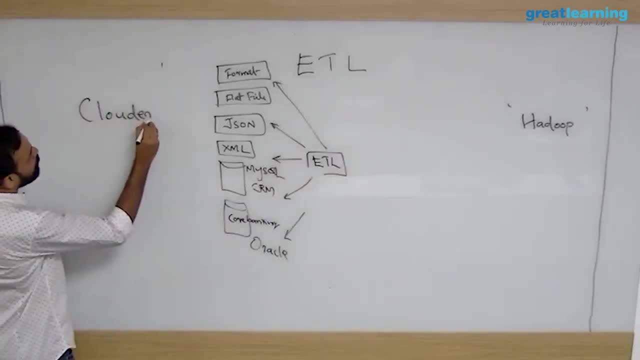 There is a company called Cloudera. You might have probably heard. Cloudera is the first company which created a commercial distribution for Hadoop and related tools. So today you can go to Cloudera and ask them to give you Hadoop. 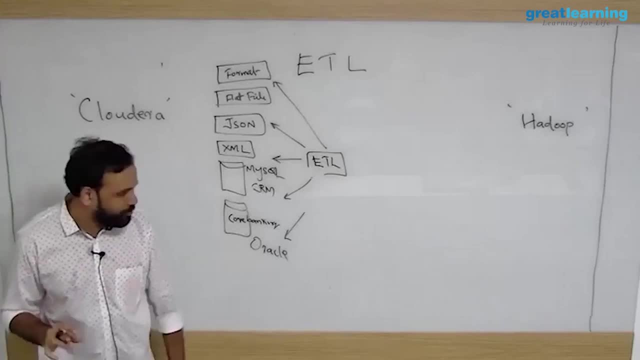 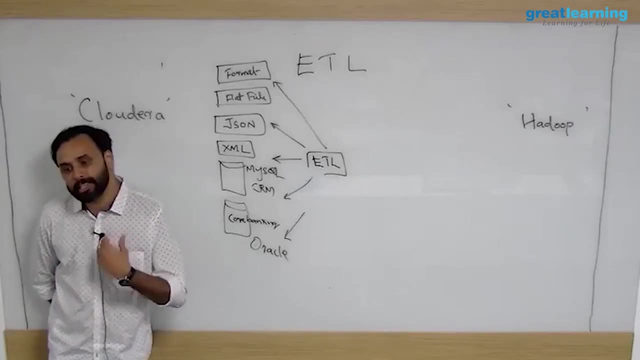 What is the advantage? You will be getting the same Hadoop, almost similar what you find in Apache website, But if you install it and if something is not working they will fix it, You have a support. Since you are paying money, you get support just like a vendor, right? 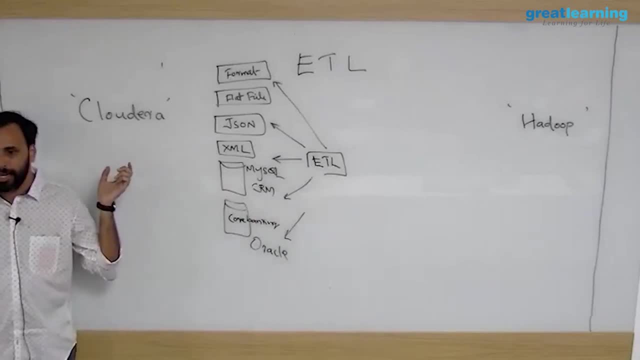 So one of the companies which is very popular in the world of big data is Cloudera. So they sell Hadoop, Spark, Right, Yeah, Spark everything as a bundle. okay, Even your lab actually has Cloudera distribution. The lab we are going to use actually runs a Cloudera distribution. 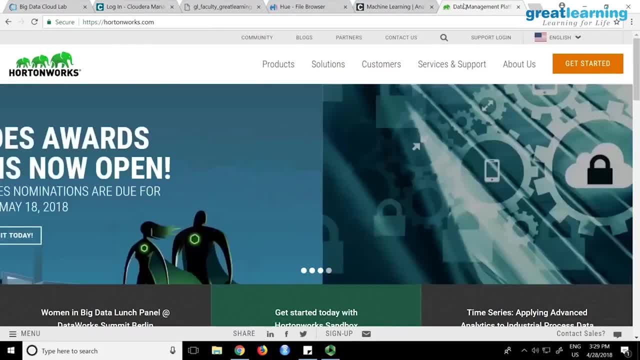 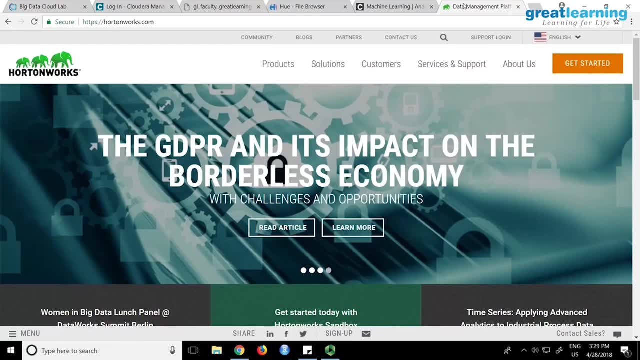 Only thing: they should also provide a free version, And they do it. So if you go to Cloudera, you can download the Cloudera's product for free. You don't have to pay any money, but you will not get support. 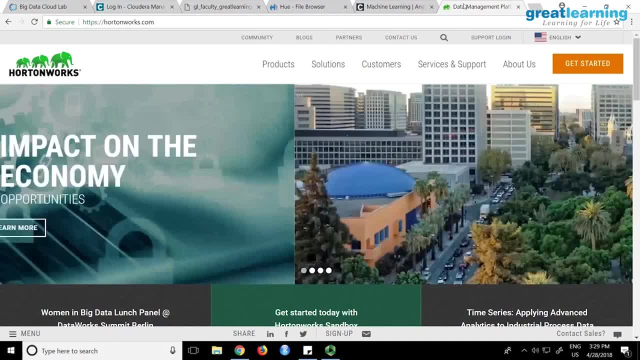 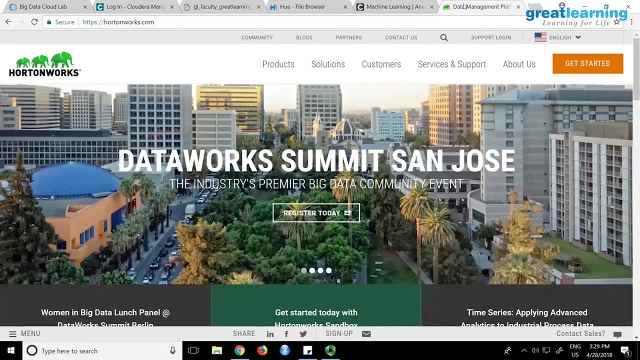 So what people do? they will buy only with support, right? So if I want to sell Hadoop, I can start a company. I can download from Apache, modify the source code. I can sell it to you guys, Right? So these are the two things. 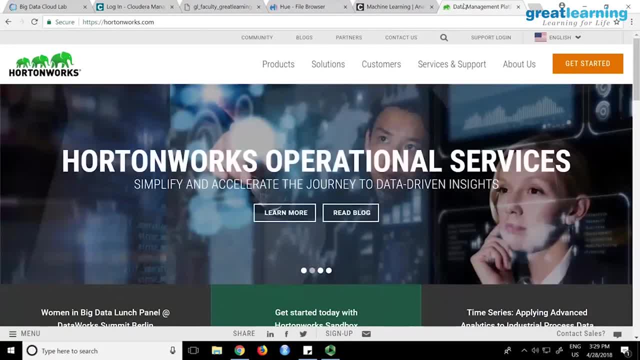 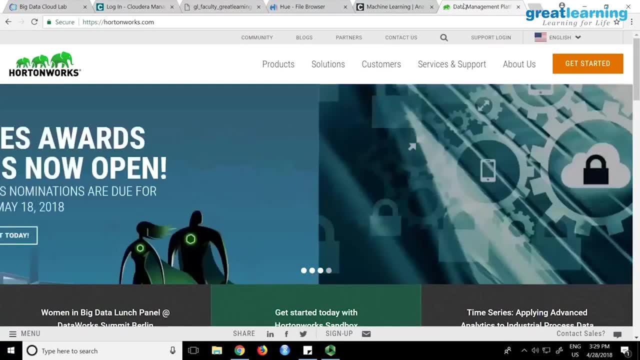 One. I should give a free offer also, No support. Second thing: that is the story with every open source. right, You have Ubuntu Linux, you have Red Hat Linux. What is the difference? Hadoop And you can download from their product. 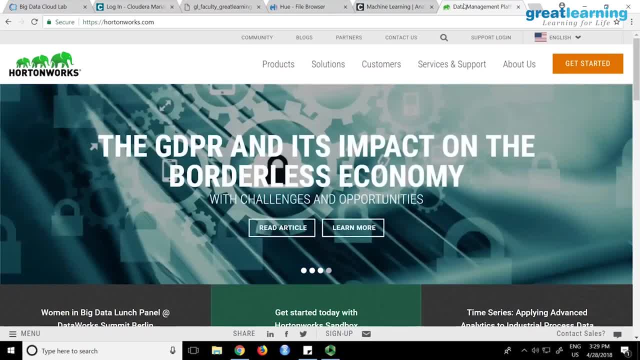 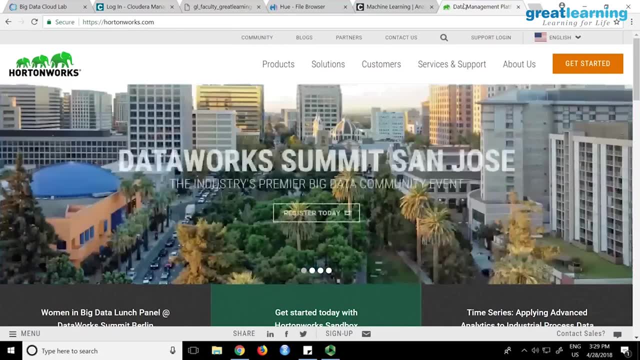 Cloudera is not 100% open source. it's a custom product, But you can download it for free from their website and install it on as many machines as you want, But you will not get technical support. So ideally people will not do it right. 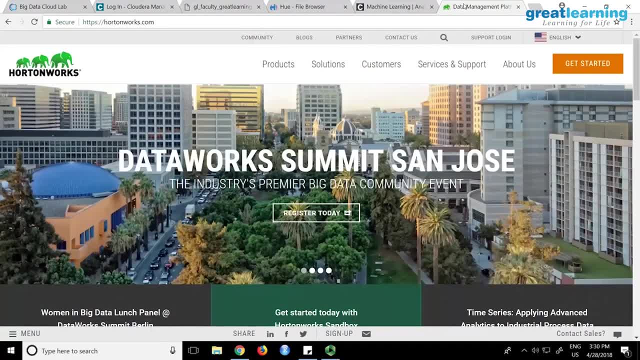 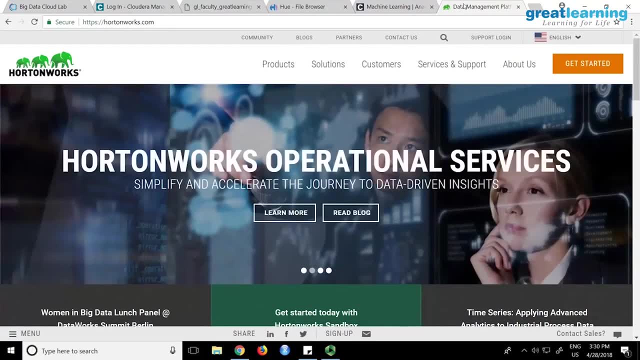 Because you need technical support. so you will pay money and get it actually Right. But these are the companies- the Hortonworks and Cloudera- as the leading vendors in the big data world. They also provide certification, So if you want to write a certification exam- probably after the Spark class- you can try. 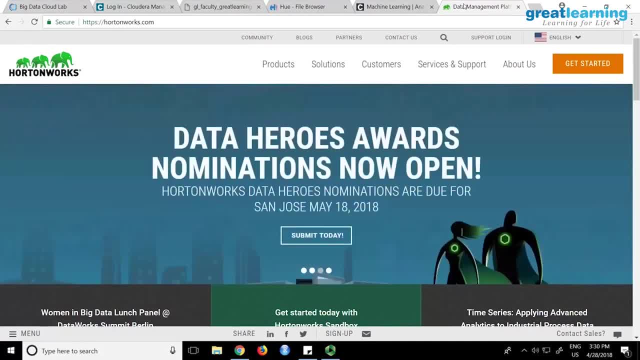 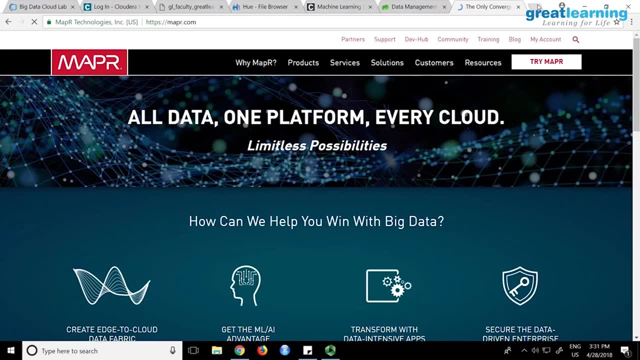 that Cloudera provides certification exams in the big data world. You can write it and get. There is also one more company called MapR. To be very fair with you, why still people are trusting all these companies- Microsoft or Apple or Oracle- they get support right. 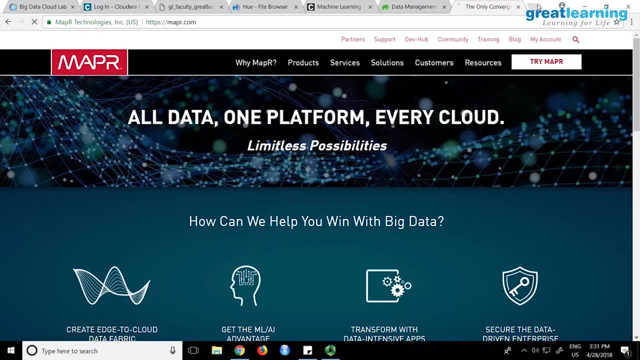 Everything doesn't work. You cannot be able to fix right. You have to call them and make them fix. So MapR is the third company which is sort of like popular. This company, if my information is correct, was created by a couple of people who quit. 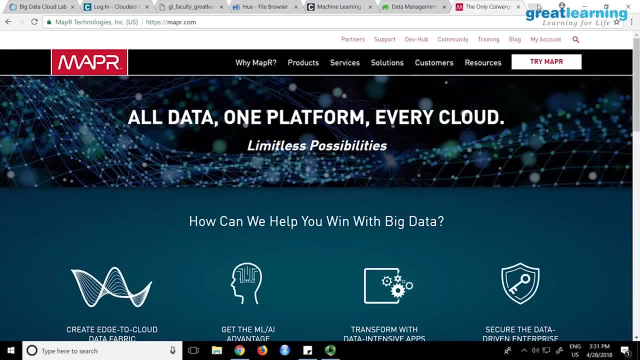 Cloudera and Hortonworks- Indians only right. And they found this company called MapR. MapR is very popular these days, actually a very, very popular vendor. The highest paid edition is also MapR. MapR's architecture is also very different, not like traditional Hadoop architecture. 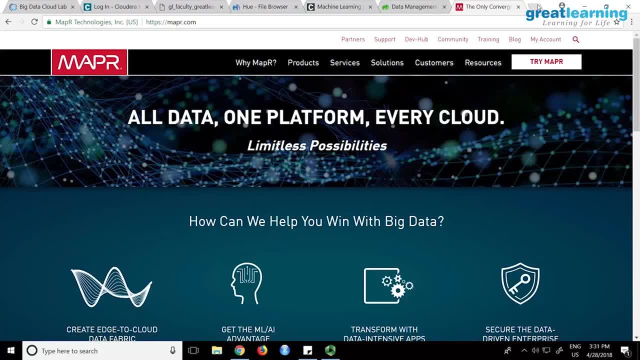 right. So for that reason, like I went to GE, I went to Flipkart. they're all using either Hortonworks or Cloudera. They don't use MapR much. Apart from this, IBM has their own flavor. It's called Big Insights. 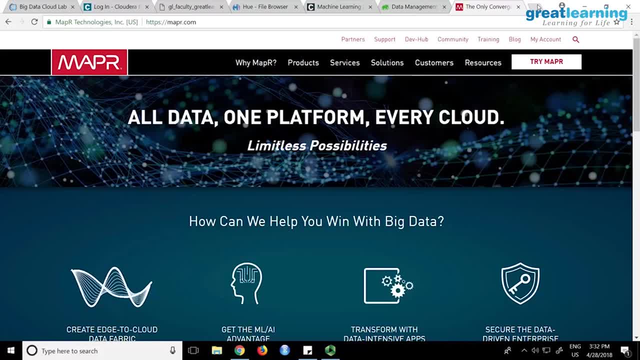 Microsoft has their own flavor that's called HD Insight. HD Insight is there. Amazon has. Every company has an edition of their own Hadoop and big data platform, But most popular ones are Cloudera, Hortonworks and MapR. These guys are the most popular ones actually. 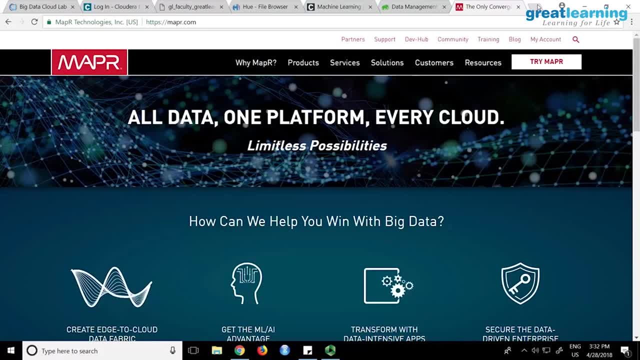 For a developer, there is not much difference. For example, if you are a developer, there is not much difference. For example, if you are writing a MapReduce program, it will run the same way on all three platforms. There is not much of a difference. The difference actually is that Hortonworks is totally open source. They sell the same what Apache gives. Cloudera modifies it a bit And they say that with the modification Hadoop is more stable. That is their claim. We don't know. 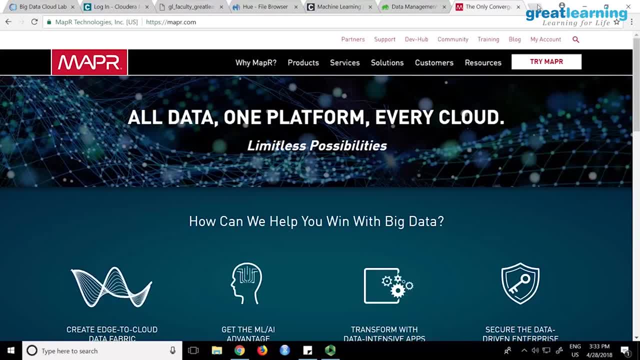 It's all marketing gimmick. It is same like buying an Android Samsung mobile phone and HTC mobile phone. What is the difference? End of the day, internally it is Android, But Samsung will say that our Android is better. We don't know. 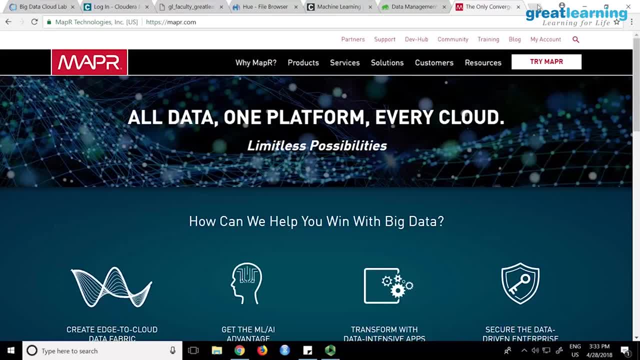 Android is better, more bug-free or something. HTC will say that this phone will never hang, So only HTC or Samsung know what they have done inside the phone. But, end of the day, if I download, let's say WhatsApp, it will run on both the phones. 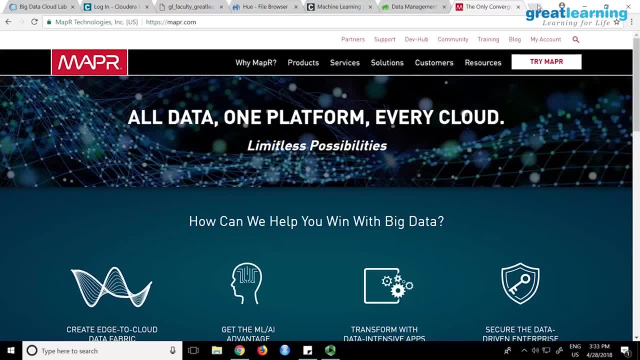 right, Because it is Android. So same thing, only It's just a commercial distribution. Same story with Linux. You can buy from Red Hat. There is also one more provider, right: SUSE. Red Hat Linux, SUSE Linux. 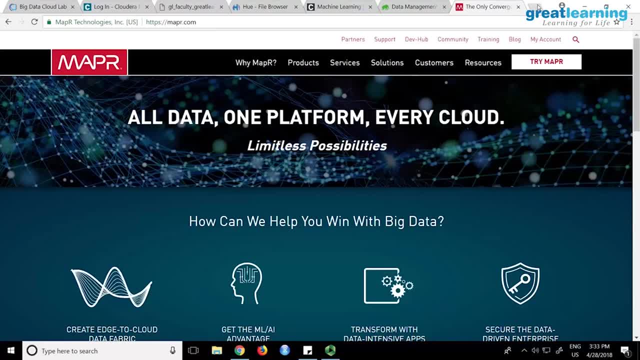 Everything is same. If I type an ls command, it will work both ways. Kernel might be slightly different, But end of the day they are paying open source original Linux only. So same story here, But considering the platforms, Cloudera seems to be more popular because they got a head. 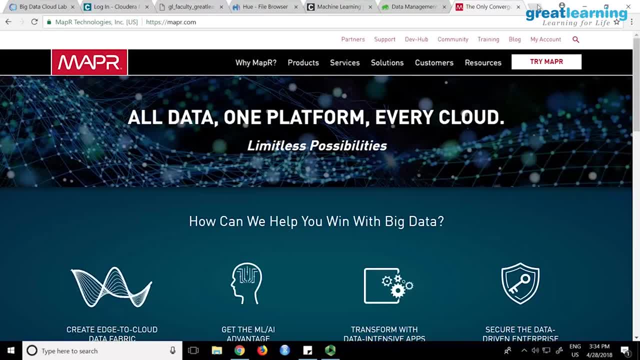 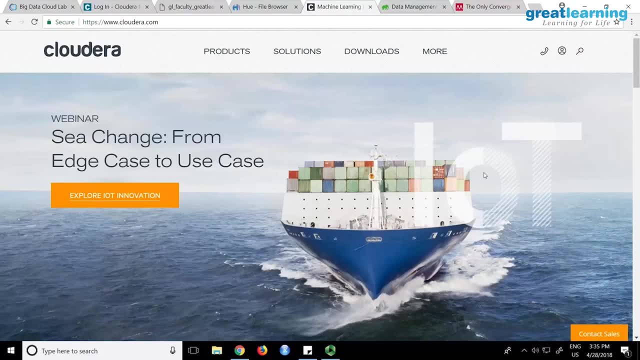 start 2008,. they started Right Long back. they started Hortonworks is also gaining a lot of popularity these days. I have been seeing that And why you are learning MapReduce. Two reasons. One is migration. A lot of companies will already have a lot of MapReduce programs. 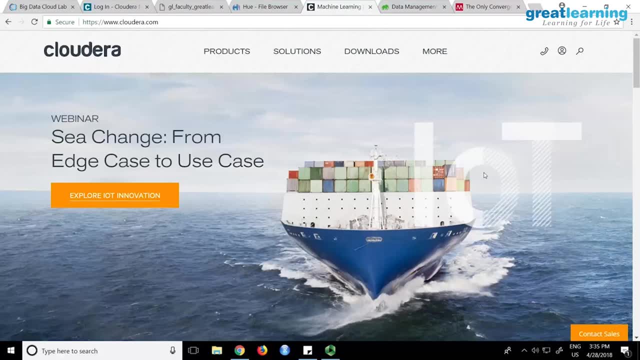 And they want to go to Spark. So if you want to go, you should know what is MapReduce. Second reason: even for learning Spark, the concepts of MapReduce are important. Spark also was built on the basic idea of MapReduce. 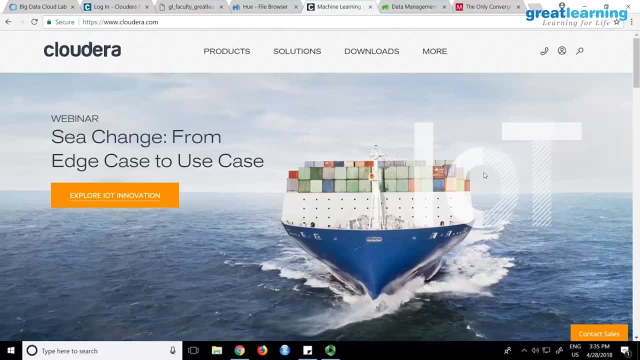 So how MapReduce works, how the program runs. these basic concepts. if you can understand, that will help you to learn Spark in a better way. That is the reason we are learning MapReduce actually In the enterprise, totally gone. 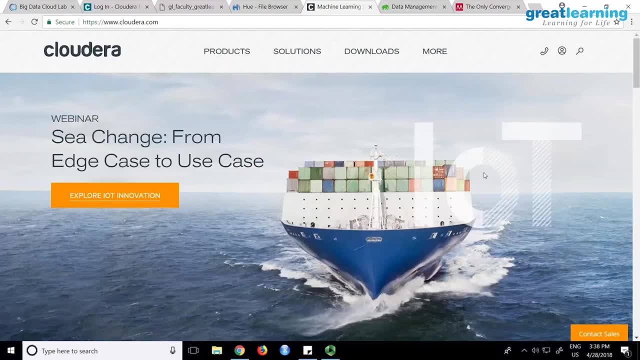 That's it. There is nothing called MapReduce, And so always, you cannot say that Hadoop is 100% a replacement of a data warehouse. It can work as a data warehouse, but performance considerations are there, So sometimes you might need some reports within milliseconds, second, two seconds, which probably 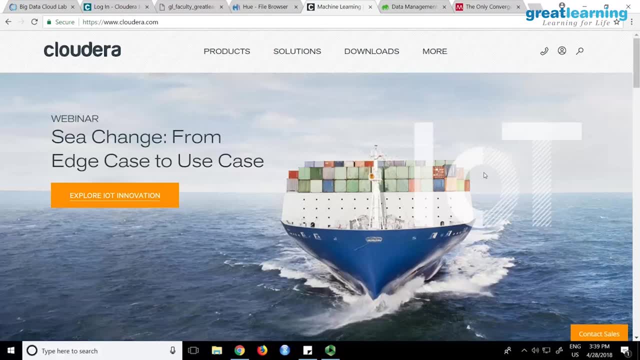 Hadoop may not be able to do. Hadoop is a batch processing system. It's not real time. So if I have Teradata or what is that- Exadata, Netiza, these guys are really fast. So what companies do? 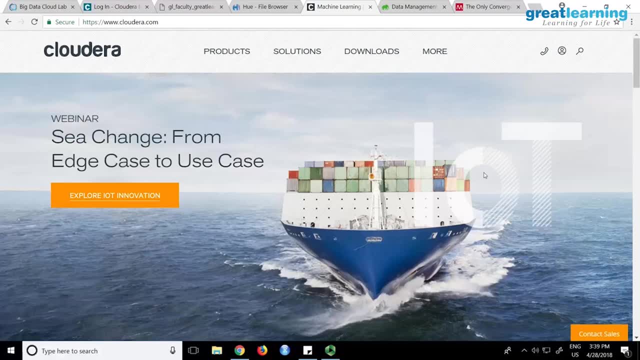 They keep the whole data there. Probably. my company has 100 terabyte data In that- 2 terabyte data I need every day. very fast, I'll keep it in Teradata. 98 terabyte. I'll dump it in Hadoop. 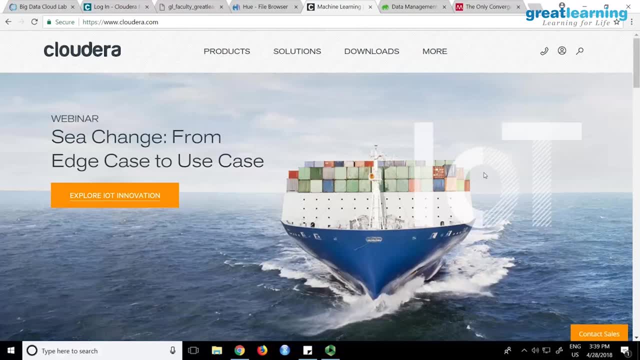 I need it once in a while and even if it takes some time, it is fine. Same story with the cloud. So most of the organizations are now deploying everything over Amazon Web Services, So Amazon offers fully managed Hadoop solutions on the cloud. 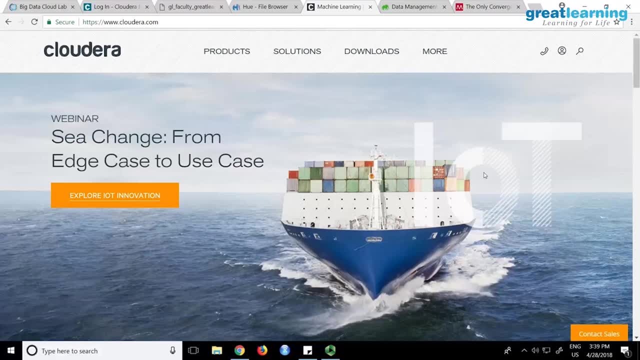 Like you can go to Amazon, ask it, Give me a Hadoop cluster. In 10 minutes you will have fully functional Hadoop solution, Everything installed up and running servers, everything automation right. So there, they also give you traditional data warehouses. 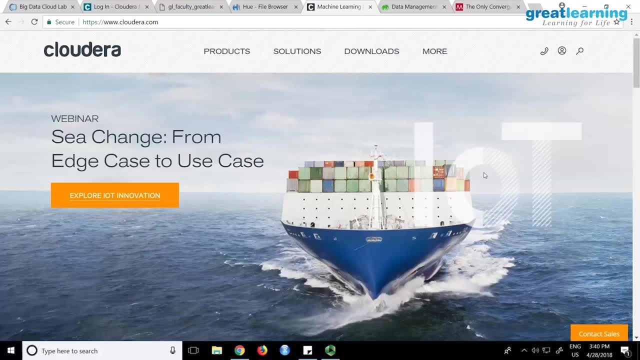 They have something called. there is a solution called Redshift. Redshift is an online cloud-based data warehouse, So Amazon offers Redshift to you if you want hot data to be installed. So, like I said, everything cannot be given in one solution. 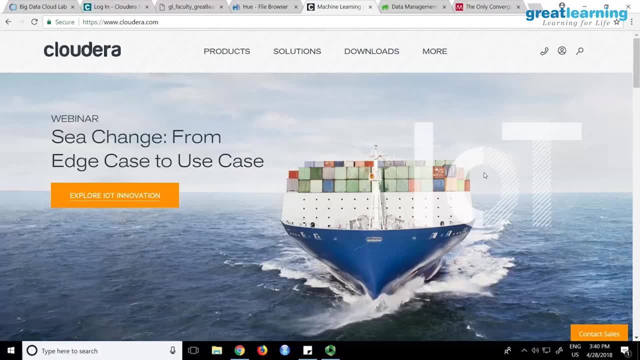 You need cheaper. You need the same speed. You know everything you have to package in one solution. You need the same speed. You know everything you have to package in one solution. It may not be possible, right? So like someone was suggesting, right. 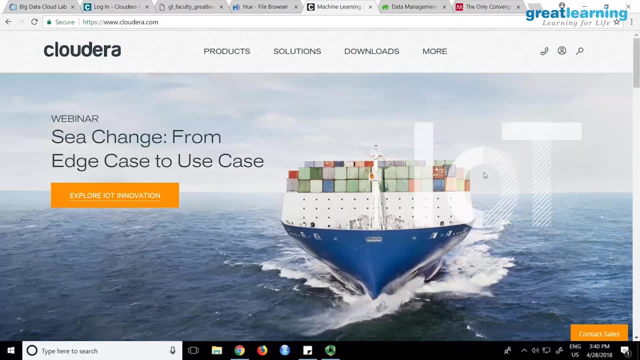 You can compromise speed, either right, or real-time access, right So same like that. So Hadoop is a solution most of the people adopt, but not everything can be guaranteed at the same time. That takes us to the question: what is Hadoop and why this is so popular, or what is the? 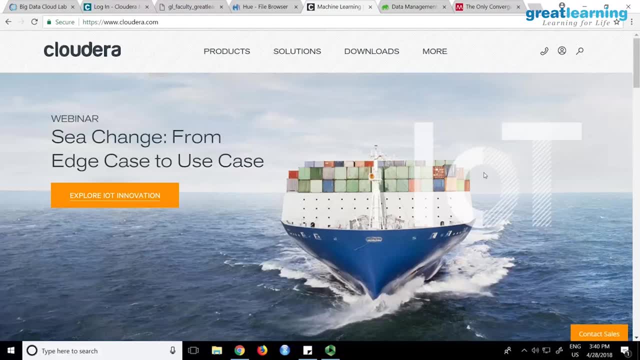 architecture of Hadoop. It's fairly easy to understand, actually, because the idea is very simple. I have a single machine. How much amount of data can I store in a single machine? Motherboard- right Motherboard- is who decides. So the motherboard will say: I'll support 10 hard disks. you can have 10 hard disks. 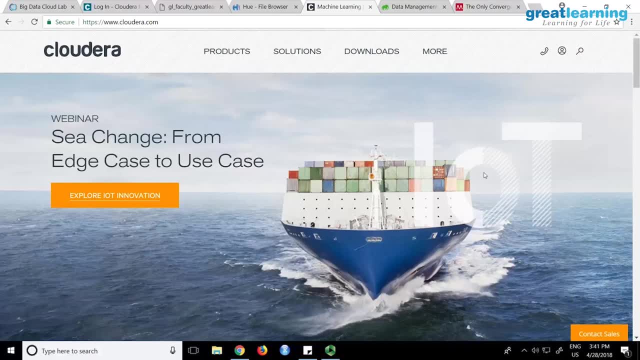 So the idea is very simple. So people initially thought I can use one machine, And when that machine was not sufficient, what they did? external storage, NAS and all right Network storage. Probably you guys are not much from storage background. 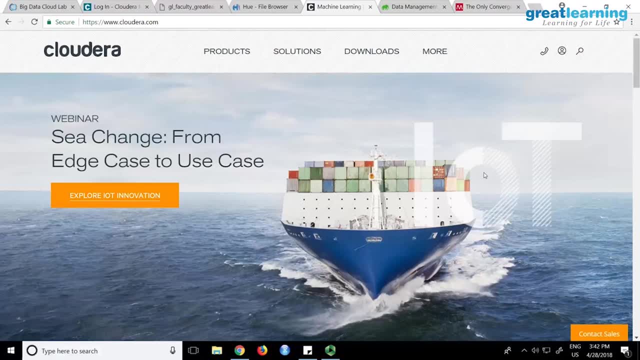 There was something called network attached storage very, very popular. Have you heard about EMC and all A company called EMC Square? They survived only because of these things. So you have something called network attached storage NAS box. You can buy a box, install the box anywhere and you can dump the data there. 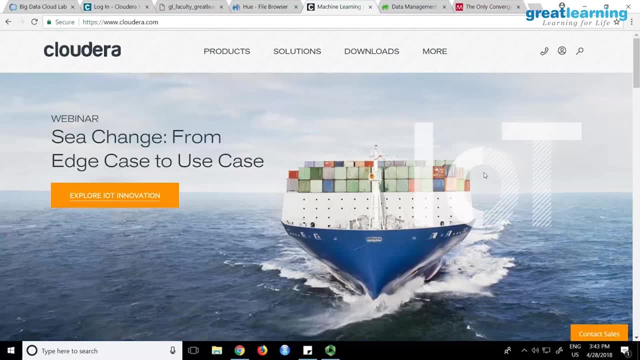 So the system can dump and process from there. That is called NAS, So that will support more storage actually, but it is not within the machine. When NAS was not enough came SAN storage area network SANs are even popular these days. 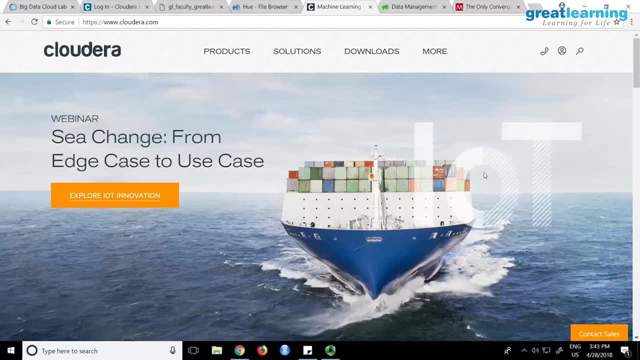 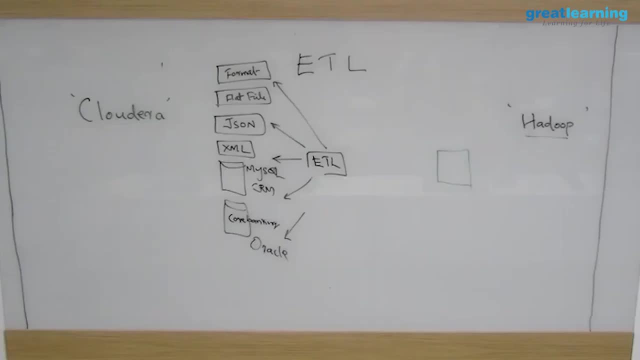 So a full room full of hard disks. you will get a fiber channel connection. So if I can dump all the hard disk there, I can store as much as I want. But the problem is, even if I'm using a SAN, this gives me unlimited storage. 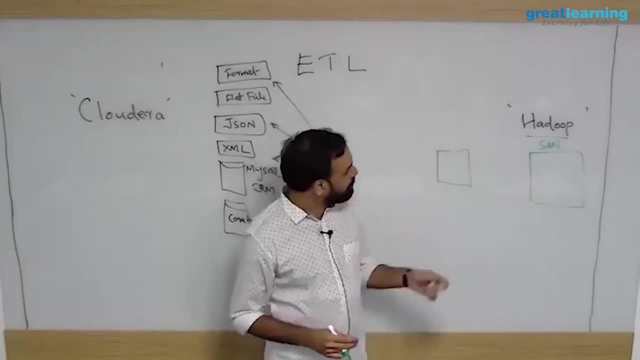 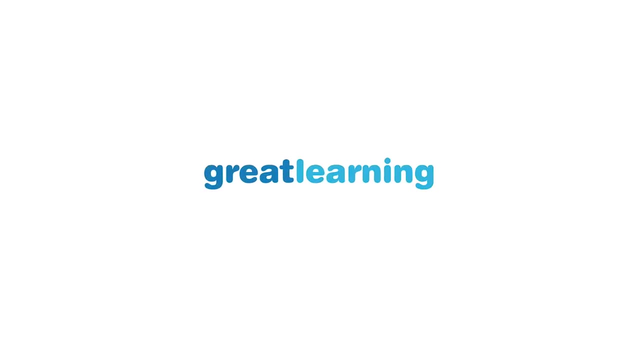 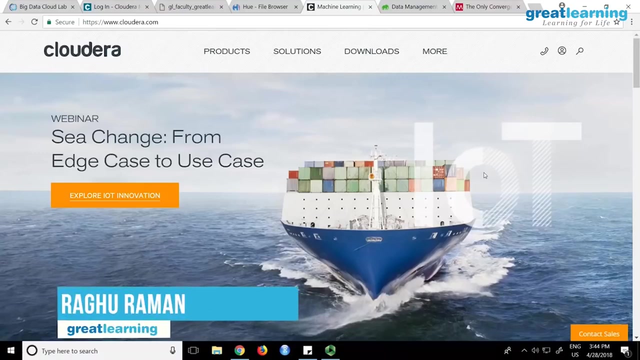 Problem is it gives me only storage, no processing. If I want to process the data, can one server process all the data in a SAN? No, not possible, right? Distributed computing is not a new idea. Yeah, It's already there. 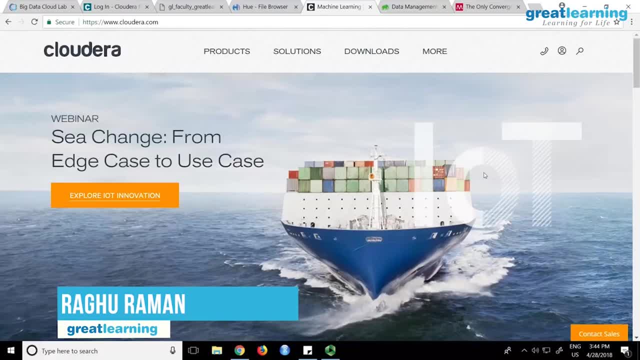 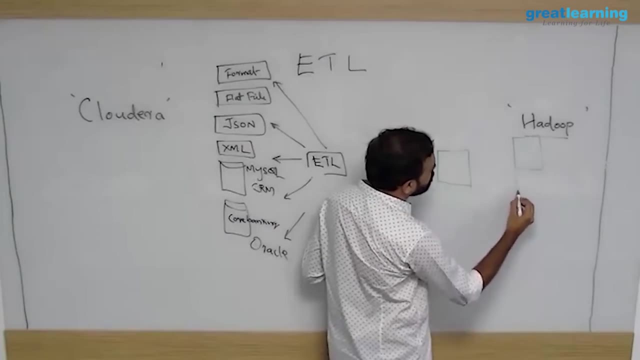 So in Hadoop what we are doing is very, very simple: Rather than one machine, you take a bunch of machines. So I will say the bunch is, just for sake of argument, four. So I take four machines: One, two, three, four. 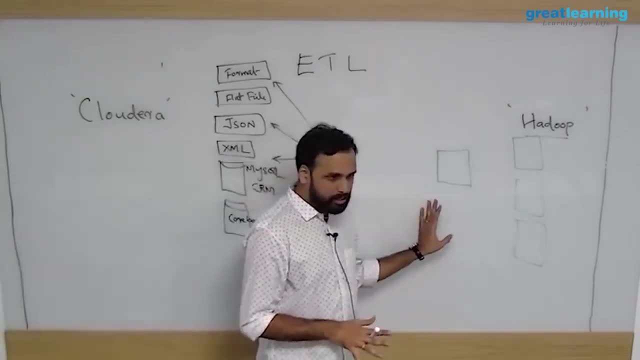 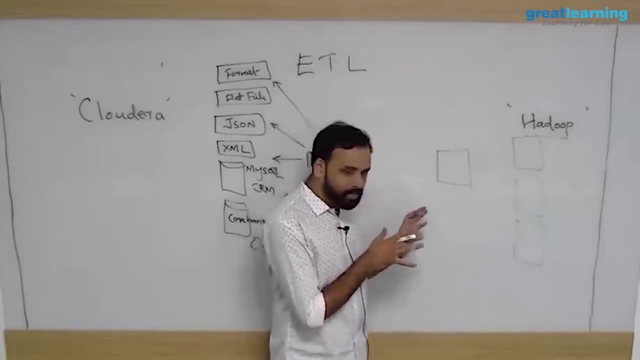 So I take a bunch of boxes, say four boxes, four servers, And I can download and install this Cloudera or Hortonworks, any of their Hadoop on this. While installing, it will ask me which machine is master, which machine is slave? 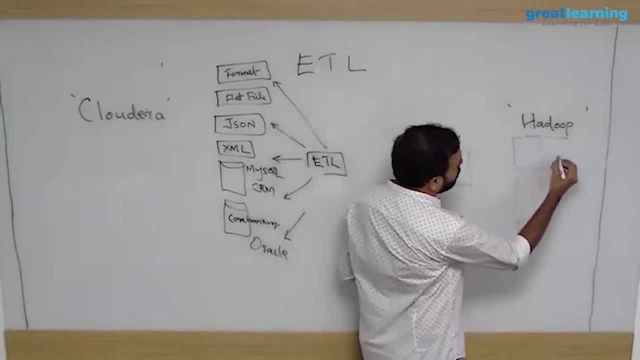 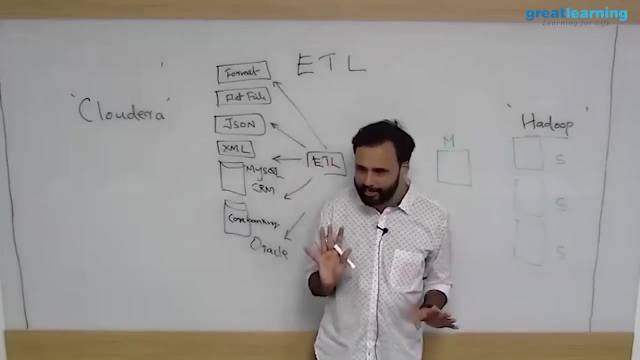 The idea is: one machine has to be master, the rest of them can be slaves. So in this architecture I come up with an idea: one guy is master and three guys are slaves. Fine, So we have not discussed what is the master doing, what is the slave doing? that's later. 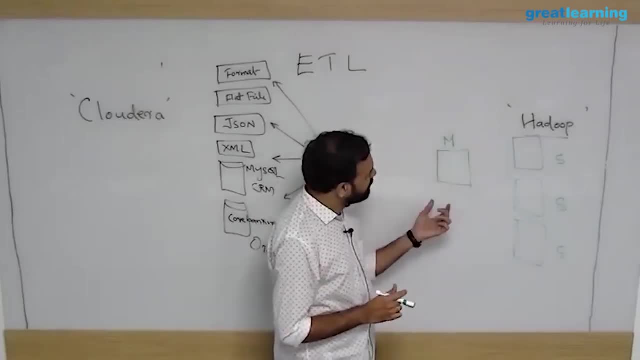 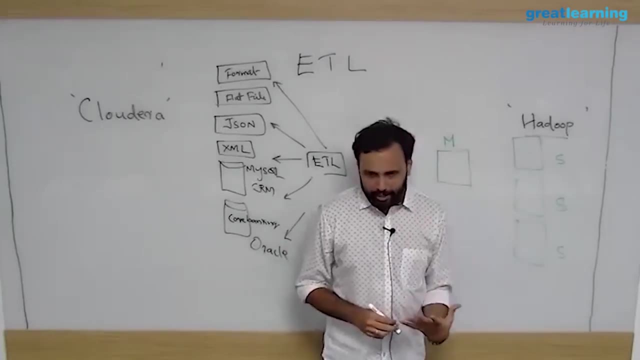 Okay, Okay. So in Hadoop, in a setup when there is one master and, let's say, three slaves right Now, the idea here is that if I want to store anything, okay, Hadoop will help me to store among these three boxes, right? 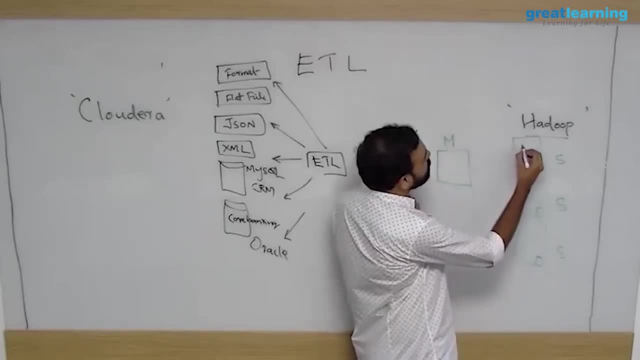 So I can use the storage space of all three boxes. So if each of them are having a two terabyte hard disk, I will get a total capacity of six terabyte. Yeah, So Hadoop is a framework. actually, It is not a software. 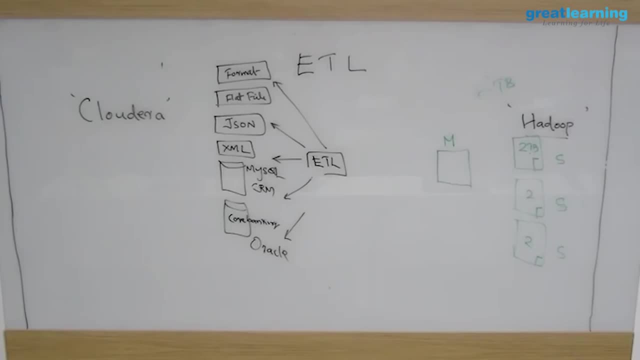 So one confusion people have is that is Hadoop a software? No, It is a platform. Okay, And I will show you the different, different components we have in the Hadoop platform. So if you install Hadoop, let's say we don't know anything about Hadoop. but let's say 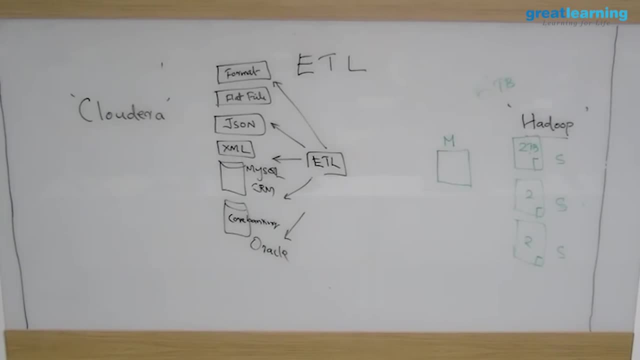 we install it in a four system setup. While installing it will ask you to select one as master, remaining as slave. So I have one master and three slaves, right, And what Hadoop can do? It can take the storage space of all these three machines. 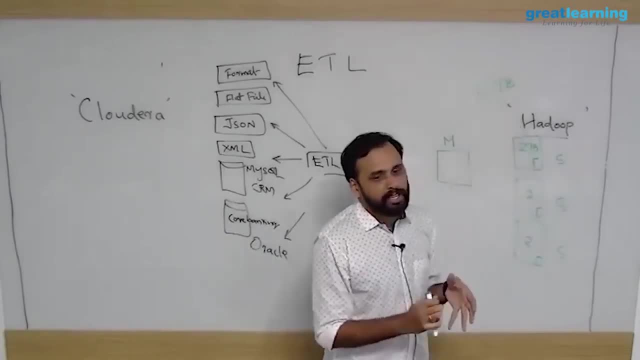 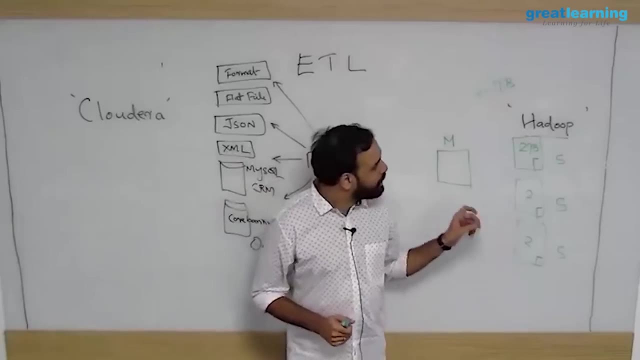 Enter these three machines and project it as a single six terabyte storage box, right? So the beauty of this architecture is that let's say you start dumping the data and the data gets stored here, And let's say your six terabyte is over. 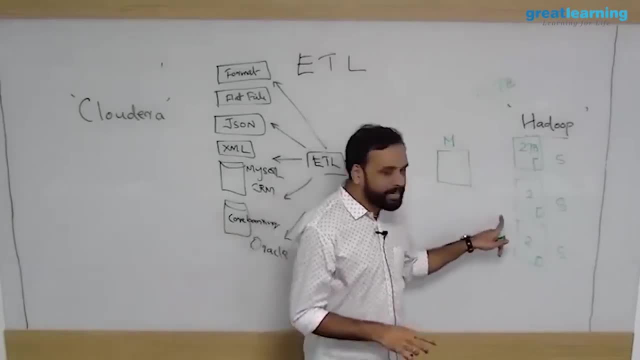 I can add machines on the fly. From three I can expand to 30,000 without shutting down the cluster, meaning your storage problem is solved. You don't have to ever worry about storage in a Hadoop cluster. Okay, Hadoop allows you resizing without any downtime. 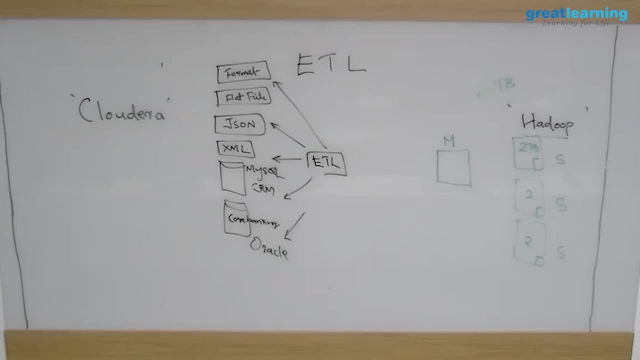 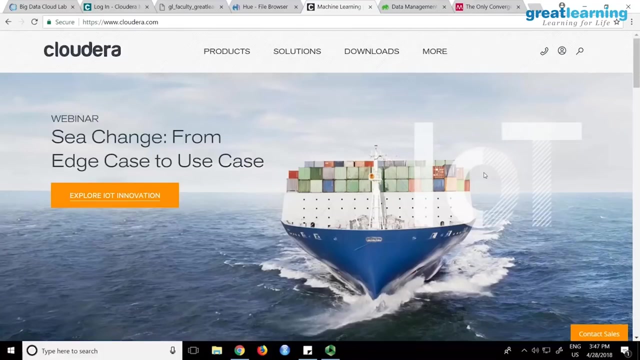 So I can add more machines or I can remove machines. up to me to decide right. But if you're removing, it will have a problem. For example, if the program is running here. if I remove it, the program might crash because 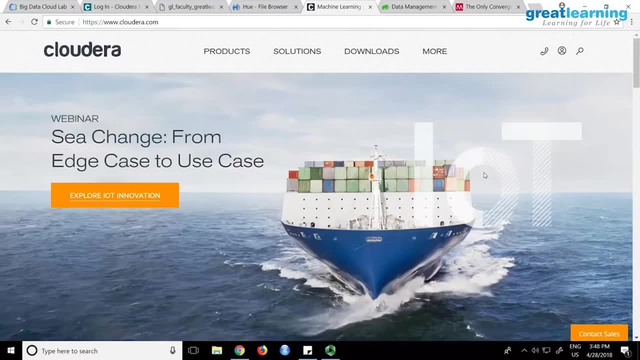 this machine is needed. That is not the idea. If you have one more machine here where nothing is running, I can remove it gracefully. Nothing will happen, So you are getting something called scaling out. This architecture is called scaling out, meaning you keep on adding more machines so that the 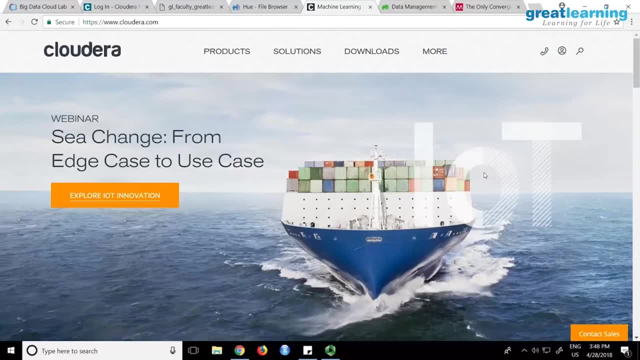 you know you can get unlimited scalability. Now I will tell you how storage happens. So far I did not discuss how storage happens, And if one machine is taking that, it will have more data, another will have less data. I don't have any way to manage it. 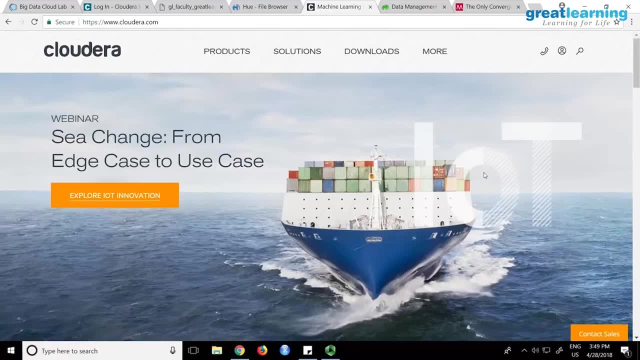 Here that will be handled. I'll show you how that is happening. So this is called a Hadoop cluster. So the technical term for this is a cluster. Cluster is nothing but a group of machines, right? So that is available in a Hadoop cluster. 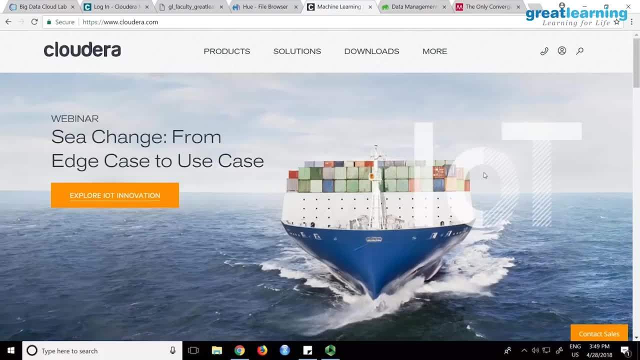 Now, typically if you go to companies, you will see a Hadoop cluster. Okay, So if you go to companies and check with them, like I was with this 24 bar 7, a company called 24 bar 7, they are called center company and they run Hadoop clusters for analytics. 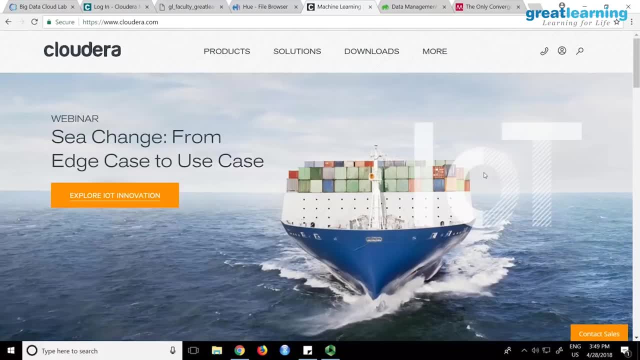 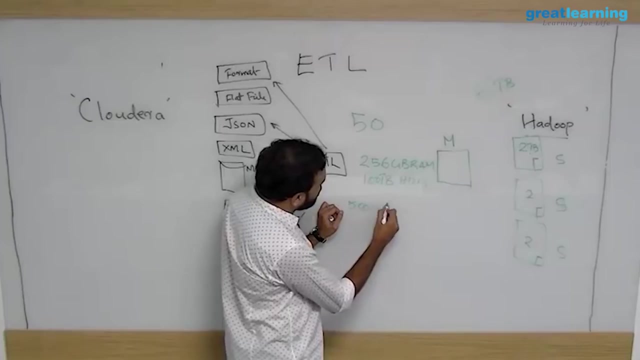 and all They had a 50 machine cluster, 50 node cluster. Each node has around 256 GB RAM and 10 terabyte storage. So 50 into 10 is what 5 petabyte of storage they had, and 256 times 50, that is the RAM capacity of the cluster. That is a very minimal Hadoop cluster, cheap Hadoop cluster. So typically you'll have 500 nodes, 1000 nodes Hadoop clusters, Because the amount of data you're storing is in petabytes. 1000 terabyte is 1 petabyte. 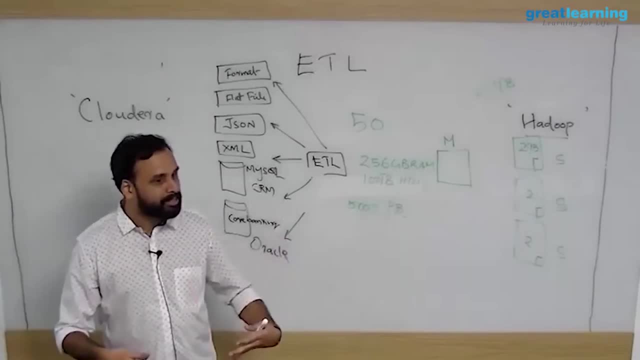 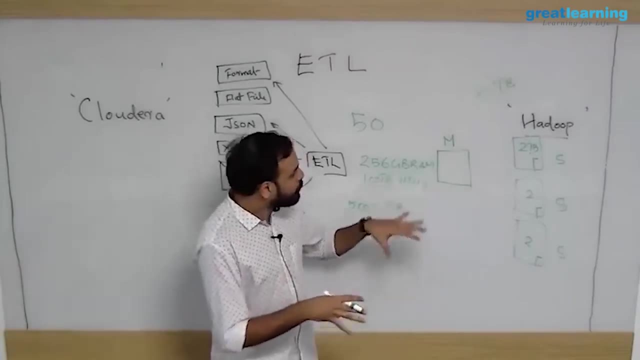 actually So most of the companies. they'll have huge amount of data to dump in this, So the size of the cluster will be in that. That is the Hadoop cluster, And Hadoop is distributed, meaning if you install it it is not getting installed in. 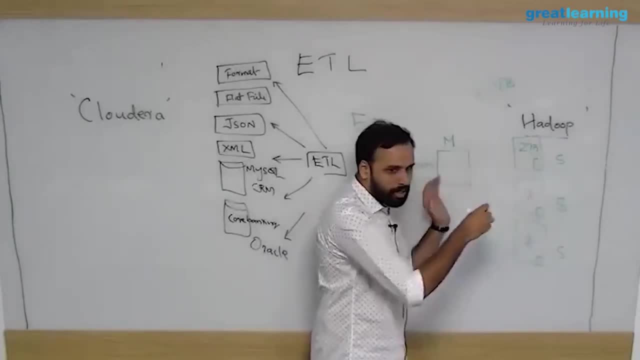 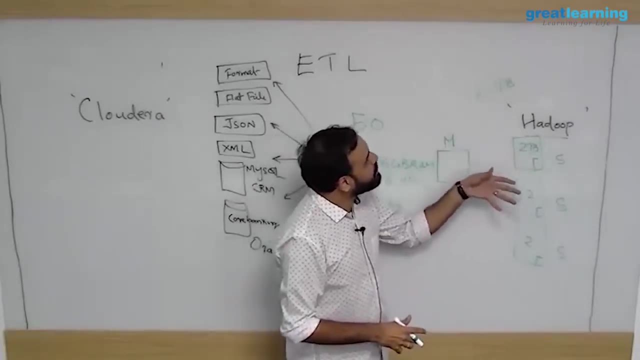 one machine. It is installed in all the machines and the components will talk, So it runs in a cluster, not in a single machine or two machines actually. So the basic idea in storage is that you can add more machines and get more storage. 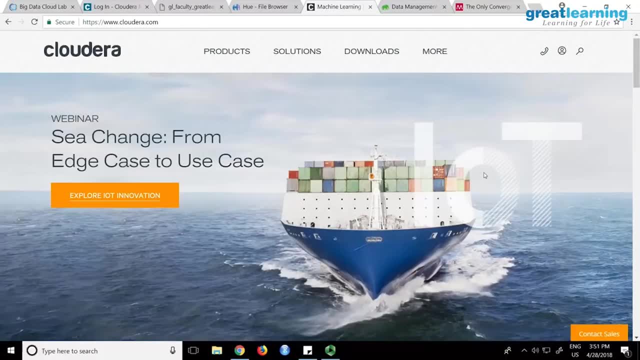 My point is: if, let's say, you're buying 500 servers, each server will cost you some money. So if I say 500 times that money, It is really a huge amount of investment for me. That is the reason we call these machines commodity hardware. 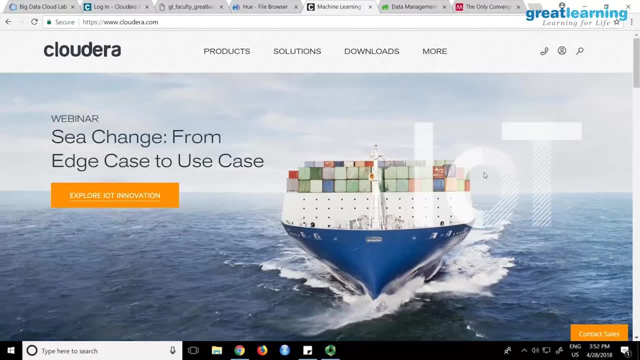 What do you mean by commodity hardware? Commodity hardware means any machine without any label. You will never buy a Dell server to build a Hadoop cluster. You will build it with cheap, throwaway servers. If you look at most of the buses that are here, what is your idea? 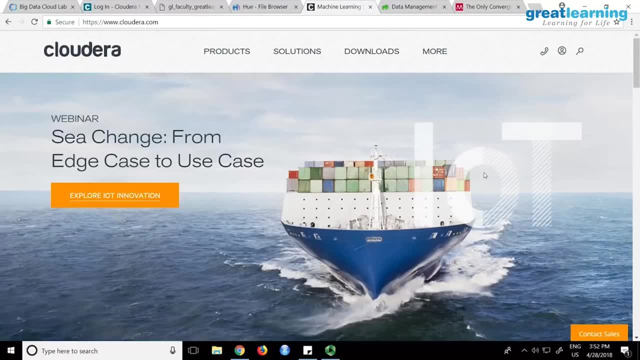 Citizens need to travel from one point to another point. So what is your idea? Another point, And the bus should be there. That's all. You are not investing crores in buying Volvo buses everywhere. You buy just some buses. Same idea here. 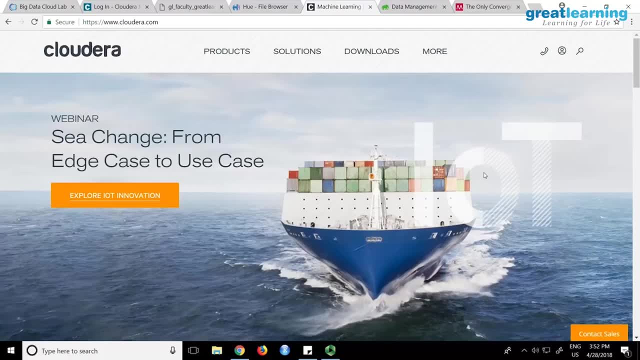 In a Hadoop cluster- typical Hadoop cluster- the machines that we use are called commodity hardware. Commodity hardware means assembled servers, So you can get it actually. So you're not actually buying an IBM server, because I was also working as a design architect. 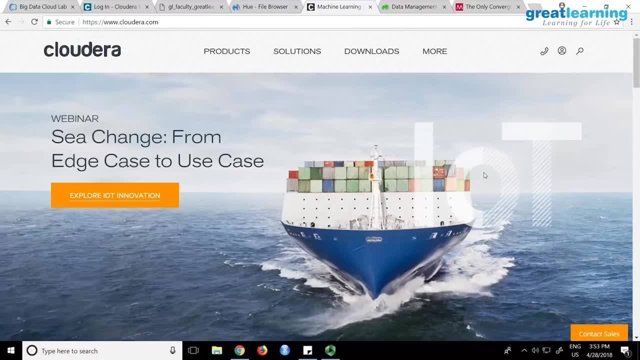 for one of the Hadoop solutions. There we got servers for around 35,000 rupees, 40,000 rupees, 40,000 rupees. You cannot buy a server. If it is an IBM server. you'll pay 2 lakh, 3 lakh. 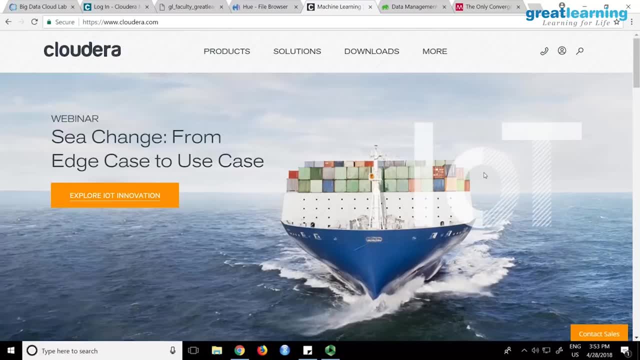 So this was like somebody will assemble and give you The only thing. it will work. it will crash. also, It will definitely crash 100%. So then you will be thinking, if I'm having a 500 node Hadoop cluster, if my slaves are? 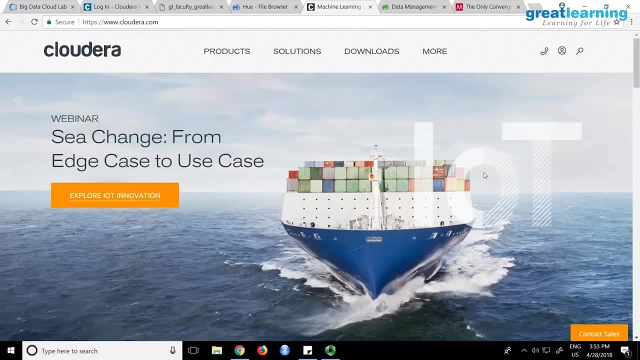 crashing. what is the reliability there? I will answer that question, Just just part the question for the time being: Server is what A server is. So this is your desktop, Normal desktop, right? So normally you have something called desktop at home and all. 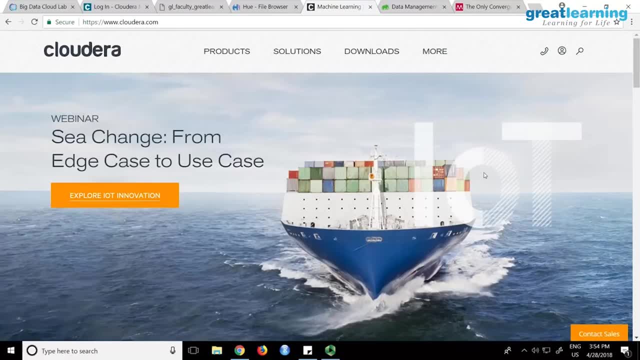 Server is something which can serve multiple clients in one way. It is a bigger box with bigger storage and processing. So if I want to buy a server, I have multiple options. One is that I go and tell IBM or Dell: buy me a server. 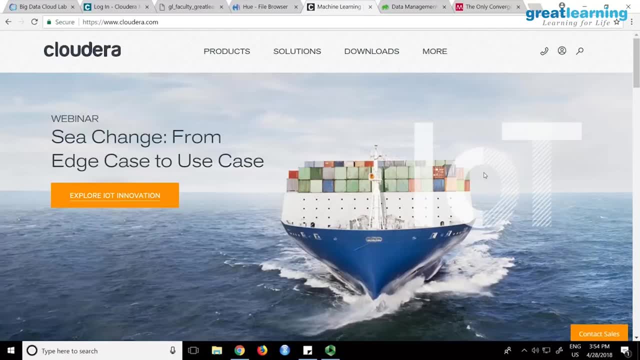 So they will give me a branded server, So they will charge a lot of money. They will also give me support and all, but I have to pay 2 lakh, 3 lakh for a server. So normally when I say server, this is what people buy. 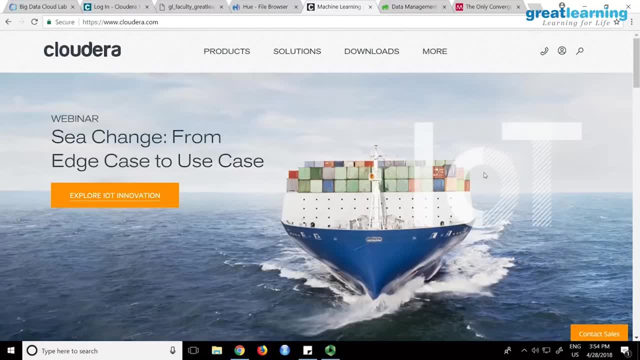 But in a Hadoop cluster you never do that. You buy The cheapest servers possible because you can afford to have failures in a Hadoop cluster. I'll show you how failures will be handled in Hadoop cluster, but you are not investing. 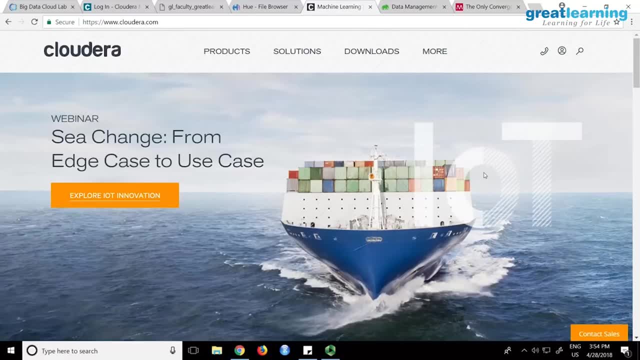 a lot of money on the hardware. That is the idea, because otherwise the solution is not feasible. If I'm buying 500 IBM servers, I can take the same money and give it to Teradata. So as good as same thing, right. 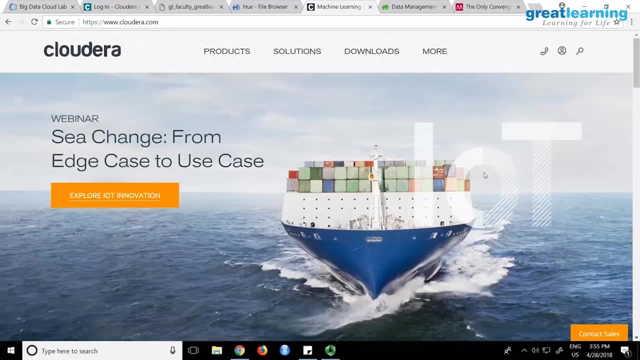 So I don't need support or anything. I just need some normal machines, and Hadoop also does not say what kind of a machine you need. You can even build a Hadoop cluster using desktops if you want- Performance will be less, but it will beautifully work- or laptops or anything that you want. 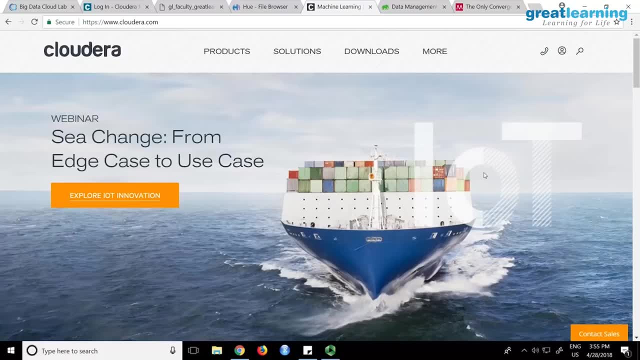 It doesn't say that. So new businesses might take Hadoop more, because after 5 years I may not buy Teradata, right? If this is the situation, I might buy a Hadoop solution probably. Data warehousing is a new, not a new concept. 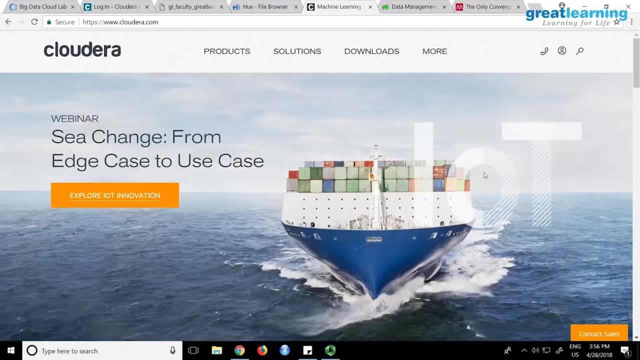 If I go to the market, I can get n number of people who know what is data warehousing and they can easily install a Teradata Teradata for me. I just have to pay money. Building a team of Hadoop expertise is not easy. 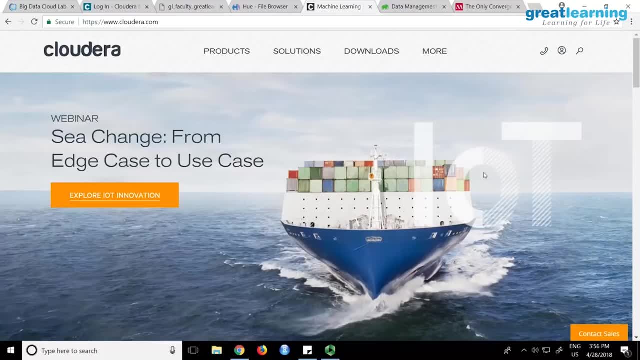 That is why you're sitting here right- I go to a company. also, If all of them have to understand how Hadoop is working- and Hadoop is not like click-click install. There are a lot of things you have to configure and tune. 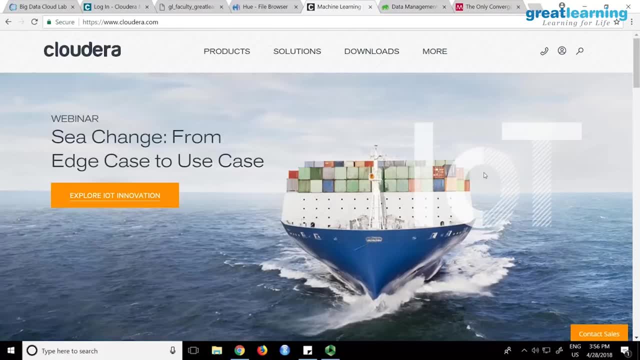 So people don't want to spend that much of a risk. So one reason is that the knowledge curve- we call right The learning curve- is a bit high. You can't learn it in a day and say, okay, I'll implement Hadoop. 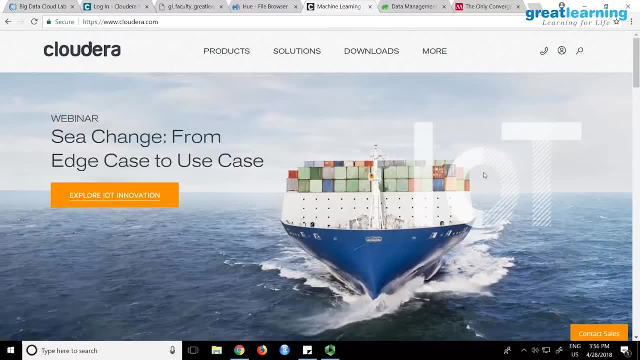 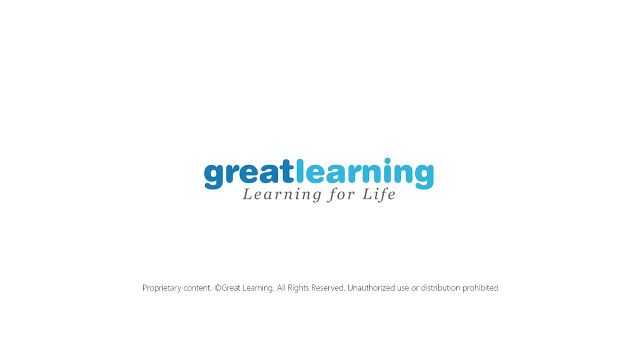 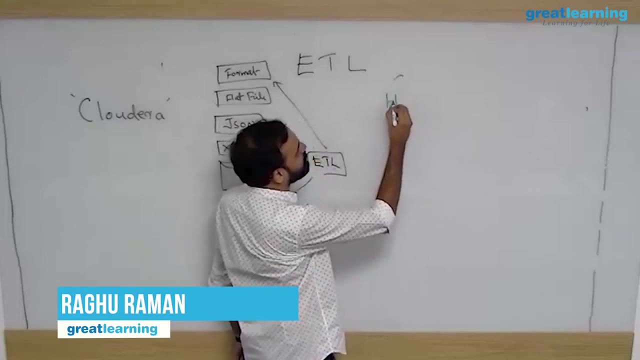 It's not possible, right? So most of the companies are stuck in this position, Right? They're stuck in this position. Now what you need to understand. so, since we were looking at the high-level definitions, only Hadoop has three major components. 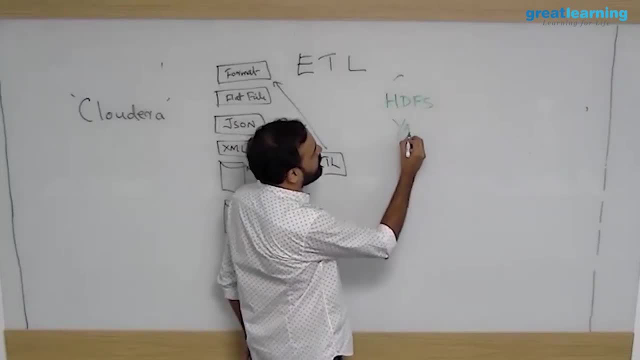 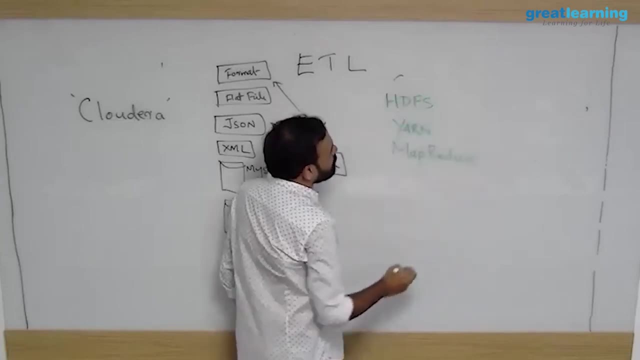 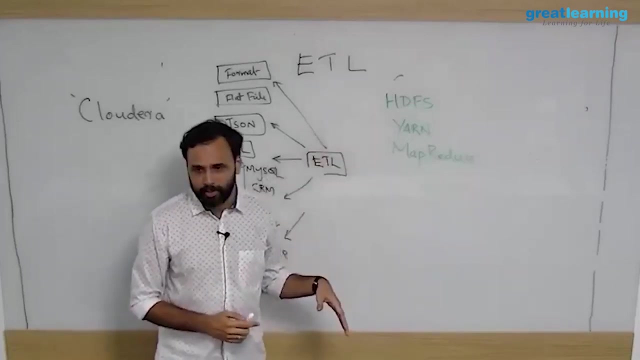 There is something called HDFS. there is something called YARN. third is called MapReduce. So when you download and install Hadoop, only Hadoop. these three things will come by default: HDFS, YARN and MapReduce. These three components will be installed by default and you don't have to do anything. 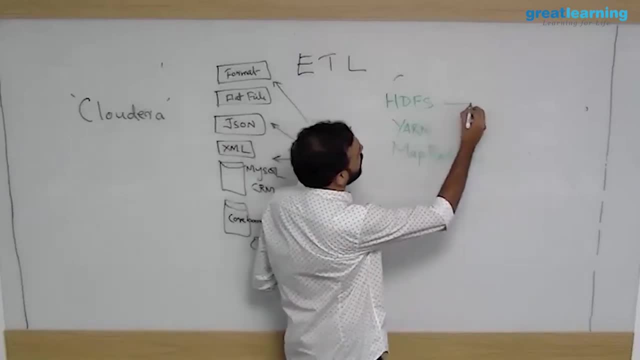 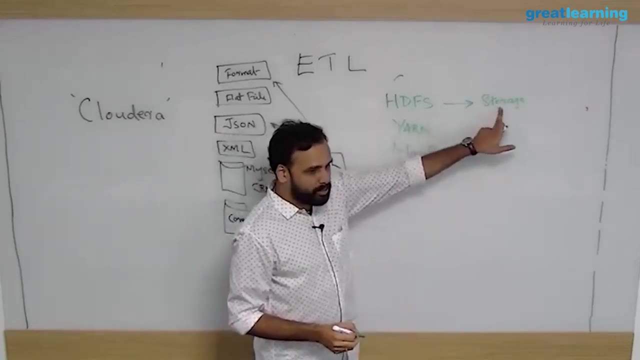 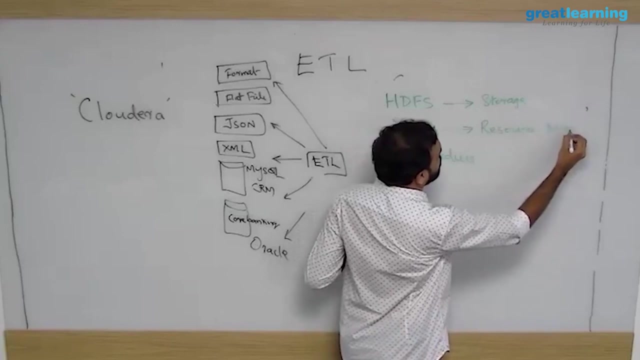 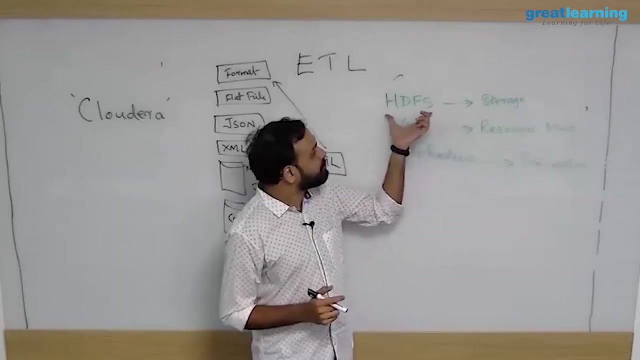 They will get installed right In this. this guy is the storage. This guy is handling storage. okay, This guy is resource management. This is the resource manager. This is processing HDFS. HDFS stands for Hadoop, Distributed File System. 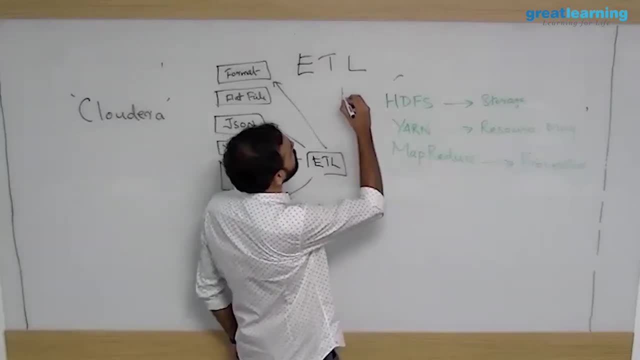 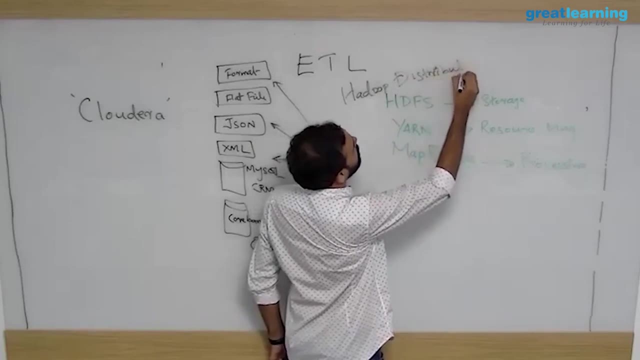 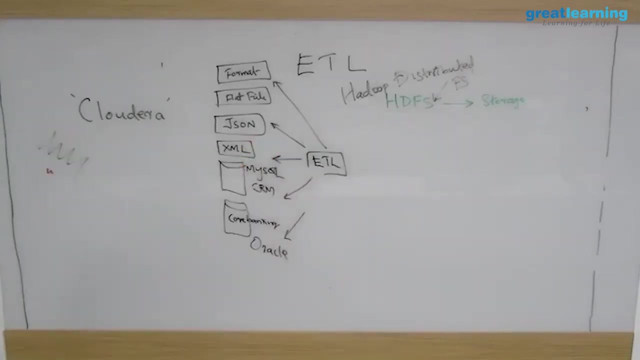 It's a file system actually. It is called Hadoop Distributed File System. I'll write it here probably: Hadoop Distributed File System. That is HDFS. First let's look at this guy called HDFS. So let's take a hypothetical situation where you have installed Hadoop in one master. 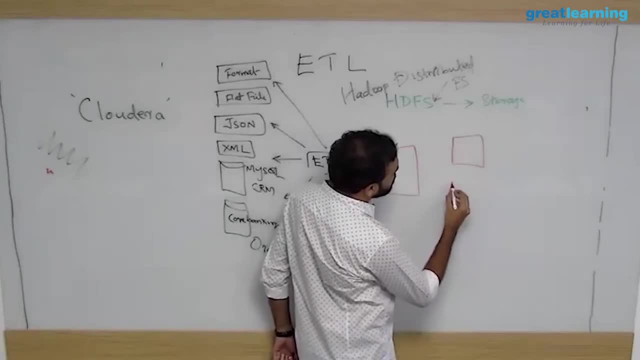 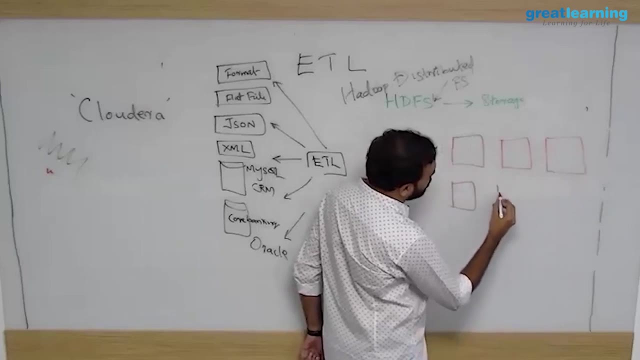 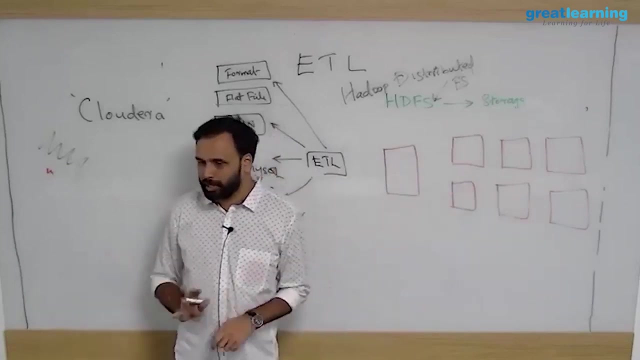 Okay, And in my example we have six slave machines. Now this picture will pose a lot of questions. usually okay And that's okay. So there is one master and six slave machines And we are talking only about storage, not processing. 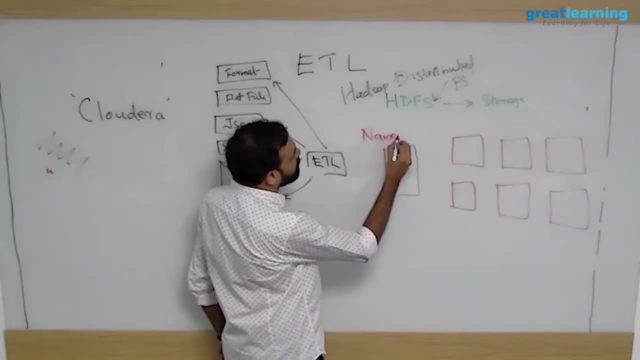 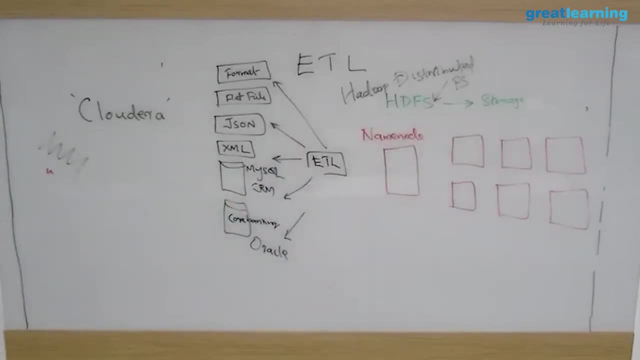 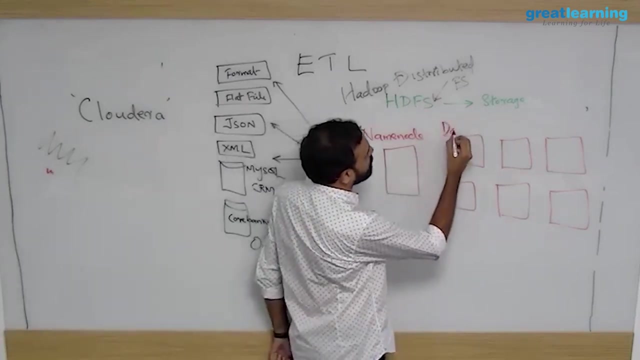 The master will have a process called name node. The master machine will be running a process called a name node. When you install it, it will start running This process called name node. Okay, The slaves will be running a process called data node. 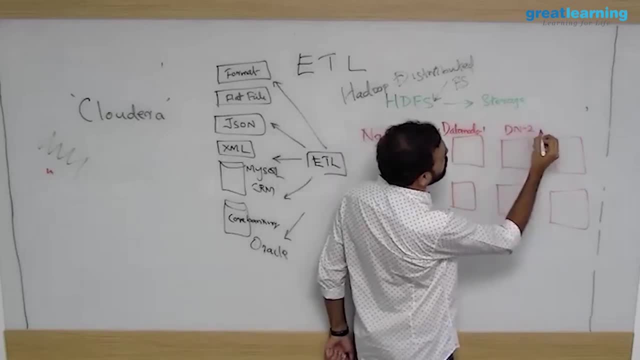 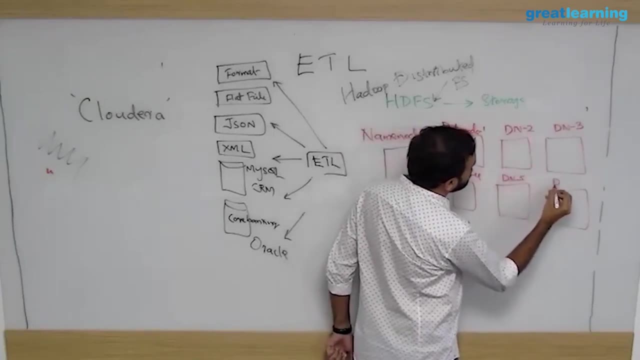 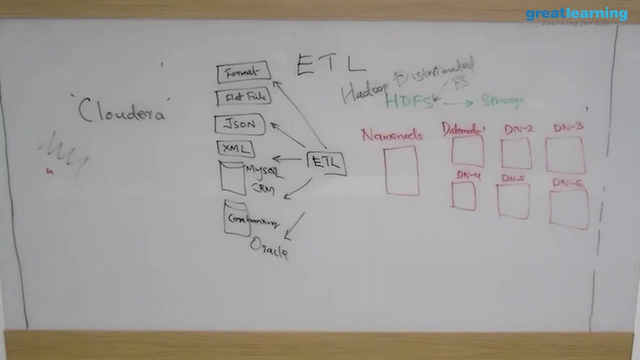 Data node. So I'll call it as data node 1,, 2,, 3,, 4,, 5 and 6.. So technically we will say that there is one name node and six data nodes. I mean that is how you say in a Hadoop cluster. 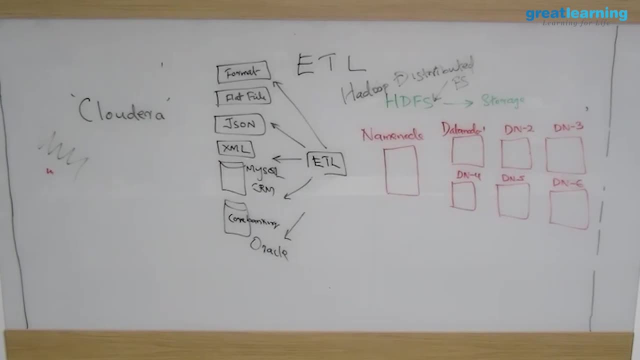 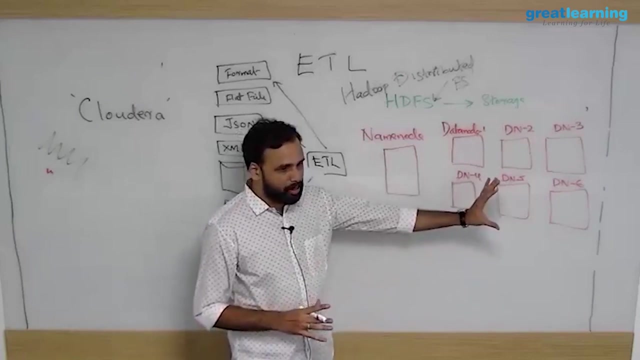 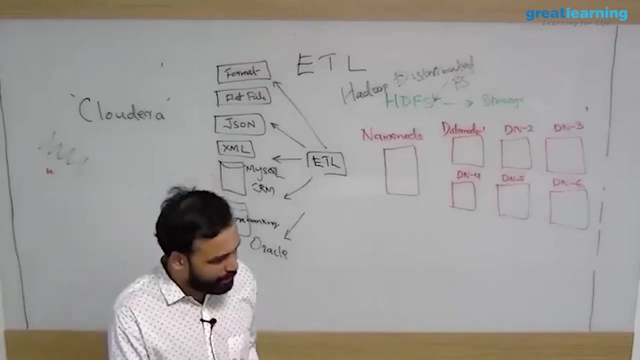 Okay, So name node is the storage master and data node is the storage slave. The next thing is that let's say you want to store a file in a Hadoop cluster. Hadoop does not care what you are storing, Meaning you can store any format. 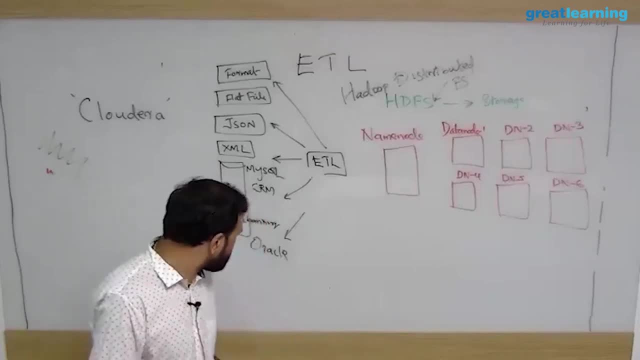 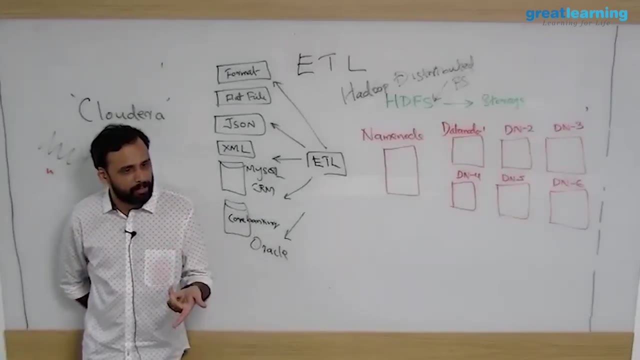 Can be XML, JSON, images, video. Hadoop doesn't really care what format of data you are storing. While processing you have to make sense of the data. So that is in MapReduce. If I store a text file, I have to write it in MapReduce. that read this text file and 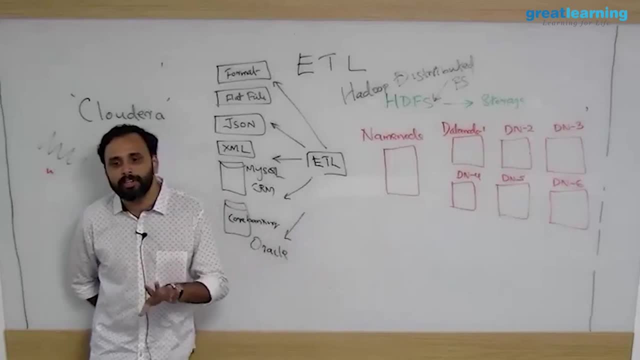 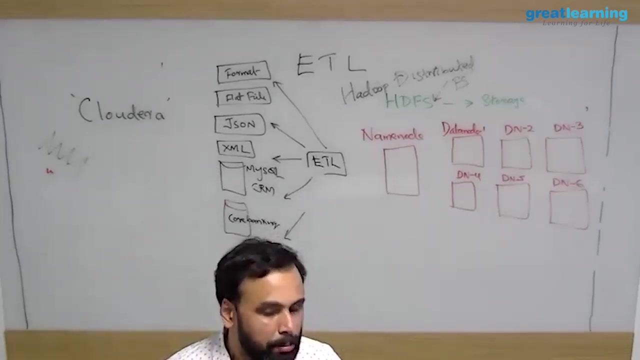 do whatever I want to do. The HDFS file system does not really bother about what type of data you are storing. Second point, and probably the most important point, is that once you store any file, you cannot edit it. Modifications are not possible. 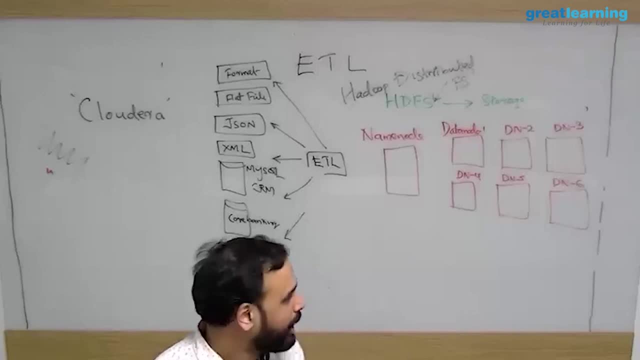 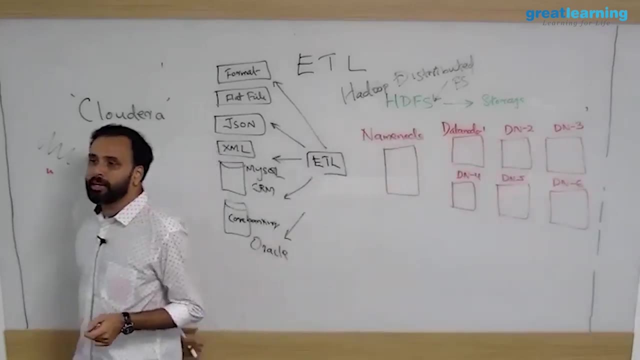 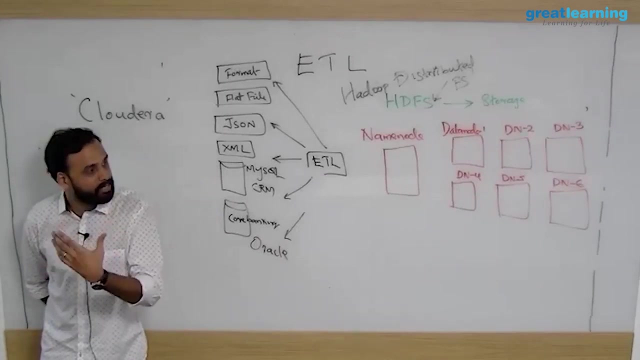 You store it, delete it. that's it. In HDFS, Modification is impossible. So why you may be asking why it is not possible? Because HDFS is designed as a file system for handling huge amount of data: terabytes and petabytes amount of data right. 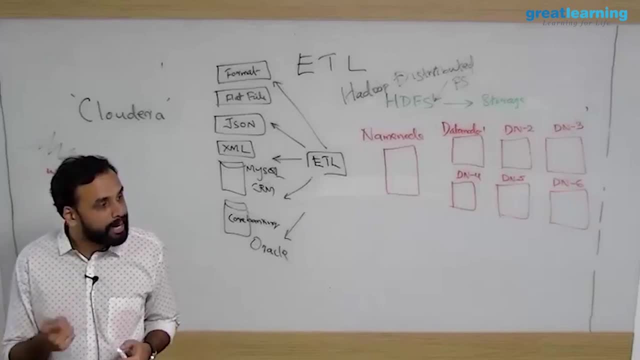 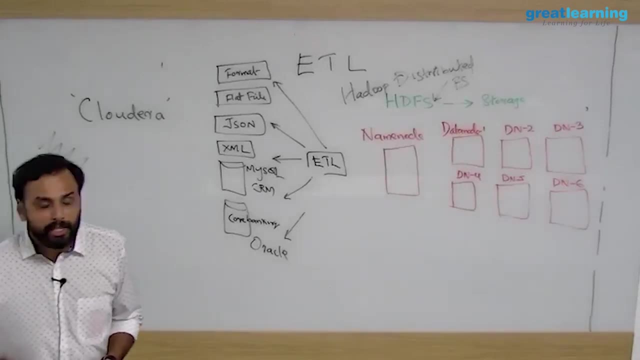 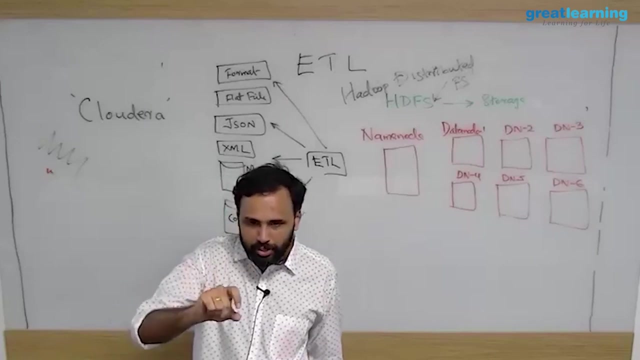 And if I want to modify or edit, you know row by row, like in a transaction, that is happening. you know it is not possible because if you look at a hard disk, right, there is something called seek time. If a hard disk wants to fetch a record, there is something called seek time, right? 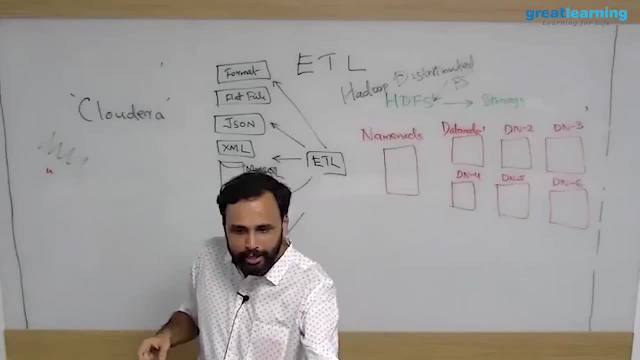 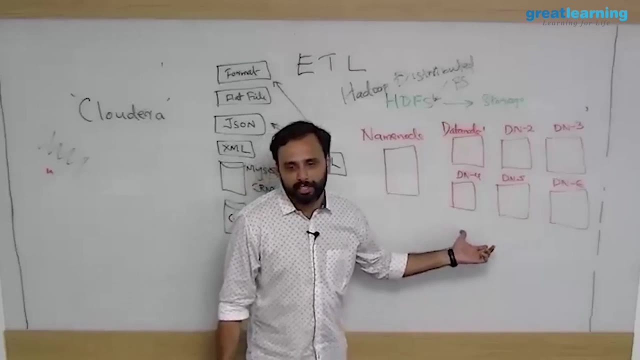 And if I am having one terabyte file, I want to edit the hundredth line. it is not possible for my hard disk to seek and get the data in that Because you are using all commodity machines here. They are not even faster. 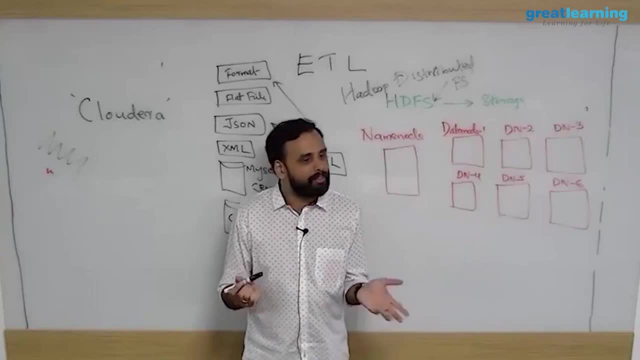 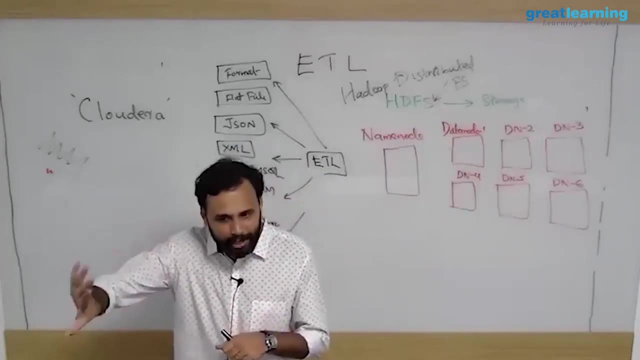 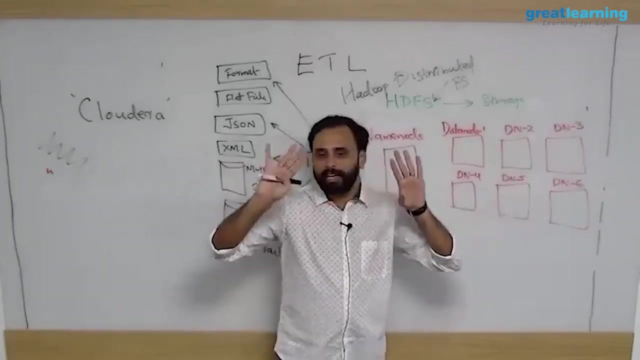 I am not using solid state drives or anything very commodity level hardware I am using here. So Hadoop's idea is that you want to read files sequentially. There is no time, There is no random access, There is only sequential access. So if I store a file, I can read the entire file and process it. 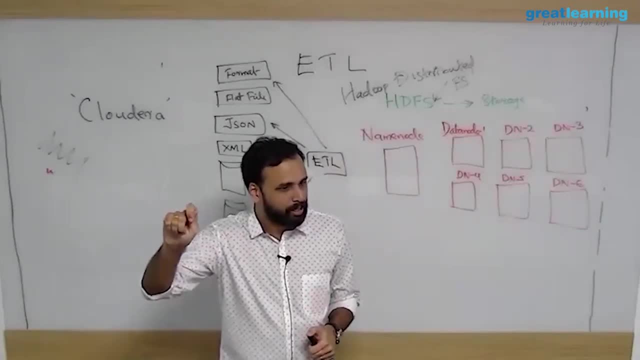 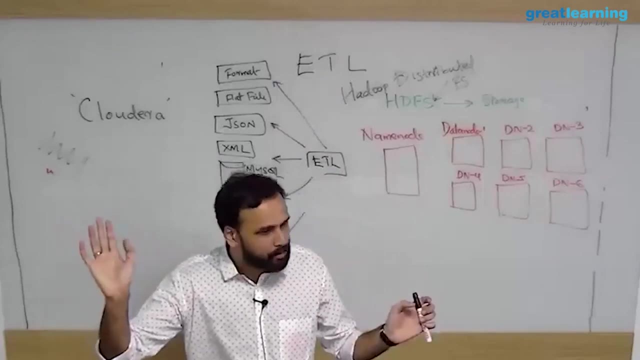 I cannot say needle in a haystack problem. Needle in a haystack problem meaning if you have a one million row table, you cannot say take the hundredth line and edit. not possible in Hadoop. at least in Hadoop it is impossible. 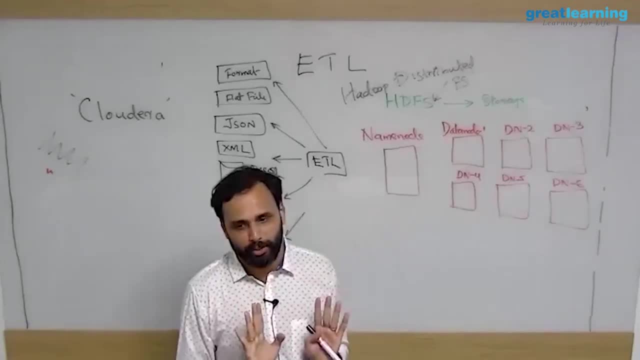 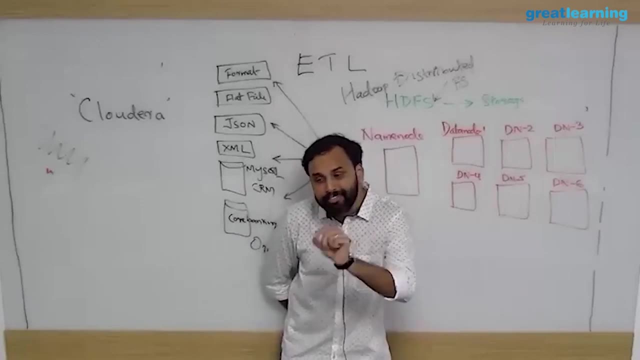 So either you can read the whole data and process it. that's all you can do, And the result can be stored. Obviously, if you process the data, you get some result that can be stored, But on the file system editing is not possible. 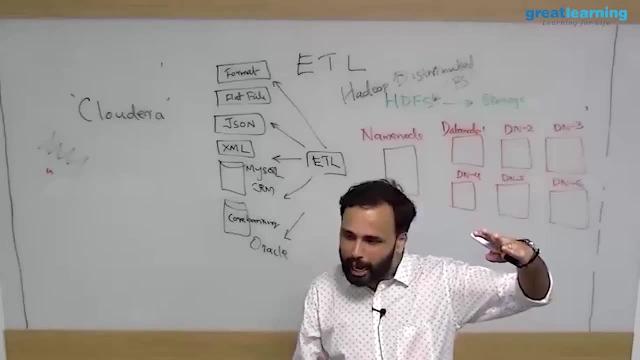 That is, appending is possible. Appending is always possible. I have a file. I want to append the data. That's okay because you are just adding in the end. But I'm just reading the hundredth row and edit. That is not possible. 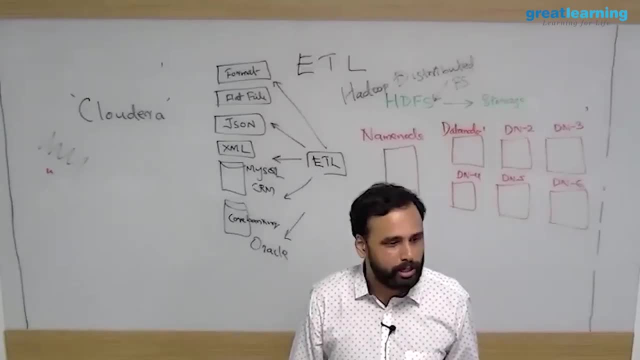 Now you may be wondering: what if I want to do it? There is a solution. You can do it. You have MPP engines on top of Hadoop which can do it. I'll show you how to do it. I mean, it is possible. 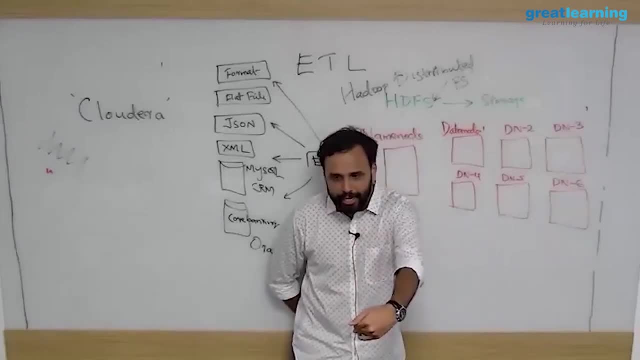 But considering only HDFS. Ideally, if you're storing a file, you can do it. You can do it, But if you're storing a file and you got some modifications in the file, you delete it and restore the file, meaning you don't edit it. actually, right. 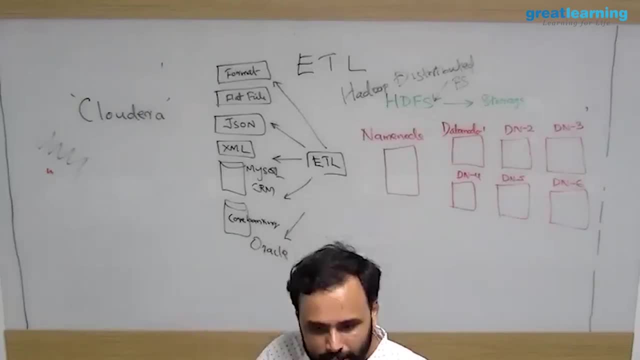 You can delete the whole file. Delete is possible. I'm saying that minute edits are not possible because Hadoop is considered to be a system where you are doing analysis of the data. It is not a transactional system. Where will your minute edits and all come? 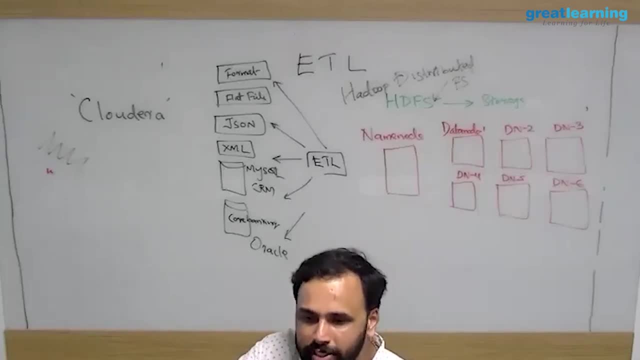 OLTP systems. If I'm having an RDBMS, I want to do insert, update, insert, update. It's not an RDBMS, right? If you're an RDBMS, It is possible. I don't have any objection. 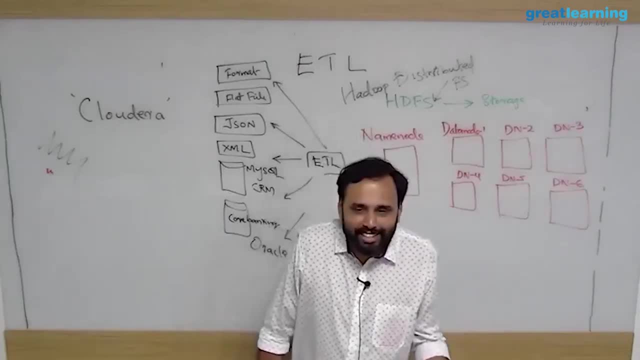 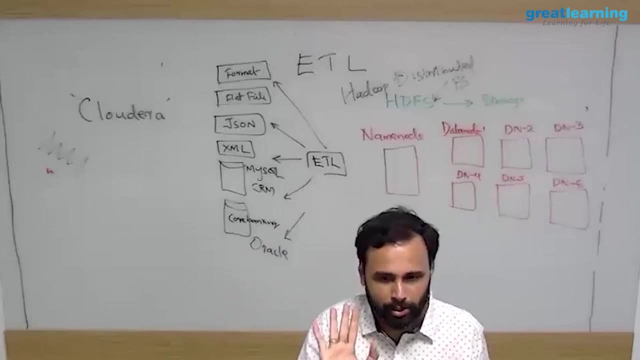 But here it is not possible by default, And also we are not doing any transactional. it's not a real time transactional DB, right. So I don't want to minutely edit also, But worst case, if I want to do it, it is possible. 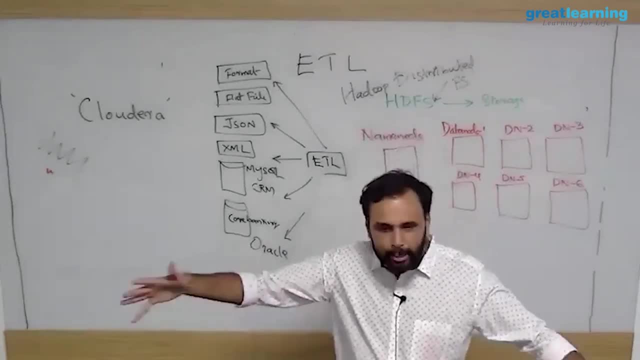 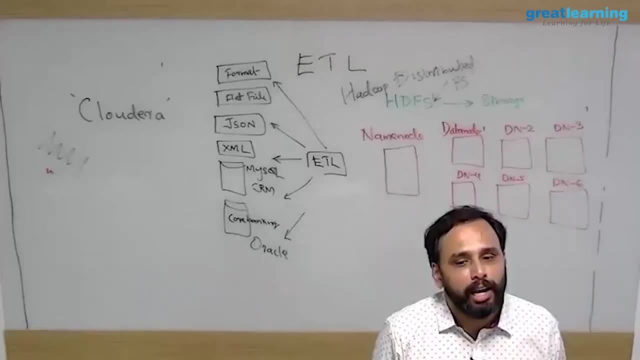 So we have MPP engines on Hadoop which can do it actually. So if I'm storing a 1TB file, if I want to process the file- probably I want to process only the 100th line- I have to load the 1TB into RAM. 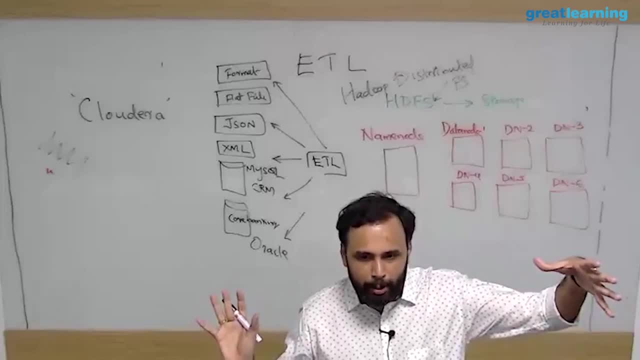 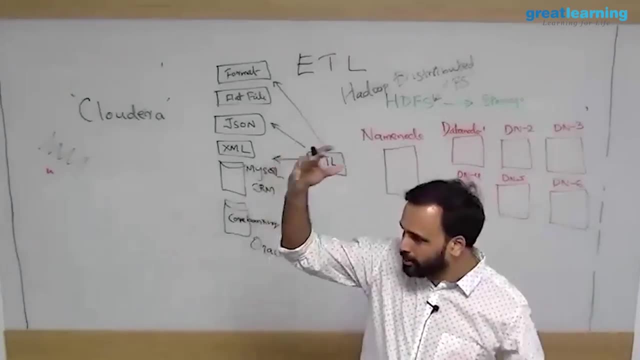 If I'm writing a group by query or an aggregate query right, Probably I need the whole data. I have a very big table. I'm writing an aggregate query right Which will say group by an order and something like that. 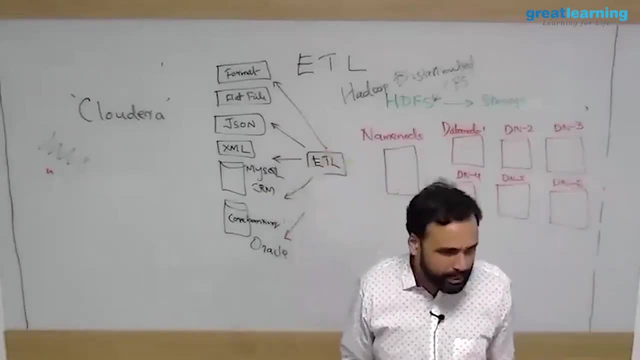 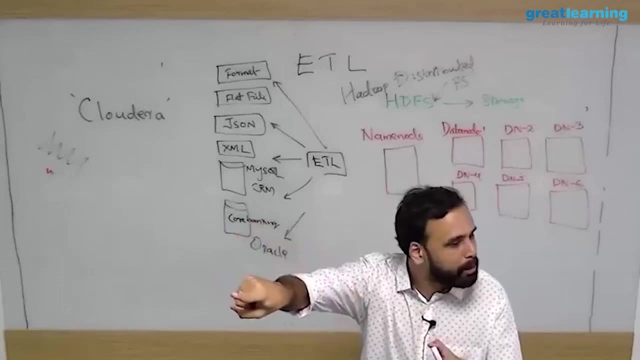 It makes sense. I load the full file because I don't know where is the data. whole data need to be scanned, probably. But if I'm doing a SELECT something, something where name equal to something, name equal to Raghuraman, only one line need to be processed. 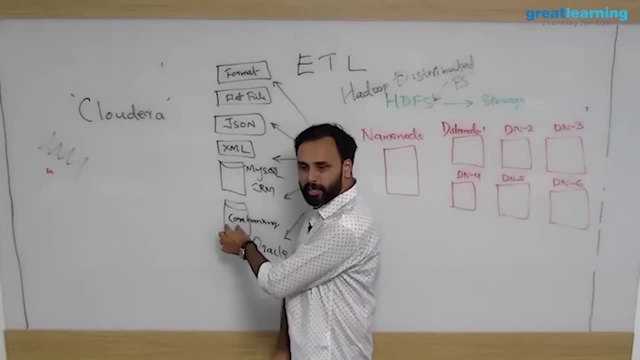 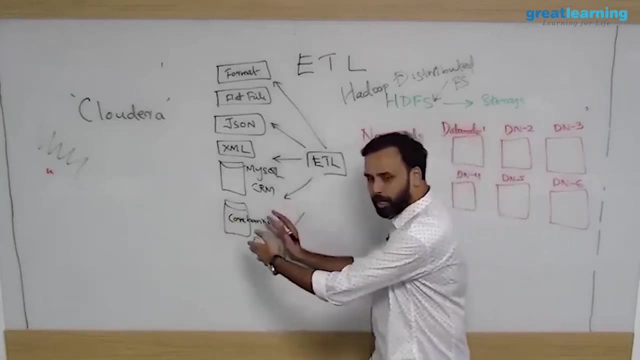 For processing only one line. why should I load the whole data? This is where customers are placing their order and this data you don't want to change. This data was created by customer. just want to get the data right, Probably. I want to modify and get it. 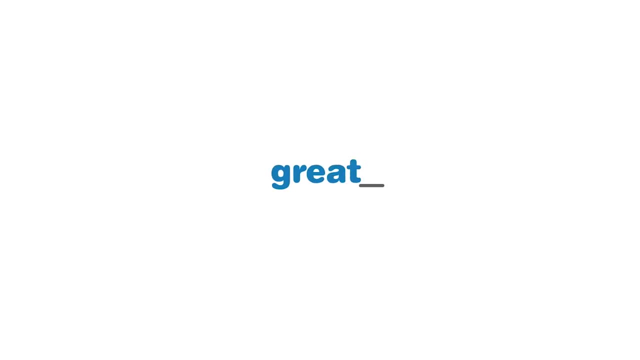 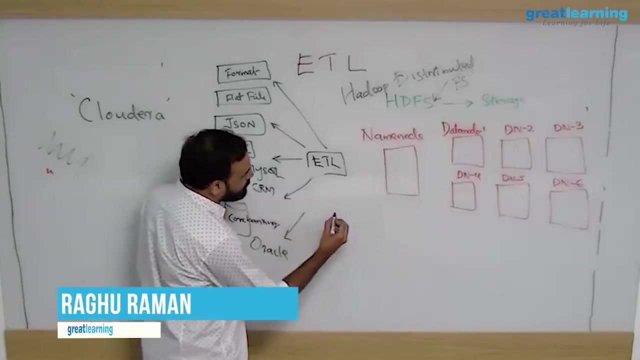 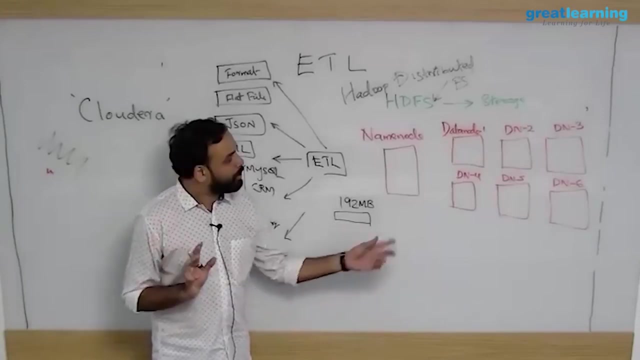 So once it is here, I don't want to make any changes, I just want to analyze the data. No, I'll tell you what is the role, What is going to happen? Let's say that you want to store, So file size is 192 megabytes. you want to store it in a Hadoop cluster. 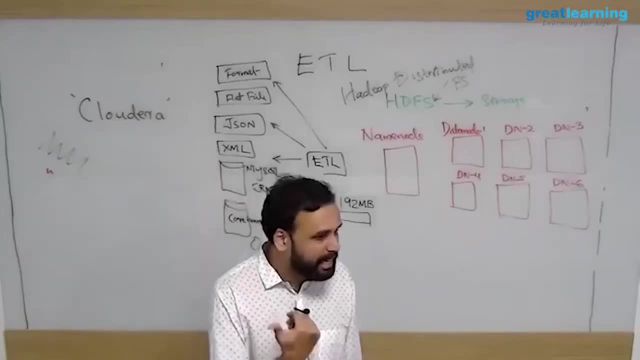 Now there are a lot of things which actually matters to your real time experience. Here we are just learning the basics, because in a real company, if you want to connect with a Hadoop cluster, the Hadoop cluster will be somewhere else. So if you are sitting here, the Hadoop cluster will be separate. you will be separate, right. 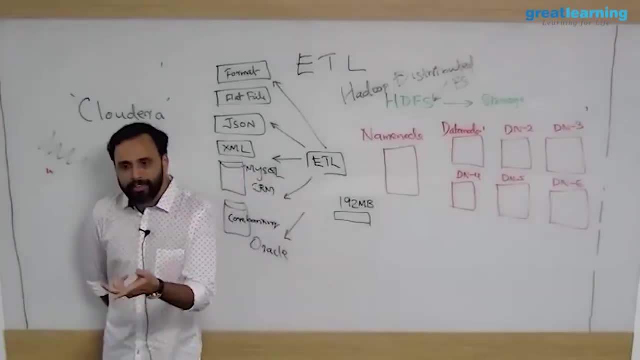 So you will get something called a Hadoop client package. So one way is that you get something called a Hadoop client. using that, you can access from your laptop. Second is that you can log into a node. there is something called a gateway machine. 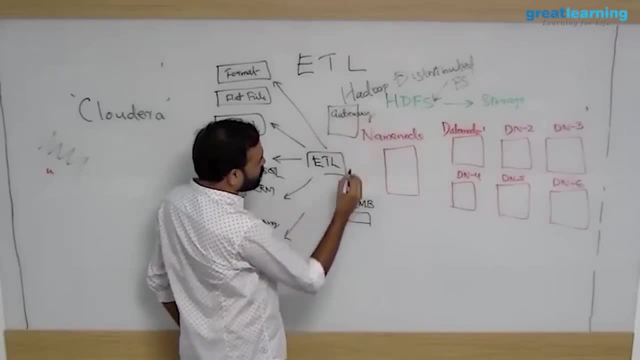 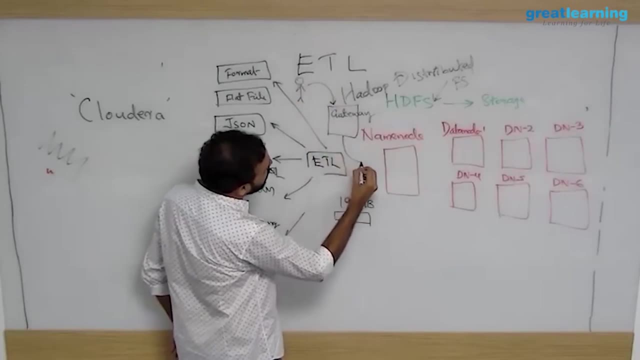 This is called gateway machine. So if I am sitting here, this is me very nice, right? So I can just connect to this machine. from this machine I can connect to the Hadoop cluster. You don't directly get inside the Hadoop cluster. that's my point. 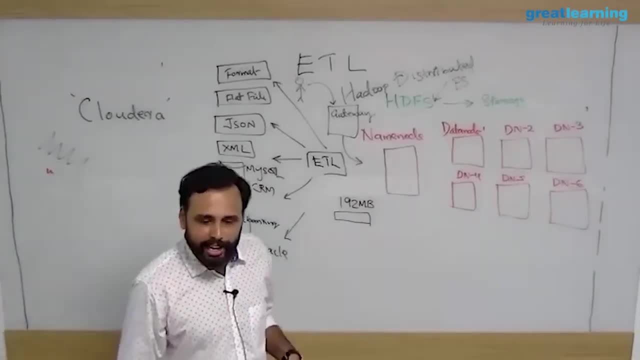 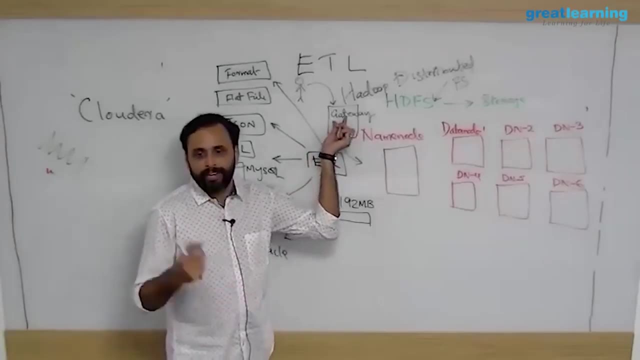 For security reasons and many other reasons. So companies do two things: either they will install something called a Hadoop client- even that is very rare What we used to do. there will be a Linux machine called gateway node. You will get a username and password. you type it, you connect to this machine. 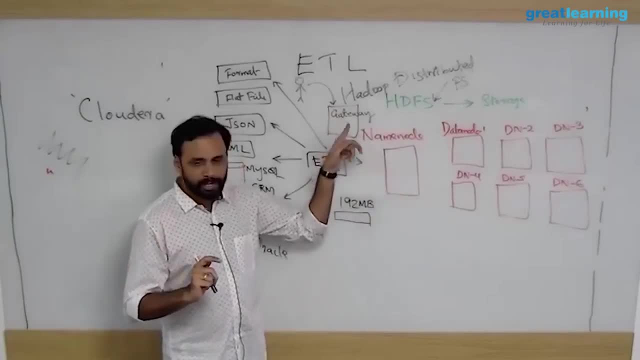 This machine will already know how to reach here. you don't have to worry. You issue the commands here, it will run here. But whatever way, Let's say you want to push this 192MB file from your machine, you connect it to the gateway. 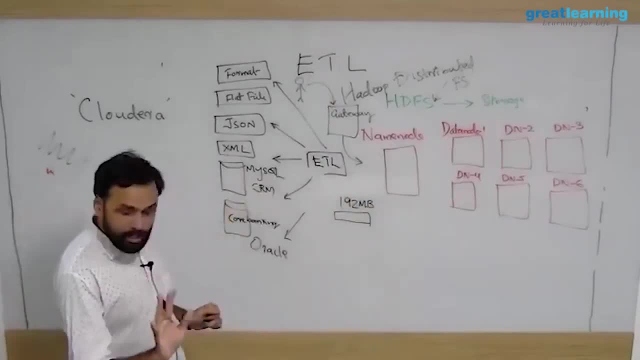 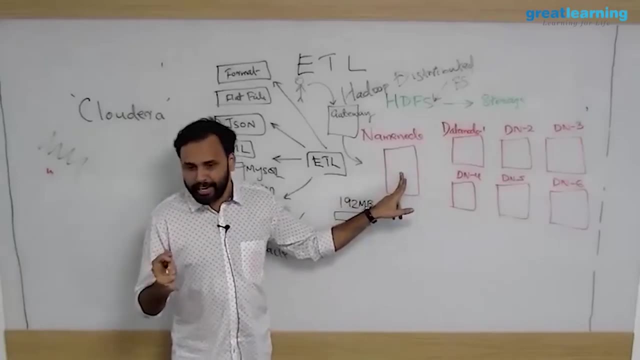 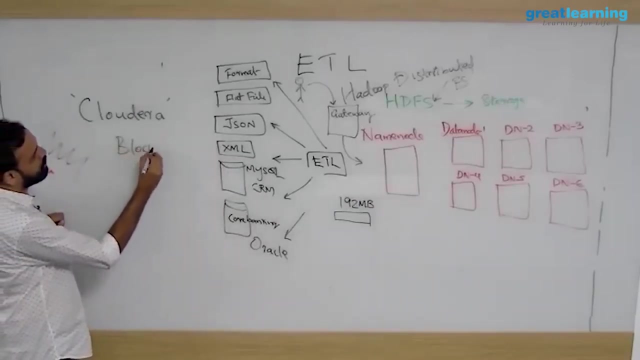 machine. you said, okay, upload the data. What is going to happen is that first thing which is going to happen is that your name node machine. this is a master. This guy will tell you something called block size. There is something called block size. 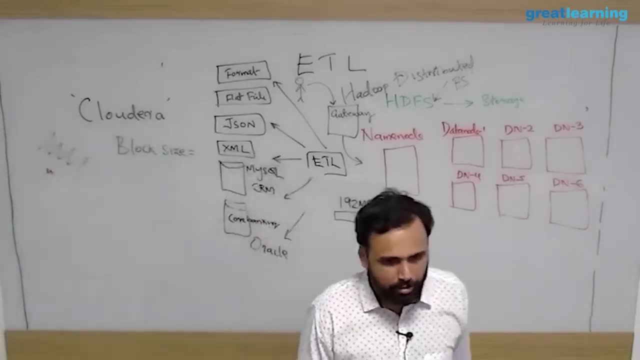 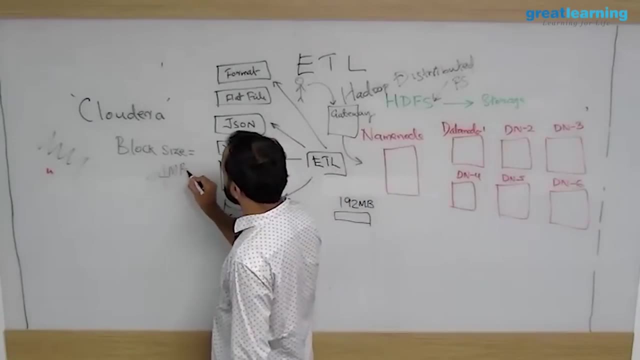 This block size can be configured for every Hadoop cluster when you are installing Hadoop. So I am assuming that the block size for this cluster is 64 MB. So what is block size? Block size will tell you what is the maximum size of data that you can store. 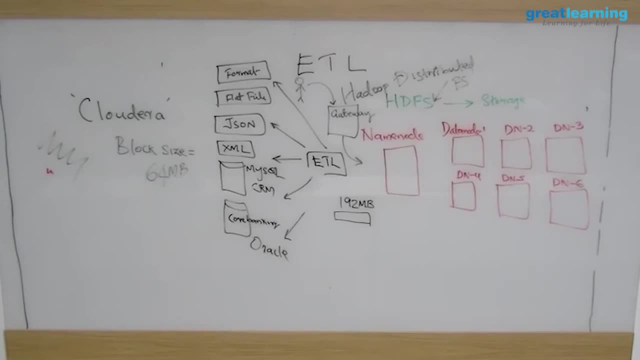 Meaning, if you are storing a 192MB file, what will happen? it will divide that into 3 blocks. Same thing happens on your laptop. If you are storing Um song on your laptop, what happens? Okay, you store a song, mp3 song, right? 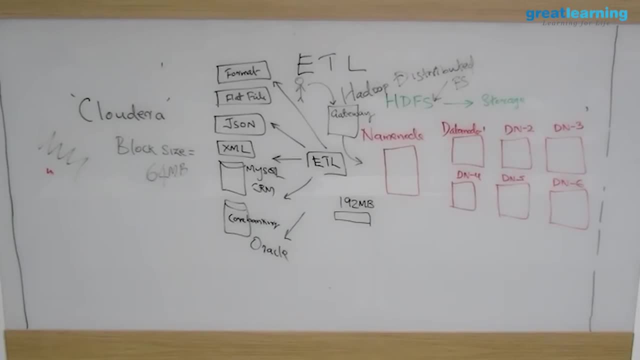 On your laptop. What do you think? The hard disk will actually take the song as it is Or it'll divide it. It will divide it. It will not store as it is. I think Linux uses four kilobyte of four KB block size. 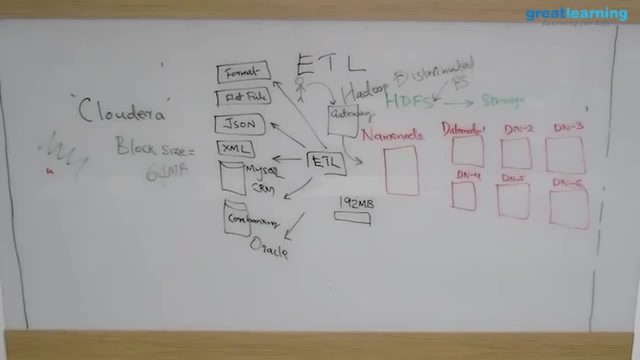 Linux. Windows also uses similar. Any file system will chop your data and store. Same thing happens in Hadoop also. So I am assuming that this Hadoop cluster has a block size of 64 MB, So this name node will get back to your client package. 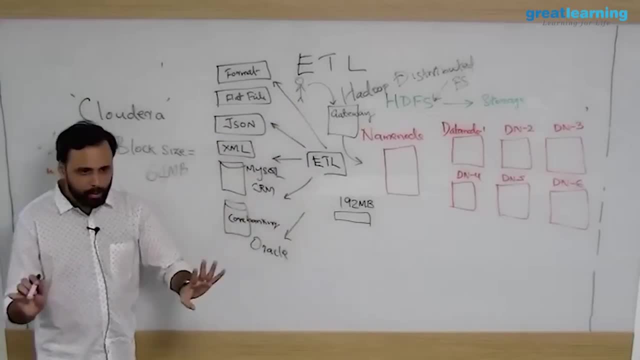 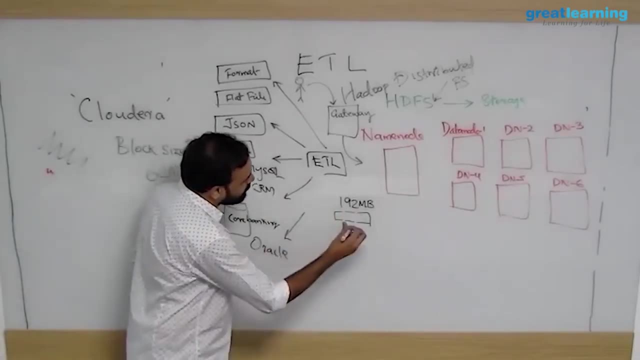 and say that divide your file into three or whatever you want, because the block size is 64 MB. So what is going to happen? This file will get divided into three block. You don't have to do this. This will happen behind the scenes. 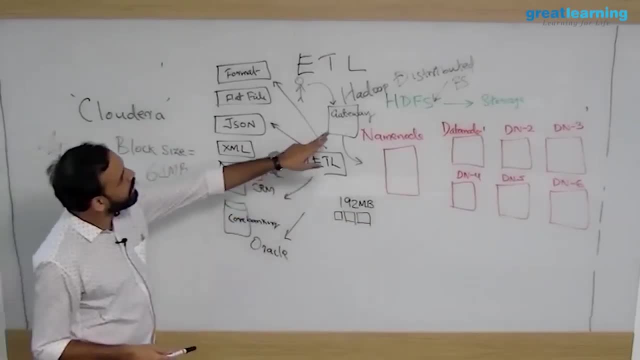 Like. you don't have to say that: what is your block size? No, it will happen automatically. This gateway has Hadoop client installed. That is what. So this Hadoop client on the gateway will already communicate. It will communicate with name node. 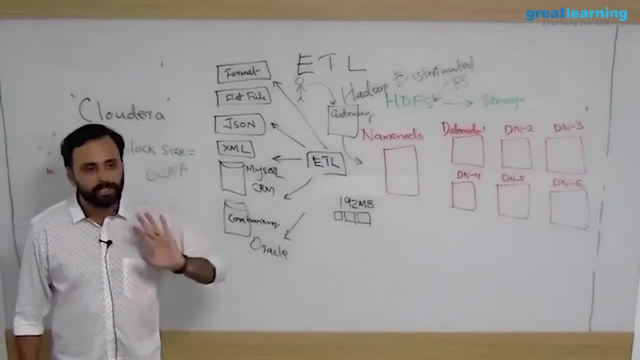 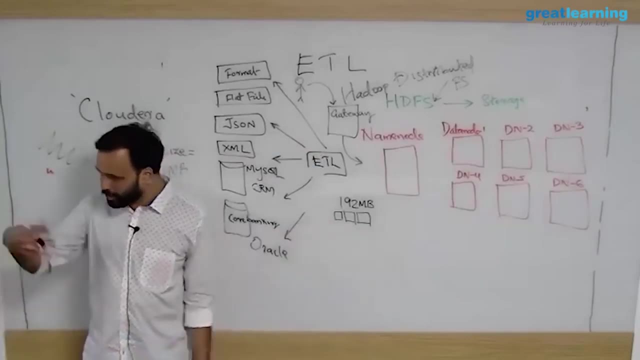 Name node will say that, boss, in my cluster the block size is 64 MB. You manage yourself. So the client will divide your data into blocks of 64, 64, 64.. Total is 128.. So now you have three blocks: B1, B2, and B3. 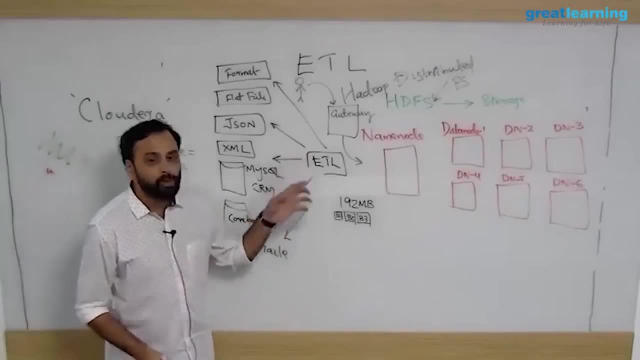 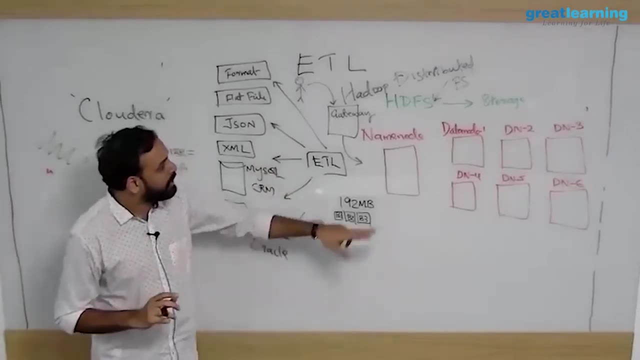 You have three blocks now of the data And then again you go back to the name node. You ask the name node- I have three blocks Now tell me where to store- And the name node what it does. it has communication with all the data nodes. 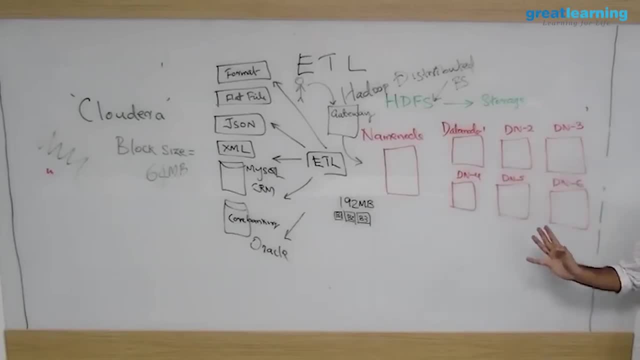 It knows where how much space is available. It will tell you that. do one thing: Store the first block, probably here, just an example. Store the second block, probably here, B2.. Store the third block here, B3.. Most of the cases, the name node will give you. 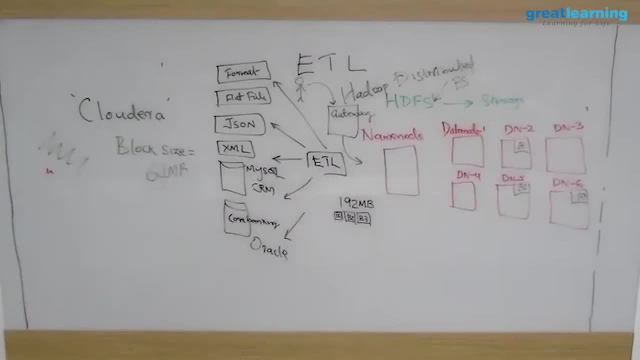 different, different machines. It will never allow you to store everything in one machine, So you divide and distribute. That is how you're storing the data. So now your data is divided into three blocks And they are stored in three different data nodes. 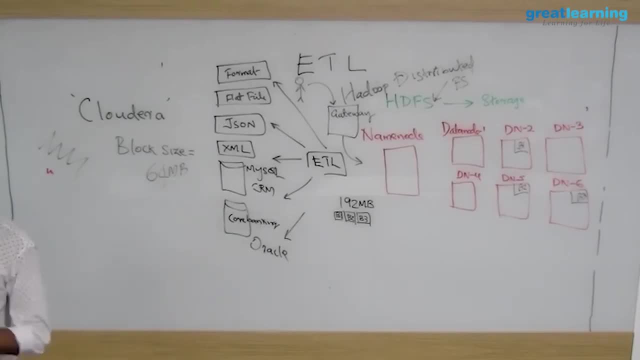 So this is like six. In reality you have 5,500 machines. So three blocks is easy, But sometimes a couple of blocks may end up in one machine. also, It depends on the storage, But ideally it gets stored like this: 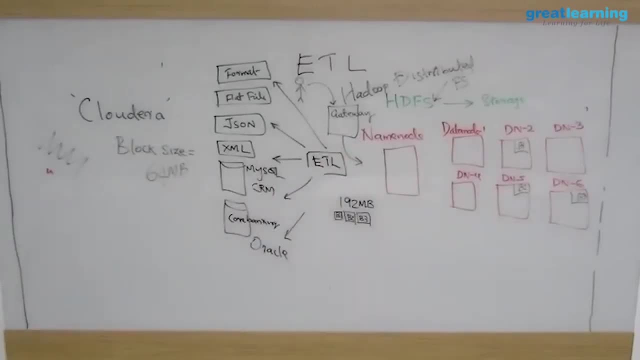 Now you may be wondering why the block size is. it's not random. It has the name node, has an idea like how much storage space is available on each data node, So it will come up with the three machines Within that. it just picks randomly three of them. 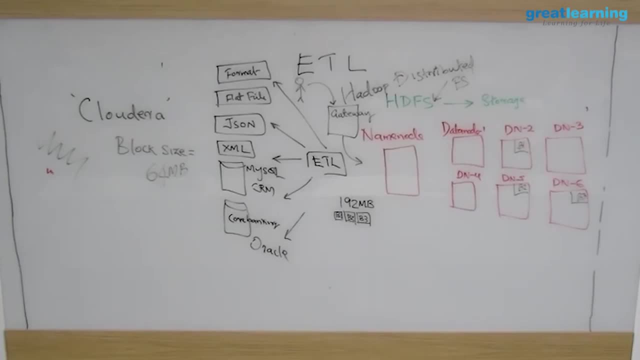 and say that you dump it there And I will tell you So. if you think logically now, if I want to process this data, three machines can process this data. If I store all the three blocks on one machine, one machine has to process three blocks. 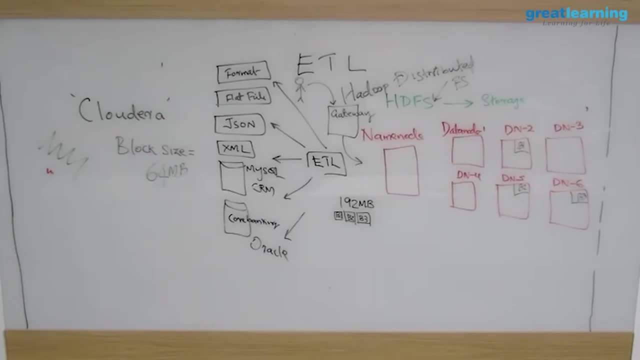 That makes a difference. So ideally, you divide and distribute the data. most of the cases You don't have to do it. Name node will do it for you automatically. OK, This is all inside a LAN. This is all inside a LAN. 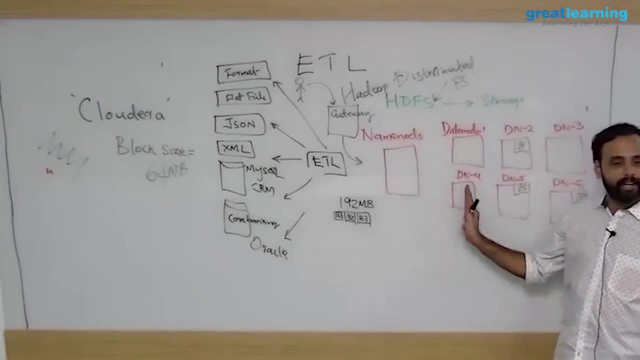 All these machines are communicating with each other. The data nodes all send a heartbeat to the name node, saying that they are alive, also so that the name node can detect how many of them are alive or down or anything. I can't get my data. 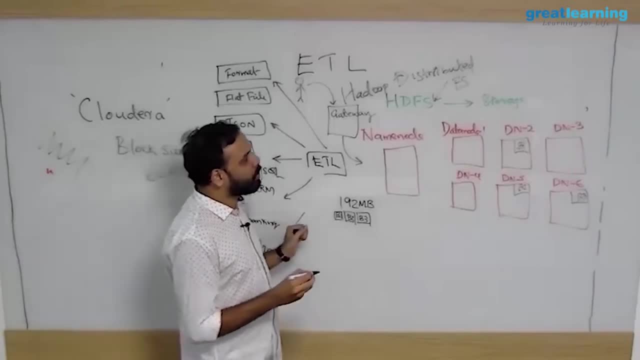 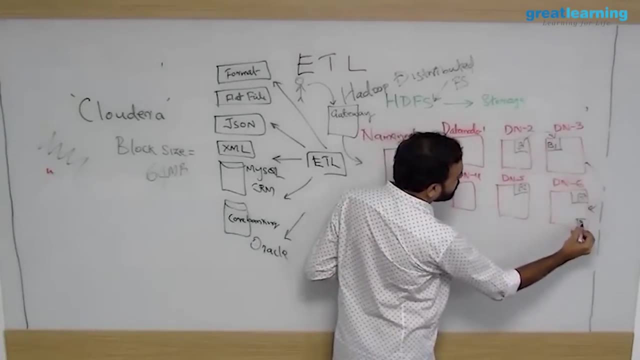 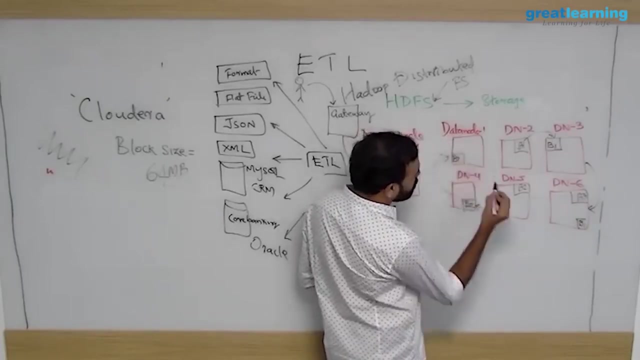 So by default in Hadoop there is a replication of three, which means each block gets replicated three times to other machines. I'll just draw this. then come to your questions. Give me a moment. B2,, again B2,, and I'm just drawing randomly. 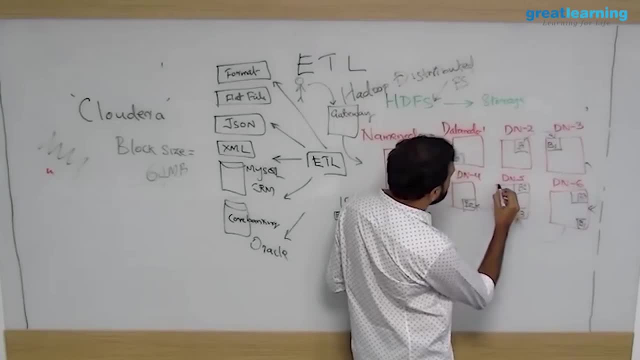 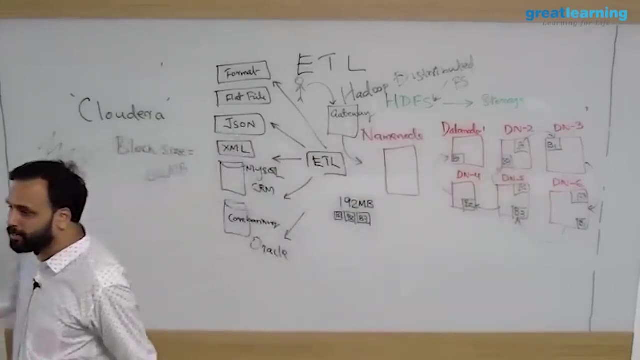 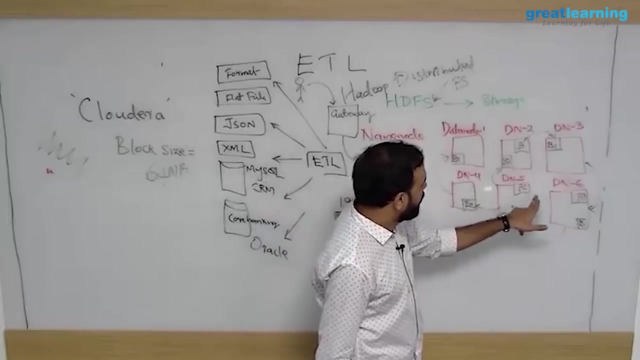 I mean just taking that. these are the machines B3, probably from here B3.. So if you look at each block, each block is replicated three times to different, different machines. So now let's say this machine crashes. This B2 is still available here and here. 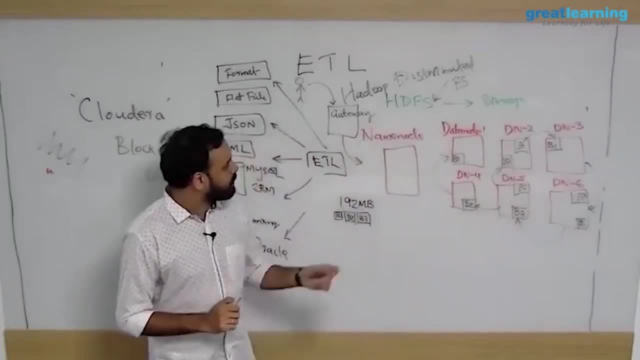 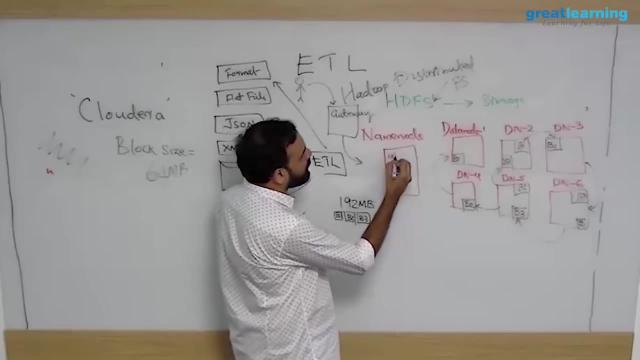 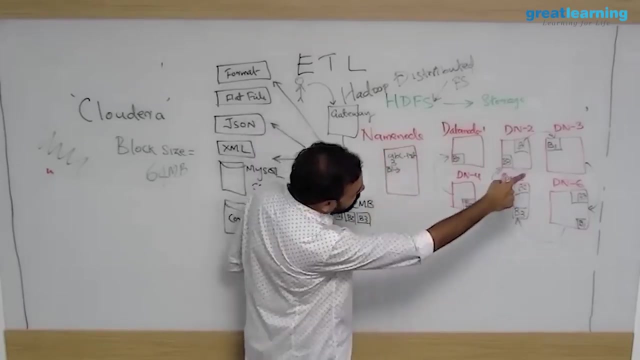 I can recover it from here And now. what happens is that the name node will store the metadata, meaning the name node will write here. There is a file called abctxt. It is divided into three blocks. Block one is available on where: 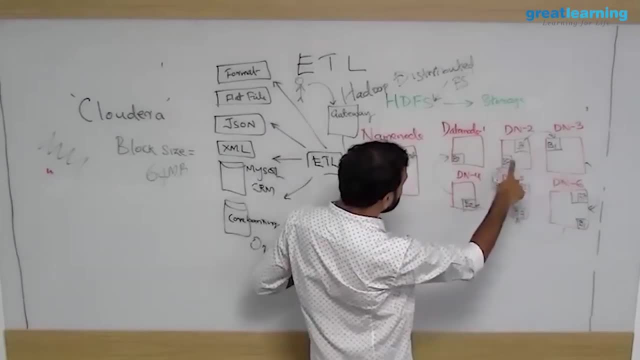 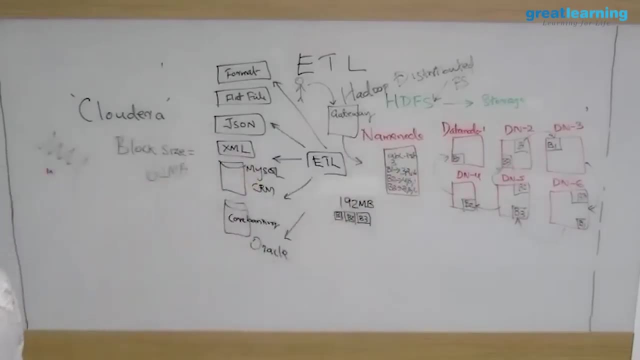 Three. Where is it? 3,, 2, 6.. So B1, 3, 2, 6.. B2, where? So the purpose of your name node is to actually store the metadata or the index. And if the name node crashes, You cannot access the cluster. That is for sure, Because if the name node is gone, then everything will be gone To prevent that. in most of the Hadoop clusters you will have an active name node and a standby name node, Meaning there'll be two name nodes. 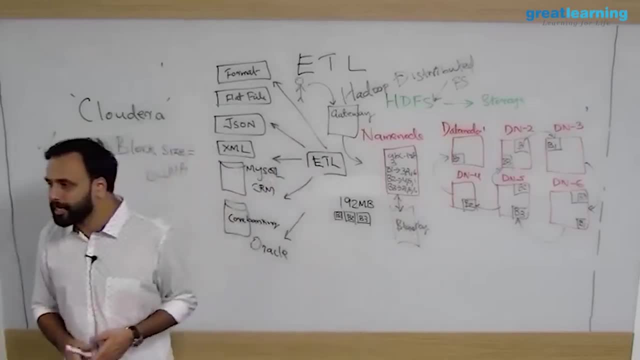 These two guys will be in constant communication. So if the active name node crashes and the disaster recovery. to set up that, there is a company called Van Disco Disco, Disco, Dance, Van Disco- Very interesting company. So Van Disco is one of the popular companies. who set up disaster recovery for Hadoop, But you don't do disaster recovery like in traditional systems, Meaning if I have a 100 node Hadoop cluster, I won't set up a 100 node backup cluster. right? That is waste of money. 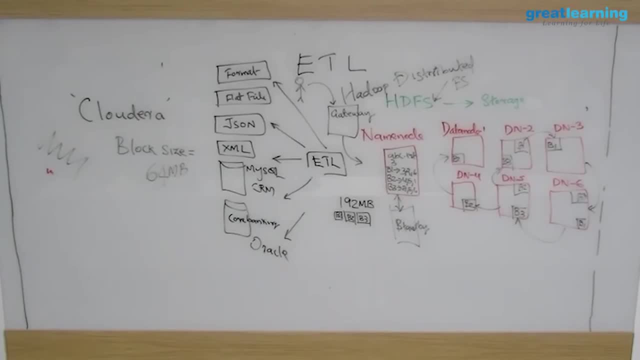 Very rare. King Jong will fire a missile right. If he fires, God saves right. So what I will do? even in the Hadoop cluster, you have to classify the data You are storing. 100 terabyte data, Probably, not all. 100 terabyte is so important, right. 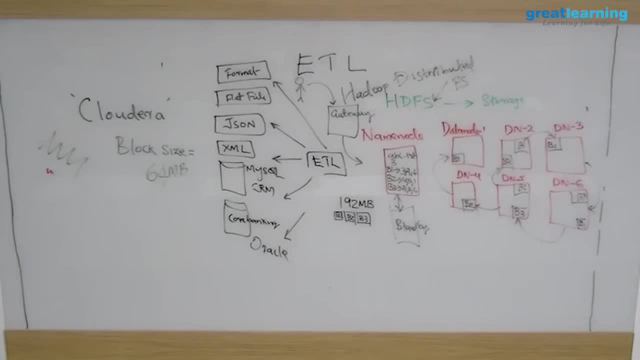 Is it? No, a lot of data is archival and all. So in the 100 terabyte data I will identify probably 10 terabyte, which is very critical, And I can periodically back up that data to my DR center. I don't set up a 100 node cluster in Noida. 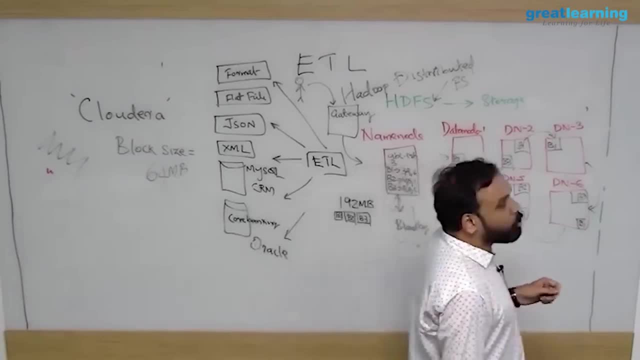 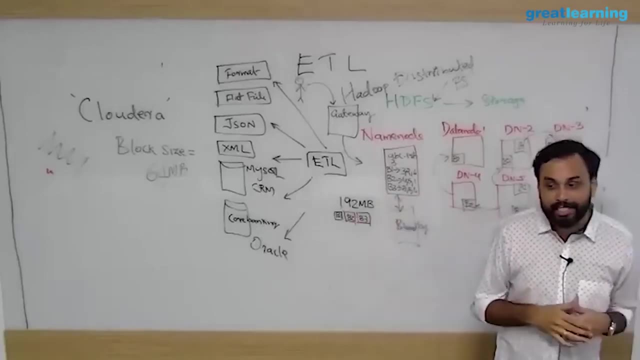 to back up a cluster from here. So we use a tool called Distributed Copy DistCP in Hadoop that can synchronize these two clusters: primary backup DistCP. it's called Distributed Copy- 100% Hadoop availability right. 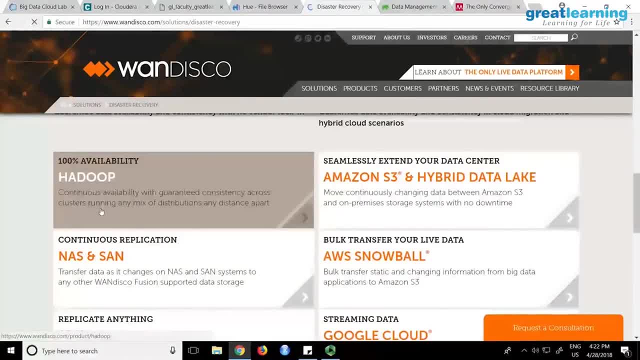 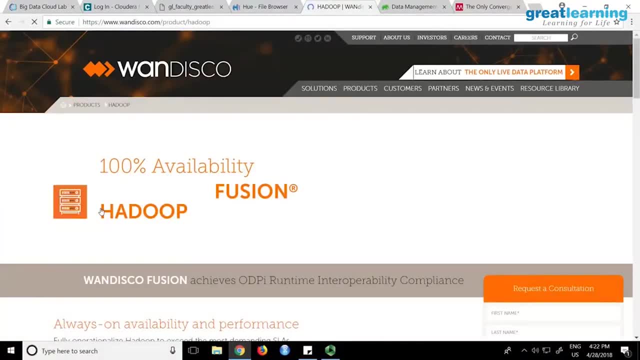 See, this is what I'm talking about. We used Vandisco in one of our projects. That is why I know Usually people do not be aware of these things, So I was working as a Hadoop administrator also for some time. 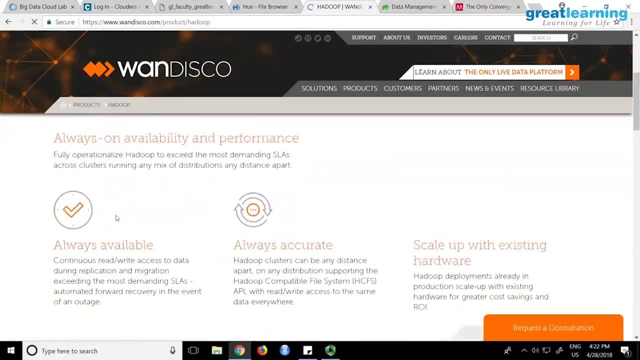 That is why I know this, Because these are all like real-time things. It is configurable. They use 64 also. There is a parameter. I'll show you where you can change block size. OK, Hadoop, the default block size is 128 MB. 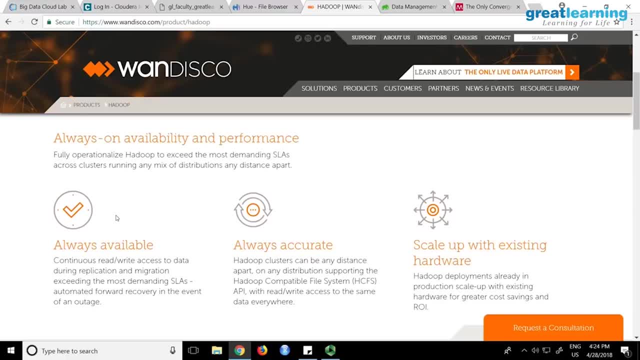 You should also understand one more thing. There are three major releases of Hadoop: Hadoop 1,, 2, 3.. Hadoop 1 is the older release And nobody is using it these days, So you don't have to worry about Hadoop 1.. 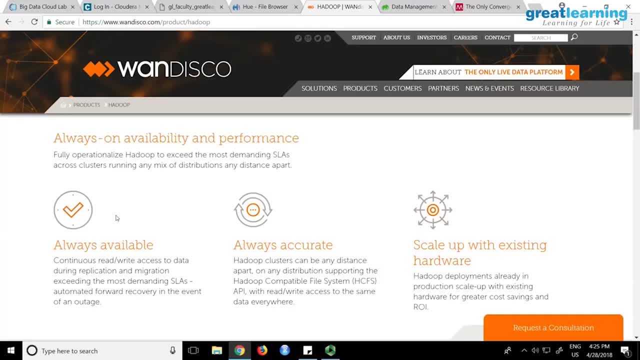 It is not available in production right now. 2013 was the last year when this was used, So no longer used. Hadoop 2 is what you are using, I am using, We are using. This is the current edition. Hadoop 3 released in 2017, December 15,. 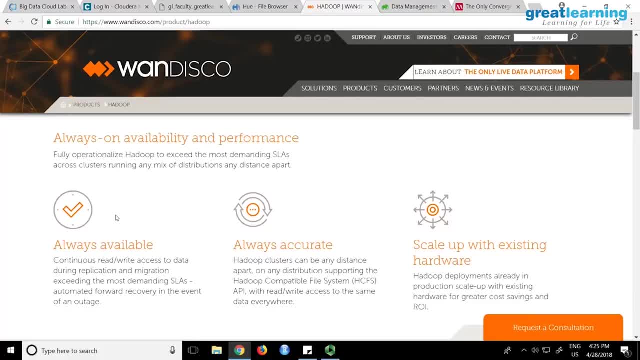 like three months back. OK, Now let me ask you a question. If you are storing 100 terabyte data in a Hadoop cluster, how much storage do you need? So there are multiple approaches. One thing is that some companies this replication factor can be changed, by the way. 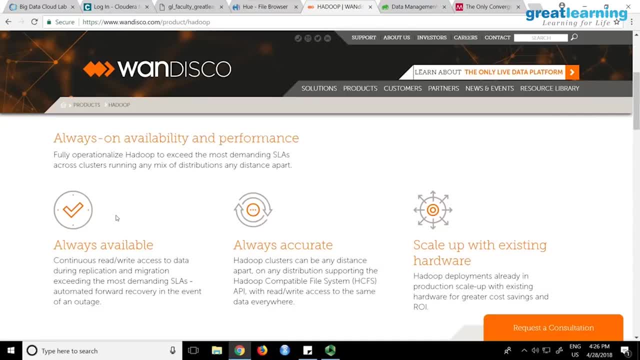 It's not hard-coded. Some companies say two Right, So you get two copy of data. Also, while copying data, you can also get two copies of data. Using the data, you can mention the replication factor- Very interesting thing. 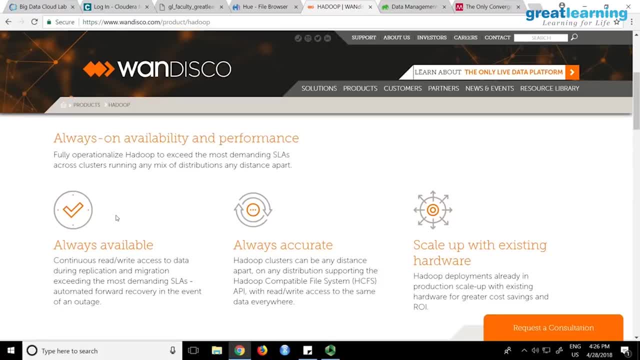 I am copying a file, one TB file. This file I can afford to lose. I can say copy with replication 1.. But it had led into a debate in the Hadoop world, So a lot of people said that this is very bad actually. 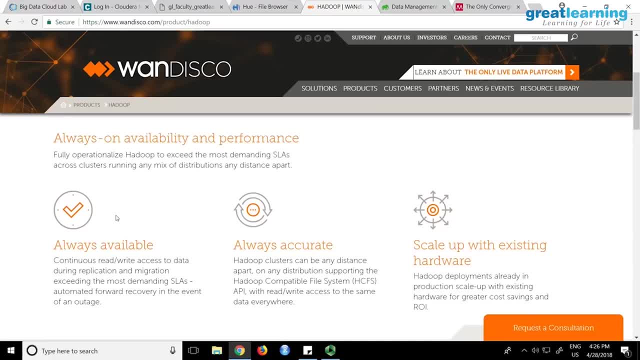 Because three times replication means you are losing a lot of space. That is why in Hadoop 3, there is no replication And there are only limited types. You can read text, XML sequence file key values. So some limited number of types of files are there. 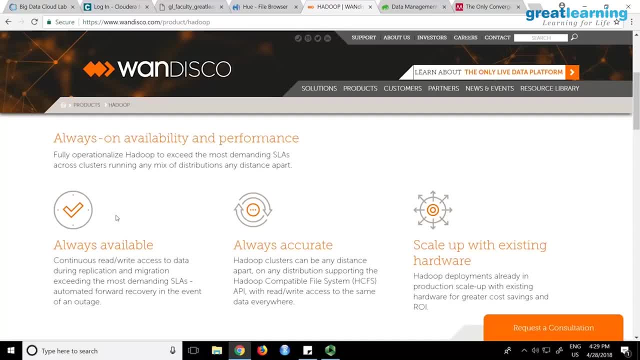 And how do you So? this is a very good question: How do you handle unstructured data? It is also a very confusing concept. Many people believe that in the world of big data, you are always playing with videos and images. Actually, no. 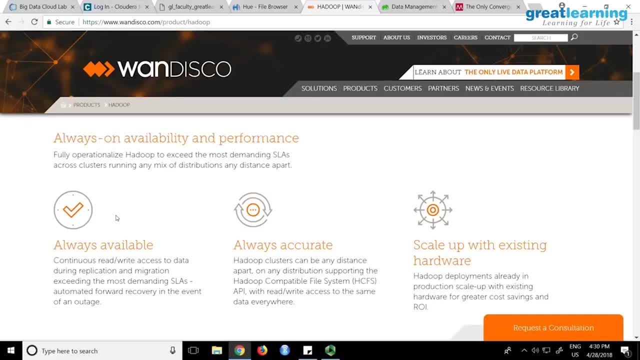 See, Many people believe every day you'll go to office and run some facial recognition, like you see in the Mission Impossible movie, And yes, yeah, I got big data. No, you don't do that. actually, You can analyze images and videos. 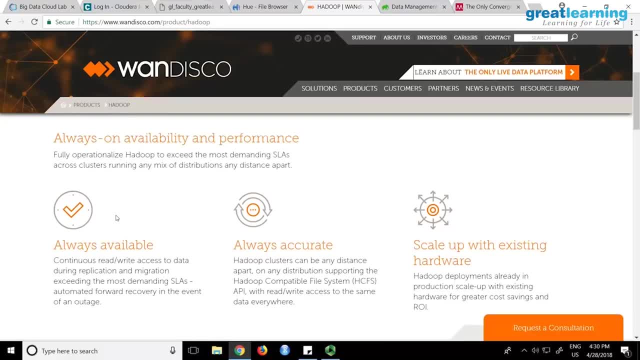 There is no doubt It's very difficult actually to do. Analyzing video and image data is very difficult Because you can't directly analyze it. You have to convert it into binary. Once it becomes binary, in Hadoop you have a format called sequence file. 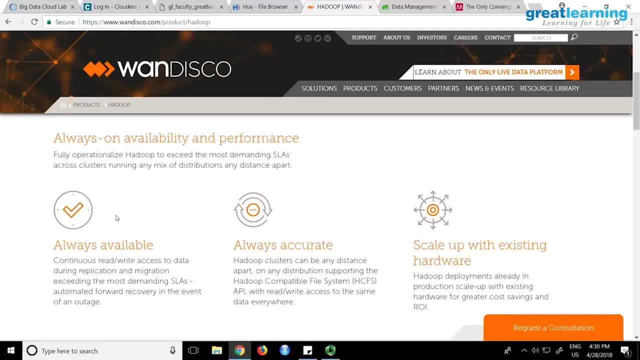 You have to read it as sequence file and write a program to analyze it. It's actually a very difficult job to analyze these kind of files And not everybody needs to analyze it. Let me give you a real-time example. I was working with 24Bytes. 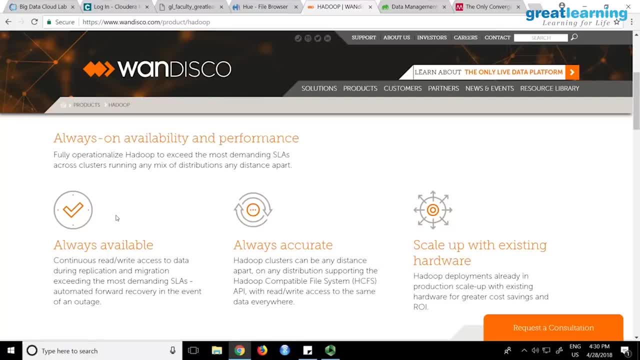 I was working with Baba7, the customer care company. What is their primary business? Customer care. In customer care, people call. Do you think they will listen to what customer is calling? You are giving support to other companies And you are running a call center. In a call center. customers will call. Do you actually listen to what they are talking? Let's say, take Idea, for example. How many calls Idea will be getting in customer care? Do you really think they analyze your calls, For example? 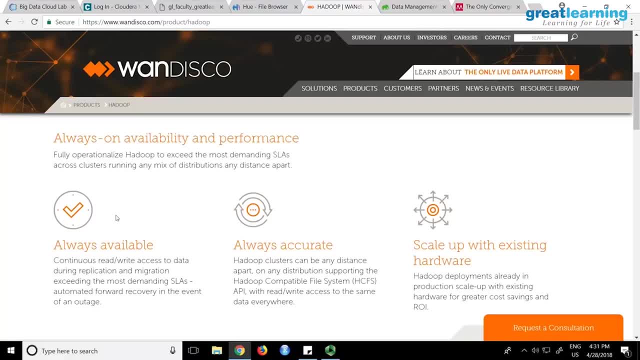 If you were an angry customer, you spoke for one hour. That call is recorded. The person who took the call will go to the manager And the next meeting manager will analyze that call and say that this was your mistakes. I'm saying, do you actually analyze? big data analytics on these kind of things? Not really. You will analyze the metadata, not the actual data. How many people called, What was the duration, What they pressed? This is the data, not the actual audio data. Because you can do it. 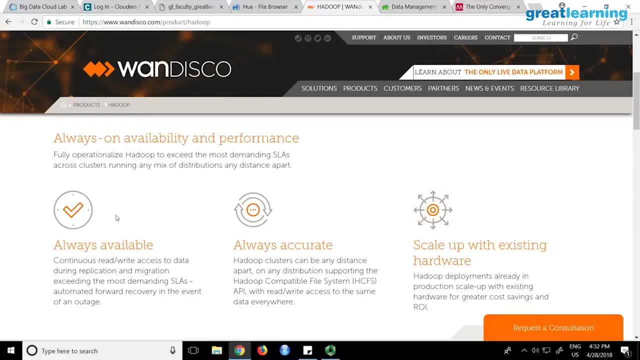 I'm not saying it is impossible, But then you have to. So how do you understand what he's speaking? And it may fail. it may not fail. You are not 100% sure If it is a US customer or something. 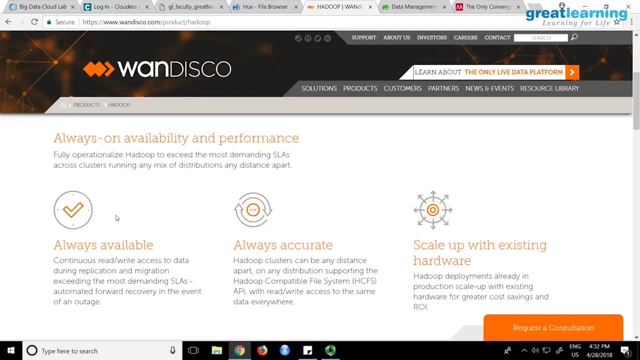 we can approximately match With an Indian customer. how do you identify all this? It's not possible, right? He may speak any language, any accent, right? So practically these things are not possible. I'm saying you can analyze unstructured data. 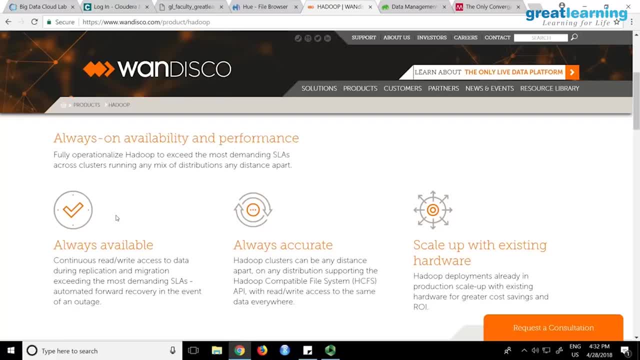 There is no doubt about it And companies like Facebook can all do. Facebook actually analyzes video data. They have to for some reasons that they have to do Right, And there they have written complicated algorithms to read and convert to binary and all. 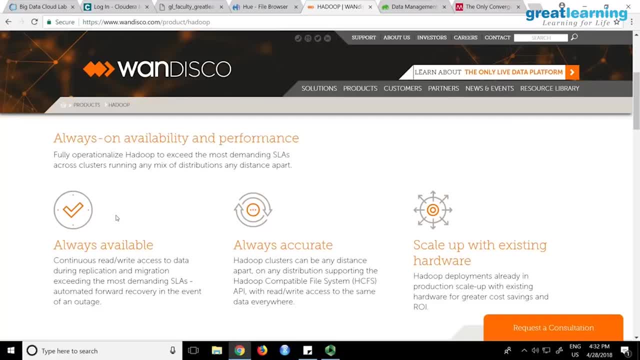 But if you are going to work in a regular project, you will always see structured data- CSV files, JSON data, normal text data- But if you're storing also, so you need a class to read this type of files. That's what the question was. 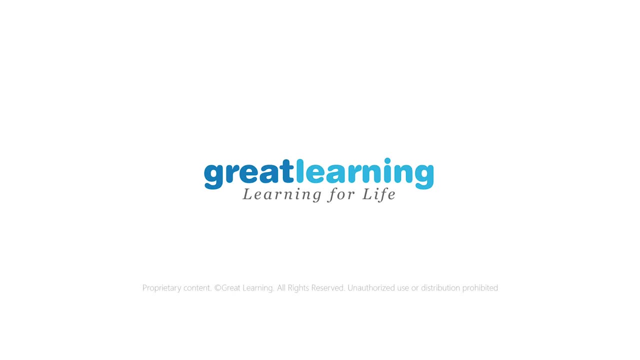 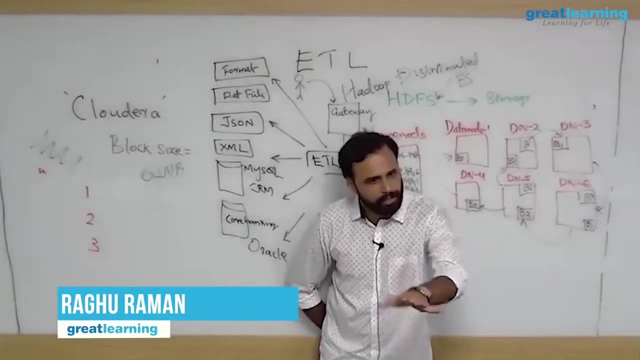 Right, We have a tool called Uzi, Apache, Uzi. Uzi is a tool actually that comes along with Hadoop- Hadoop when you install as a tool. So in Uzi you will be scheduling your program. 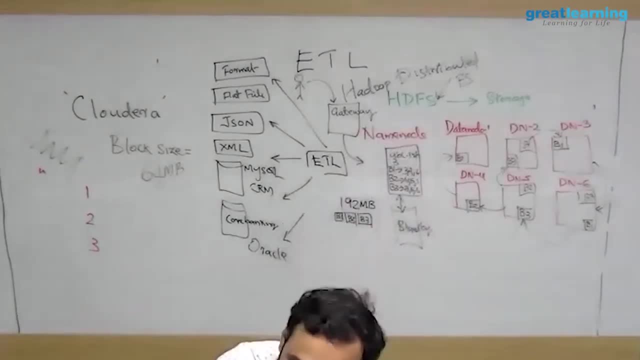 You wrote a Spark program: Analyze 100 TB data. If you immediately submit the program, probably the program will not work, Because already somebody is analyzing the data. Where do you have space to fit all these things, Right? So what you do? you write it in Uzi. 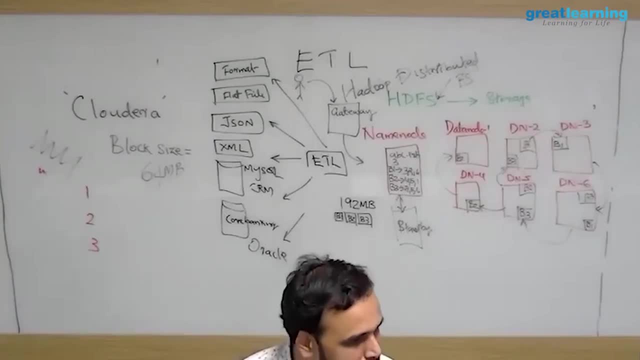 and you contact your Hadoop admin, Say that I want to analyze 100 TB data. When can I run this? He will say tomorrow, 11 October. Most of this analysis is batch, not real time. Real time is a different case. 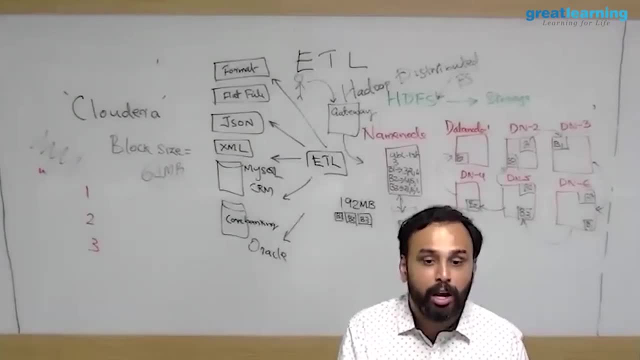 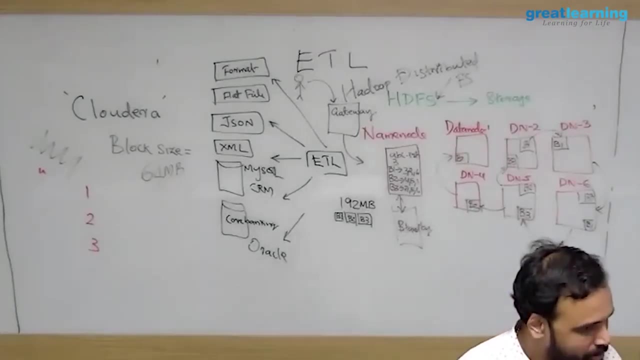 But batch jobs you schedule it via Uzi. Also, you have something called queue. in Hadoop, For example, you are working as a developer, I'm a tester. Can we have same access in the cluster? Of course testing cluster will be different. 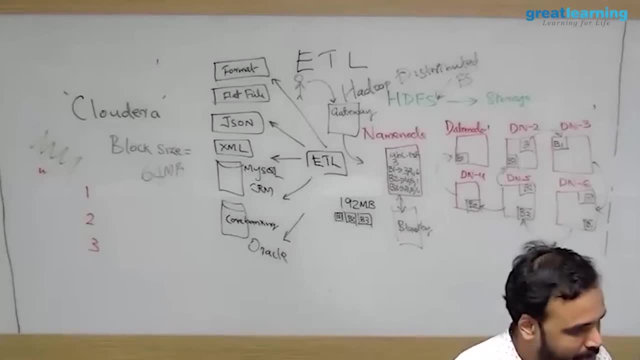 But let's say I'm a researcher, You are a developer, He's a data scientist. Can we have the same access on the Hadoop cluster? No, Probably. you are a developer, You need more resources. Probably I need less resources. 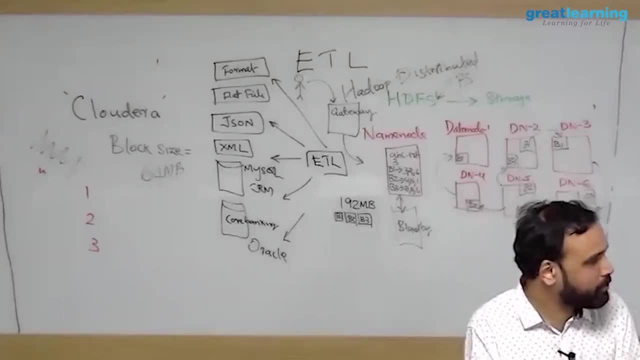 So what we do? we create something called queue. There is something called queue. There is something called queue. There is something called queue. We create In those queue, we allocate resources. If you are coming from the developer team, you will get 30% of the resources. 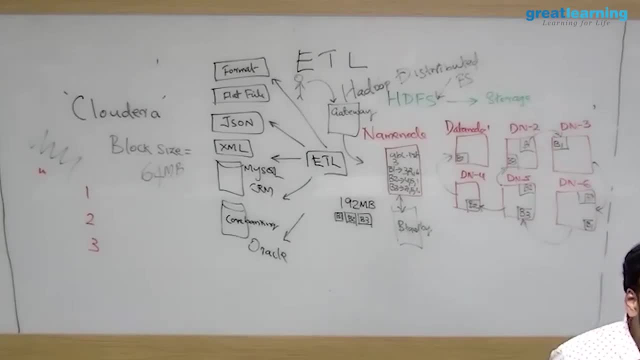 If you are coming from other team, you get 40%. Otherwise I can utilize all the resources. If I write a program, I can make the cluster only for mine. That's not possible in a Hadoop cluster, So management is entirely different. 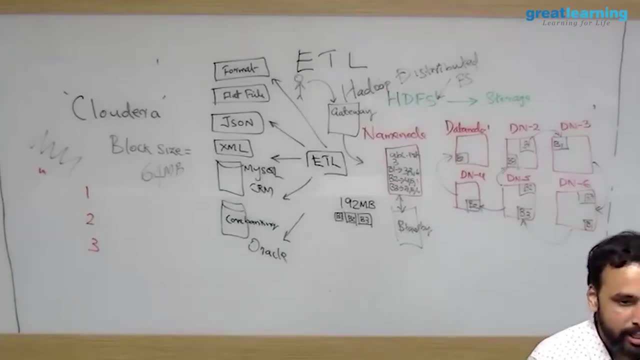 How do you run these? jobs are all different, But to just answer the question why you are dividing, is that you can use parallelism. Otherwise a single machine has to process everything. Queue means multiple teams will be there. Each team can get a queue. 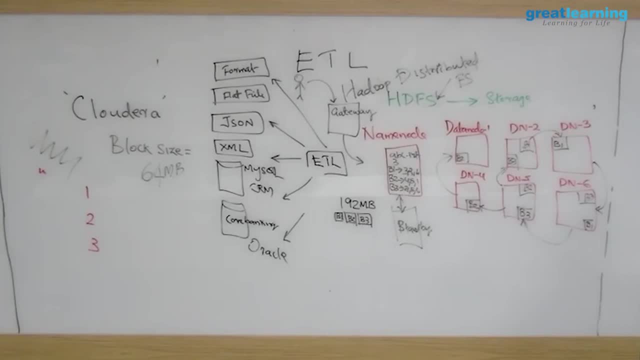 So when you submit a program, you will submit to a queue. You will not directly submit to the cluster Queuing in terms of resources. Say, for example, in your Hadoop cluster have 10 data nodes. Each data node has, let's say, 10 GB RAM. 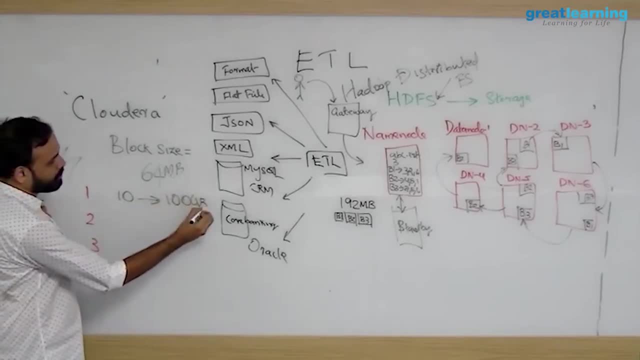 So, totally, you have 100 GB RAM in the cluster, right, And let's say, 10 data nodes each has four core processor. So you get what? 40 core processor right Now. if, If somebody want, they can get all these resources. 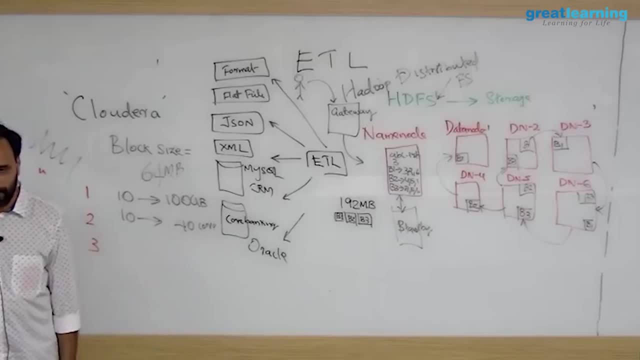 in their program. If he is getting, nobody else can run a program in the cluster. Should not be like that. So what we do? we create four queues, let's say, or two queues. In this queue I will say 60% of the resource should be there. 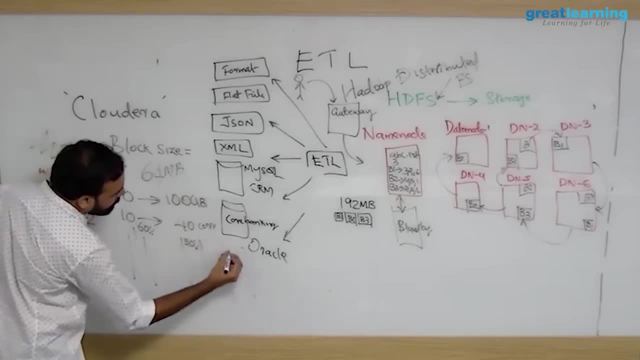 Here I'll say 30% should be there. Here I'll say 10% should be there. So this will be the developer queue. They will get 60% of the resources. That means 60 GB RAM, 60%, right. 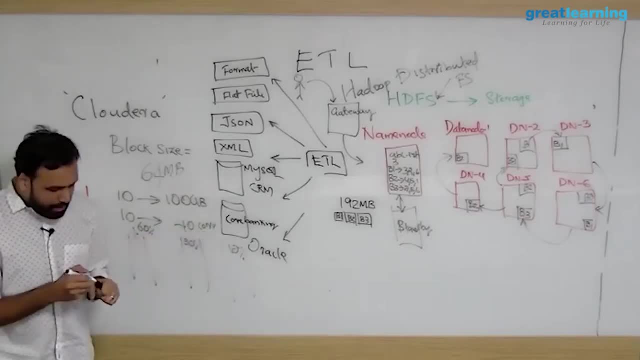 24. 24 core processor, So they will never get more than 24.. So multiple ways of scheduling is there. In the normal scheduling they will get maximum 60% only, Or if the other queue is empty, they can claim the resources from there. 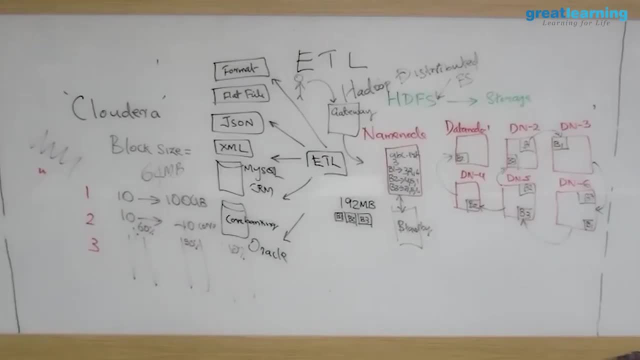 There is something called capacity scheduler, fair scheduler and all So the scheduler is called a queue. So if I'm creating something called fair scheduler within fair scheduler, it will allow me to create queues. So I can say, create three queues. 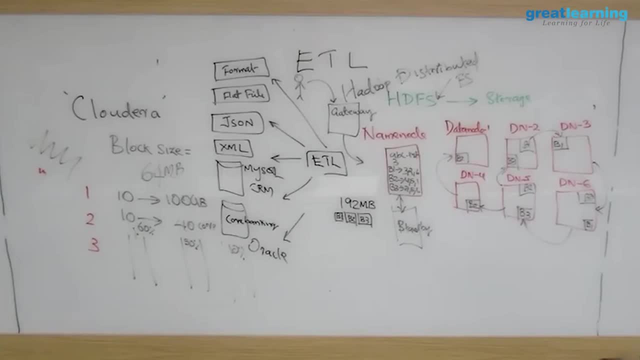 And whenever somebody is submitting a program you have to mention the queue name, otherwise the program will not work. So when you submit a program you have to mention the queue name. So when you submit to a queue, inside the queue you can write a policy. 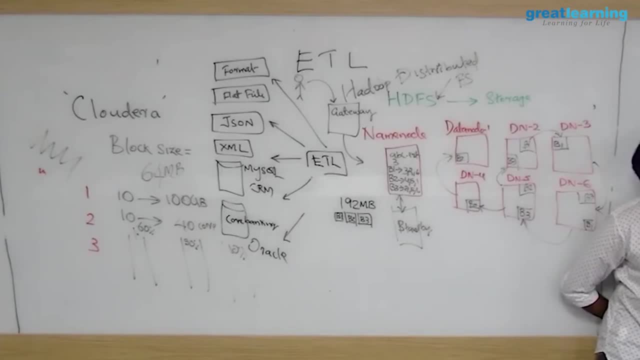 The default policy is FIFO, first in, first out. right Apart from FIFO, you can also have priorities and other things. You can write your own policy. So here it is text file or flat file, Any file you can select. So by default, like I said, if you're storing something, 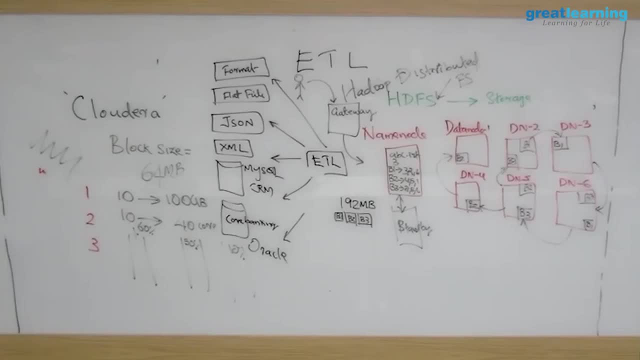 on HDFS. HDFS does not care what is your format. You store an image. it will store this image JPG. You have to make sense of it while reading the data. It is not like RDBMS. That is one thing. 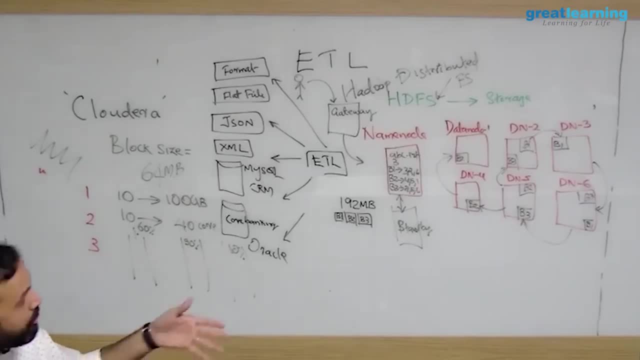 It is not like RDBMS at all, because HDFS is a file system. So if you dump, say for example, on my Windows machine, can I store an MP3 file, Can I open in Notepad. I can store an MP3 file in Hadoop. 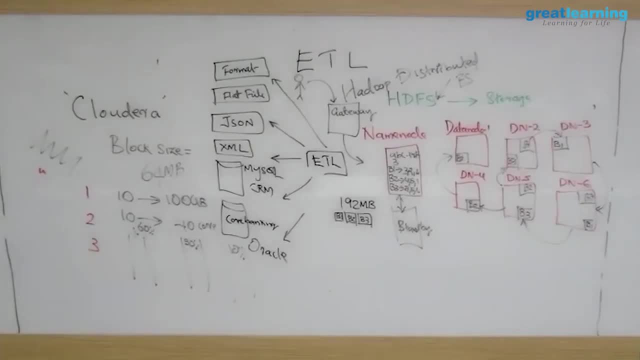 If I want to process, I should write a logic to process it. actually, That is for only queries. MapReduce is not query. MapReduce is programming language Queries. we are talking about Hive, So Hive is your data warehouse. on Hadoop. 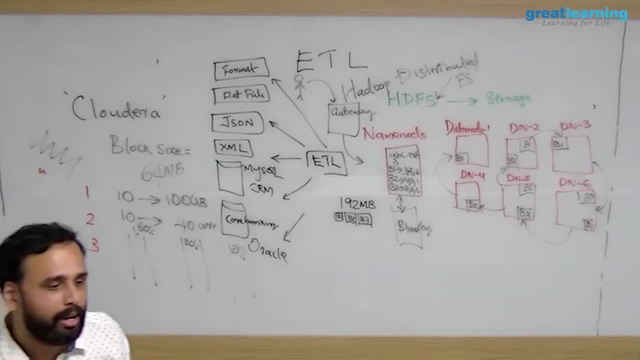 Hive will accept normal SQL queries. whatever SQL Indexing will really work well if your data can be managed by the RDBMS system or the data warehousing system. If I'm indexing the data in Hive, the data is actually managed by HDFS. 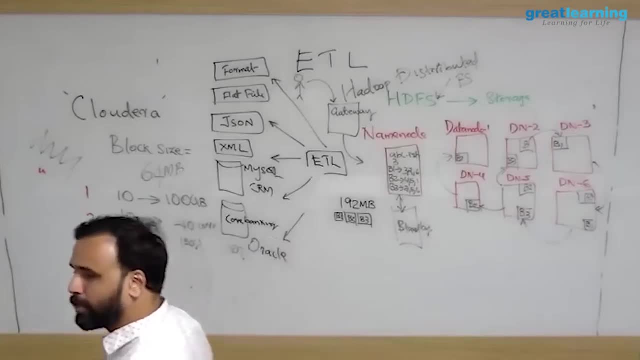 So I can get some performance improvements, but not like in your RDBMS. Never compare Hadoop with RDBMS. At the most you can compare with a data warehouse, because it is not transactional. It's equal to a data warehouse. I can say: 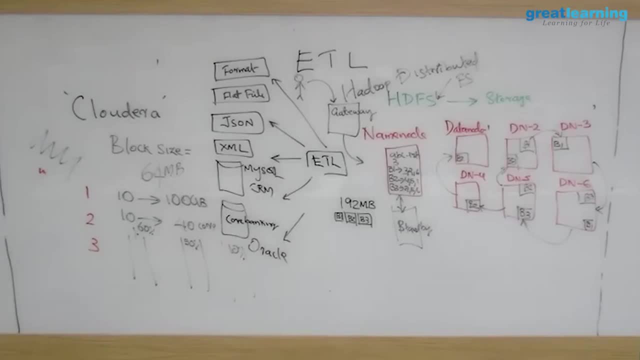 See, this is a big data platform, So you dump terabytes of file. You are not creating a record. Very rarely you edit- That's what I'm saying- This needle in a haystack problem, right? So very rarely you say that I want to create a new record. 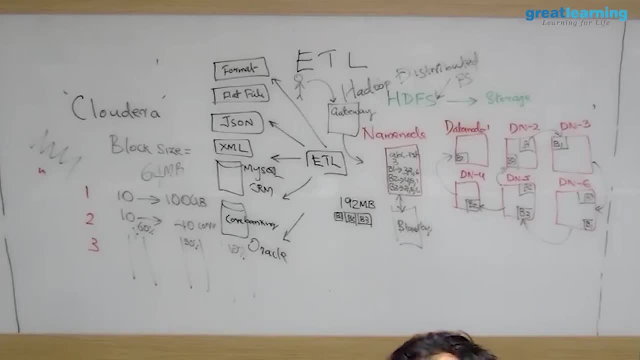 You will be adding files, continuous streams, that will be huge in size. You can afford to lose. You can afford to lose the data. I will talk more about that in the ecosystem side. So I will just talk about something called Hadoop ecosystem and then we will discuss further. 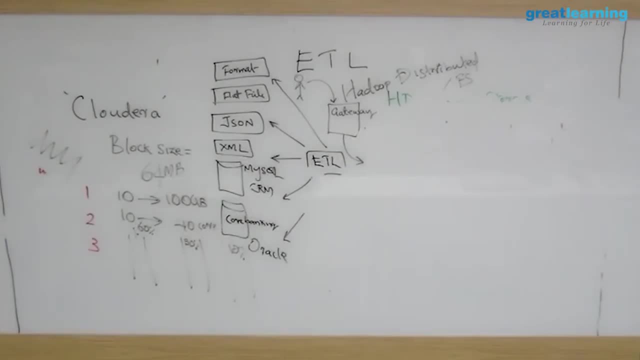 So Hadoop is actually written in Java, So the client is also in Java. Everything is a Java method actually. So you are just invoking a Java object. There is a fs read object which you call, And this object will get all this metadata. 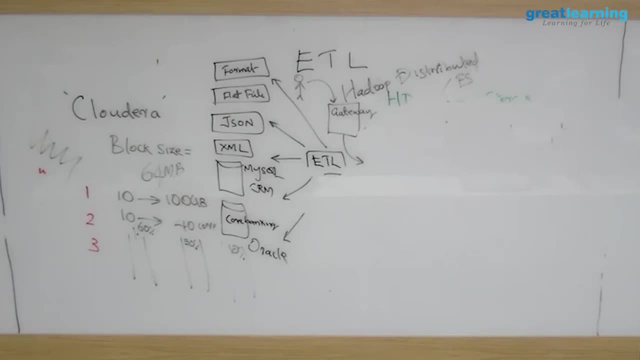 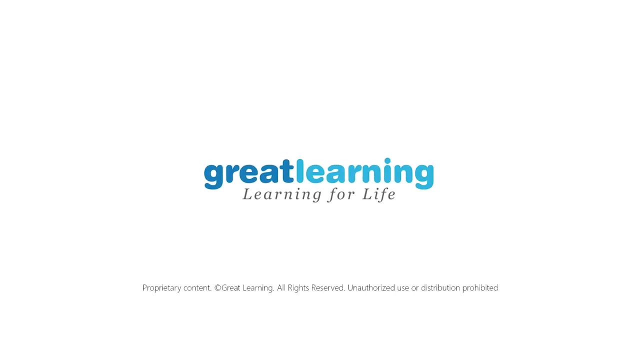 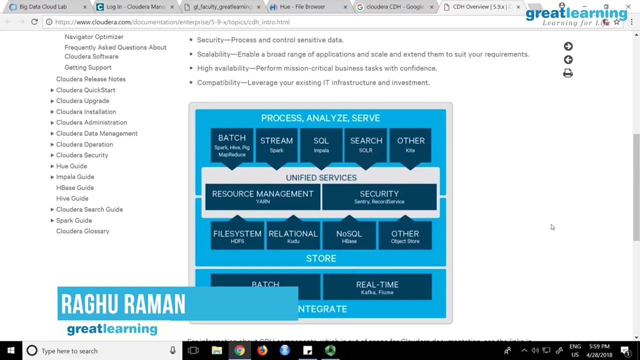 and give it to the client, And the client will keep it in memory and then go and read one by one from wherever it went. So I'll show you a Cloudera cluster. In the cluster we are using for the lab, we have only read-only access from the admin side. 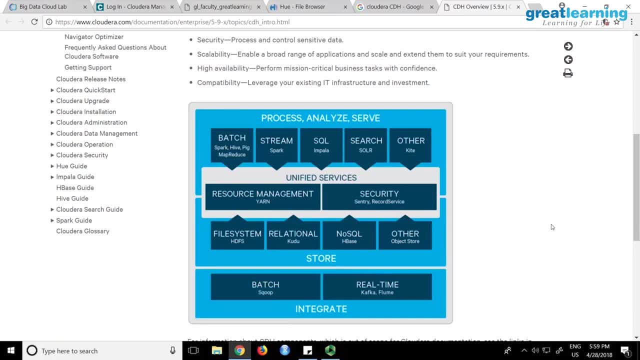 Which means you cannot change the replication factor or block size or anything. These are all done by admins. You can upload the data and then say that run the program, That will work, But that we will do tomorrow. But let's look at the cluster. 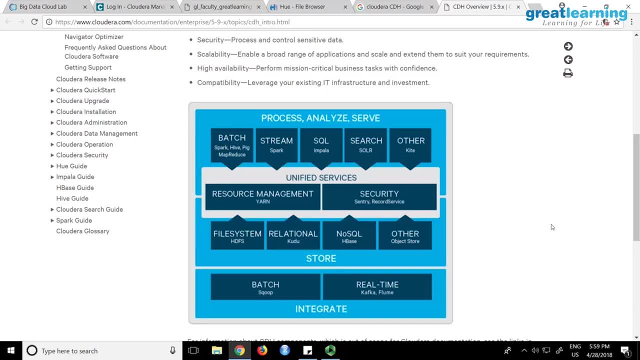 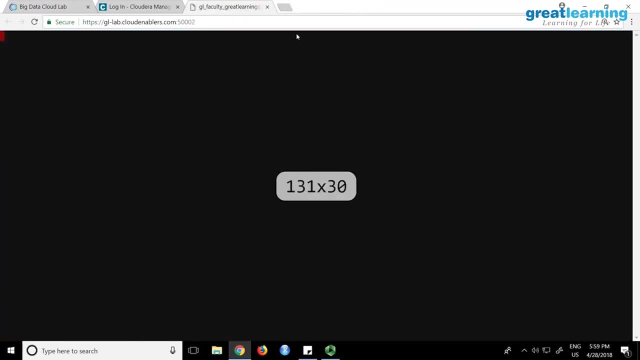 So so far we are talking cluster, cluster and we are not seeing any cluster so far. So I think Cloudera, Hortonworks and MapR, these three are getting used. All the three companies are sort of famous, I can say. 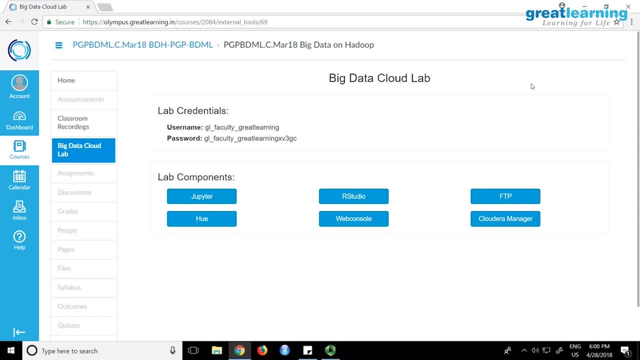 So do you have this In your LMS, like your lab and all So? because some of the things are a bit confusing. so I have to tell you we have to use Web Console. Web Console will connect the Linux file system where Hadoop is installed. 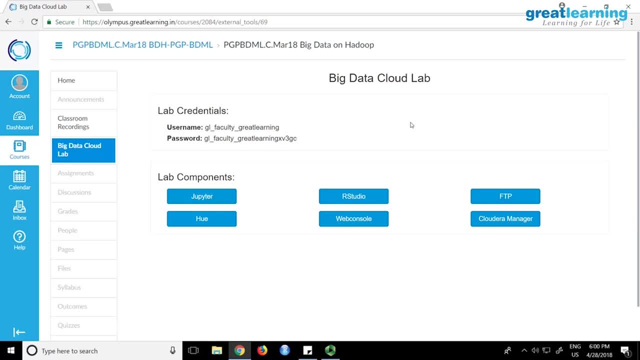 We will do that later. Cloudera Manager is the admin interface of the cluster So I will connect with it. but we will not be able to modify. but we can see stuff. So if I go to Cloudera to administer the cluster, like 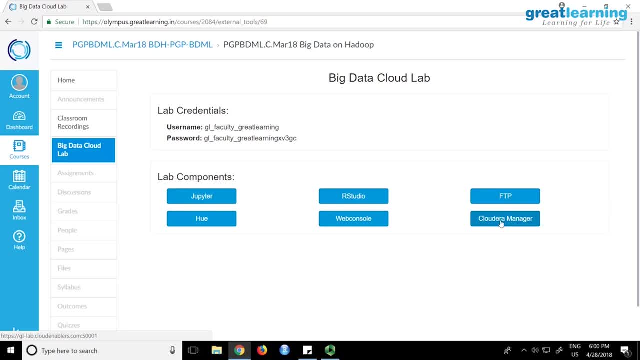 you want to add a server, Add a service, remove a service. add a machine, remove a machine. So the administrator. if you are a Hadoop administrator, you have to do all these things: add users, remove users permissions. 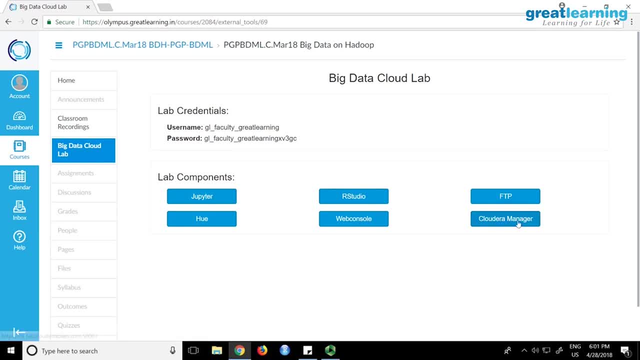 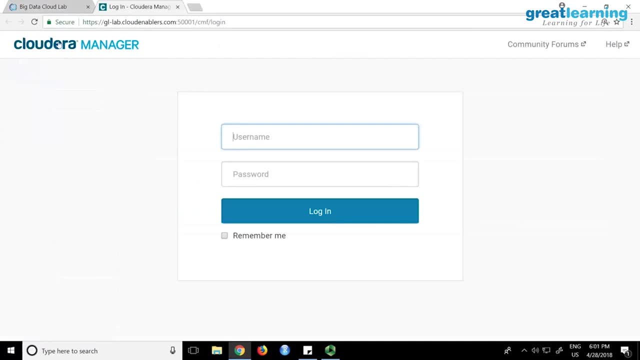 Everything can be done by Cloudera Manager. And why I did not speak about this? because we will not be doing anything. It's an admin utility. But to look at the cluster, this guy is good. So let me show you that. 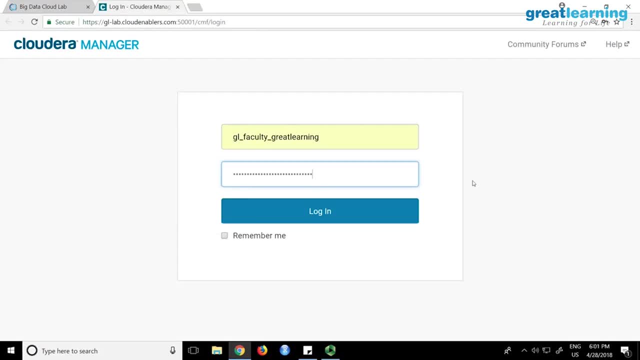 Now you have to install it. So if I am running in a company, I have to purchase, let's say, 20 machines. Basically, yeah, And then I have to. there is a process of installing Hadoop. This cluster already has installed. 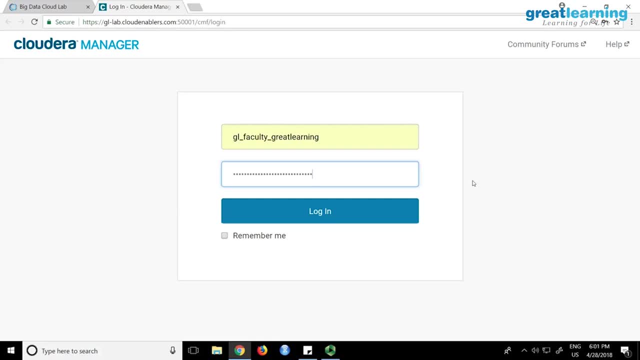 It's a running cluster. If you're creating from scratch, you have to purchase, let's say, 20 machines and download something called Cloudera Manager and run it And it will help you to set up the cluster. It will tell that which is your master, which is your slave. 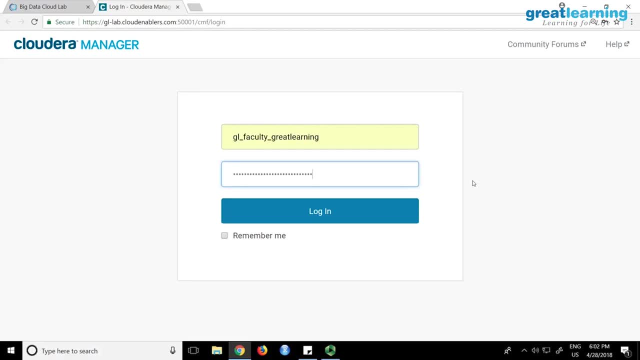 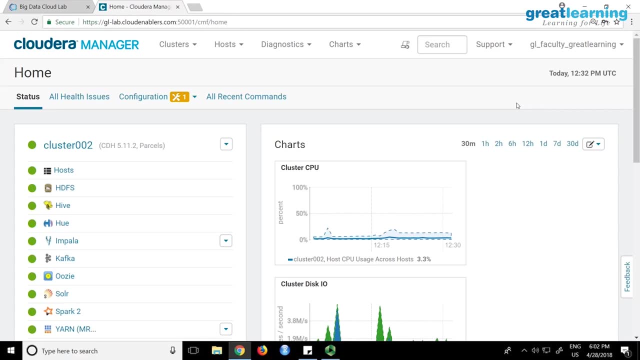 what is your block size? what is your? You will have access to this. I mean, if you want to practice, this setup is already available to you. So this is your Cloudera cluster. This is just an admin GUI to the cluster. 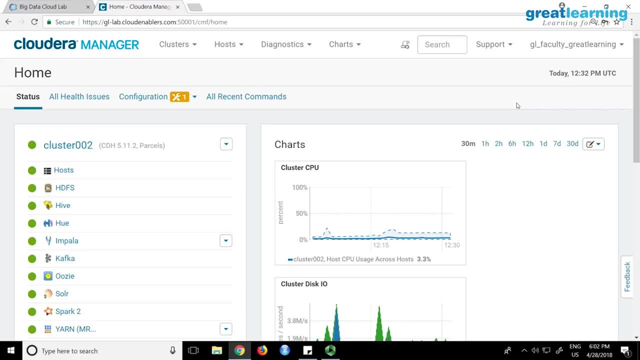 And once you log in, this is your dashed code. So you are looking at a Hadoop cluster. First point you have to understand. Second point: what is there in the Hadoop cluster? These are all the services installed, See HDFS. OK, HDFS, Hive Hue- I will talk about it. 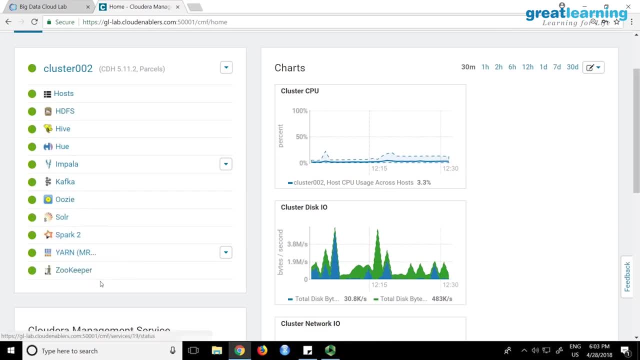 Impala, Kafka, Uzi, Solar Spark, Yarn, Zookeeper- all these services are running in the cluster. You see a green right. This is just to get a quick overview of the cluster, like what is running in the cluster. 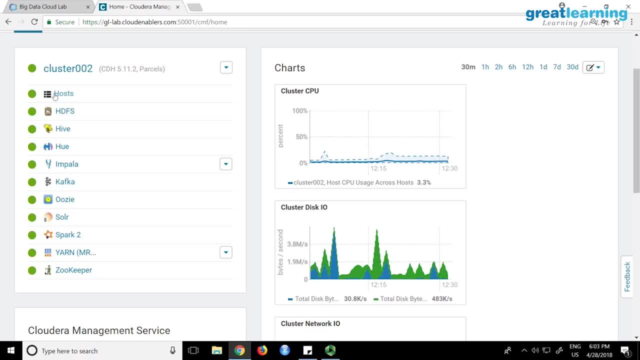 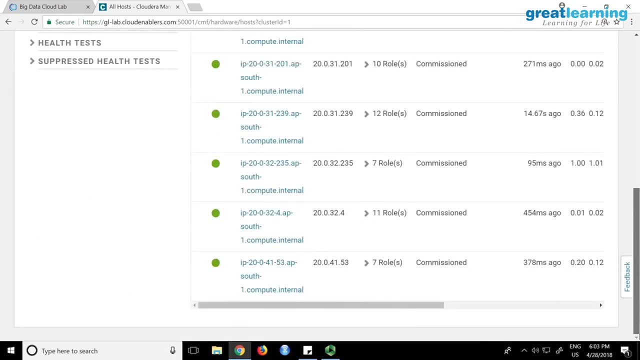 Fine, How many machines are there in the cluster? You click on this host menu, Can you see? Can you see these machines? These are all machines, one one, one, right? So how many machines are there? I think there are nine machines. 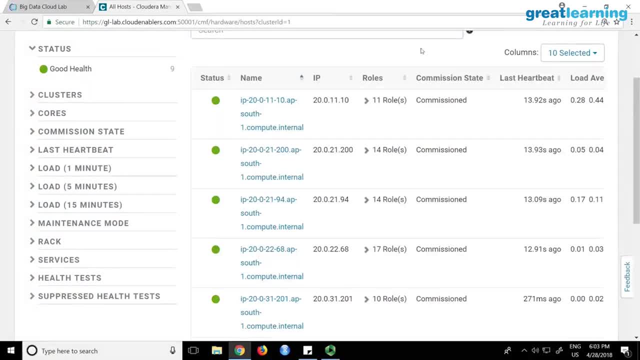 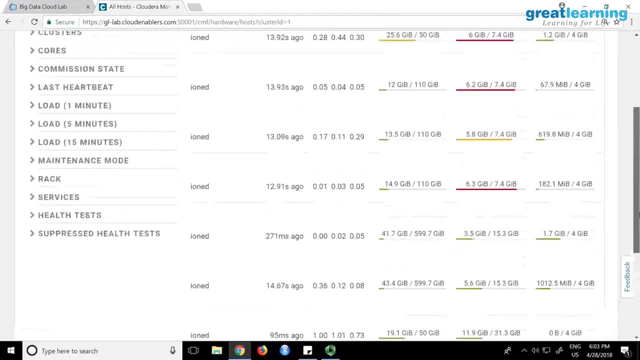 See good health. nine, Nine machines are there in the cluster And you can also see their configuration. If I scroll here, can you see their RAM and hard disk. What is the physical memory? That is the RAM. The first two machines are. 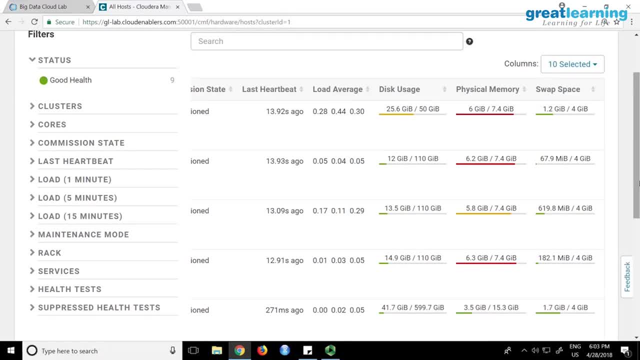 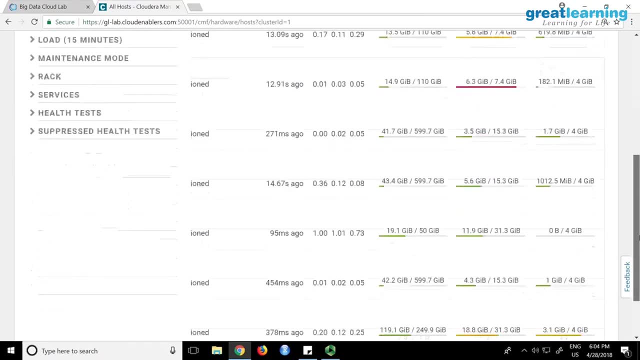 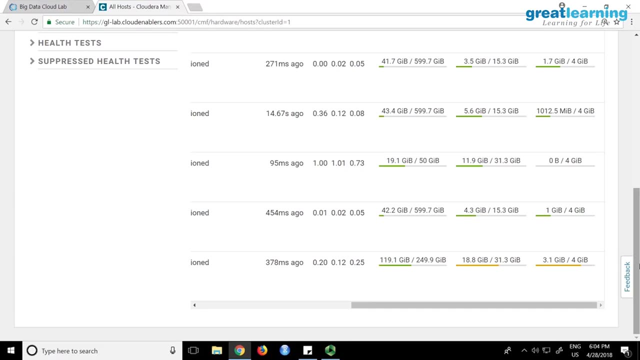 First four machines are 8 GB RAM. Next one is 16 GB RAM. These are their hard disks, Can you see? And you can see how much storage is full and all everything right, See here. So this guy is having 32 GB RAM and 18.8 is currently used. 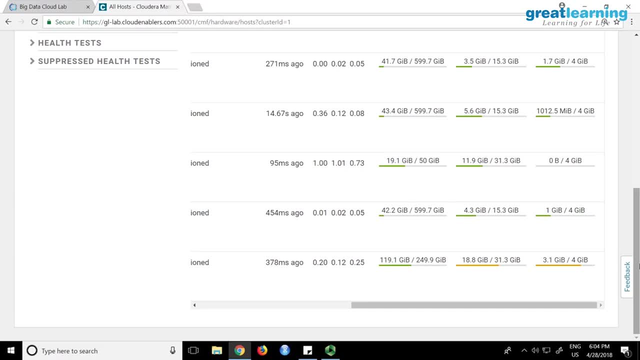 Some process will be running. This guy also had a 249 GB hard disk, 600 GB hard disk, 50 GB hard disk. You can all see from a single window. It's very easy, So it is not as complicated as you thought, by the way, 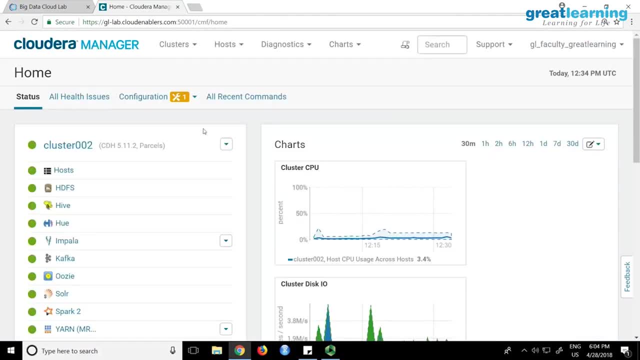 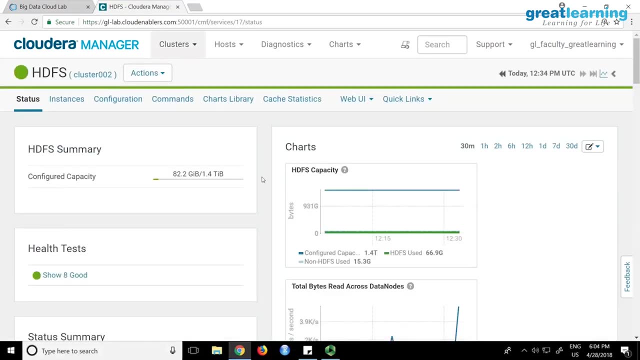 Right, So this is just the host menu. Now, if you look at HDFS, this is HDFS. Click on HDFS. You will see this HDFS menu. This is all related to HDFS. In HDFS, what we learned? replication, block size. 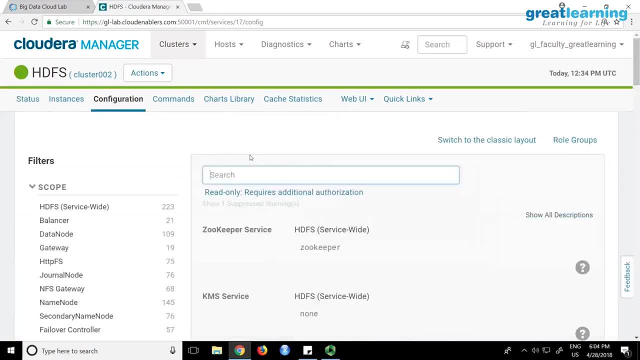 So where do you configure this? There is something called configuration, And do you want to change the see? it is saying read only. I cannot change it, But do you want to see the replication factor of this cluster DFS? What is the replication factor? 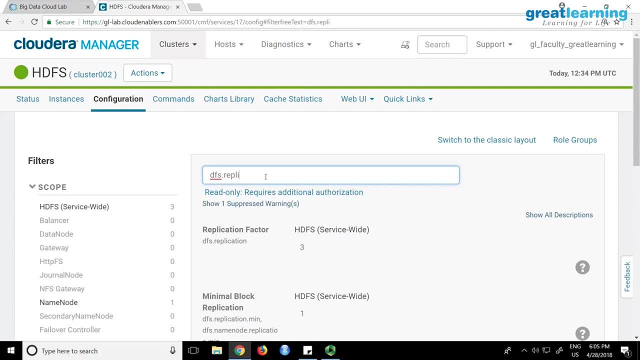 3. Click there. you can change it to 2, or 10, or whatever you want If you are an admin. you are not an admin. do you want to see the block size? DFSblockSize? So I can click here and change if I'm a Hadoop admin. 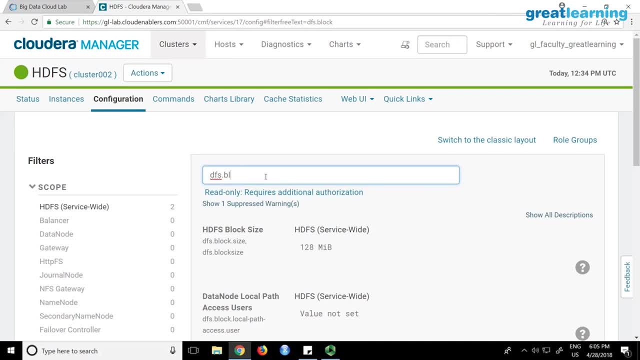 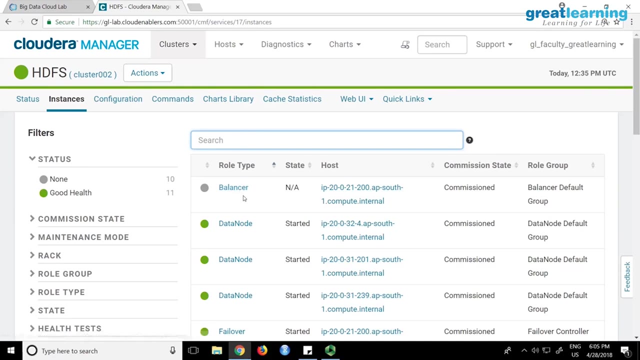 and it will be applicable to everybody immediately and all. Somebody was asking about balancer. right, Where is balancer? I can say actions. The problem is that some of these things I will not be able to run Now. this is balancer where it is running. 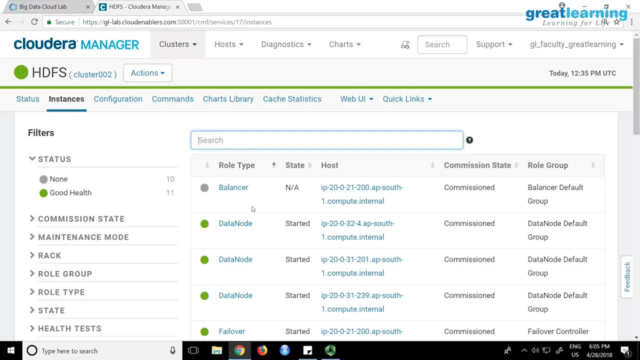 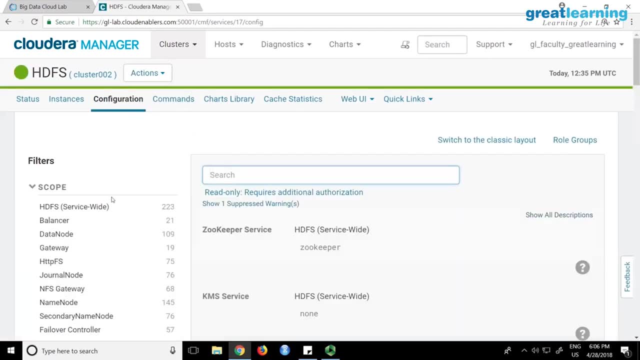 But I can run a command. It's not green, It is not running. If it is running, this process will come as green actually. Then chart commands configuration. So there is a lot of configuration. So that is one thing we saw. 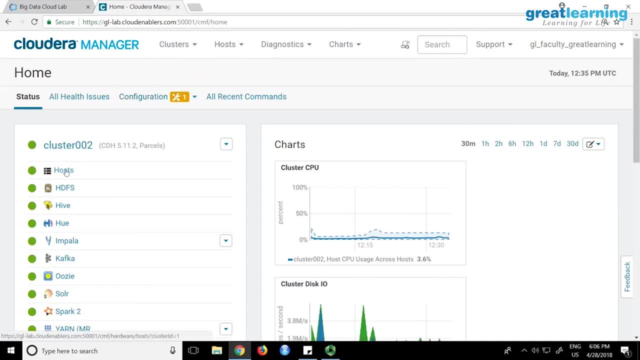 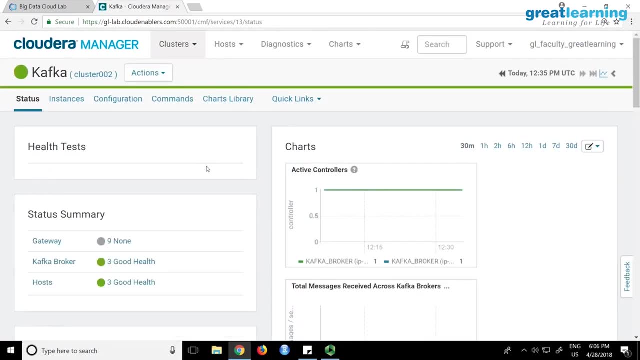 And host menu. we saw already right. So so far we discussed only HDFS. And here is Kafka. If I go to Kafka, just go to Kafka. OK, Kafka says Kafka, Broker 3.. That means three machines are running Kafka. 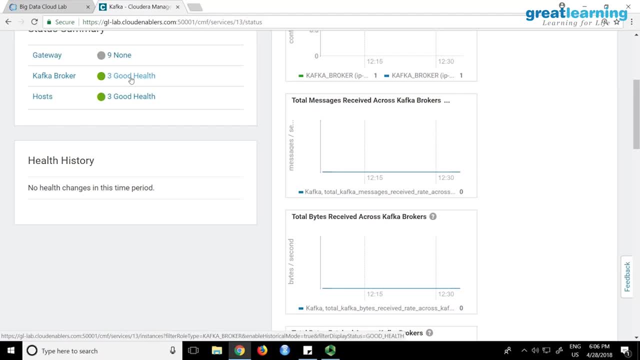 I told you Kafka will be running in a cluster. Since this is a lab setup, they are running Kafka inside Hadoop only. Ideally we run it separately Because it needs storage spaces to hold your data, But here Kafka brokers are three. 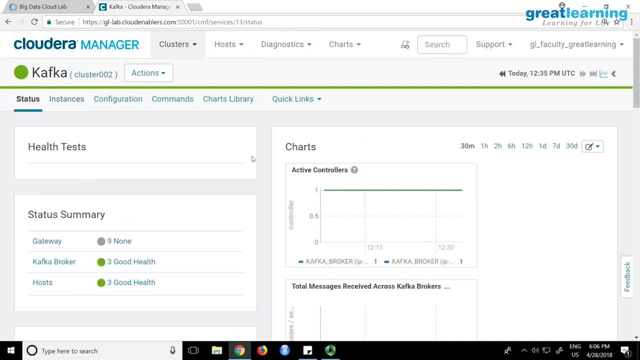 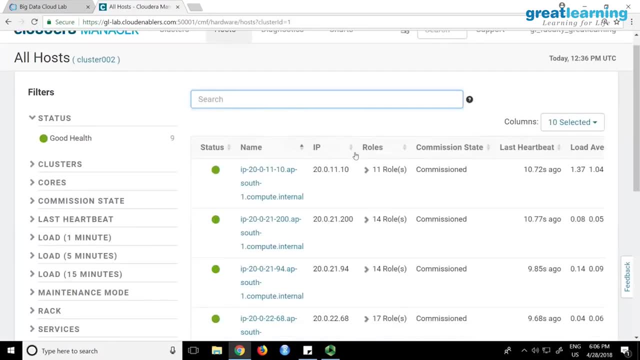 They are running inside here only Because this is only a cluster we have. I mean these machines. if I go to these machines I will show you. If you go to this host menu, you can expand a host and see what it is doing. 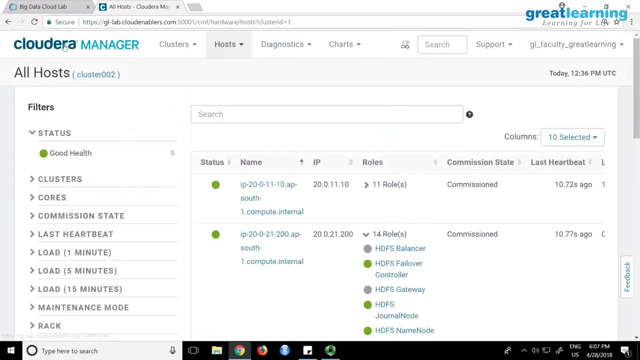 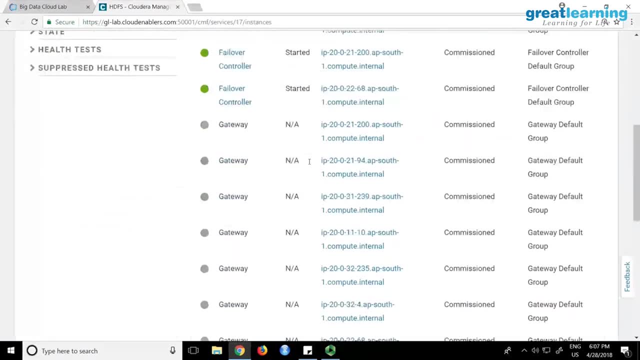 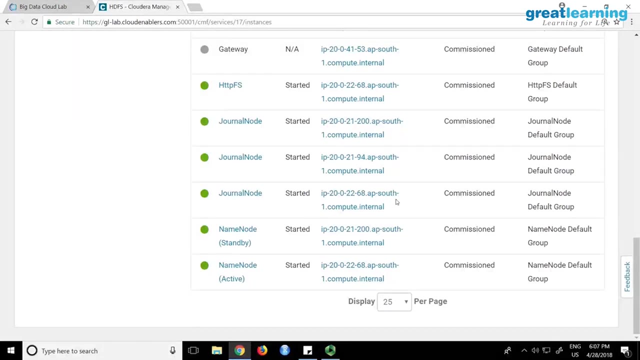 For example, if I expand this guy And also I can go to HDFS and see that, For example, I go to HDFS and instances. What do you see here? Active standby, two machines, two name nodes, I told you right. 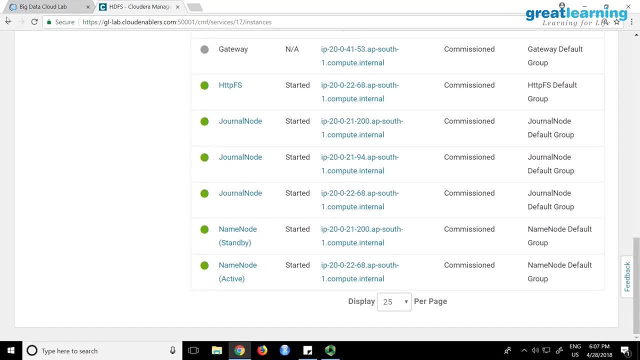 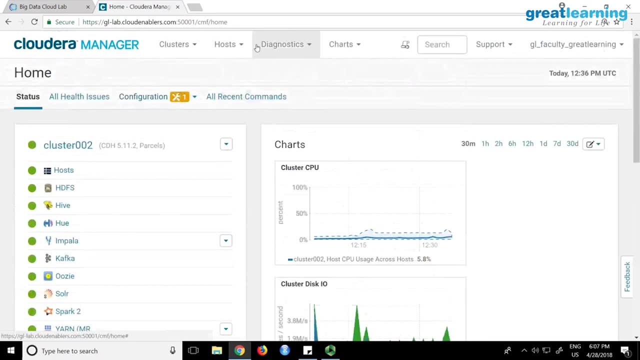 Active and standby. they are running right. So the same machines are running Kafka here. It's not a separate cluster, by the way. That's what I meant by that. I don't have really admin access, Otherwise something could have been done. 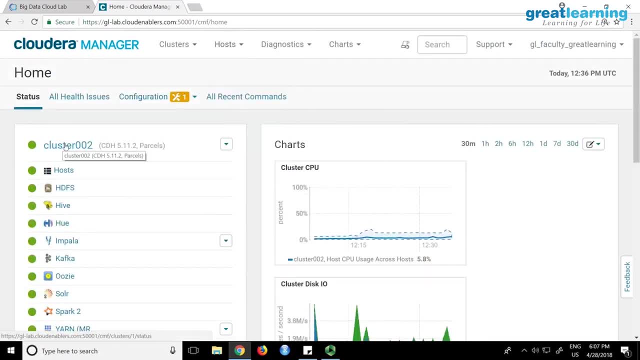 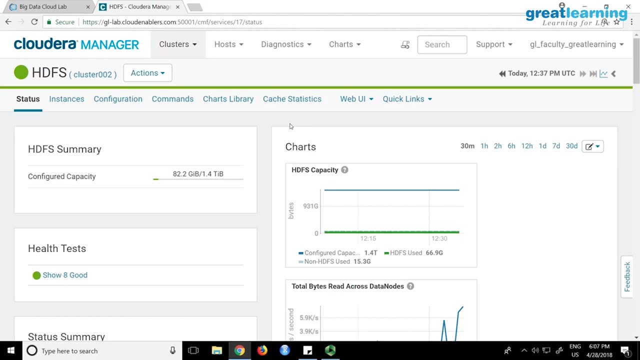 I don't want to mess up the cluster also, by the way. So some of the menus are actually disabled. We can't run them. Ideally that should not be the case, Because then it is not utilizing the proper space right. 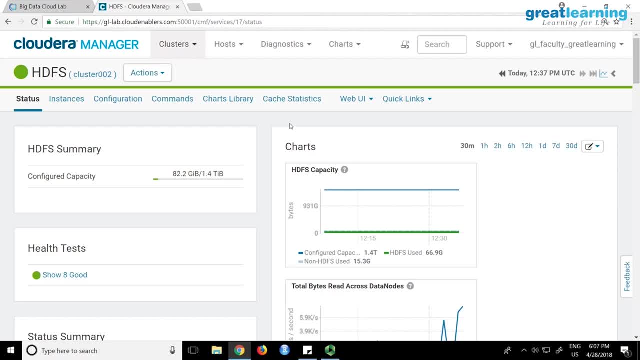 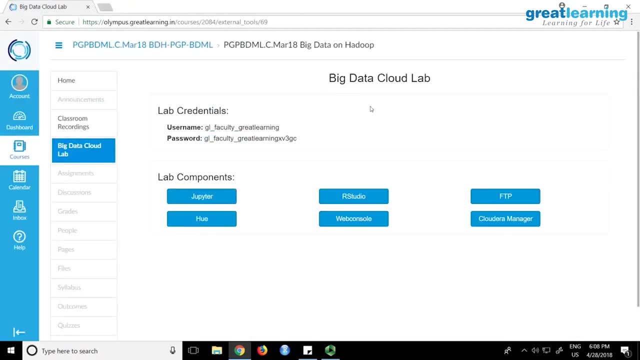 So ideally, you will set up a separate broker And that will download the data. actually, They are all running on AWS. I want to clarify one more thing. If you go to this big data cloud lab, this cloud data manager, you don't really need. 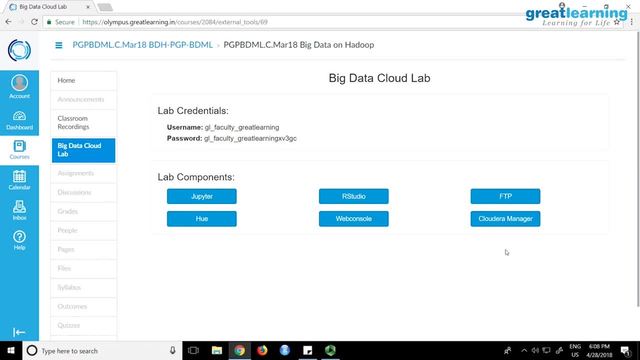 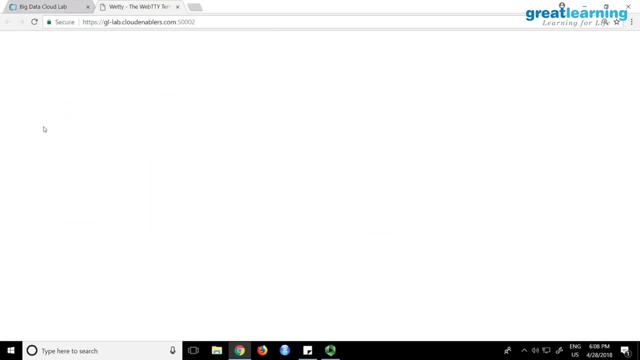 Because that's the admin interface. You're not going to do any admin. You're going to do any admin activity. The important thing that you need is web console. So if you click on web console, I just clicked on that And there is a product called Hue. 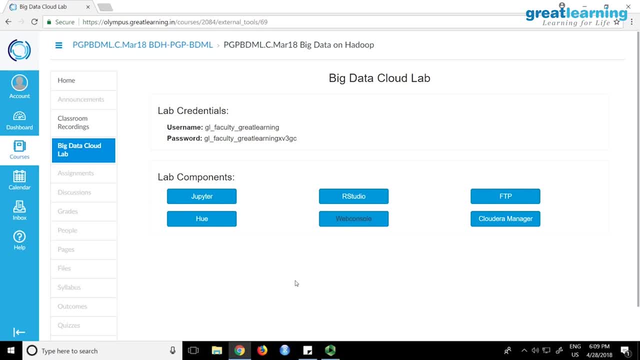 This is very important. There is a product called Hue. This Hue is a third party application, But it is very, very popular. Why do you need Hue? is that if you're a developer and you want to upload your files to Hadoop? 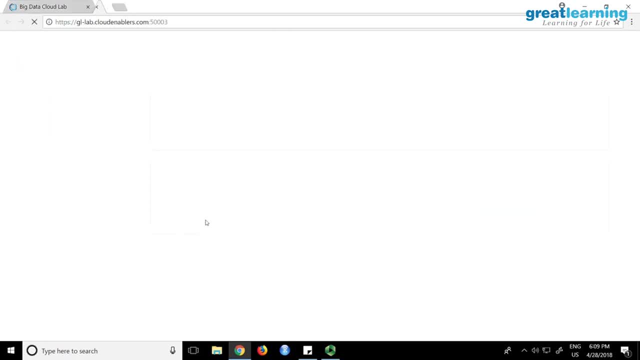 you can use Hue, one of the use cases. For example, I can click this, I'll click Hue And last the username and password. If I sign in, I'll just sign in If I click on this HDFS browser, see there. 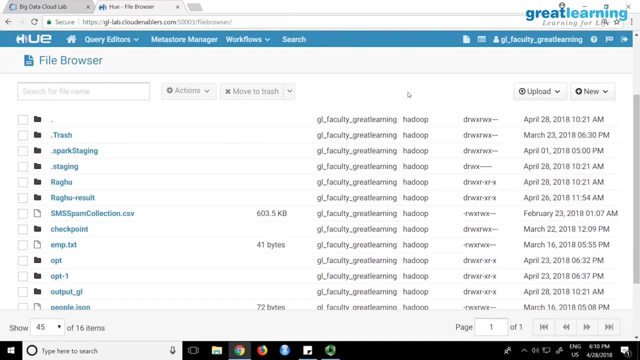 This is my Hadoop. These are all the files in my Hadoop. So Hue is like a web UI to the Hadoop HDFS file system. So these are all the files and folders. If you connect you will not see anything here. 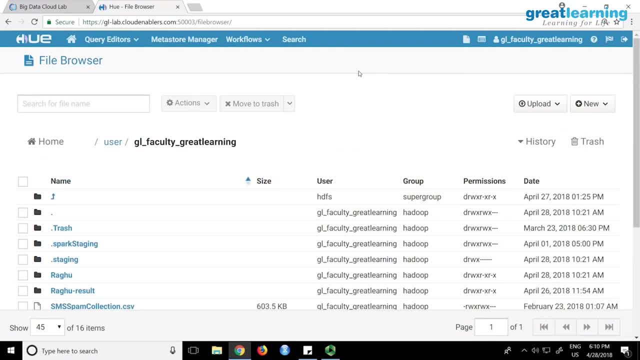 Because you are having a fresh account. One more, A very important point I want to tell you is that in Hadoop you will have a home directory- user slash- something I have, GL faculty- You will have your own directory. Can you try this Hue thing on your PC? 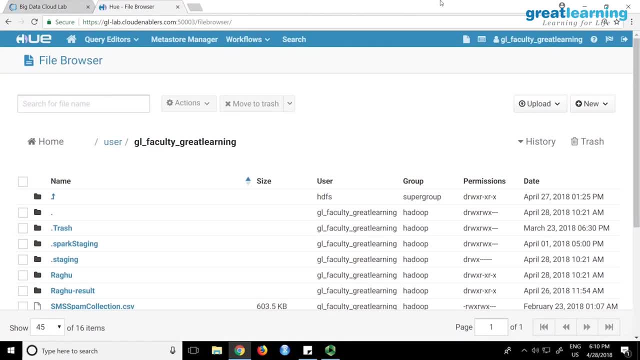 Just click on this Hue type username password. See whether you can see this thing. Another point is that sometimes the cluster will become very slow Because it is not designed to accept requests from 36 people. If all of us try to log in, it will say timed out. 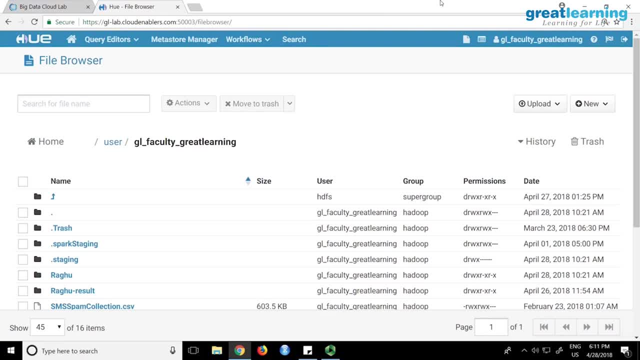 and other things. So different, different users are created in the Hadoop cluster. So if you log in, you will get a home directory, like in Linux. In Linux, what happens? if you log on, you will get a home directory. 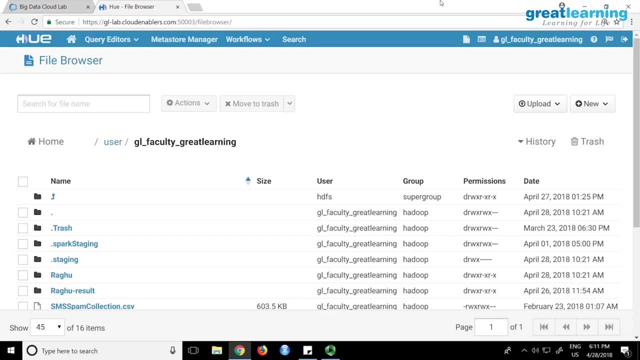 So this is my home directory in HDFS And since I already created some files, I can see them. You may not be able to see because it is a fresh home directory for you. Now it will be in a non-commodity hardware. 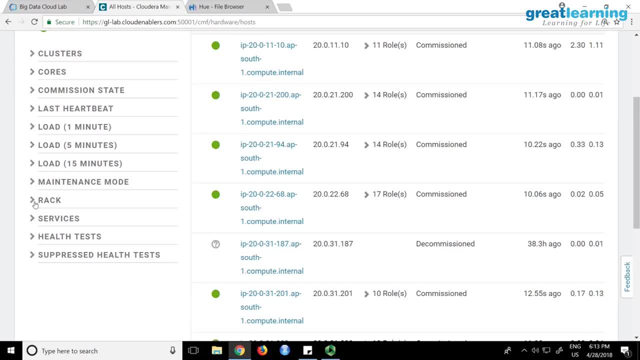 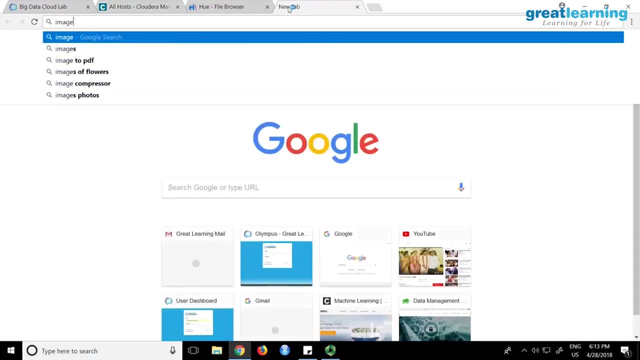 like a real server. You know what is a rack- Server rack, Because from the point of view of Hadoop, this might be It's a server rack. This might be important. I will explain this one and then pick up your questions. 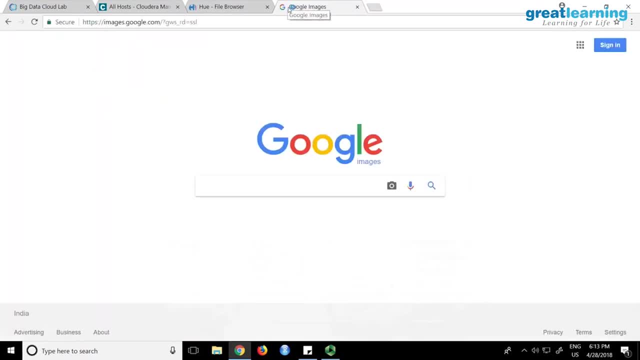 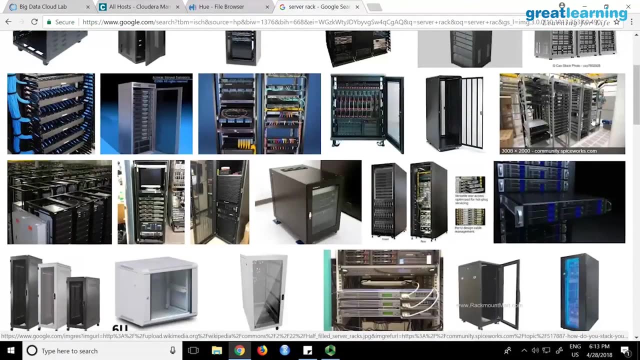 Majorsgooglecom. So this is for people who do not know Server rack. Do you know what is a rack? now, This is a rack. It's a housing where you push all the servers. In all the hi-fi movies you will say: 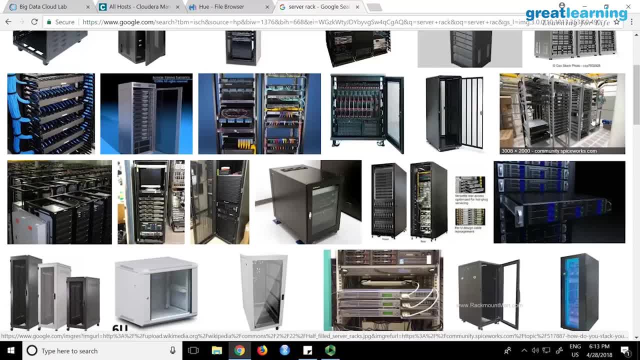 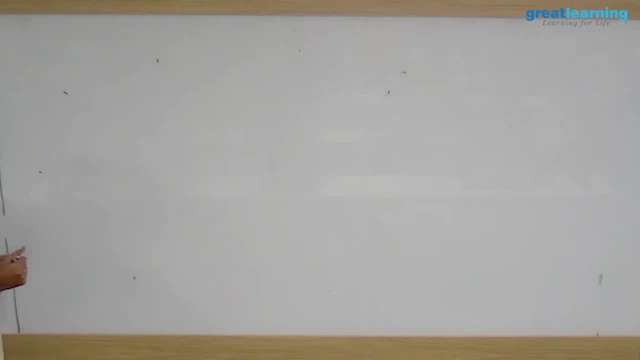 somebody's eating something, typing something in a very big data center, and all right, So that's a rack. Why racks are important? They are important for one reason: because, let's say, you have three racks, You are having three racks. 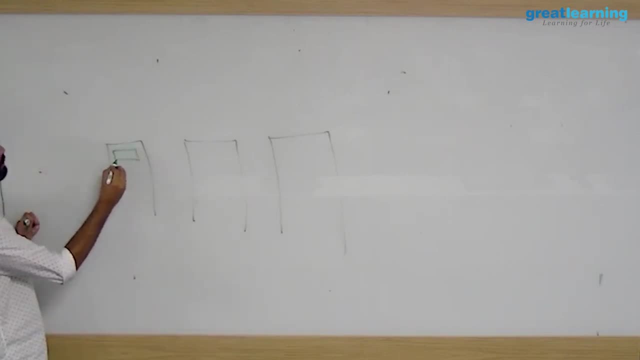 And each rack has a data node, Not one. There are many, So let's say, two data nodes are there. So, In reality, when you are installing Hadoop in a cluster, this is how you do it right, Because in a data center you will have racks. 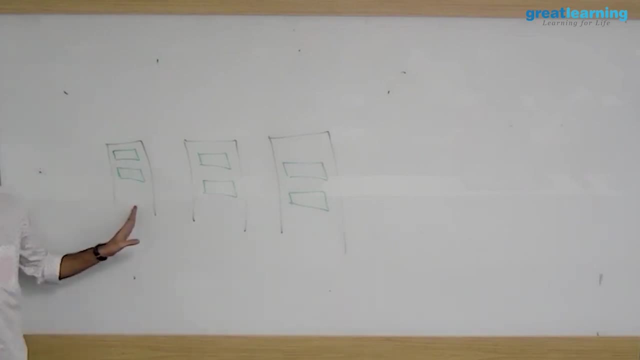 and you will have servers. These servers are called your data nodes, right? So I have six data nodes in three racks. Now there is something called rack awareness in Hadoop, meaning if let's say you are copying a block, what you can. 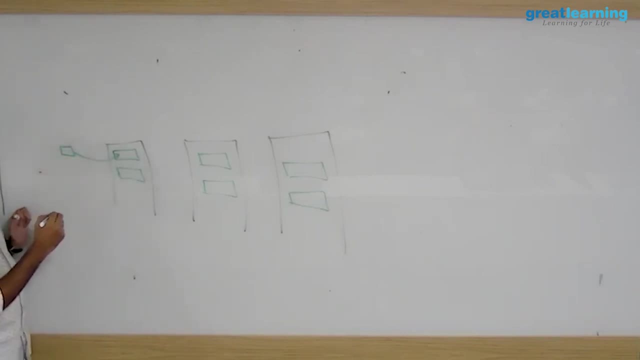 do this. first copy will go here, Second copy will go here. Imagine, And the third copy will go here. Meaning, if you enable, this feature called rack awareness Hadoop will ensure that the blocks are spread across multiple racks. Why: 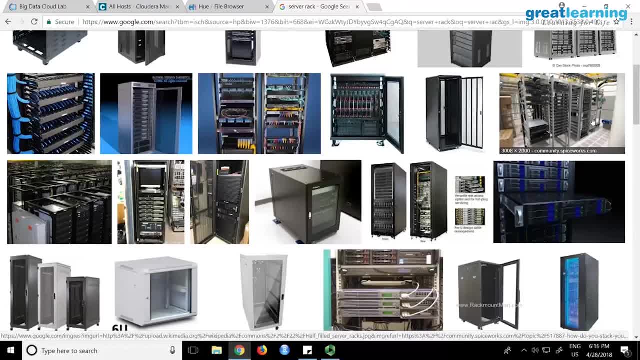 A rack is a point of failure because normally you will supply this power and network everything through rack. So if a rack fails, if I'm keeping all the three blocks in the same rack, if that rack fails, then my blocks are gone. 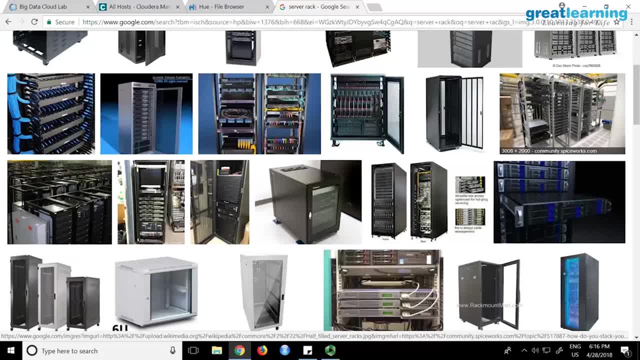 So Hadoop can. if you enable rack awareness, you have to tell Hadoop which data node is in which rack. If you do that, it can place them like this. But why don't it keep all three in three different racks? Why the rest of the two copies are in the same rack. 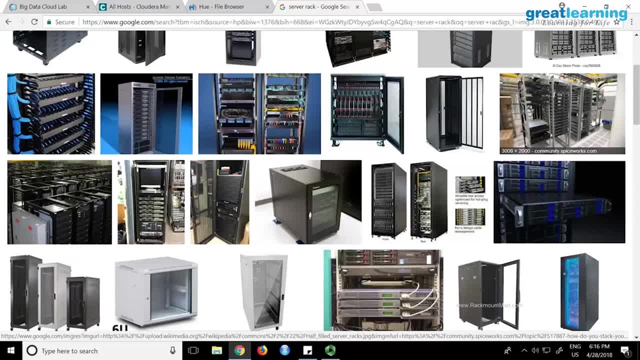 But same location means these are all in the same data center, right? So this inter-rack bandwidth is very important. Rack to rack the bandwidth is very important. So this is just replication, Right. We're using a lot of programs which will use this bandwidth. 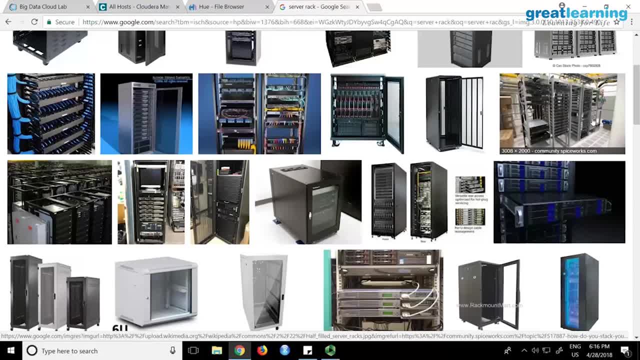 So to save that bandwidth, what it does is that the next replication will happen within the racks, server to server. But this is enough Now, even if one rack and all the three racks going down is very remote possibility, And my point was- I can show you that here. 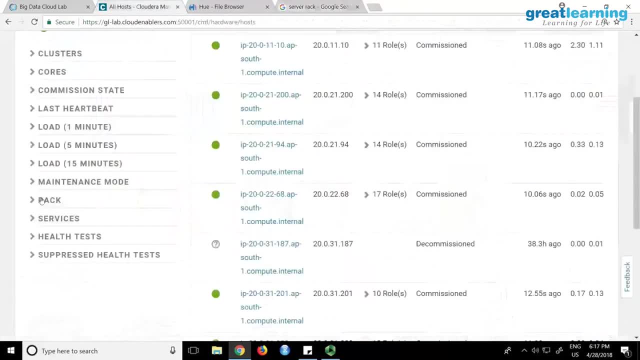 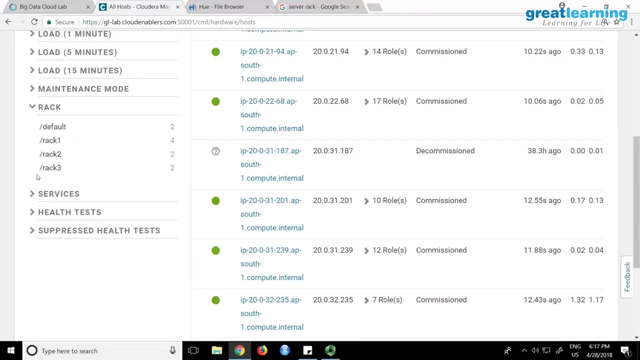 So when I saw that, if you go to all host, can you see this? So in the rack one, four are there, Rack two, two are there, Rack three, two are there And default rack two are there. Default means I don't know. they have kept something here. 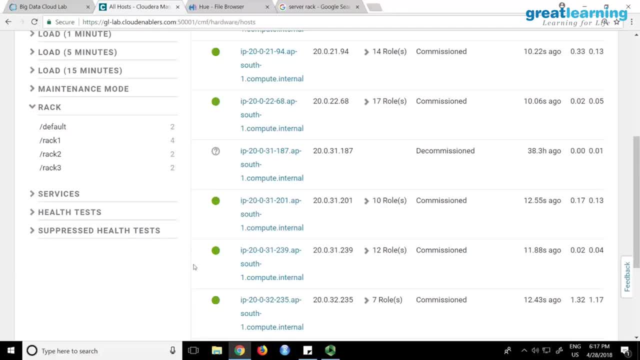 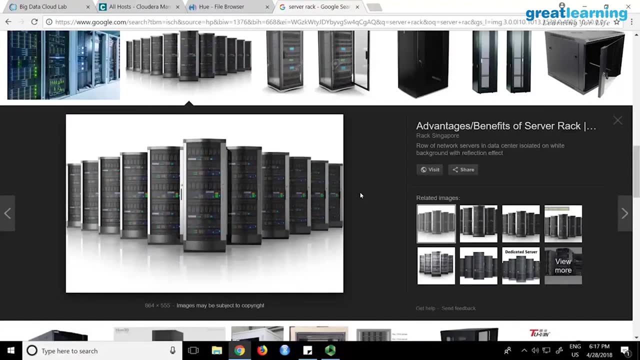 But four, two, two. So this is actually the distribution. It is actually available in your Cloud Data Manager. See, if you look at this picture right In this machine, some 30 data nodes will be there. Each slot you'll have one server. 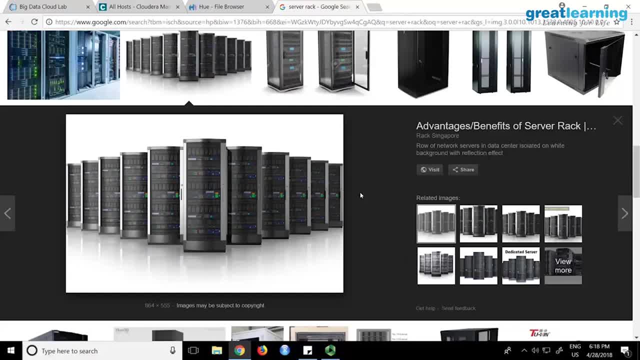 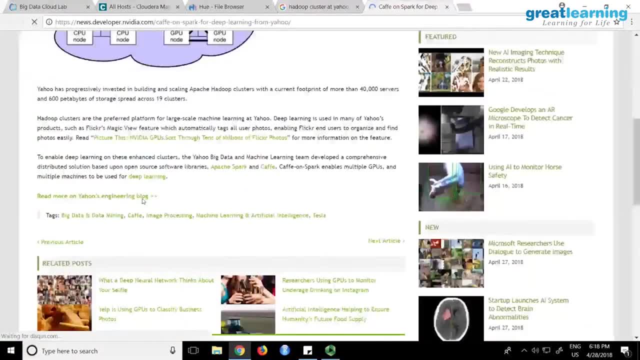 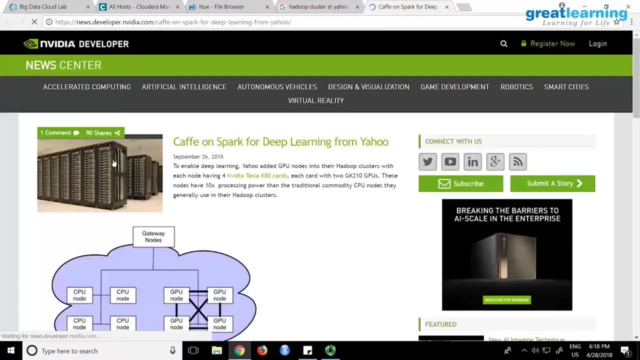 They are all rack server, So server is not like this, It's like this. So the biggest Hadoop cluster on Earth is with Yahoo. actually, Yahoo holds the record for that. They have 42,000 machines And still they went bankrupt, sold it to some useless company. No, that's a good question. So can I have multiple name nodes? Yes, The concept is called federation, meaning ideally, if you cross more than 5,000 data nodes, you need one more name node. Like 42,000 machines, I cannot have a name node. 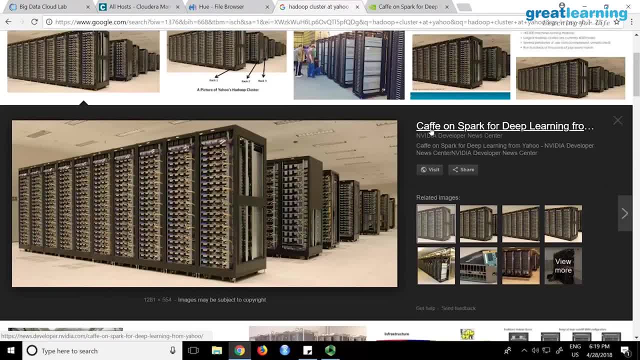 I cannot have a single name node to handle because the amount of metadata will become slow. That is a problem, So ideally, Yahoo has done some R&D. They said that if you cross more than 5,000 data nodes, you need one more data node. 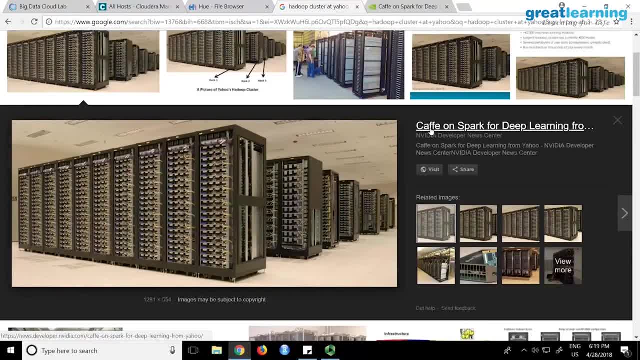 That's called a name node, That's called federation. Federation means multiple active name nodes. Like you can have 10 name nodes, all will be working. They'll share the load, actually, right? So like that, Federation is called it. 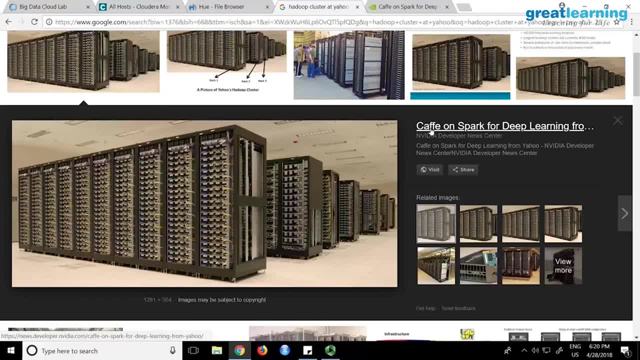 All in one rack. actually, you can put it Inside the same data center, only you need all of them, right? So that's the idea, Because all the data nodes are in one LAN, so the name node also should be inside that. 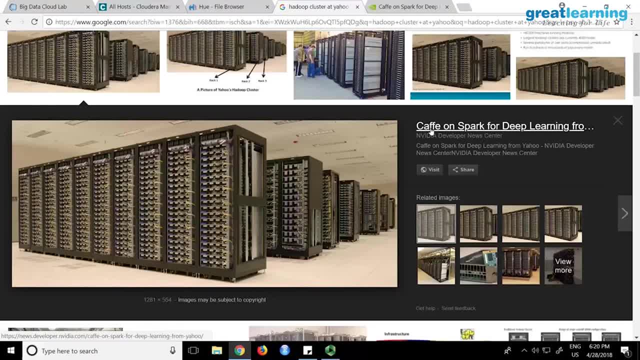 only, But they will handle the load actually. So some data nodes will be this name node and all They can handle load. File server can store, but it cannot process right. That's the use case. Hadoop is not only for storing. 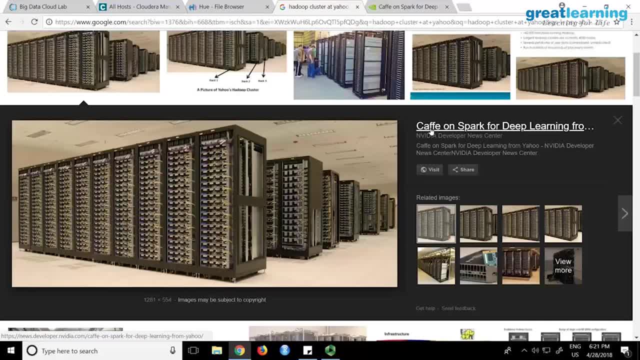 Whatever data you store, the data can be processed then and there by the machine. So there we are not using Hadoop, right? We discussed it in the beginning of the class. No SQL database. If you don't want processing, if your use case is such that I just want to dump a bunch, 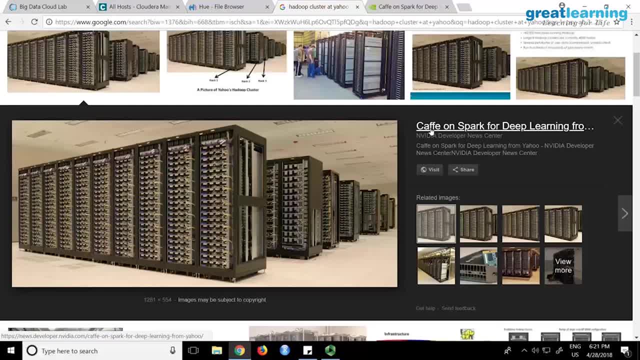 of images- let's say 1 million images- I just want to process and display in an e-commerce website. I don't use Hadoop. Hadoop is not used for that. There you have no SQL databases like DynamoDB or MongoDB, right. 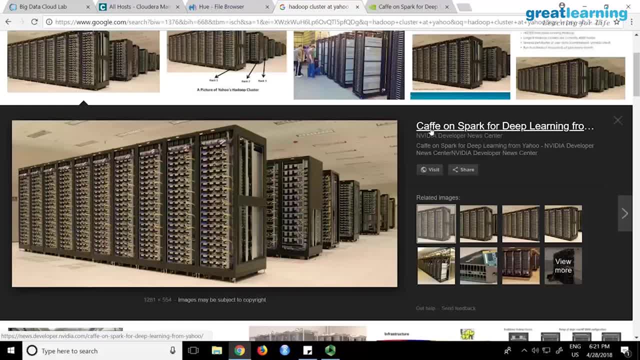 SharePoint. If it is a smaller setup SharePoint you can use. So it is all business use case. The question is that: what do I want to do with the data? There are other companies, Other companies who generate terabytes of data. they just archive the data. 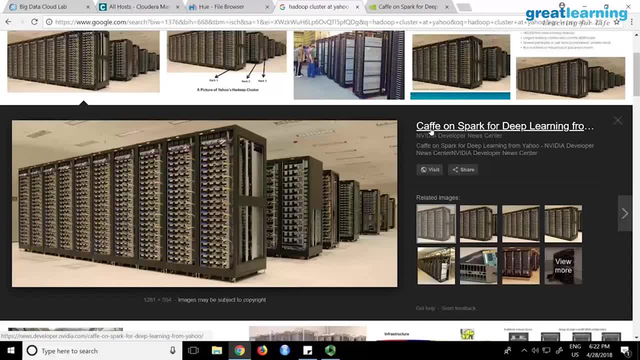 I just generate data. I don't want to analyze, I just archive the data. Who cares? So it is up to me to decide. what should I do with the data? right, I was working with GE- very interesting use case, GE right. 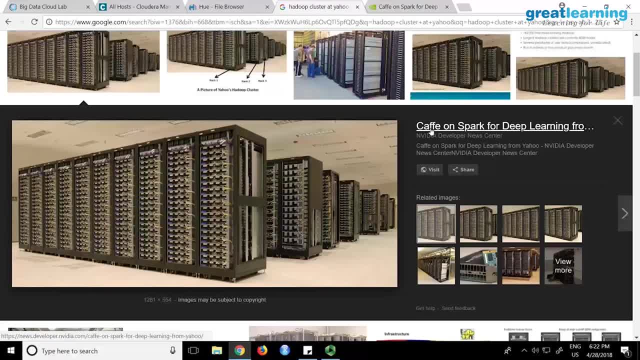 The company called GE. I have a training next week there, So they have an aviation department. GE is building this aircraft engine. you know that Flight engine- Eighty percent of the commercial aircraft engines are from GE And what they do. 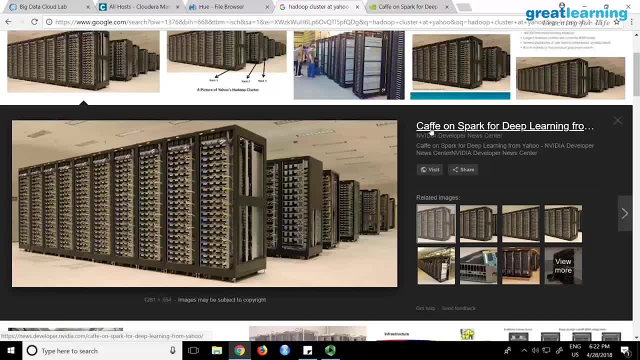 So they have an aviation department. So most of the planes are flying with GE engine. There is also Rolls-Royce and one more company, So all these aircraft engines are having sensors. So when the flight is flying they capture the sensor data like pressure and blah blah. 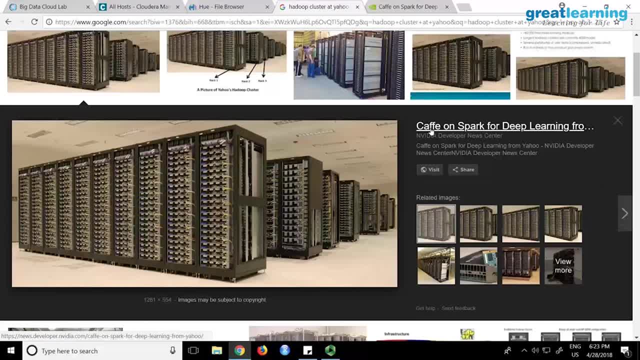 blah And they analyze it to predict when the flight will crash or turbulence will hit or something like that, whether you're going to die or something. So the idea is that. but so I said, okay, good deal, you're doing this. 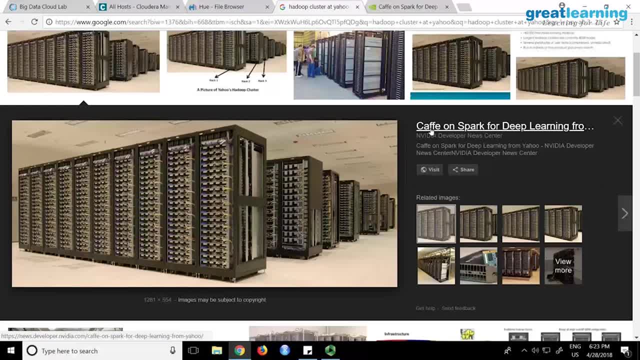 They said, no, it's not a good deal. The problem is, if a flight is flying from, let's say, a plane, It's not a good deal. If a flight is flying from, let's say, Dubai to Bangalore, there'll be two engines. 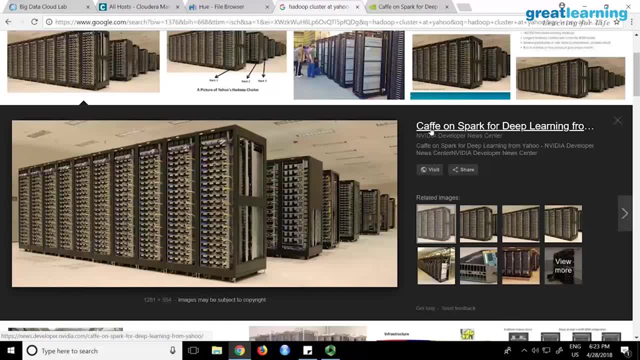 It takes six hours. Each engine will generate one TB data. How many flights are there in total and how many flights fly every day? Can you imagine the amount of data They don't analyze? How can you analyze, I mean, if I'm giving you, let's say, a thousand terabyte every hour or every minute? you can't. 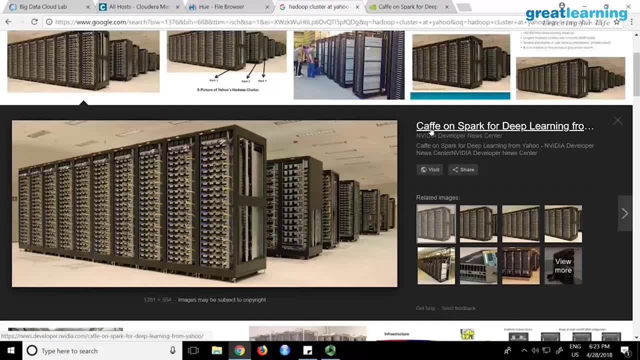 analyze it, So they take a subset of it. They have an algorithm which takes a subset of the data and analyze. The rest they delete and dump Because it is not humanly possible. Also, you don't need that much amount. Every sensor data need not be analyzed. 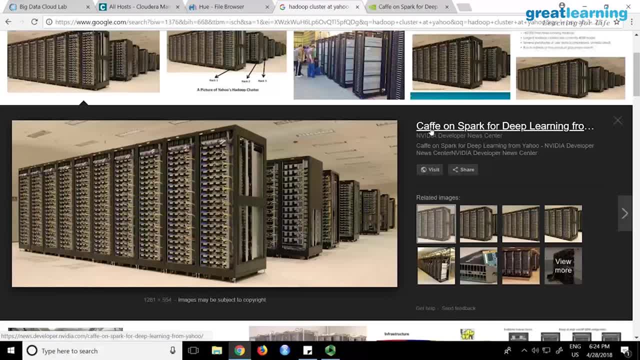 These are interesting because they also have locomotive engines, train train. All the Europe and US. they run trains And these trains are having sensors, So they get also that It's very difficult to work with GE because huge amount of data. 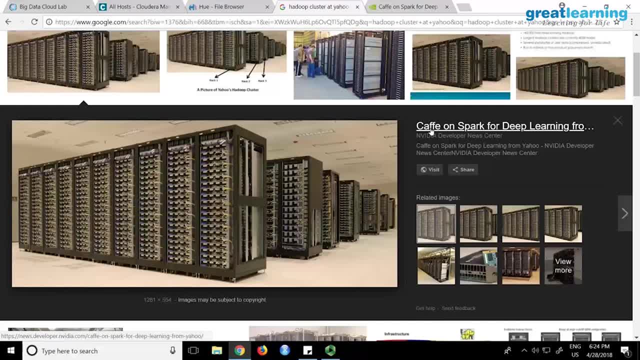 They also don't know what to do with the data right, And they have no clue how to make sense of the data. Locomotive data is huge actually, So the trains will generate a lot of data, Okay, Actually, so they get it, and then they take it and clean it and just get only a part of 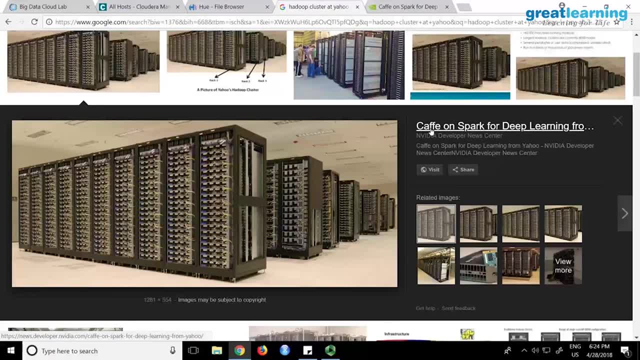 the data and they analyze it. In Hadoop you also have certain file formats, for example Avro. You may not have heard about it. Avro is a file format we use only in Hadoop Parquet, ORC. 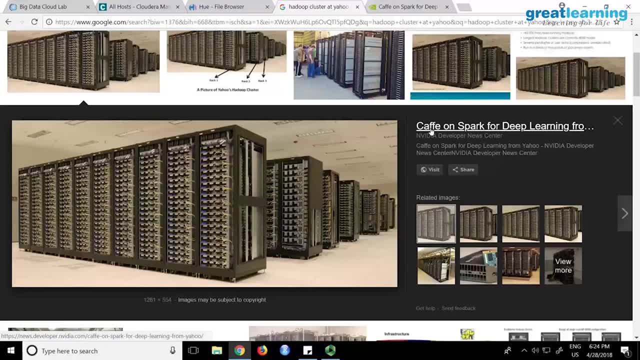 These are all used to compress and store your data. in Hadoop You can also have compression techniques, because sometimes storing the data as it is stored as it is, is not good. Why don't you compress it? But what is the drawback of compression? You have to decompress. You need a lot of processing power if you want to decompress it. So Avro is a serialization format. It doesn't compress the data. Parquet and ORC will compress the data columnly and push the data. 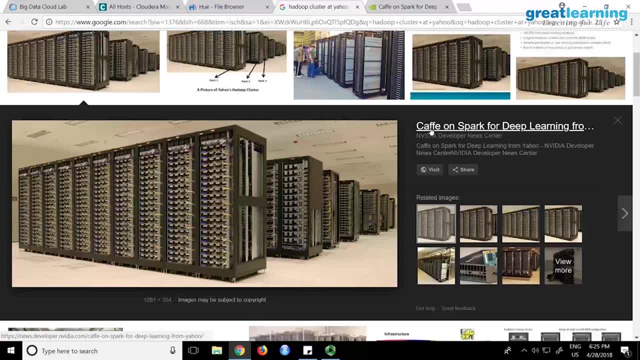 So I will show you in Hive when we discuss Hive. When you create a Hive table, you can say that the data has to be compressed. You compress and store the data. So my point is: not everybody wants to analyze all the data in the world. 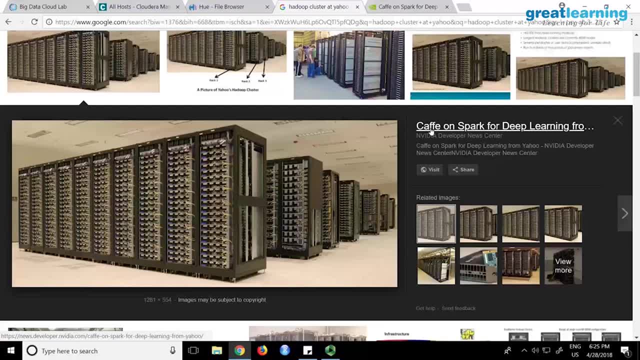 That is also humanly known. Think about Facebook. how much data they will be getting. Probably they are not analyzing the whole data. a subset of interesting data. That is all they will be doing. Yes, Spark is memory intensive. Ideally, Spark requires RAM. 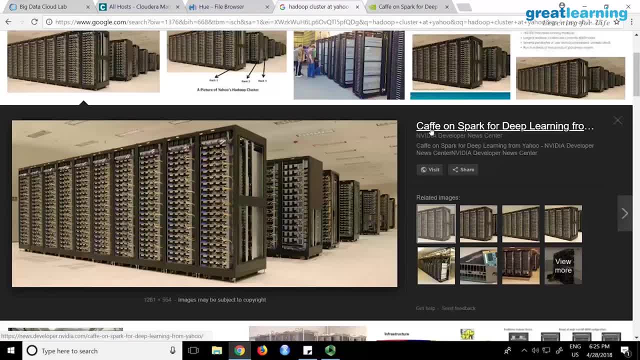 So if you give RAM, it will perform better. If you don't give RAM, it will use hard disk. I mean the rest of the space it will use hard disk performance will be slightly degraded. So for streaming and all, We need a lot of RAM. 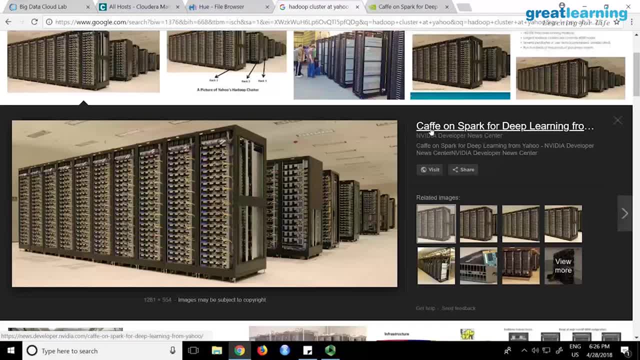 The problem is Football World Cup is going to happen, right? So let's say you want to write a program which will download all the tweets and find out the most favorite player for Football World Cup possible, right? So I can easily stream the data from Twitter. 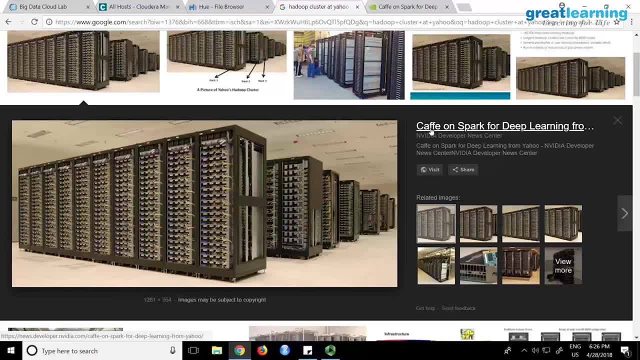 The problem is, I want to find out. you know the most popular player every five minutes? imagine, Probably not five minutes. you want to do So. I want to get five minutes worth of data. hold it in my memory and process. 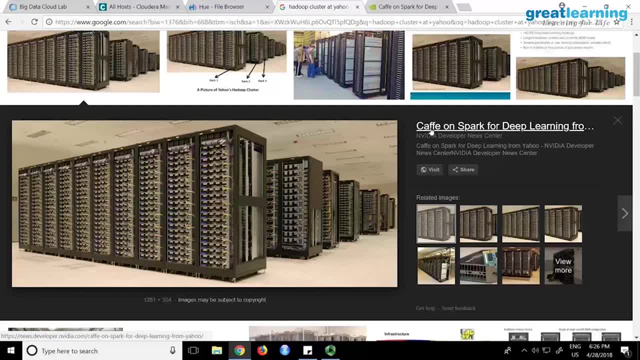 What if five minute data is so huge I cannot hold it in memory. then it will be slow. Yes, I'm just giving an imaginary situation where if five minutes worth of data is in terabytes, you can't hold it. actually, Not only Twitter, any data that you have. then you might want to process into disk some. 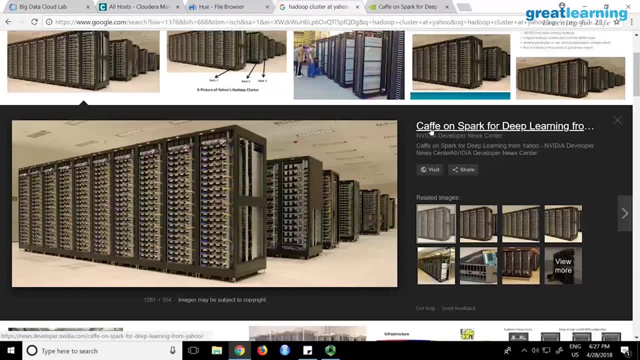 of the data, then processing will become slow. it is not real time, So when you are running Spark, streaming and all you know, your RAM should be available, Otherwise it will become slow. Today's match: you will predict tomorrow, right? 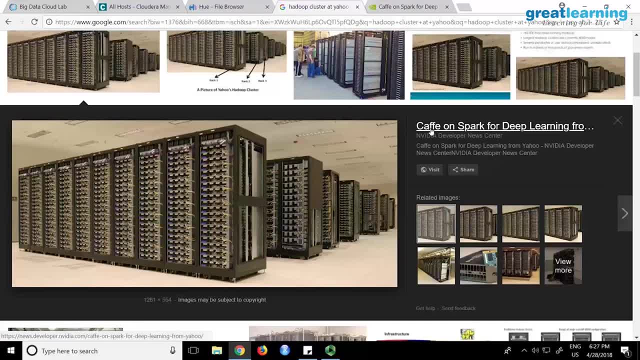 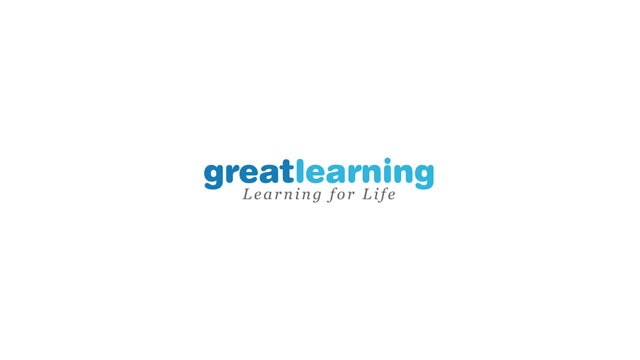 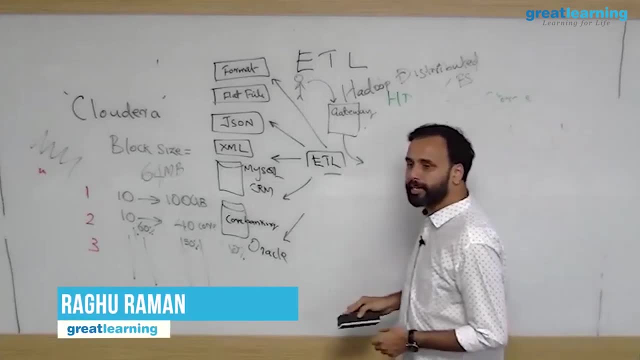 So things like that can happen. So that's not really good actually. So a lot of considerations are there where you have to use all these things They don't use. if it is a bare metal virtual machine you can guarantee there are two types. 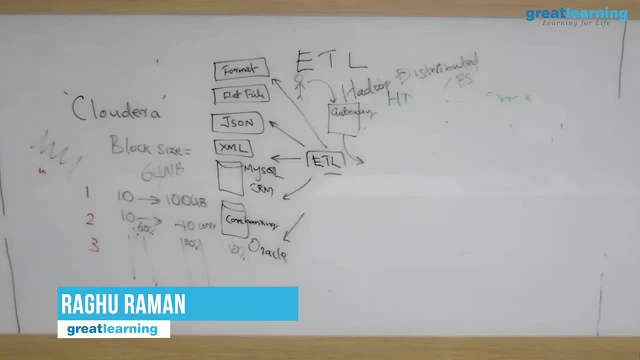 of VMs. right, There's something called bare metal, like a Hyper-V and all. there you can get good performance or VMware. If it is not a bare metal, no performance will be compromised because again you have to go through one layer, then talk to the storage and all. 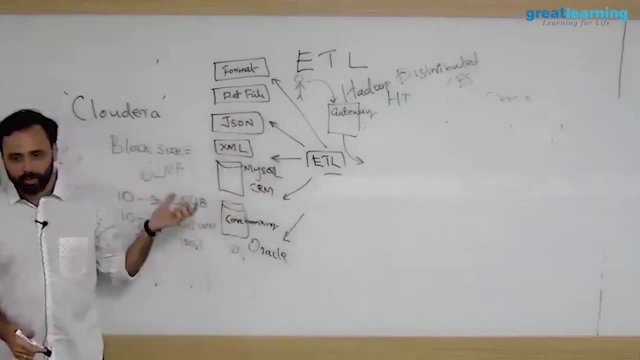 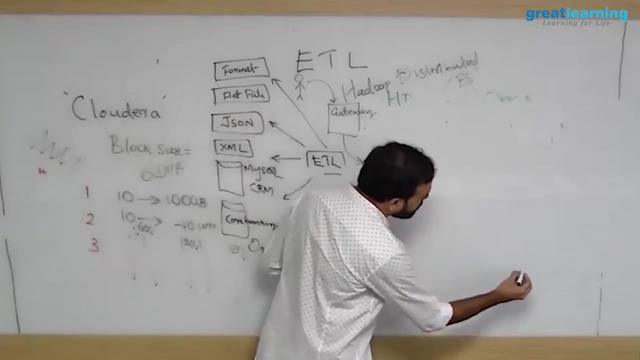 So I'm just taking this ICICI use case so you guys will understand better. So traditionally we do something called ETL to bring the data right. And now what we have? we have this Hadoop. So I'm just writing here: HDFS. 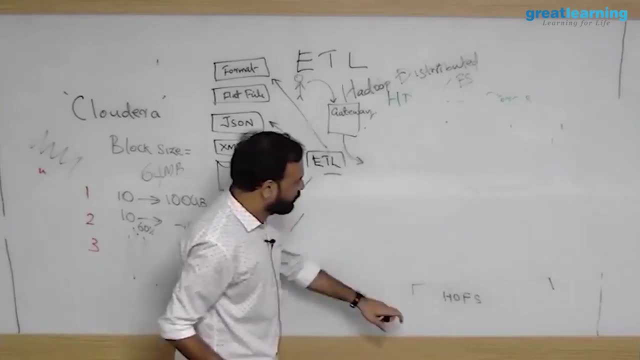 So this is your HDFS file system. This is HDFS And in the world of Hadoop, we very rarely do ETL. Why? Because ETL means you are reading the data, transforming the data and dumping the data. If you are getting big data, transforming it on the fly is very, very difficult actually. 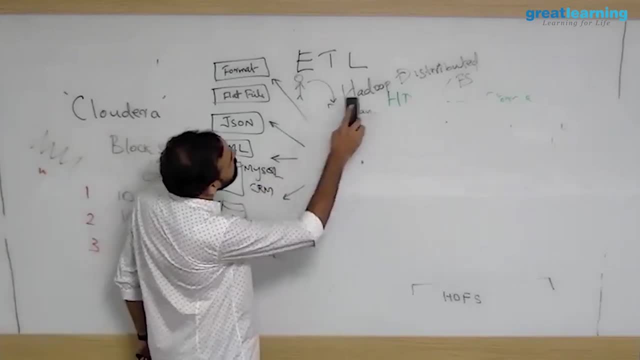 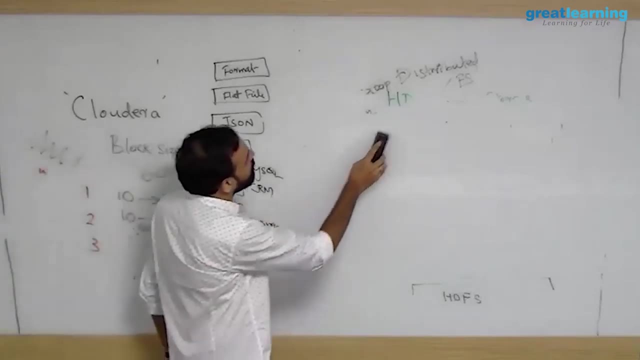 So in the world of Hadoop, what we do is something called ELT. instead of ETL you will do something called ELT, that is, extract, load and transform. So first thing is extraction. How do you get the data into a Hadoop system? 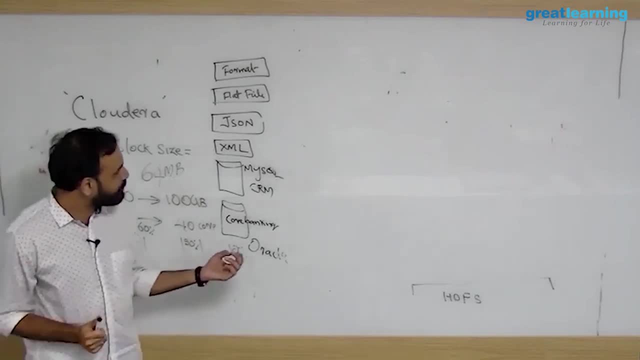 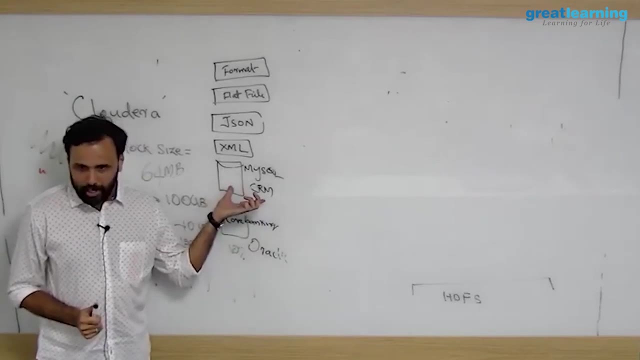 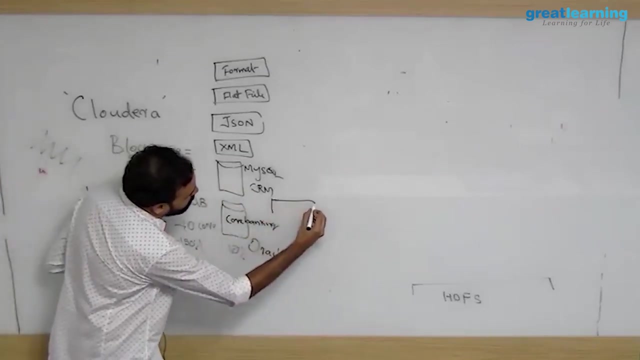 So there are multiple tools. First of all, if you are having structured data, say, you have data in Oracle, you have data in MySQL, So this is all structured data which understands SQL. There is a tool called Scoop. There is a tool called Scoop. 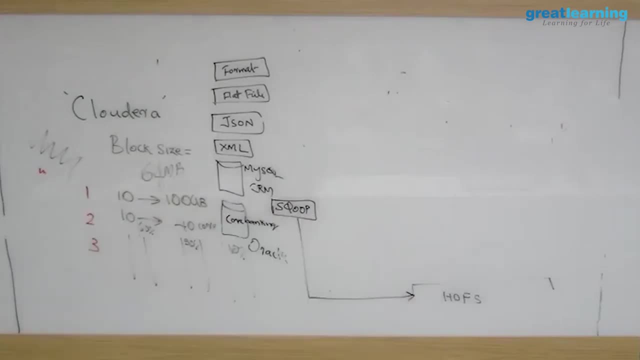 Scoop can get this data to your HDFS. You can't call it as an ETL tool. Scoop is used to bring the data from any Hadoop, So this is a tool called Scoop. Scoop is used to bring the data from any Hadoop. 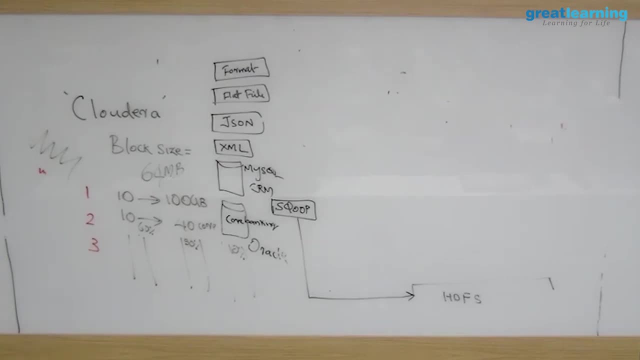 It can bring SQL system to Hadoop transfer the data. So what is going to happen? when you say that you want Hadoop from Cloudera, Cloudera will give you Hadoop. On top of that, it will give you all these tools, which I'll be explaining now. 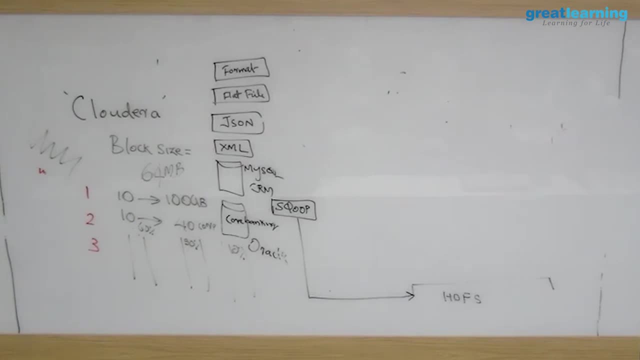 So Scoop is part of your Hadoop ecosystem And Scoop is used to bring data from SQL stores. It can take from, let's say, Oracle, It can take from MySQL, But it cannot take from Flatfile JSON. nothing, nothing. 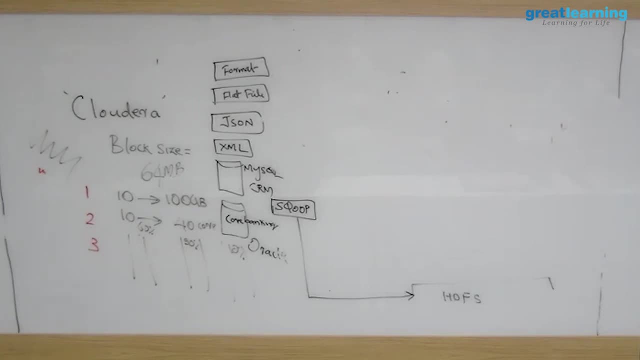 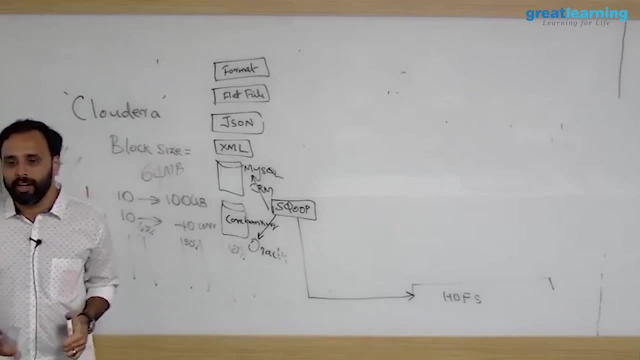 Only Python. But it cannot take from Flatfile JSON nothing, nothing, Only SQL, Only places where SQL understood. So from ICICI use case we got all the data from CRM through Scoop to Hadoop. So Scoop is an Apache, a tool. 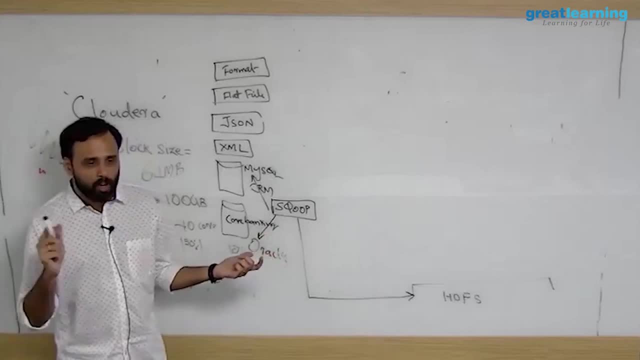 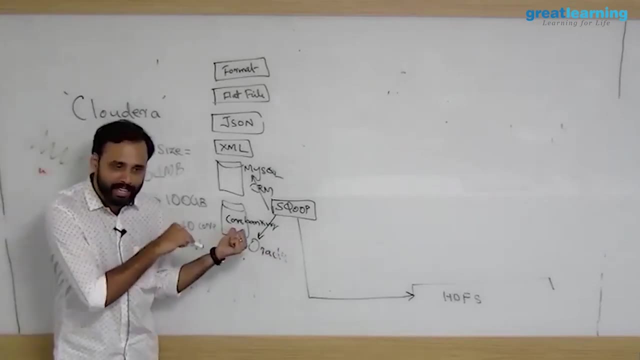 It is a very lightweight tool. We faced a problem there and I wanted to discuss that. Let me ask you this question: This is ICICI banks core banking Oracle database. Do you really think they will allow you to touch it? Then how do you get the data? 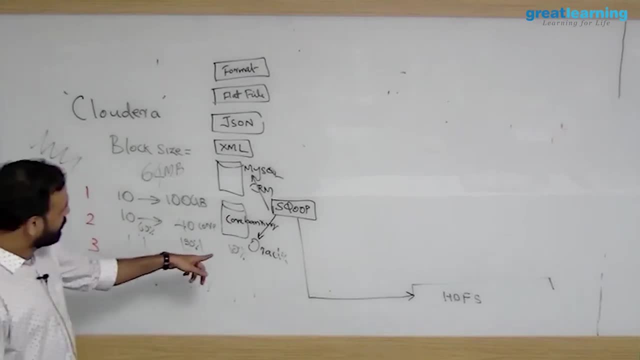 CDC change data capture, So we face the same problem. There is GoldenGate. Oracle has a solution called GoldenGate. So CDC change data capture, meaning they will not allow you to touch it right, So they will have some replica solution. 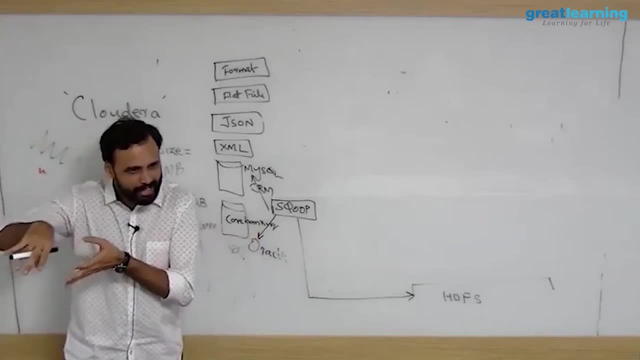 So where they will write it into a replica DB. it's actually a log file From there. you have to capture and get it. They won't allow you to directly touch their Oracle DB by any way. It's called CDC- change data capture. 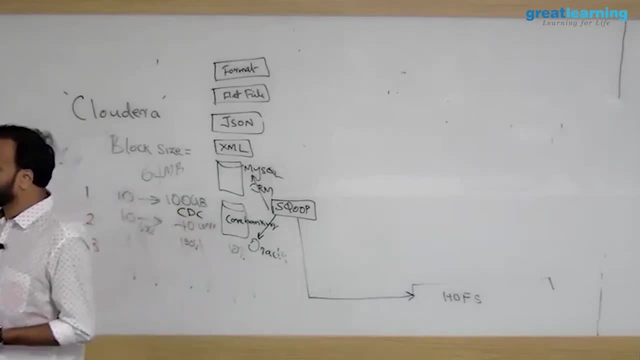 No, that will have only the delta. So what they will do, they will give you the original data, backup data they have. The CDC will capture only the changes in the database, Got it? And then you have to from CDC. 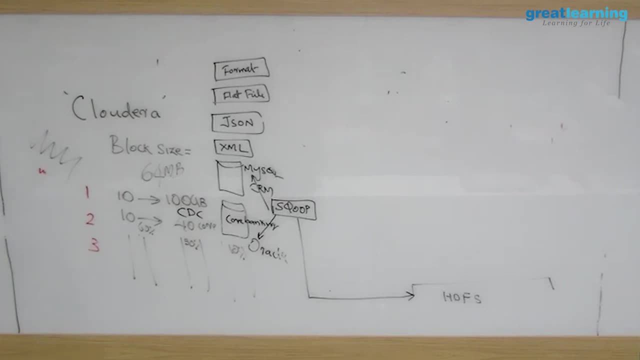 you can write a Java code and then get the updates dumped into here. That is how you get it. So GoldenGate is a product that Oracle uses for CDC. Anyway, we use Scoop to get from here and here. right Now comes the place where we are having 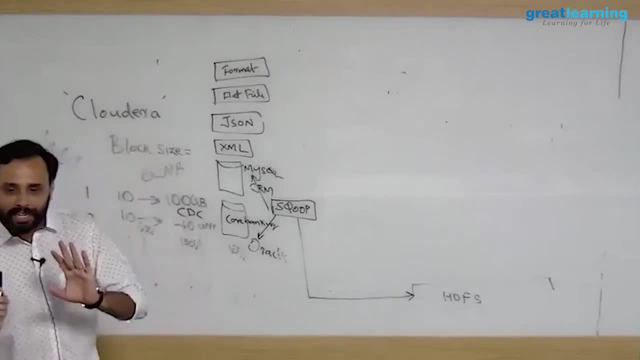 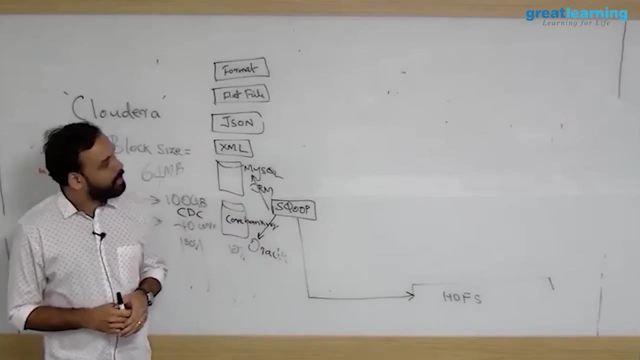 a lot of debate actually. Okay, Now the real question is that: okay, I know how to get the data from here through Scoop, right? What about the other data Right Now, if you want to get the other type of data? 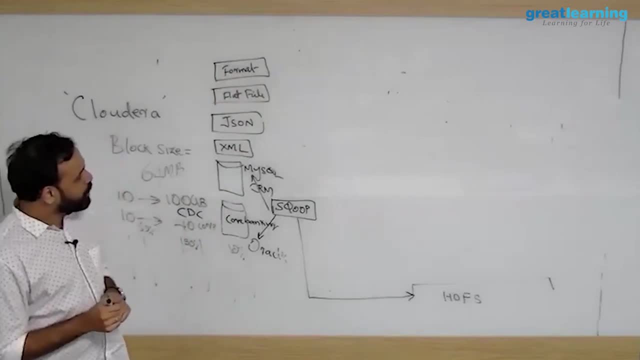 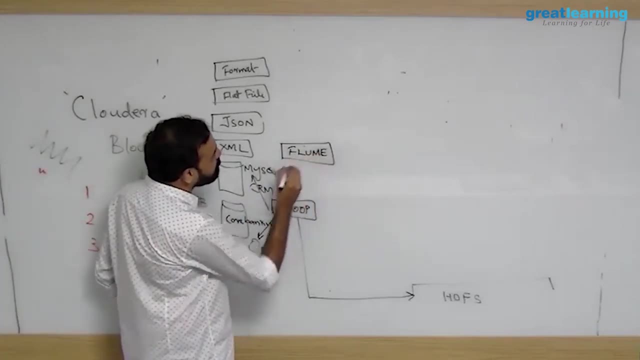 there are multiple ways you can get Okay. One of the most popular used tool is called Flume Apache Flume. Flume is a point to point delivery tool. What Flume does? it takes the data from source to the destination. 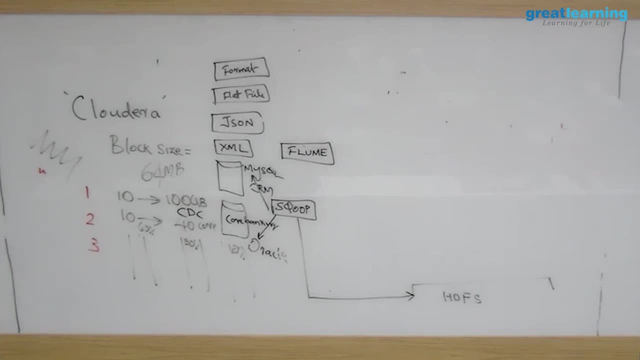 The source can be anywhere, And normally Flume is used for unstructured data. Say, for example, in a folder you're getting all the JSON data or XML data or flat files. I can create something called a Flume agent. 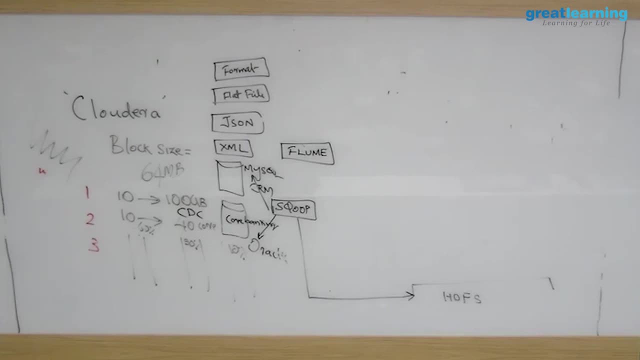 And this guy will keep on pulling that folder. Whenever there is a new data, this guy will read it And it will send it to HDFS. This is what Flume does. Now, the real interesting thing is that Flume can do two things. 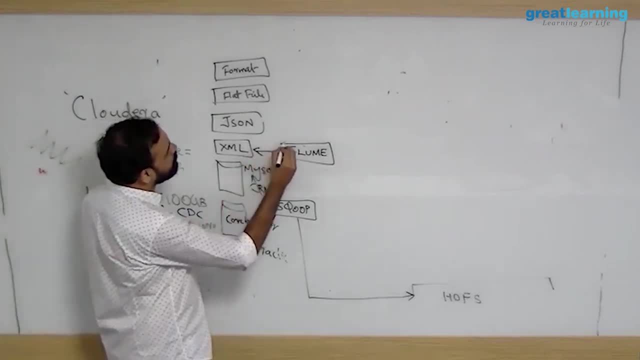 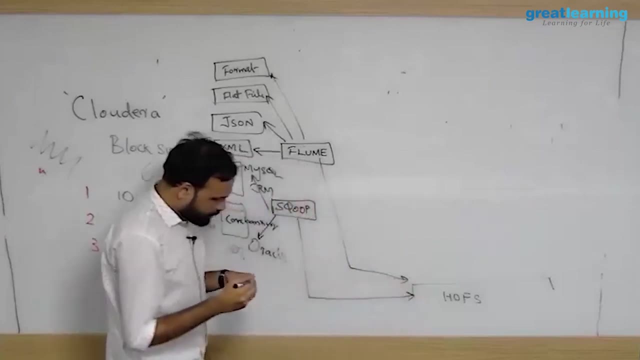 One thing is that it can simply read all this data. Let's say this is in a folder, Okay, It can simply read this data and say: send it to Hadoop. This is fine. But ICSA Bank also had another requirement. 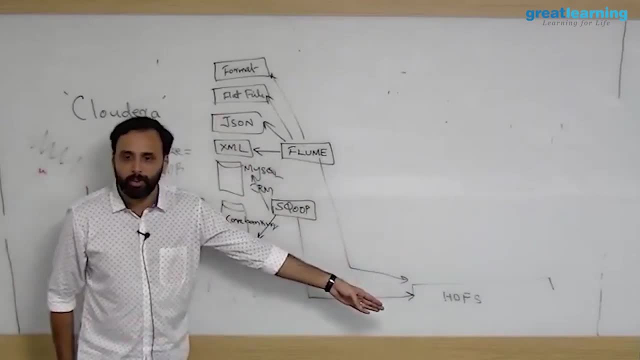 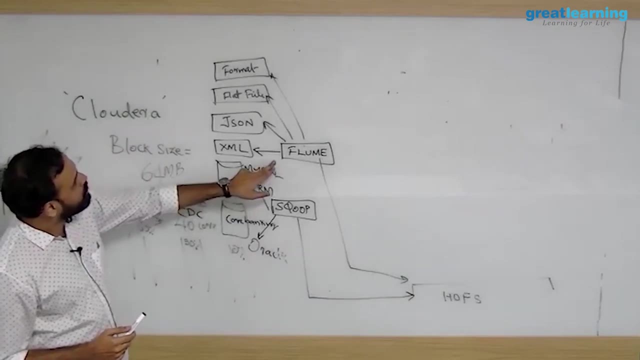 So this is simply: you're collecting the data and dumping it to Hadoop. They don't want to do that. Okay, So they wanted. they had a requirement in which what used to happen was that this Flume was capturing some data. 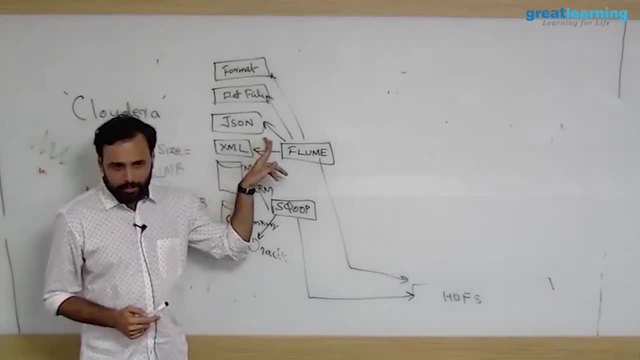 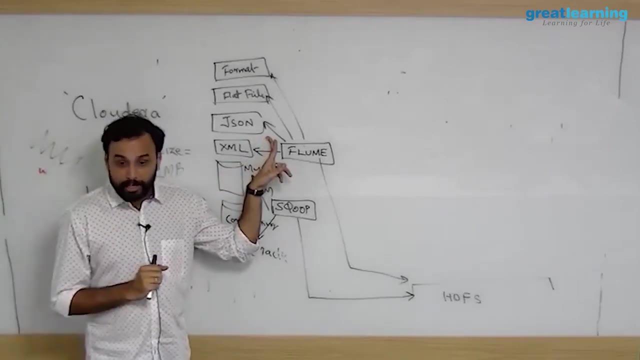 Okay, Some data was getting generated in the form of JSON here. So in the social media, if somebody is clicking on one of their products, they wanted to send an SMS real time. So this JSON data will keep on coming. You will keep on getting it. 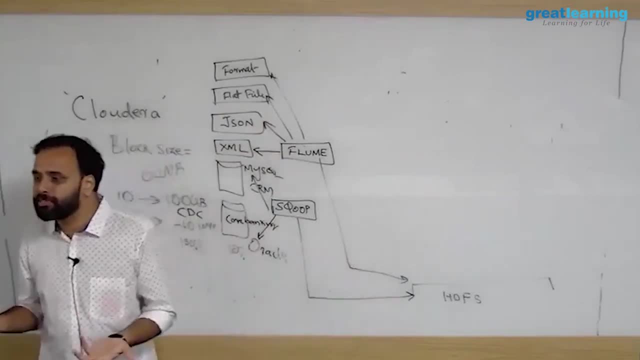 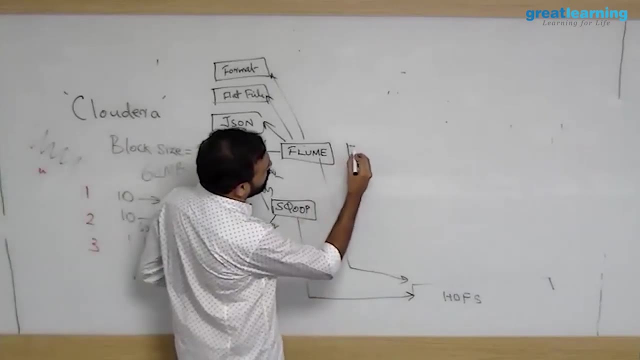 And Flume can directly dump it to HDFS, But that is useless for me, Because I want to analyze the data Whenever the data is getting generated. That is where this guy comes into picture: Kafka, Kafka. So there is a difference between Flume and Kafka. 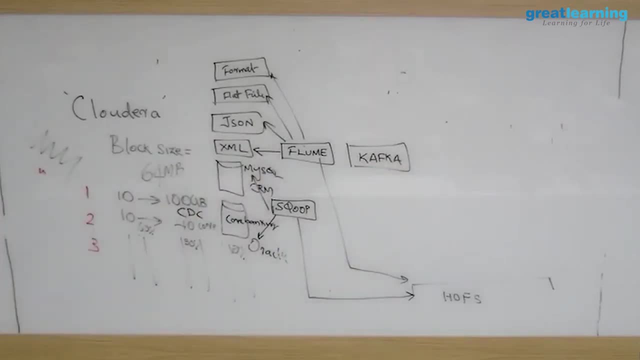 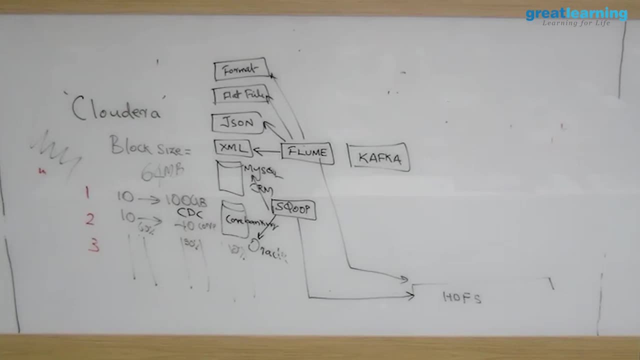 That is all flume does. It doesn't do anything. And flume does not store the data anywhere, Meaning it will take the data temporarily. it may store and then immediately push the data. So, Kafka is your message queue in the big data world. 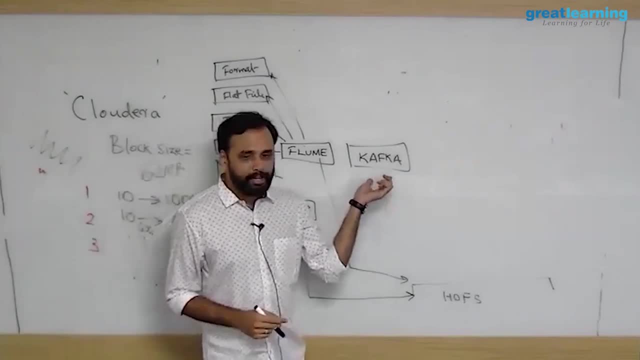 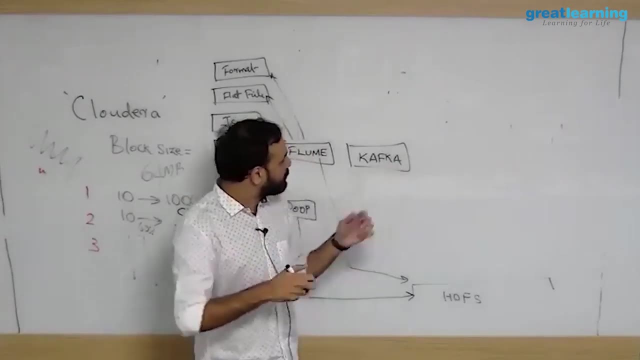 Meaning what this guy will do. this guy will be running in its own cluster, No Hadoop cluster. This guy will run on its own cluster like 30 machine, 40 machine. This guy flume can send the data to this guy, Kafka. 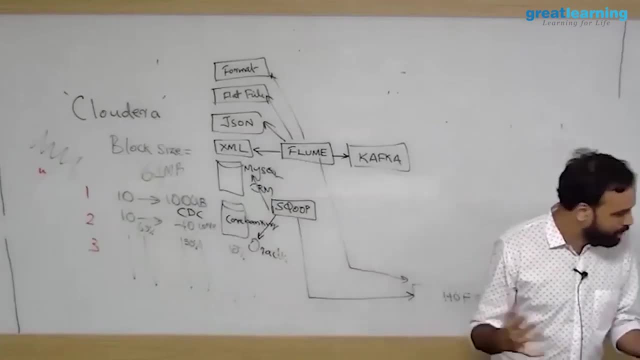 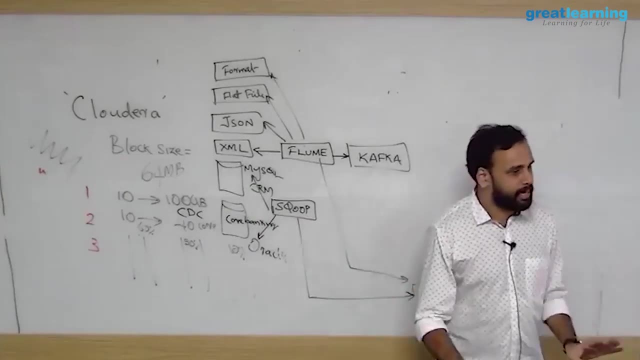 And Kafka is a cluster so it can store the data By default. it can store for 7 days By default. Anybody can go to Kafka and get the data Publish subscribe system. we call it. The advantage is: 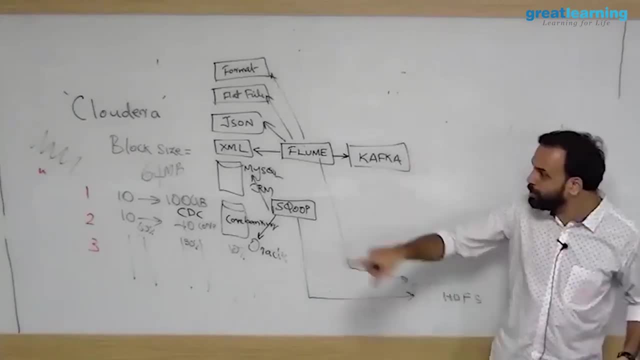 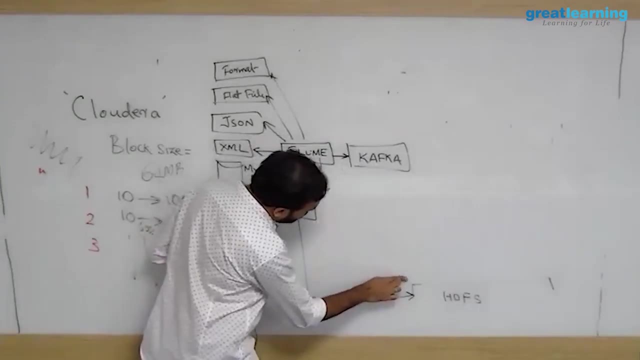 it will store the data so that multiple people can ask it. Flume is point-to-point. If flume gets the data, it dumps the data here. So here what we used to do. we didn't do this. We got the data to Kafka. 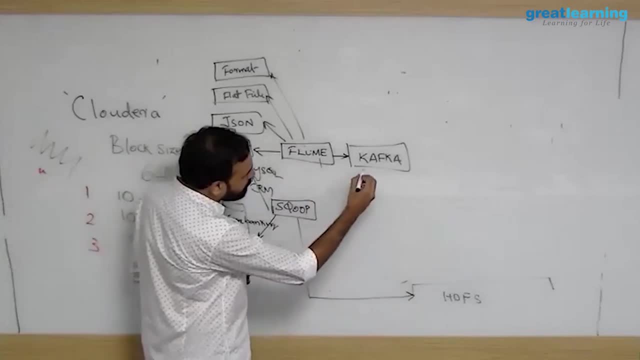 From Kafka. I can push it to HDFS one way, So I'm getting the original copy here Now in ICICI bank. so the next question is that: how do you analyze data in real-time? So somebody is clicking on Facebook. 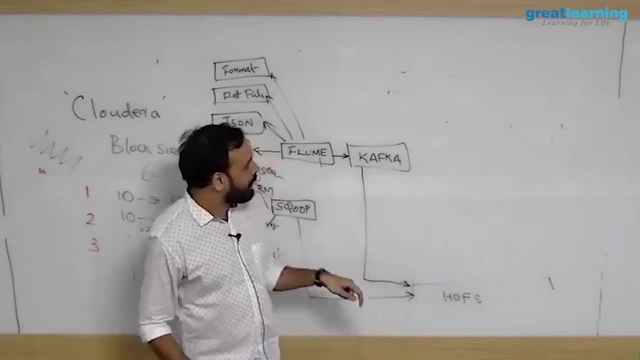 the data is coming as XML right And immediately when the data comes, flume will read it, push it to Kafka. So now the data has reached till Kafka, but I want to analyze the data in real-time. That's the first step. 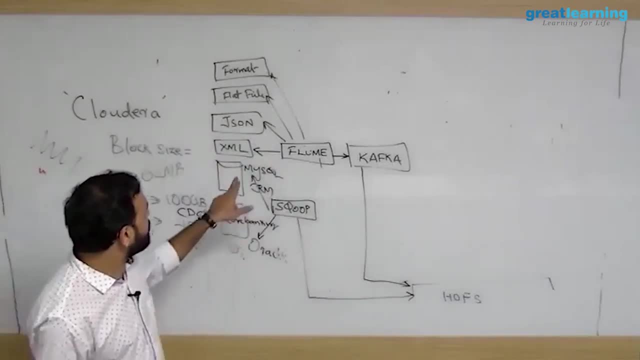 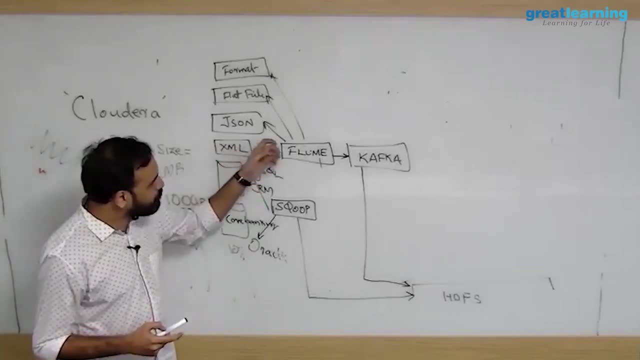 Shows exactly when it's coming as XML right And immediately when the data comes flume, will read it, push it to Kafka. So now the data has reached till Kafka, But I want to analyze the data in real-time. 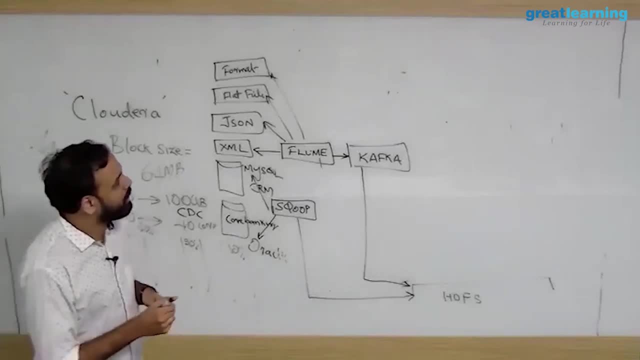 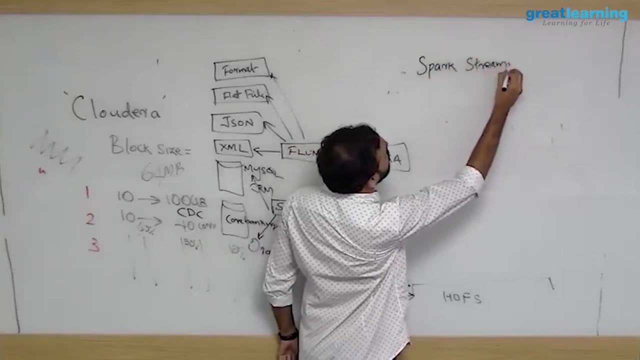 That is where your Spark comes into picture. That is where your Spark comes into picture. There is something called Spark streaming. In Spark, you will learn this. I think. I'm not sure. I'm not sure. Okay, There is something called Spark streaming. 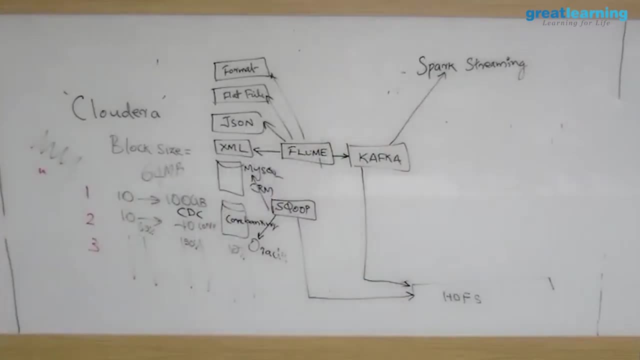 There is something called Spark streaming. So Spark streaming is a utility which analyzes real-time data. Now Kafka can also directly Спасибо, get this data. now this is a bit confusing, i know, okay, because this is very new to you. first of all, 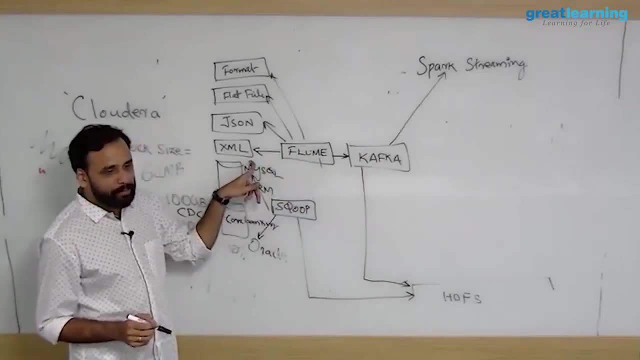 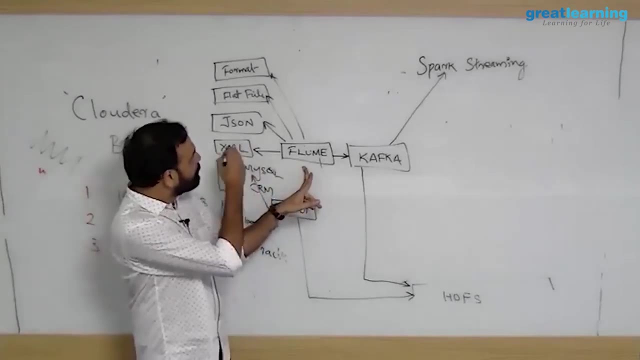 but kafka can also directly get the xml file. but the advantage is that flume is pull based. pull based means if i install flume without disturbing this setup, i can pull the data. kafka cannot pull the data. you have to install a tool here and modify the existing setup. 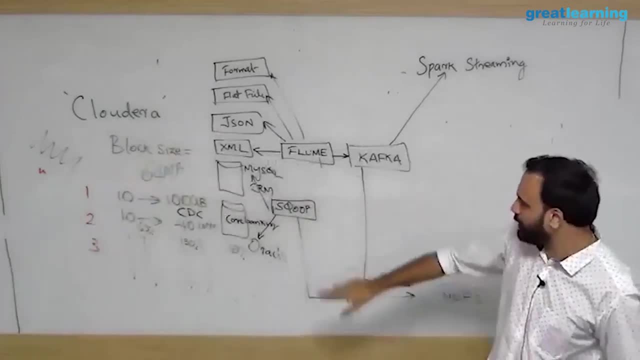 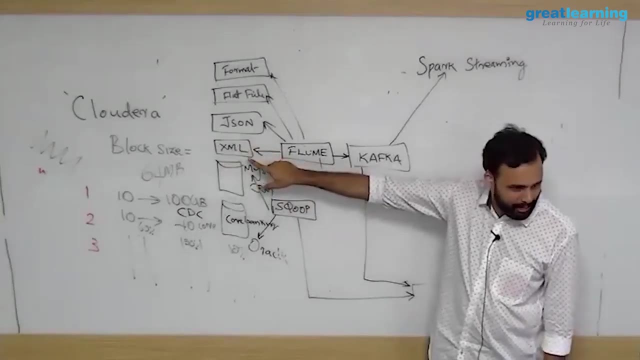 flume is pull based, meaning if you install flume here, it can start reading the data automatically. i don't have to modify anything. if i install kafka directly, kafka can also get the xml data, can read the xml data, but i need something called a kafka producer. that has to be installed here. 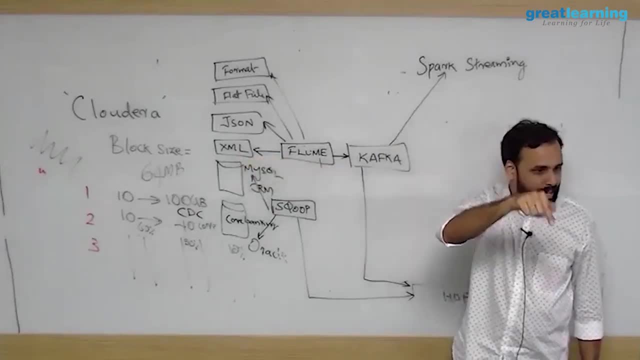 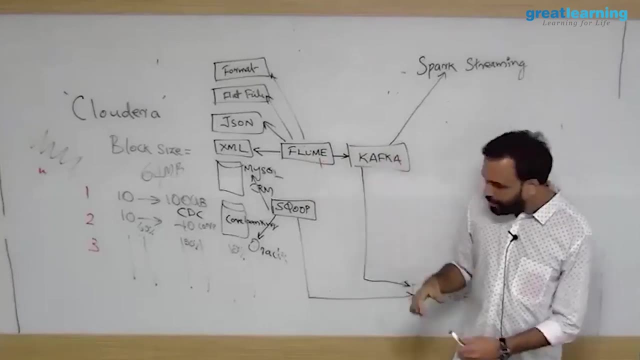 on the icica source system. that is not possible, right? so since it is an existing setup, i can't directly get through kafka. i get through flume. flume will give to kafka. kafka will send one copy to hdfs because i need to keep the original data. second copy it will send to something called spark. 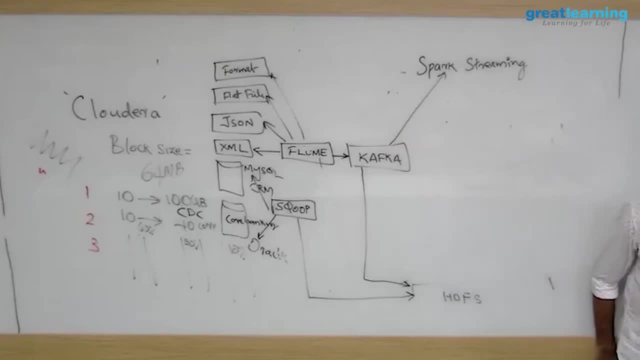 streaming. spark streaming is a library available in spark where it can do real-time processing. the moment you give the data will process it real-time. somebody clicked on that immediately, the data is here, spark streaming will process it and say: send an sms or you can take an action, whatever. 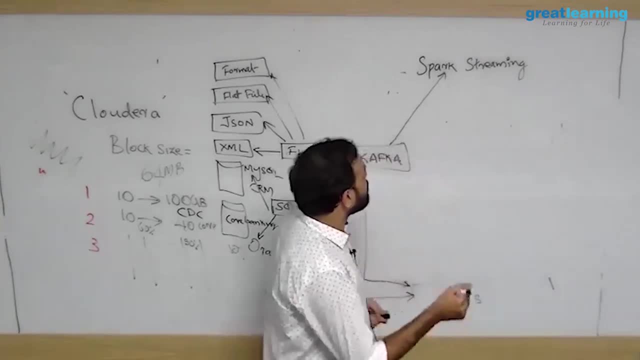 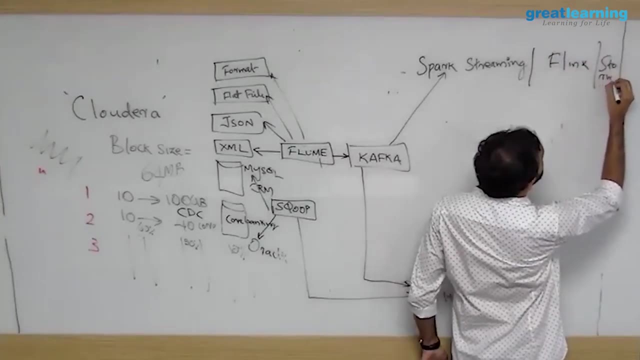 you want. now, what are the other tools which can do real-time apart from spark streaming? you have something called fling, you have something called storm. these are all real-time processing tools. you might have to make a note of that, so in whatsapp. you might have to make a note of that, so in whatsapp. 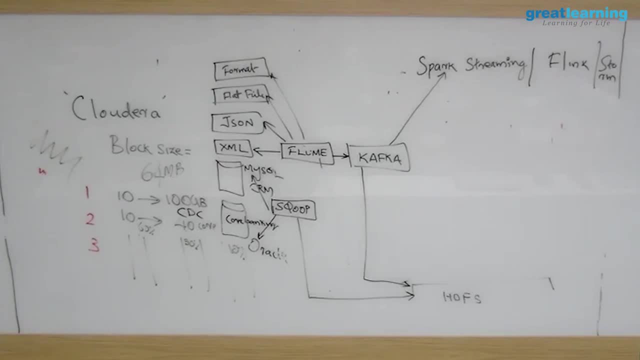 it is push right. flume is like whatsapp. okay, once flume gets the data, it will push it. push it to somewhere, it will not store the data. kafka means it will get the data and store it for you as long as you consume it. so in in icica bank. this was the architecture. we got it through flume sent it to. 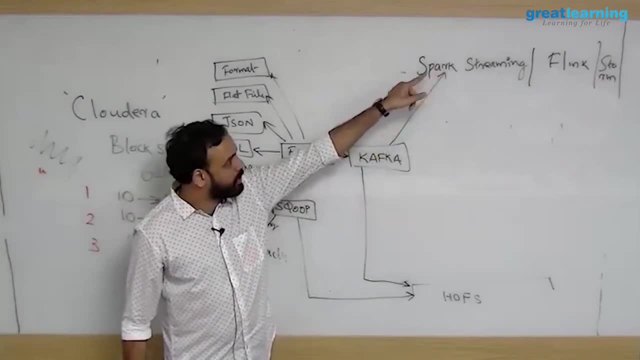 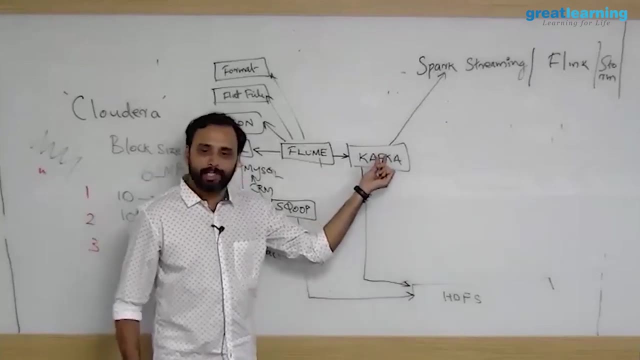 kafka here. one copy will go to spark streaming, so this guy will do real-time processing and do something. okay, one copy will go to hdfs, so the data will remain in kafka as long as you want. you can configure by default. it is seven days. you can also mention the size of the data i want to keep. 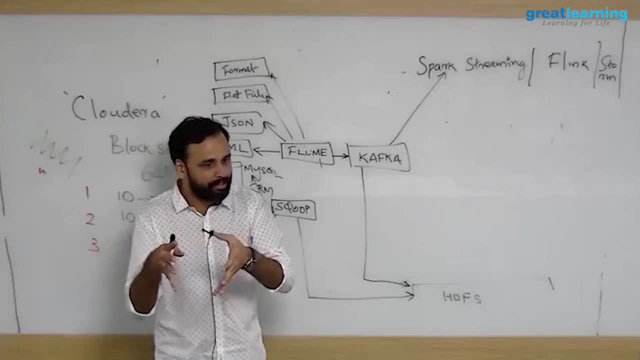 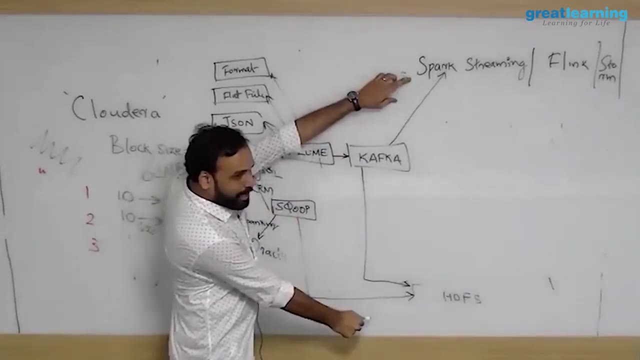 only 10 gb data, 20 gb data. there is something called topics in kafka where you can mention how long the data should stay here. it's a cluster. right flume can send here, then this will not happen. it is point to point delivery. i need a copy here. i need to send there also at the same time. 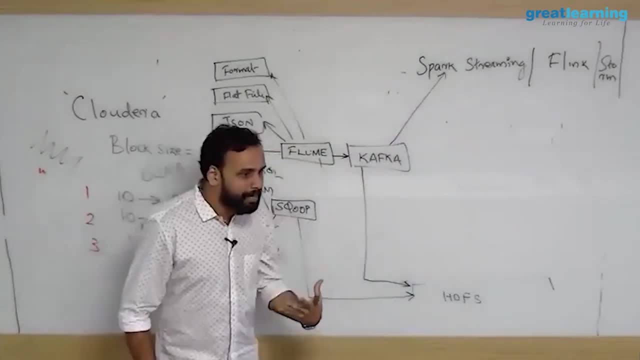 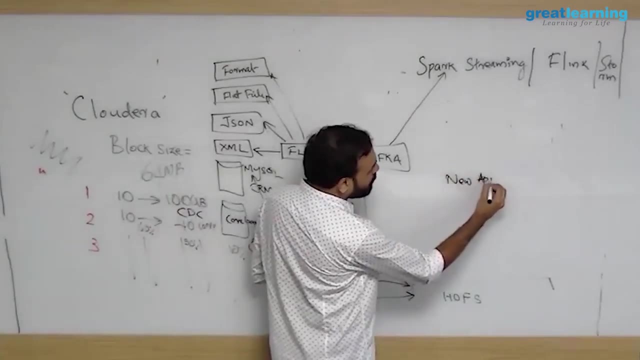 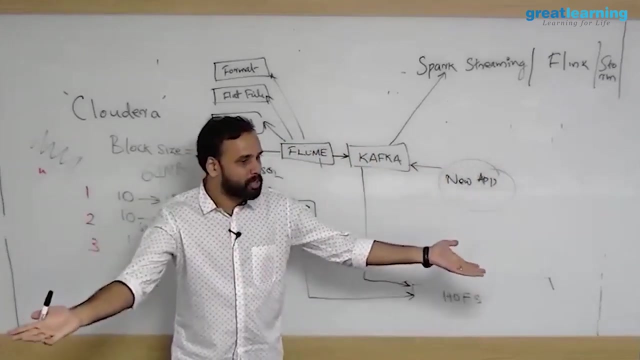 also probably tomorrow. i want to build one more application, okay, which will do something on this data and that application. i have a new application i build tomorrow that can also get the data from kafka. kafka is like: if you give data to kafka, anybody can take it from me. i will store it for you got it. flume is like point to point. 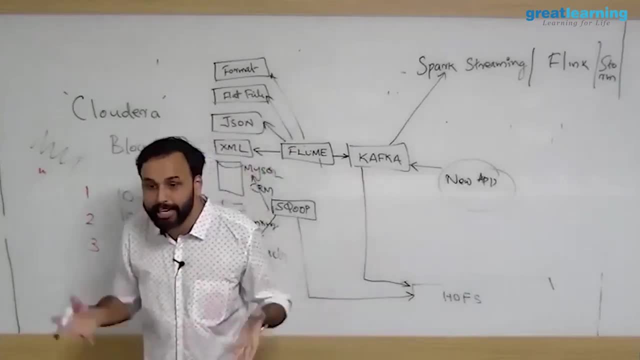 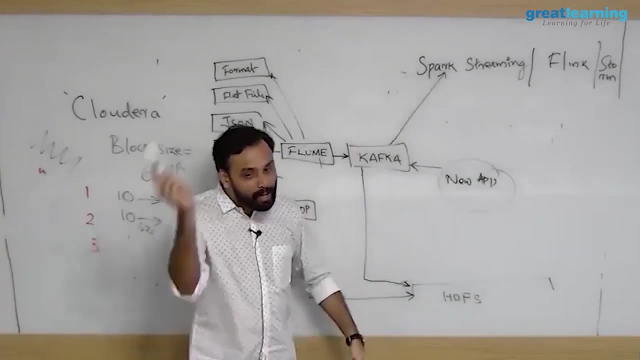 got it. kafka will store it so that anybody can come and get the data. 10 applications can read from kafka: very slow, hardest to read. i can directly push in real time right. so before you get out of panic shop, i want to send an sms right now. this will be one golden copy will go here: the 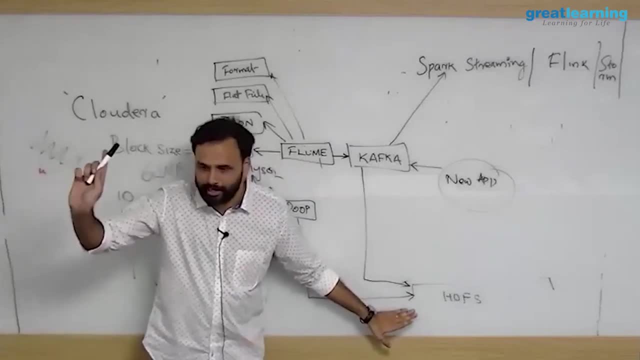 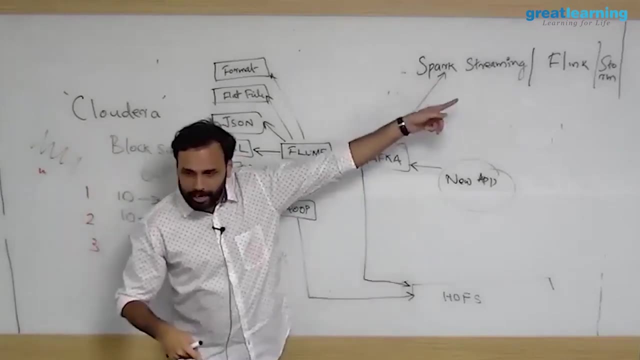 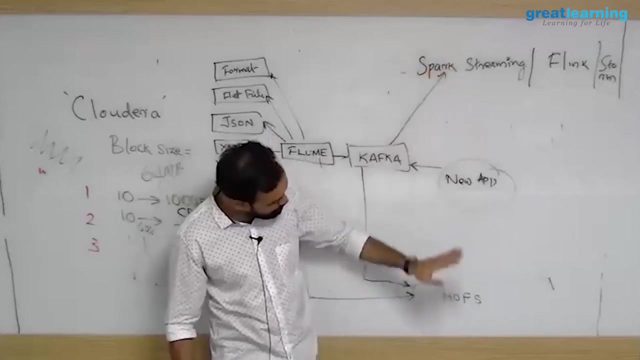 original facebook clicks and all golden copy will go here that tomorrow you can analyze. now you clicked on a page- insurance page- in facebook. i want to immediately contact you. so it has to be processed and understood. and then some decision has to be vacant. so i'm sending one copy here, one copy here here. the processing will happen here simply. 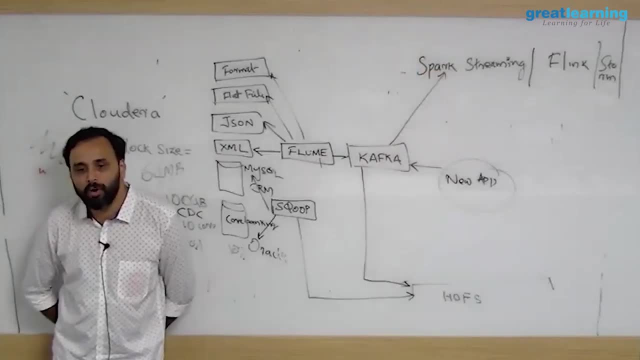 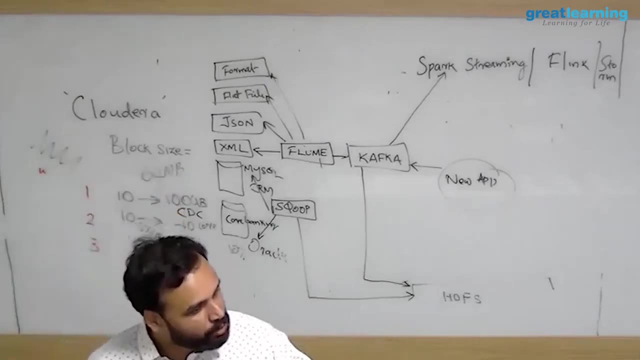 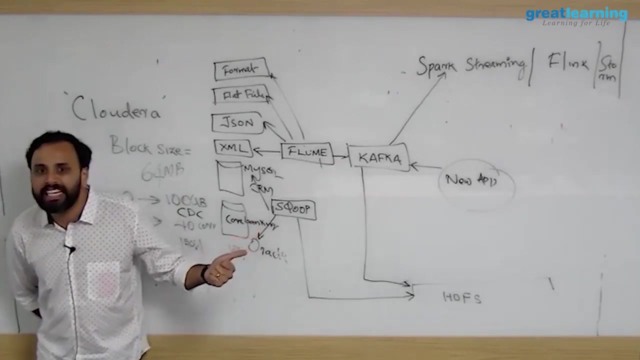 the original data will be stored. no, no, no plume and kafka cannot only scoop, can read from sql based tools. now, kafka is a very interesting thing. i teach a three days course only for kafka. elk cast out right now. elk stack will not come here. in this example we didn't directly use 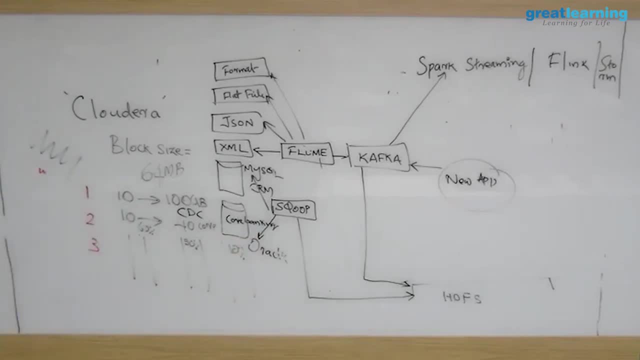 alk stack we were using. that's what i was telling in the break to somebody. what we were doing is that we used to store the data in hadoo to process we were using something called splunk. there is a tool called splunk. splunk can actually replace your elk stack. it does el k- both in one. 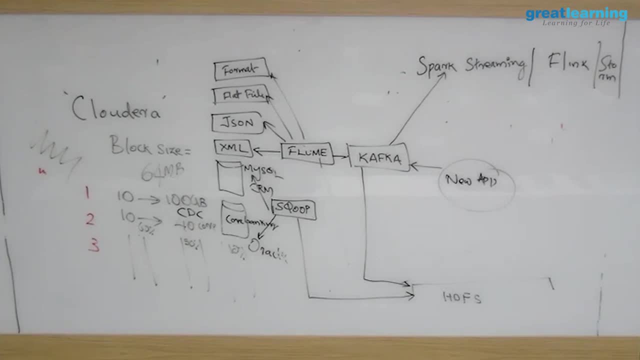 tool. so that is for visualization, right, you have some log files, machine learning, you can just apply. We were using something called Splunk, So this is the big pipeline I'm talking about. You can also build it using ELK if you want. I'm just saying. 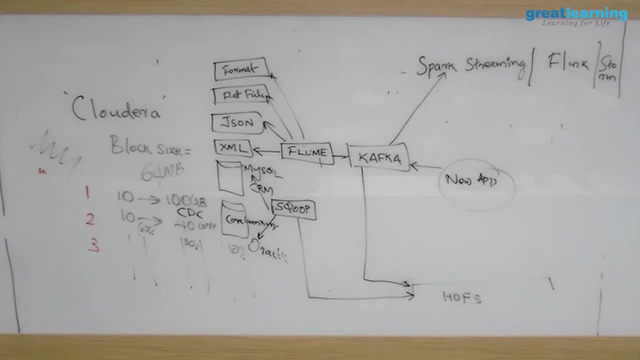 ELK is a stack actually Elasticsearch, Logstash, Kibana, It's a. probably you can explain right. So let's say you're getting a lot of log files. You want to make sense out of it right from different, different places. 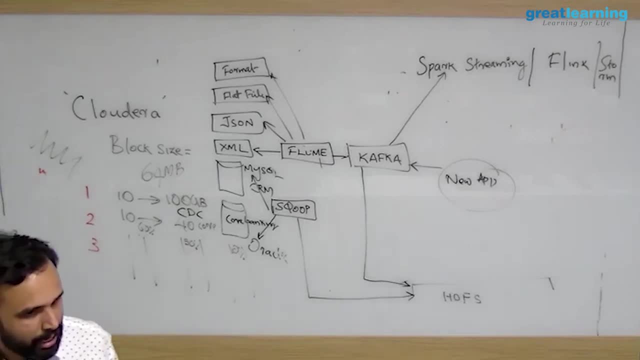 Let's say I'm collecting all the logs from this network. I want to make sense out of it, So I need a tool which can easily collect it, clean it and then display in a dashboard, That is ELK, what it is doing. 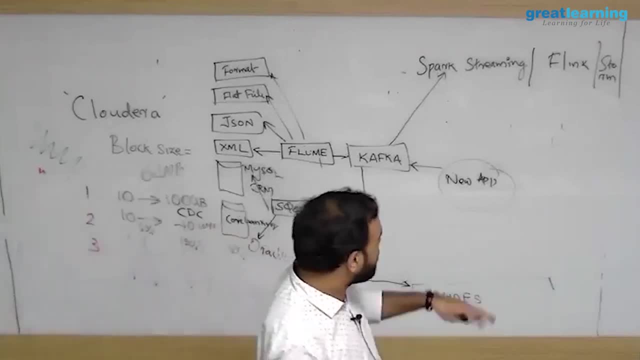 There is a tool which is very similar That's called Splunk. That is not in the big data, In the Hadoop ecosystem. it is not there. That is a third-party tool, actually, Exactly so that's a good question. 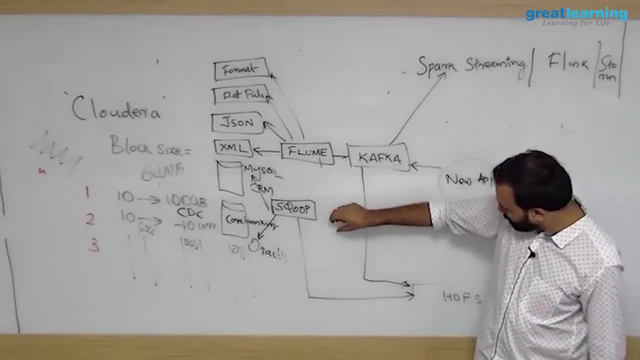 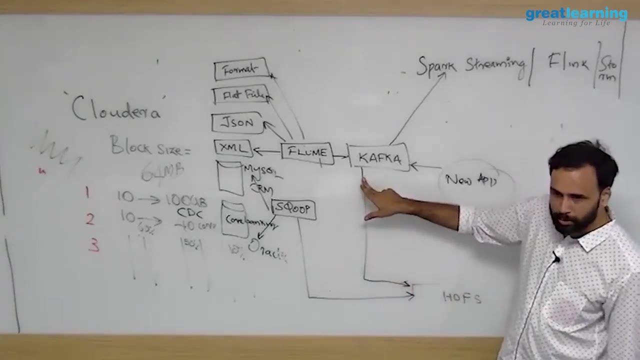 So when Scoop is getting the data right, Scoop will ideally push only to here- HDFS okay. But I can say Scoop will push to Kafka also. That is also possible Once the data is available in Scoop, okay. 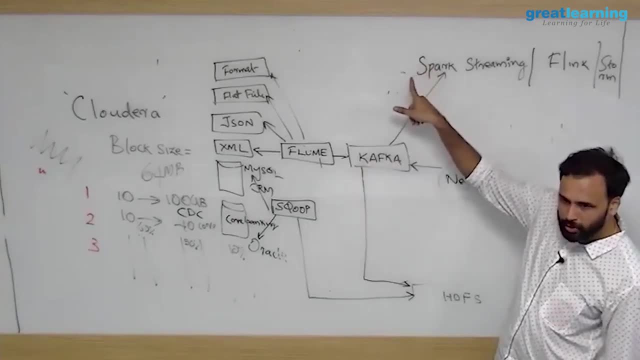 I can say: give it to Kafka. So either it can be read for live processing or Scoop can push to something called Hive. We have a Hive here which is a data warehouse. From there I can analyze in live if I want. 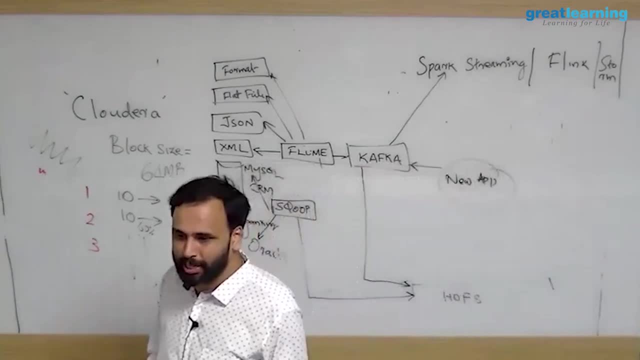 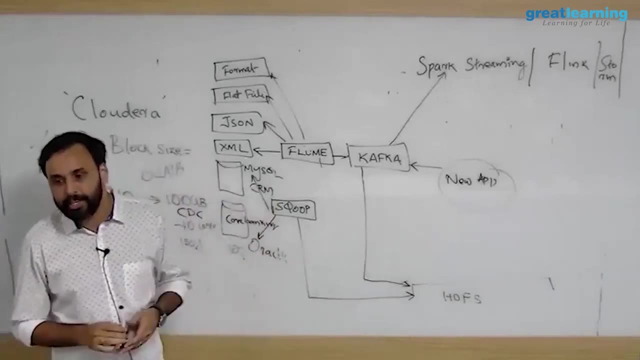 But normally this transactional data is not much use for real-time processing. You are doing it based on this Facebook clicks and all Based on this transaction. I can get it Now, just to answer his question. that's a good question actually. 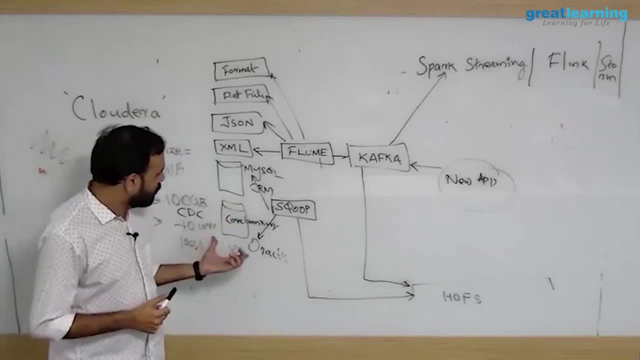 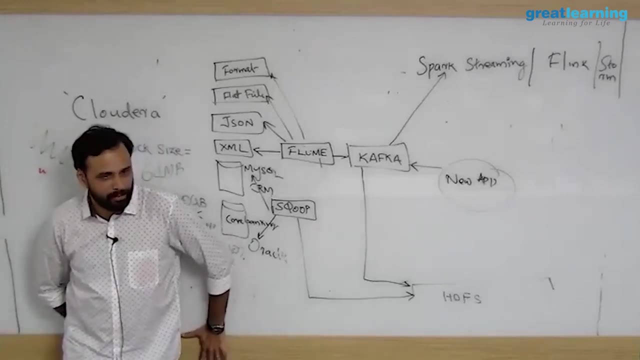 So can you give me a suggestion? So a customer is a customer is making a transaction. A customer is making a transaction using ICICI credit card. He made a transaction for 50,000.. I have to immediately send him an offer. 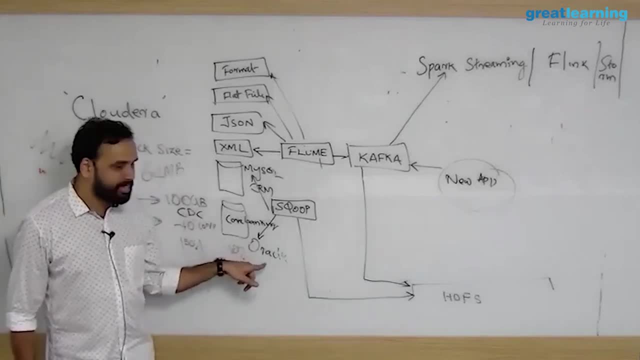 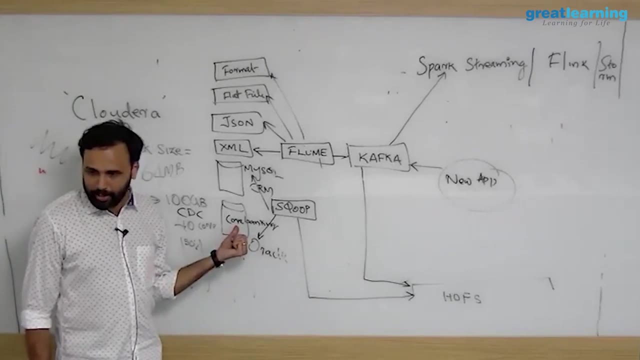 So if he's making a transaction here- I made a mistake here. I want to show that If he made a transaction here- 50,000, okay, where will be the data in Oracle? How do you capture the data from here? 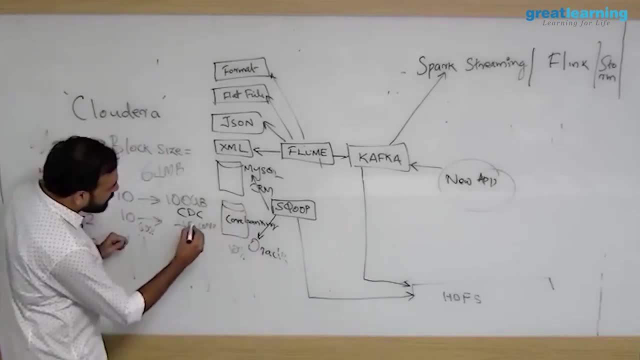 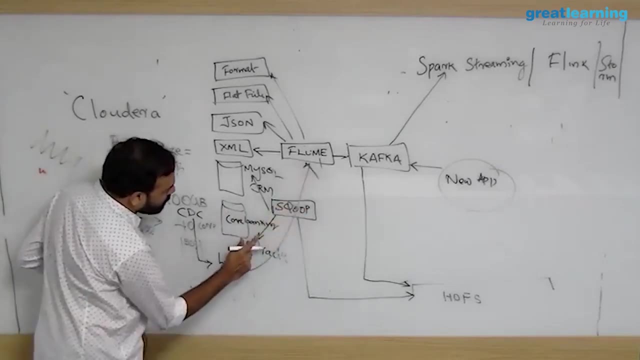 You will say: Scoop, they were using Flume, because your CDC will be producing a log file. The log will be captured by Flume, not Scoop. So here Scoop will not come into picture, Here Scoop will come. 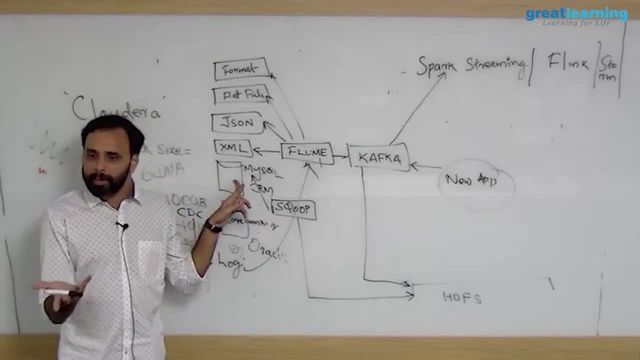 because I'm directly reading from CRM. My CRM is in MySQL. MySQL is original table And I can read directly. But in the Oracle case I was not directly reading the table. If I want to read a table, Scoop. But we were reading the CDC change data capture. 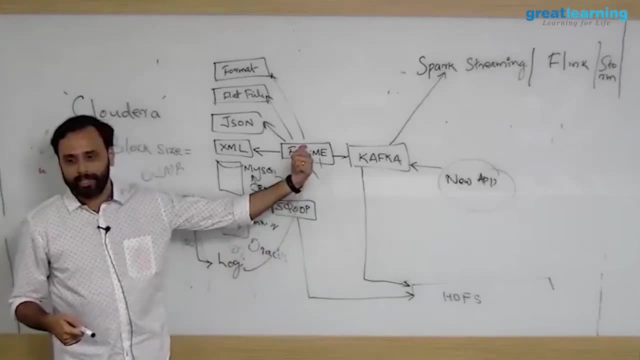 That was a log file That was being collected by Flume, actually, So you can understand that Scoop can actually make it. So this is the answer. If you want to make real-time, okay, you need some CDC system. 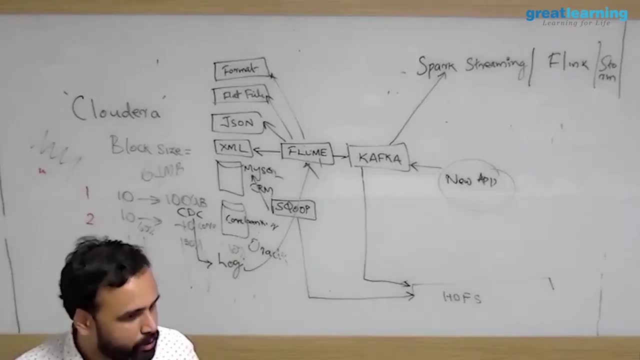 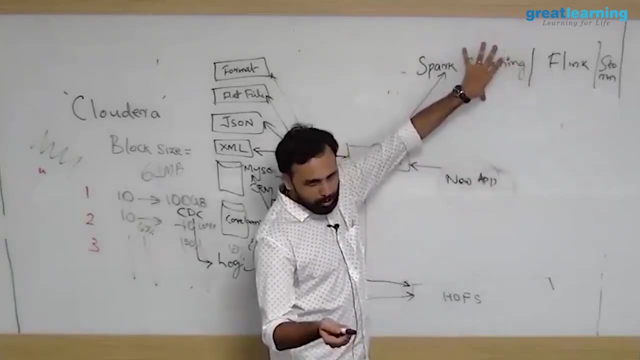 which can push the data to Flume. I have worked on a banking use case where. so I'm talking about this site, Spark Streaming, Flink, Storm. So Spark Streaming is what you will be learning. Flink and Storm are other frameworks. 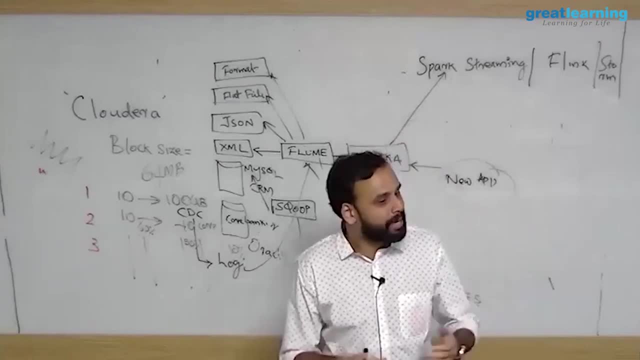 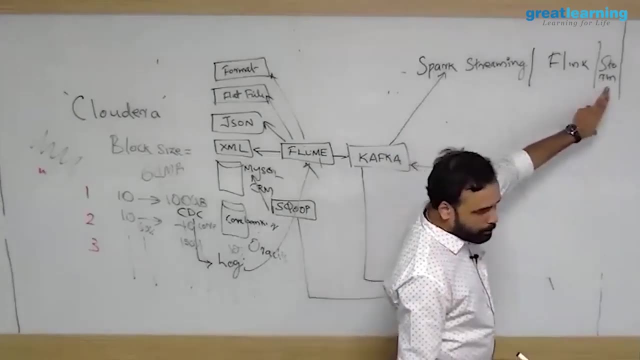 which can do real-time data processing. So you will be wondering why real-time data processing is so critical. All three are real-time. You may use any of them. Flink is Apache Storm is also. Apache Storm is almost out of the market okay. 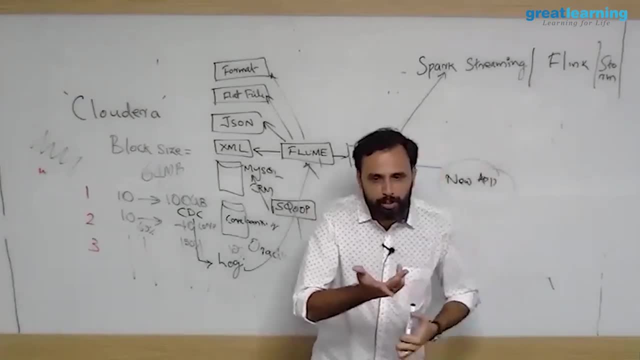 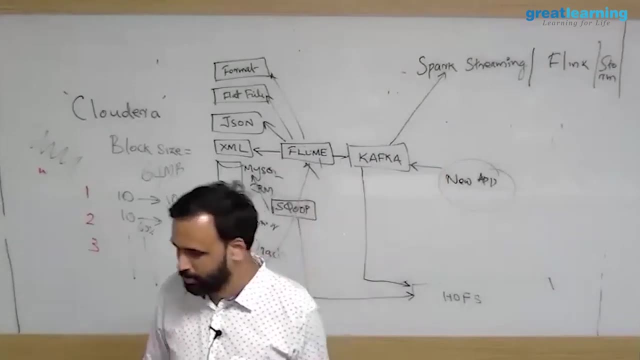 Spark Streaming and Flink are popular right now. We have worked on a use case with Citibank. You swipe your credit card, right. How do you know it's a fraud or not? You're swiping your credit card? I want to find out whether it is a fraud transaction. 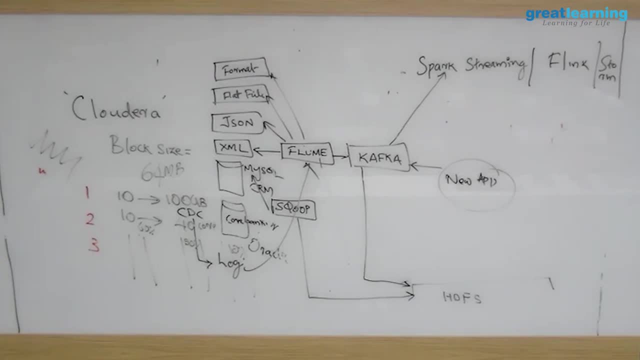 or a real transaction. You don't have to be a fraud. Let's say, I use a credit card regularly. If I one fine day, if I suddenly pay in US dollars or something, I'll get a call from customer care. Did you really make it? 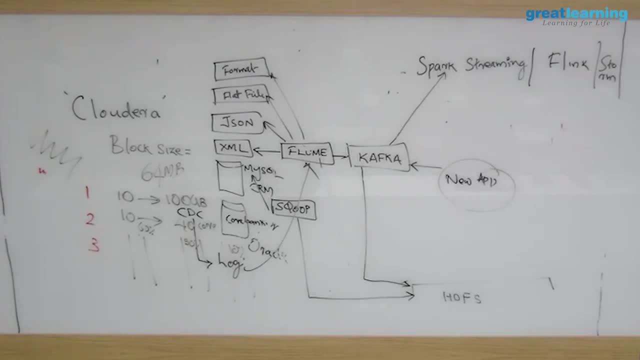 That means: imagine, say, HDFC Bank- how many credit cards will be in circulation and how many people will be transacting every day. Do you think somebody is sitting and monitoring every swipe? You are collecting all the data. All the credit card transactions will get dumped. okay, 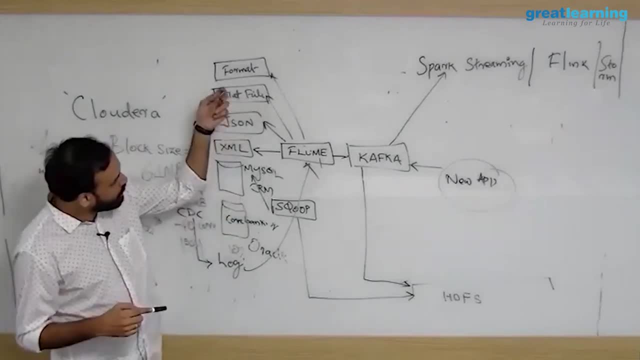 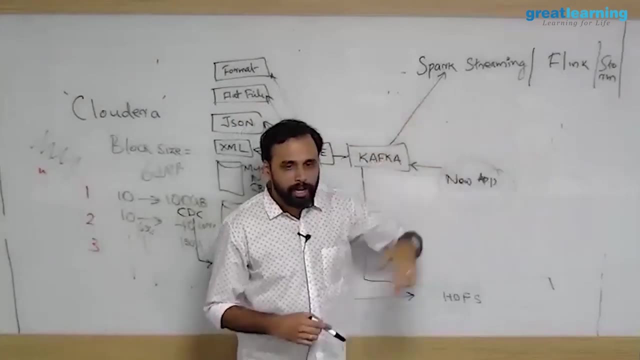 They won't come in a relational form. They will come in some flat file or something. Your flume will catch it The moment it comes. it'll push it through Kafka or directly to Spark Streaming or Flink or Storm, And there I could have written a logic, okay. 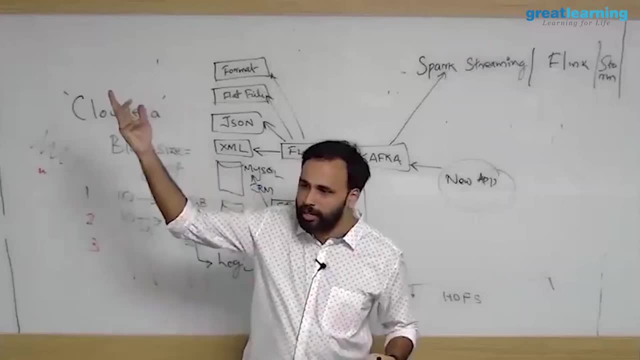 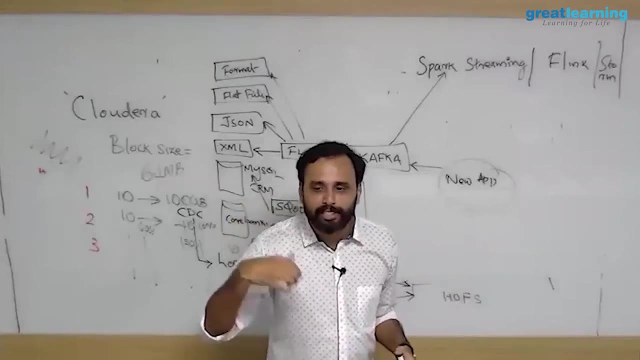 Match this transaction. If this guy's limit is something, or his last transaction made places outside India or something, trigger a mail to customer care. That is how you are getting this EMI calls. also, When you make a big transaction, immediately they will call and say: 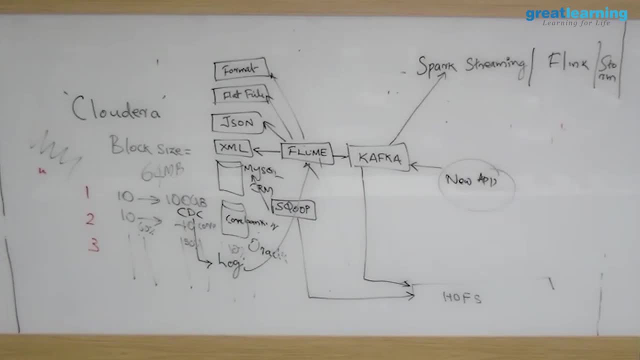 do you want to convert EMI? right, These guys are responsible for that. What is the difference? This Storm can process one event also, Meaning one credit card transaction. Storm can process Ideally one credit card transaction. it will process Minute. 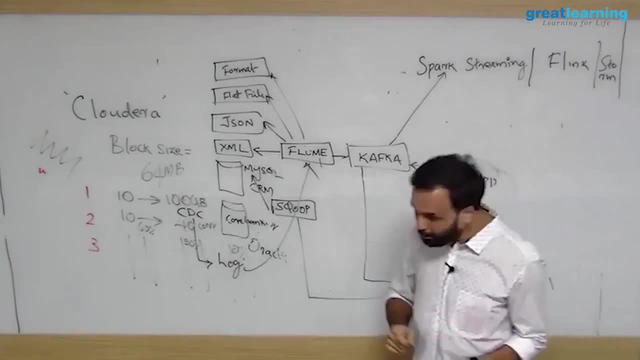 Streaming can process only bunch. It cannot process one, Meaning it will collect probably two seconds for all the transaction and predict, I mean so that's called micro-batching: It is creating a batch and then from that it is processing. 100% real time is only possible with Storm. 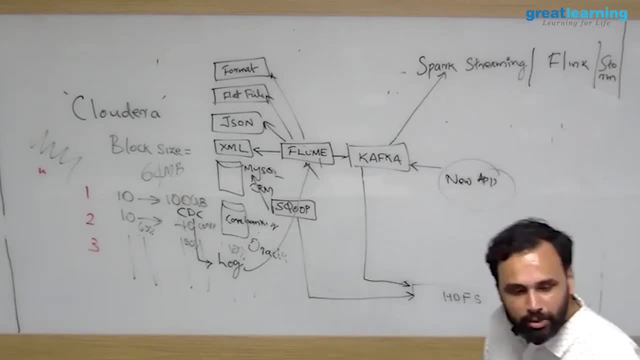 And Flink also does the same either. Now, this security is we were not handling. I'm not 100% sure how it is working. Our use case was only limited to this right, But now I have a question. okay, 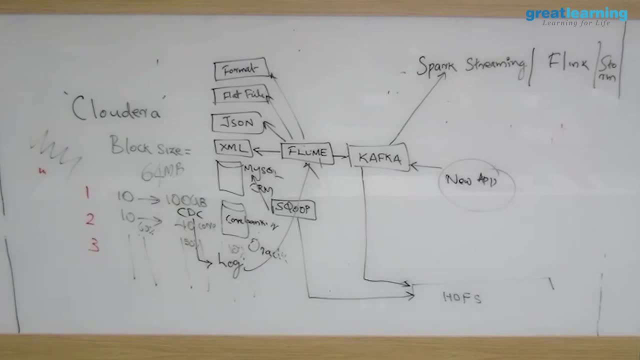 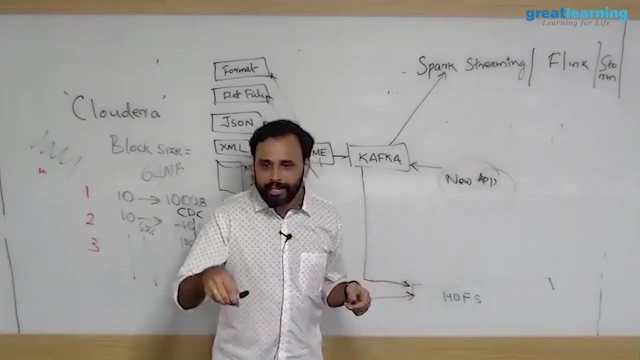 The question is very much valid. You are making a credit card transaction and Spark streaming catches it. Spark streaming catches it, but that is the real time transaction. How does it know that this is a fraud based on the previous transaction? So if I am making a credit card transaction today, 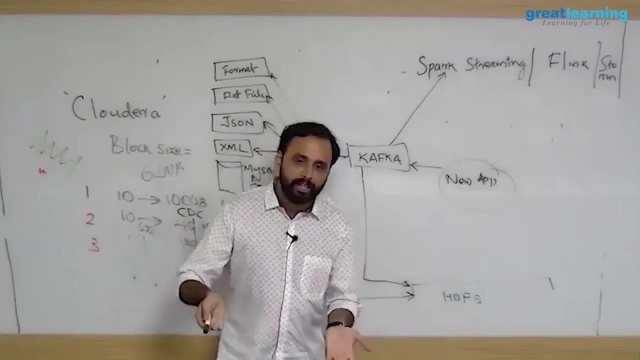 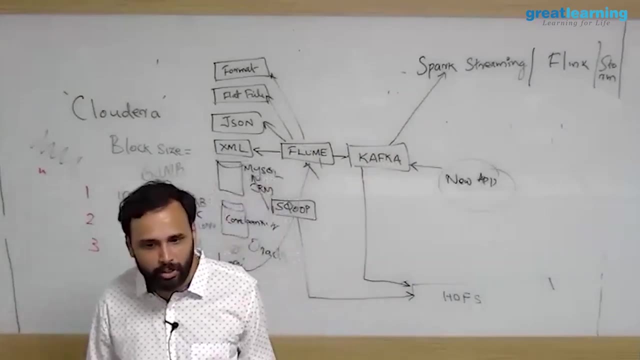 all my previous transactions are already here. They could have already built a machine learning model And if you simply feed this new transaction, it can predict. Otherwise, how do you compare with batch data? I cannot run a batch job. It will take a lot of time right. 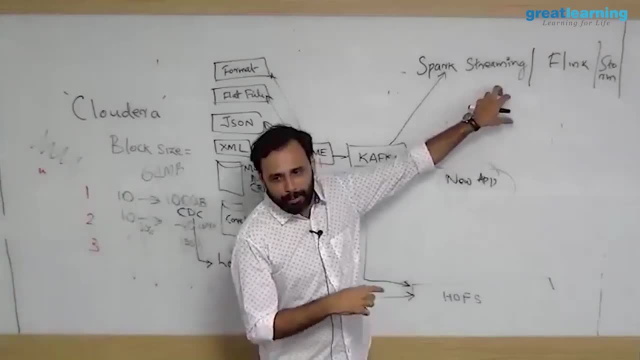 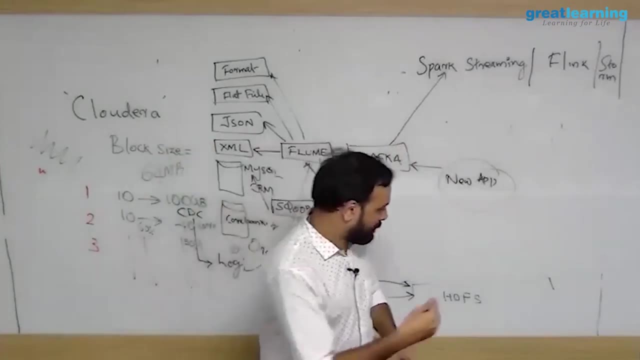 All the customer data. So they will run a MLLib. it's called MLLib in Spark Machine learning model will be running. That will easily compare and say it's a fraud. If you want to compare the batch, see now. I'm just making a transaction, right. 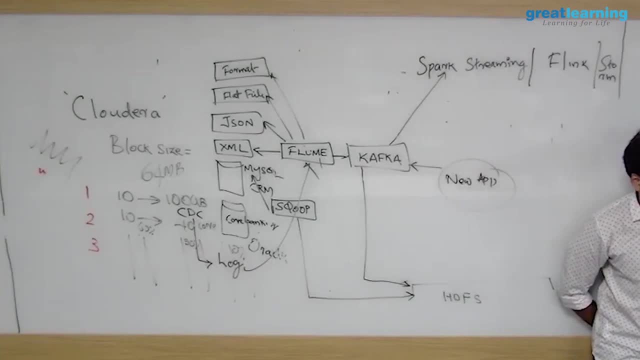 It has to compare with my previous transactions to understand whether I'm a fraud for the past 10 years. Today I'm swiping in New York, New York swipe. if you want to understand it is an anomaly. you should compare it with previous swipe right. 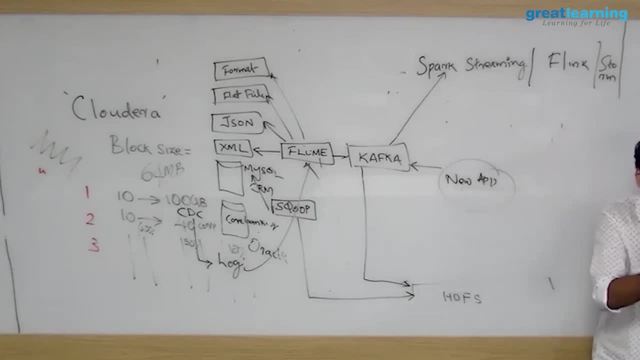 Now, each time you cannot go and compare for each customer, So they build a machine Machine learning model based on all this data that can. if you feed a data, it can predict you know whether he will be a fraud or not. 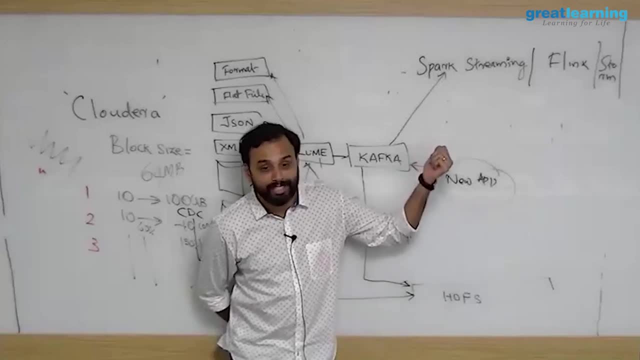 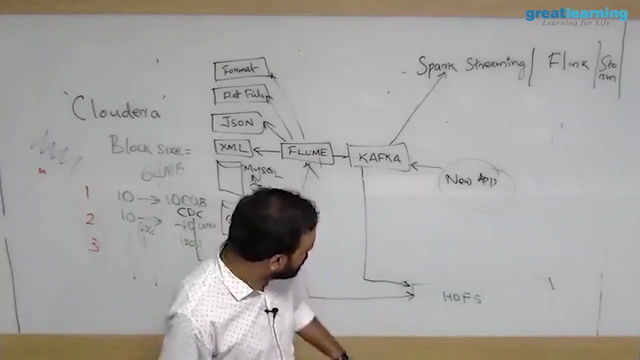 And it will not directly compare and get this. I'm talking only about fraud detection. So your use case is your- this thing right- Stock market price variation. So my point is this: historical data will be huge. It'll be in terabytes, right. 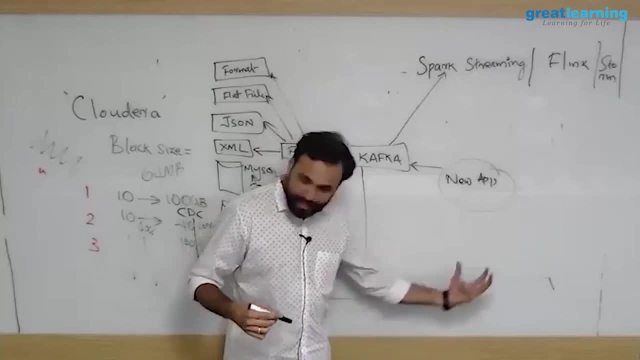 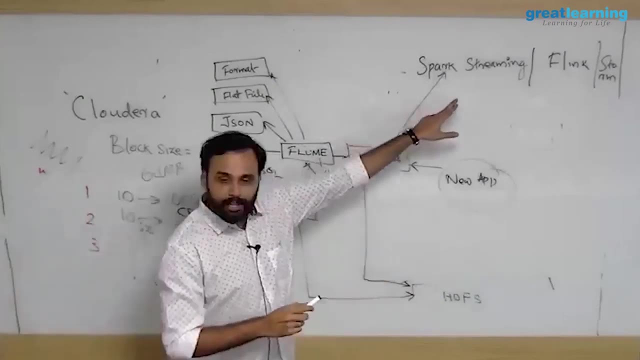 So you could have already created a machine learning model by feeding this data, which, if you give any new data, it can predict whether it is fraud or not. That is happening in real time. I cannot say that once if somebody swipes a credit card. 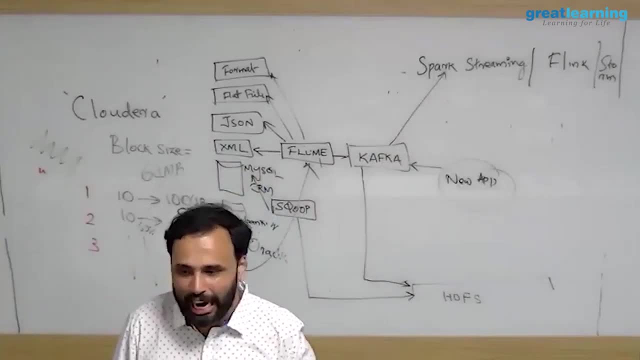 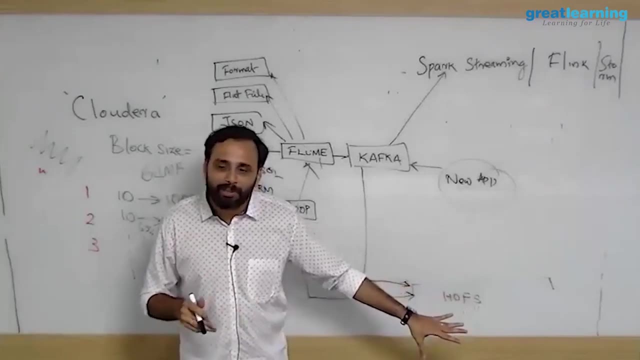 I will tell you whether it is fraud. tomorrow Doesn't make any sense, right? I could do it immediately. Now, the flip side is that all this requires resources. Nothing is going to work if you don't have resources, So you need to give enough resources. 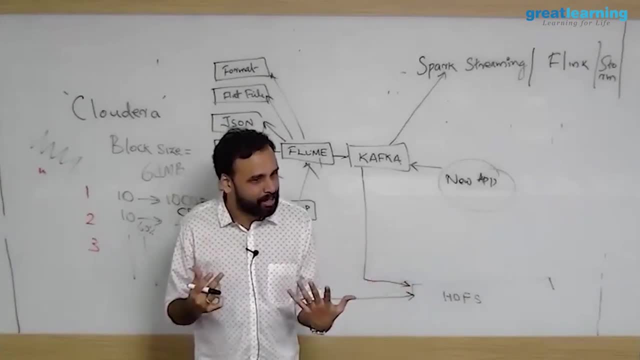 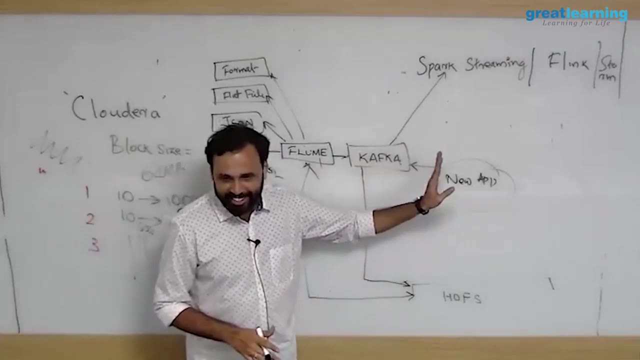 for all these things to work- Machine learning and all are very resource hungry- CPU power, RAM power, right, So these clusters should be capable of doing this. Anyway, for the time being, let's see. Let's move on from Kafka, right? 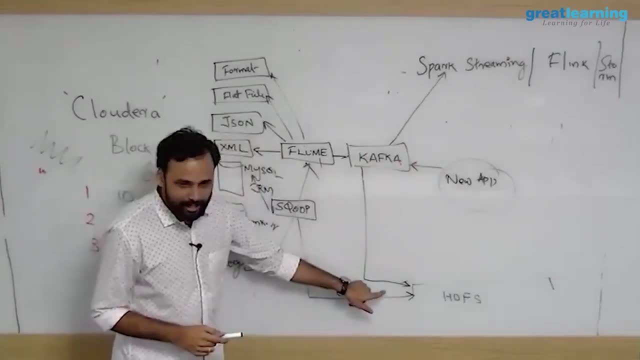 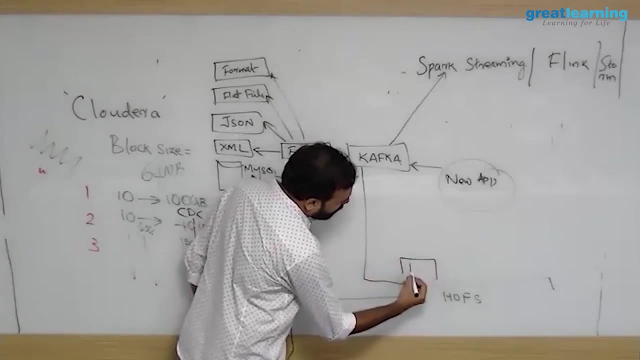 So we are just taking a use case right Now. I'll go here Once your data is in HDFS. if you want to do batch processing, the default framework is MapReduce MR, But I have my data. I want to do batch processing. 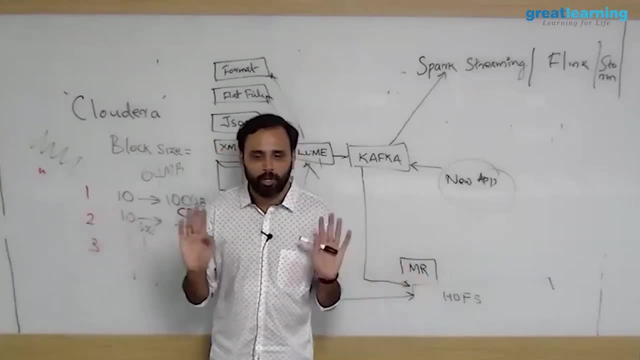 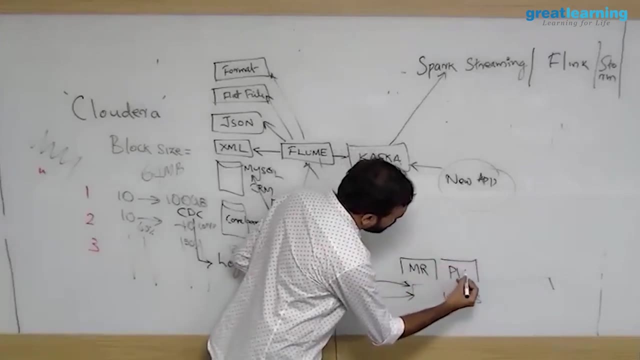 I don't care how much time it takes- One day can take- I just want to process the data. I can use something called MapReduce, right, You also have one more guy called Pig. This is almost gone from the market. Pig Pig, the animal Pig. 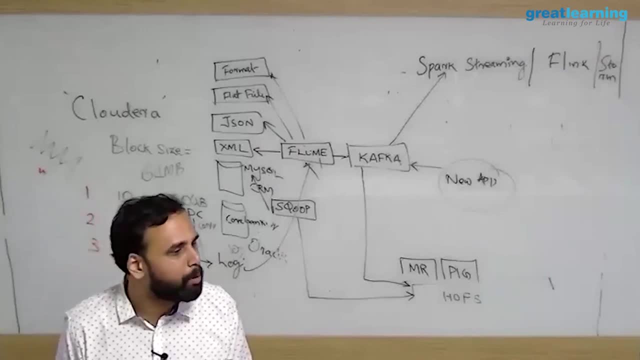 Pig is a scripting tool on Hadoop, but not very popular now because of Spark, So nobody is actually. so even if you're not aware of Pig, it is perfectly fine. I think, Okay, you don't have to worry. And then you have somebody called Hive. 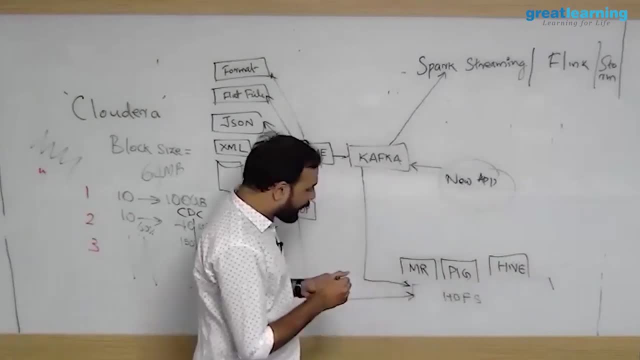 This is there in your syllabus. So, Hive, I will teach in the next month. but basically, what Hive allows you to do is to write it. So, basically, what Hive allows you to do is to write it. So, Hive, I will teach in the next month, but basically what Hive allows you to do is to write it. 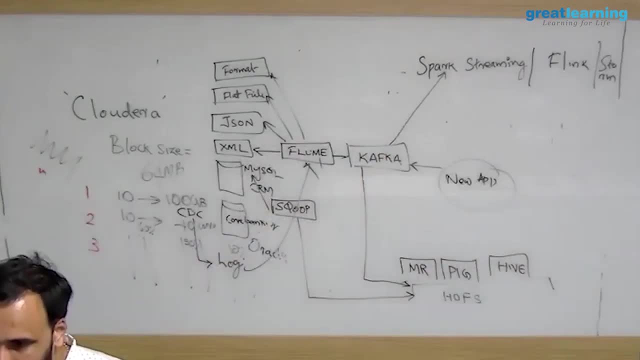 SQL on top of Hadoop. But the drawback is you say create table and select count star from the table. hit the query. It will convert your query into a MapReduce program. So it's a translator. It is not a native SQL engine. 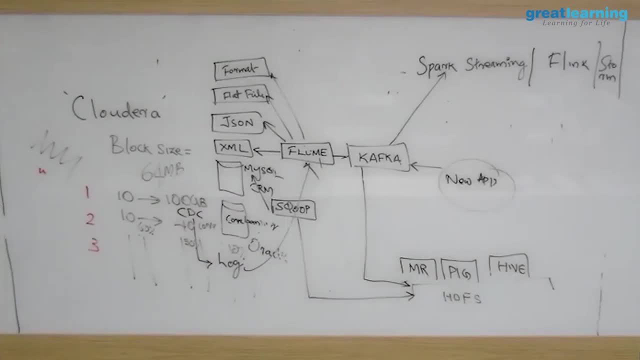 Instead of learning Java. right, We will learn. We'll stick with SQL. ETL jobs will run. They created this tool called Hive, So if I'm a Hive developer, I don't have to learn anything. It's SQL. I say: create table. create table join. 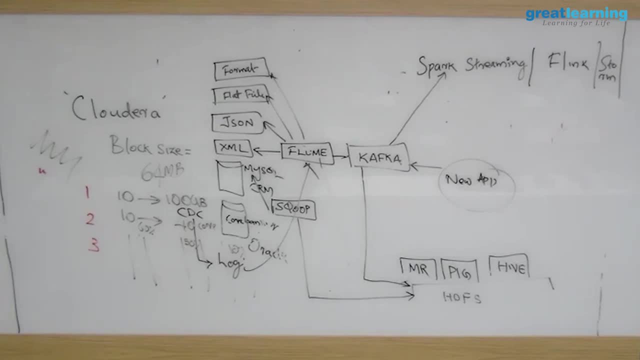 But once I say join, it'll write a MapReduce for me. then the MapReduce will run. I may have to wait for in fact in Flipkart there was a Hive query which took around 12 hours to run. Then they fine-tuned it and all. 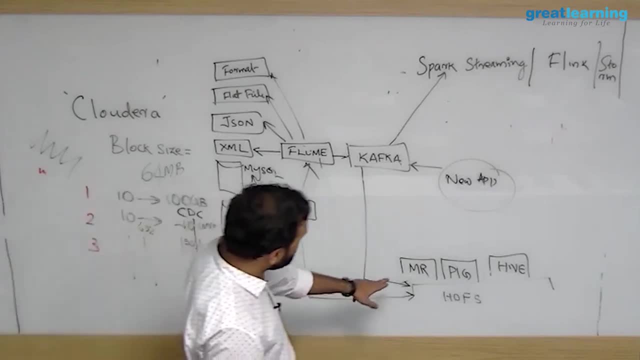 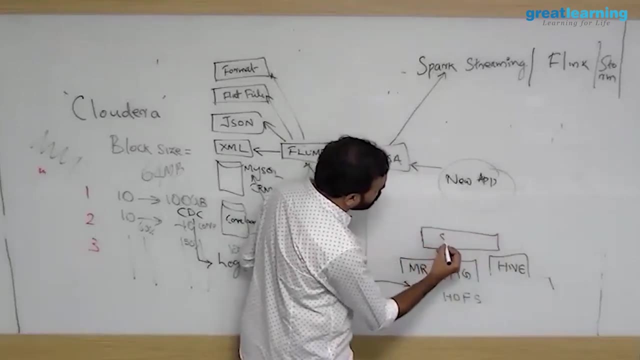 but that's a different story. But these are all batch processing systems built on top of Hadoop, right. And then you have Spark. you will learn Spark later. I don't want to confuse you a lot. So Spark is there and this guy is inside Spark, okay. 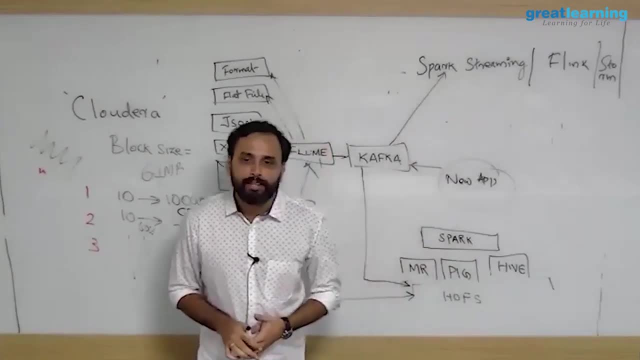 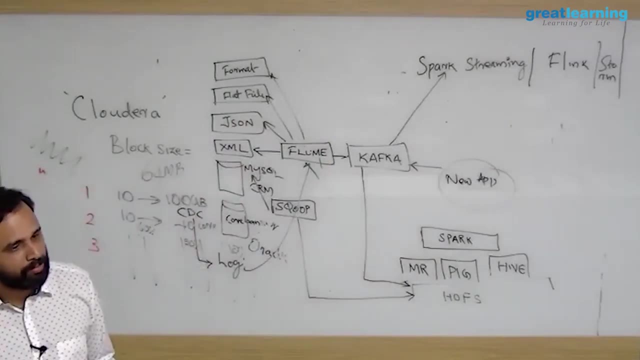 Even though I wrote it here, this guy is inside Spark. Spark is an in-memory execution engine. Spark is again classified as a batch processing system, but very, very fast than MapReduce. Only difference is that Spark programs are faster than MapReduce programs. 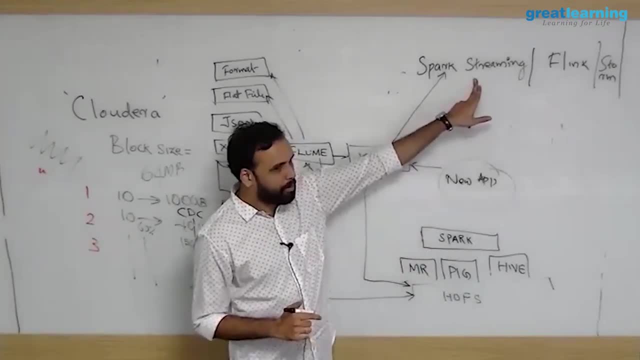 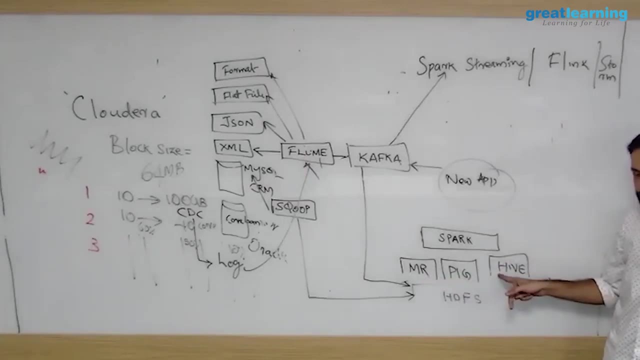 near real-time, not real-time. So Spark streaming is actually real-time, but it's near real-time, not like 100% real-time. MR and PIG are obsolete. Hive is not obsolete because Hive is your data warehouse, where you create tables and store the data. 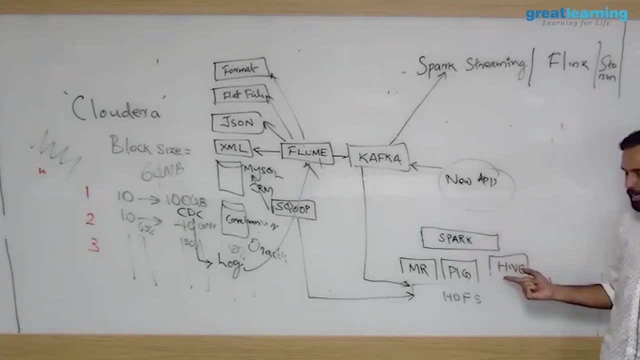 So this guy will remain. but now what is going to happen? Spark will connect with Hive And Spark can write. ah yeah, So here you can write a SQL. okay, Spark has a Spark SQL library. You can read tables from Hive and run on top of that, right. 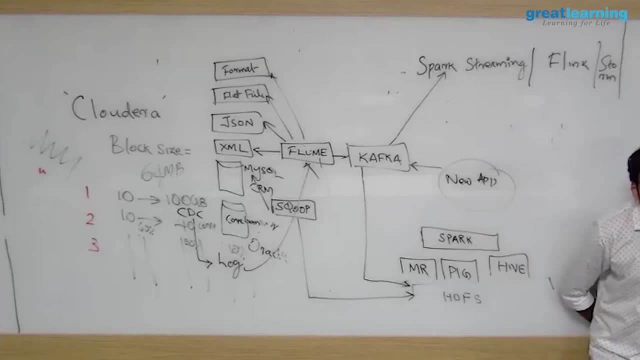 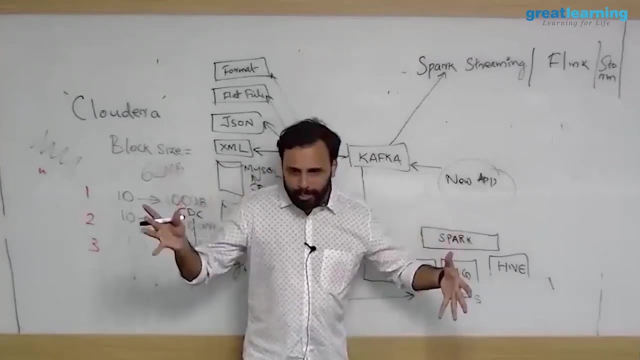 So Spark will start talking to Hive. So Hive is not really obsolete Hive. so if I want to run- okay, again there is a confusion- If I want to run a very big group by query, let's say I want to read the full table scan and run a query. 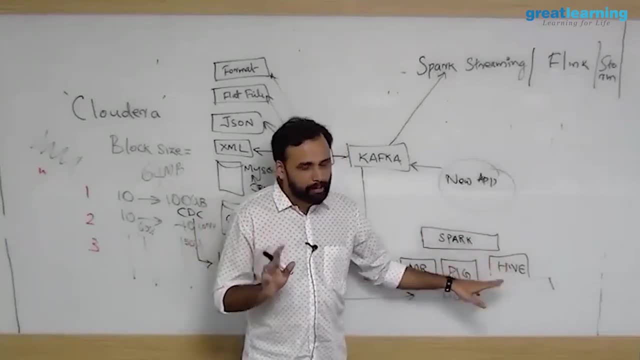 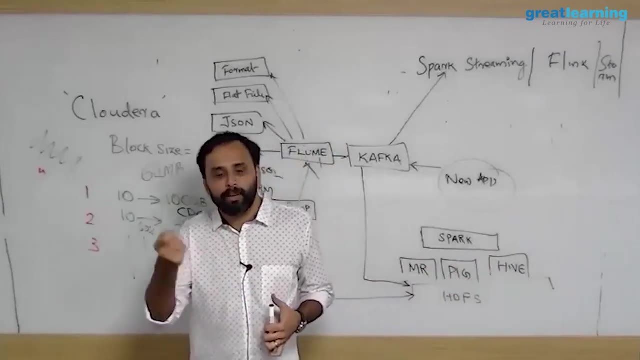 Hive is great. Even Spark SQL with Hive is great Because they will read the whole data and process it. But if I have minute queries, let's say select something from the table where name equal to Raghuramani, Only one row it needs to process. 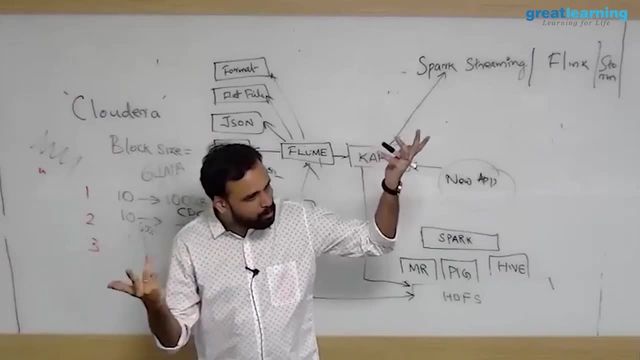 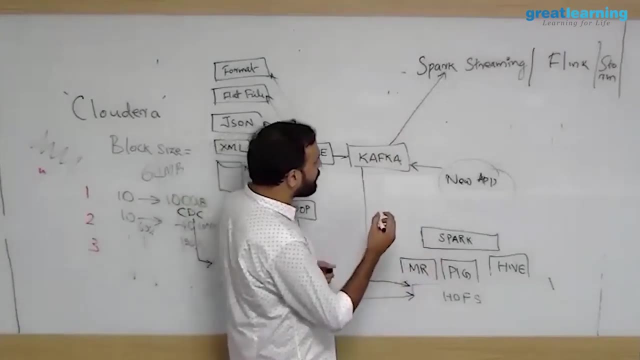 For that. why should I load the full data and process? It is useless. But Hadoop says: load everything sequentially and then process. that is only possible. That is where you have this. MPP engines Impala. There is one guy called Impala. 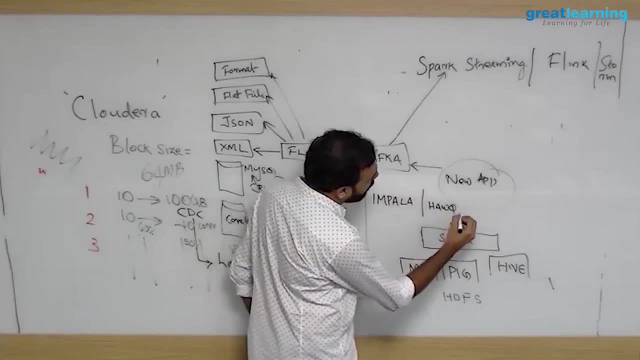 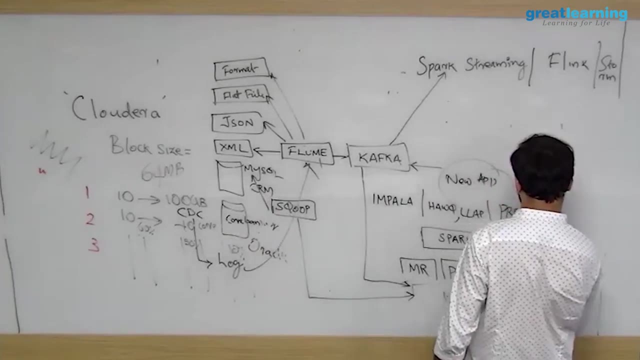 There is another guy called Hawk Hawk and LLAP. There is something called Presto Presto. There is also something called what is that? Drill Phoenix. These are all MPP engines. What Impala does is very simple. 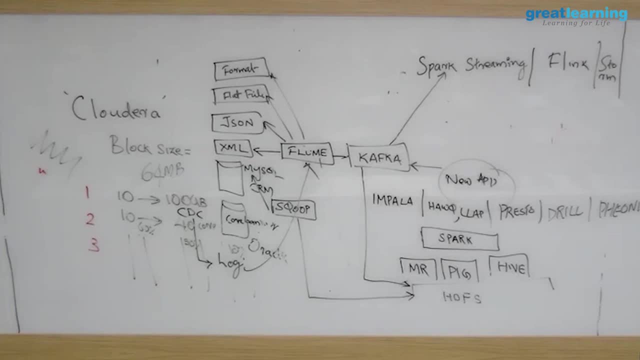 It has its own execution engine. You fire a SQL query, it will run it for you. No MapReduce. So what is going to happen for these queries like where name equal to Raghuramani, you can fire an Impala query. 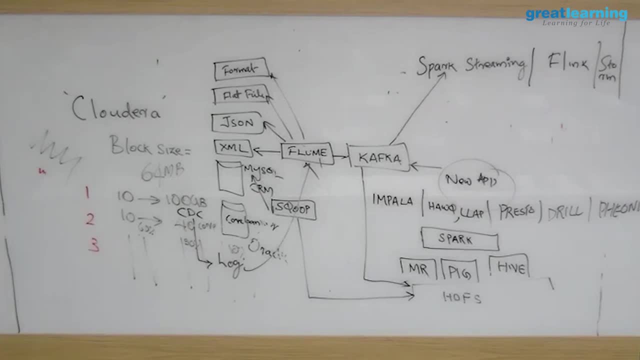 It will scan only that data. So it can connect with HDFS and pick only the data, because it remembers the metadata: Where is what data available? It can columnar, It can pick that data and query. But then you will be wondering why can't we? 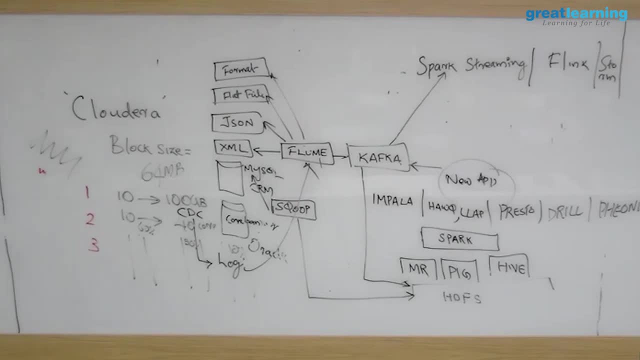 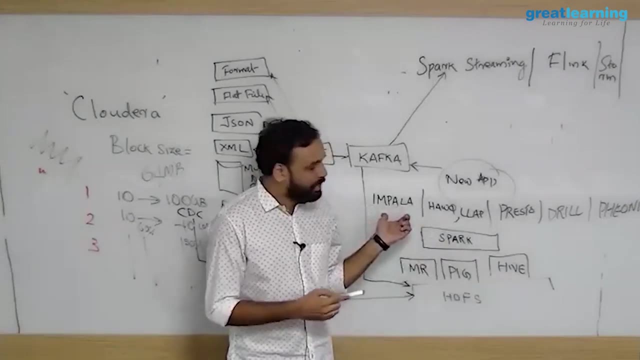 use this instead of Hive If- and these guys are very fast, So if these guys are too fast, then why don't I use them instead of Hive? They don't have reliability. They are all in-memory queries. If an Impala query is running in my Hadoop cluster, 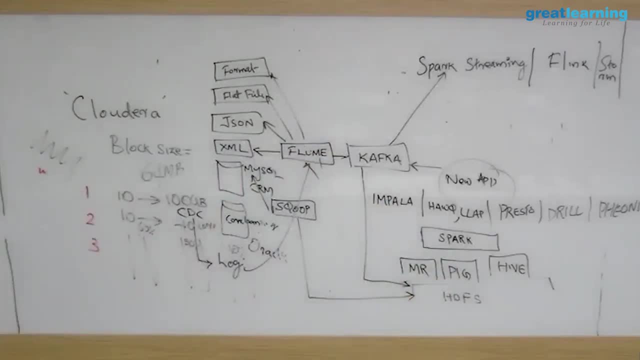 if any one of the machine crashes, my query will be gone. If a Hive query is running, even any machine crash query will complete. It is MapReduce. Built-in redundancy is there? MapReduce will never fail Or Spark will never fail. 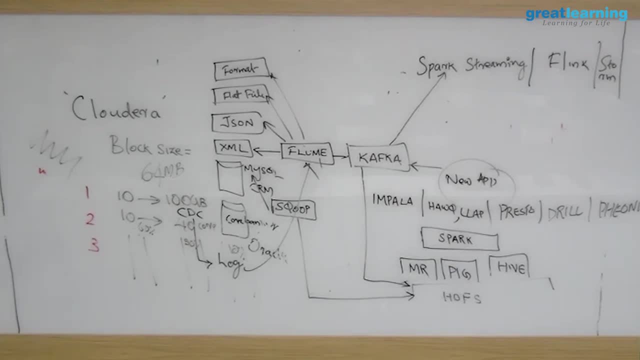 But if I'm using Impala, it has its own metadata. It knows where is the data. It knows only that and queries will be faster. So if I run an Impala query considering a Hive query, Impala queries are much, much faster. but no fault tolerance. 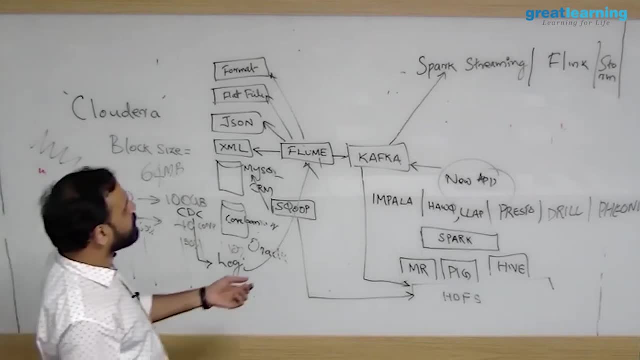 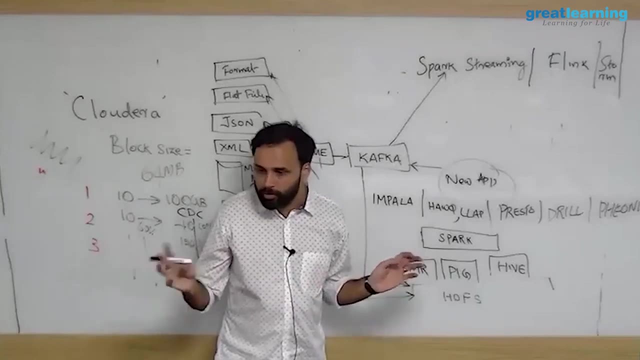 So for these very fast queries like your queries can take like two minutes, three minutes time. you can afford to lose a query using Impala But if I'm having a ETL job where I don't want the job to fail, run it using Hive or Spark. 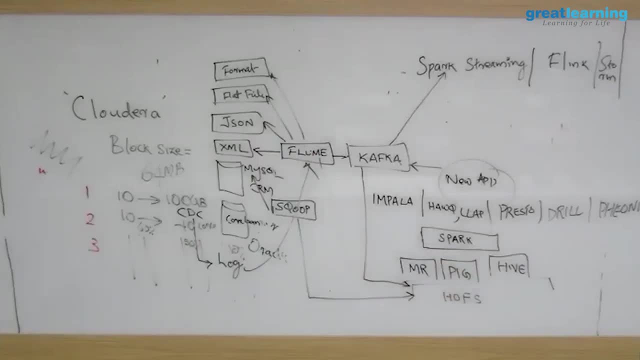 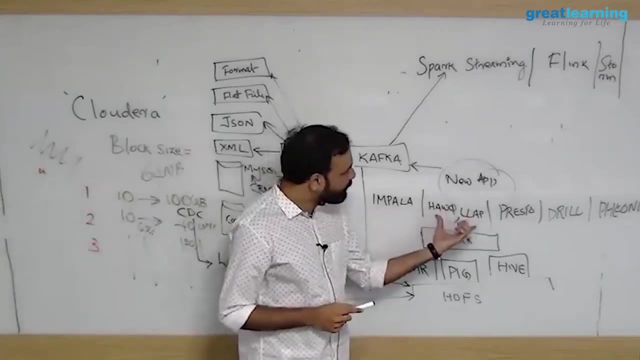 Because these guys will never fail. So all MPP engines are like this, I think in the traditional world also. In this the difference is: Impala is on Cloudera, Hawk and LLAP are Hortonworks. There is a competition. 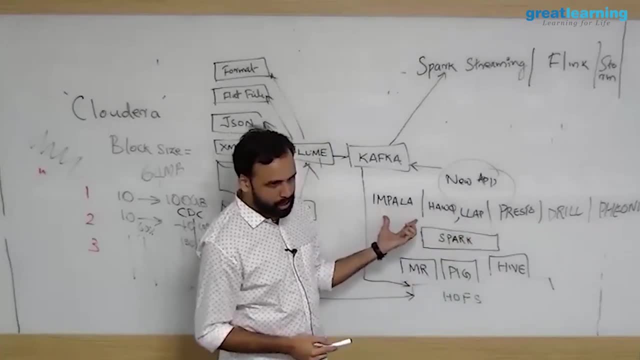 Impala was originally created by Cloudera, So they promote it. If you're on a Cloudera platform, you will see Impala. If you're on Hortonworks platform, you will never see Impala. They will promote Hawk. 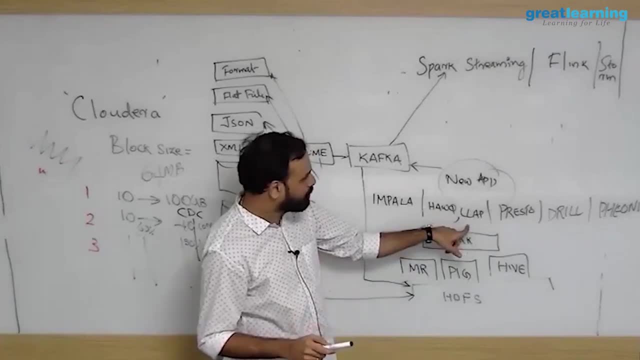 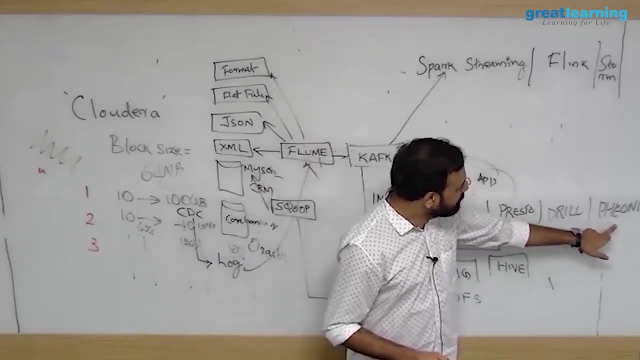 They will say Hawk is the best engine And LLAP is the new version of Hawk, Presto Drill and all are similar ones but not by default available. This guy is very, very interesting, So There is something called HBase. 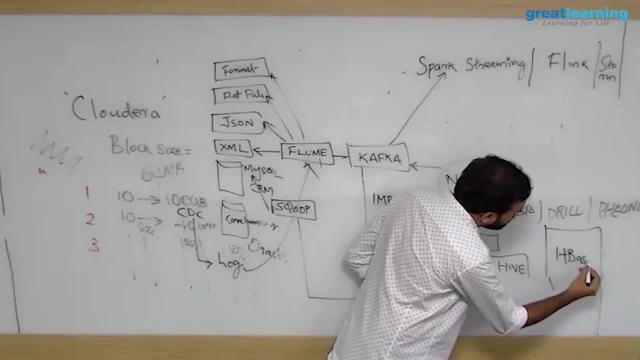 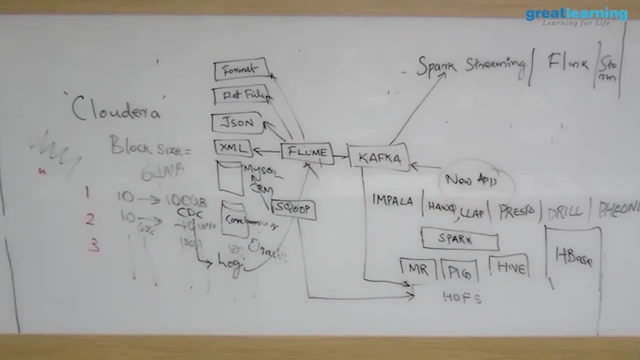 I will add it here. Somebody was asking me: what is HBase? HBase is your database of Hadoop, No SQL database, Real-time database. Real-time Because HBase will get installed on HDFS. That is your storage right. 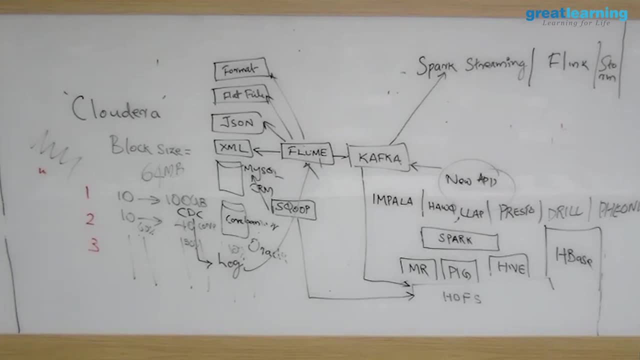 But it can do random reads and writes, not like entire block. So normally when you are reading the data from HDFS you have to read the whole block, Right? But HBase has an API. So if you install HBase on top of Hadoop, 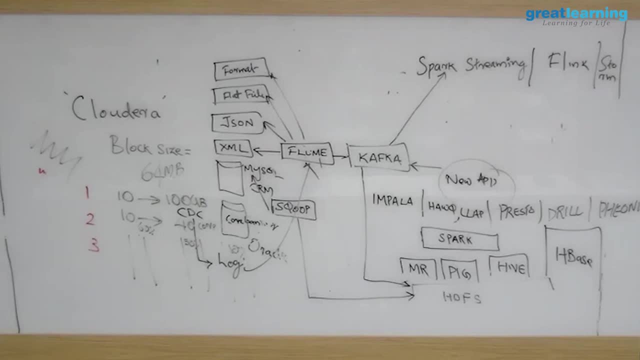 it can do random reads and writes Individual records. it can read and write and process Because it is a NoSQL database of Hadoop, The default NoSQL database. But the drawback is HBase has its own language. So if somebody has to work with HBase, 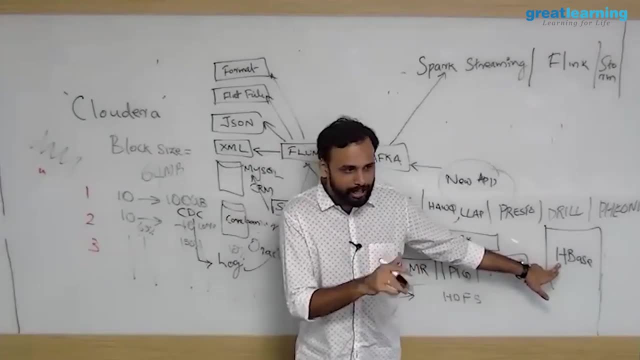 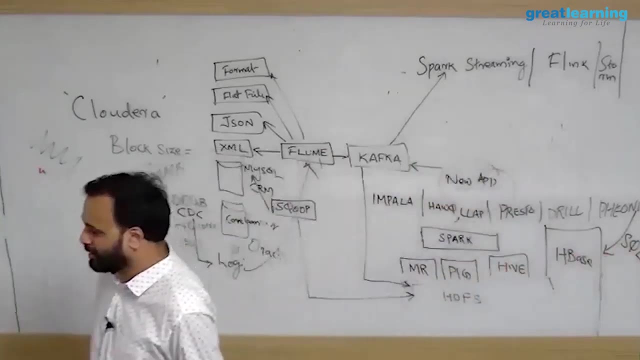 you have to learn the language. It will not allow SQL queries. Phenix is SQL on HBase, Right? Yes, Yes, Yes, Yes. Phenix and HBase is like roti and paneer butter masala: Deadly combination. 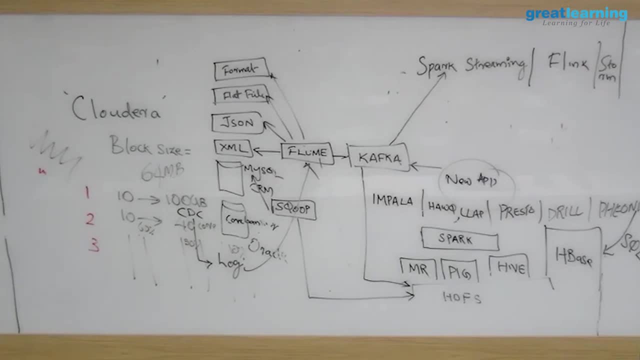 I mean very deadly combination Because you are writing SQL on top of NoSQL, Right. Very deadly. So they say that in another two years It will not be slow. It's really fast Because HBase itself is fast SQL. there is a conversion. 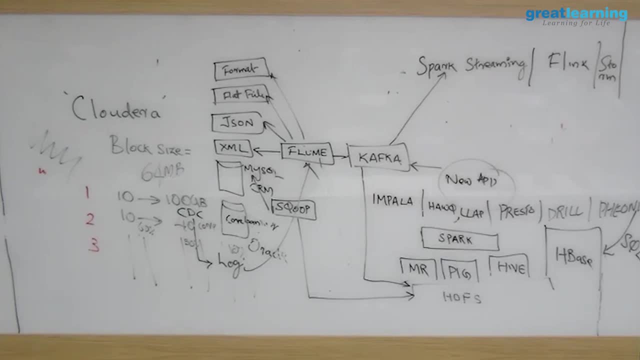 But that's already built in Any SQL query. there are some limitations, But so Phenix will get all the metadata And already it's going to be a lot faster. Already all the queries are converted, Whatever query SQL you are writing. 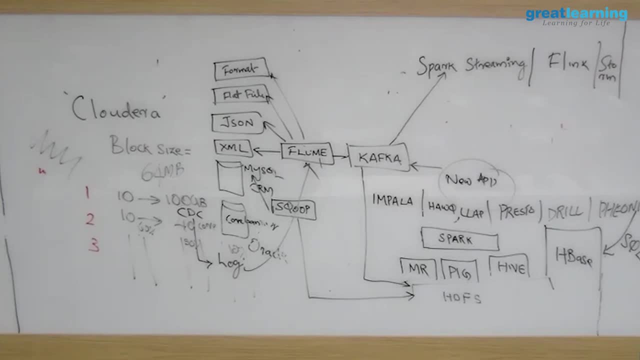 it knows what is the equivalent HBase query, So it doesn't just push the query, So you just write a SQL, it will run on HBase and give you the result And it can do things like secondary indexes and all It can index your data apart from HBase. 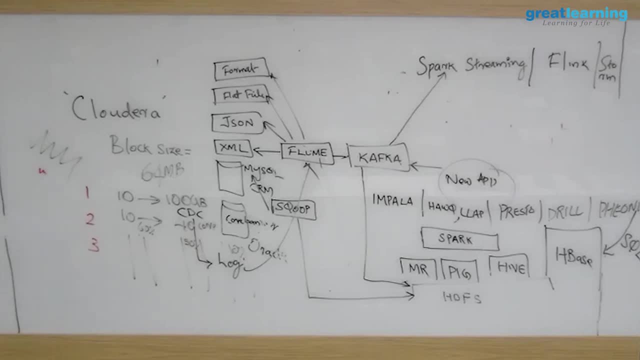 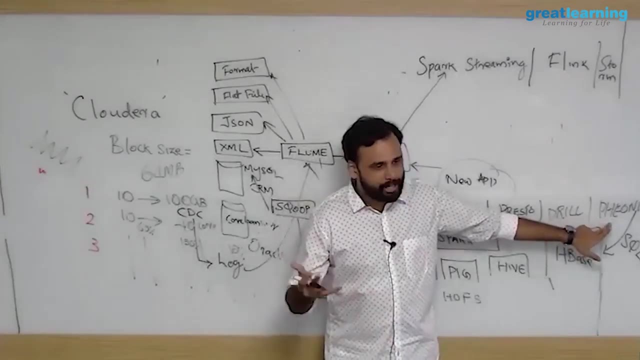 It's very fast Now. the real news is that in another two years, what is predicted is that this combination. the drawback is Phenix is still in alpha beta. Phenix is not production ready. Once Phenix becomes production ready, this is OLTP. 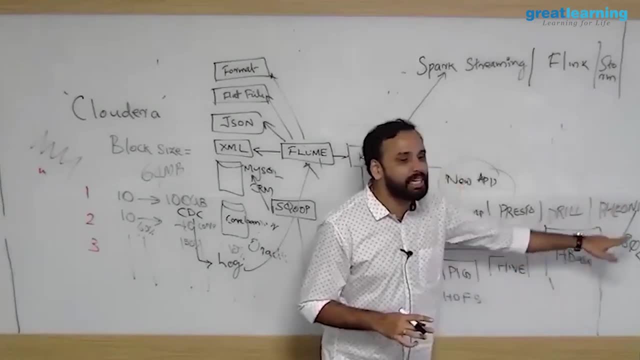 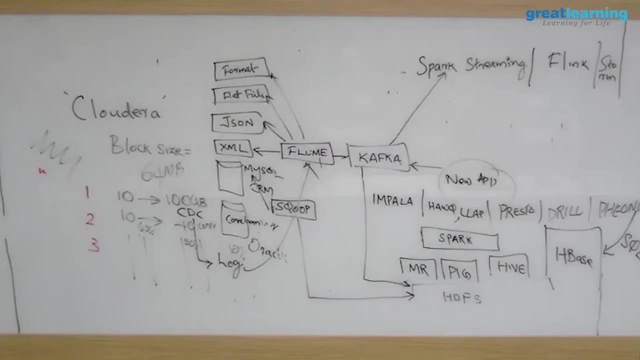 So they are trying to make it asset support, so that this entire combination will become an OLTP system like that. So then what will happen? You will get transaction management in Hadoop. So far, it is not there. Another two years down the line they say that. 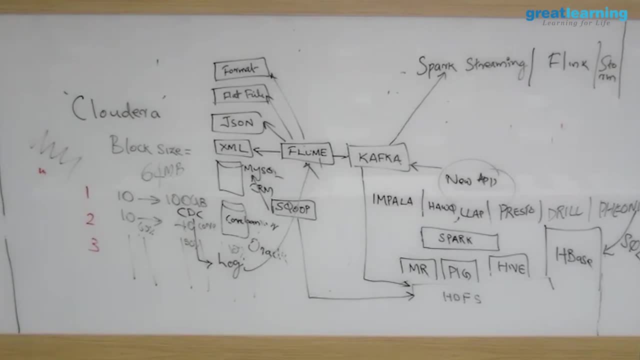 So Phenix is getting integrated with HBase. Originally HBase was only there. The drawback is it doesn't understand SQL, So Phenix started. Phenix is a layer on top of that You can write SQL. So in another two years they are going to be able to do this. 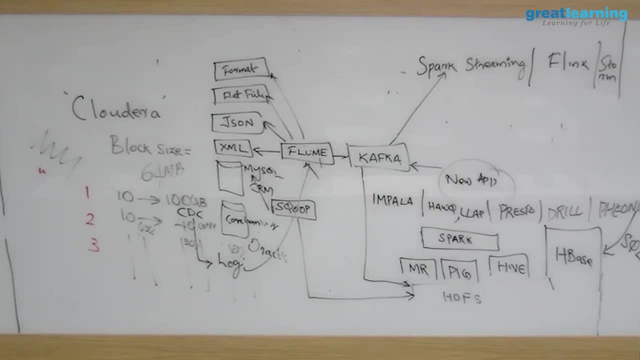 They are developing this as a system for transactional management, So you'll get true transactional management in Hadoop. So if you talk about the Cloudera and all, if I'm going to Cloudera and say that I want your product. 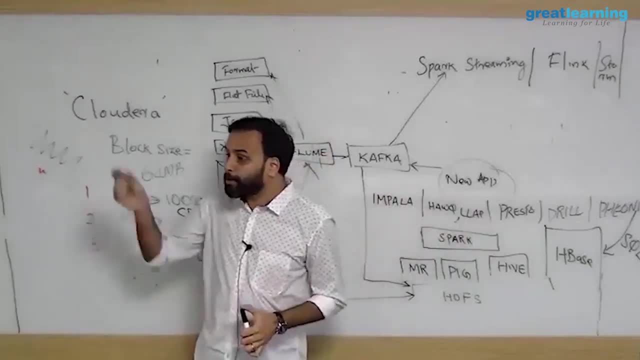 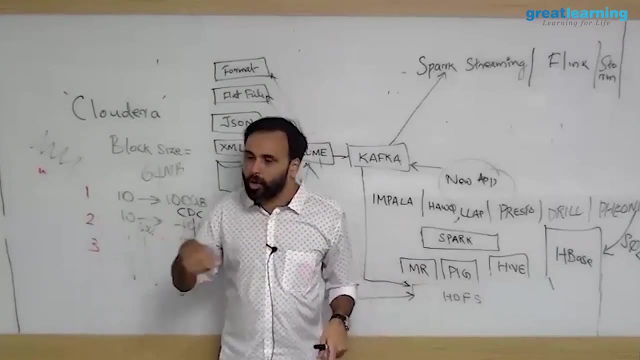 they will give you all this in one package. But if you go to Apache and download, you get only HDFS, MapReduce and Yarn, only Hadoop. All this you have to separately install. So commercial distributions will package it. 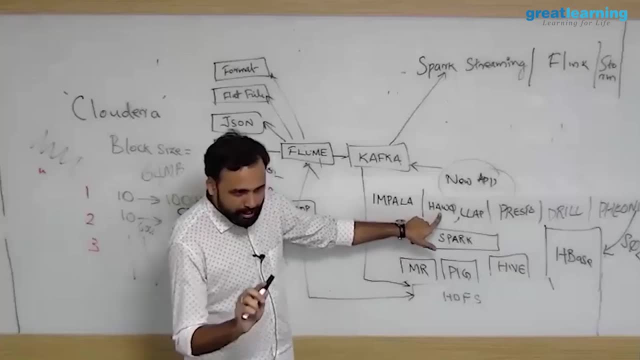 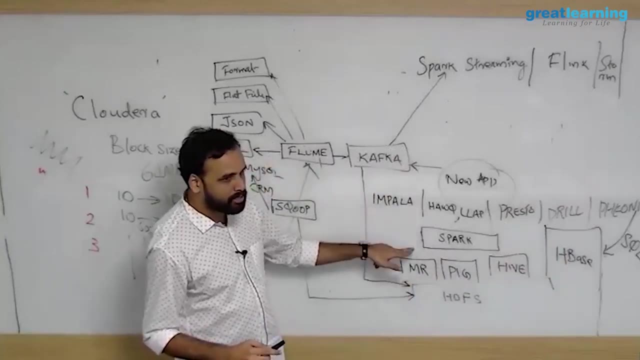 You will not get everything. OK. For example, Hop will not be there, This Presto Drill Phenix. You will get HBase Hive Fig, MapReduce, Spark Impala. So these things you will get. Look at here. 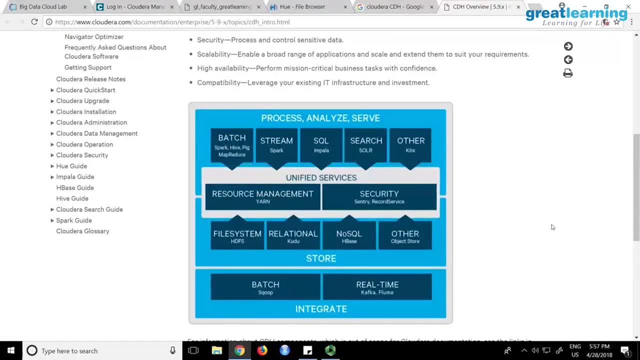 Spark Hive Fig MapReduce. Spark Impala Yarn right, But you have HDFS HBase, Kafka, Flume Skoo. This is a real product from Cloudera. You go to Cloudera, this is what you get. 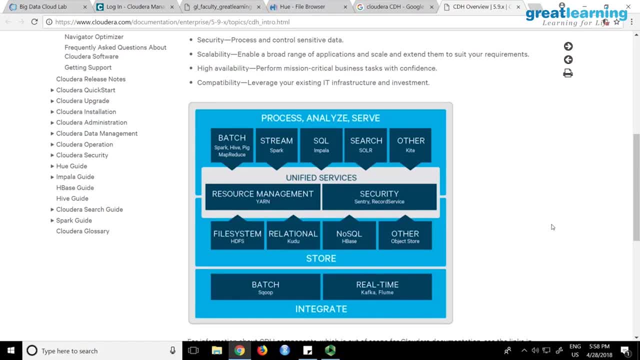 Some of them I have not even explained because I don't know Kite. I don't know what it is. to be very honest, Kudu is a new file system, relational Even I'm not sure I'm not aware of Kudu. 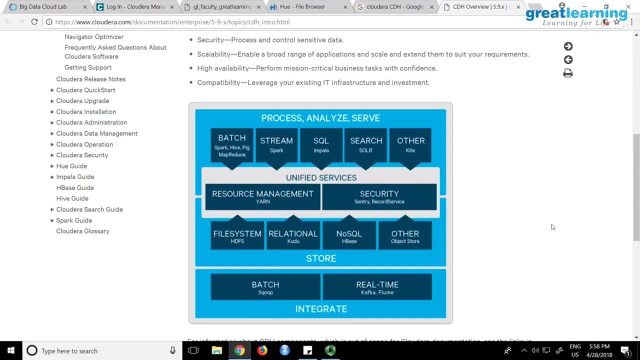 I don't know what it is, But these are like new entries. Even if you don't know them, you will work without any problem. And for security you have something called Sentry. So a lot of people are worried about security. on Hadoop: 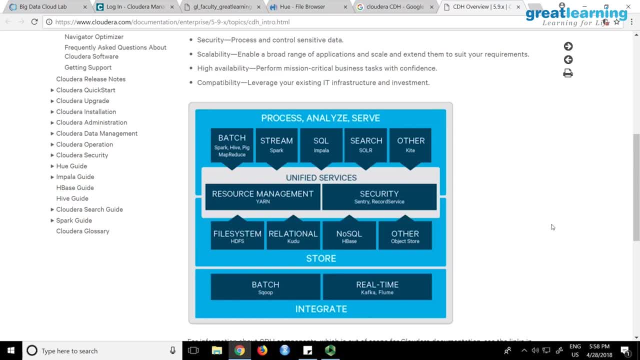 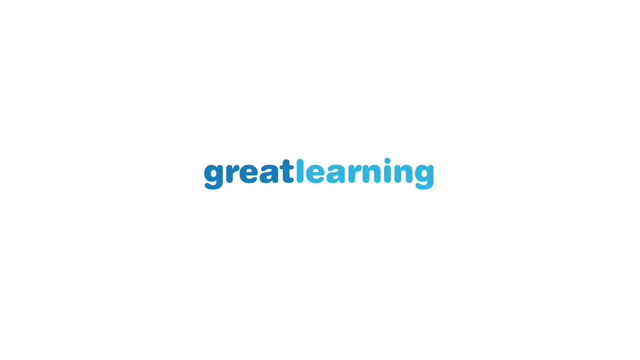 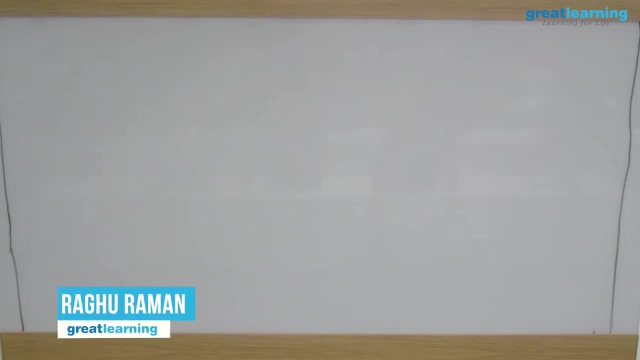 There is a service called Sentry which will handle access management, authorization, authentication. All this will be handled by Sentry. So MapReducecom- MapReduce- need to be understood in a very simple way. The problem is that MapReduce is very complicated and people mess up. 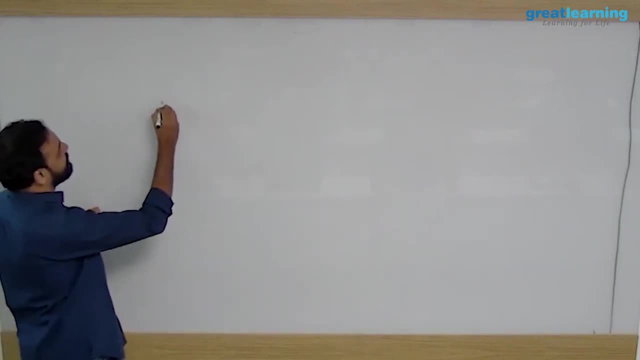 So the basic idea is: divide and conquer, Divide and conquer. This is the basic idea behind MapReduce and it is not a very new idea. Also, MapReduce is not a new framework. MapReduce was there in 1970s and it is a general concept. 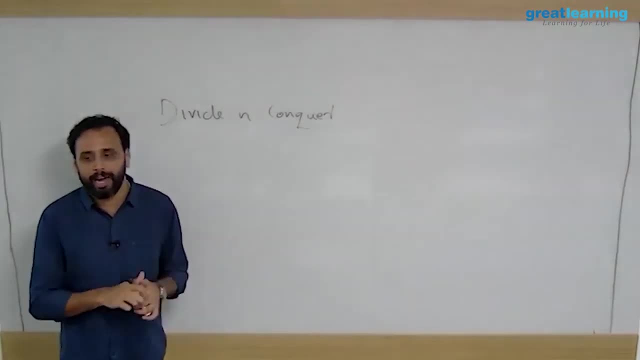 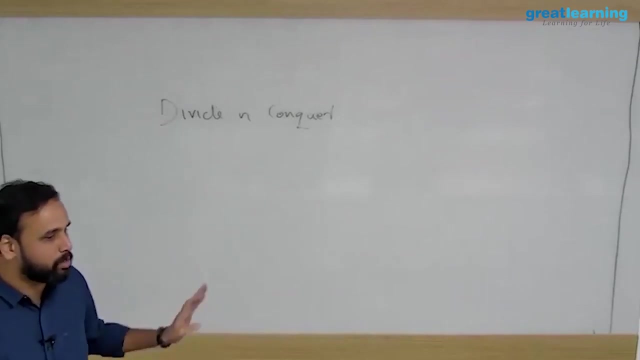 It's not like Only to Hadoop. you are using MapReduce. So I have been working with different tools like MongoDB. MongoDB uses MapReduce, Splunk uses MapReduce. Hadoop also uses MapReduce, So it is not only to Hadoop. 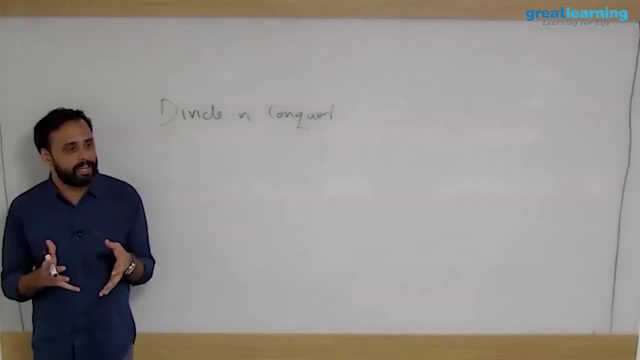 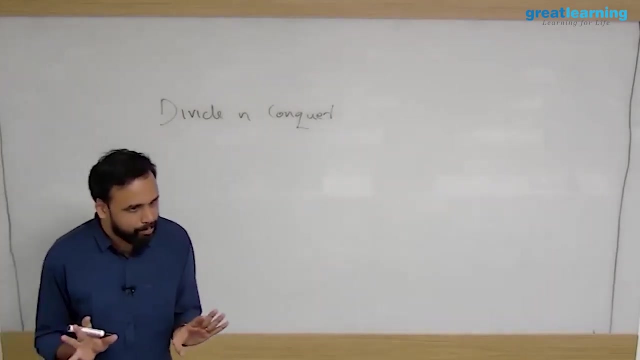 Some people have this concern. MapReduce means I can write only in Hadoop. Second thing: MapReduce is a framework, which means it is not a language. You can write MapReduce programs using any language you want: Java, C, C++. 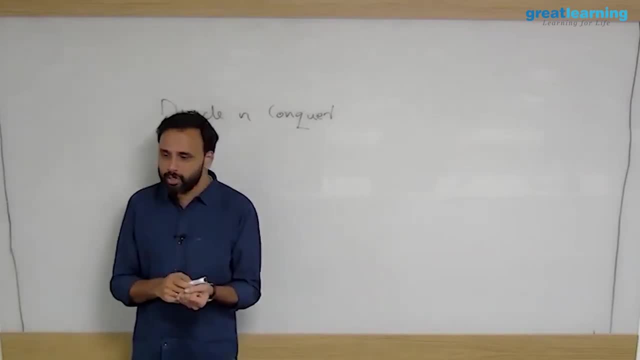 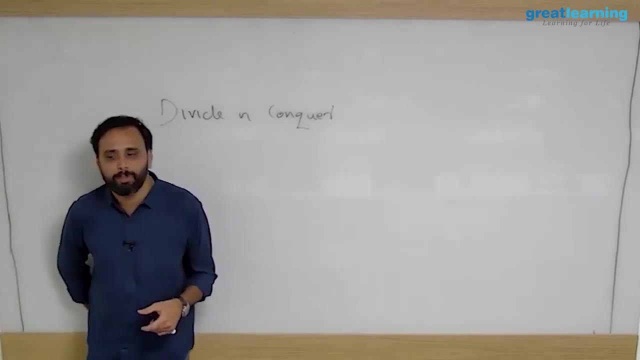 Python, C++, Python, Ruby. So it is not a language, It is a way of programming. So if I'm a C developer, I can write a MapReduce program using C, No problem. No, Google was using it in their project. 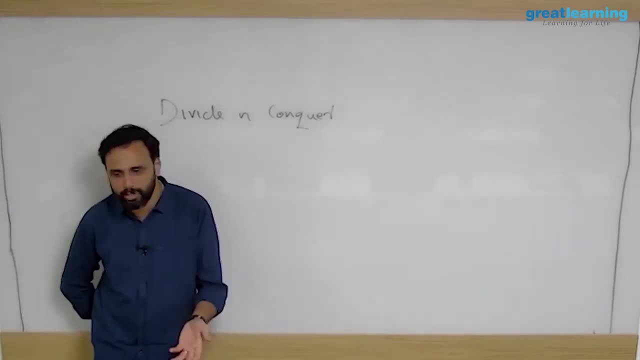 So Google published a MapReduce paper. That is in 2001 or 2002.. Google was also using it. Google has their custom technology to manage their distributed network. They were also using same MapReduce And Hadoop was modeled after that. actually, 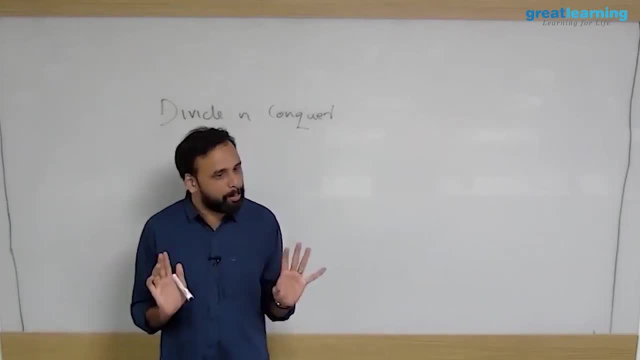 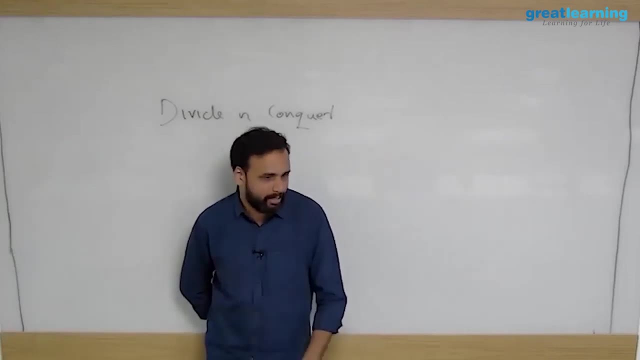 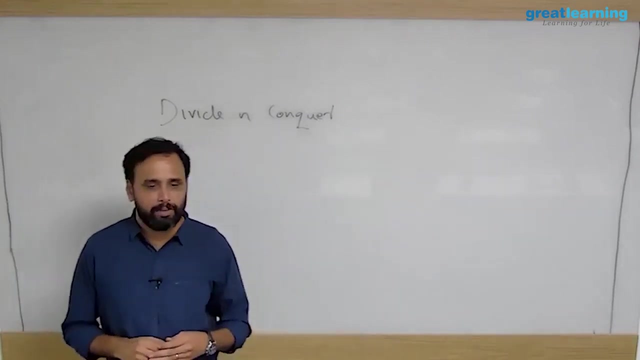 What Google was published. My point is: the idea is common. Google did not invent MapReduce. That is my idea. MapReduce was already invented. Google was using it for their network And nobody was bothered about MapReduce, because MapReduce is typically used for a large amount of data. 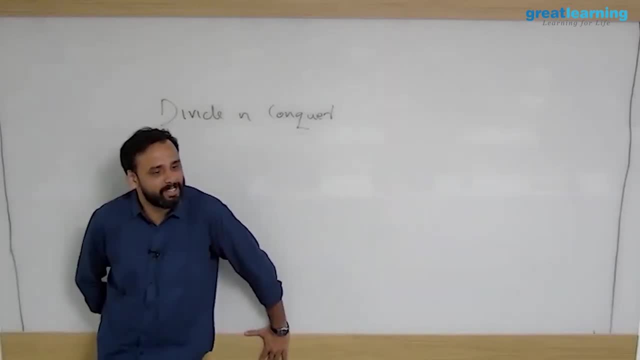 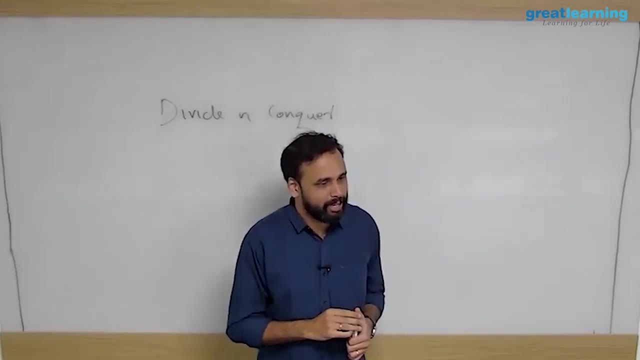 What if I appoint you as an election commissioner? Who is the current election commissioner in India And we are going to- or let's let all of us be election commissioners And we want to run elections in India? Now I am telling that let's do one thing. 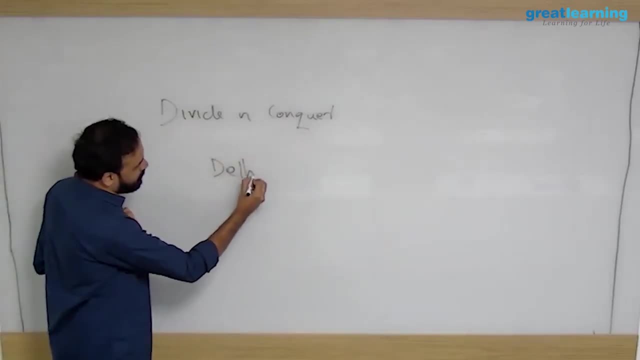 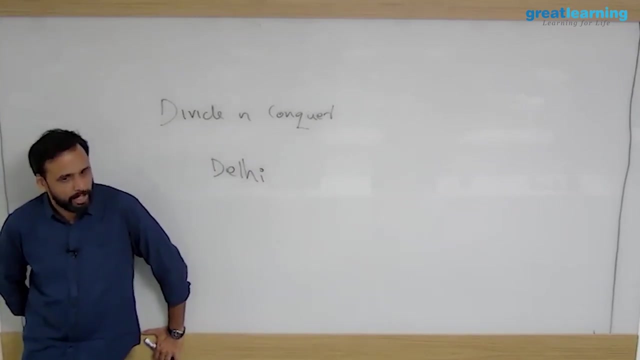 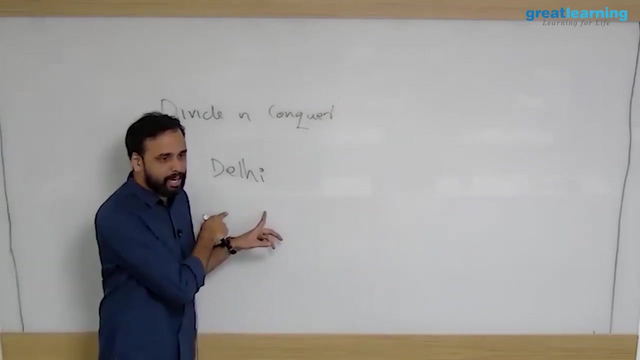 We will conduct the elections in Delhi. The idea is that there will be only one election That will happen in Delhi, No individual constituencies or nothing. Anybody who wants to vote has to come to Delhi and vote. Imagine, I'm just giving a theory. 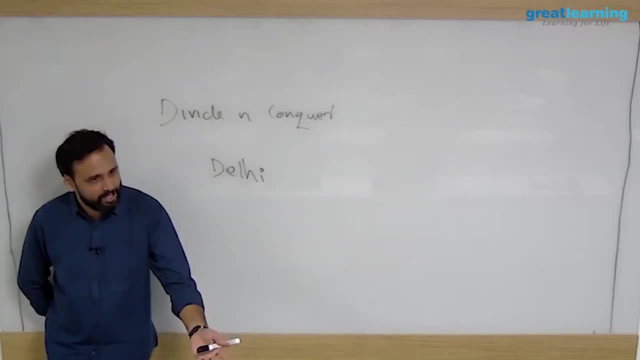 So I'm proposing today that 2000,. when is the next election? 2019.. OK, Right, In 2019, national election. this is what is going to happen. You want to vote. you come to Delhi, Otherwise don't vote. 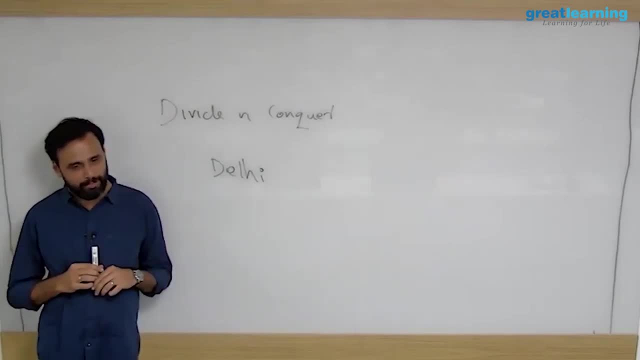 So can I say the problem here is movement of people Right. The process is election. What you're running is election And people want to travel to do elections. So if everybody come to Delhi, it will create a lot of chaos because people 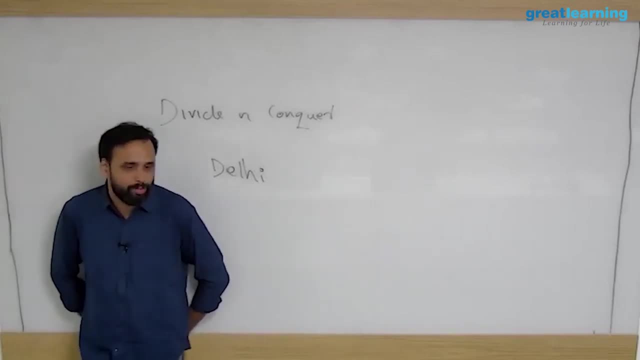 have to travel all over And it will mess it up. Probably people will say I will not vote. also, What is the single advantage of this is that I can run everything in one shot. That is the advantage. Now, if India was a very small country, 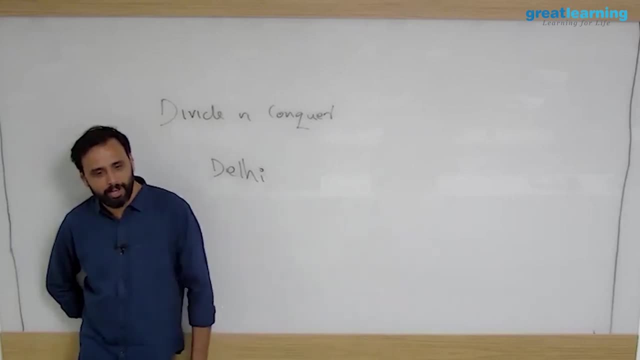 let's say we had only 10,000 people in India. will this work? Yes, Right. If India was a small country in size and population, this will work. This is your traditional programming, This election is your program And the data will come to your program. 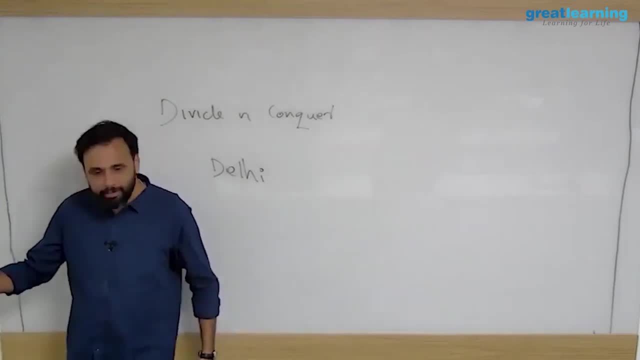 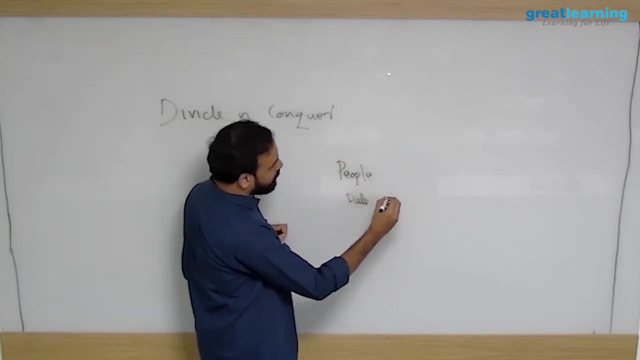 I write a Java program, I run it. OK, My program will be running in my server And it will read the data And it will process right. So data comes to the program. So people, is your data right? They come to election. 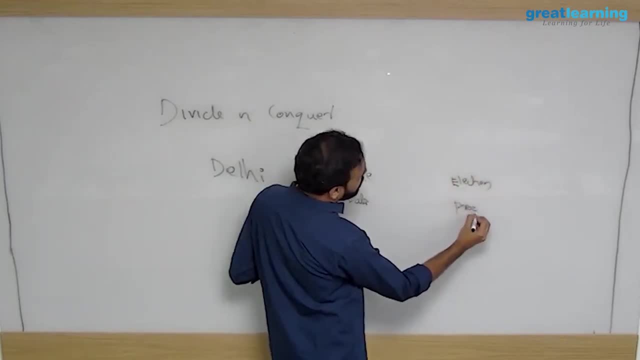 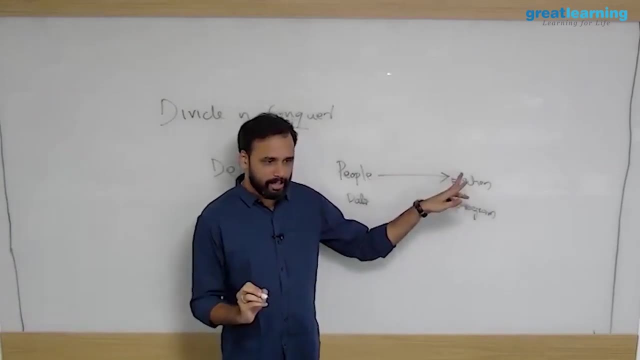 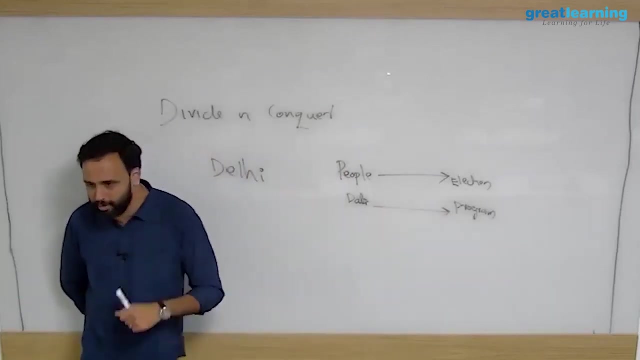 Election is the program. So what happens is that if you had a small country, all of them can assemble in one place and cast their vote, Just like your data will be sent to one program and the program will process your data Like you run a normal Java program. 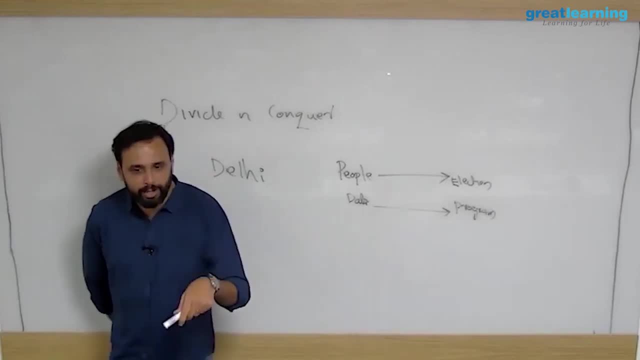 In the world of big data. the problem is this, Like right now, if I try to do this in India, the people are more. Size of country is more Meaning, data is more Right. So if I have a Hadoop cluster, let's say we have a Hadoop. 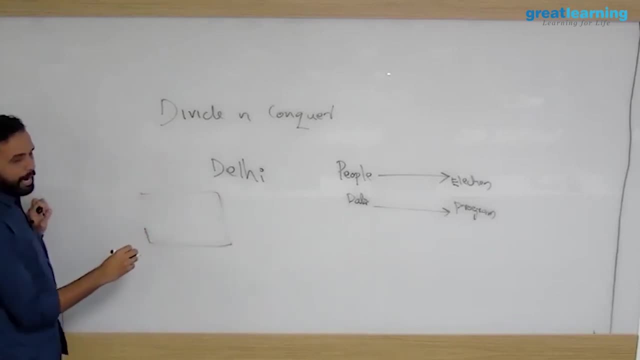 cluster. there are a lot of data nodes inside that. I write a MapReduce program. We have not discussed what is MapReduce, but I wrote a program And if I have to get data from this program from all places, places and then process it will be chaos. 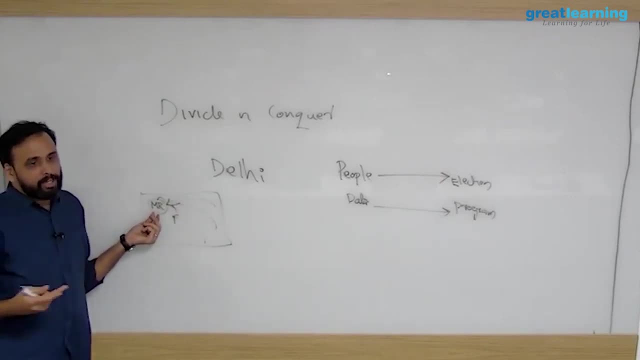 Because my program will be running on one machine. let's say, Data has to travel from blocks, from every data nodes, and come here and process. That is useless actually. So we do the reverse Rather than the data coming to the program. 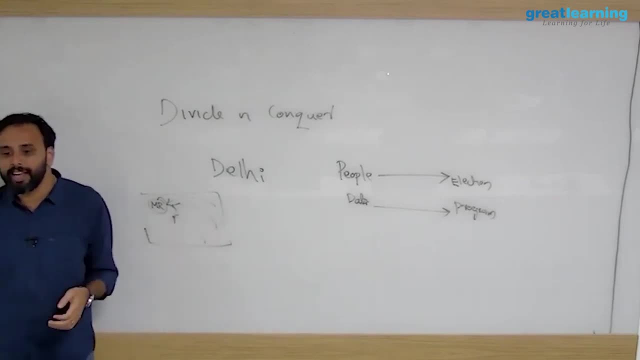 the program goes to the data And that is exactly what is happening in election. How does election normally run? Election is your process. The process will go to people. People will vote. People will not come to the process. See, I stay. I live in Kerala. 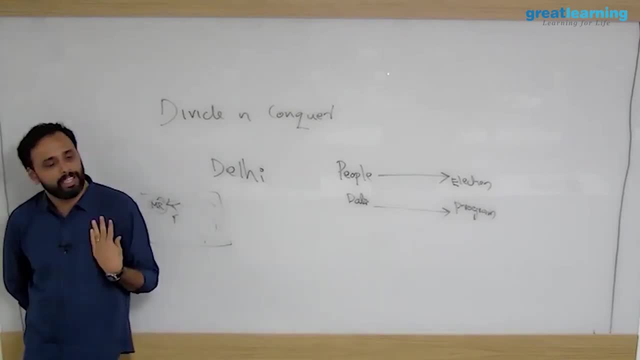 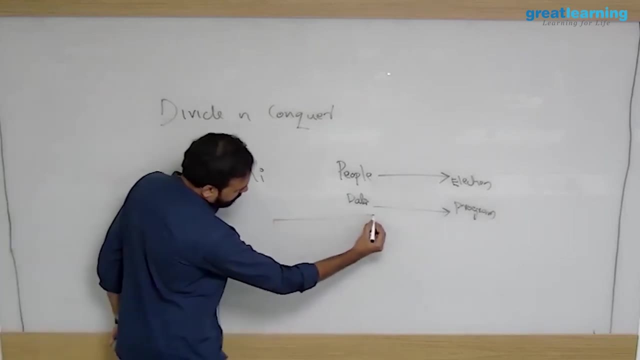 Right. So I have a constituency nearby. If I want to cast my vote, I go there. Election will be running everywhere. So normally, if you take India, for example- just an example- OK, you will have a lot of states, right. 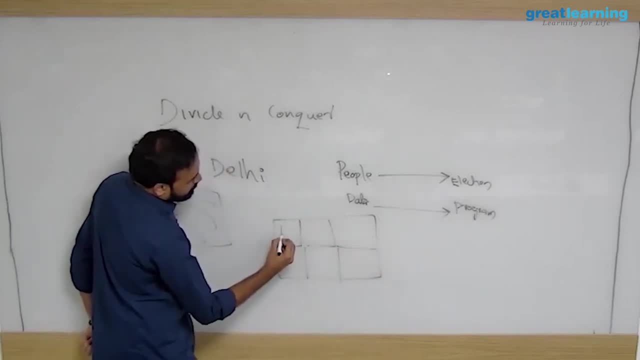 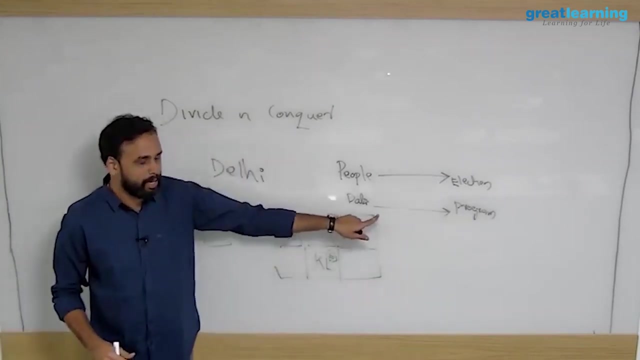 You will have n number of states. Let's say you have Karnataka. Let's say you have Andhra Pradesh. Let's say you have Kerala. Just an example: Same election process. We'll go to every state and get run there. Every state election will happen. 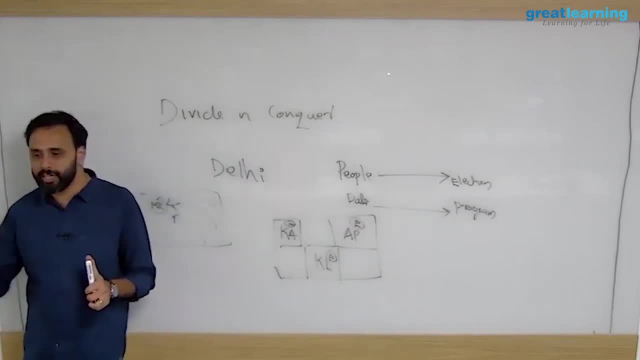 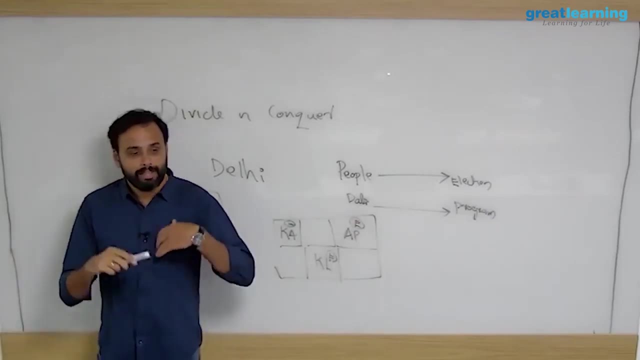 Now the election process in Kerala is independent of election in Andhra Pradesh. I can run same elections on one day, parallel process. But the other side is that so if in Kerala I'm not being political but still let's say in Kerala BJP wins. 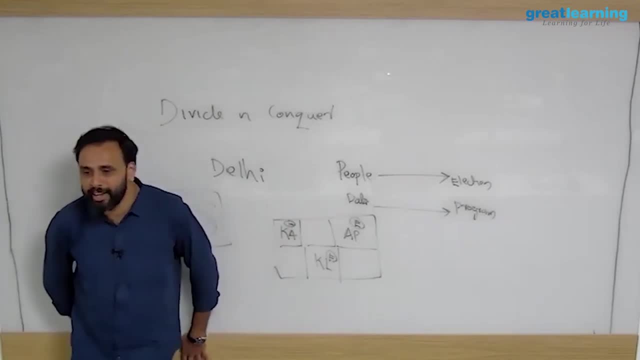 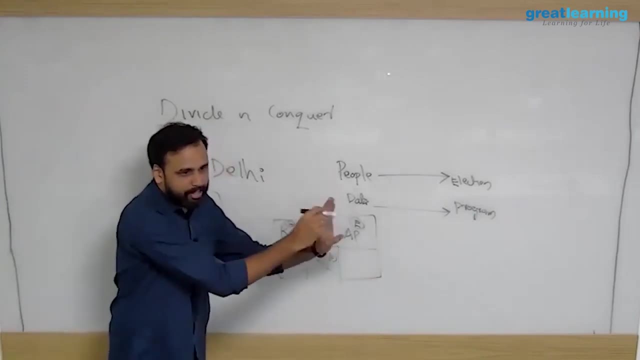 Does that mean BJP wins in India? So what is the result of Kerala? is a local result, Only to Kerala. So one first phase: I have to do the total election in every, every state. Once that is over, what do I do? 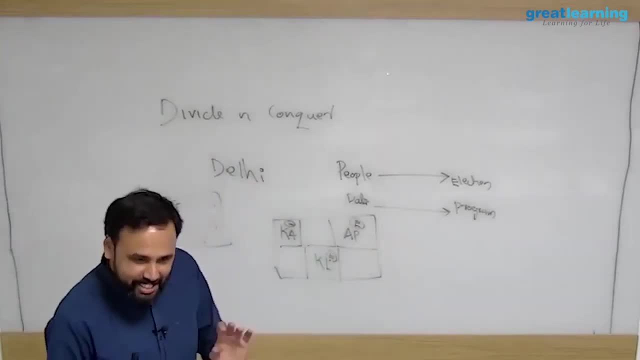 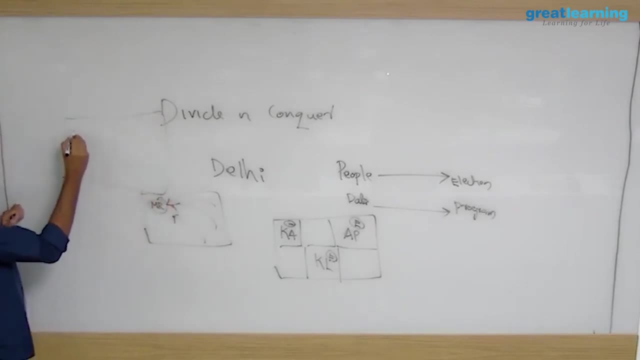 I will consolidate and give the final result. This is MapReduce. Very simple: In MapReduce, what we do is the same thing, right? So you have a Hadoop cluster and you have data nodes. This is your data node, right? 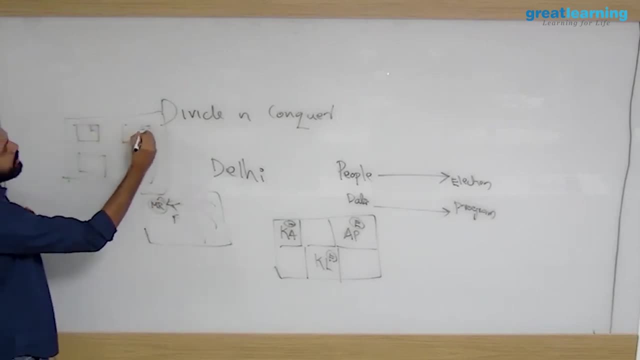 This is your data node, And imagine my data is here, here, here and here. I'm just assuming. I have four blocks of data And I want to analyze the data. I write a program called MapReduce program. In MapReduce program there are two programs. 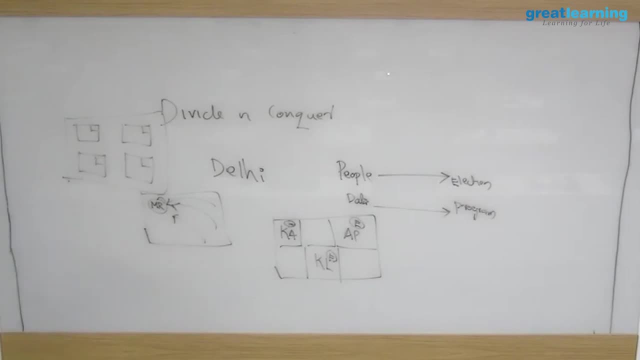 One is called Map and other is Reduce. That is why you call MapReduce, right. So when you are building a MapReduce program you will be writing a Mapper program and Reducer program. Mapper program is phase one of election. So easiest way to understand that is: Mapper is election phase one. 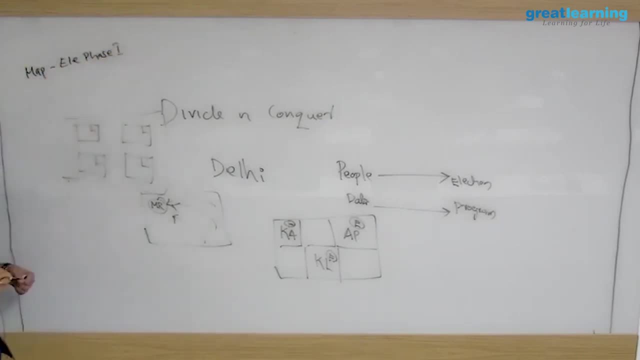 Okay, Mapper is election phase one, Meaning whatever you write in the Mapper program, the Mapper program will divide itself, I mean replicate itself, and this guy will run parallelly on all the four machines. I will tell you internally how it works, but my Mapper program, whatever I wrote now I 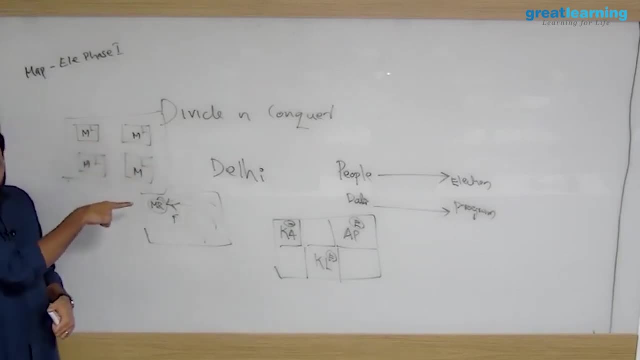 have only four data blocks, What will happen? Same Mapper program will run on all four machines at the same time. This is like running elections on same day in different states. So this is how it works. This is how it works. It is like running elections on same day in different states. 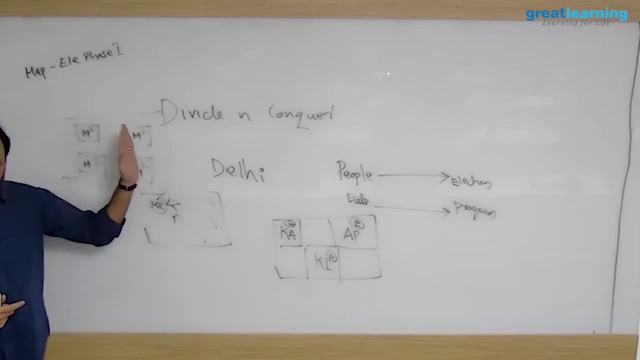 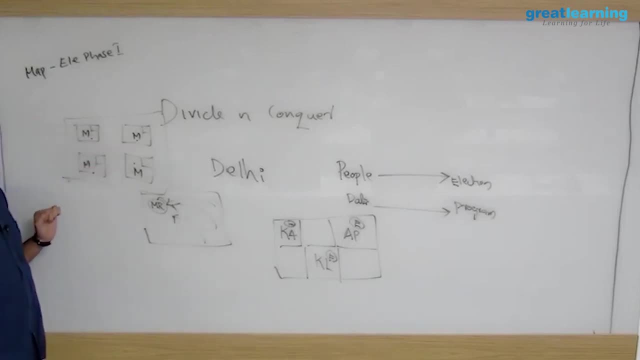 Then the Reducer program will kick in. Now, assume there is only one Reducer program, That guy- let's say it starts here- all this will be collected by this guy and it will produce final output. That is MapReduce. So in MapReduce you need to understand Mapper and Gopro. 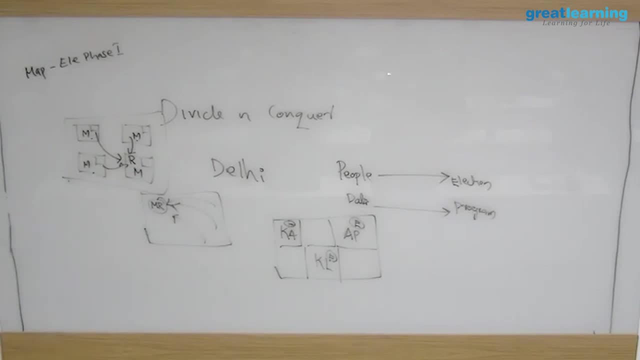 Okay, So let's see. Let's see reducer. that is the basic idea. the mapper program, whatever logic you write, will execute on every machine where you have a block of your data, whatever file you are giving right, and it will produce an intermediate result. this intermediate result will be fed into the reducer. so when 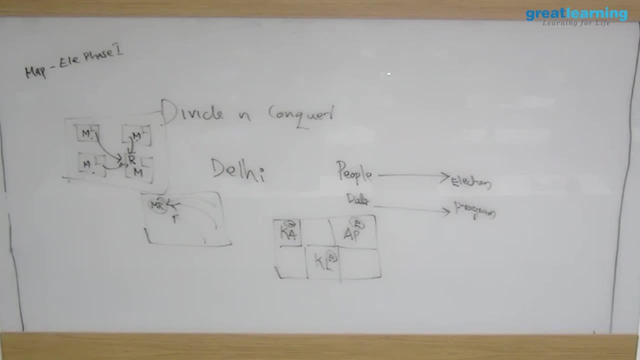 writing the code you have to figure out in the reducer. what should i write? because reducer will be getting the output from the mapper. so what is the output of mapper? right, so that will be fed to the reducer. the reducer will process that and then give you the final output. this is the. so this: 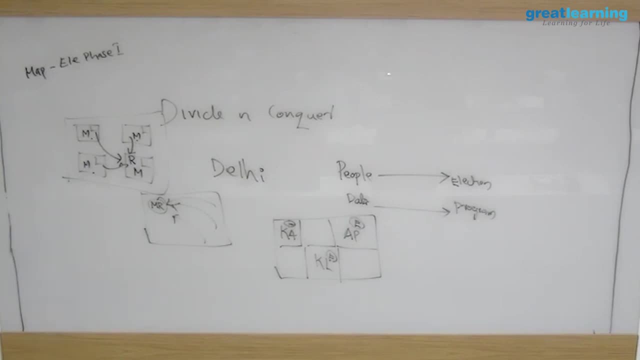 is the divide and conquer rule right, and the same concept is being applied in many, many areas in it, not only in hadoop, because wherever you have distributed data, this is how you process: first you ask them to process individually, then you collect the output and merge them in the second. 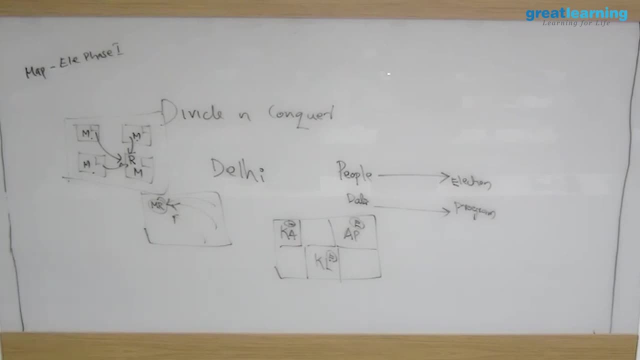 phase of the program. so this is just a high level overview. i mean, technically, there are more things. this is just a high level overview. i mean, technically, there are more things. this is just a how it works. actually, you can decide by default. there will be only one reducer in a map: reduce. 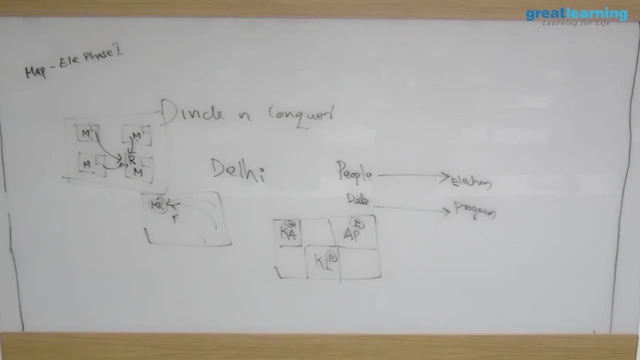 program. if i simply write a map reduce program, it will call for one reducer only, but sometimes so. in this example it is okay. i have only four blocks. one reducer may be able to finally aggregate everything and give me the result. but if you're having huge amount of data, let's say you're running. 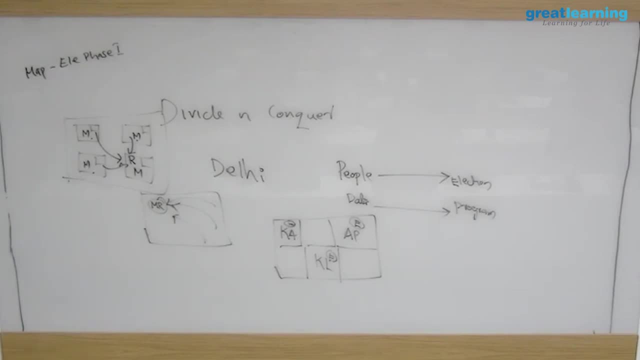 100 mappers, the output. if all of them send to a single machine, it will become your omr road evening 6 pm. right, what will happen? full jam, right. reducer cannot run so the developer can write in their code how many reducer you want. so there has to be some logic for this. you have to calculate. 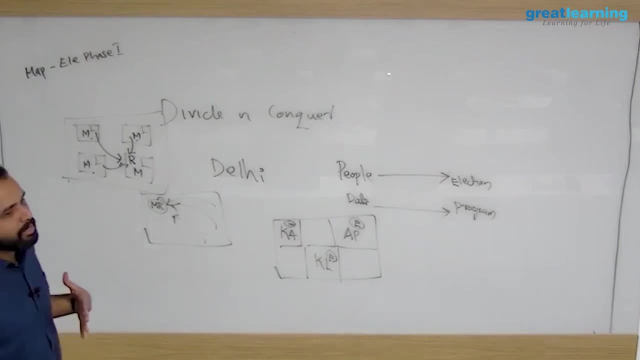 that and the developer can say that. so usually so different trainers teach this in a different way. in my practical experience, we usually say 10 percentage of mappers. that is a normal rule, like 100 mapper. if you have a call for 10 reducers, usually there is a trick. we have a. 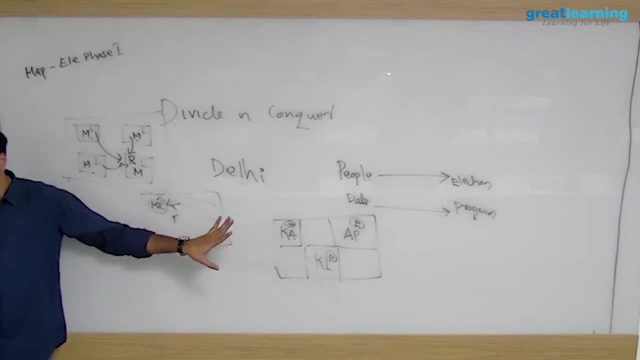 not discussed this part. we know storage. storage is handled by sdfs. forget that is done. map reduce runs. this is a programming, but map reduces just a programming way. i mean you will write a program. who actually runs this? when i submit a program, somebody should take a responsibility to run it. 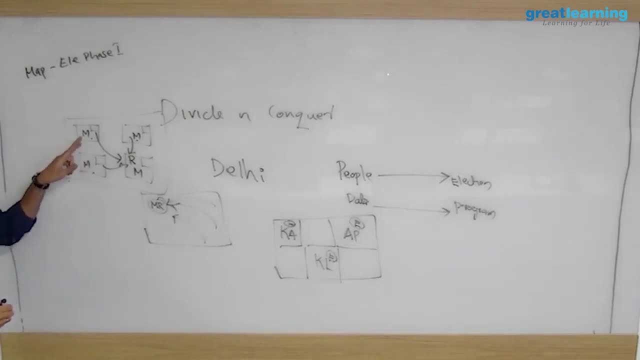 and get the output right. for example, if these four machines need to run a mapper, they need ram processing power. everything is, resources are required, right. so who will run the mapper? if these four machines need to run a mapper, they need ram processing power. everything is, resources are required, right? so who? 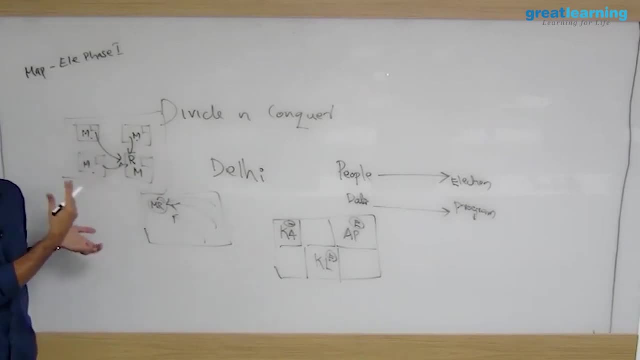 will go to these machines and say that some, some resources are required. that is your yarn. this guy will come later in the picture. yarn is your resource manager in hadoop- yet another resource negotiator. that's the expansion. yarn is the guy who will handle this execution. you write: 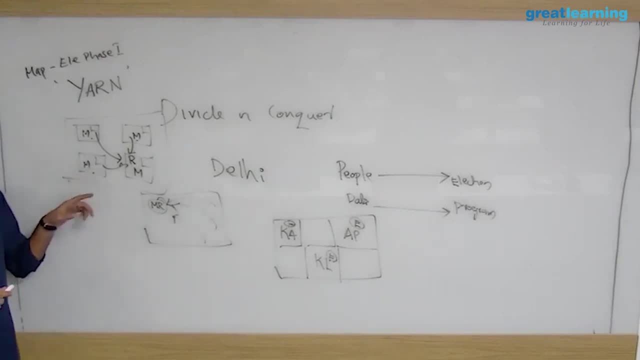 a program and give it to yarn, and yarn will ensure that it will go to these, these guys and say that, okay, give me some space to run the program. it will push the mapper program first, then reduce our next, get the output. so this is a facilitator, yarn is a facilitator, it doesn't do anything. 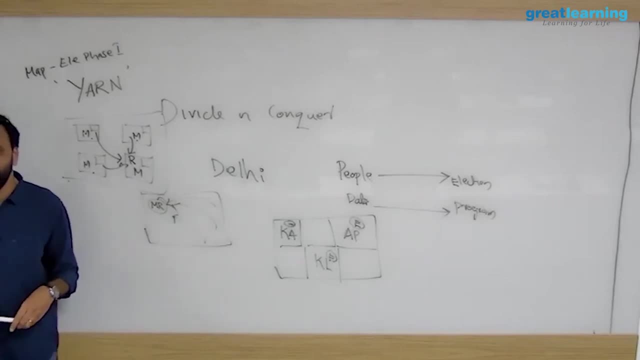 yarn will not write the code for you you have to write, but it will ensure it runs with proper resources in a cluster. we will discuss yarn in a bit more detail later. for the time being, the execution is handled by yarn. just that understanding is enough. right, you will? 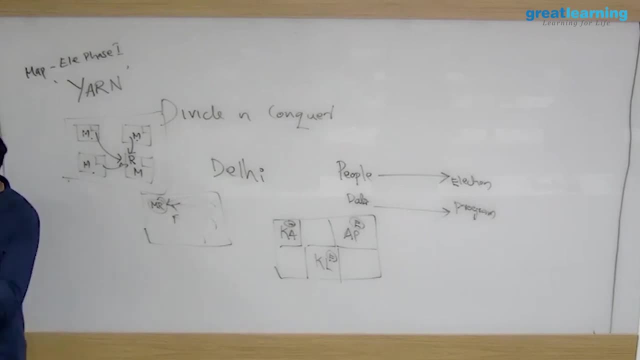 package it as a jar file. you will have a class files. then it will become a jar. you package and give, so inside that you have mapper and reducer. you have to mention which is mapper, which is reducer. and there is a driver part in the program where it will first send the mapper to the 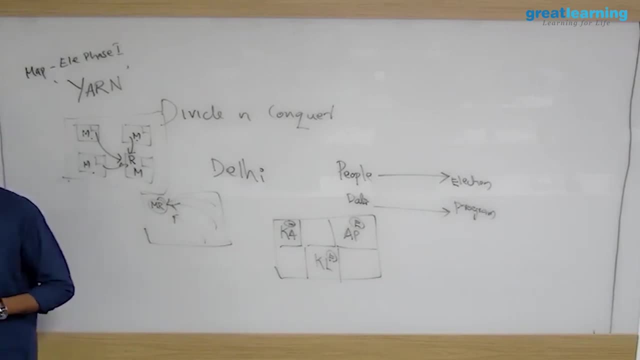 yarn. it will run everywhere. then the reducer. there is an order in which it runs. concept might be same, but the distribution here actually matters because i can run map reduce on thousands of machines same time, right, so that is the actual use case. if i'm having small amount of data, i don't need 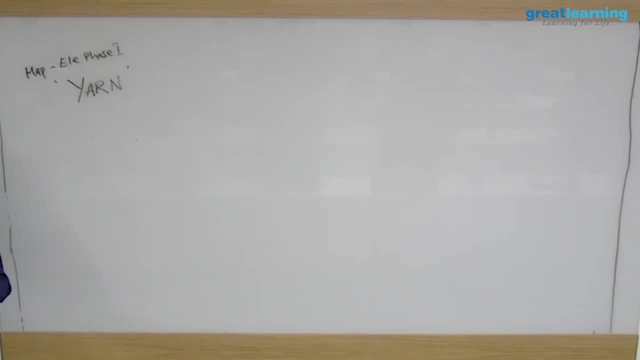 map reduce. i can use any traditional way to process it, because you don't need multiple machine to process same machine. i can do everything right. map reduce becomes obvious when you're having multi bytes of data in multiple machines. you know so. and also, another important point, a lot of people 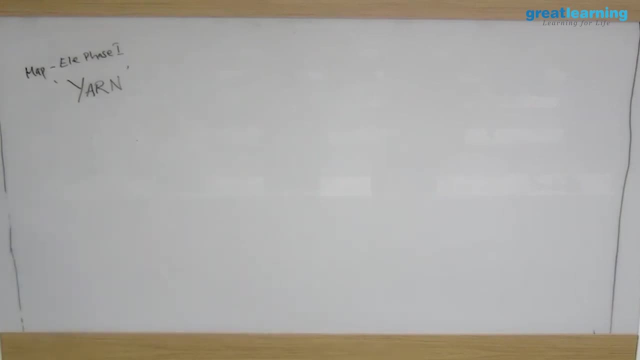 ask: when you write map reduced programs, not all the files can be processed. point number one. point number two: the dependencies will be very, very less meaning if i'm storing a file- so let's say you're storing the transaction data from a bank, right? if i divide it into 10 or 20 or something? 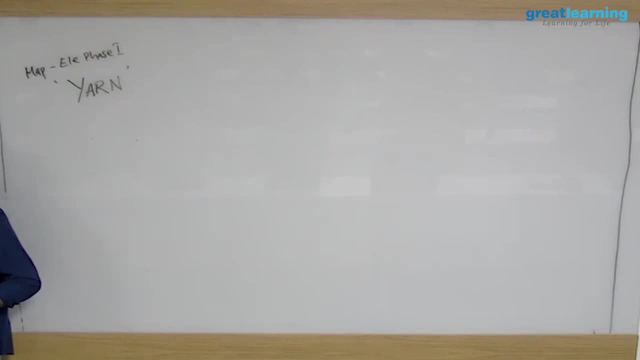 it doesn't really matter, right, because there is no dependency between the first line and 10, and so when you write the transaction data, then there is no need for jard or little oneлоardha line. all are transaction lines only, right. so typically when you store the data in hadoop- 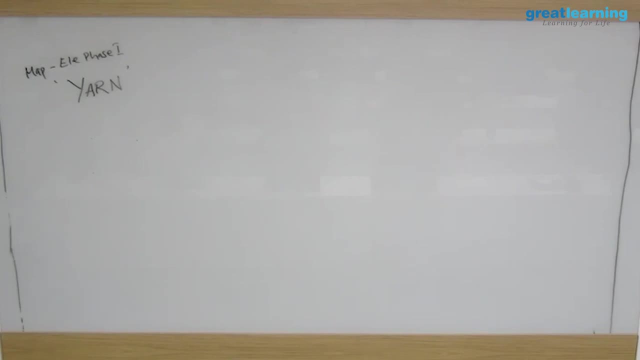 also, there is very less dependency for the data. that is why you are able to process, if you are having dependency. if elections in one state has to depend on another day, another state, i can't run election same same time, right? so the processing has to be independent, actually local processing. 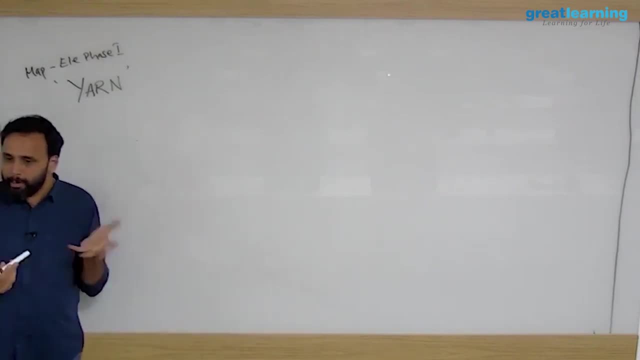 so one of the data node is running a mapper, it will just complete its job. it doesn't know what is the other guy doing. okay, or you have to handle it in the reducer. if there is a dependency, you will collect all the outputs in the reducer. you should write a logic to handle the dependency if. 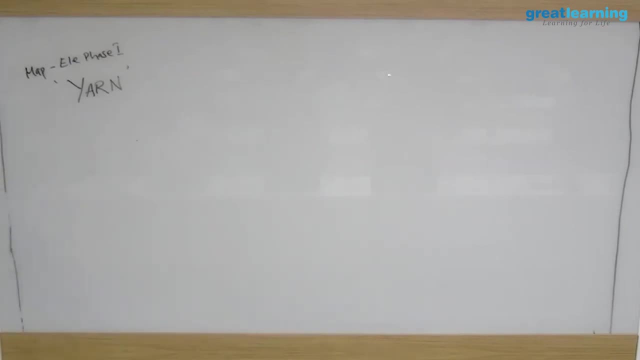 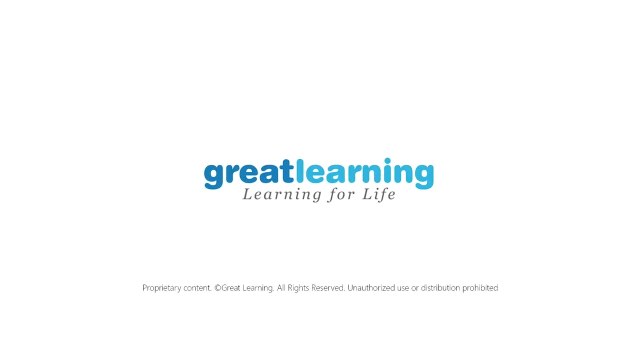 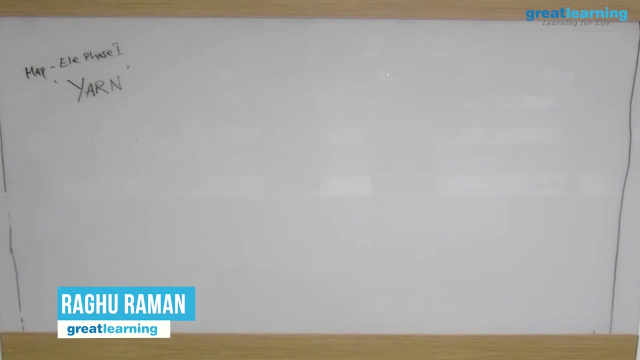 you want mapper, it will simply independently run. they are not dependent on any other process running, so we will look at it technically. i mean, i'm just talking in terms of a theory only right now. now, in order to understand map reduce in a better way, i should take an example, right? 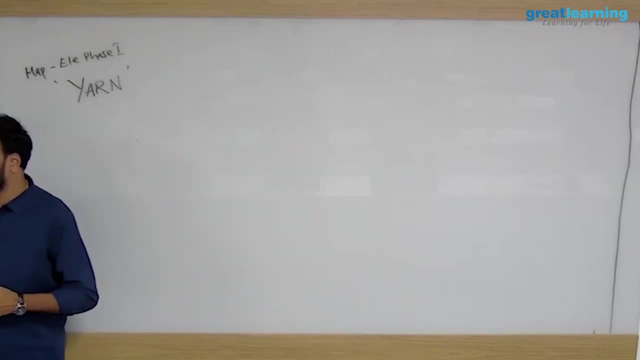 now this example will help you to understand map reduce and it is like a hello world. so in java, if somebody want to learn java, what you do? you write a hello world and you say system dot out and you will print it and say that this is how a java program is working. so that's like very basic. 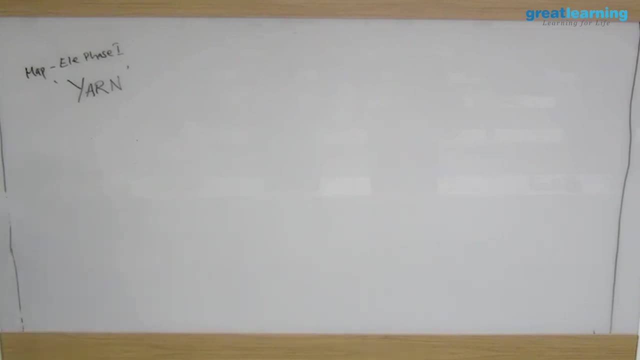 of java, if somebody want to learn. same way, if anybody want to learn map, reduce at least the basics. we propose a program called word count this. you can google for this, this word count program. this program is very, very popular in the sense like: this is the de facto. 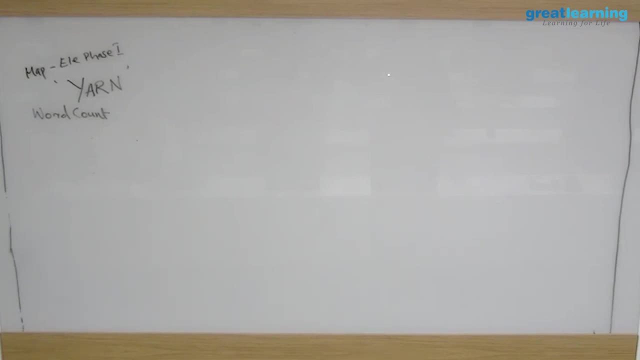 hello world in map reduce. anybody want to learn map reduce. the first program they write is word count. you can write other programs also, but typically the first code you will be writing will be the word count program. to understand how map produce is working right, let's take a. 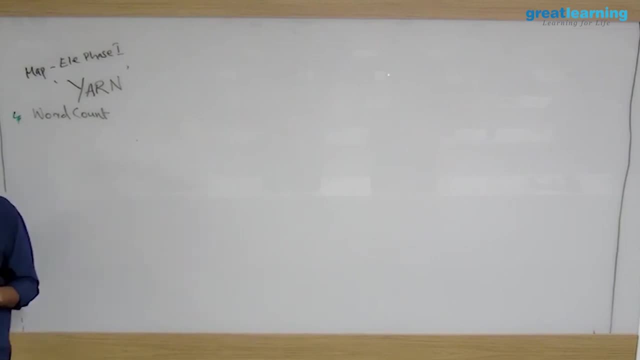 use case. to understand the word count right, i'll tell you what is this word count program, right? let's imagine you have a text file and you have stored the text file in three data nodes. the text file is so big. so i have a text file and i'm storing it in. let's say, 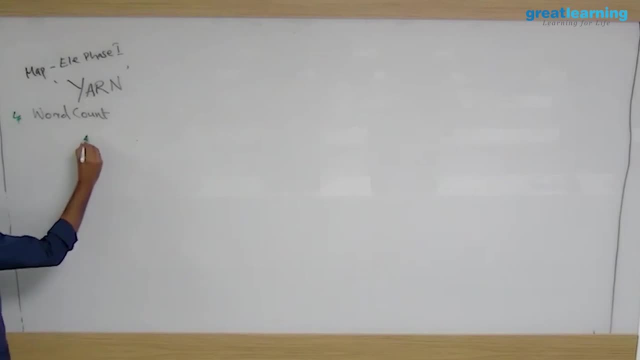 three data nodes, so i'll just write them here. so this is one data node and you have another data node and then you have another. so this is my data node. one, two, three. and what is my text file? it has some words, imagine, so i will just write here, can you see? 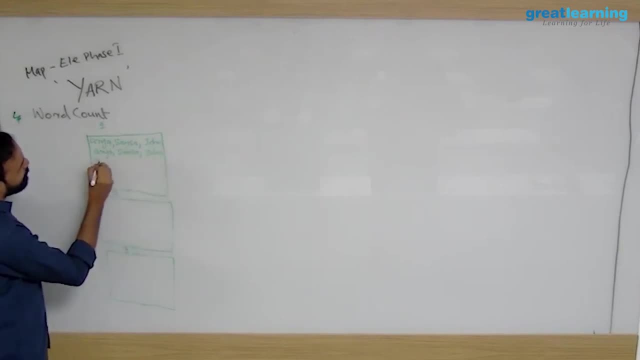 i have to write. there is no other way to explain this, so i hope you will allow me to write right. arya sansa, john, that's fine. a man has to explain arya sansa, so others are thinking: what is he talking about? these are game of thrones characters, by the way. if you don't understand, 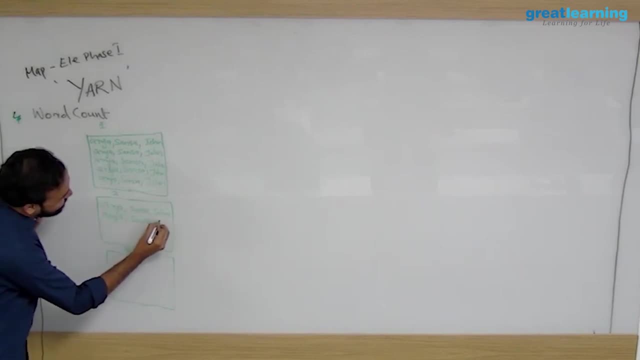 it's okay, you don't have to be an expert to learn hadoop. i just thought i'll pick something which people understand. i was wondering whether somebody can write it for me. so many things i have to write, okay, so it has some repeating words, nothing else. aria sansa john. that's my first line, one line. 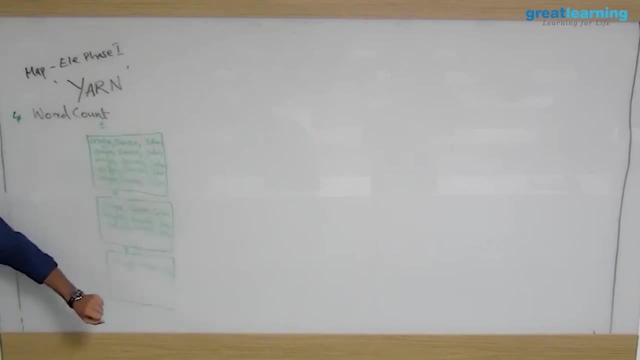 and this data node has five lines. this has three lines, this has two lines. imagine let's take one more, etc. right, so you, when you store your data as many lines as possible, you can write it in a variety of ways. did it begin like this? imagine the real use case is like you have millions of lines. this is to make. 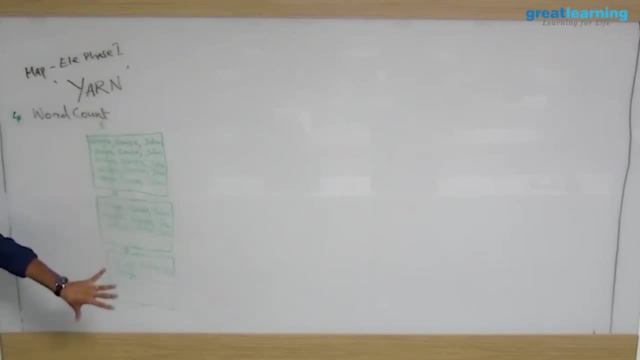 you understand. okay, so there are three blocks of data right now. now you have to write a word count program, so what is the purpose? i want to find out how many times each word is repeating, so by looking at it you can easily say, i think, what is that? 5 plus 3 plus 2.. so each word is repeating 10 times. 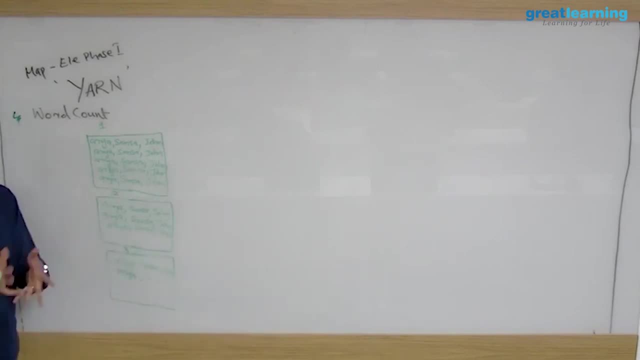 so your final output will be aria 10 and sansa 10, john 10. that's the final output. you can do that because only less number of lines are there. there are millions of lines. you cannot do it. so you want to develop a map, reduce program which will count, you know, the number of occurrence or the frequency. 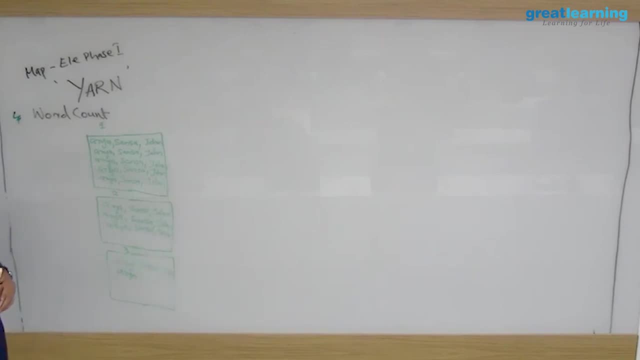 of each word. now how do i do it right, theoretically speaking? now, to do that, the first thing you have to understand is that first you have to develop your mapper program right. map reduces, map and reducer. in the mapper program, the golden rule is that the output of a mapper program 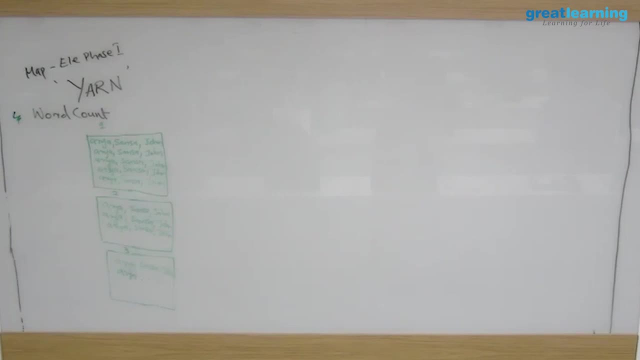 is always a key and value pair. you know what is a key value pair, key and value. the golden rule as per map reduce documentation- is that if you write a mapper program, the output has to be in the form of key and value, whatever you do. so, if i am a java developer, right, so we. 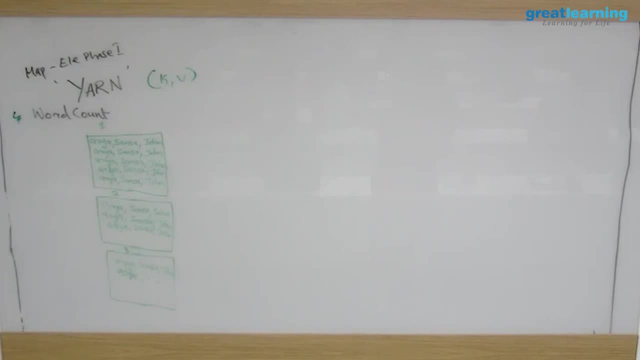 are going to write map reduce programs in java. okay, so let's write mapper as maintain cál Local and chili asORE clapping. so what i can do is that i can develop a logic using java in which what i will do in java there is a class called string tokenizer. everybody will be knowing those who understand java. 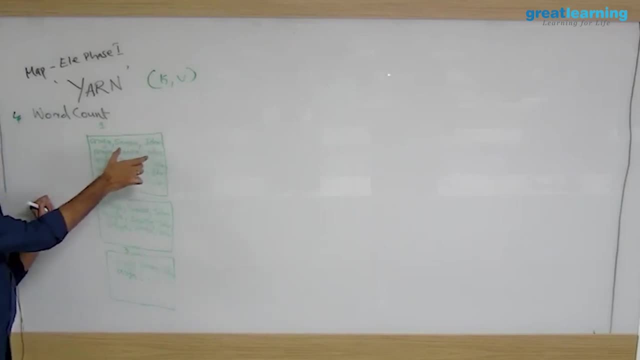 right, i can call the string tokenizer class. what that will do is that if i give a line, okay, by looking at the delimiter i can mention it will extract individual words. program that in java there is a class called stream tokenizer, right, so i'm formulating the 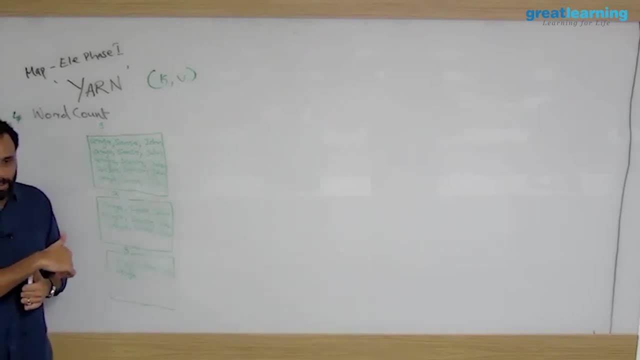 you know logic for my mapper. now, internally in map produce there is something called record reader which will give me line by line data. so you don't have to bother about that. line by line data will be supplied to your mapper, right? so you will be thinking in the mapper: how does it get each line? 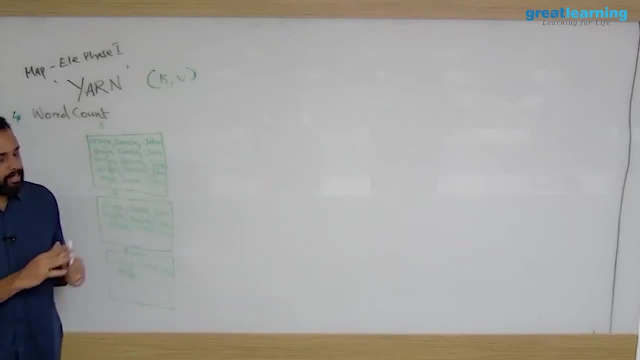 of data. so there is a record reader. i will talk about it. that will push every line to the mapper. so if you write a mapper program, mapper will run here, another one will run here, another one will run here same time. they will run right. this guy will get this block of data. this guy will get. 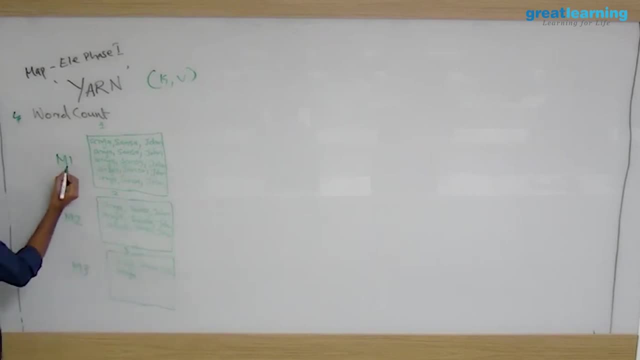 this block. this guy will get this block right. and what this mapper will do? it will read a line using the string tokenizer. it will extract individual words. the word will become the key. every word i'm extracting will become key. the value will be one. i will hard code the value one. i'm just saying. it is like counting. 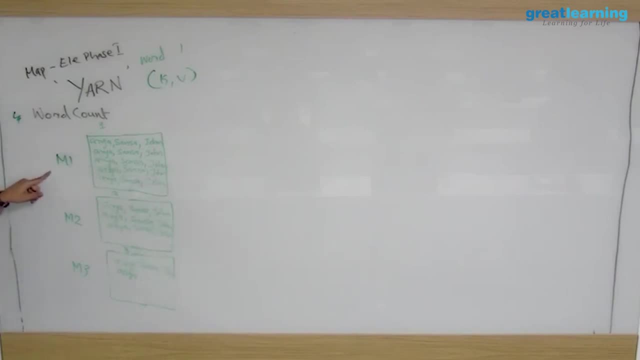 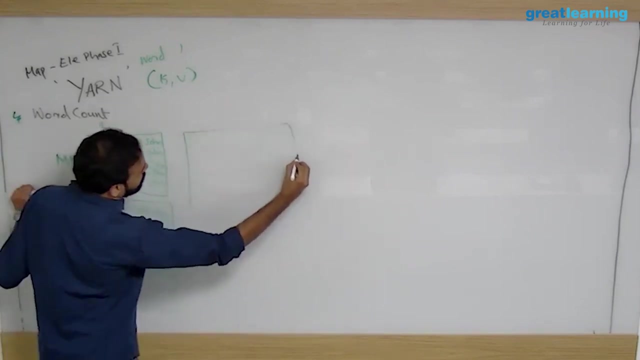 the occurrence of each word, so that if my mapper runs on all these nodes, okay, can you tell me what will be the output here? it will become aria, comma one, right, again. what will happen? and john, comma one- again, same thing, right. how many times it will be there? five times, right? so i'll say aria, comma one. 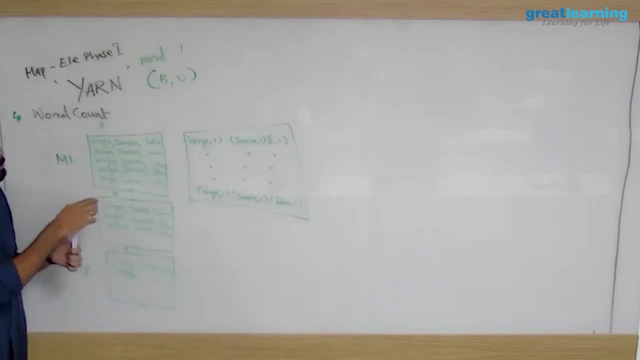 sansa, comma one, because every line you are processing individually. i'll take one line and what my string tokenizer will do, it will give me the words from that line. so i'll get aria sansa one. i'm saying that, keep the word as the key. i can write it in the java. i'll. 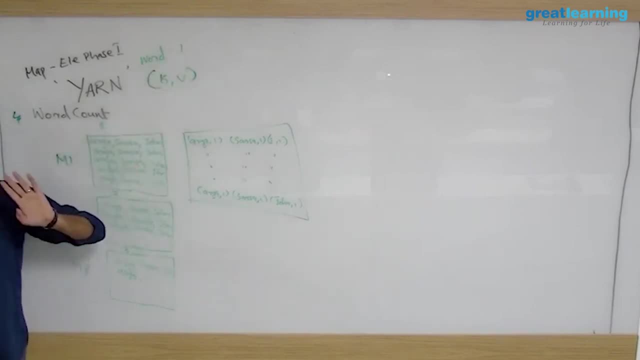 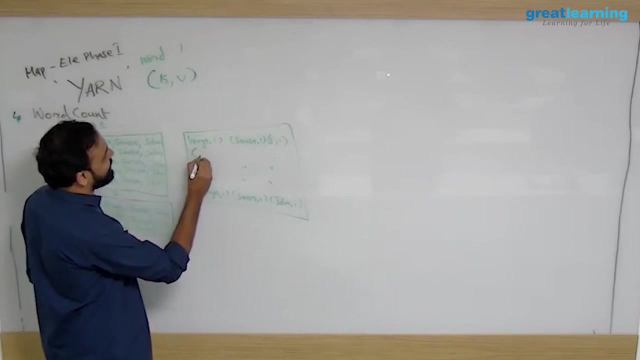 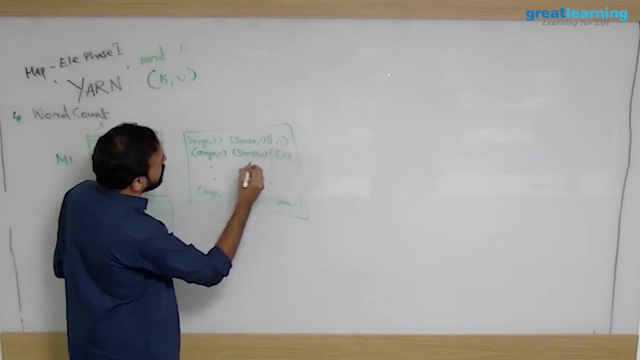 show you the program and hard code the value as one. any word that comes i'll keep it as one. so even the second line, third line probably- will write it. i mean just to avoid the confusion. every line will be converted into key value pairs. now you may be asking why am i doing this? because map reduce says: 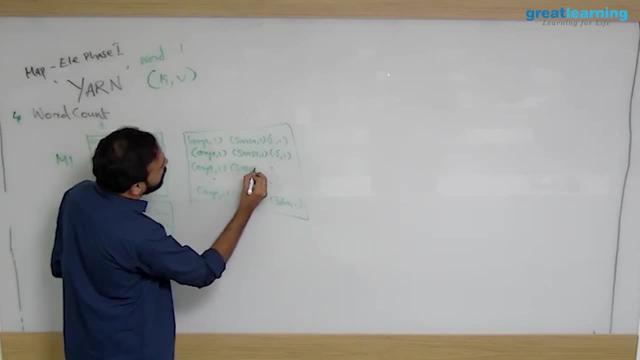 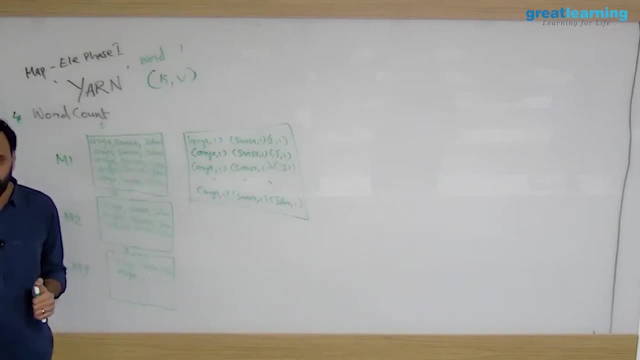 that the output of a mapper has to be a key value pair. i don't have any other option. aria sensor, john aria. again, that area will be counted as one. yeah, so the mapper logic: whatever you write it to a key value, it will be applied to record by record. so in this file this line is a record one. 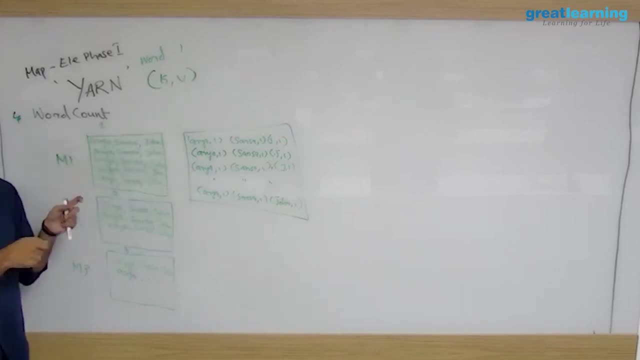 line will be taken as a string tokenizer. it will extract individual words and i will say: take every word as a key and one as the value. now let me explain the whole step. then you will understand why we are doing this. you will be wondering why you are adding a one right. there is a reason for. 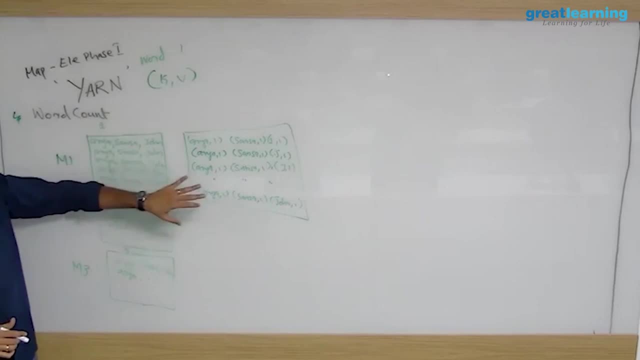 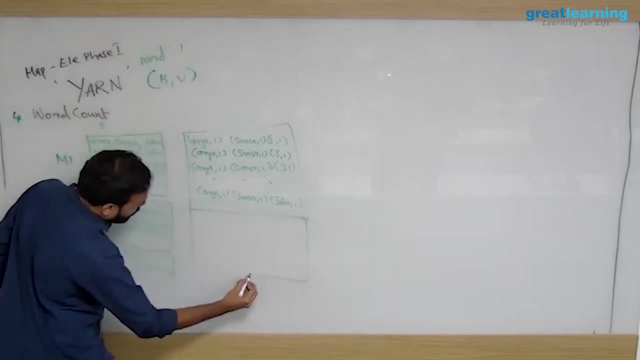 that. so in my first data node, once the mapper runs, this will be how the output is going to look like right now. what will happen here? say, mapper runs, is running right. so what will happen here? you will get again arya 1, sansa 1 and john 1. again arya 1, sansa 1 and john 1. i just say a1. you will understand, i think. 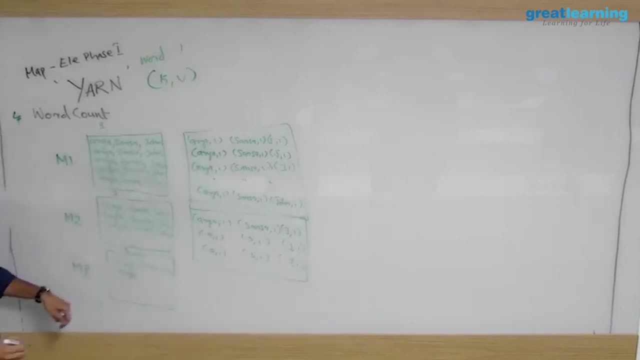 sensor 1 and john 1.. now the same is running here, also same mapper, so this will also produce same output. so two lines: arya 1, sensor 1, john 1- again this. now, one more very important point is that once the mapper runs- now this is like 10 lines of data. if you have huge amount of data, it will. 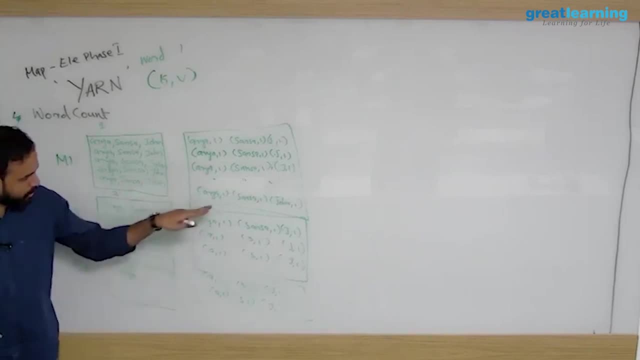 persist the output to hard disk, map reduce will. this output will be pushed to the hard disk. that is the reason my produce is slow. so a lot of people ask this question: why map reduces slow? my produce is extremely slow if you run because there is disk read and write. so ideally the final output only should be stored. 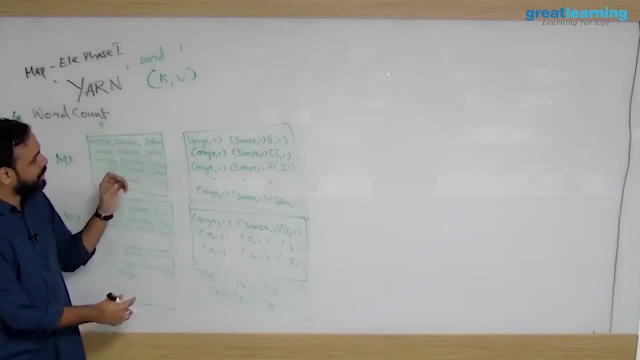 but since you are processing a lot of data, what will happen is that once the mapper runs, each node, this output, you know it will push it to your hard disk local file system so that you don't lose it. actually, and this is fault tolerant, let's say this machine crashes. let's say this machine crashes. 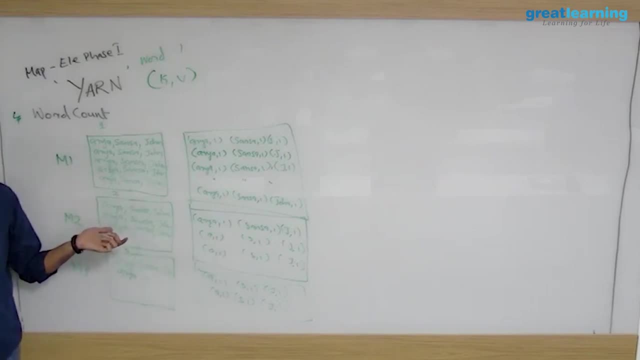 couple of things can happen. in one scenario, it will wait for this to come up, or the replica block can be processed for another advantage of replication fault tolerance, right? so if this mapper is crashed, what will happen? your map reduce framework will wait for all the mappers to complete. 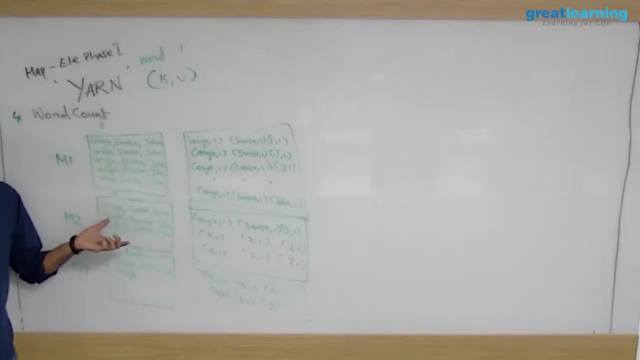 so this guy crashed means this is not over. right, automatically your yarn will figure out where is the replica block. it will start a mapper there and that guy will process and get the same output. it is a replica block only, so you are getting the same output anyway. the technical: 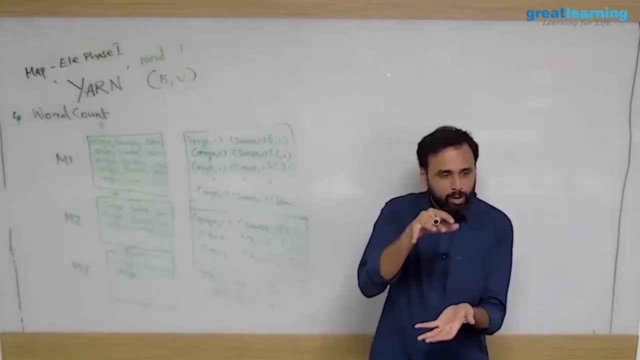 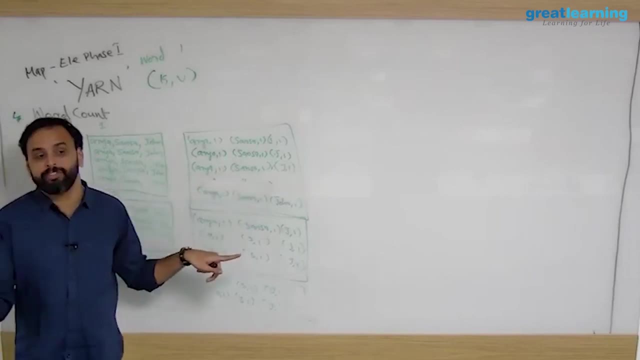 documentation is that if it is more than 100 mb it will be persisted. 100 mb it will hold in the ram, 100 mb to push to hard disk. that is a technical documentation because typically we process billions of key value pairs, billions, not even millions, billion bb. so if this output is more, 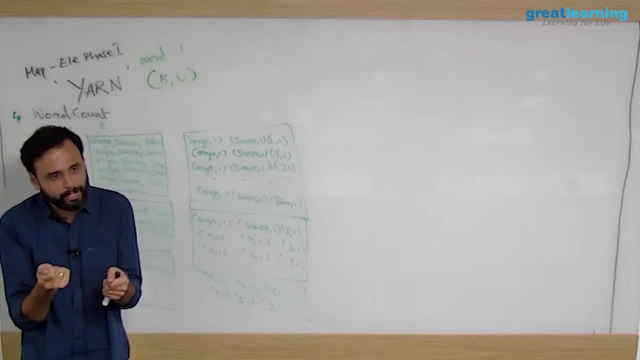 than 100 mb it won't hold in the ram because reliability should push it into the hard disk. if it is less than 100, it will hold, but even if it crashes it will again. it has to run, so at no way. the map reduce can fail. that is a beauty. if these two machine crashes, will fire on another only. 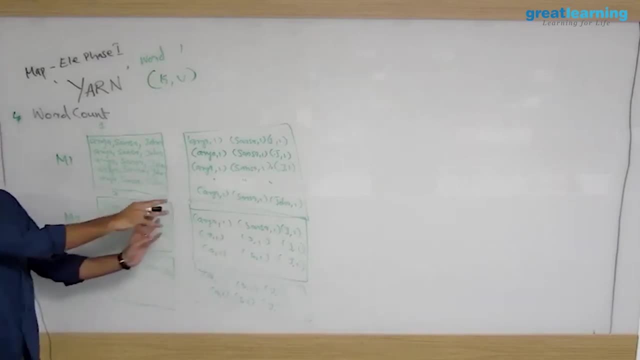 thing. you have to wait for longer, you have to wait for some more time, but end of the day, you will get the final output in most of the cases. so now your data looks like this right now is the interesting fact. what is interesting is that i am not writing everything, but one machine will. 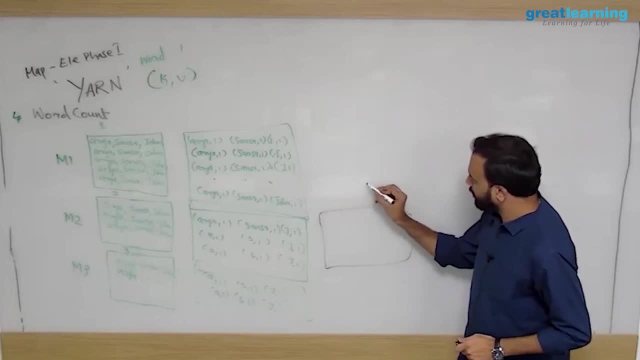 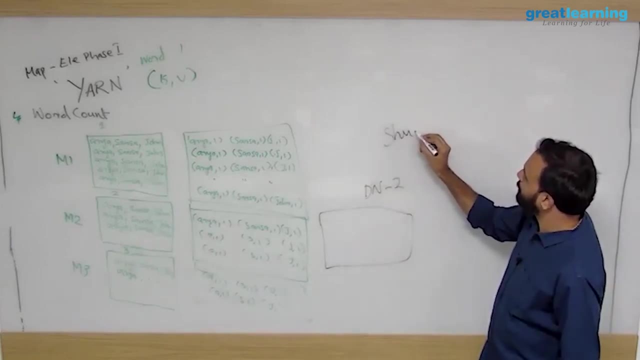 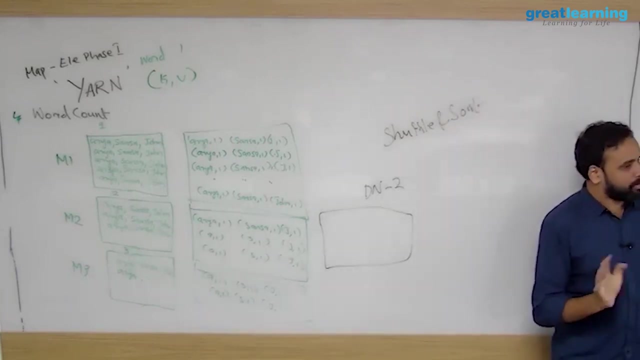 be picked. so i am assuming it is your data, not too? just as an example, one machine will be picked and something called shuffle and sort will happen. there is a phase called shuffle and sort and this will happen automatically. you don't have to write a code. so what is happening in? 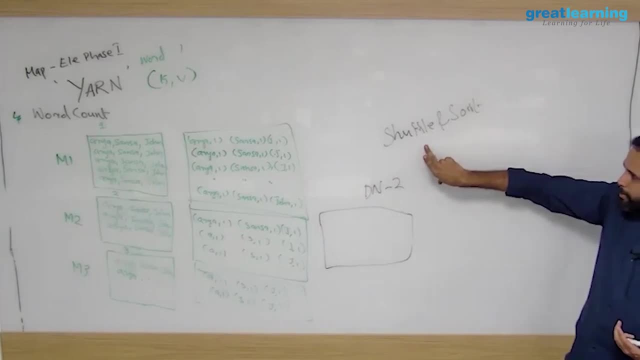 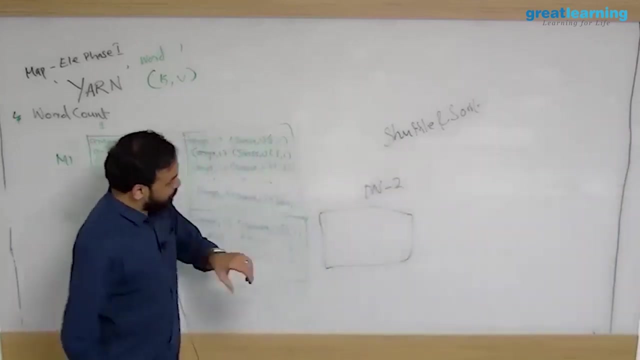 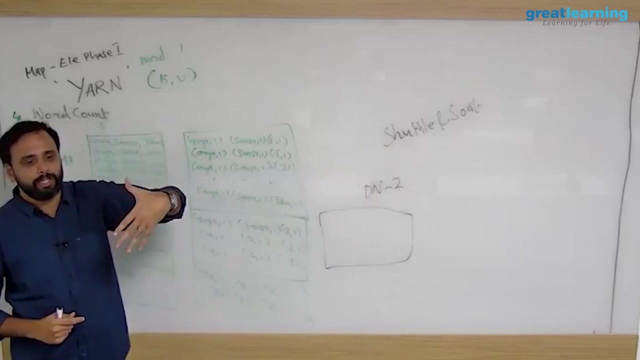 shuffle and sort right. shuffle will sort will happen only when all the mappers are completed, all of them are pushed right. so once this is over, map reduce, shuffle and sort will kick in. what this shuffle and sort will do? it will sort your keys based on ascending order. for example, here it is. 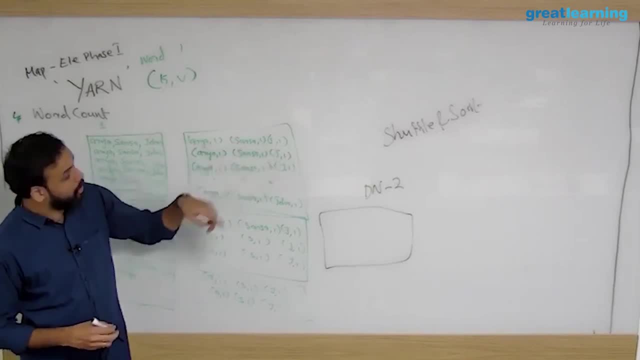 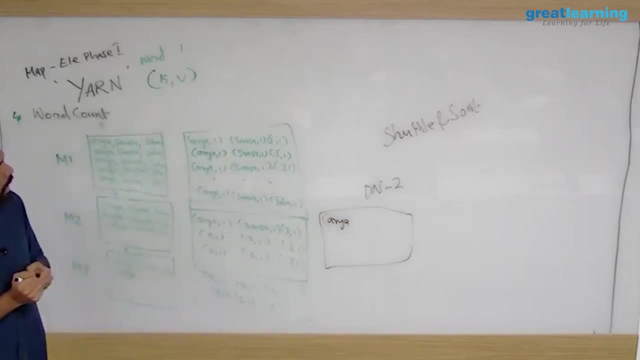 going to be one key, then next will be john, next will be sansa- right, alphabetically. more than that, what it actually does is it will pick the first key, aria. aria has five values here, right. it has three values here. it has two values here. it will assemble them like this: 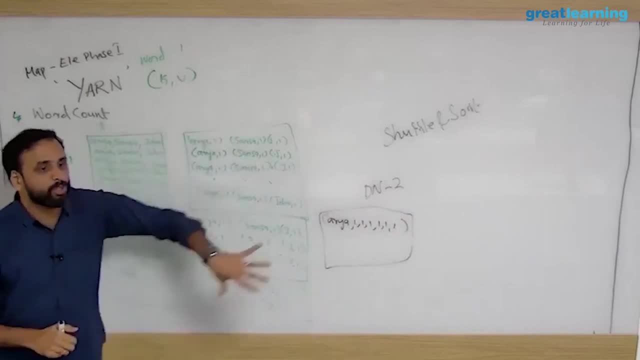 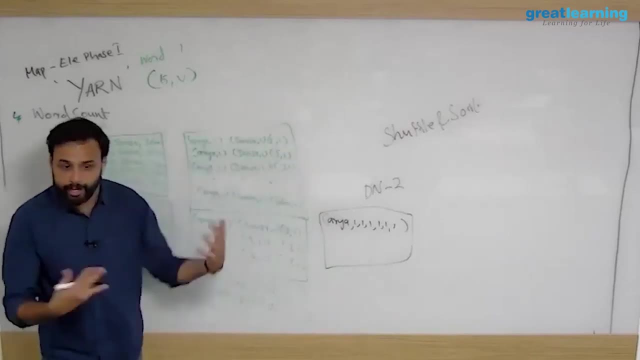 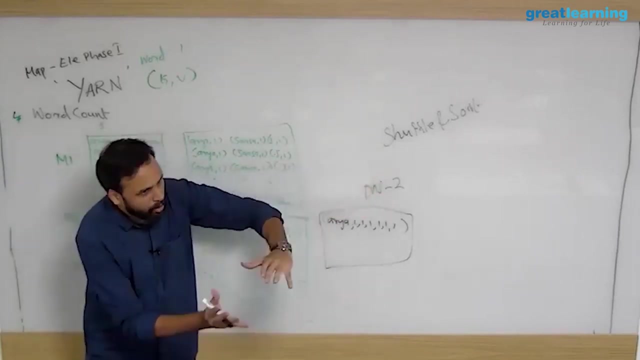 so it will pick up a key and assemble all the values of that key together. it will read from all these three, because till this point it is local processing, they don't talk to each other, but you have to aggregate them anyway, right? so in the shuffle and sort phase, what is happening? all the values of a given key are brought together. 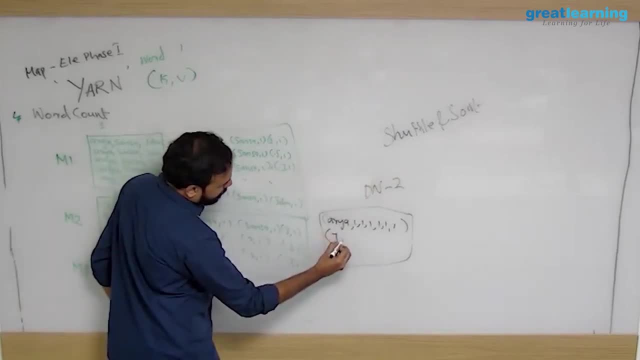 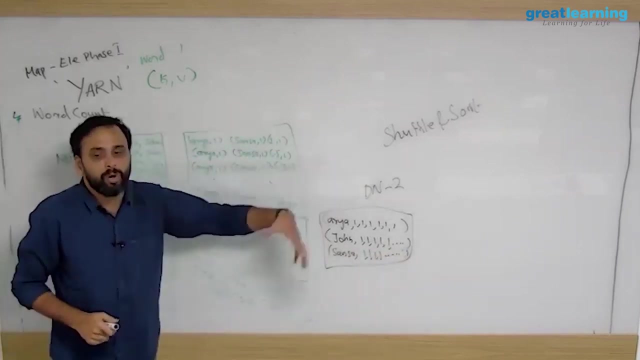 so same will. so next will come john, because it is alphabetical for john also. i think 10 ones are there, right, i'm not writing all the ones right- and then comes sansa, right, and that also has these many things. so this shuffle and sort phase is actually very costly in map reduce, because if your map 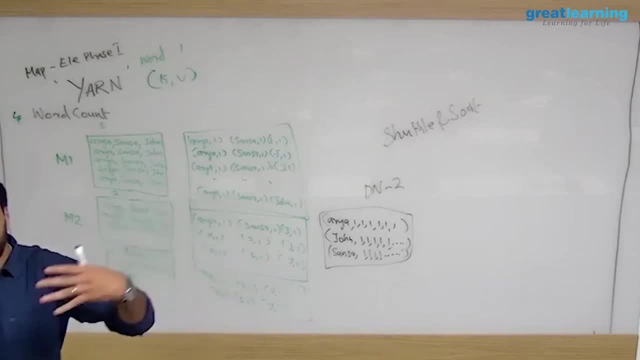 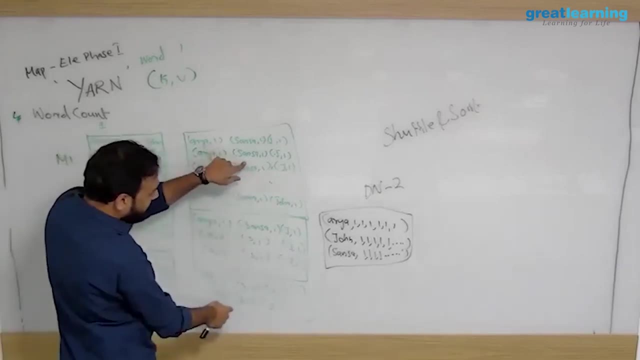 reduces running on hundreds of machines, it has to collect this from all hundreds of machines right over the network. these values need to be transferred, right? i have to get from here here. here, these are network machines, right? so all this data has to be collected from here into a single. 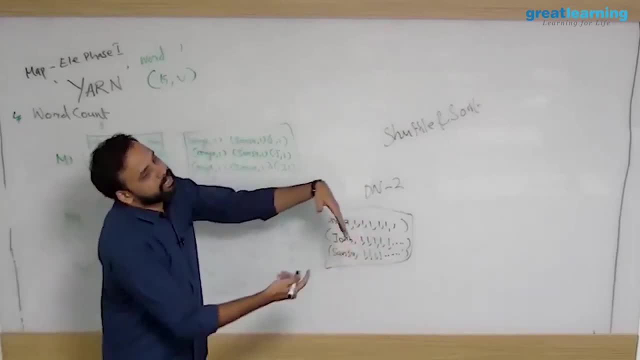 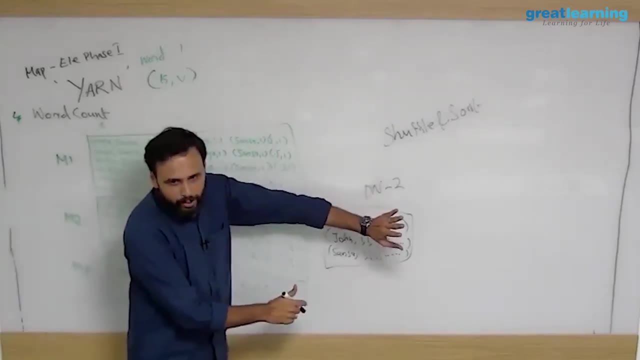 machine. most of the cases it can be in a single machine, but you can say shuffle can run on more than one machine. also depends on the size of the machine, but it can be in a single machine. also it depends on the size of the data, whatever you have. so in the shuffle phase, what is going to happen? 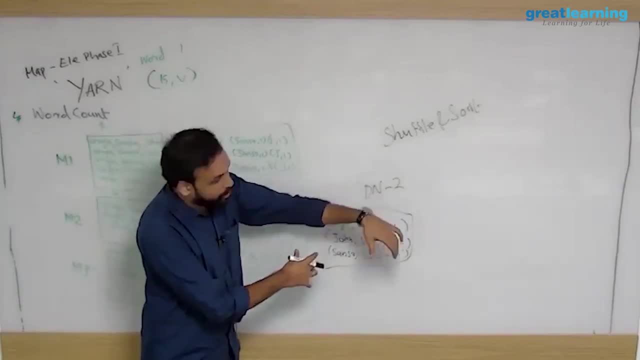 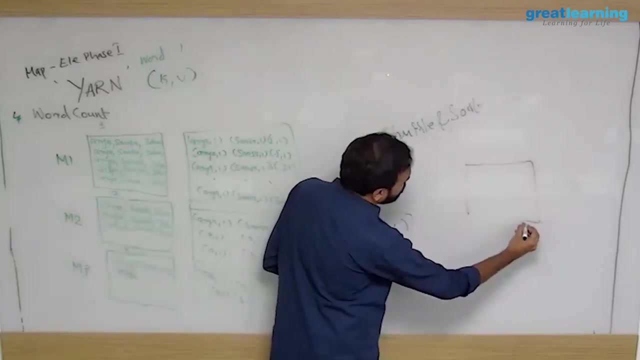 all your values will be assembled automatically. now you don't have any control on the shuffle phase. it happens automatically. so this thing will happen automatically. then your reducer will kick in. now i am assuming we have only one reducer, so your reducer process is running on, let's say, data and or two, again same machine. so once the 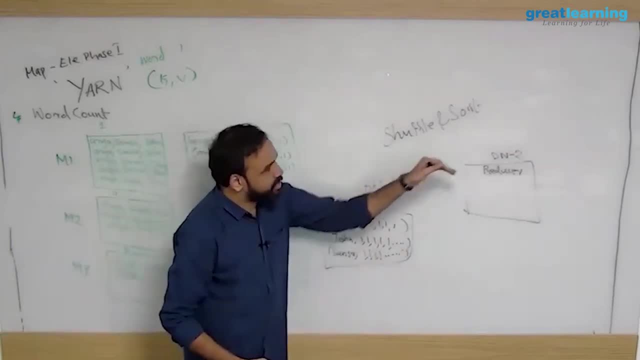 shuffle is over, you can let the data flow into the main machine and in that machine you'll run your values. data looks like this. then the reducer process will kick in. okay, now reducer is a program you have to write. you have to write a reducer program in MapReduce. 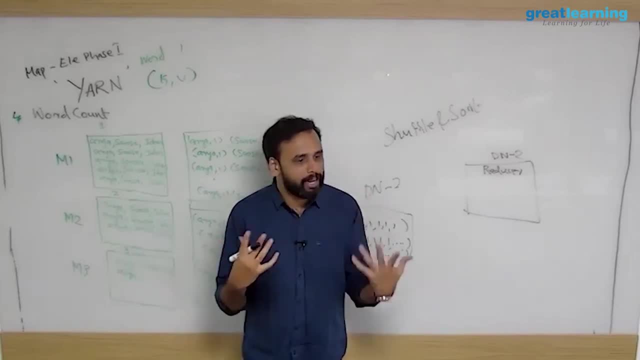 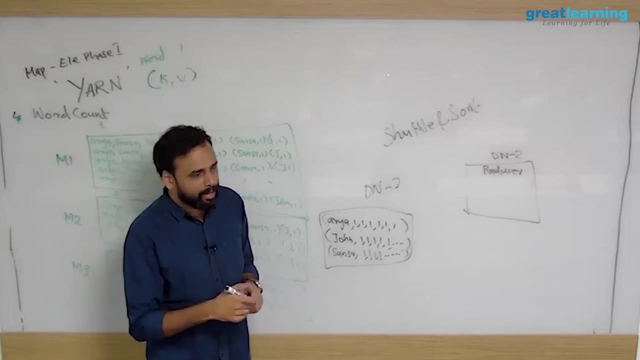 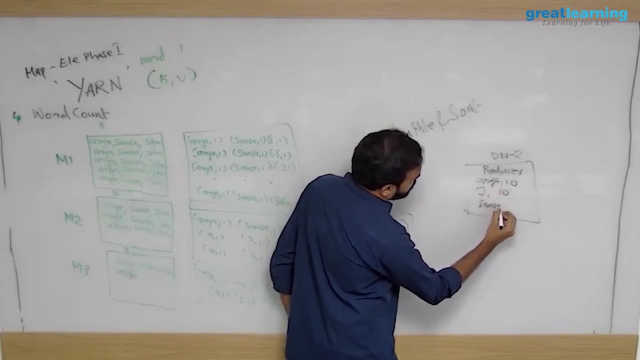 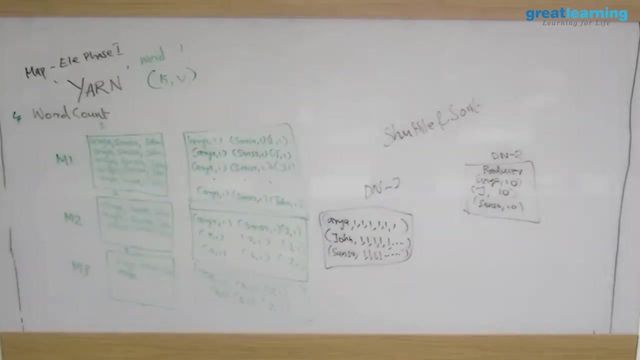 right. so if, if I was a Java developer, what will I say? I will say that read the key and then what sum? all the values. I will write a simple Java logic so that what will happen? John 10, sensor 10. so the basic idea is that whatever you define in the mapper logic will pass on. 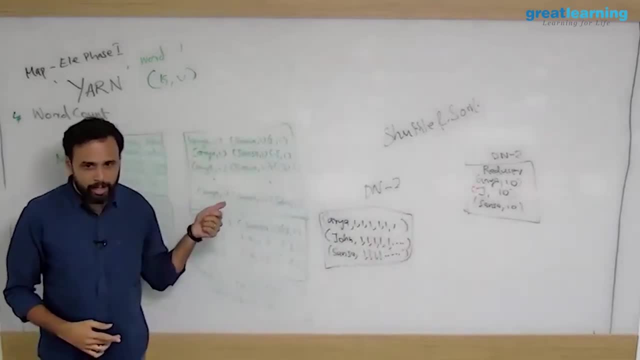 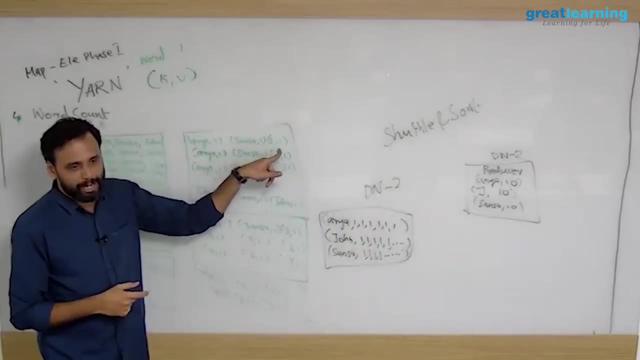 to the reducer. if your logic defined in the mapper is wrong, shuffle will be wrong, reduce also will be wrong. right, because if here I am so this is the reason I said that comma 1, so that I can add all of them. you can use any other. 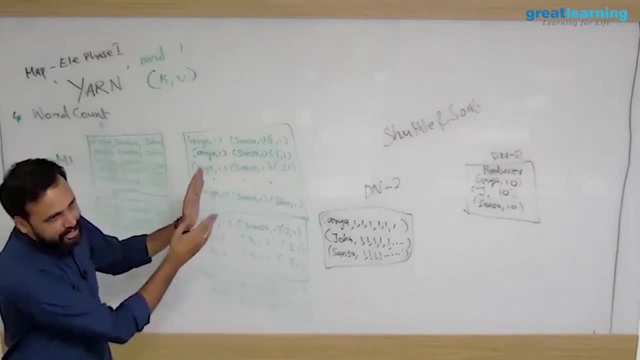 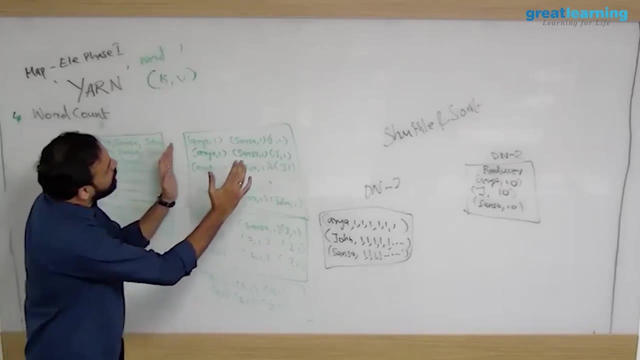 logic. if you have a better logic you can use. I mean, I'm just saying, I'll just say comma 1 so we can add them. any other logic is there? that is also fine. it is up to you, to us to decide the logic. but if your mapper definition is wrong, the way you, 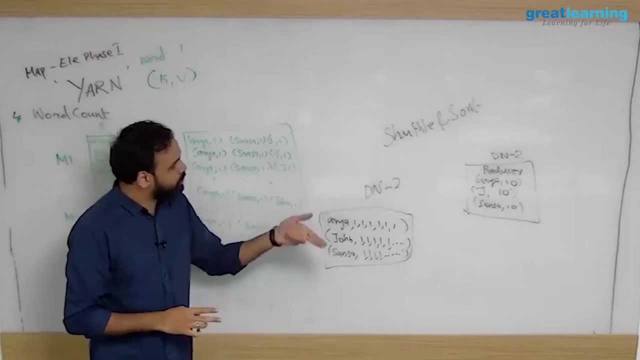 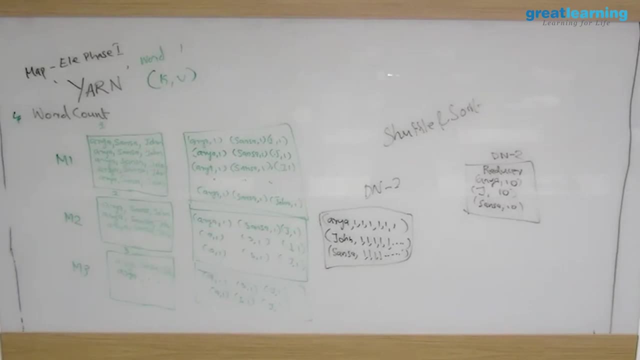 write a mapper is wrong and what is going to happen? your reducer shuffle faces. everything will get you know: changed right. shuffle and sort will happen automatically but it needs input from mapper so mapper has to complete. then that is taken by shuffle and sort and will manipulate and produce this. 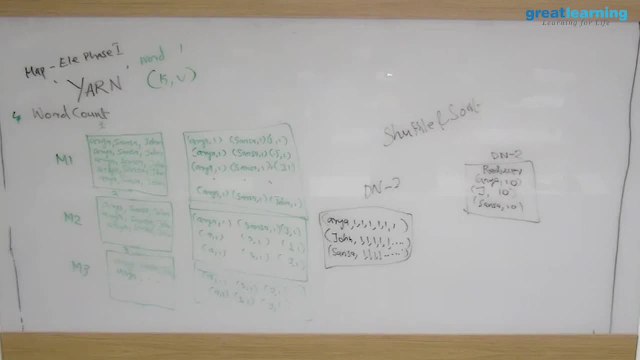 result, that is the input to the reducer. so when you write a mapper you have to write a reducer, and when you write a reducer you should know what is the output of shuffle. otherwise how do you write right? so you have to formulate your logic in such a way that you understand what is. 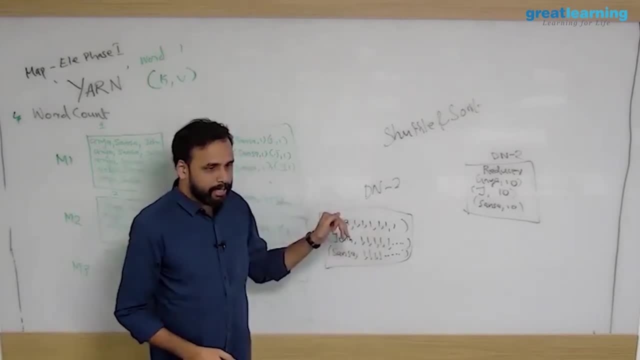 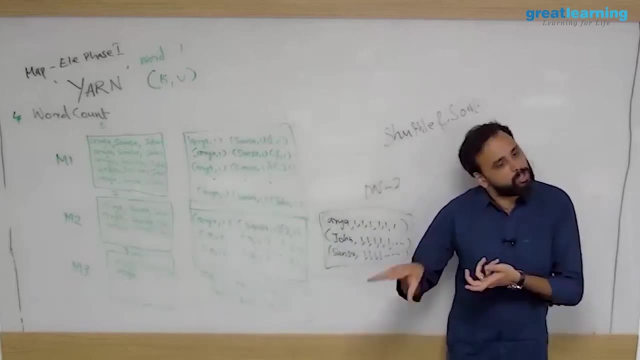 the output of shuffle and that logic only says: get the key and all the values. now, if you are having more values, like billions of values, it will use the RAM and HARD disk to store them in intermittently- like I have billions of values, it has to just assembled as a data structure where you have a key and 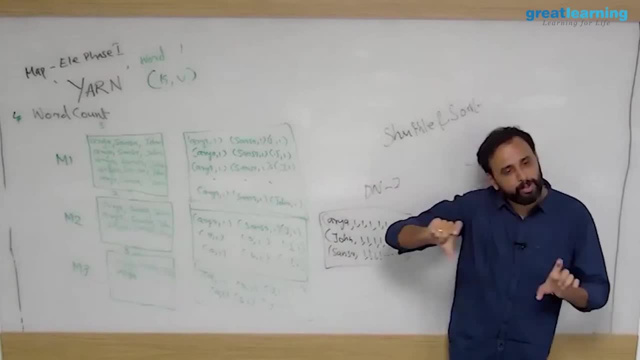 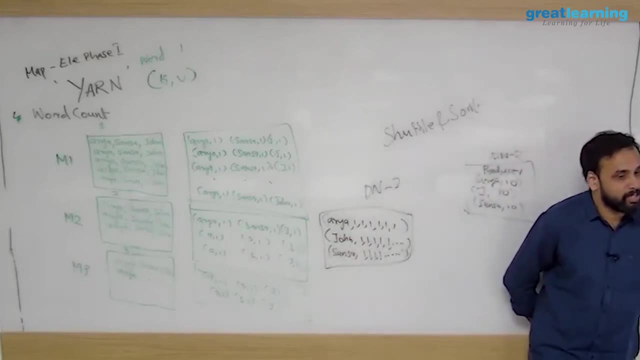 a set of values, so the more values you have, it will produce an output with a key comma, whatever values you are having. so it is just assembling all the values. it can shuffle can run in more than one machine. also, it is not always one machine you can configure for shuffle because 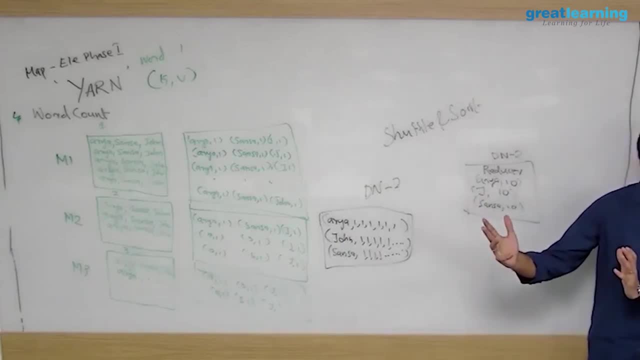 if you have billions of values, i can't arrange all of them in a single machine. that may not be possible, so i can. so that is what. so the next question is that: how do you decide whether you need one reducer or more than one reducer? in this example, one reducer is enough, because i'm just 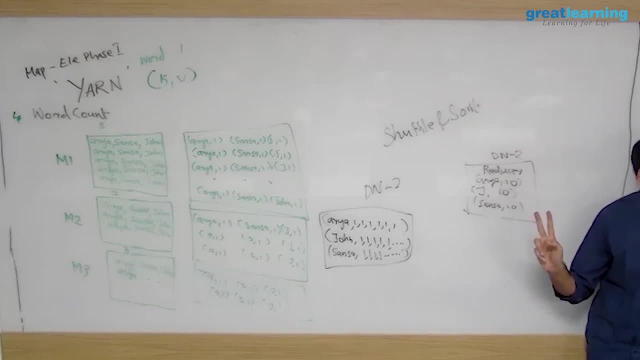 adding adria, john and sansa. for that, one reducer is enough. what if you have multiple reducers? this is a very interesting question. i will answer this and then i will come to your questions. if i call one more reducer, there is a problem. can you tell me what is the problem? 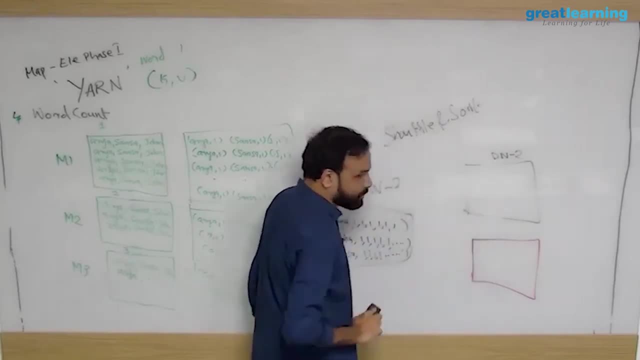 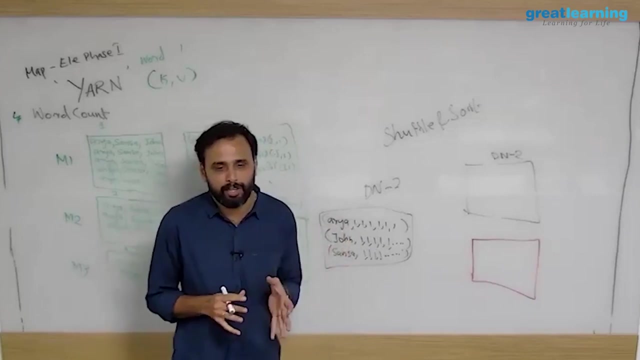 how the data will go to multiple reducers. right, this should go to here and here, how, by default, map reduce has something called hash partitioner. it is a logic what it will do. it will do. it will calculate the hash of a key, okay, and try to evenly distribute. 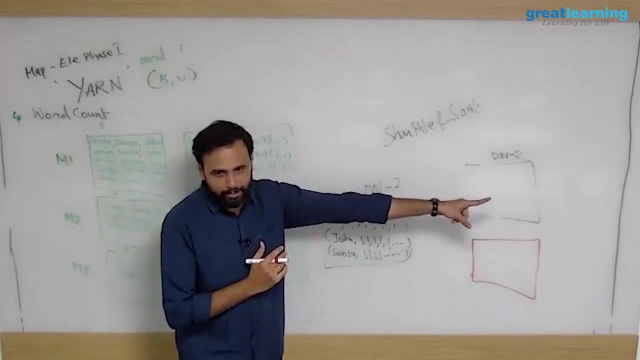 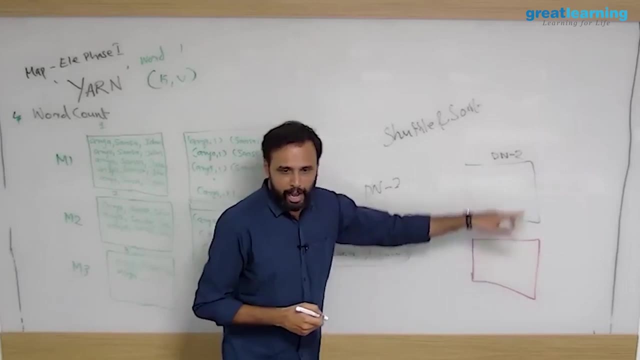 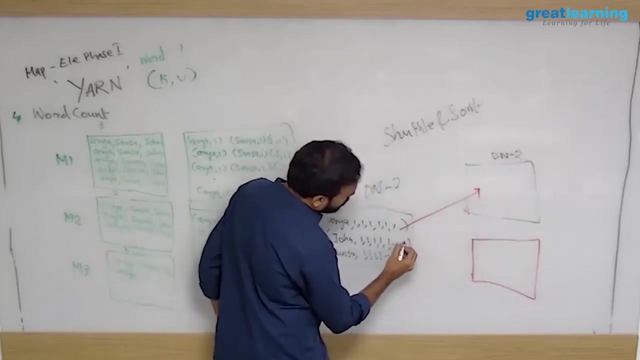 them. you cannot give half of a value to one guy. this guy has to add all the value. so i cannot say that area 5 will go here, area 5 will go here. that doesn't work. area has to be added by one guy. so if you are using the default hash partitioner, this might go here. this might go here also. this might. 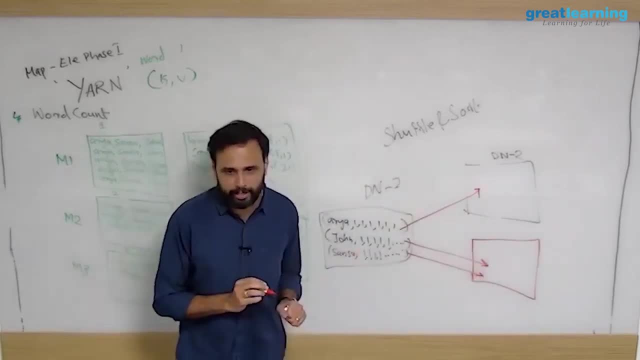 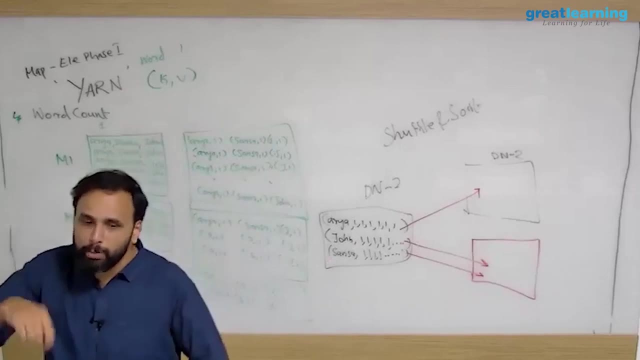 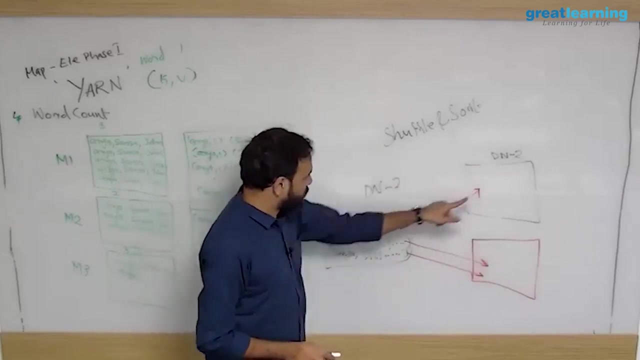 go here, that's okay, almost equal distribution. we can say: now think about billions of values, then it makes sense actually. or you can also write your own partitioner. you can say that there are two reducers. okay, this idea should go to this guy, this should go to this guy, this should go to this guy. 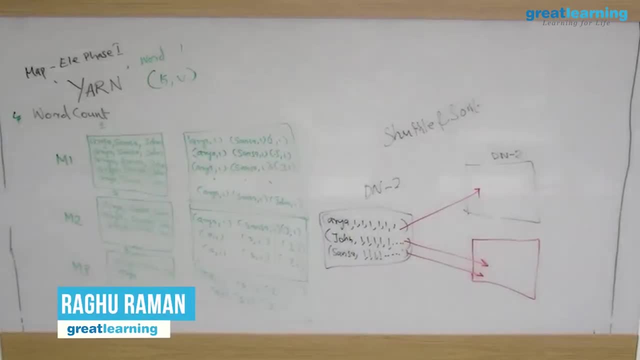 now, coming to a practical example again. uh, icica bank use case same i. we did not write map reduce for them, i did not write dance wamல, i did not try to actualize it, did not write anoulw for the example. again, icici bank use case, same i. we did not write map reduce for them, i did not try to add hang. 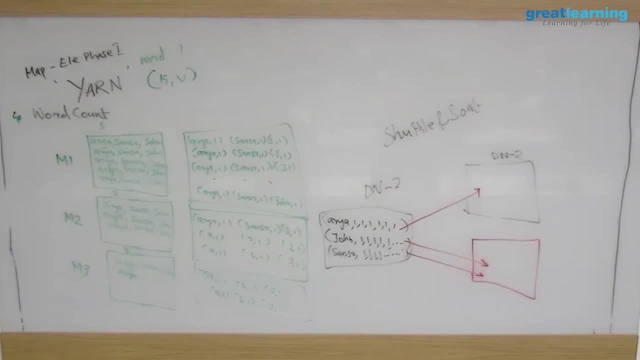 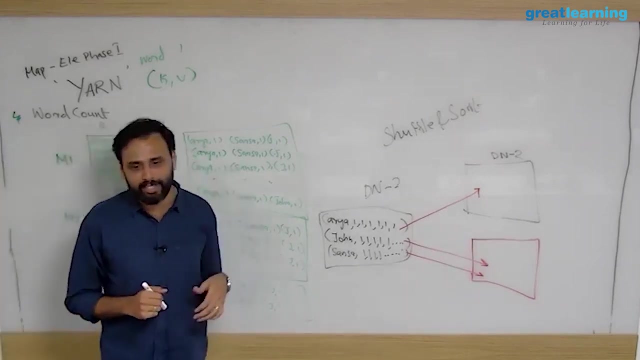 actually, but I saw there one of the batch jobs they were running, So there they were using MapReduce, So they had multiple branches right, So they were collecting the transaction data from each branch. okay, So they will probably have a Bangalore branch. 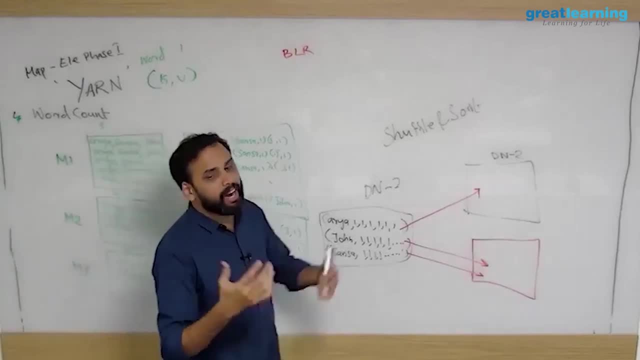 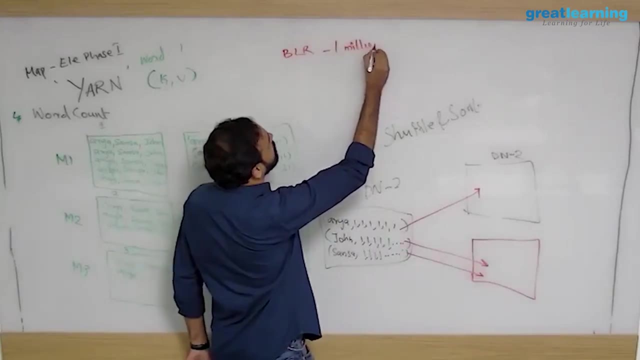 They have a Bangalore branch. In the Bangalore branch it's very high number of transaction, right? So in a month, let's say, 1 million transactions will happen. Let's take example, okay, Because Bangalore branch is very, very heavy okay. 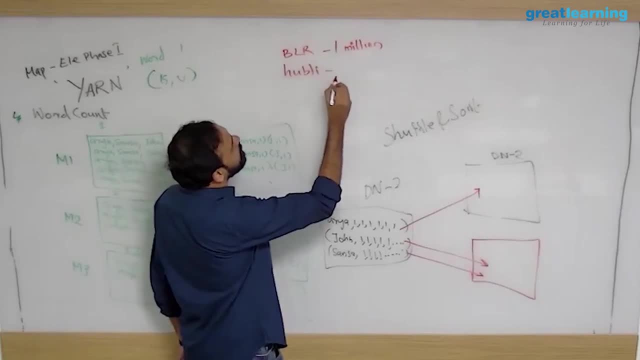 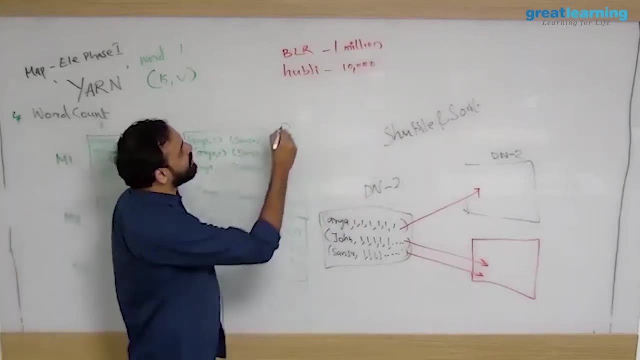 They also had a Hubli branch. In Hubli in a month probably 10,000 transactions will happen, Because Hubli is not as big as Bangalore actually. And then they have a Chennai branch right In Chennai again, let's say, 2 million. 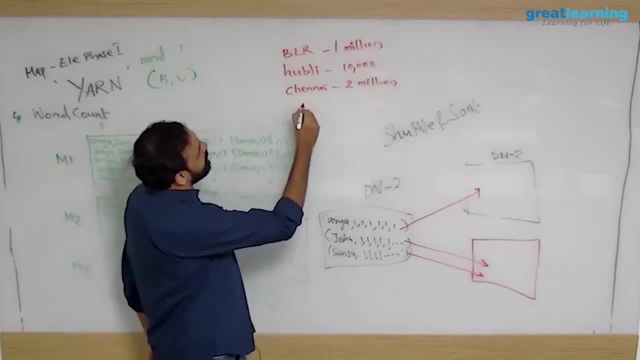 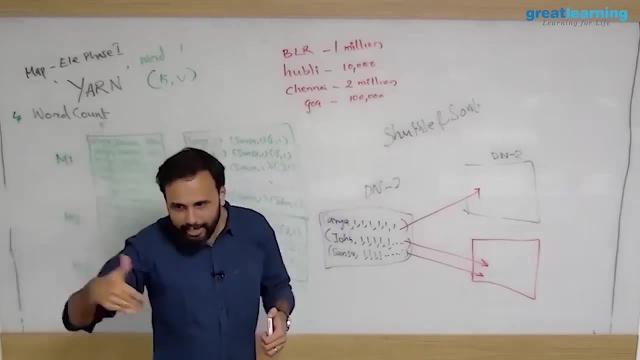 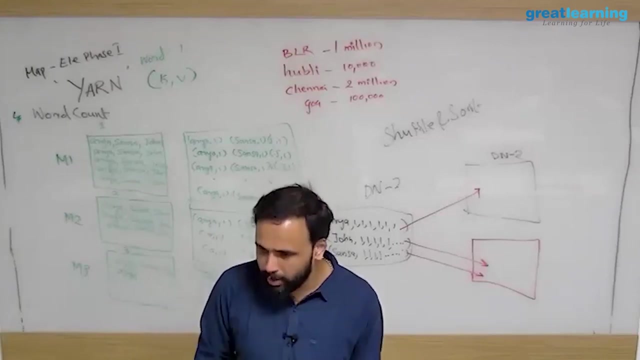 Probably there are a lot of customers here, okay, And they had a Goa branch. Goa had, let's say, 100,000.. So this transaction data will be stored already And the transaction data will have multiple items like customer number. what amount he transacted? 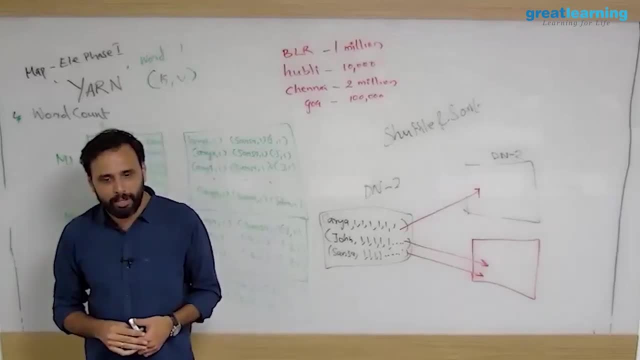 So they want to figure out branch-wise total. Same example. So the branch will become the key, Each transaction will become the value. So if I'm collecting all the data from Bangalore branch, there'll be a branch code That will become the key. 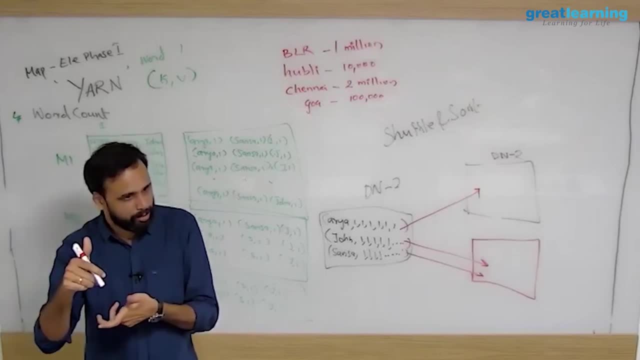 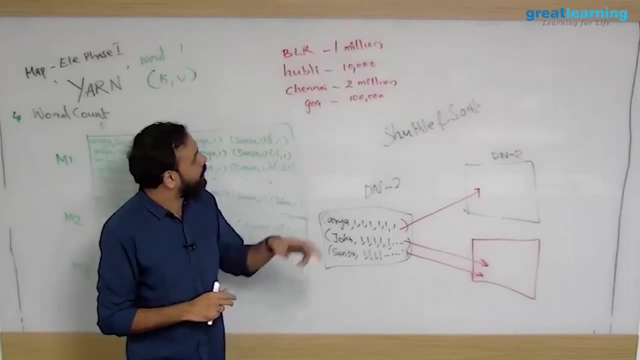 And each transaction the amount will become the value for that. So for Bangalore you will get 1 million key value pair. For Hubli you'll get 10,000 key value pair. Again, Chennai: 2 million. 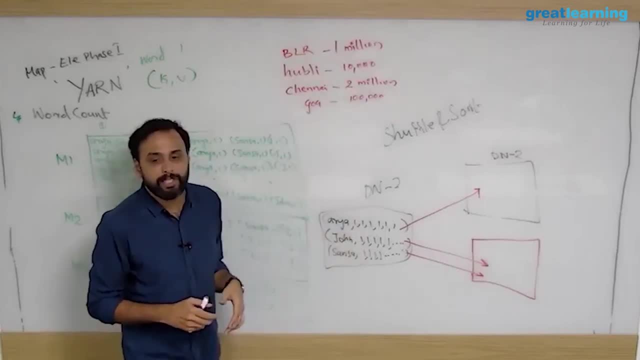 Goa 100,000.. Like that, so many will be there. So this is called a skewness in data, data skewness. Data skewness means somewhere you're having more data, somewhere you're having less data. Now the problem is: imagine you had only four branches. 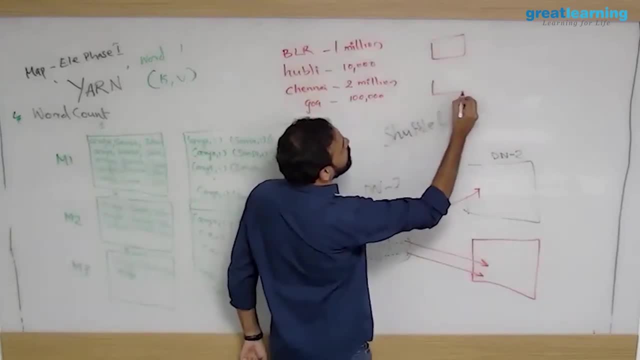 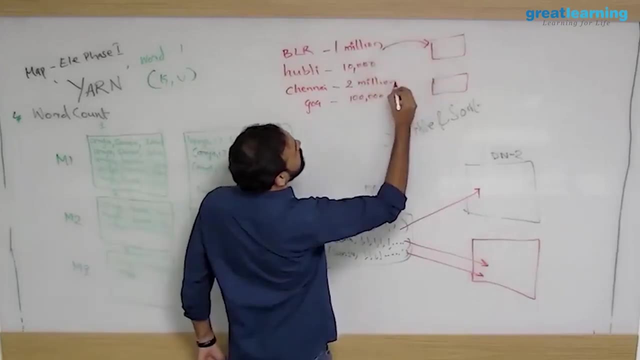 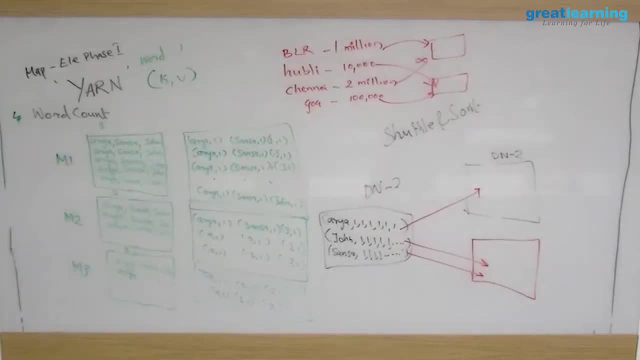 You see the problem Because by default in MapReduce it will try to evenly distribute the data. There is no guarantee Right And ICICI bank AC. if I do like this, my first reducer will take a lot of time to complete. 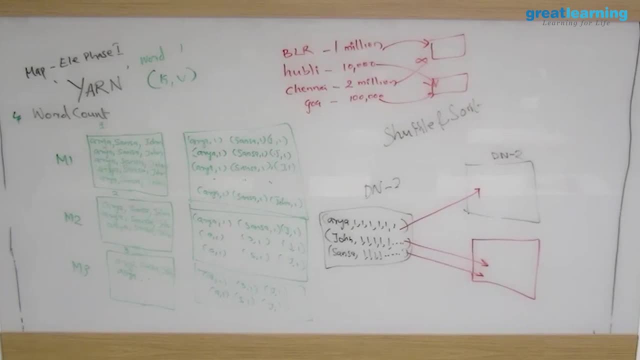 because it has to add 3 million values. Second, reducer will be very fast because only 100,000. values. that is where you will write a custom partitioner. you can write some. it's a class in java custom partitioner where you can say, once the shuffling is done, which key you should give to. 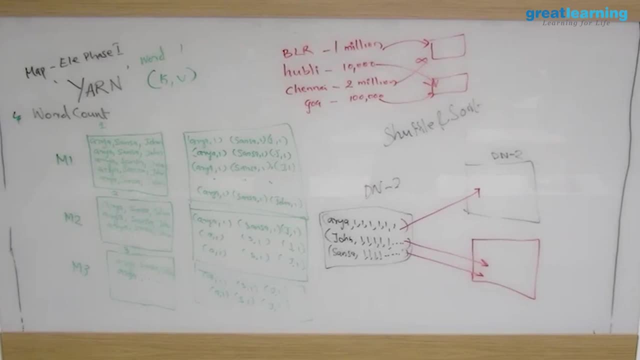 which reducer you can manually mention so you have control on the distribution. otherwise it will automatically shuffle and some reducer will pick it up and will be slow also sometimes. yeah, the hash partition will try, but there is no guarantee. that's why. so it is better to write. 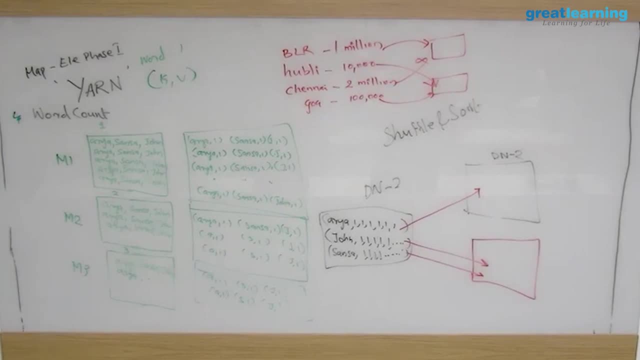 on your own. so production use cases: we never use hash partitioner because you can't get a guarantee. and also, once you write a map, reduce program- it's very difficult to again modify your. see, we are learning now in the real world. it is different, right, if a program is already running. 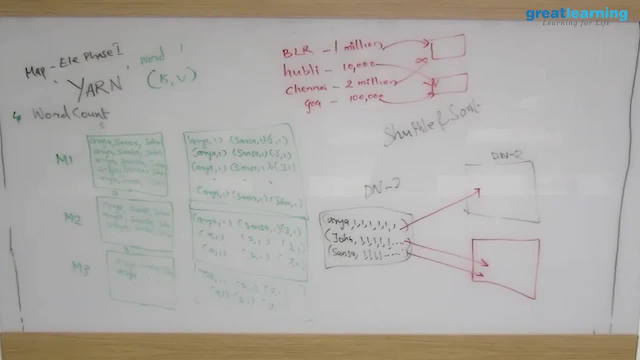 nobody will allow you to modify it. you have to stop the process, then write a new program, and nobody will allow you to do that. so when writing itself, you optimize it. so there is no problem later. spark also relies on the similar idea, but the difference in spark is here. 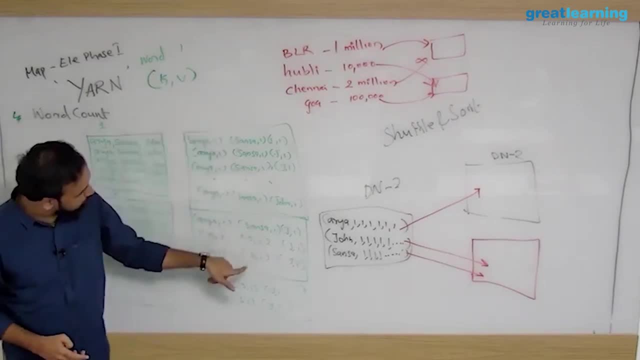 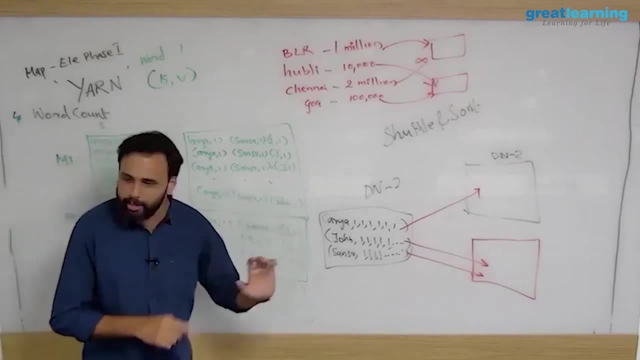 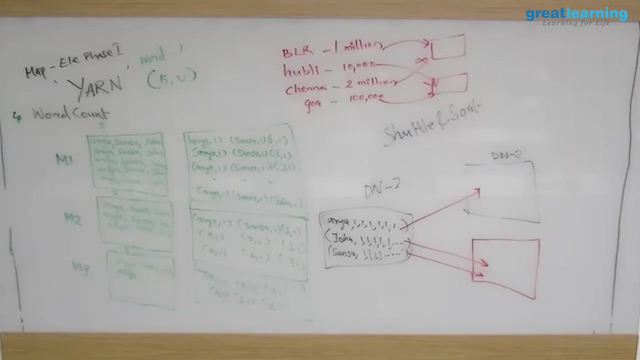 one thing is that after the mapper reads the data, it will push this to hard disk. spark doesn't do that. spark keeps everything in memory ram, so it can do this whole thing in one shot. give you the final result. so spark is 10 to 100 times faster than map reduce. it's proven that it is 100 times faster. 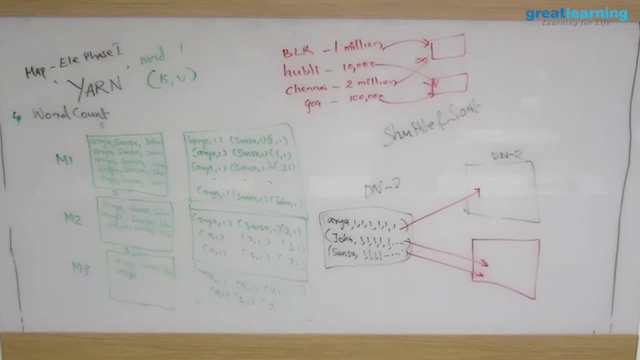 in many cases. point number one. point number two is that in map reduce, originally hadoop is written in java, so a lot of people started writing map reduce in java and i'll show you the code. to be very fair, it is very difficult, right? it's not very easy to write a java program in. 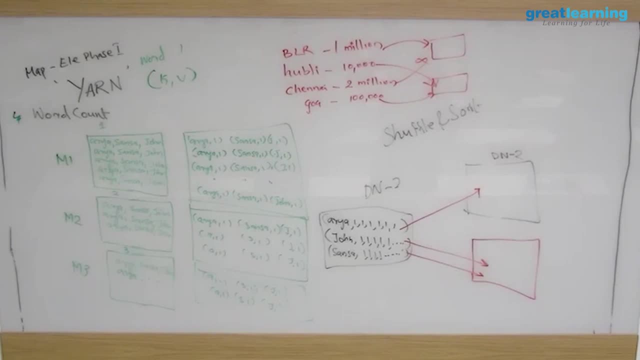 mapper. it is too complicated actually, if you write it right. so the learning curve is very high. if you go to spark, people prefer either scala or python. you can learn scala in a day. today you can learn. tomorrow you can start writing spark programs easily. you have a way of programming which is 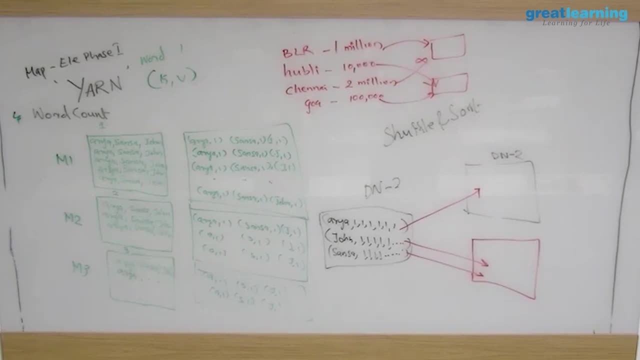 very concise and short, not like java. so writing a python program it will take one by tenth of a time. also supports python. another thing: right, support is added, but still, comparing with you know, spark it is much faster. anyway, you are taking transaction data. how does transaction data look like you will 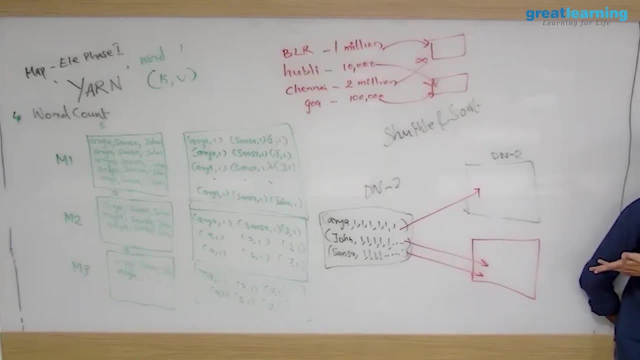 have customer number. customer, do you need all all of that for this? no right, i need only the branch code and how much amount, key and value. well, you can have composite key and all, but don't discuss right now. but normally you have a key and a value. so from 27 column unit, only two columns, 27 column. 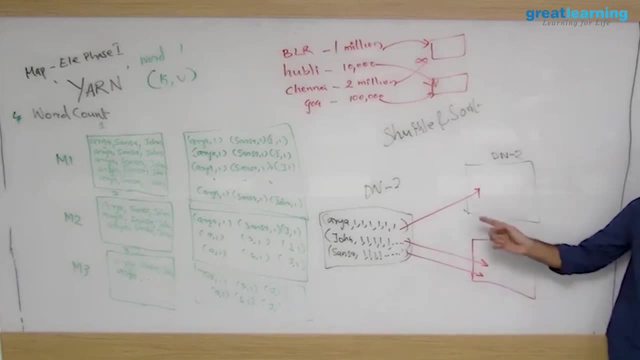 terabyte. two column data will be one terabyte. so usually it can accommodate on one machine. that's what i'm saying usually most of the cases. theoretically it runs on multiple if possible. but we have never come across a situation because even these boxes, these data nodes we are handling 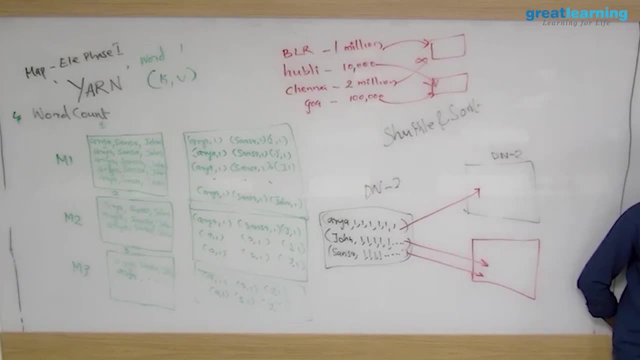 are also very high capacity hard disk right, so it will be at least 60 terabyte plus. very rare that you get 60 terabyte like. we had a use case where there were 2 billion values. 2 billion values is 2 billion. that's easily accommodatable, right most of 2 billion values we had. that was a use case. 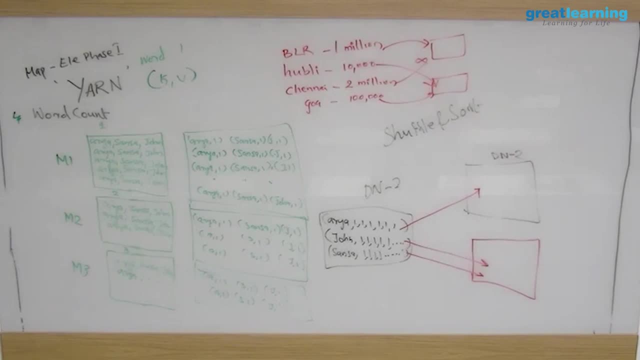 we got around 2 terabyte of data total required for doing the shopping. so it can do any sort of operation which can be represented in the key value format. so the only rule here is that whatever data you want to process, okay, it has to be represented in the form of a key and value. 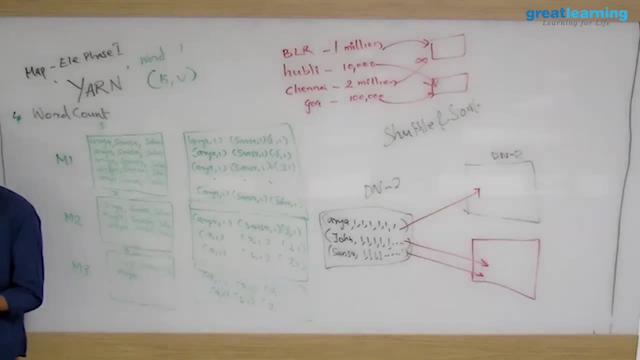 for example, you can use it for image processing. okay, i will show you an example of that. and there is another: flight delay analysis. i will show you. so, rather than telling, i'll show you examples of where it is actually used. you know different that you have to. 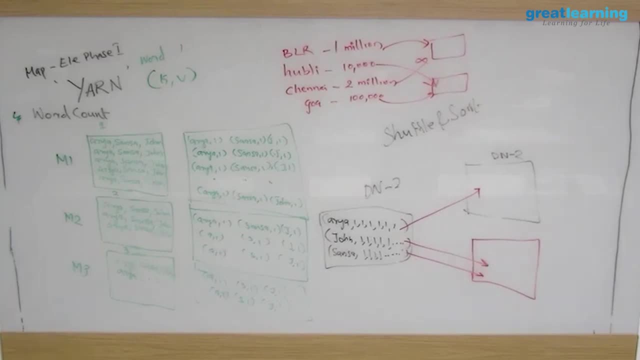 write the logic in the mapper. yeah, exactly, because you will have the original data. from the original data you will get key and value. key and value you have to process because that is why you're extracting. so if you don't want to process something, you have to remove that in the mapper. 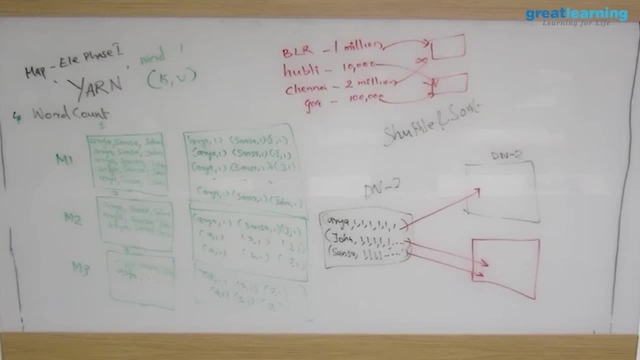 side the mapper output will be processed anyway, or in the reducer, i can say: probably write a logic. if the mapper output will be processed anyway, or in the reducer, i can say: probably write a logic. if the key is this: don't process it, it will not process. but that is useless right, because anyway it will. 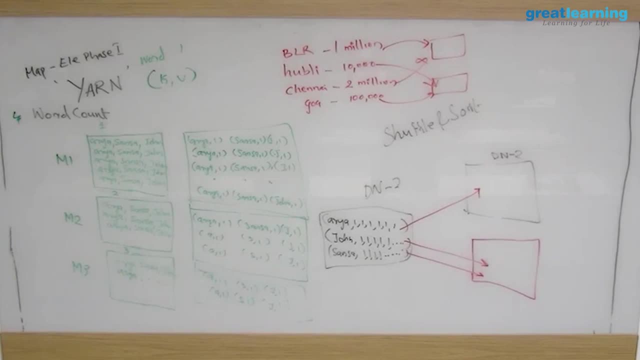 come through shuffle and everything. if i'm not processing in reducer also, it doesn't make any sense. text formatting, cleaning, everything has to happen in the mapper phase, like so, if i have a unstructured line of data, okay, i want only this as a key. this has a value. i can write a. 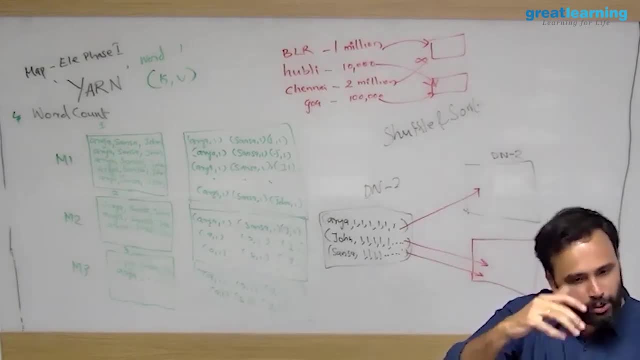 logic for that. other things i can avoid. so the custom partition is actually a code in your map: reduce program. if you're a java developer, you can write a java program in that or python or any language. but the difference is that if you are writing a java program, this is for java developers. 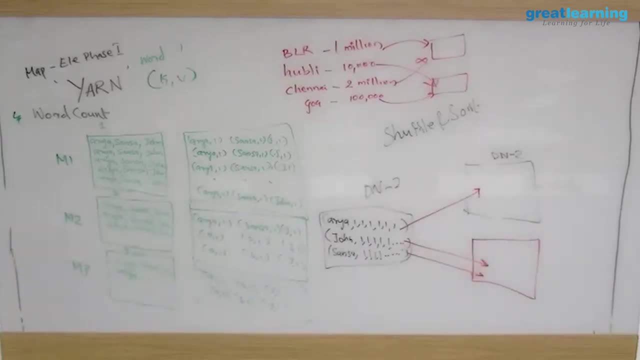 you have to compile it. to produce a class file, then you'll package it as a jar file and then you will submit it. to mentioning your public class you say run. if it is a python program, there is no compilation. if you dot py file, you will have something called hadoop streaming utility. 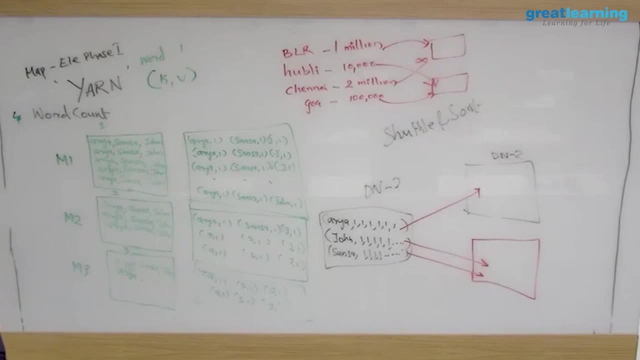 you will tell hadoop that it's a python code, not a java code. so hadoop will give you a jar which will run this as mapper and reducer. because python, you don't get a jar out of it, it's a dot. py file doesn't compile as such if there is an intermediate result and if that node has crashed, it has to. 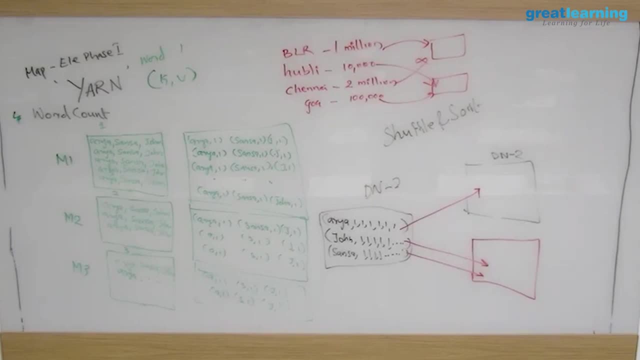 rerun because it is not persisted anywhere. and, very interesting point, the intermediate result is persisted in local file system, not in hadoop. if it was in hadoop, you will get a replica. are you getting my point? it is in linux, it is persistent, so if that machine crashes, it's gone right, so it. 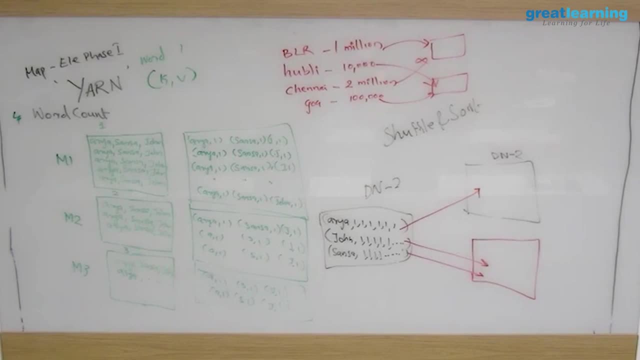 again has to run that mapper on another replica block and get the output. there is no other way to get it right. it can be configured when you are running a java program. it can be configured when you are installing hadoop. there is something called map reduce scratch directory, where you 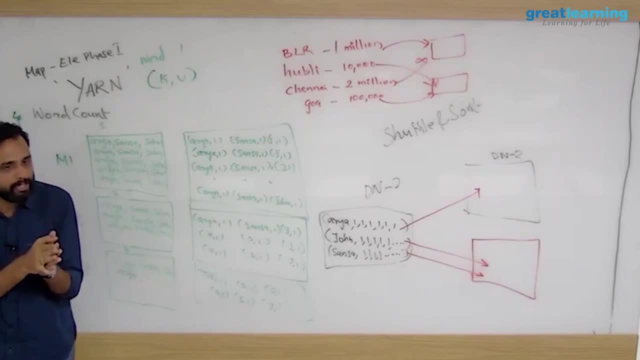 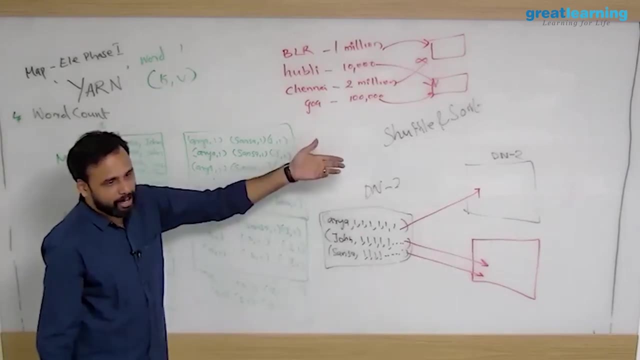 have to mention. in each machine you have to create a folder and say that this is where i'm going to store my output and when the shuffle starts, once mapper is running and the shuffle phase starts, this data is automatically loaded into the ram. each machine will load the data. 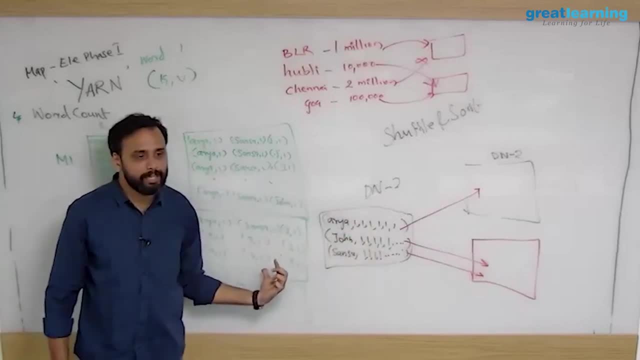 actually this guy does not need to know, because why you are persisting is so that if, uh, you know, some machine crashes, right, you can still recover the data. that is why you're persisting. so if the shuffle and sort starts, okay, this data will be loaded into the ram. it does not have to. 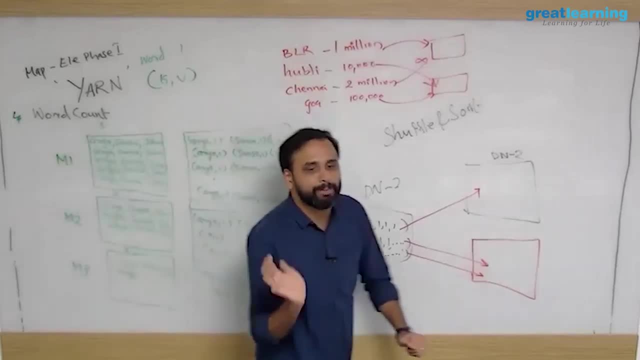 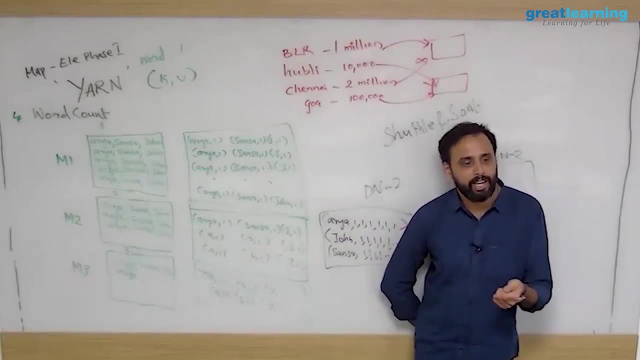 read from the hard disk. that data from scratch directory will be pushed to the ram. you start reading from there. storing to the hard disk is persisting. ram is non-persistent, meaning if your machine restarts, whatever is there in the ram will be gone right. hard disk is persistent storage if you store in hard disk, even if i restart my box. 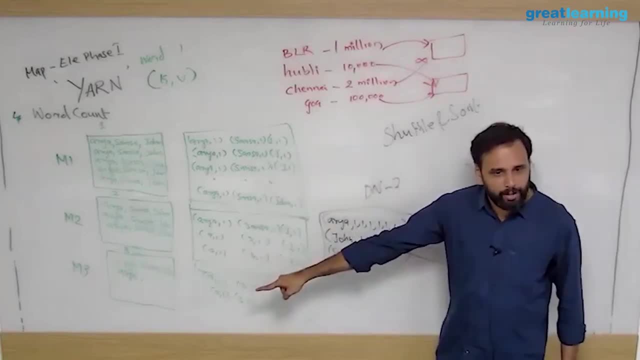 it will be there. so otherwise, if it doesn't persist, what is going to happen? if you want to, if, let's say, the reducer was running, okay, this machine crashed, right, they're not persisting here. probably this is in the ram. it can lose again. you have to start from here. all the faces, right? 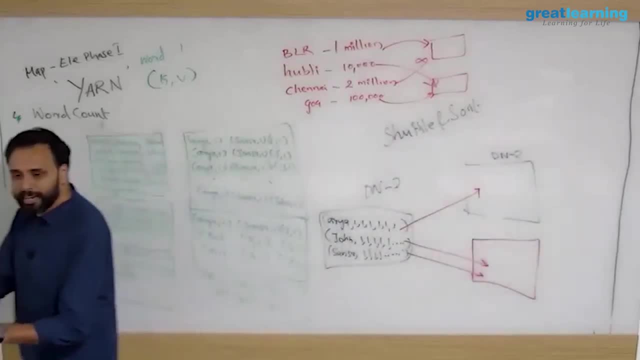 so in like, in the middle stage, you are just temporarily, you're storing the output. that is persistence. there is a format actually in the ramp. it's not like the data will be directly loaded. all this data has a specific format so you can identify what it is and the process can read. 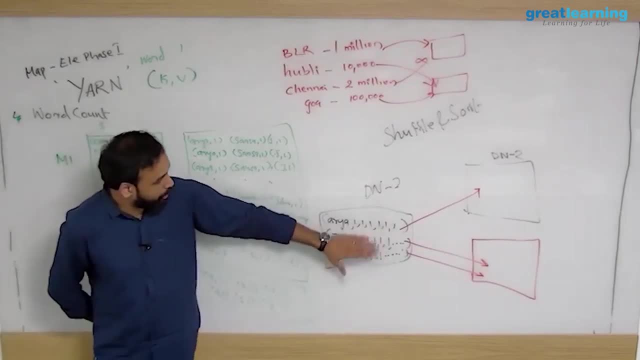 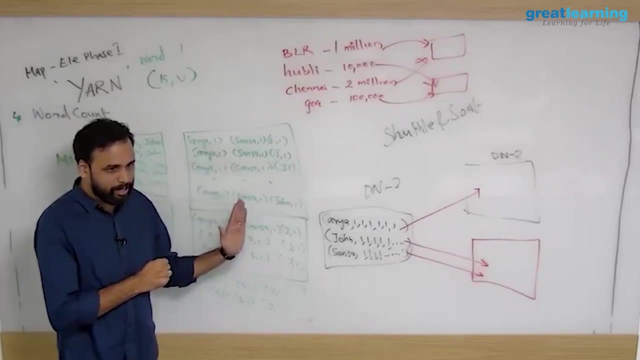 from there: no shuffle, and so data is normally. uh yeah, once this is done, this is also persistent. so all these are java processes, so it happens step by step. once the mapper process is done- okay, it could have persisted the data, right. the next process kicks in is shuffle and sort. 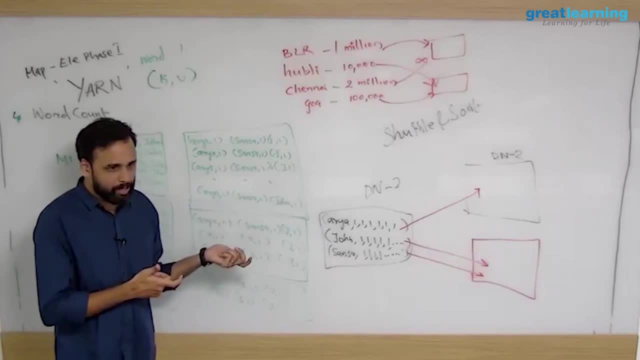 shuffle and start process will start and it will request for data. so this is a distributed framework, like it will, and it could have known that mapper ran here here here, so it needs data from here here here. so, whatever this temporary data you persisted will be loaded into the ram. 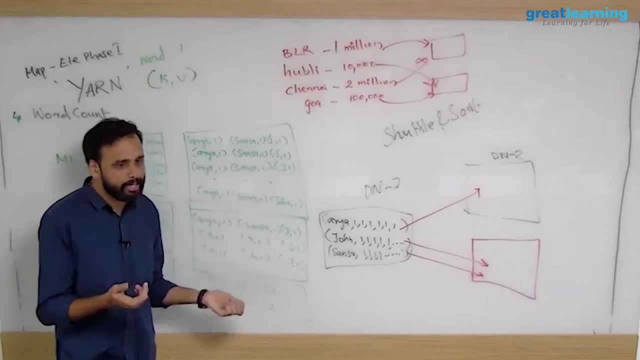 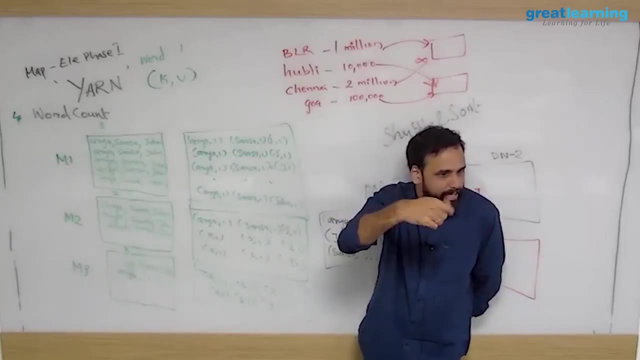 so data will be available as key value pairs in all these ram. it will read it. all this will have association index. it will tell which data belongs to which key, which value. then only you can understand right where is the data. these are all happening as part of one framework you don't have. 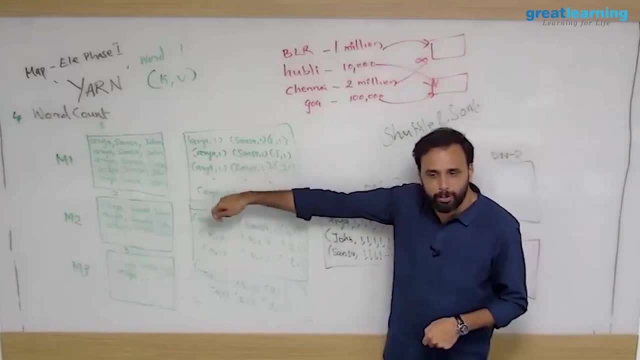 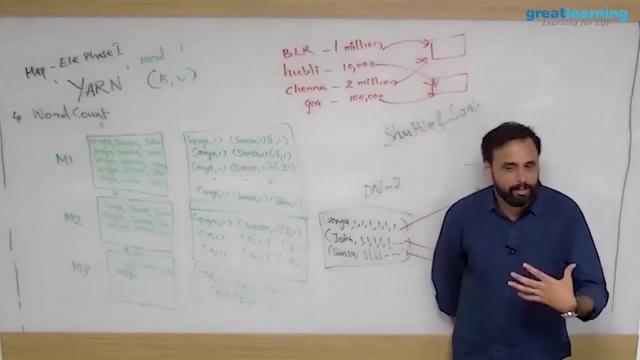 to bother at all, because all you need to bother is mapper code should be written properly. this part will happen, will be handled by the framework. so there is a java class, java object which handles all this right. this java object gets acknowledgement for every read and write that you are doing and it has something called an associative array where it store the index of 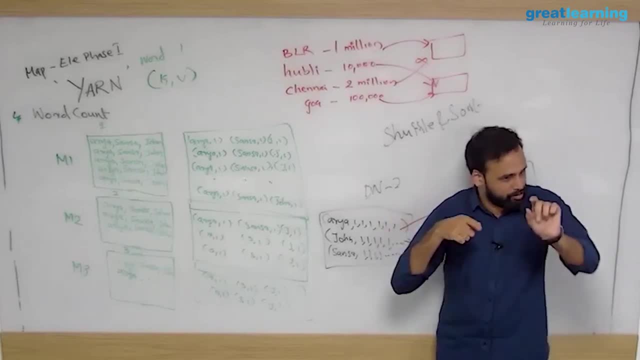 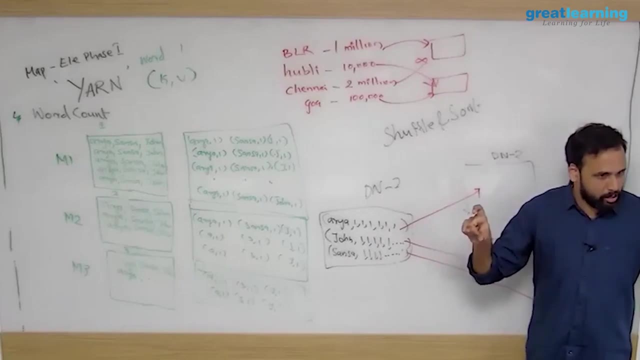 each key and value you are persisting and where is the location, which folder it is there. so once this process is over, this java object will look at this array. it will understand. you have 1 million to go to the shuffle phase and these are the locations where it is and automatically the 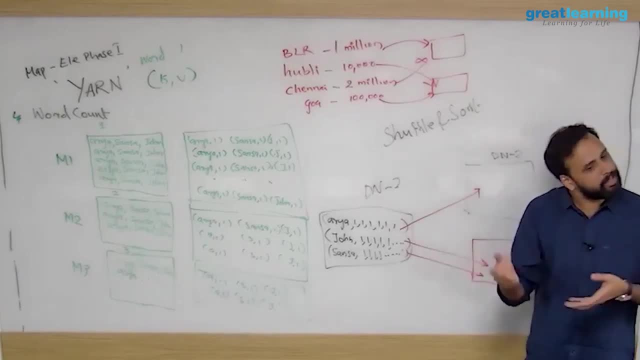 machines will load the data because it is a continuous process. it will match and give it to the second phase and that will process from there. also, fine tuning map reduce is very, very difficult because internals of map reduce is not really easy to learn and to use. it is not easy to 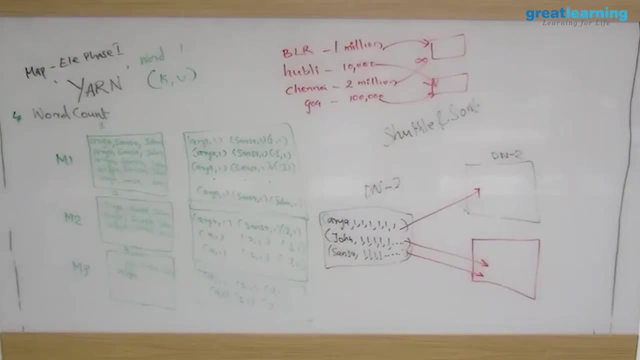 read when you're writing the code right. basic code writing is very simple. you can write and run the code. that's not a big deal. but internally writing the code and tweaking this will take a lot of java knowledge that. so one of the reason i feel map reduce became obsolete is that it's very 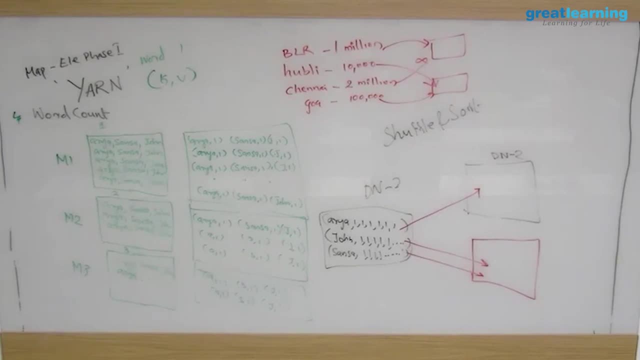 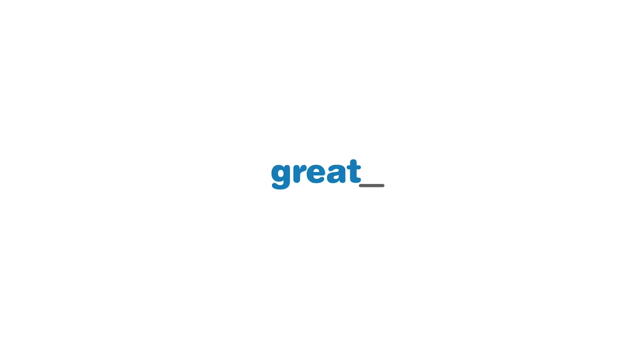 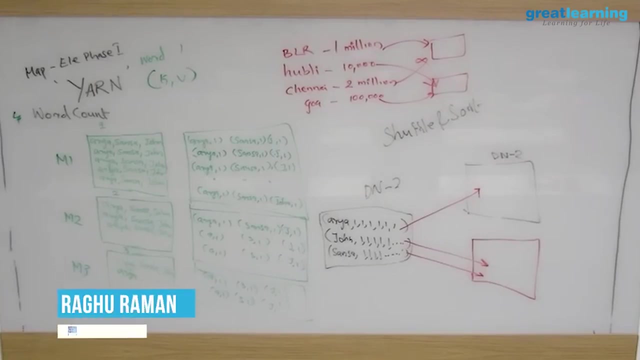 difficult to learn and practice in day-to-day life, right. so even if you are a java developer, if you have to write a map reduce code, you can't write it in a day. another important point for java developers is that for key and value, we don't use normal data types in this. 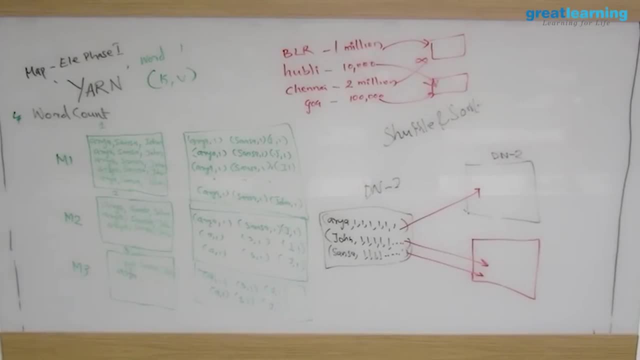 key will be string and value will be integer. that's what you think. no, key will be text, value will be something called interwritable. why? because you know what is how, how to pass data from one machine to another machine in java: serialize it, right? so what is serialization? convert to binary. 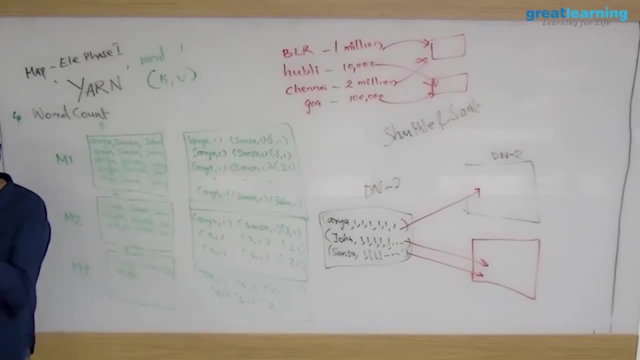 why are you doing it? so there is a serializable- uh, what you say in java, what you call interface, right, serial episode in a serializable interface is there where you serialize the data, right here. what happens is that, since it is running on three machines, this shuffle face and 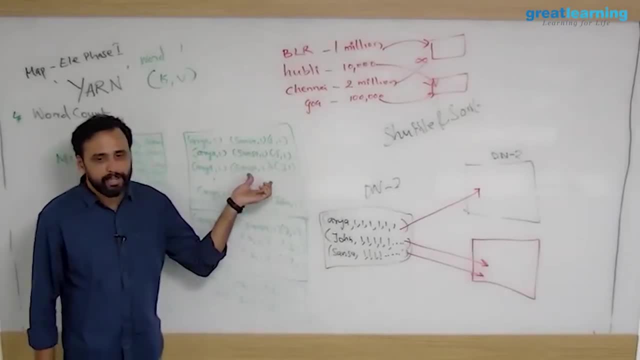 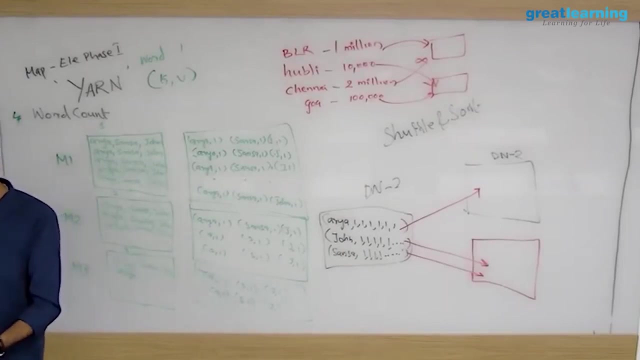 all can be very costly because if i have one million values here, it has to be read into one machine over the network so this has to pass from here to here over the network. so there is a wrapper class. are you aware of wrapper classes? yeah, so there is a wrapper class called a writable. okay, 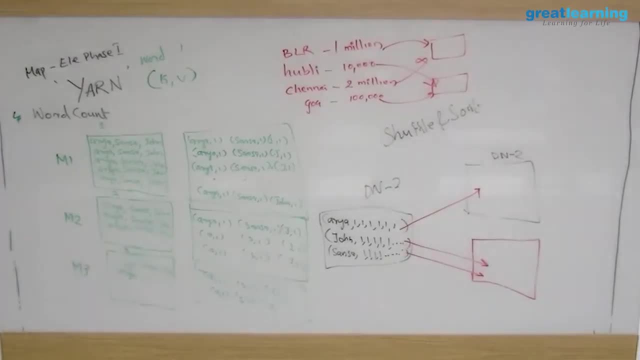 map reduce has done, they use that wrapper class. so instead of integer, okay, the wrapper class is called int writable. so serialization will be done by this in writable. the advantage is that it will compress the data while sending through the network, right? so in the shuffle, face and all. 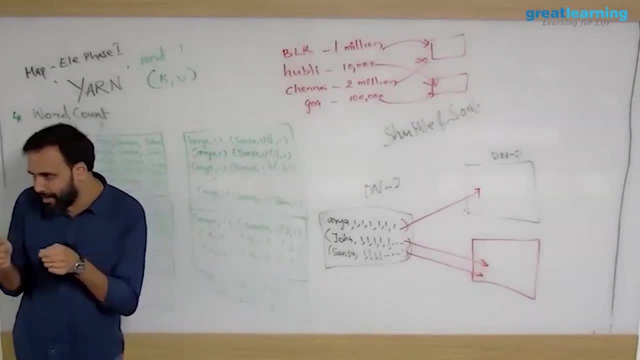 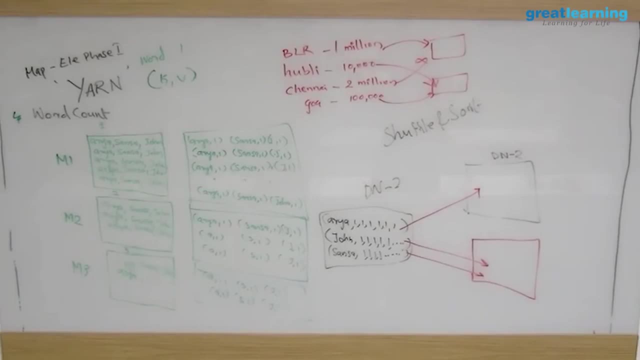 it can be faster. so whenever you want to represent your key and value you, you cannot use your normal classes. you have to use these wrapper classes in your program. this is to actually compress and save output. serialization is handled by map reduce. we are not using java serialization interfaces. 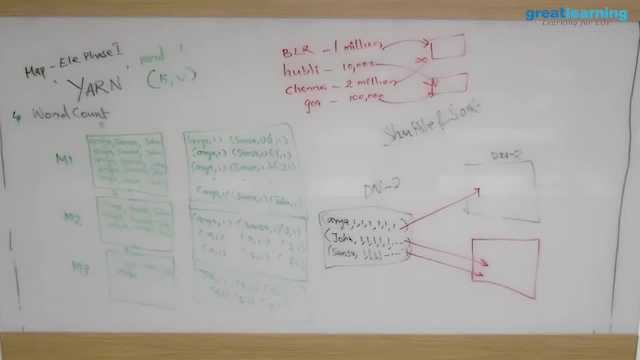 this is only for java people. others may not understand. but just understand it is compressing and sending the data, serializing and sending the data. it is tcp only, pure tcp connections. only only the serialization differs. apart from that everything is same. only all the machines will be talking through our tcp port numbers, only for communication. but you will. 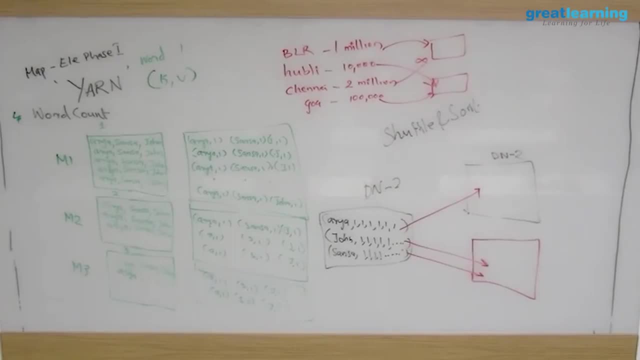 not use the regular classes. that is the difference. you will not say i want to use string. i have not asked the most important question. when i say i am reading a file from hadoop, what kind of a file you want to rewrite, file you want to read? for example, this might be a text file. 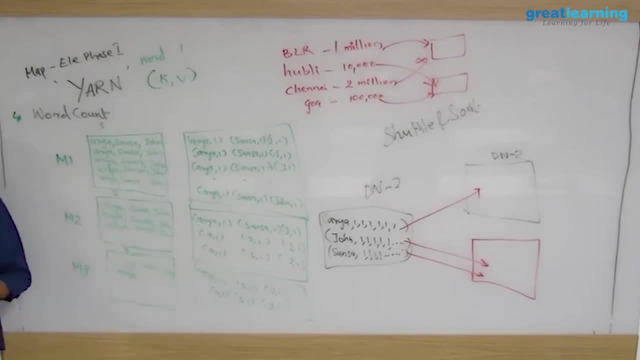 these text files only supported. no, you might have xml files, you might have video files, audio or any other type of file. so how can you read a file? first step in map reduces. this is all the running steps. but before all this happens, it has to read from these source. right, i will explain how that is happening. but that's one point i wanted. 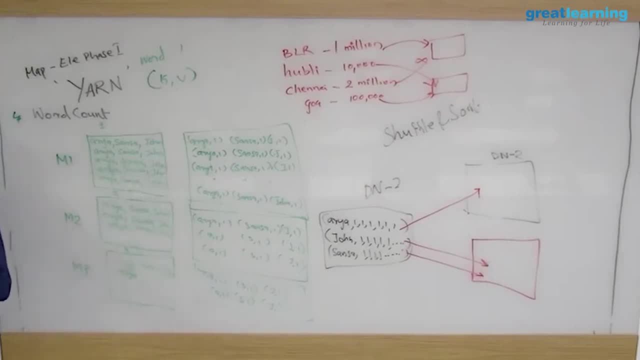 to discuss. so you have certain classes which will be invoked to read a different type of data. what we will do: we will run a map reduce program. since lab is pending, we will run a map reduce program. same word count: we will run, so you can see how it is running. uh, i will come back and i 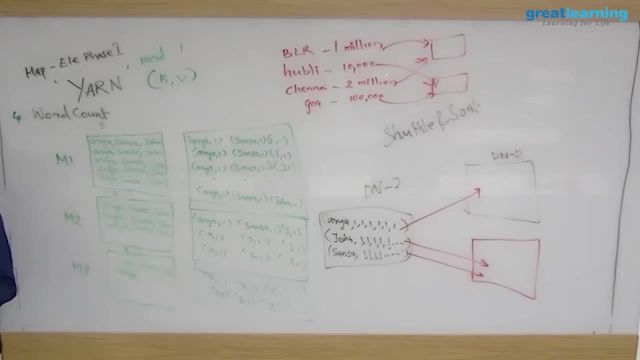 will explain the code. i'll do a code walkthrough and we will understand a little bit of yarn also. so i think lab is going to explain a little bit how to do so. we are just та99. we are going to do a C culture available. yeah, reducer will give the final output. you can say where you want output. in most of the 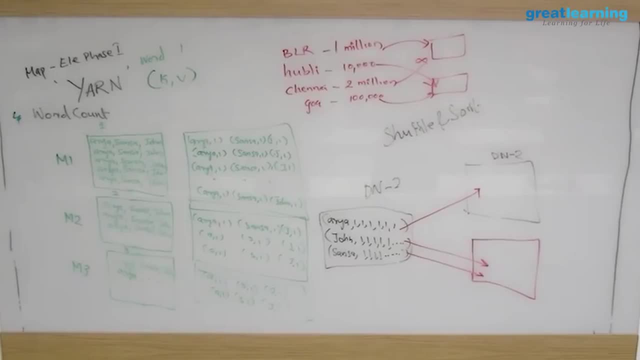 cases you will say: store it on a directory in hadoop. there it will be storing the output. you can open and see the output. actually python it supports, i know, but optimizations are mostly done in java because natively map reduce is written in java. so if i have to optimize in python it may. 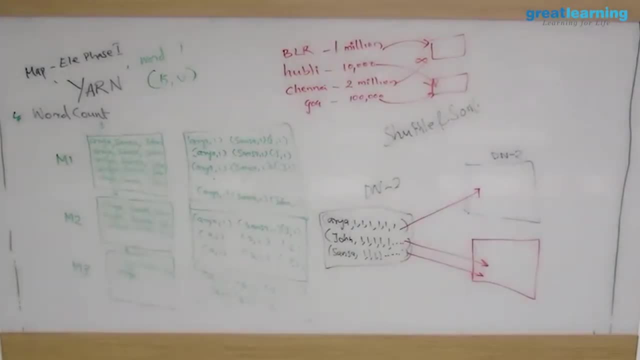 not. it may not be as efficient as i am doing it in java scale. i am not 100 percent sure, because when you say scala, you have spark, so why should you come to map reduce? that's the question, right? scala came in 2005. the language was created in 2005. it became popular only around 2010. 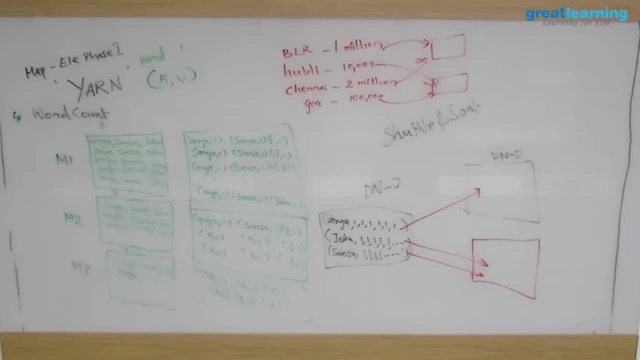 it's not as popular as java. by 2010, we got spark. spark is written in scala, right, so by that time we got spark. so when scala became popular, the support was added to spark than map reduce. by that time, map reduce was already in the dying phases, almost right. so what is this? this is one of the machines in the hadoop cluster. 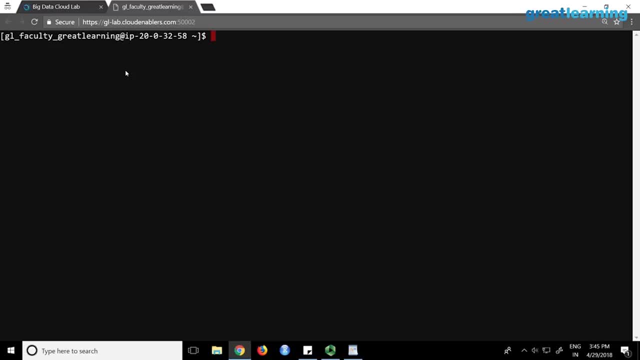 it is linux, right, so i may have connected to one machine. you could have connected to another machine. for example, can you try host name command type host name- is it the same that you see on your machine? so if it is the same name you are seeing, this is the gateway machine. 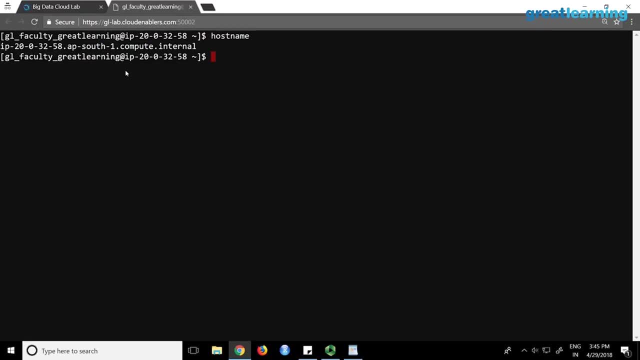 so this is the machine where the hadoop client packages are installed. actually, right, so you are connected to the gateway machine. now this is just a linux box. there is no hadoop running here, it is just a linux box. but this guy has connectivity with the hadoop cluster so you can issue all the hadoop commands or anything that you want to do from here. 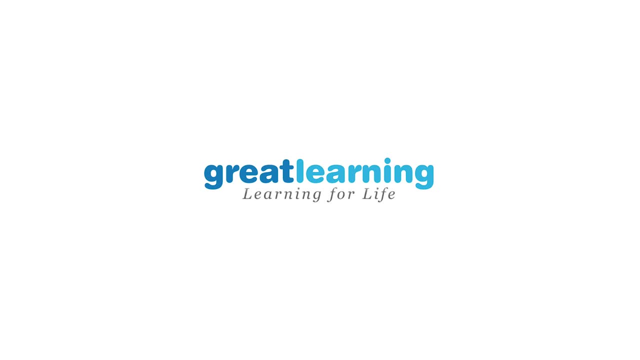 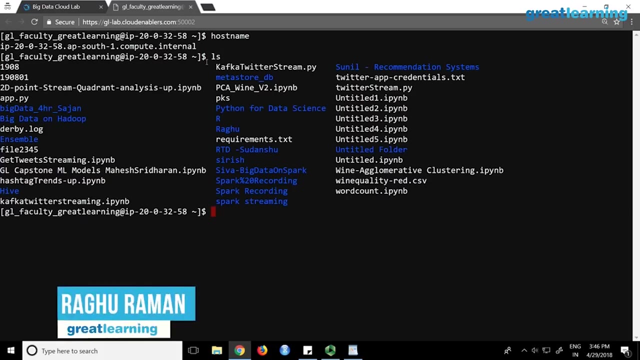 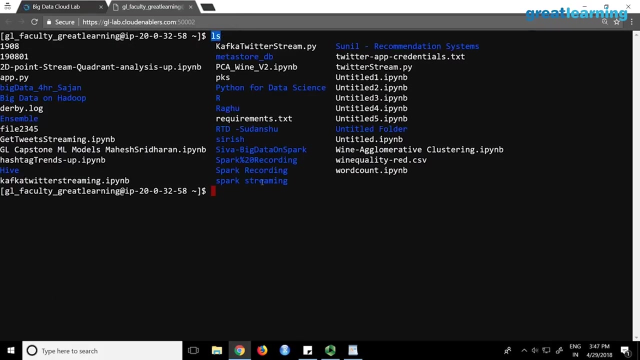 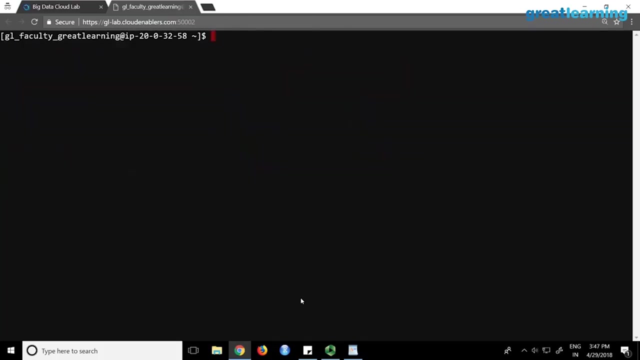 actually right now, first thing, just check, do an ls and see whether you have any files and folders. so if you do an ls here, you may not see anything because you have a fresh account. this is the faculty account. that is why you see a lot of files and folders here. that's okay. okay, not a big deal. first thing i want to show: 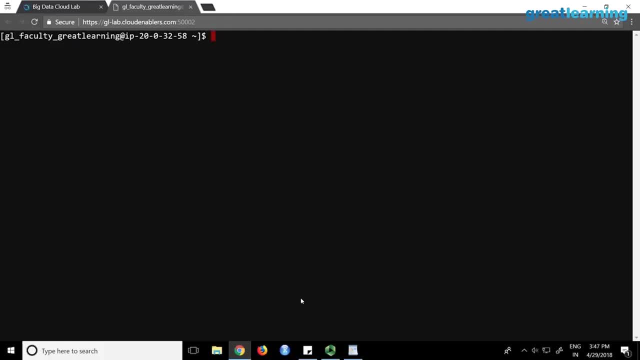 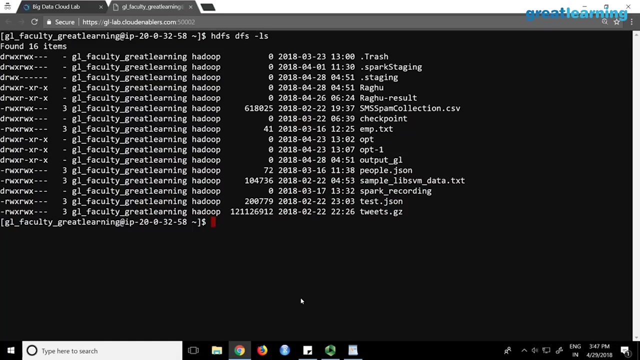 you is how to access your hadoop file system from here. the command is hdfs dfs, dash ls. just run this command: hdfs dfs, hyphen ls. as you can see, it is a linux command, ls is a linux command, but you are prepending hdf dfs. that is a syntax right. you won't see anything because there is. 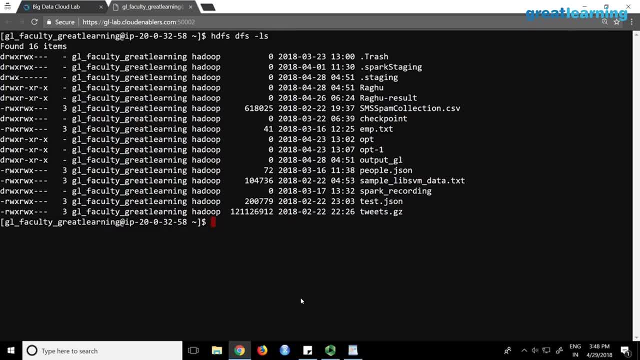 no file or folder created in hadoop for you. everybody will have a user account in hadoop. this is the faculty user account. you can see my files and folders, whatever i created. so let's create a folder in hadoop: hdfs, same thing, dfs, hyphen, mkdir. the command is make directory mkdir. 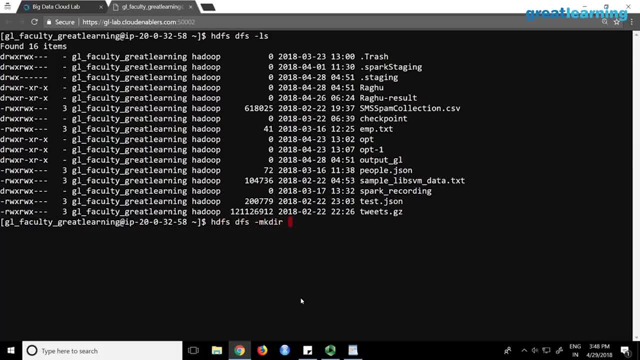 same thing: dfs hyphen mkdir. the command is: make directory mkdir, mkdir, Linux command and just give a folder name whatever you want. I'm just calling it as del, Anything, OK, I'm just calling it as del. And now, if you do an ls, you should be able to see that. 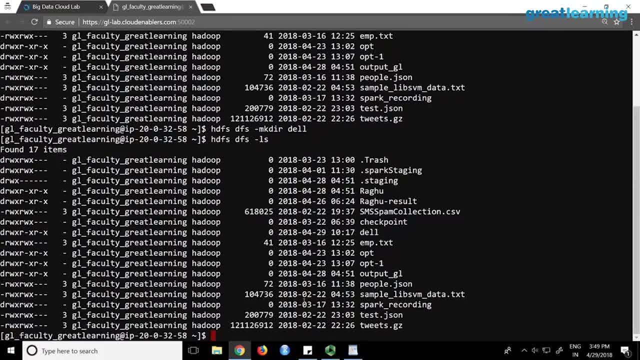 Just try. So. the mkdir command is make directory, create a folder. You just created a folder in your home directory in Hadoop And you are listing it. It should show the folder, whatever you created. And this is your username. This is my username. 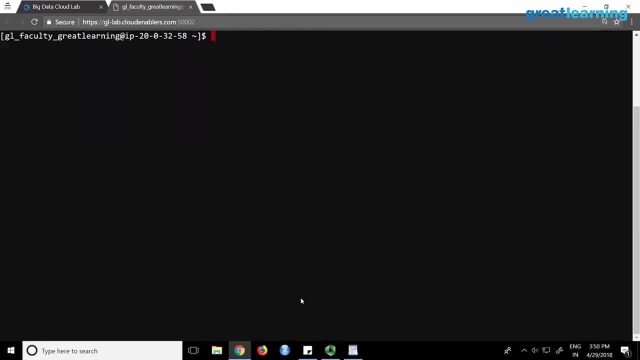 You should have your username, whatever. there There is Hadoop client installed. That is how it knows, Otherwise it doesn't know. So this is a gateway machine where the Hadoop client is installed. The Hadoop client has name, node, IP and port number. 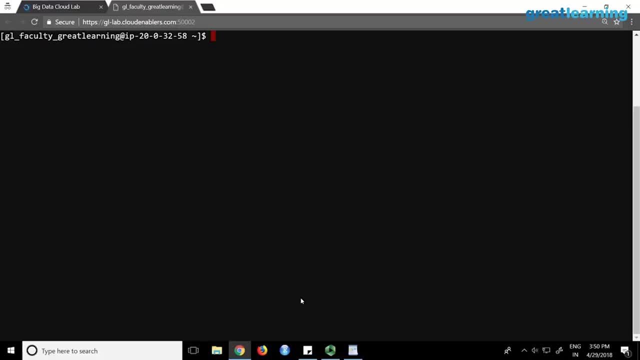 And the environment variables are added. So when I say HDFS it will talk to name node IP. Not all the commands- There are some yarn commands which may not go to the name node- But most of the commands first it. 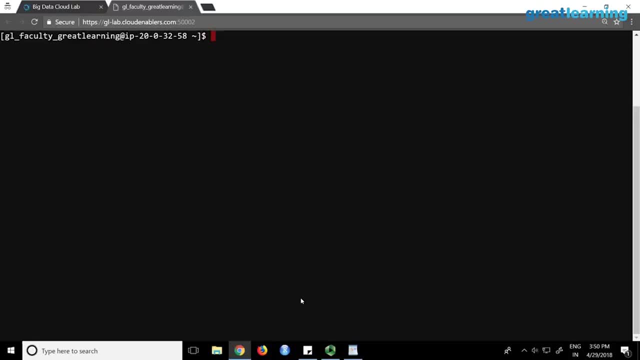 may go to the name node, Because you are creating a folder asking for a file. Name node is the guy who should do that. Now create a text file on your gateway machine Text file. So do you know how to use vi editor? 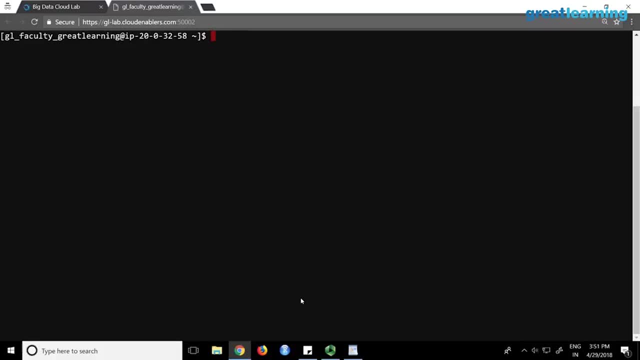 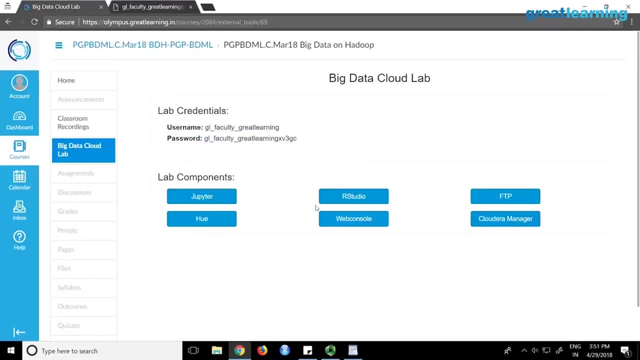 I'm comfortable. You can do two things. If you know how to use vi editor, you can use vi editor, Or what you can do, probably this is better: Go to this, cloud this page. You have FTP. Can you see FTP? 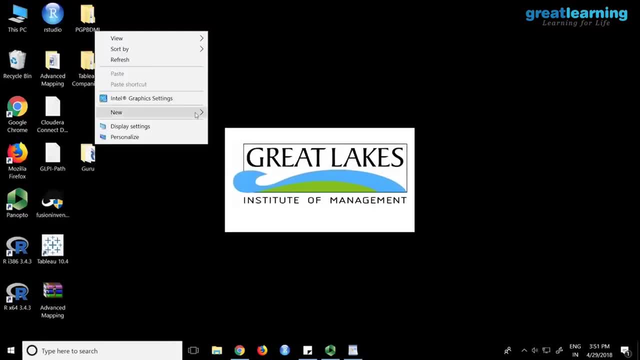 Don't do anything. Create a normal text file on your desktop. See I'm creating. Look at what I'm doing. I'm creating something called- I don't know- input. I think there will be a file extension, right? 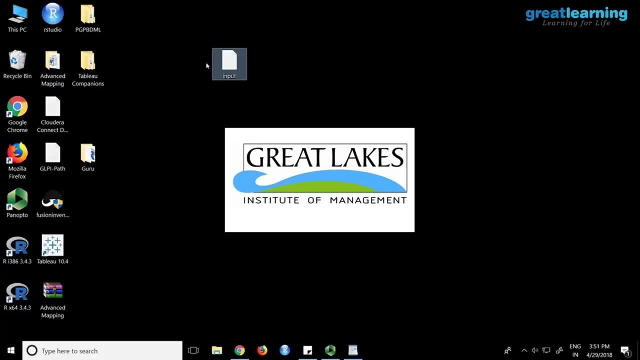 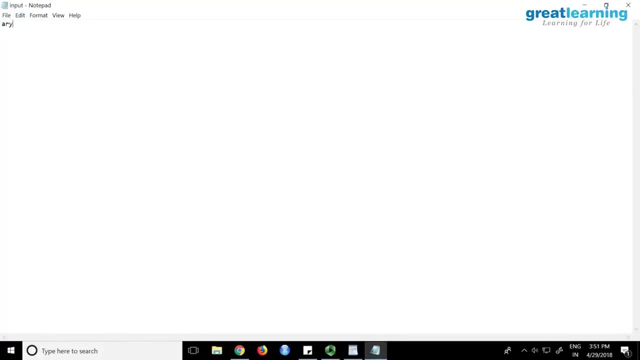 This is actually inputtxt, right? Fine, So create a text file. So we are going to do the word count program right, And let's stick with the rules of the game. So I have written the code in a slightly different way. 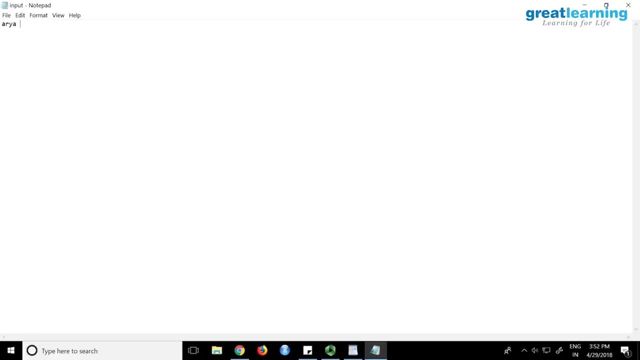 Let's keep space as the delimiter for the time being. Aria, What is that? Sansa and John? And just copy paste it so that you are. Oops, I'm just copy pasting it So that some lines will be created. 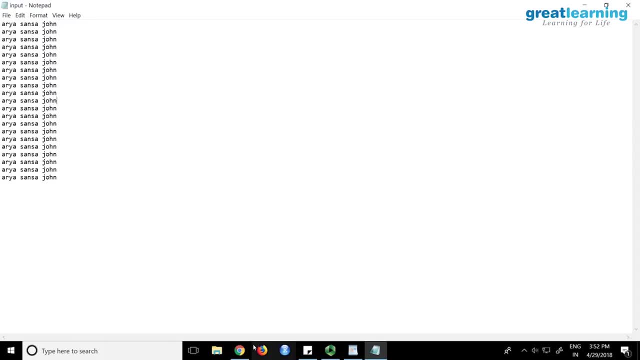 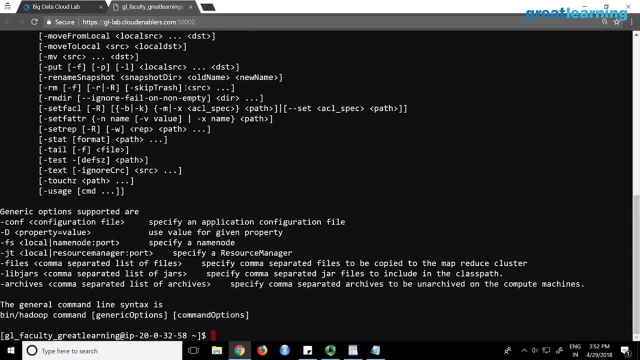 If you want to know that I mean what are the commands which will work, you can simply go here and simply say HDFS, DFS, just hit Enter. It will show you a list of commands which will work. So most of the Linux file system commands will work. 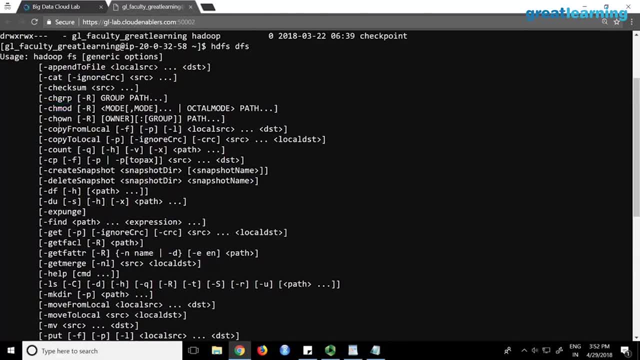 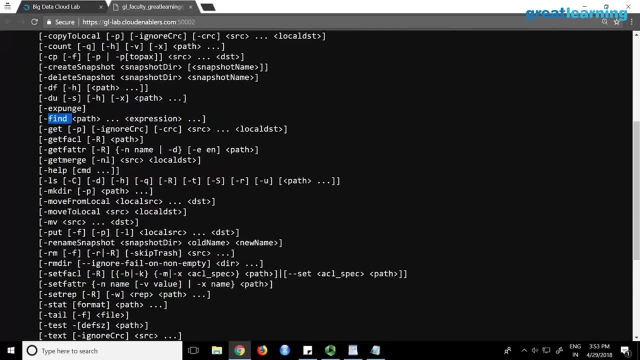 For example, cat change, group change, mod, chown count copy find. Most of them will work. One very confusing point which a lot of people learned at the last only, is that there is no CD command in Hadoop. 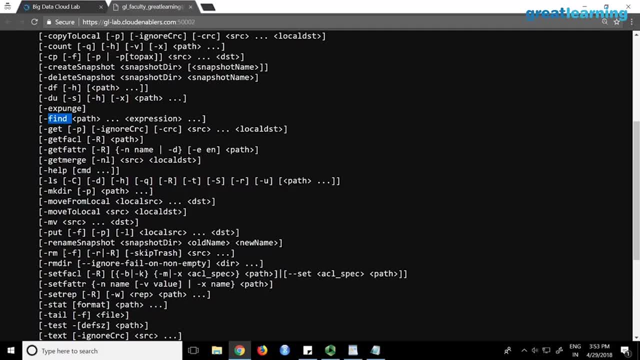 It will not work. You can never do CD in Hadoop. That means I cannot say move from here to here. I have to give the absolute path where it has to be or complete. There is no CD command And many people are very much confused. 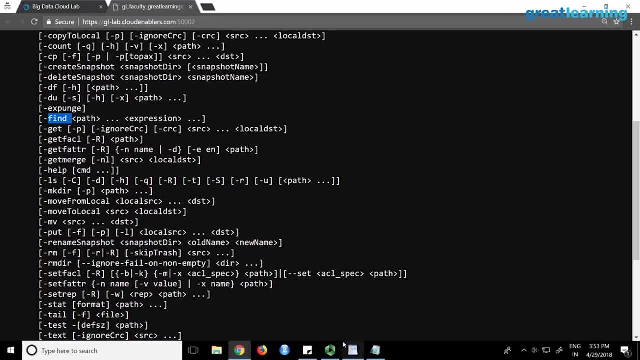 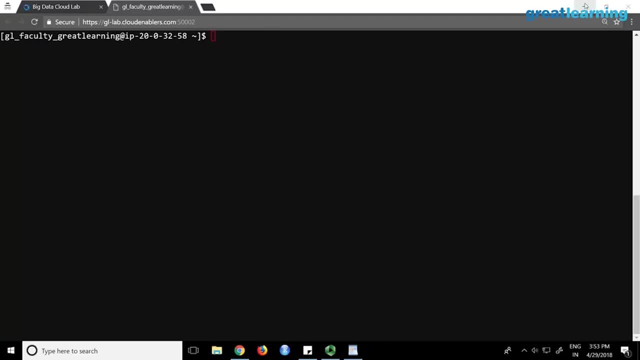 This command is not working. Why it is not working? Meanwhile, if you guys allow me, let me just check One thing: just create this file as of now. This is on my desktop And what you can do, you can do an FTP. 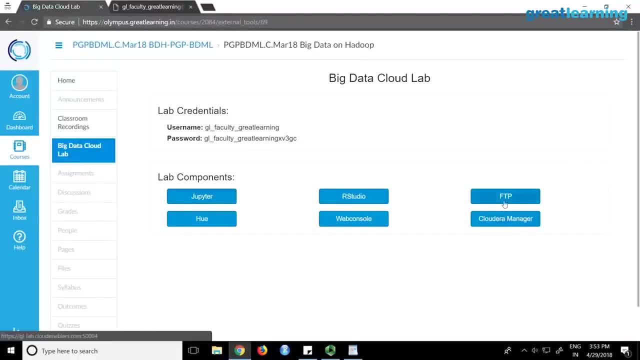 Just go here, OK. Big Data Cloud Lab. There is FTP. Click on FTP Type in your username and password. This is for people who are not comfortable with VI editor. Otherwise you can directly create it in VI. So I am in my FTP server. 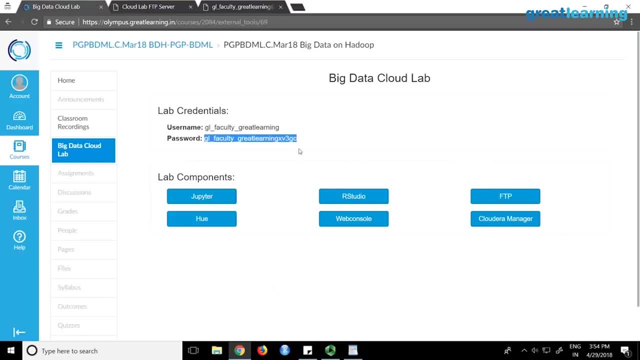 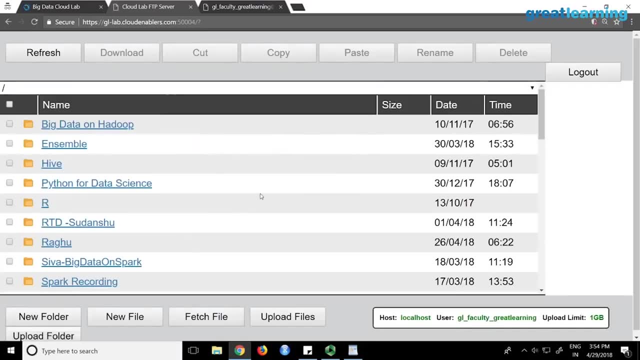 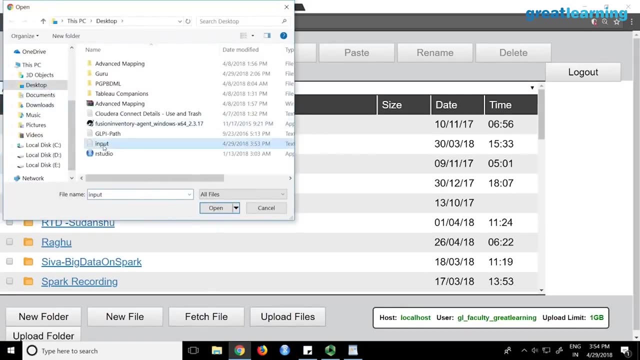 Type in your username and password, Say log in, And here you can say upload files. There is a button And you can simply search for the input file. Say open, But there is a no. no, don't do that. 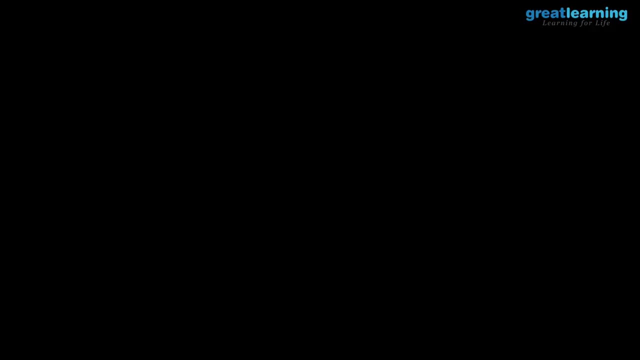 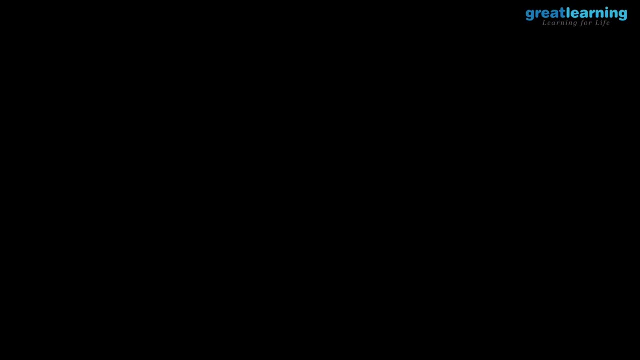 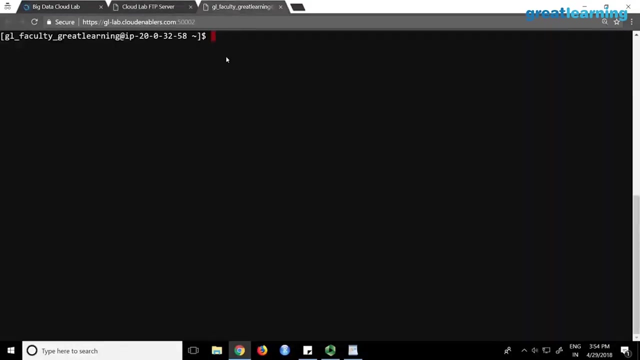 It's not working. Where is it? Where is the del folder? Oh, I'm sorry, I'm sorry, I'm sorry. Yeah, FTP, you are connecting to local Linux, right? Yeah, you can upload in the home folder. 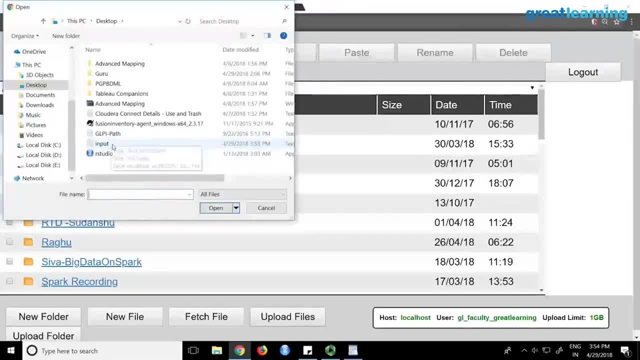 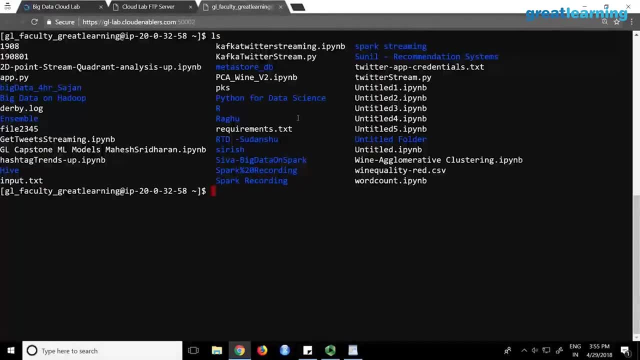 I'm sorry, I got confused. So I'll say: upload files. OK, This is my input file. I'll say open, It'll just get uploaded. And if I go to here, if I do an LS, there is the input file. 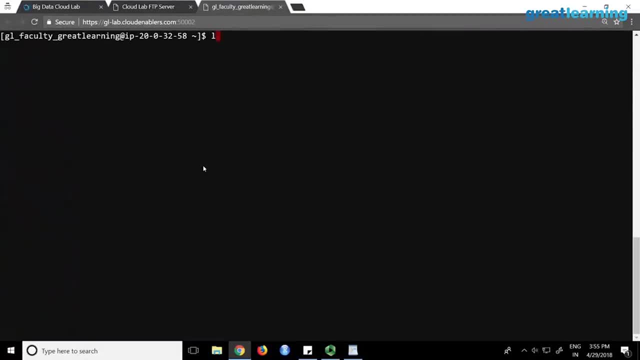 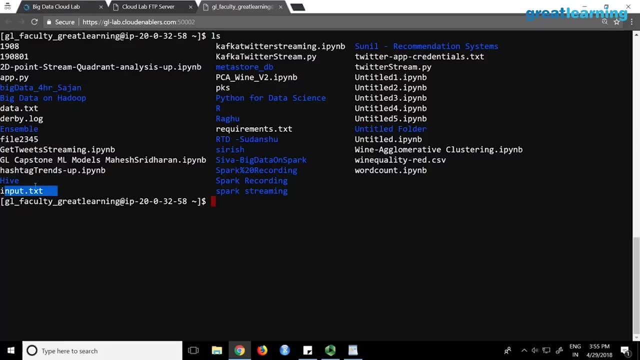 Where is input? But anyway, make sure that the file is loaded in your Linux file system. So when you are doing an FTP it comes to your Linux file system, right? So this is my inputtxt in here. OK, Now, FTP is just a tool to bring to your gateway Linux machine. 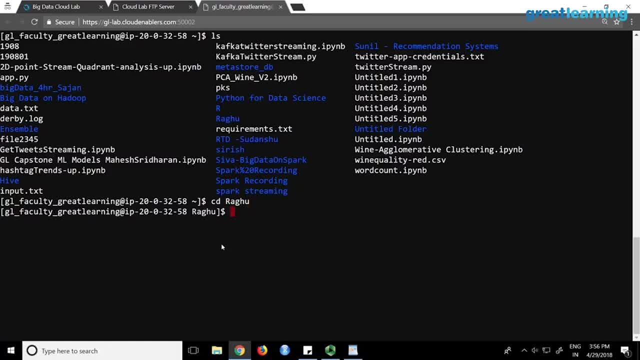 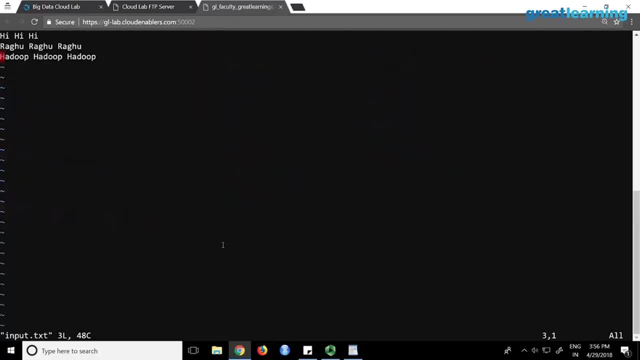 You are uploading from your local machine to the gateway machine, Linux, So let me just check. I'll go here. Oh, I have another input here. This is different, I think. No, this is not. That's OK. So are we all on the same page? 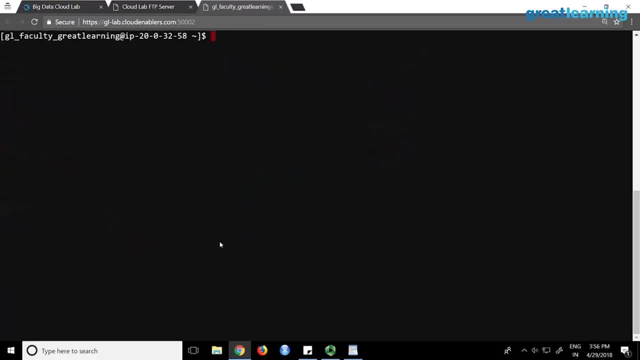 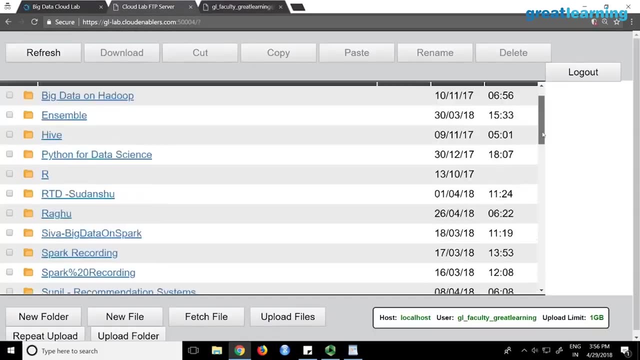 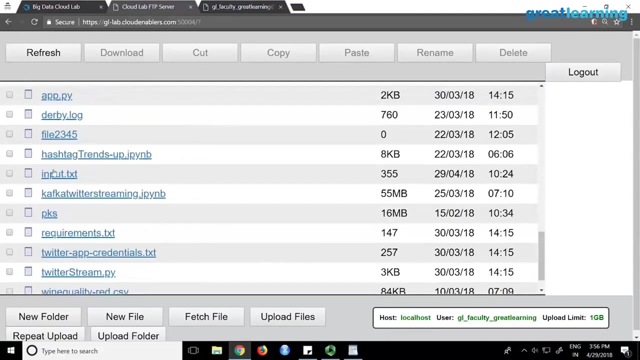 Yes, Yes, Yes, Yes, Yes, We are all on the same page. Like you have this input here. Is it listing here? Yeah, See, now I can actually see the file. Where is the file? Yeah, inputtxt. I can see in FTP. 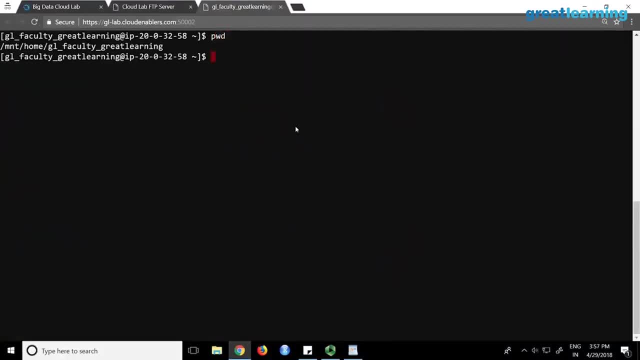 Same way. can you see it in FTP: Do a PWD. Do a PWD. You should see something like home, like this. So I think the file is available for you right Now. what we should do, We should upload this file to Hadoop. 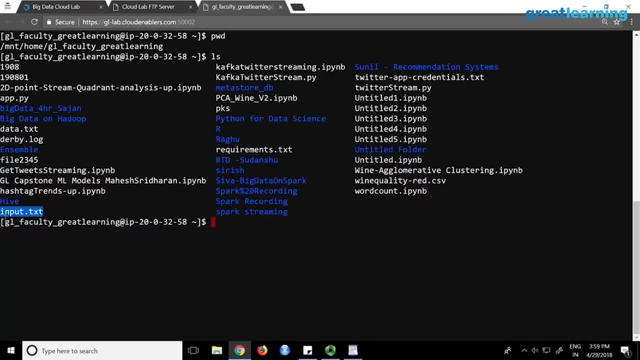 Right, So this is the file called inputtxt. I have to upload it to a directory called Dell. I created a directory called Dell in Hadoop. So how do you do it? You will say HDFS, DFS, hyphen put, And then you can give the file name and then the folder name. 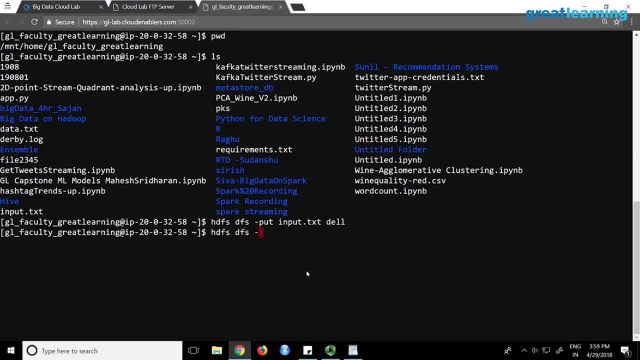 And then if you do an HDFS DFS hyphen LS in Dell, you should see the Sorry. Yeah, If you do an HDFS DFS Dell, you should see the file in Hadoop. So put is the command to upload the file. 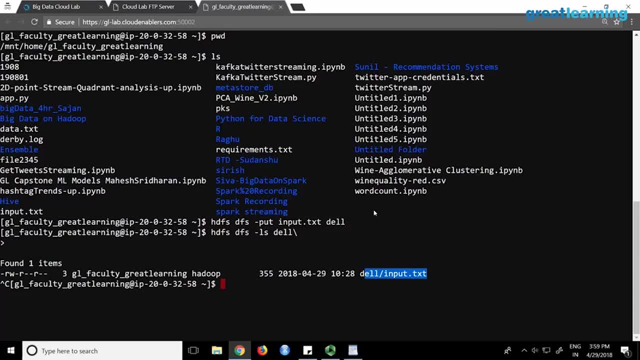 You say: put then the file name and then the folder name in Hadoop. Dell is the folder name in Hadoop. This is uploading command. You say: don't type this root This last. This came by mistake actually. 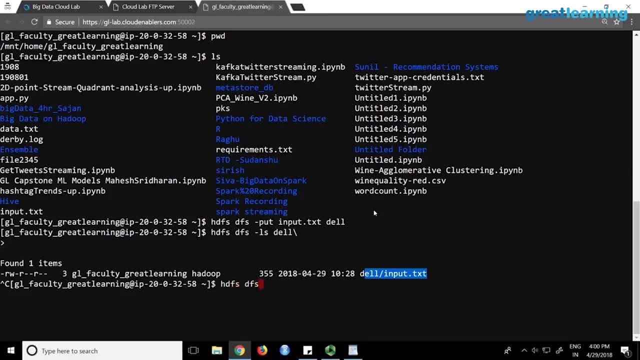 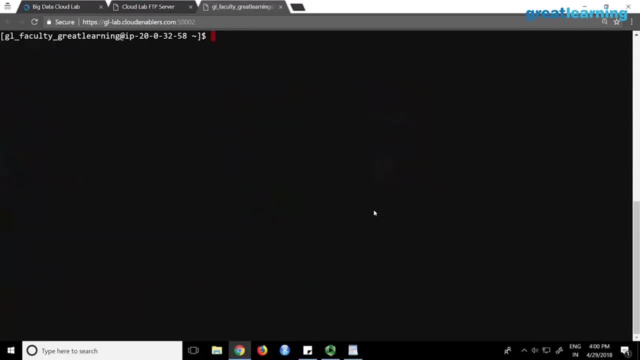 So to search the file HDFS, DFS, hyphen, LS, Dell- My folder is Dell, So it should see there. This is how the put command is. I'm doing an LS and inputtxt is here And this is how you type it. 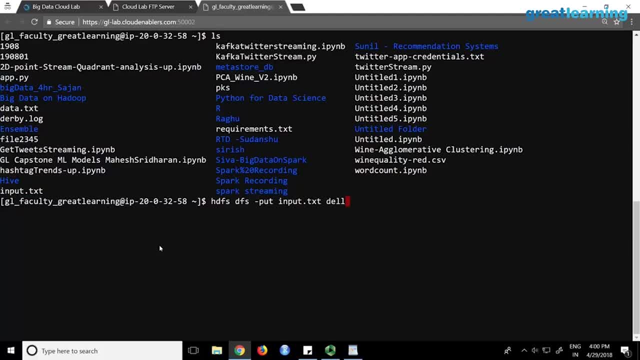 HDFS. DFS put file name source, destination folder in Hadoop, I know. So that is just to Clouder and Hortonworks. So these commercial distributions, by default if you do an LS, they'll go to your home directory and fetch all this. 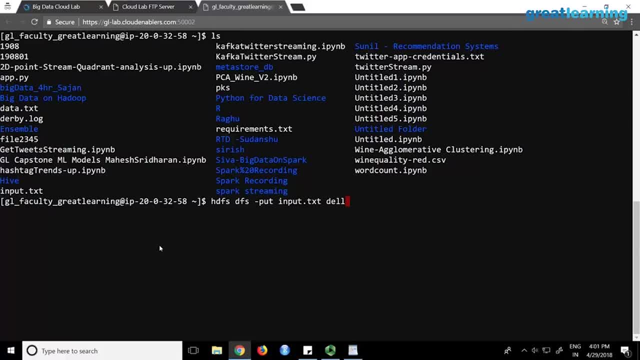 Actually it is appending the absolute path I'm showing you. So this DLL directory is created in your- what you say- user. User is the top Earlier. there is a root folder in HDFS, Then there is a user folder. 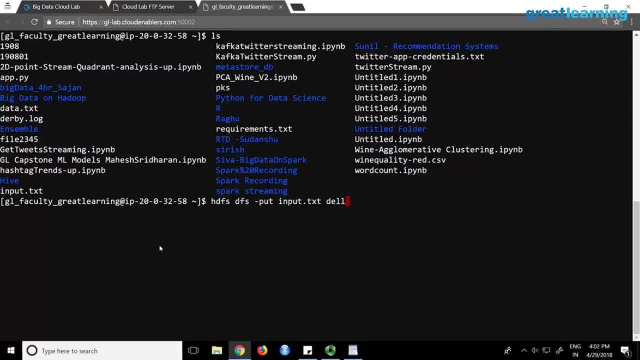 Within that you have to define the name of the home directory. Oh, that when you're creating a user it will define. You have to. So the administrator, when he's creating a user, he has to define that it is under user, this user name. 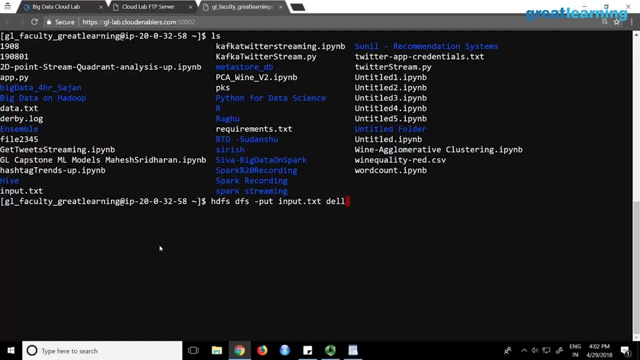 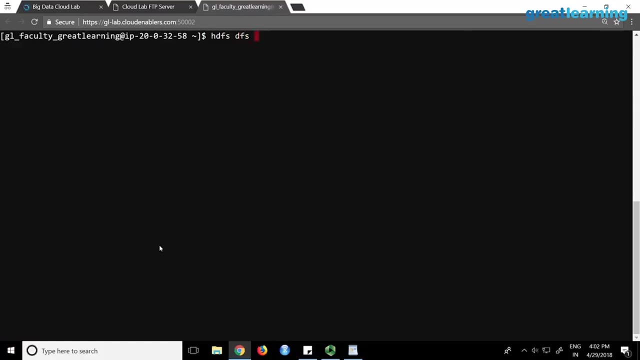 Like Linux, only Linux. if I'm adding a new user slash, home slash, come same Here. it is user. That is it? So all of you can see the file in Hadoop? If yes, you should be able to do this. 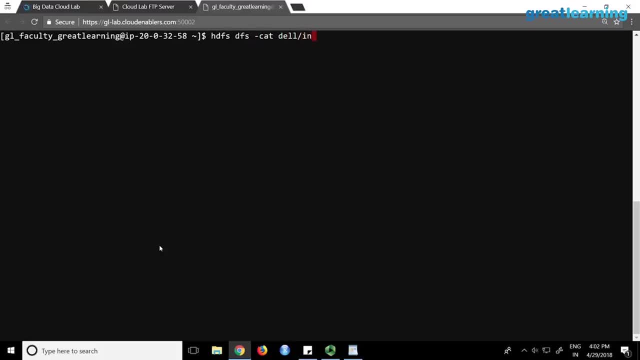 Cat, Can you try this? Change the folder name. Okay, My folder name is Dell. Your folder name will be something else. in Hadoop You are logging onto the client with the same username and password. The user accounts you are creating in Hadoop are synchronous with your Linux user accounts. 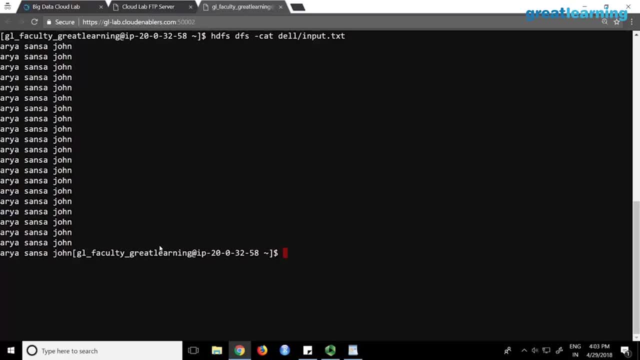 It actually takes your Linux username. If you can check, your Linux username and Hadoop username will be same, Almost same, right Same same. you are using Cat is like looking at the files concatenation. If you are installing Hadoop on Windows, it is a whole different story. 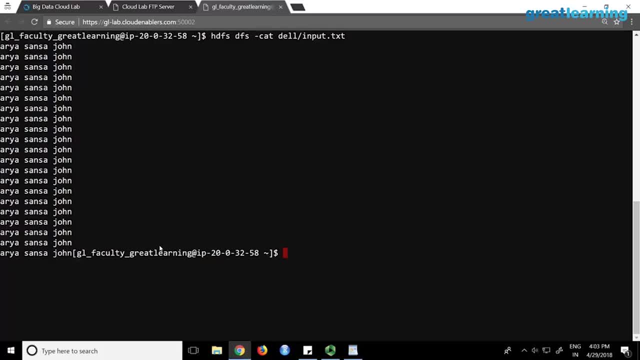 It is. Cloudera doesn't support- I think Hortonworks supports There- the user accounts and all are pretty different. Not like this, actually, But mostly we are seeing on Linux. actually, Your data is actually on Hadoop and you are just listing, I mean, the content of the file. 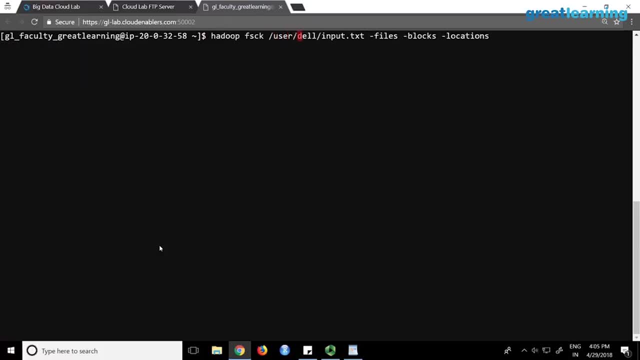 So that will be slash user slash. What is my username? GL underscore, No underscore. learning right, Great learning, Why they are keeping such a big name. Nobody is able to type it. actually. Eat this Hadoop. 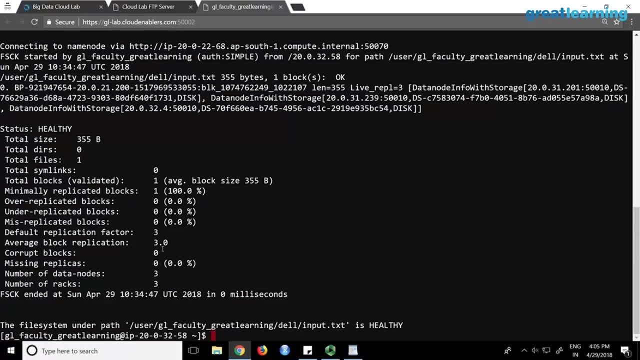 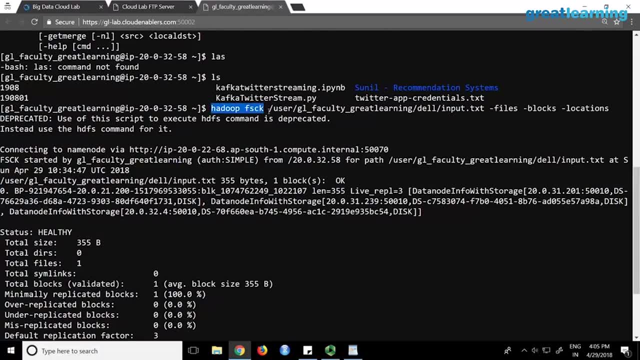 Yes, it works. Okay, so I will explain. then you can run. I ran a command. If you look at the command I ran, this is the command. Where is it? Hadoop fsck? Fsck is actually file system check command. 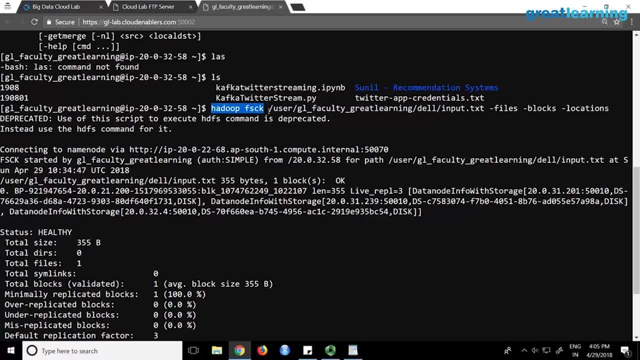 It is used to check whether your file system is healthy or not. But you can use this command in another way. I said run fsck on the file I uploaded, Complete absolute path. you are giving User GL faculty Dell input. 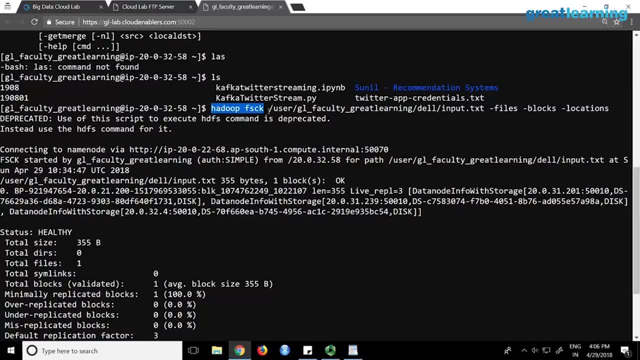 Then I am adding three arguments: Files, blocks, locations, Meaning: I want to know where is this file, How many blocks are there, Where are the locations? And what it shows me is very interesting. It says connecting to name node, since it is a Hadoop client. 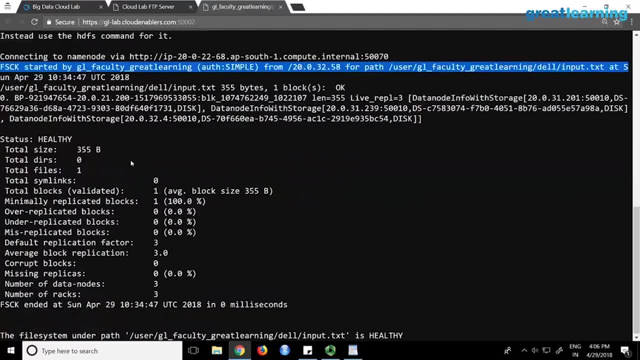 Right, It says fsck started and all You know interested in that. Look at here. See, these are your blocks. blk. It says length is 355.. This is internal to Hadoop Live. replicas are three, So there are three copies of it. 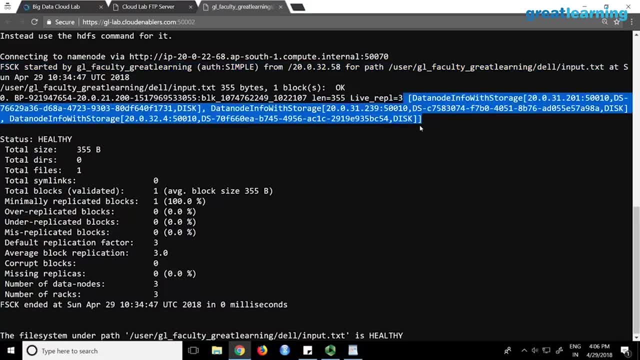 And these are the replicas: Data node info with storage. One of the machine is 20.0.31.2.0.1.. Another one is 20.0.31.2.39.. Another one is 20.0.32.4.. 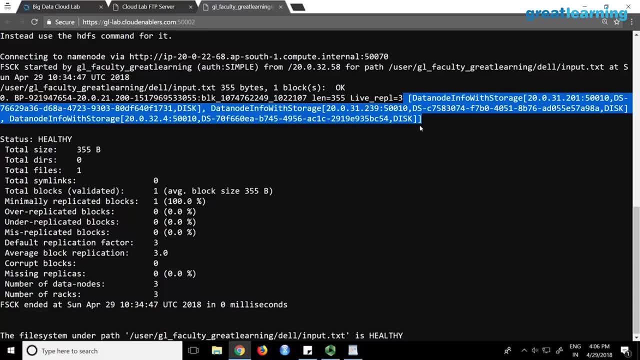 Three data nodes. Three data nodes, Three copies. So these are the data nodes which are holding a replica of your block. There will be only one block because small file, There is a data store. It's a format actually used by Hadoop. 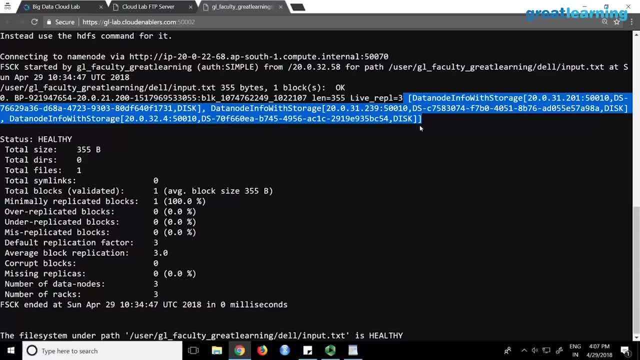 That are symbolic links created by Hadoop to that file. Those are internal to Hadoop, You don't have to bother. Number of data nodes: three. Number of racks: three. Yeah, Here it is keeping in three racks. Probably they have configured it in that. 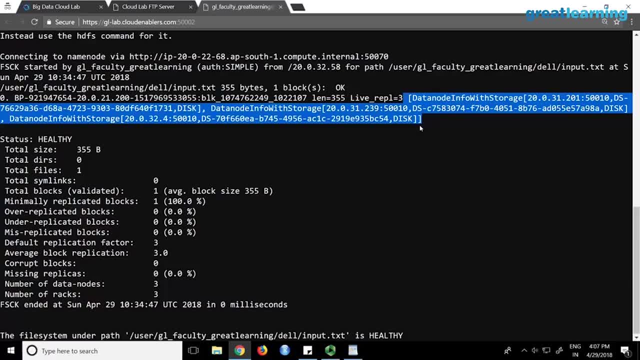 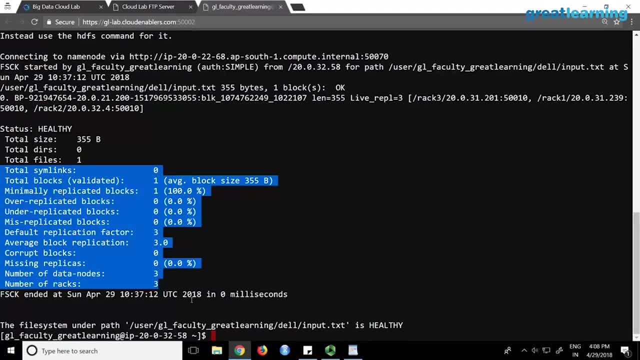 Rack awareness: we can configure. So this is like a lab setup only Right. So I can say: keep it in all three Production. we don't do that. ideally, Health is rack two, Right, Exactly, Yeah, So it is appended. 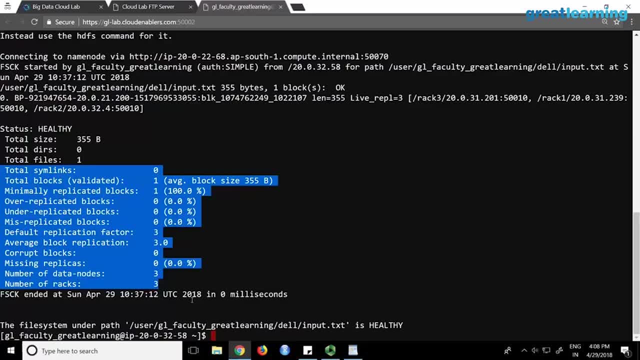 So it says: this is in rack three, That's in rack one, This is in rack two, So you can even see in which rack the data nodes are Right. Another interesting thing is: total file is one, Total blocks is one. Okay, 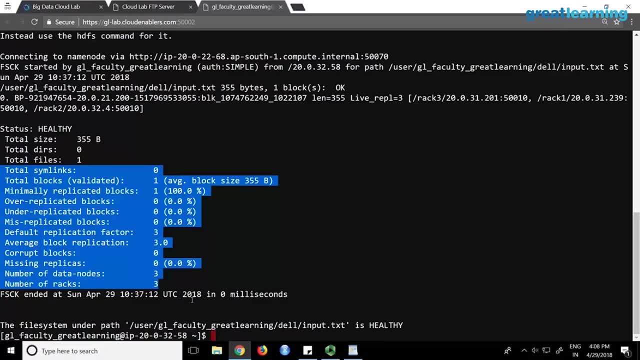 That's okay. Minimally replicated blocks: one Over replicated, under replicated. This is over replicated means I told you right, If a machine crashes it will create three And again, if it comes back again, it will be four copies. That is over replicated. 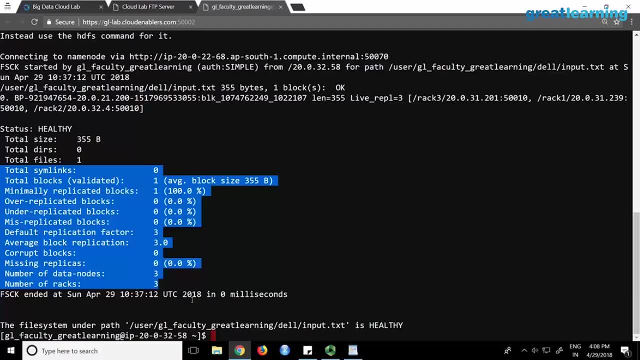 Under replicated means. if a machine crashed, immediately it will become two. Show that this is under replicated, Misreplicated. There is something called misreplication. Default replication factor is three. Average three. Current blocks: zero, Missing replicas: zero And there is something called a data node block scanner report. 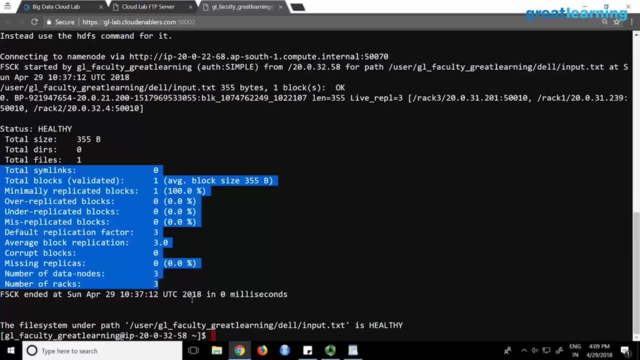 Every ten seconds, data node will send a report to name node. It will scan the blocks and send If there is any correct blocks or missing blocks. How does the name node know? Right? So data node has to tell the name node: Hey, one of the block is missing or correct. 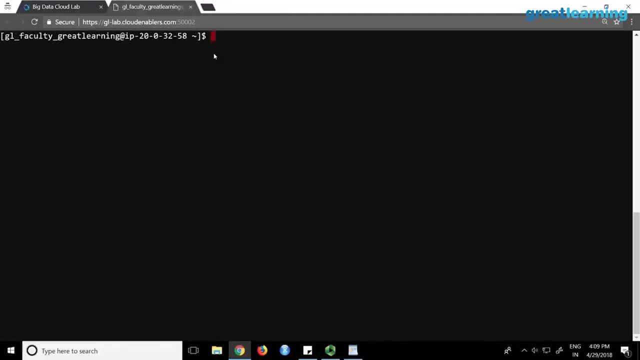 So this statistics will be sent to name node. Yeah, So anyway, this part is simply HDFS architecture and all That is. if your data node crashes and comes back online, Then you have four blocks. So now, another thing is that shared location. 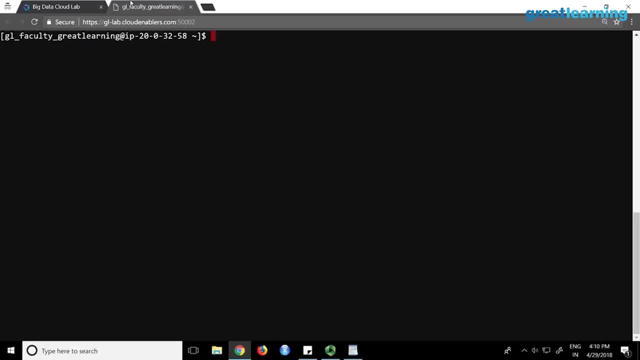 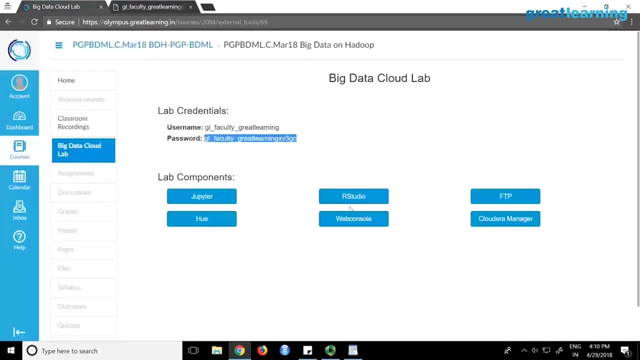 That shared location folder. So let's run the MapReduce program, Right, So? but I think we have to do one more thing. See, I created a folder called a del Right. Ideally, it will make sense if we have the same folder name. 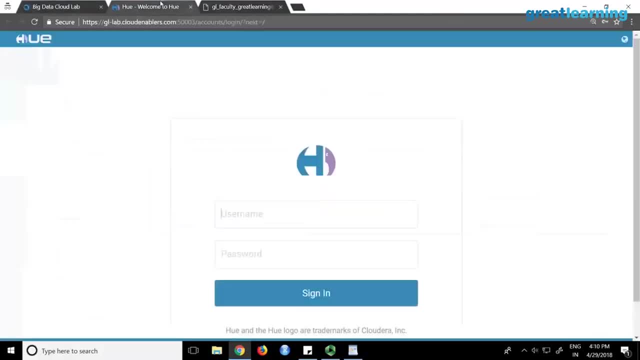 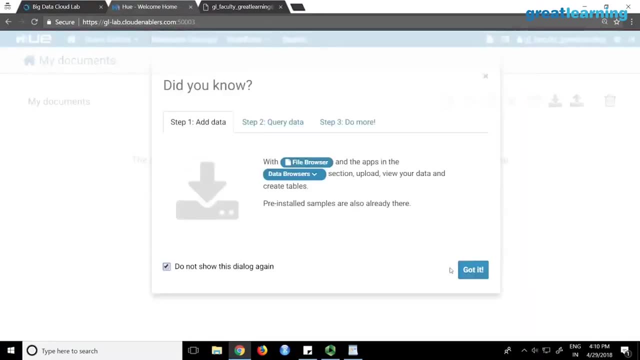 You could have created a folder with a different name, Right? I don't know what folder you created, So let's create a common folder. Otherwise, if I say this, you say this, then it's very difficult to troubleshoot, Right? So can you create one more folder? 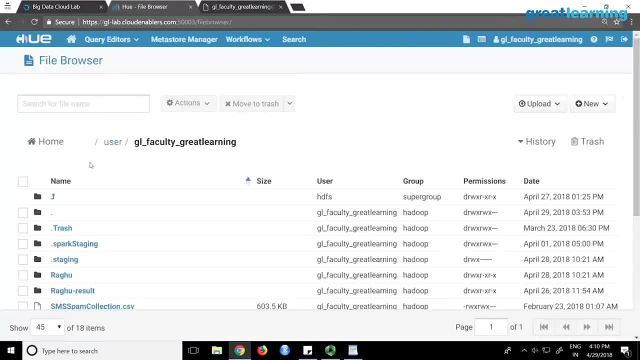 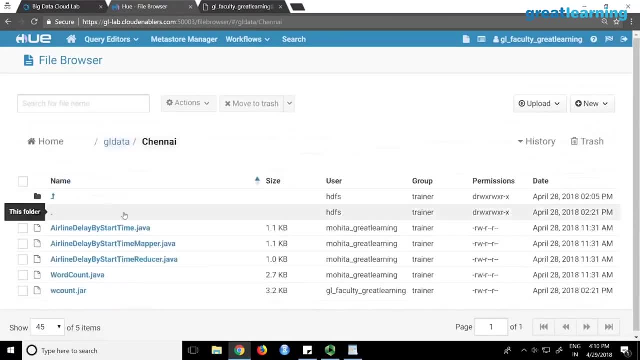 Do one thing: Create a folder called del. I have created del so that I can save some work Right. Create a folder called del. I am very lazy person. I don't want to create one more folder: HDFS, DFS, hyphen, mkdir, del. 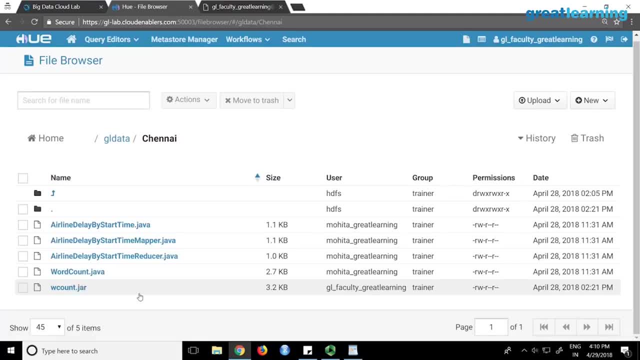 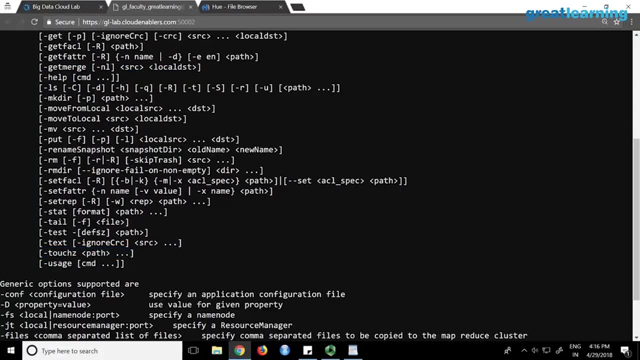 And then what you do: Upload the data Same way to this folder So that we are having the same. There is a touch command, Touch C, But we never do it Because there is no situation where you create a file on HDFS. 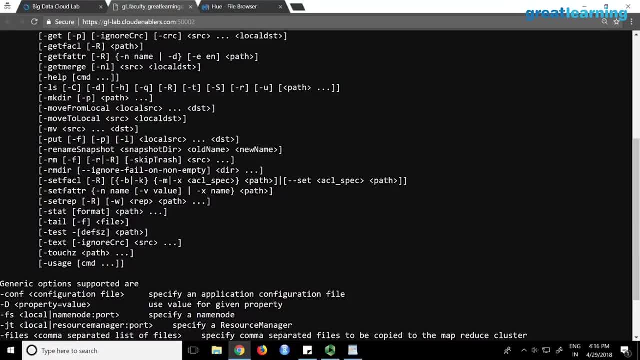 Because HDFS is a file system where you are dumping terabytes of data, So mostly you upload the data And then you create. See, if I am working on a normal laptop or desktop, I will create a text file and do something, But here it expects data to be in the order of GBs and TBs. 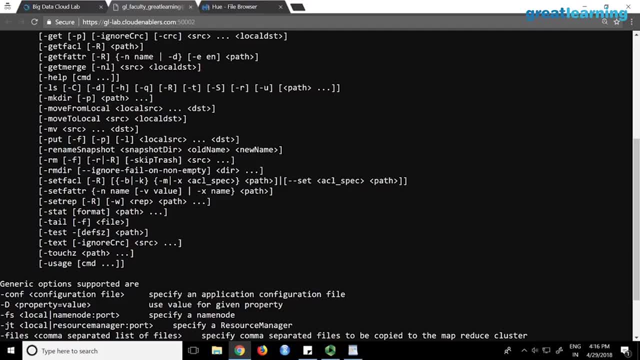 So very rarely There is a touch command- I think I have never tried it actually, I don't know actually the command also- But very rarely. we have created a file on Hadoop Right, So we upload the data normally, Right. 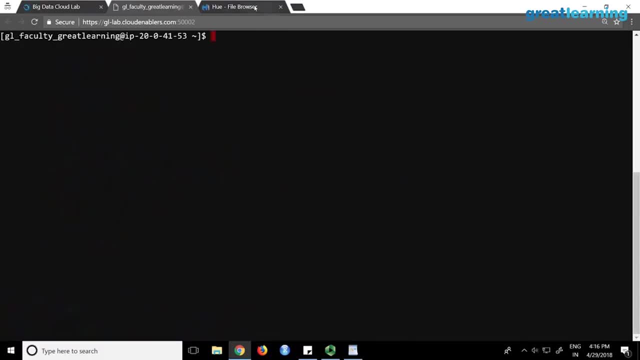 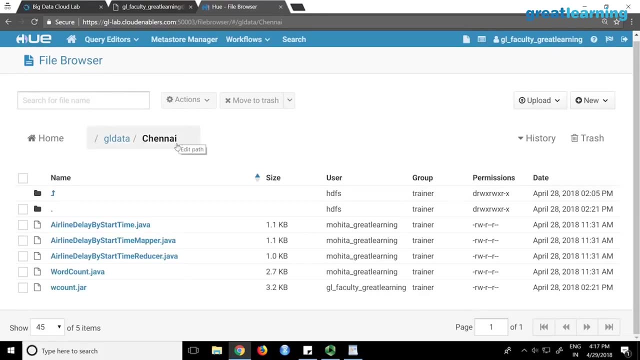 So we have created a file on Hadoop. Ok. Now I want you to do one thing. If you look at this folder in Hadoop, This is Hue, Ok, And there is a folder called GLData Chennai. It's a shared folder. 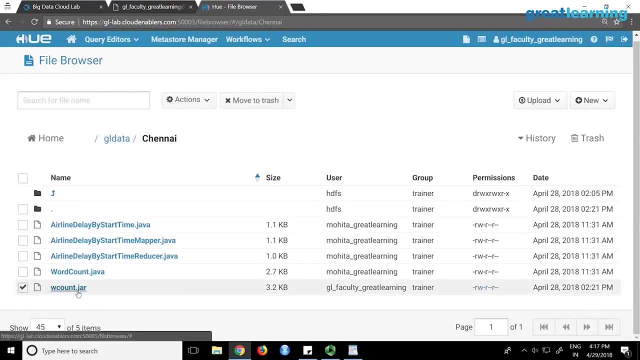 Here I have a file called wordcountjar. This is your program for wordcount. I have already written the program, Compiled it Created as a jar file. This is your wordcount program, MapReduce program. So this program you have to download on your gateway machine. 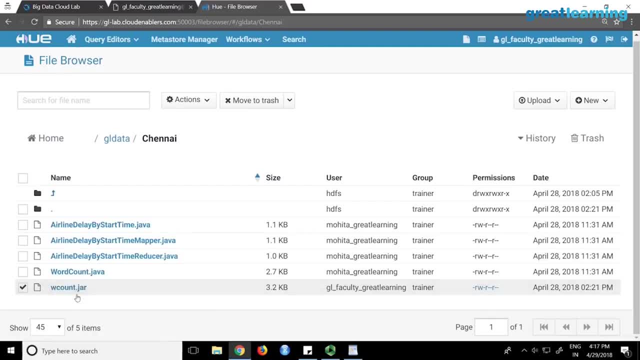 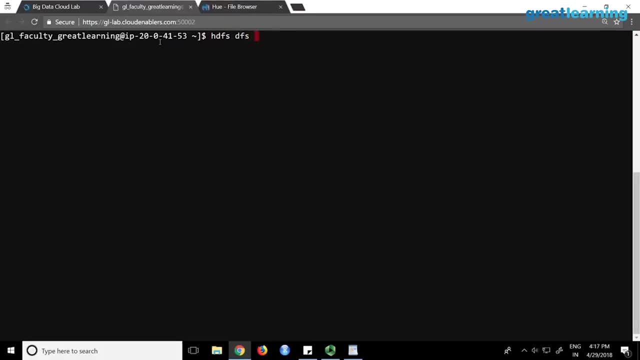 Linux machine. I will tell you how to do it Right, Because it is already in Hadoop. Location is GLData Chennai, So what you need to do- You have to say HDFS, DFS, hyphen, get, Get- is to download the data. 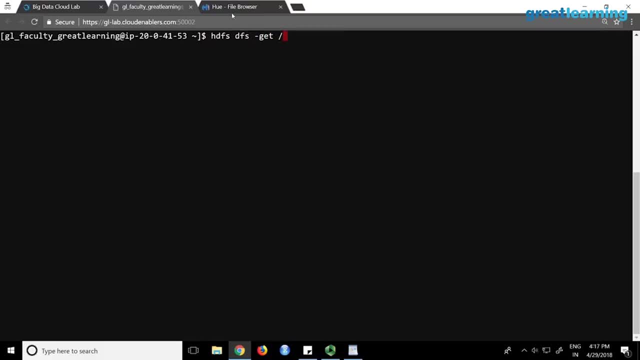 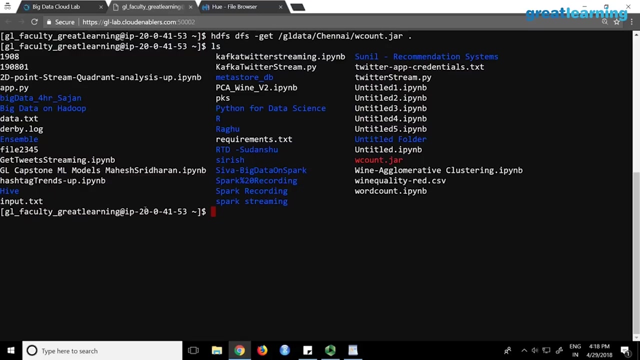 And where is the path? It is GLData Chennai. I will say GLData slash Chennai, slash wordcount dot, jar And you say dot Ok. Dot means current directory And if I do an ls I should see the file somewhere. 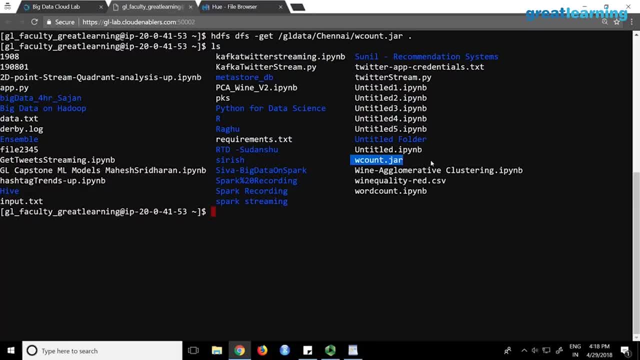 Yeah, Wordcount dot jar. So, in order to upload a file to Hadoop, You will say HDFS DFS hyphen. put To download, you will say HDFS DFS hyphen. get Another thing If this command fails. If this command fails. 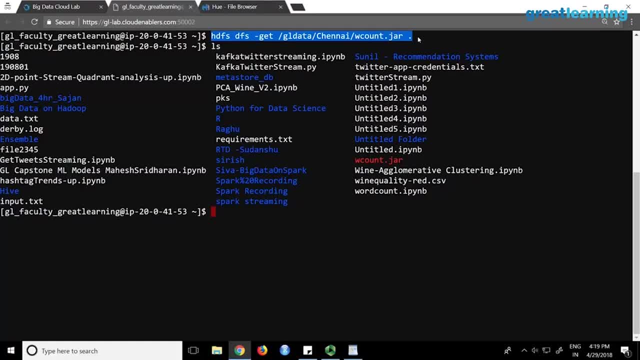 It will throw an error. I cannot find the file or something. If it runs means you got the file. Non Linux people: There is a dot at the end. That means your current directory. You are downloading into current directory. This is to non Linux people. 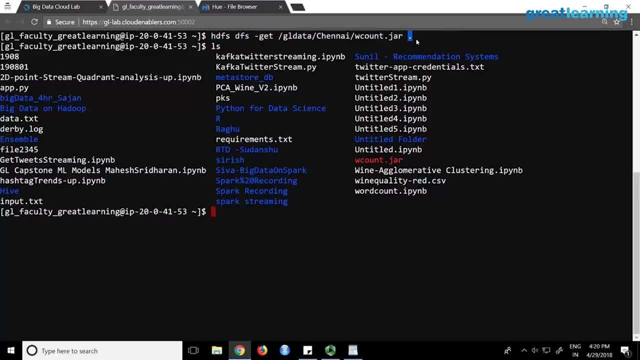 There is a dot at the end. Another very important point: Your HDFS is a file system on top of Linux. HDFS is a file system on top of your Linux file system. So easily you will get confused Whether my data is in Linux or Hadoop. 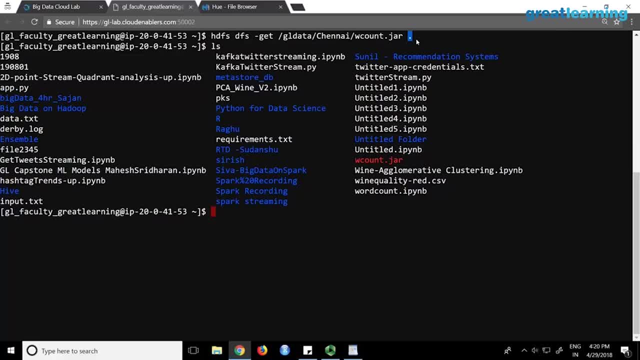 You know Hadoop or Linux, Right. So now this wordcount program is available in Linux. This is in Linux, Ok, So when you want to run a MapReduce program, The program has to be in Linux, Not in Hadoop. 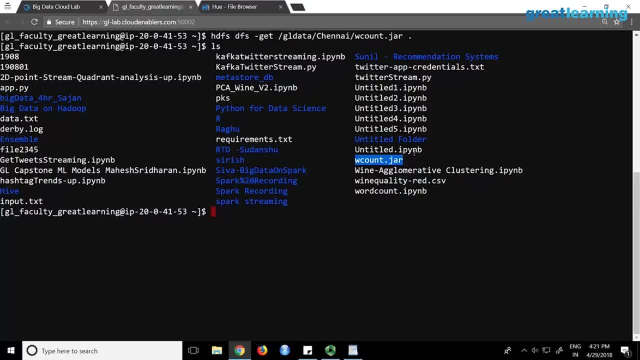 Data should be in Hadoop. The program should be in Linux. Ok, So many people get confused Because they will upload the jar file to Hadoop Right. Then it will not work Because the jar file has to be here. That is the same thing I am saying. 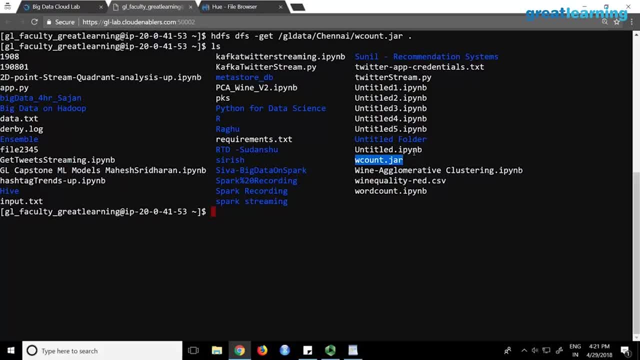 So please make this very clear. You have two file systems. One is called Linux, Another is called HDFS. HDFS is running on top of Linux. All your data will be in HDFS. So the Dell folder, your inputtxt, everything is there. 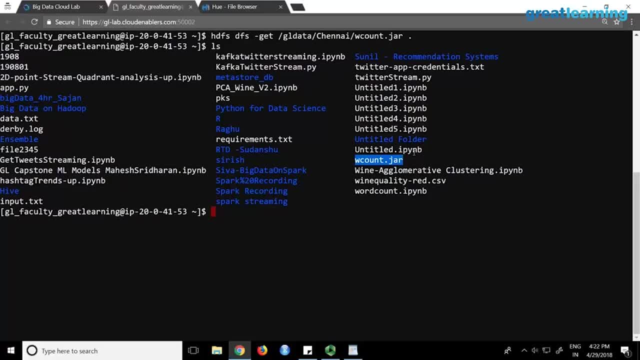 The program, the code should be on Linux And while running it will stream the code to Hadoop. That is a different story, But the code has to be on local file system, Right? So I mean, it is very easy to get confused. 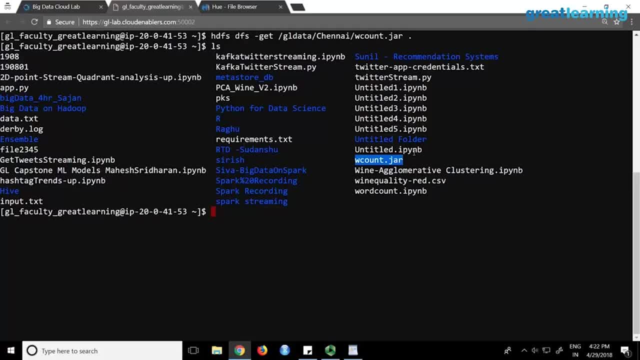 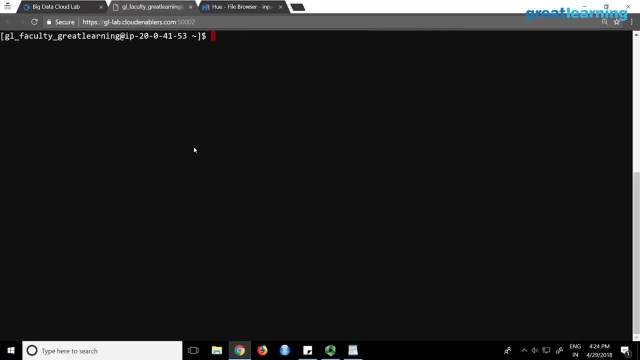 Even I used to do it long back Right So now we want to run the code, Right So I want to analyze the data. You can run hive queries, big scripts, MapReduce programs, everything from Hue. But the problem is it is a GUI. 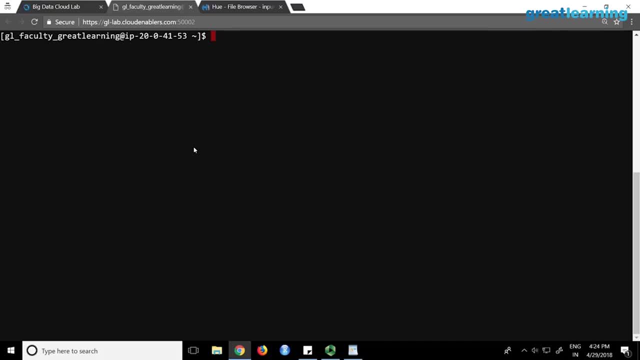 Since it is a GUI, companies actually don't like. It is like giving over permission. People will mess up A lot. GUI graphical user interface is always less secure than the command line. Actually, Right, You will also have restrictions. 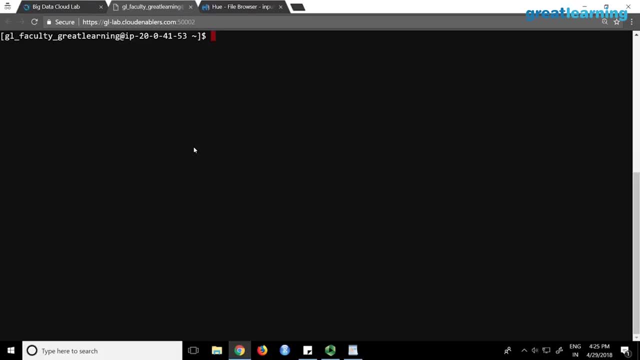 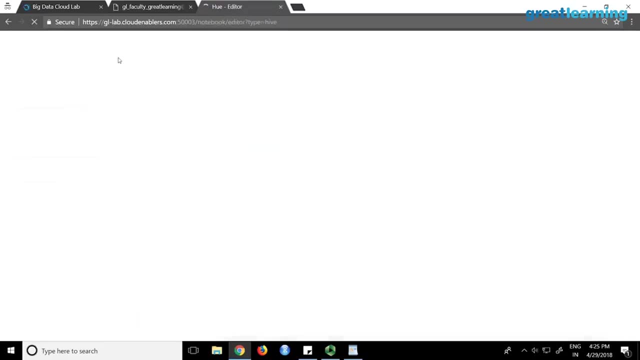 But so if I look at my Hue, I mean you can also do that. If you look at the Hue, you will have a lot of options here, For example query editors. there is Hive. So if I go to Hive query editor I can run a SQL query here. 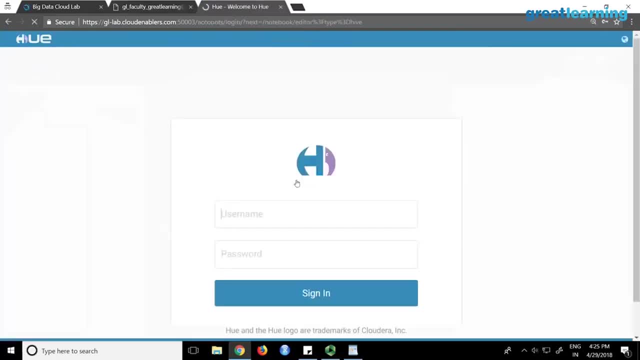 Let me just show you See, Reload this page One moment. Okay, So I can see that it is being inspired Why it is taking this much time. Yeah, So I see you can query the data from Hive here. You can create tables, query the data. 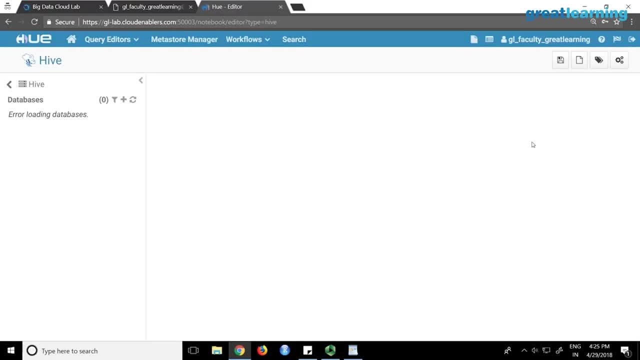 You can do all those things, But I don't know. Companies do not give access normally For learning purpose. it is good, actually Very easy to learn, But here also auditing can be enabled. Hue supports auditing, So Hue can send all this login information to CloudARAM. 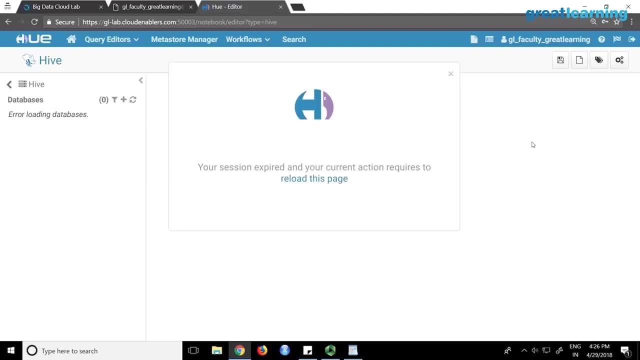 It cannot be audited. But I don't know People don't use it. I don't know why. I have seen some companies using Okay, Because another advantage is that if you have Hue, you don't need web console. Right. 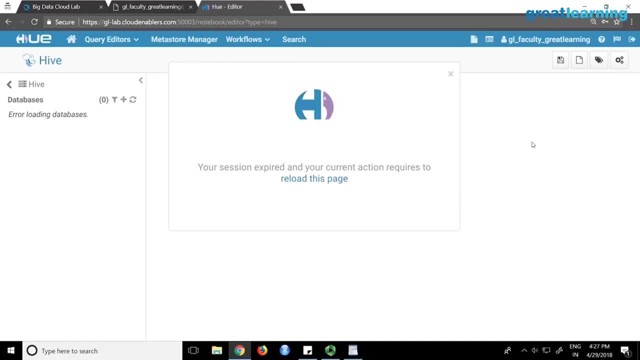 All I need is a browser. If I have to catch all this, then I have to catch all the web activity. Probably that is the reason people are not using it, But it is very user-friendly. actually, I have seen a couple of companies actually using Hue. 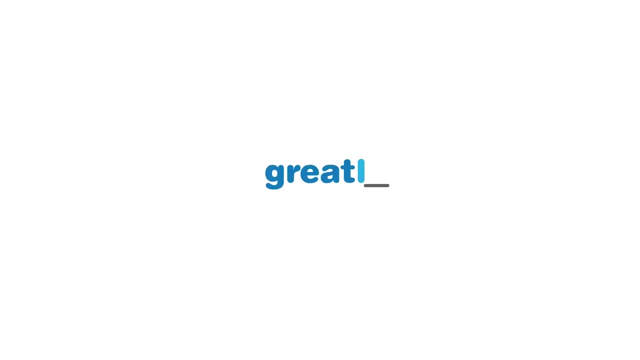 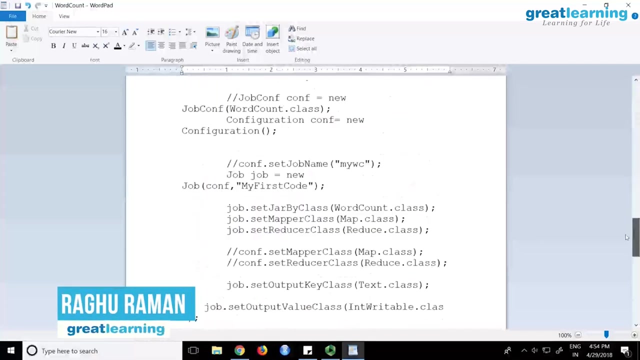 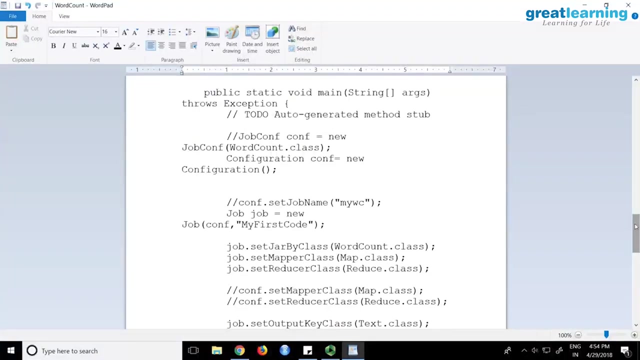 But they are small companies, not like very large organizations. So this is the word count program. This whole code is word count program And what you need to understand is that the MapReduce program has three parts. One is the mapper side mapper part, where the mapper logic will be written. 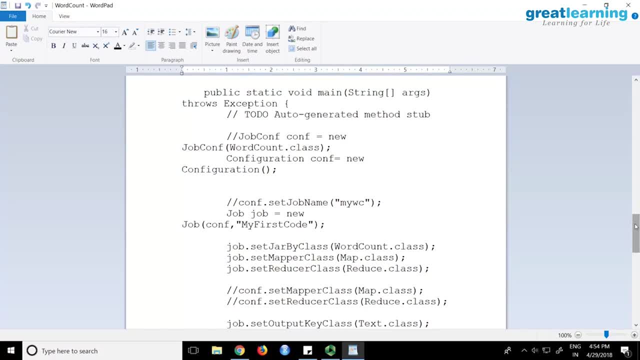 Second is the reducer part, where the reducer logic is there. Third is called driver. You know what is a driver, So driver is the part of the program which controls the program execution. Like what type of file you have the main method and all will come in the driver. 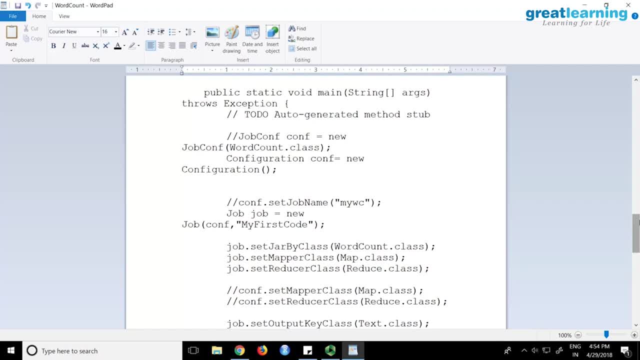 This is my driver- See Java people. So I have my main method here. So this is the main method. Driver will have the main method, Right? So this is my public static void main string argument. So this is a regular boiler plate code you write in Java for main method. 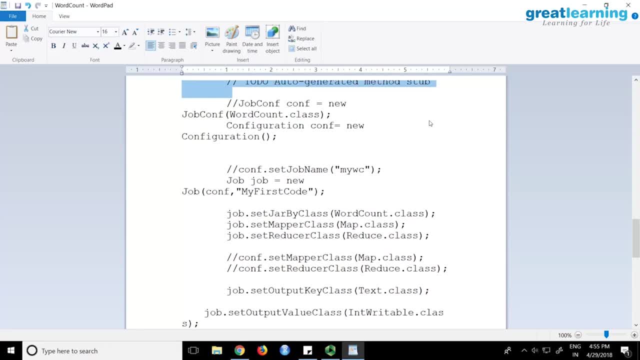 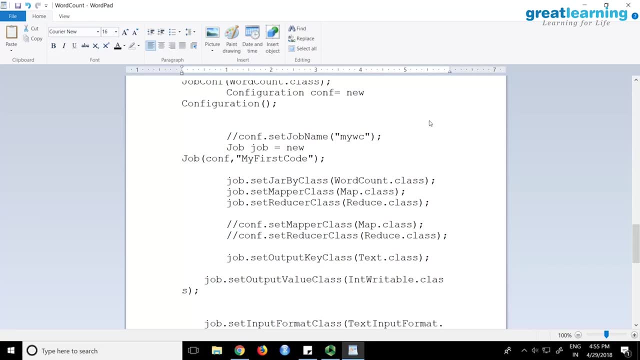 Then what is interesting here is that this one I have commented- You have to create something called a configuration object. So I am instantiating a new configuration object. What is this configuration object? See, if I submit a program to a Hadoop cluster, look at the possibility. 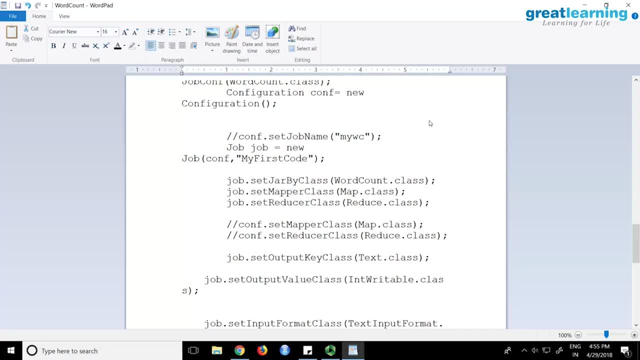 I created a program. Does that mean this program can be submitted only to one Hadoop cluster? No, I can submit to any Hadoop cluster wherever I have the data. So when the program gets submitted to the Hadoop cluster, it should know where is the name. node running, yarn running. 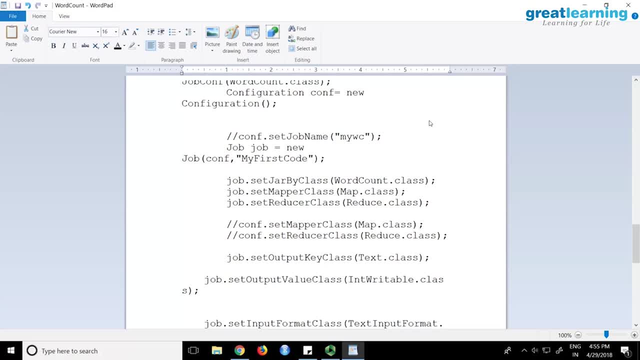 It should understand the cluster configuration That will be read by this configuration object Automatically. So Hadoop configuration is actually stored in a set of XML files. I will show you that. So this part of the code in your driver will go and read your Hadoop configuration, whichever cluster you are submitting. 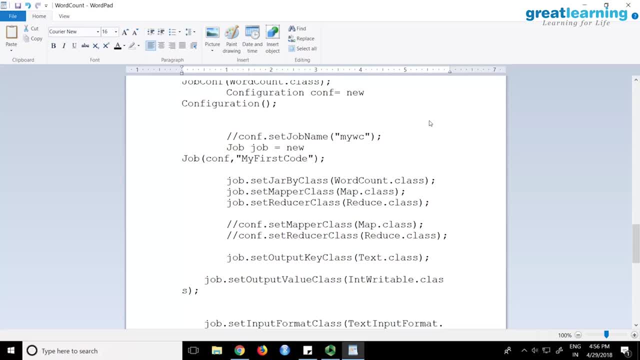 And understand the cluster configuration, Like where is the name, node running and all these details. So this configuration object is used to read your cluster's configuration And then you have to create something called a job object. So I am saying that new job object. 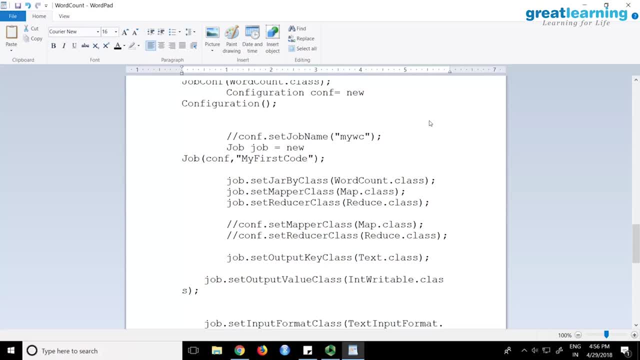 I am creating a job object, I am passing the configuration, I am also giving a name for my program, My first code. Any name you can give Doesn't matter. So this job object is responsible for actually running your program. Okay, 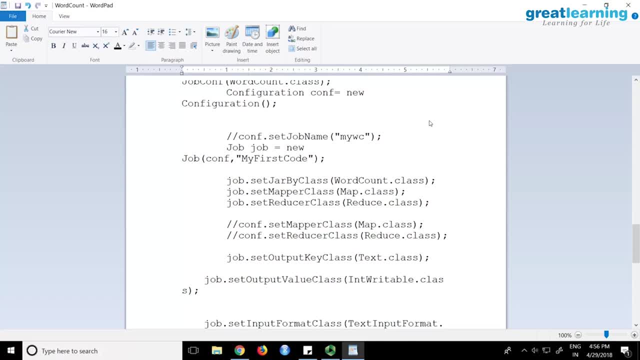 And this job object has some setters. You are aware of getters and setters, right? So here I am setting the mapper class, Map dot class. So the mapper logic will be written as a Java class And the name of my class is map dot class. 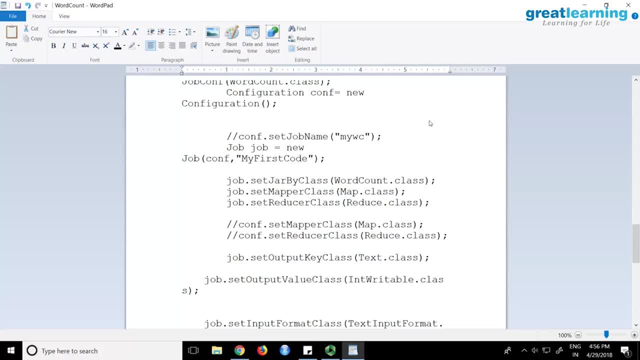 I will show you that. So I will say that job: dot set mapper class. map dot class. Set reducer class, reduce dot class. I will also say: set jar by class, word count dot class. This is my public class Which I define. So in this job object you have to tell. 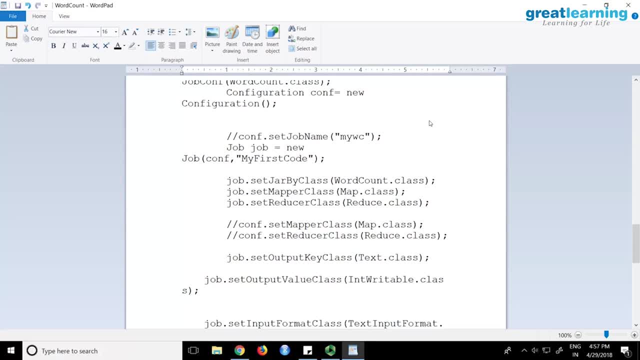 This is how you are telling in the map reduce, Which is your mapper? Which is your reducer? If I have a partitioner, I will say set partitioner class. This is my partitioner. So here I am doing the settings, Okay. 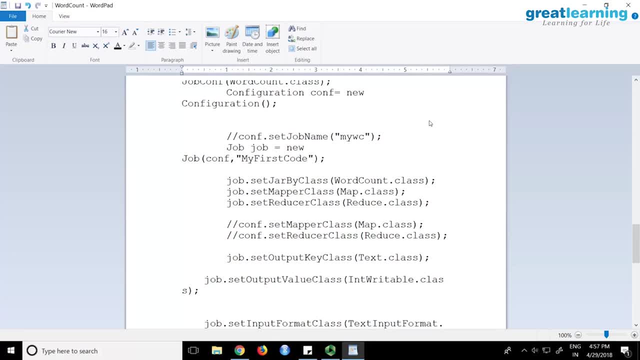 And this is commented. Look at here: Set output key class. output value class. So what is going to happen? What will be the output of word count? There will be a word and count, Say, for example, aria 9.. So aria will be the key. 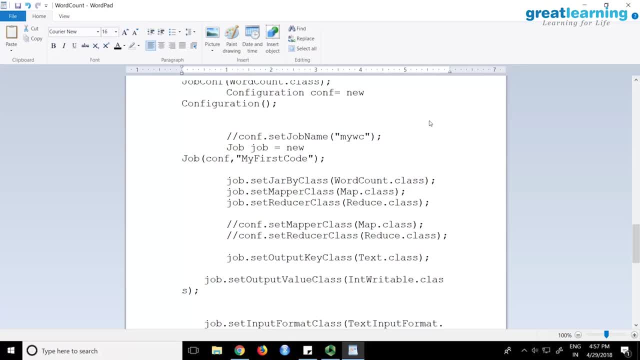 9 will be the value, And aria is ideally a string. I told you, for we don't use string, So I am saying that the key we are using a class called text. This is the wrapper class: Text dot class. I will import it in my java. 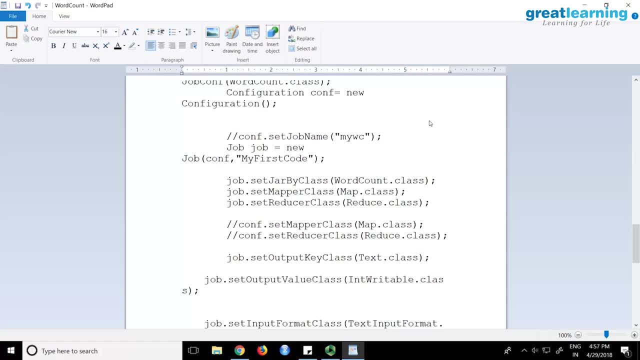 So this is the wrapper class for my key, Because my string String is represented as text And value is interwritable. This is again another wrapper. So in the driver part of the code You have to mention all these things. What is the data type of your key? 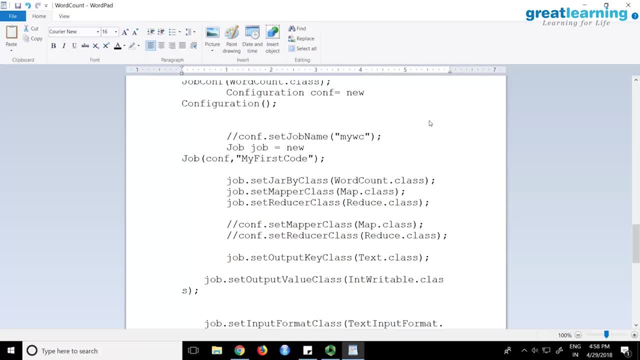 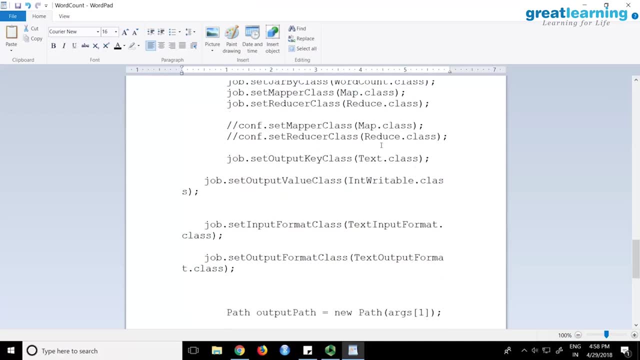 Value, Which is your mapper, class, Reducer, class Configuration, All these things you have to mention. Plus, You will also have Input format class And output format class. I told you that I will explain about this, So the question is that. 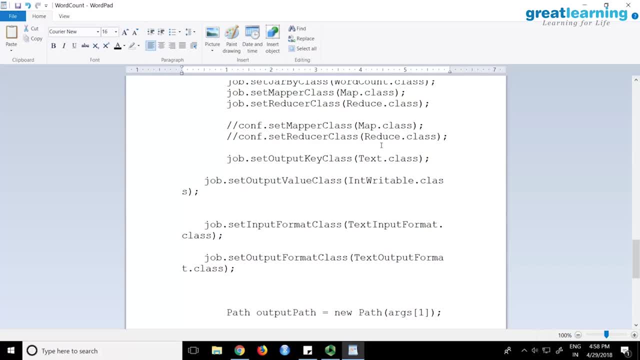 How do you read a different type of data, Right? So there is an abstract class called a file format And that abstract class, Or the parent class, Has multiple child classes To read a different type of files And the most commonly used child class. 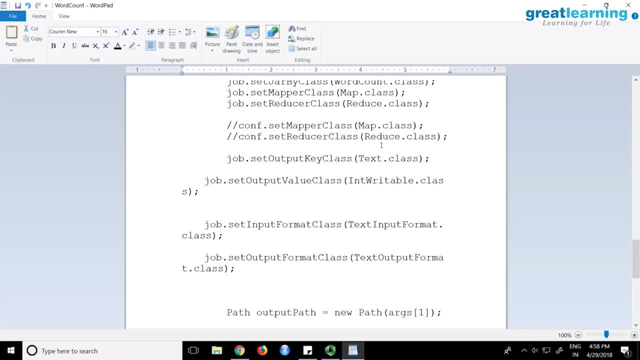 Is input file, Text text input class. now we have worked with text input class. there is xml. if it is xml, look at your root tag and row tag and extract. you know there is text, there is xml. there is key value input, there is something called sequence file input and then there is binary. understand this? 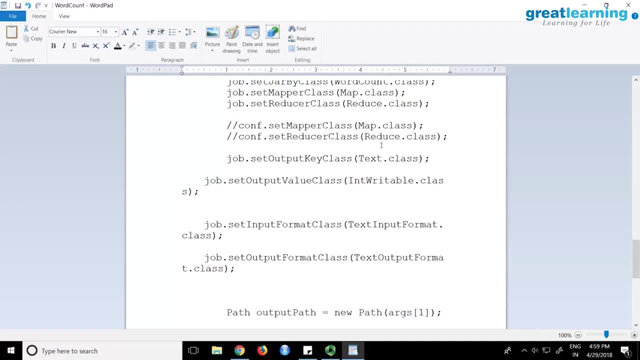 if i'm having image files and all i cannot directly process- see look at the philosophy of map reduce. how can i say an image is a key and value? not possible, right? so first i will convert those images into binary file. then there is a class called binary class, which will understand. 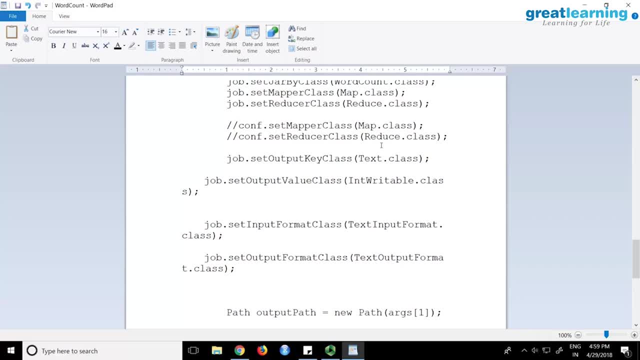 binary data and read it, so that class i have to call to read those files. i cannot directly process my images or anything. normally if you store an image and read it, okay, it is a dot jpeg extension of something. right, you can't process that, that extension. you cannot process dot. then 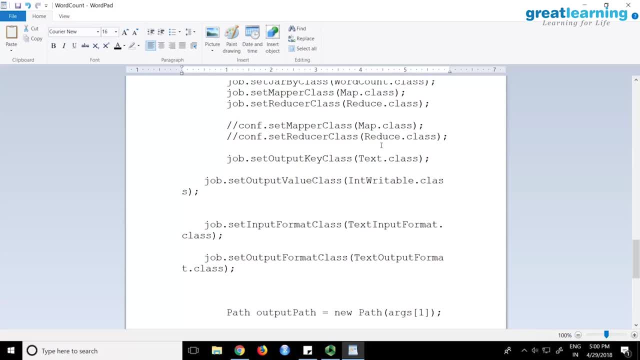 what you have: jpeg and g5 for a bitmap, so they will have their own encoding. you can't process it actually. that's what the output is, always key value pair that you can mention what format. here i'm saying it is text. even in the mapper you're producing key value pair, so mapper is the guy who first produced the. 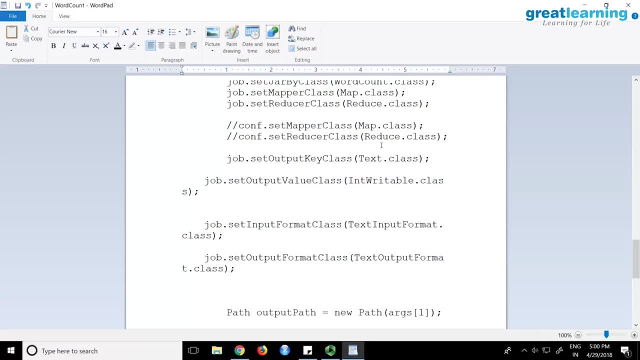 key and value and mapper's output is word comma one. what is that word? it is string. i don't use string, i say that word is text. right, i will say output, key, output, value. this means the final output only. but even in the mapper output this is same applied whatever key and value you want to use. 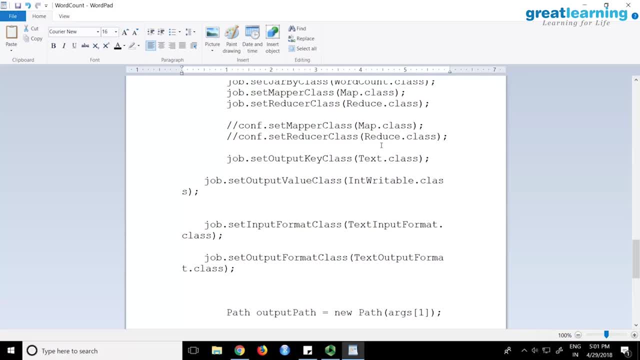 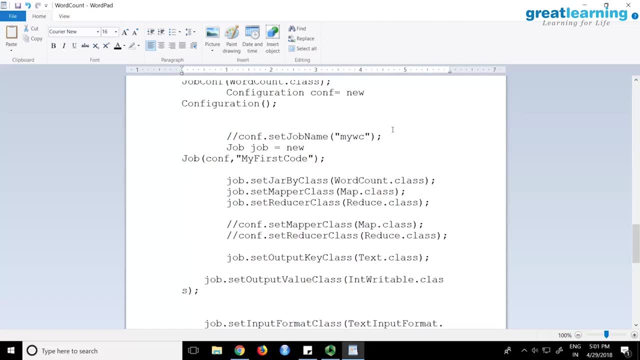 and this is my input format and output format to read. this execution has nothing to do with edge node. the execution is handled by somebody called yarn. driver program will go to the cluster. right now your entire code is on linux, that's jar file. when i say run, it will read and push. 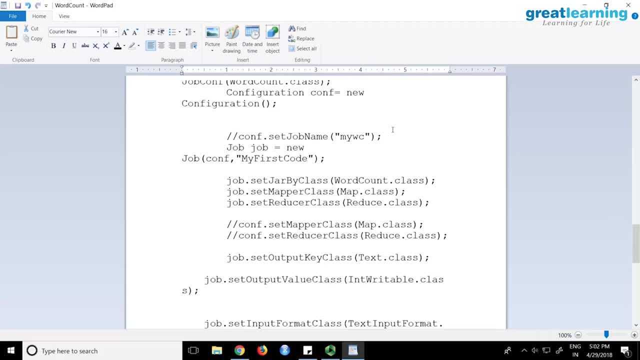 to the cluster. it will go to the cluster on data nodes. only the program will run any anyone can run. i mean it doesn't have any importance, but you can track where it is running. i will show you once you run this. i will show you where your mapper ran, where your reducer ran. 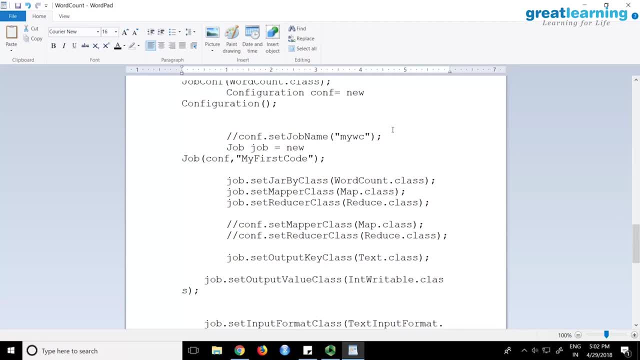 there were developers who were integrating that also rather than manually setting right. yes, that is possible. this is a very simple program also, like here, i can manually set, doesn't matter- also the uh variables, what you say, uh, private, public properties and all it might be a concern. 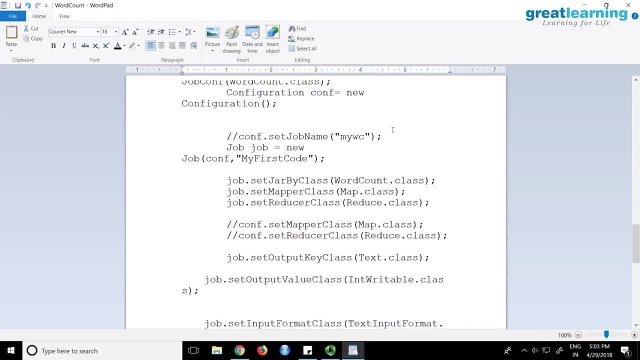 right sometimes. so here i'm simply doing a set, i'm not doing anything else. spring can be integrated normally, but again coming to the point, right now nobody does, because nobody want to write a map at all. right, because it's very obsolete actually. one more point i want to tell you is that if the 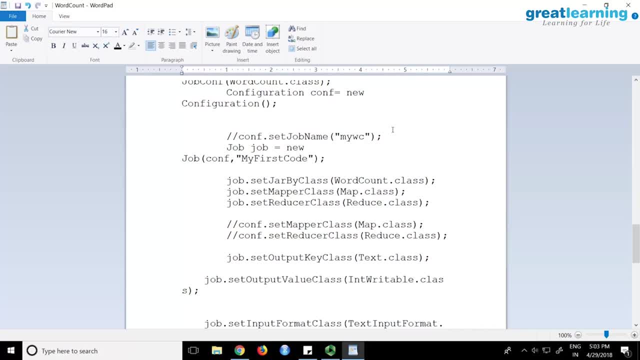 cluster administrator wants, he can decide how many reducer should run, meaning by default. if you simply install hadoop, there is only one reducer which will be called for every program. a developer in a program can say: i want five, you will get five in my program. i have not written anything. 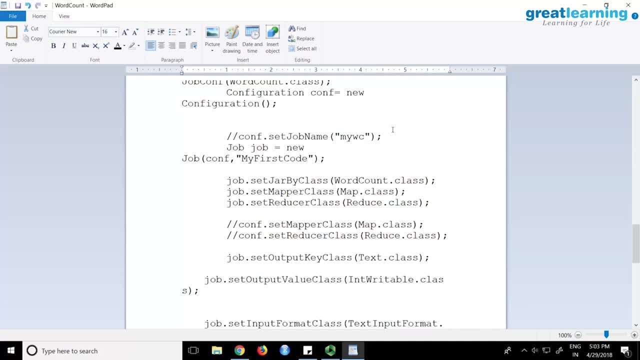 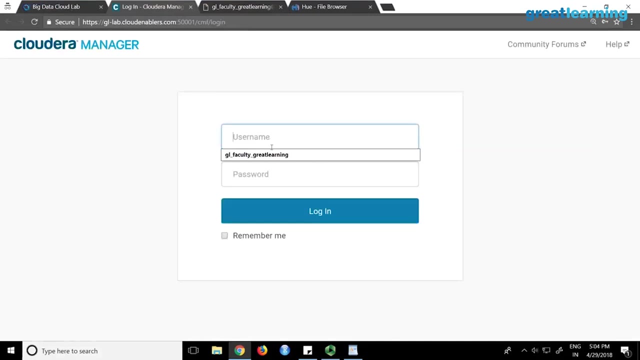 so ideally it should run with one reducer. but in my cloudera cluster the administrator has said any map reduce program runs by default. you will get three reducers in the cloudera. i mean, i don't know who set it. i asked it to change because if you just go to this cloudera manager, let's login and where you set it, you set it in. 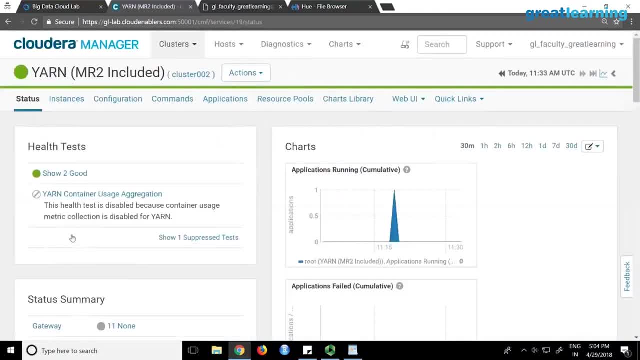 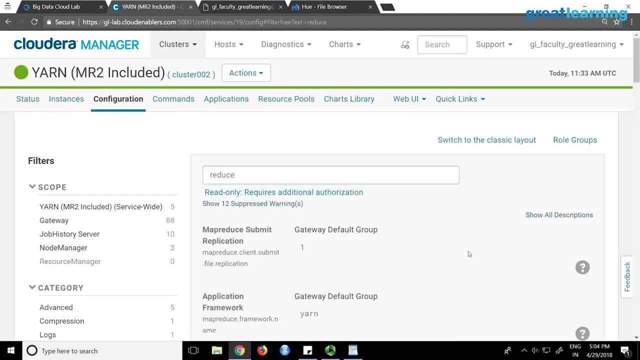 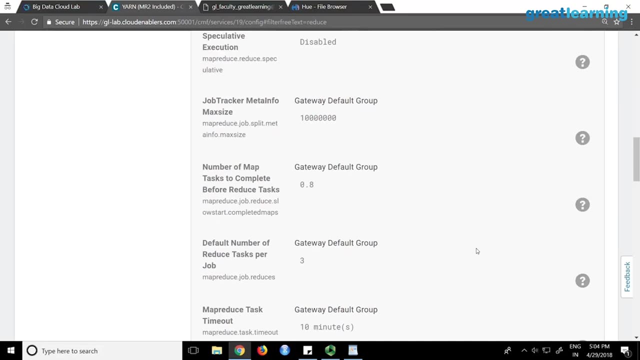 yarn. if i go to yarn, this is yarn, okay. i go to configuration of yarn and if i simply search for reduce, this is how it will run. read, read, read any map reduce program you run three reducers will kick in. that is useless. probably the reason is that the administrator might be believing that you will submit huge. 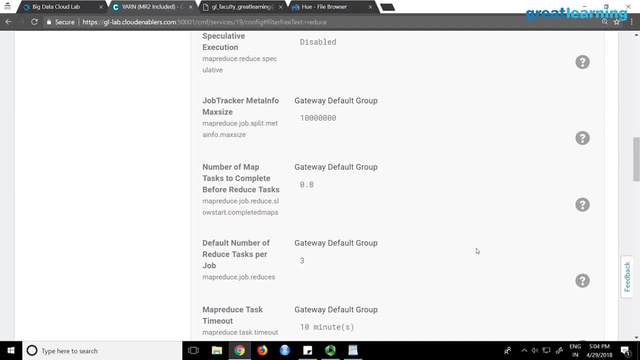 map reduce programs with, without mentioning the number of reducers, at least three can run, so it is easy to handle the load right. so in my application i did not write anything, so this will run three, because we are doing simple word count doesn't make any sense, but three will run. yeah, in the 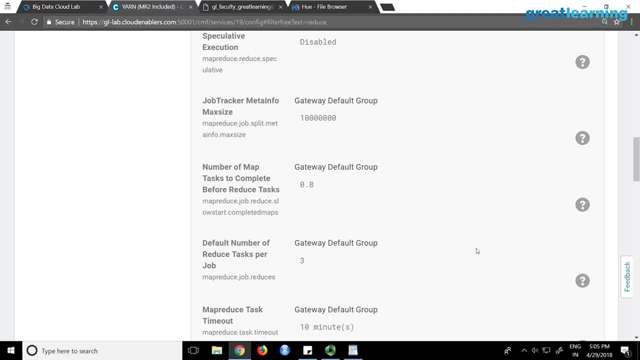 code you can override. i'll show you a different code. in the next class we will run a airline delay program. now the point is i actually wanted to run that program, this class, but when we ran we ended up in an error. the problem is that that data is 700 mb input file, so when i uploaded into 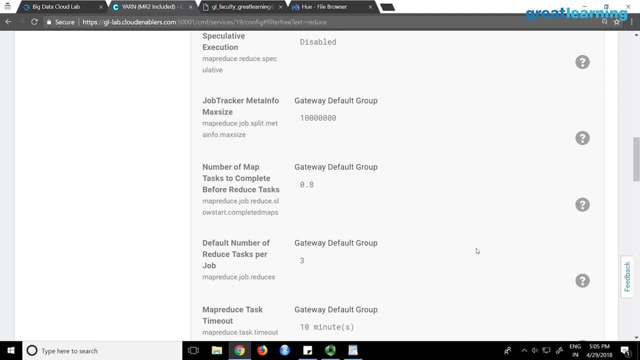 hadoop it became 1.5 gb and when i ran the program it crossed the quota limit and the program didn't run. everything is fine, but we have some restrictions so i didn't check it. also. i thought it will run, just so. i talked to them and great learning said: we will fix it in the next class. 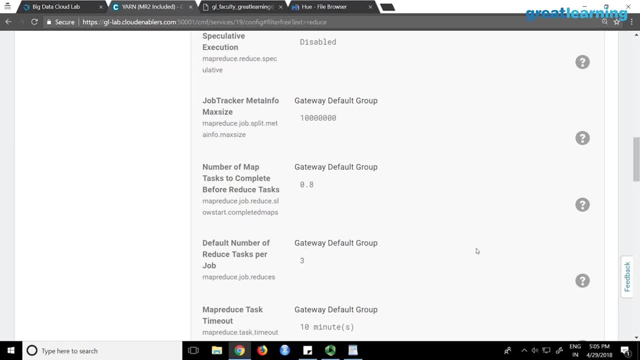 so when i'm running that what you say- airline analysis map, reduce program- i will show you how you can manually ask for reducers like you want: four, five, six, how many you want you can ask in your program, i'll show you that. so i think this part is clear. our driver part is also clear, clear. 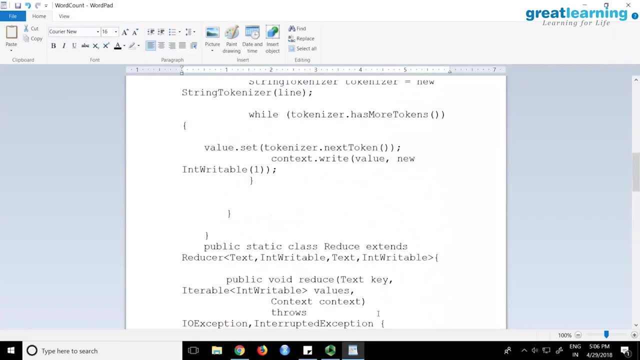 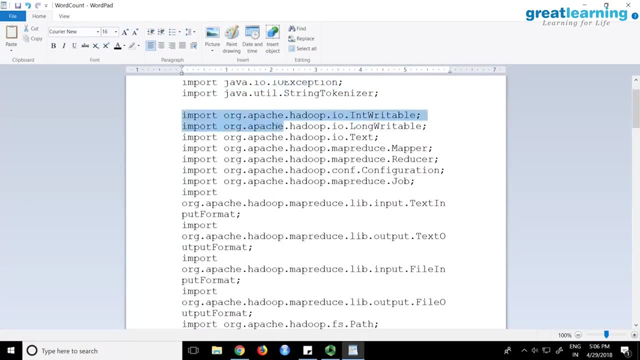 at least whatever we are discussing. you and somebody was asking about imports. this is the imports, so these are normal java imports. and look at here: import apache, hadoop io in writable, long, writable text, so this is integer long and string corresponding data types. okay, wrapper classes and i'm also importing map reduce. 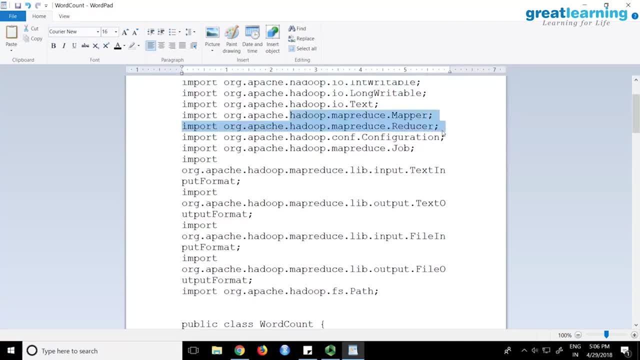 dot, mapper, reducer. why? because mapper and reducer are classes which you will inherit. if you're writing a mapper logic, you don't write it from scratch, you will extend it. you will already have a class where you can just extend it and write it okay. so that is why i'm importing these classes. this is the 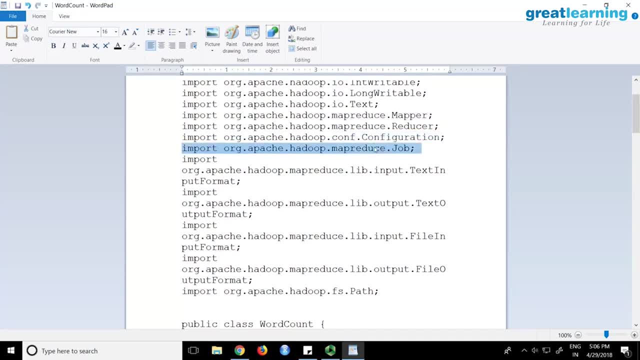 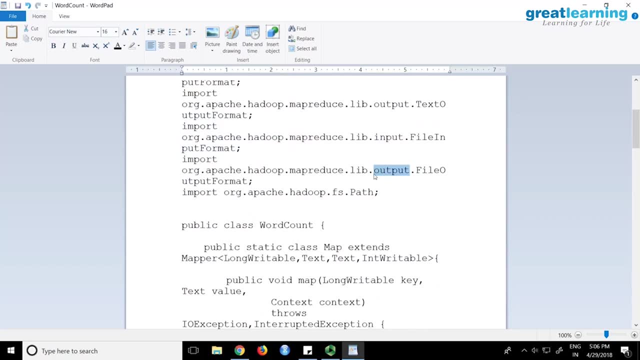 configuration object we created and this is a job object. this is a text input format. uh. text output format. file input format is the abstract class. okay, file output format. fs dot path is used to read the data input data. so these many imports are there standard imports, most of the programs. 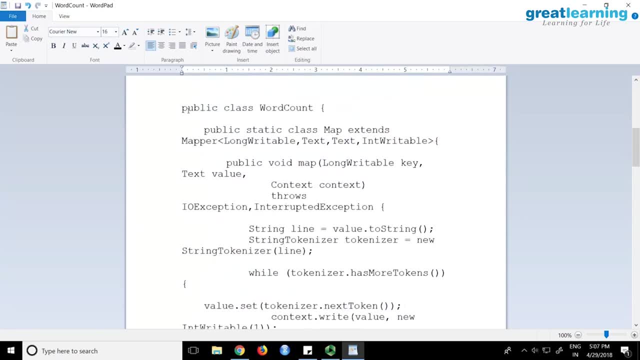 will have these imports. and here is your public class word count. so this is where your program starts. right, i'm in the public class. now i create a class called a map. this is my mapper, which extends mapper because, uh, you know, mapper is your base class, right? i will tell you what is this. 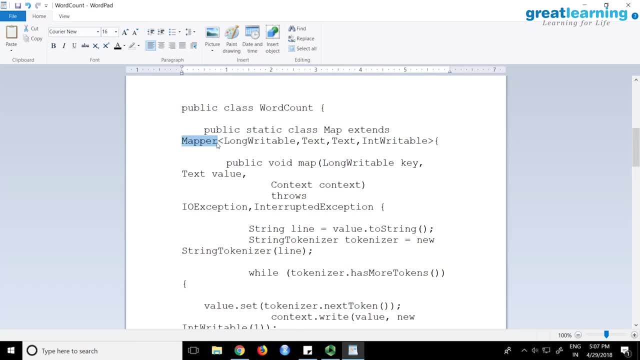 okay, i'll tell you what is this mean. but if you look at the logic, just scroll down little bit. if you look at the logic, i will read the data to a variable called line. i will call for a new string tokenizer and i will open a while loop. i'll say: while tokenizer has more tokens, i will say: go to. 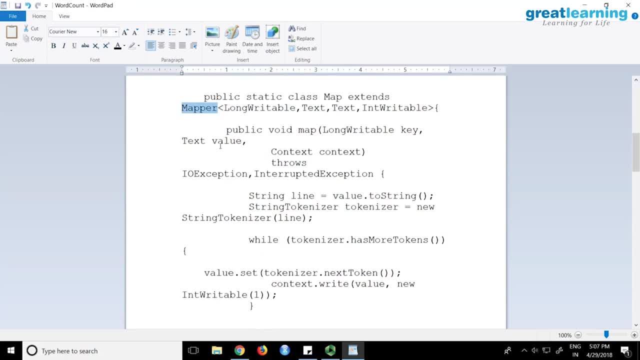 the next token. and finally, in order to write the mapper output, you will say context: dot. write value comma int, writable one. so this is where you're writing word comma one. this is the output. this context is an output collector. you can map reduce. in java you have system out print like that. in map reduce you have a context. you. 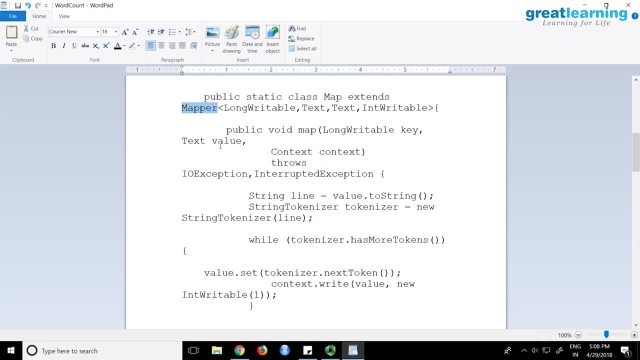 say context dot, it can, uh, you know, uh, write the output, collect the output. so this is where you're actually saying that word: comma, new int, writable, one, new one, your hard code in this. but what is happening here? right, this part, this is a very interesting part, this part, even for non-java guys. 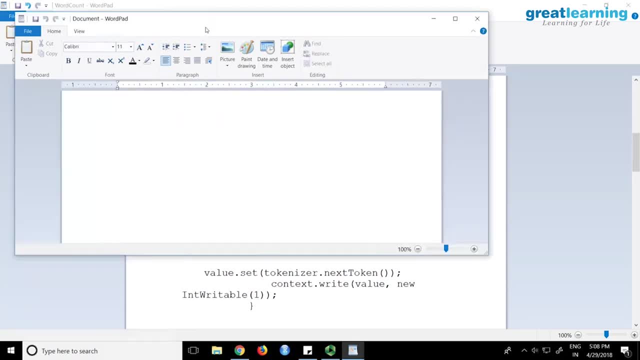 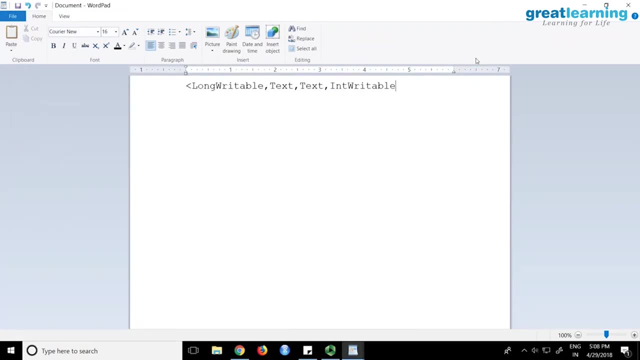 because i'll just copy this part. give me a moment. yes, so if you are com, so uh. another question is that: how do i compile this? so in production, what we do, we will have jenkins. you know, jenkins, right, it is a builder engine. so you say, you push it, it will combinate. 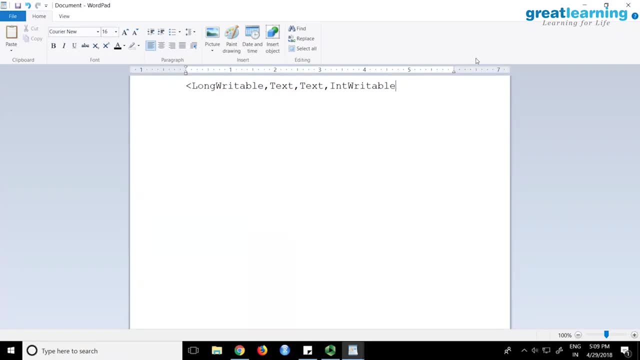 actually it will download all the dependencies because you will be using maven. maven will have your pawnxml one way. second way that i used to do is that you have to download the hadoop from apache. it will have these jars. you will add it in eclipse as. 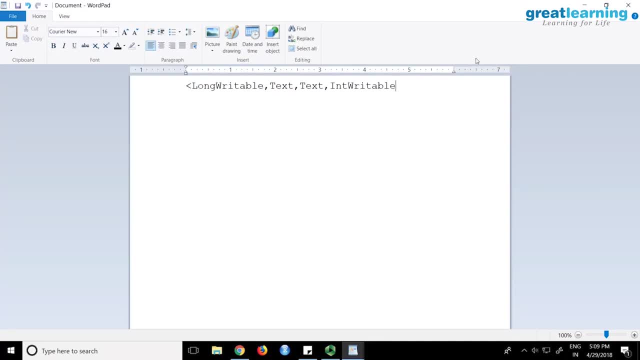 external jar. you say compile, it will compile. both is possible. these are external jars only. i mean in eclipse it is added as an external jars only, not part of this, so you have to manually do it. so very rarely i have seen people doing like that because in most of the projects you will have this: jenkins. 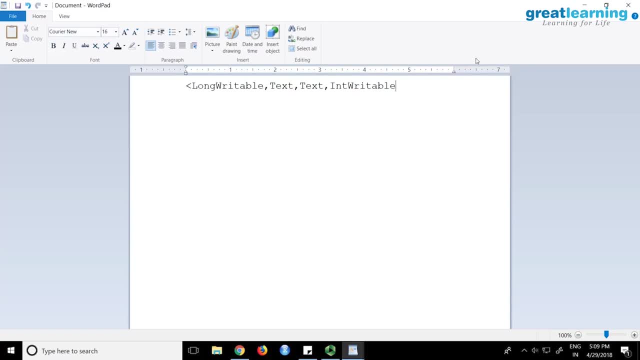 guy. so you'll push through maven only. that's easy for you because you can just add the dependency right. it will say i don't know what is an intratable how to download all the jars and add it right. but i just thought i will explain the basic stuff that you mean. so this piece of code i took. 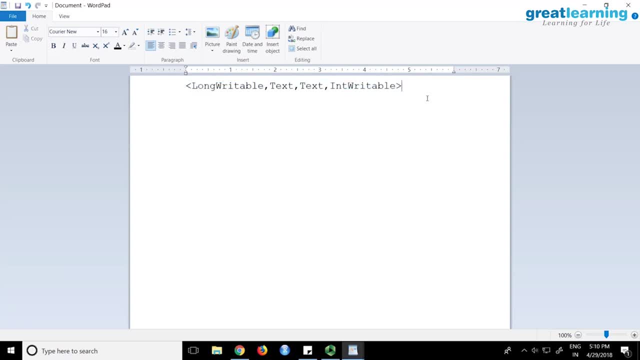 from the original program. i just wanted to explain this, okay, because see what is our input data. so people who do not know java could have been practically fainted out by this time by hearing the class names and interfaces and other things. that's okay. so this is my input data right now. 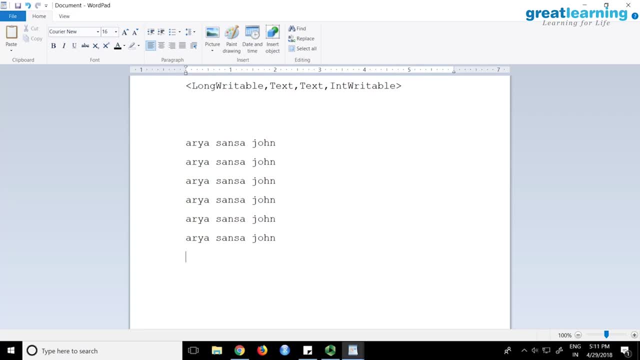 what did i tell you? i told you the mapper will read each line. and then you wrote a logic: get every word. but i lied to you. that is not the actual way. there is a reason. map reduce says: if this is your input data, you should give it as key value pair to the mapper. map reduce says you have the. 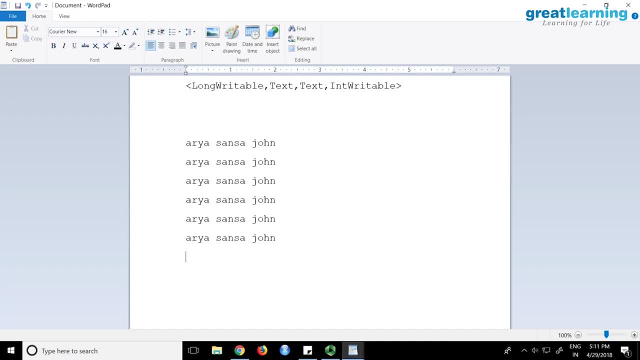 data. okay, this data cannot be given to a mapper as it is. it says: you first convert this data into a key value pair, then give it to the mapper. honestly, i don't know why it is like that, but that is a documentation, what it says. now the question is this: is my input file right? how do i further convert this into key value pair? 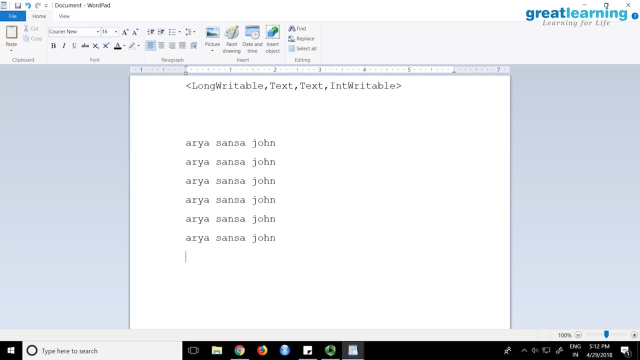 that's not possible. this is my original data. i don't want to convert or do anything right. so what happens is, when you are running the program, your framework will automatically convert this into key value pair. how, that's the question. so what is going to happen? it will add keys like this, so first key will be zero. 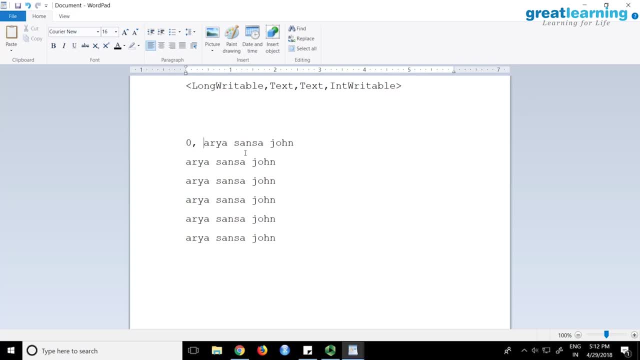 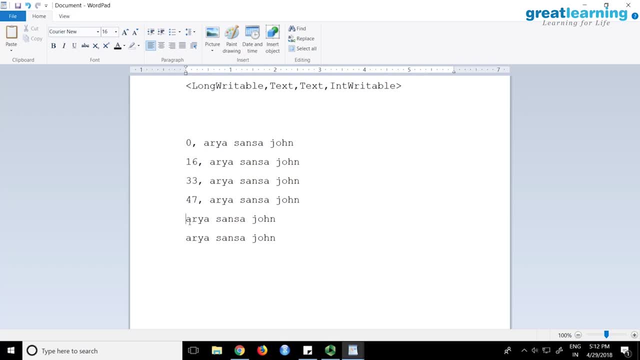 correct. okay, just to prove, i'm just writing: let's say 62, let's say 77, meaning each line. it will look at the first character. what is the first character? a right, the position is zero. zeroth character: zero will be the key. this will be the value right now. it will read: zero, one, two, three, up to 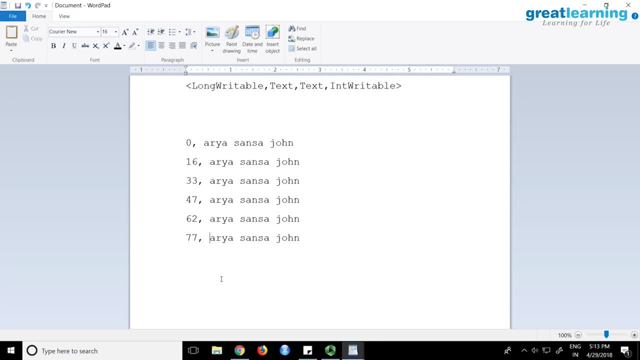 fifteen. next a will be what? sixteen? sixteen will become the key. this will become the value meaning, if you mention text input format class, there is a sub class called record reader. what this guy will do: it will pick up each line. okay, this record reader. it will convert them into this. 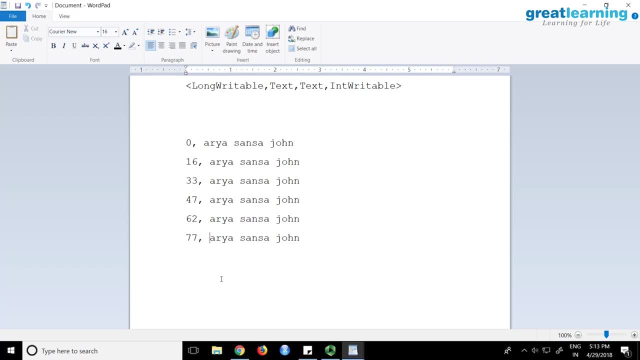 format and feed it to your mapper. so your mapper is getting data like this. it is not getting original data. the problem here is: this is key value pair. this is your key capital k. this is your value. you are getting key value pairs into the mapper so and key is useless, right. 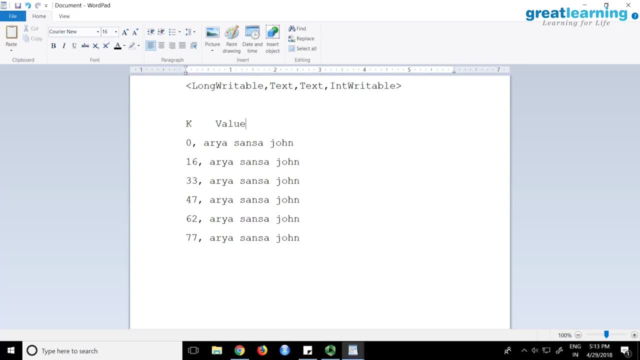 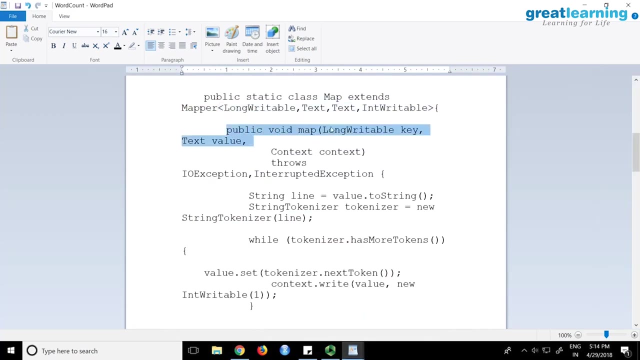 do we need the key? no, but something has to be added. so this was added right. so in the mapper i should say what process the value. right, that is what you see here. it says i create a map, long writable key text, value and context and exceptions and alt value to string. 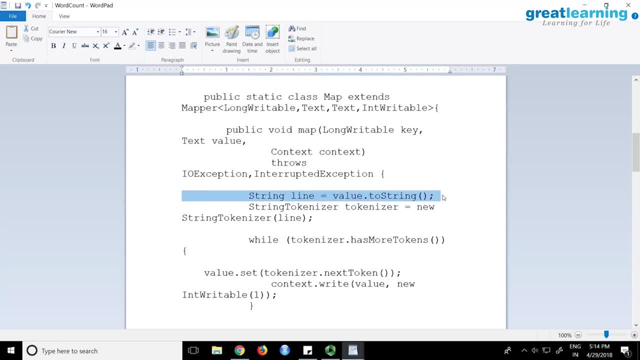 look at this line. you are converting the value to string and storing in this variable because the key is useless. so if you read the code you should understand right. this is a golden principle of map. produce any mapper you look, even in python, they will discard the key. key is useless. 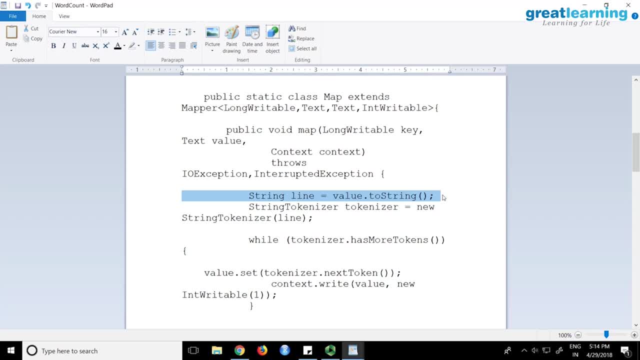 because the principle of map produce says the input to the mapper has to be key value pair. so the system will automatically generate some random key. in this case it is numbers, sometimes in python, and or sometimes we see some random numbers will be generated. whatever is the number, you can discard it. take the key and take the value and process it. that is what you are. 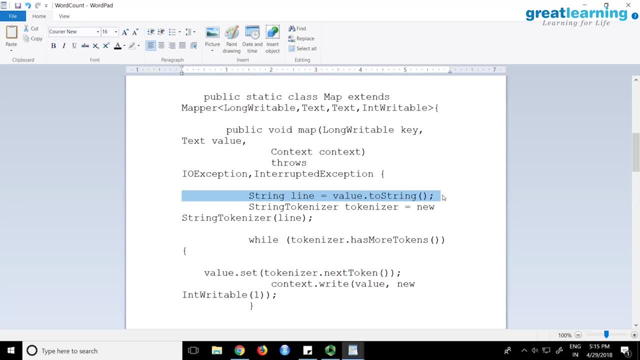 writing here. and what is this big code? this says: input is in the form of long and string. output is again string and integer. this is the input format. key value is the output format: xml. also, there is a random key generated. it is not the character position. i forgot what is there for xml? we have done very less xml processing. but even in xml you discard no. 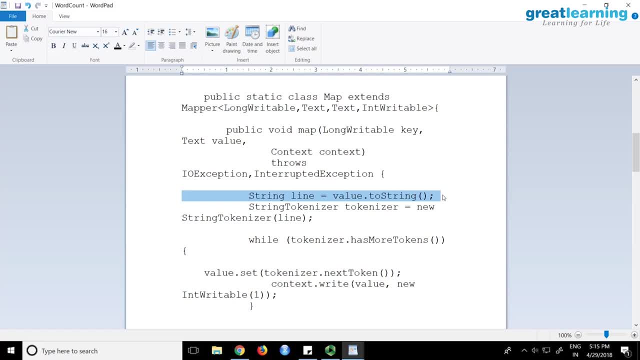 no, no, no, xml. you don't discard xml. the root tag and row tag it will identify as key. how is the structure of an xml file? you will have a root tag, then you have row tag. right, that is how the structure of xml, so it will identify them as the key and the corresponding data as the value. the 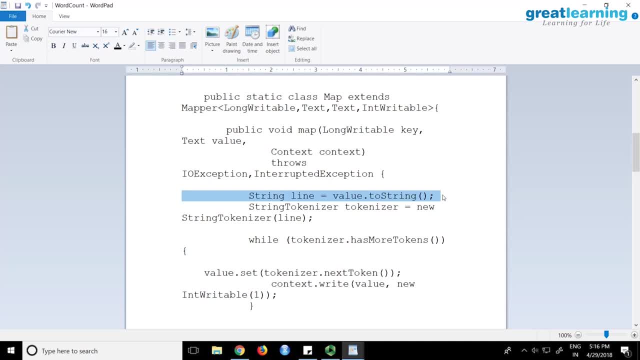 row tag will be your key and whatever row tag represent will be your value. so it is like a table right, like an rdbms table. the raw tag is like a column header, similar to that. so there, if you want, you can keep the key, because that is your row tag. if you want to process something, you can. 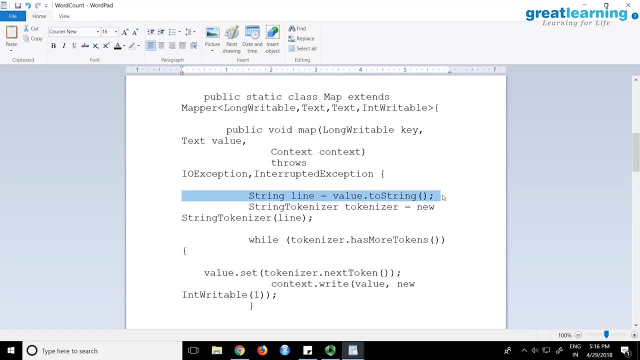 use it text file. this is the format actually, so it can start and end anywhere. but xml file processing is actually a bit complicated. for every raw tag it will create a key. what it does it? simply read it and create a key. then you have to make sense of that in your mapper, you have to read it and 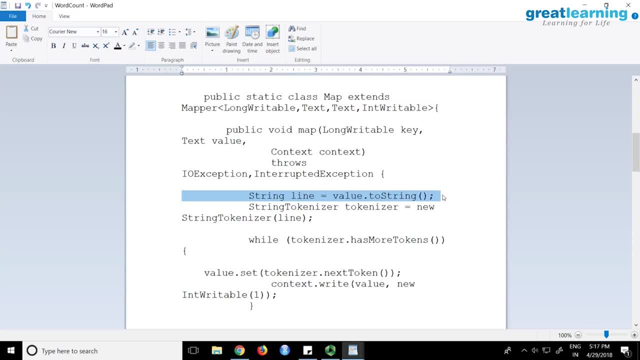 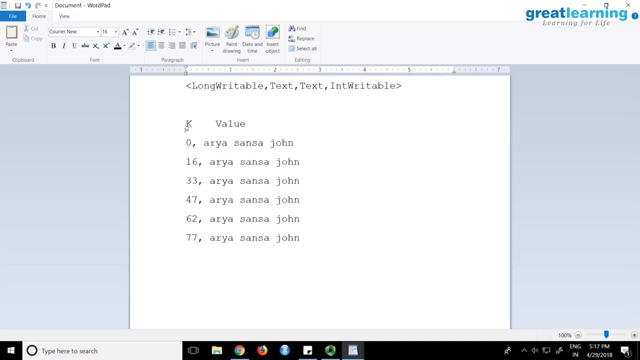 say that, if this is the raw tag, do something. if here it is ending, do something, because somehow it has to pass as a key value pair to the mapper, otherwise it cannot process. right, this is the input to the mapper, right? so if i take, this is one line, this is one line of input, right? if i just take? 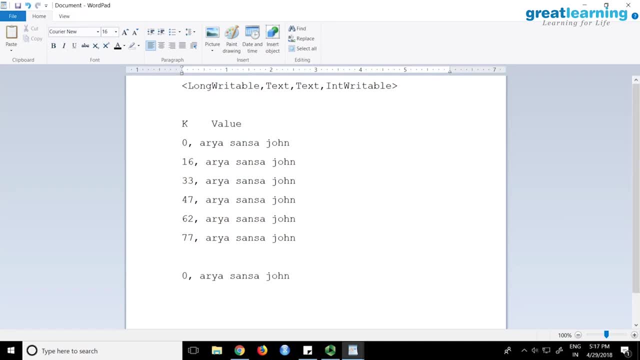 it. if i want to represent this, can i say: the data type can be long and string possible. right, that is this long writeable and text. so this is the input, but what is the output of mapper? the output of mapper will be, let's say, aria, comma, one, right, one of the output. what is aria? string, what is one? 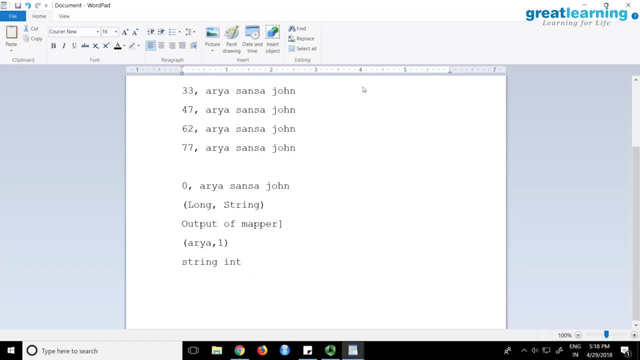 integer right doesn't become so. you are saying that the input of the mapper is key value pair. what is the data types? output of the mapper is also key value pair. what is their data types? you're just mentioning the data type of key and value. that is what you're doing. so these first two lines are input to the 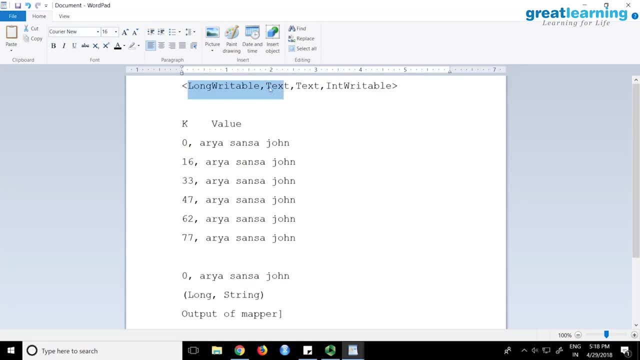 mapper. this is input to the mapper. key is long writable value is text. output will be word, comma. one word is string, one is integer. the point is hundred. percentage will be like this: i have never seen a case where you have a full line because you are splitting exactly at point: 28 mb hdmi. 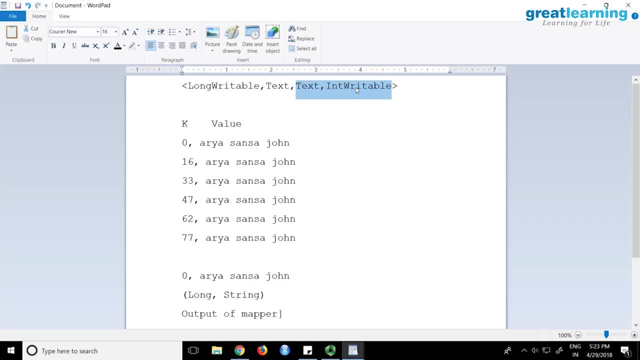 dfs says i'll divide your file exactly at 128 mb. what is there at 128 mb? how do you know? can you predict it will be a new line, character or end of a character? can you predict no, so the data gets stored like this. now you have a real problem. 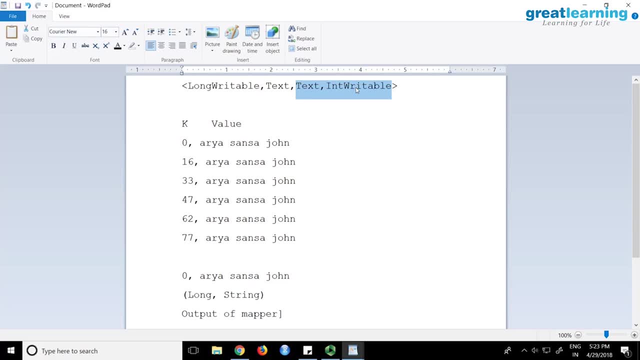 what is the problem? mappers run independently. one mapper will never talk to another mapper. tell me what is your problem exactly. if the mapper runs here, it will consider aria as a word. second word will be sa. this mapper will say: nsi is a word. and john, how do you solve it? possible, right? 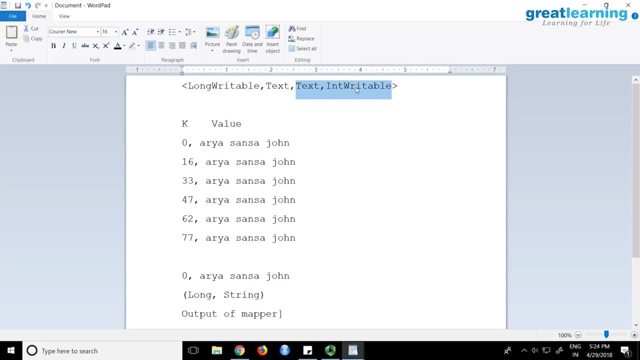 very much possible, so i thought somebody might ask this question. i mean normally when i say everything works in a perfect world, but this answer is also a bit confusing. i'll try to convince you, okay, or i'll confuse you. one of that will work. good question, right. 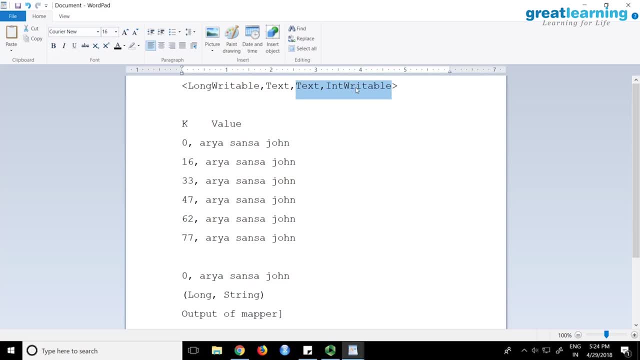 you are storing a bunch of images, is it guaranteed a block will have exactly 10 images? then how does mapper will process? okay question: can i take this line and add it here, this split line, why not? yeah, it's already 128 mb. i cannot increase the block size, right, so i mean it's not. 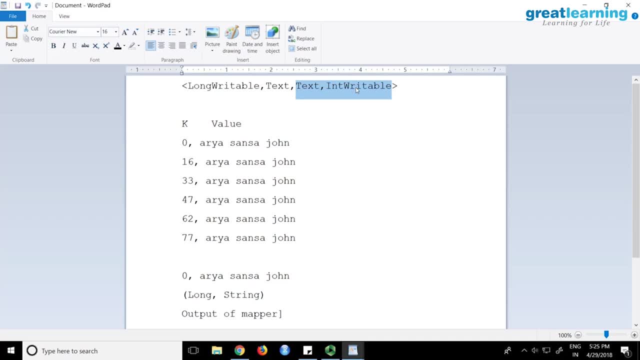 easy to answer it also okay, and it is very difficult to convince. also, what is answer? see, how do you know whether the block has incomplete data? who, who will know that's it? who is knowing? is it you or is it hadoop, or is it somebody in hadoop? there is no data. 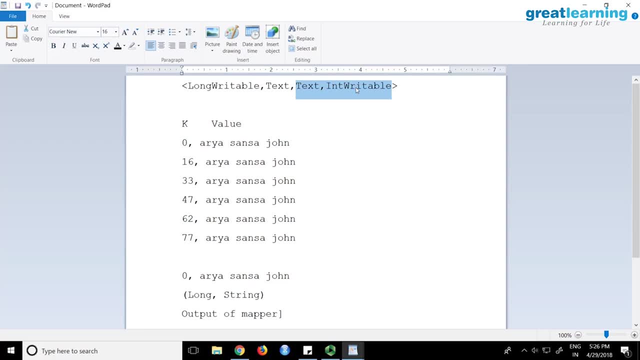 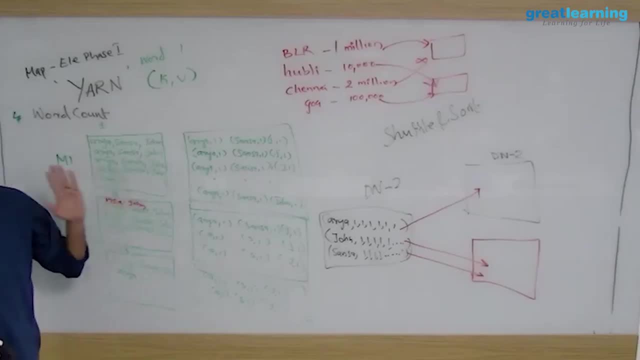 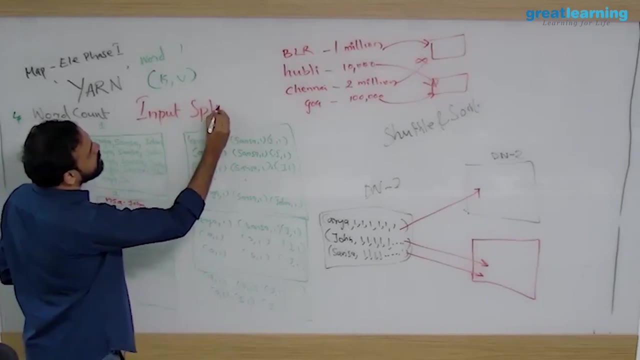 movement. in hadoop we are not moving the blocks right because that is extra processing. i have to move the block because every block will be like this: in in map reduce. before the mapper runs, there is a phase called input split. input split is a phase you know which will happen in map reduce automatically. you. 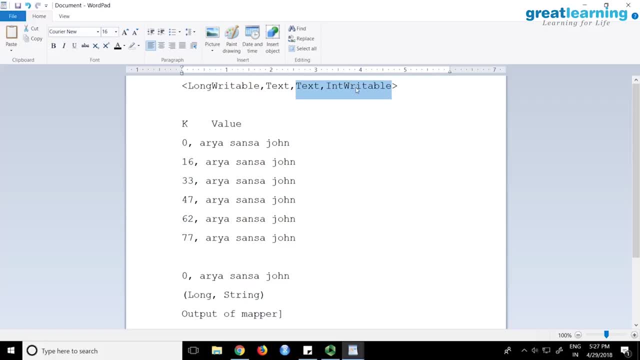 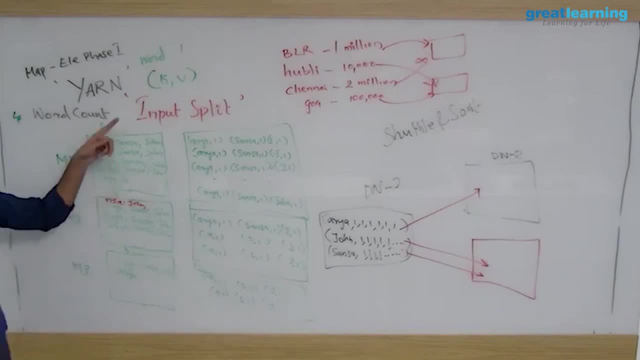 don't have to do anything. it will run automatically before any map reduce program you run. what is the purpose of input split? it is run by map reduce framework only. your logic was correct. it will analyze every block and based on text data- i'm talking new line character. it will understand. 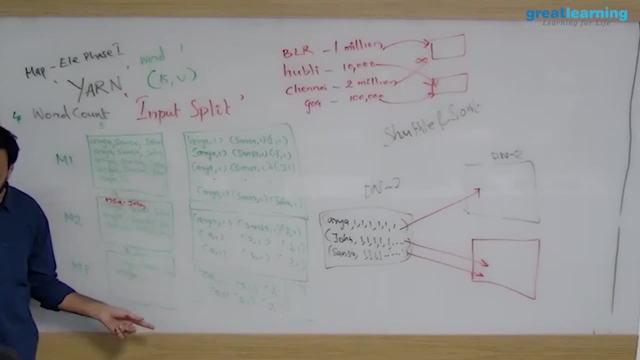 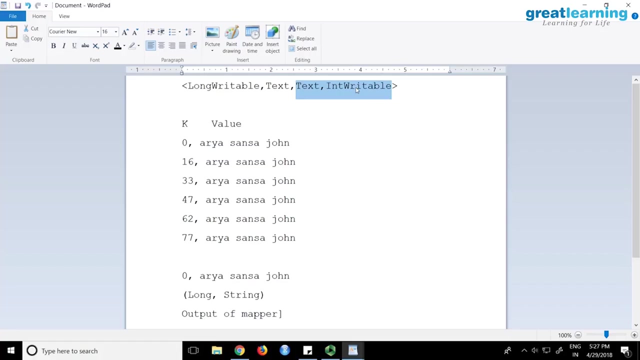 here it is split and these blocks are having a sequence as well. it understand. this is the place where the extra data is there. step number one: you identify there is a problem. the problem has been identified, but now the answer is very simple. what you need to do, you have to simply add this data. 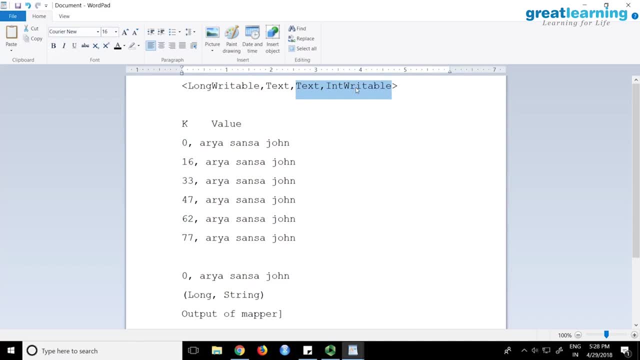 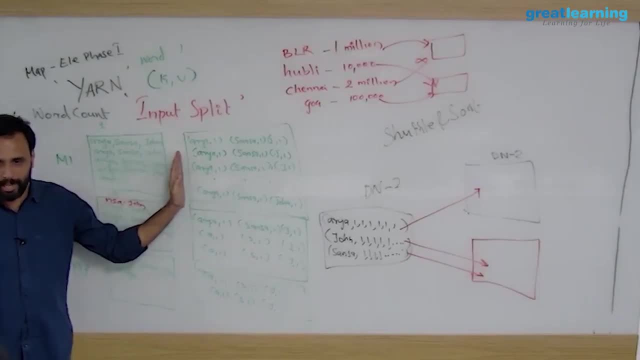 here problem solved. where? where does processing happen? in the hard disk or in the ram? yes, so this block will be read into the ram once it is in the ram- there is no block size right- and it will read this over the network and add it here in the data node ram. so all these 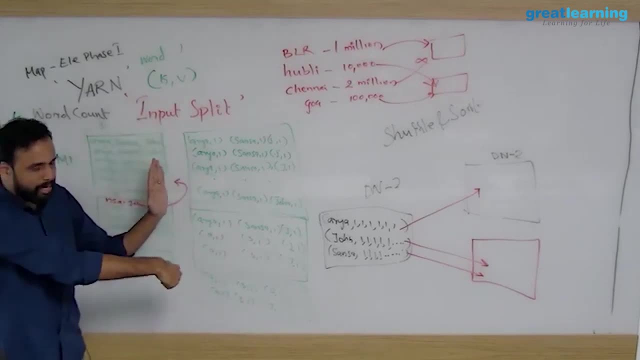 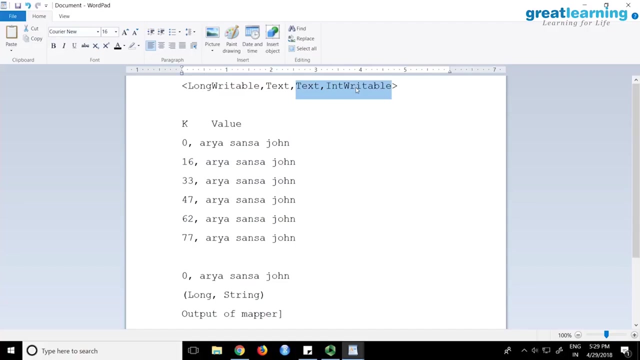 blocks are in the ram and then the input split will run. it will understand there's in this ram. there is a missing delta. read it from here and add it. it is simple and complicated. because why it is complicated? if it is a simple data like aria, sansa and all, it will work for other type of data. 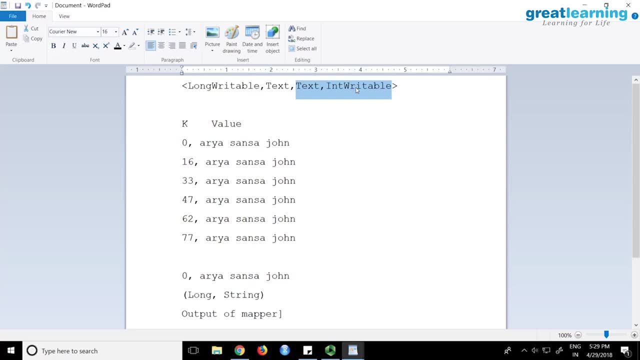 you have to. you might have to write a custom uh input split meaning. so try to understand. let's say, three line is one record here, one line is one record json or something. then json built-in. there is a reader which will understand what if you have your own format file. 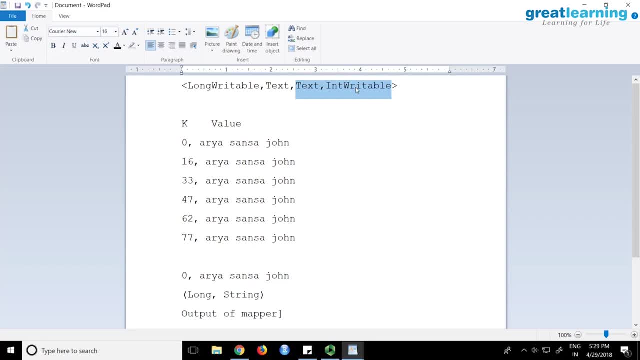 format, your own format in your company, where your company says: four lines is one record. if i want to process, i need one full four line. then you have to write your own input split class and say that hey, map, reduce, look for four lines which are not cut, if ever anywhere there is four. 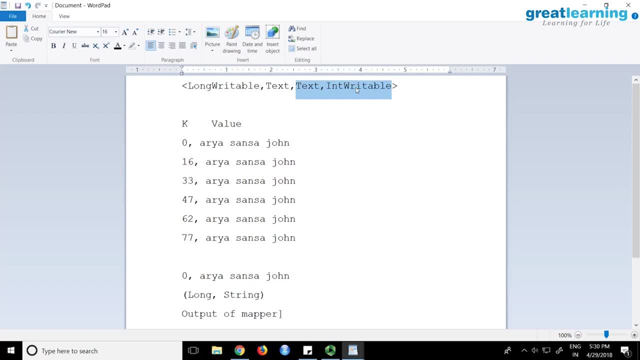 lines cut, you add it. and you did not ask one important question: if you run a map reduce program, how do you know how many mappers will run? you said depends on the number of blocks, not really depends on number of input split. for example, if here i had 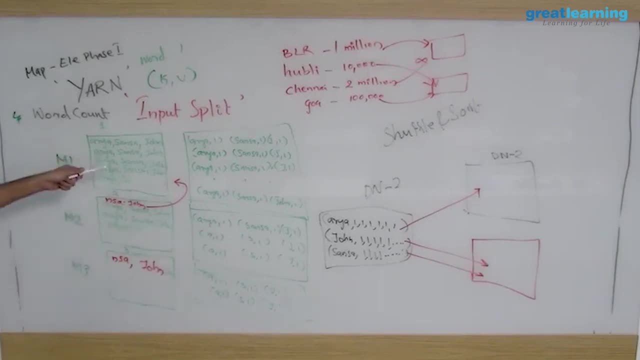 i have three blocks and two mappers. are you able to understand? there is a physical block here, but it has only a delta data. if, while running, map reduce, this will be added here. right? will there be a mapper running here? three blocks- i have two mappers will run, so this two is called. 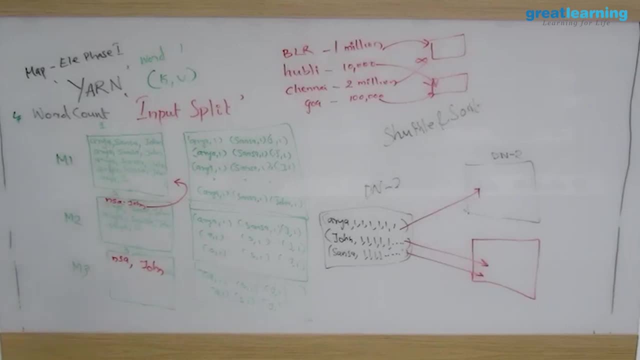 input split logically, how many blocks of data you have? no, no, the blocks inside the blocks. data will be same, only right within the block. i'm saying i mean this is a very rare situation, but you cannot always say that number of blocks are equal to number of input split. uh, always, it can be lesser. 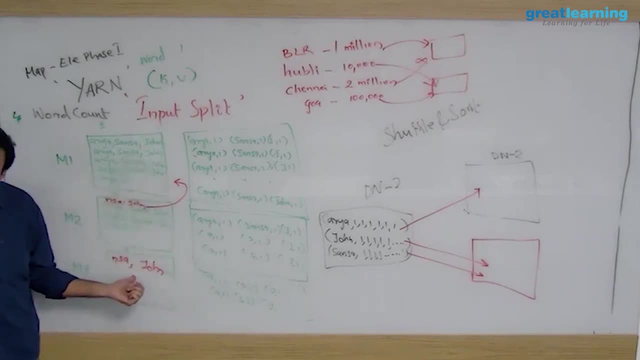 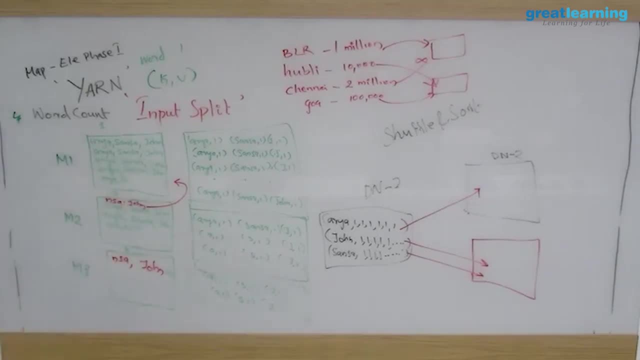 run. you can control it. also like- and you can never control how many mappers you need. it is automatically decided based on your data- you can always control how many reducers you need. that is your control. so these points you need to remember when you go to spark, rather than writing a code. 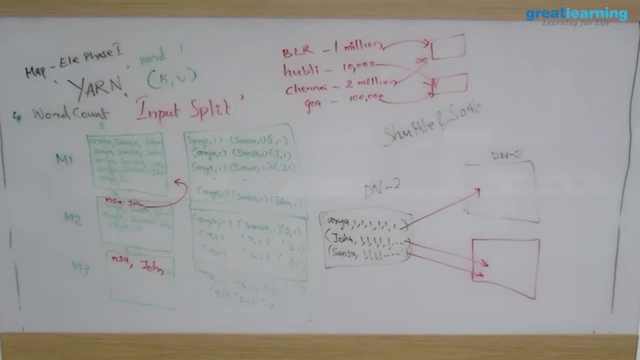 that anybody can write. even people without this knowledge can write a map reduce code if they need java. but these things actually matters because this is how your resources are utilized. when you run a map reduce program, you will see suddenly 10 mapper 3 reducer. from where all this came? 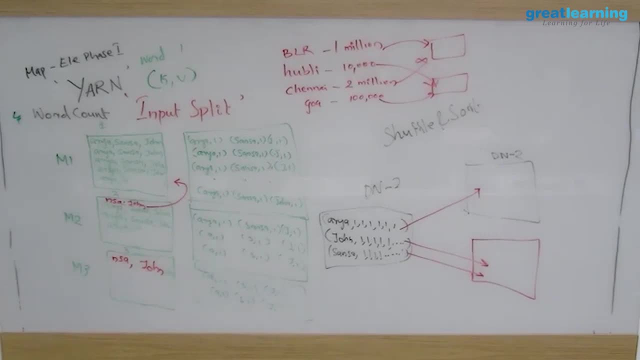 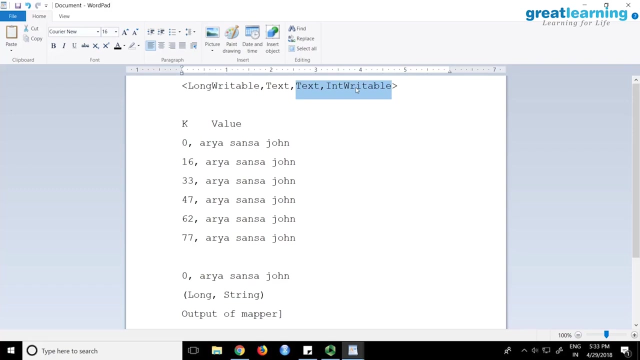 right. you should be able to figure out: oh, i have this. that is why the data is right like that. now that poses a question: what is the size of a mapper? when you say mapper is running? typically in a hadoop cluster, it uses one processor core and one gb. 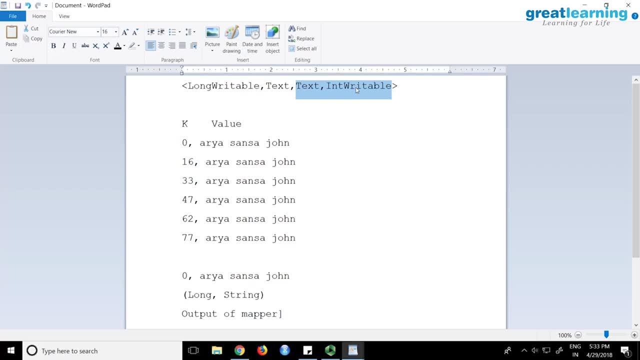 ram. one processor core and one gb ram. that is what is allocated to a mapper right now. let me ask you a question. uh, if you are processing a lot of data in java- normal java, jvm- right, you have a problem of garbage collection and overloading, and all right. here that will not happen, because in one 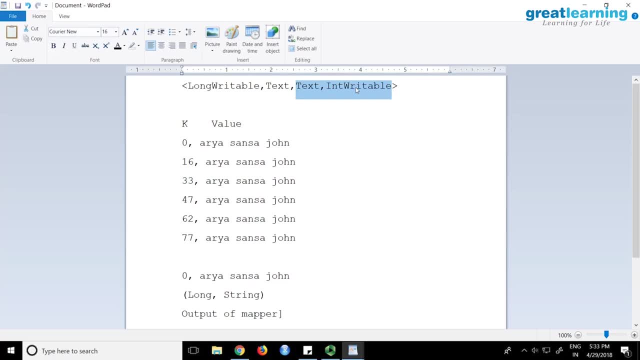 gb container jvm. you are getting a jvm of 1 gb. you are loading 128 mb block. see your data is only what- 128 mb, but the resource is 1 gb actually you are getting okay so it can get enough space to run and process and. 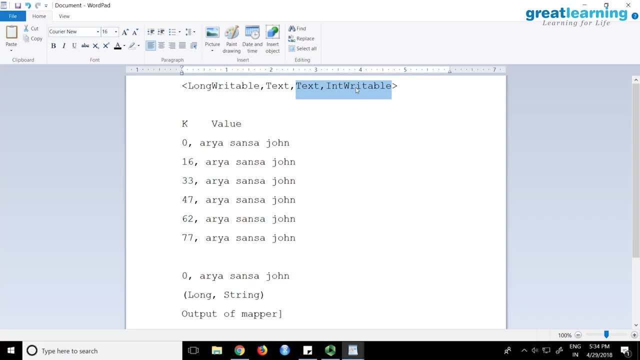 execute. actually the default is 1 gb. you can change it. here i am saying: in one of those that is having every. so here i'm saying: one mapper is running, that is running in a container, a jvm with 1 gb ram. that's what i'm saying. yeah, so this, this: when a jvm starts, it might load multiple blocks, also jvm. 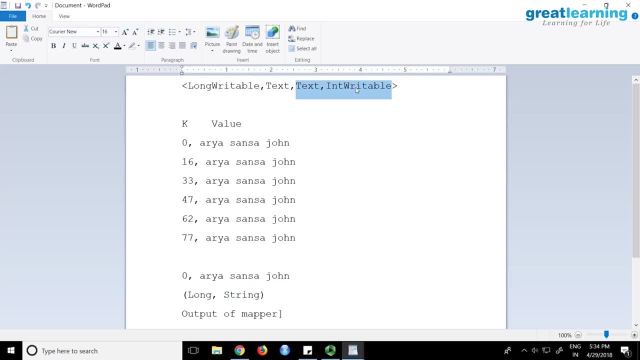 is just a container. it can read this block and another block also. right for another guy's program, right. so these two no matter the block. and the jvm video is too big and it sets the vão. other block can load by the jvm single block. there is way. only one block is grainy. so if that block there 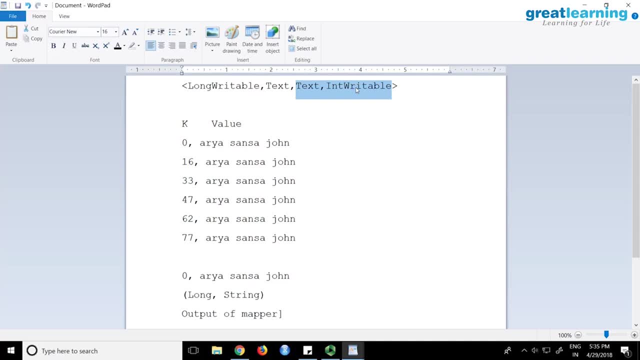 okay, another block can also be loaded by the jvm. it can track it right that case. two blocks will be loaded from each. uh, you know. so ideally that is how it happens: two blocks will be loaded and that will be processed by the jvm. but again, the ram is not the only thing that matters. processor. 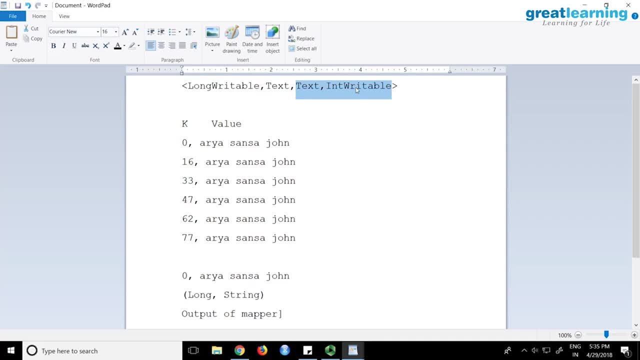 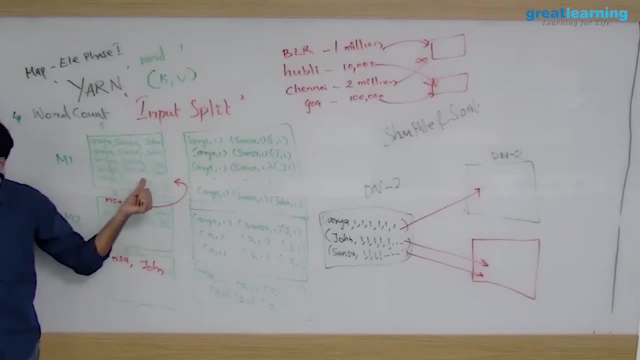 core also matters. inside a container, no problem. but if the processor can process only one block, even if you load two blocks, it doesn't work. got it right. your processor core also has to be there. that is only in this case. i'm saying: see, everything will be in the ram only. but in this case the this line is broken. 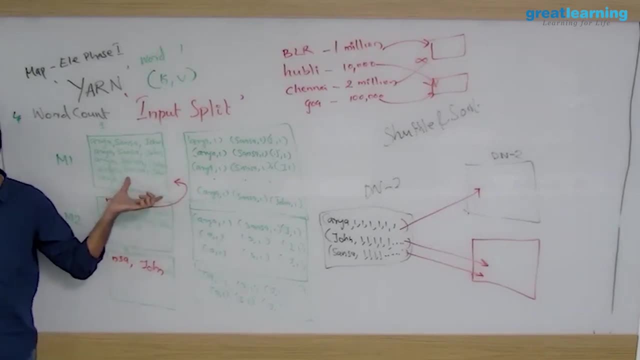 right. so i'm saying that this line can be added here to complete a single record. you need one line to process three blocks. you are not merging. three mappers are running on all three. but this mapper gets only half a line. right, only this line. this line will be combined here. that will happen. 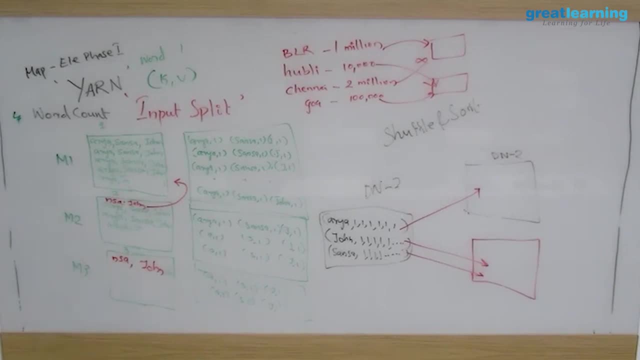 after shuffle and reduce right. this is the mapper mapper logic. i'm saying before mapper runs, only input split happens first you have to extract the key value pair right in the mapper. the final piece you will see only in reducer. zip file cannot be directly processed. you have to uncompress. 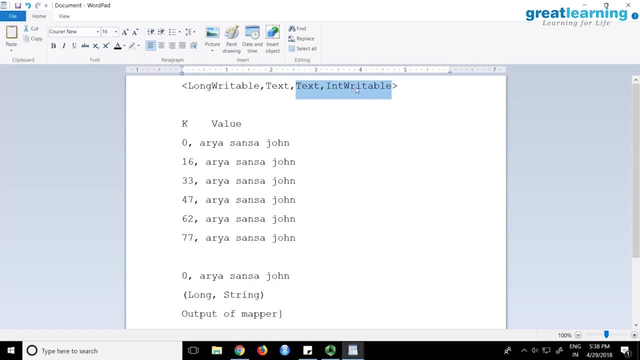 and process. so what is corrupted, what is not corrupted, depends on what is you want to process in this. i want to process line by line. so if i get one full line, it is not corrupted for me. am i clear? if i get single line of data, say aria, sansa, john, that is one record for me. technically it is called a record. so when 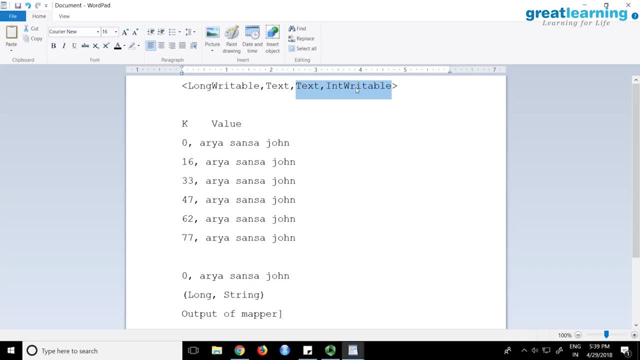 processing comes, you have to say record right in an excel file one line is a record. same way this is one record. so if this mapper looks, it says i have four records. i can count the words. fifth: the record is corrupted, so only this. it has to add here to complete a record. that's the. 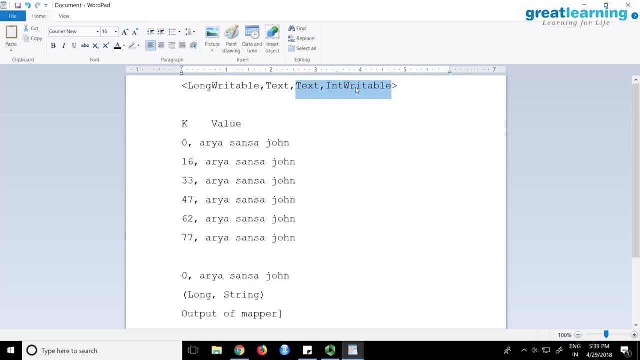 what i'm saying. yeah, so by default for text file it is new line character, one line, but it already read this, right, so this will be communicated. when the input splits happen, inputs will say that this line i am reading and adding here in the ram, so don't process start from here. only it is not mapper. 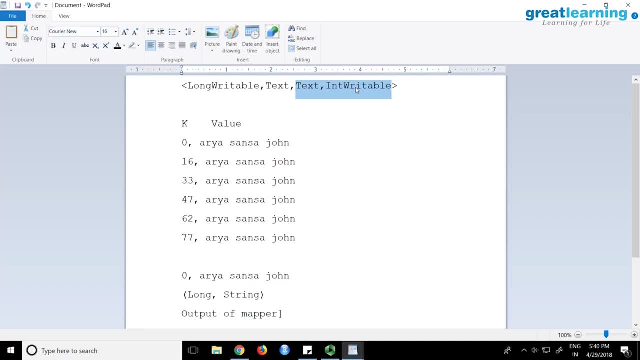 one which communicates, because mappers will not come here. my produce framework will inform, so it will produce these input splits in the ram. okay, so in the ram it is all getting processed right. so if this data moves to the ram over the network, you are copying this to here. 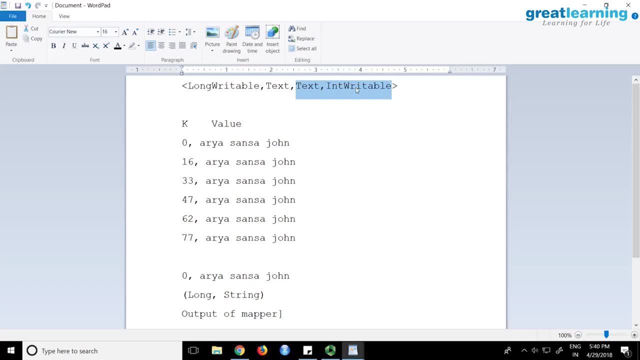 a cut paste operation, this data doesn't remain here then, because in the ram you are moving it right, so it doesn't remain there. no, no, ideally it will not be one mapper. ideally for one block you have one mapper. the idea is that for one physical block you run one mapper and in that 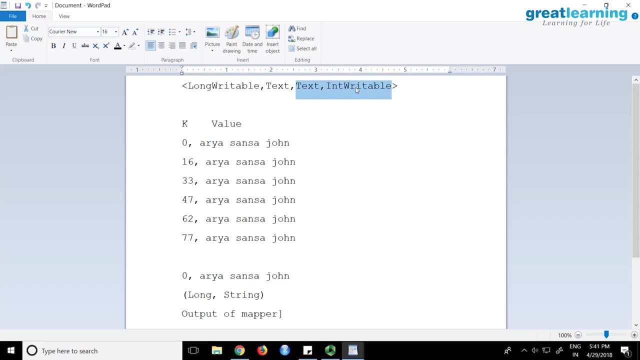 block. if you have a missing record, you get from others. you are not combining two blocks. if one mapper is combining these two, then it can come combine hundred blocks also. what is the pro use then? you are moving data over the network. you have to minimize the data movement. 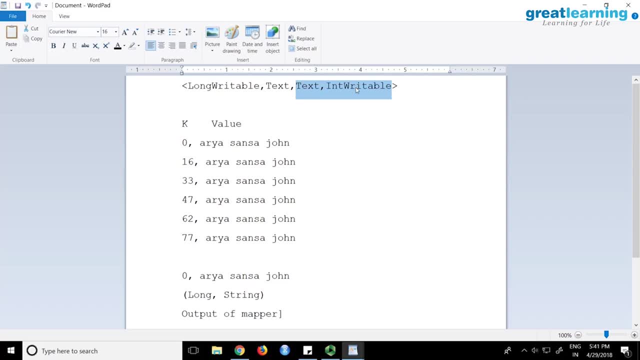 you have to minimize data moment. yeah, sure, i mean, i just took as an example. it might be this way also. this is just an example. it doesn't mean like always you are adding from here to here. it can be. from here to here depends on the size of the data. yes, so if here you have small data, 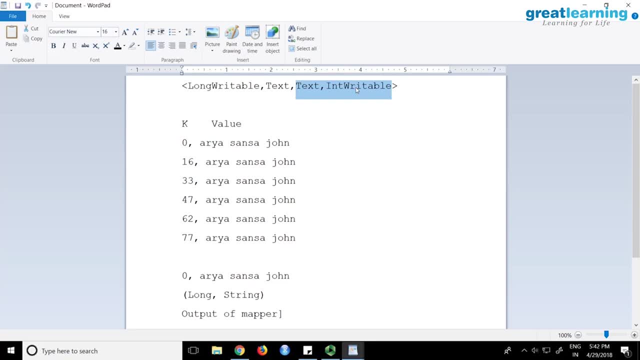 it will push here because the idea is to minimize the data moment. whichever way you can minimize the data moment, it will process, unless you want to process your own custom files, not the mapper code. this inputs plate class is there where you have to write how does your file looks like and all mapper. 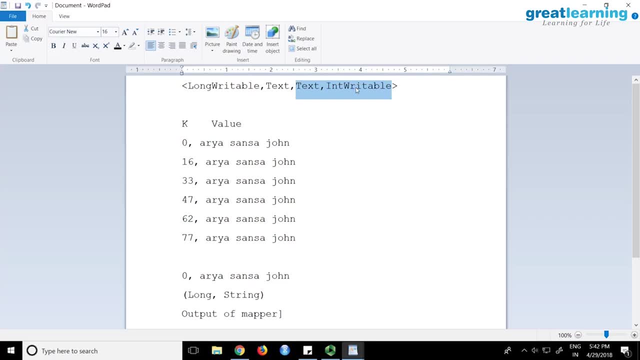 file as standard only. so if the file is how's itagi it, i will say it's standard. only this is happening before the mapper code runs right. mapper should get perfect data. it will not mess with the data. you can probably say: my one record is one lakh lines. what will happen? everything will load into. 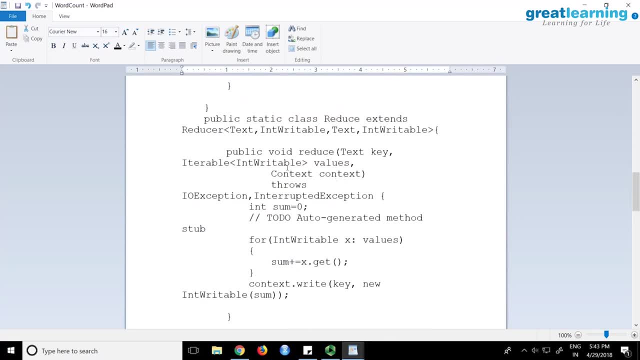 one mapper and process it. that's also possible. the reducer code is similar. i don't want to explain much, but if you look at the reducer code it has again a public void: reduce where you are getting a text. this is the key. then you have something called iterable on values. i triple is a. 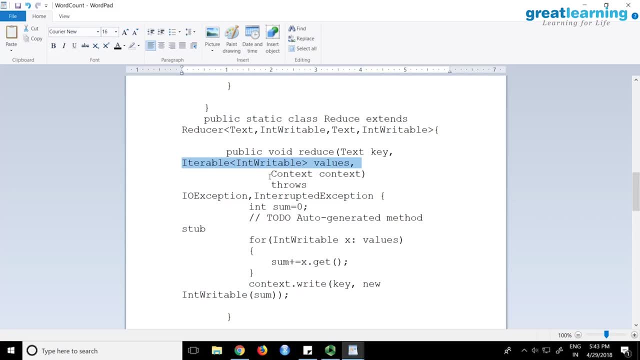 the values and then you have context. so what is that you are doing? in the reducer you will say sum equal to 0. you will open a for loop. this x dot get method will get all the values. remember, shuffle output is given to reducer, so shuffle will have a key and 1, 1, 1, 1, 1. so this x dot get will. 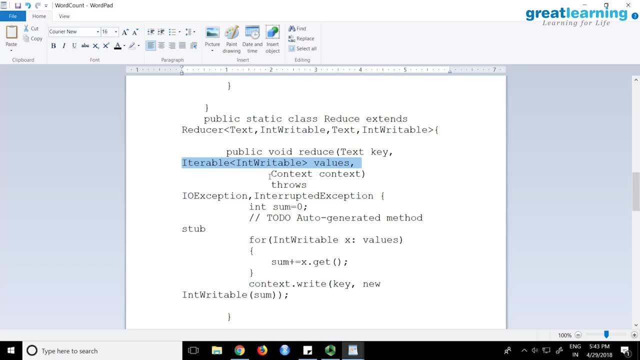 get all 1 1, 1. it will increment for this sum. so sum will keep on incrementing. you will get the final output, same java code and finally you will say that key comma, new intratable sum. you will call this sum here. you will get the final output. now let's run the code and come back to this again. 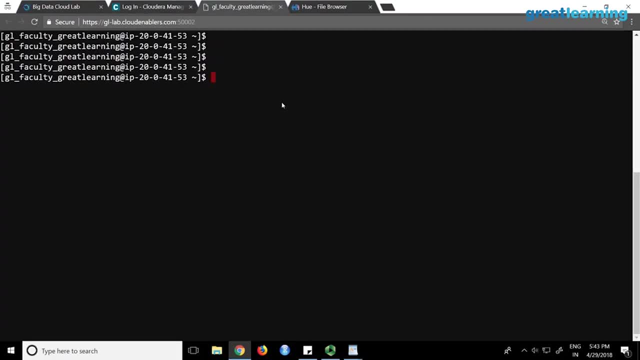 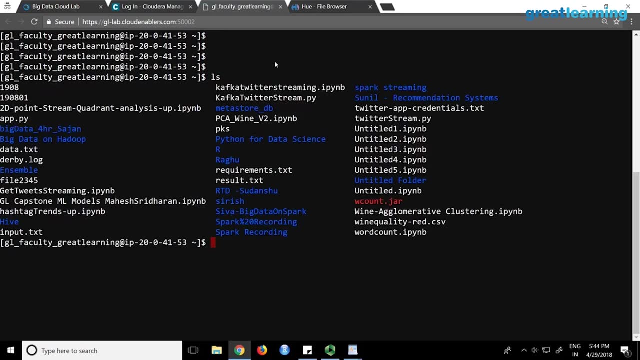 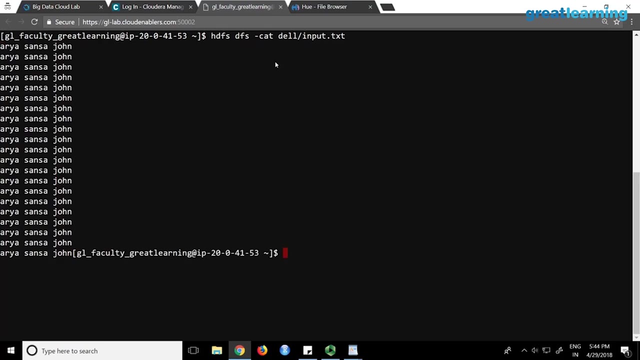 i want you to be so. can you access the cloud lab? can you check? because the net was down. internet was down. can you log in and see? is it available? i am assuming you have your file here, right? this input dot txt. is it space separated? can you confirm? 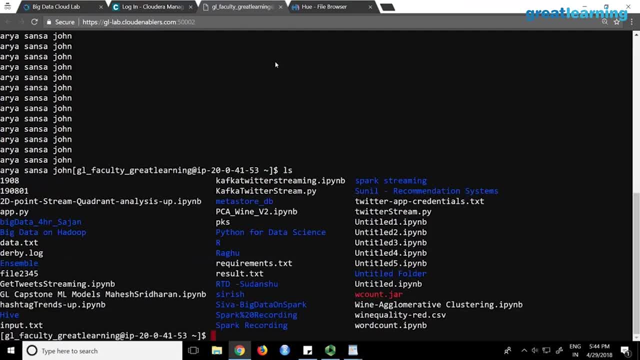 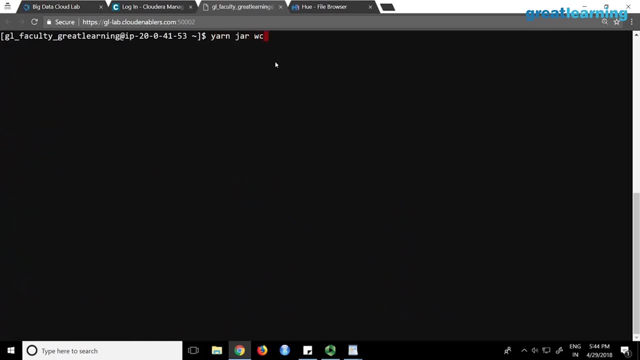 you: yes, right, and if i do an ls, you should see this: w count dot jar also. can you see that? yeah, now, in order to run the map reduce program, i will. you will say yarn jar and you will say word count dot jar. this is the command. yarn jar means you are submitting the jar file to yarn. 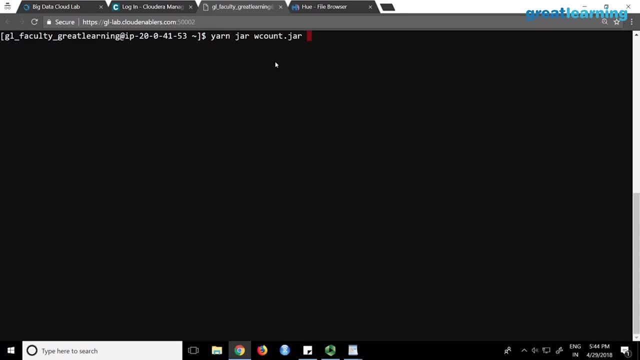 yarn is the guy who is going to run it. word count dot jar. then you say: where is your input data? in hadoop it is in del slash input dot txt. that is where the data resides. so you are passing it as an argument. where is the you know input path? and once map reduce. 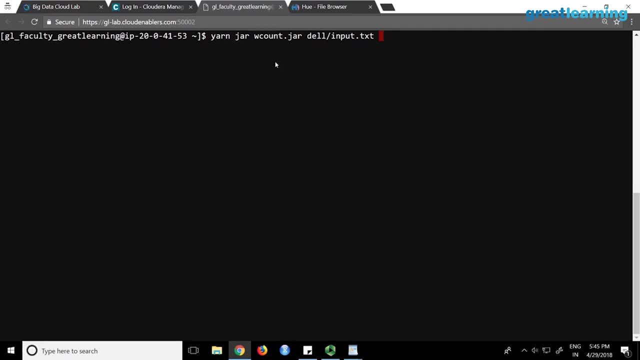 program runs. the output has to be stored in a folder in hadoop. now you have to give a new folder name. if you give an existing folder name, the program will fade. what will happen? map reduce will create a folder and dump it, dump the output. so i will say that i need the output in a folder. 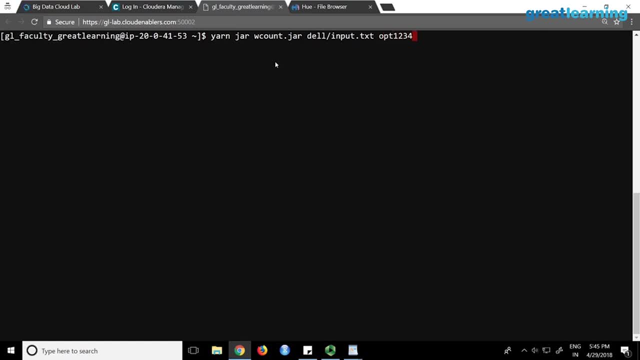 let's call it as opt1234, any name, any name which does not exist. so i am saying that: run the jar file- my data is in del slash input- and once you get the result, create a folder called opt1234 in hadoop, store it there and if i hit enter, if everything works fine, it should run. okay, see. 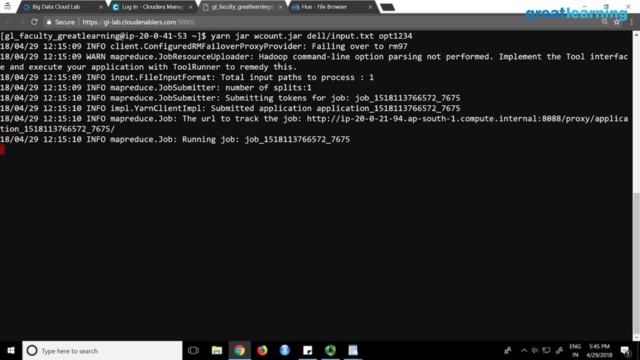 number of splits. one very important point: input split, number of splits. one it already calculated. it's a very small file, running job. so the job is running. yeah, see, map 0, reduce 0. map reduce phase started. okay, map 0, reduce 0 and i will say map 100 and reduce 0.. the small data, right, you have. 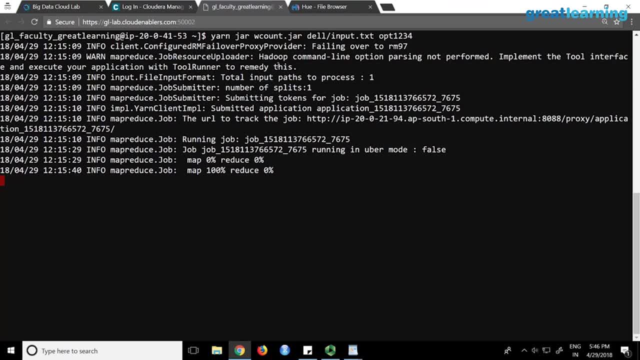 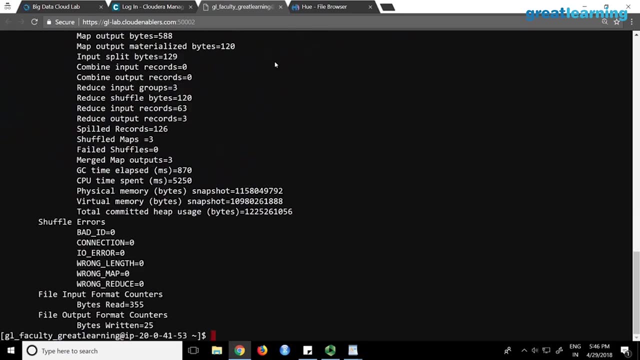 only smart map 100, reduce 0. so map phase is over now. produce phase is still starting. reduce 0, reduce 33, acquire, because a lot of people are accessing the cluster right. that's why see reduce 67, 33, 67, reduce 100 and over program 1.. so if you see this, your program ran successfully. this opt1234 is a. 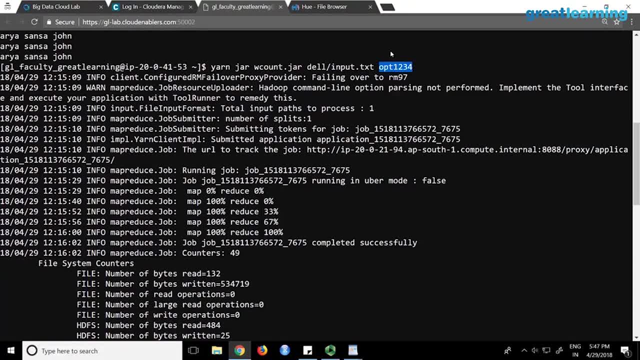 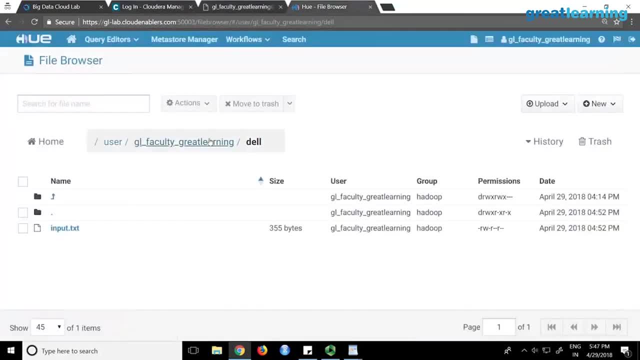 folder in the program you can tweak it. you can say that if there is an existing directory, delete it. so it should have created this folder now. so if i go to my hue, i'll just let me check this whether it ran successfully. if i go to hadoop, there is a folder called opt1234. if i open that there are. 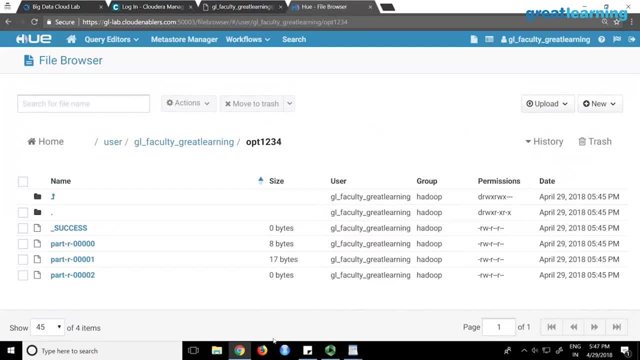 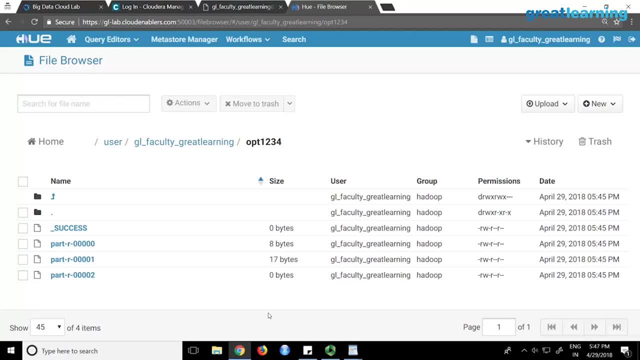 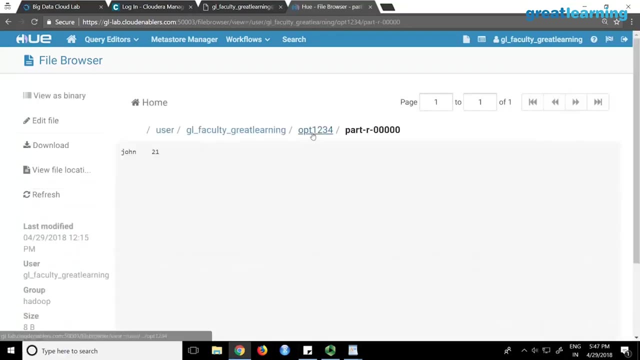 file does not have any output. third reducer simply ran. it didn't get any data. because very small amount of data, my shuffle could have thought let it go to two reducers only. third reducer didn't get any data and if you want to see the output, just click on this guy. john 21 was processed here. 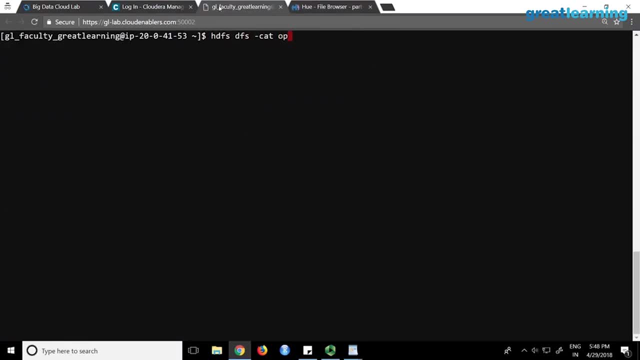 fs hyphen cat. what is the folder? opt1234 slash star. so this command you can run from the command line. you are saying that. show me the output of all the files combined in opt1234 folder. that is, opt1234 slash star. not really, because you are running multiple reducers, so the reducer 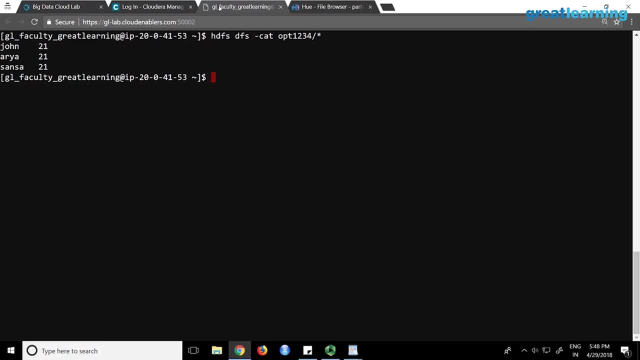 output is not sorted, reduces themselves. internally will sort right, but now i have two reducers, so one guy was having john right, the other guy was having aria and sansa. the other guy is having aria and sansa. this a and s is sorted. ah, that is displayed randomly, so here it could have been sorted. aria. 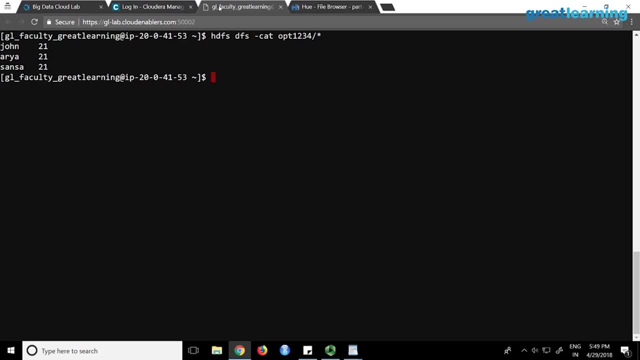 and sansa will be sorted within a reducer. it is sorted. actually, you, i asked it to create a folder. right, i don't need to know the name of the node to get the file right. then my name node is useless. so i said: show me the output of opt1234. so when you uploaded the inputtxt, did you know where it? 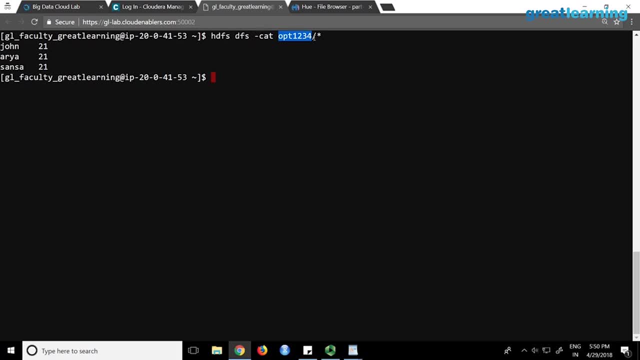 went. that is where we run that files racks location. so when you uploaded the inputtxt, did you know where it went? that is where we run that files racks location. yeah, yeah, so if you run this ideally- um, i will talk about this- there is somebody called resource. 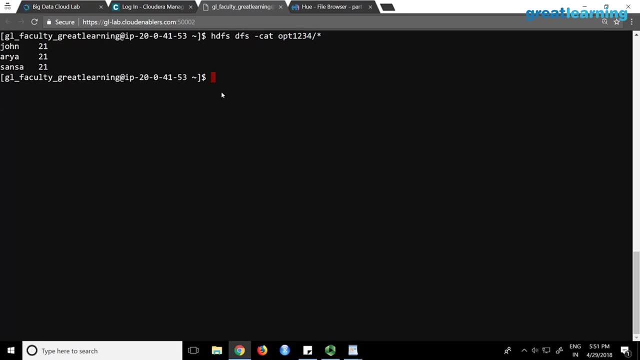 manager. so a little bit about yarn. yarn is your resource management framework, so there is somebody called resource manager. in yarn it is the master. so if you submit any program it will go to resource manager and this guy will decide how many resources to be allocated, where it should run and all it. 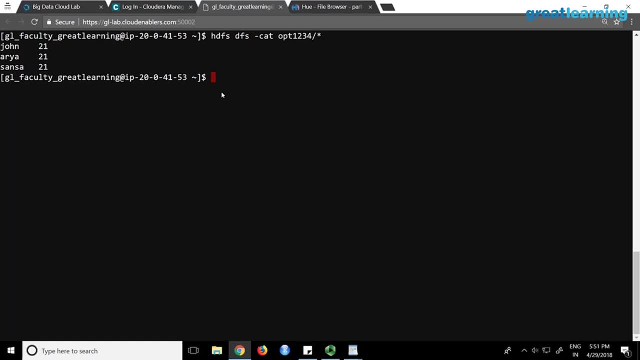 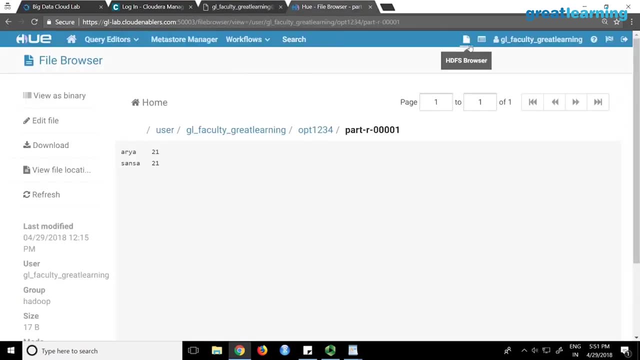 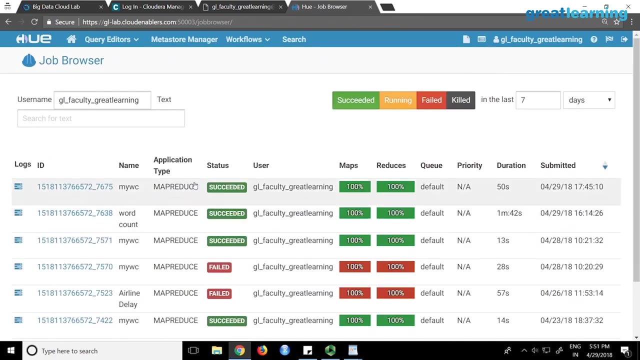 will run it actually. so from the resource manager, you can see the logs. one thing, but more than that if you are having hue access, right, yeah, so this is there. if you go to hue, there is something called job browser. can you see job browser? you can see the program which ran. okay, see, this is the job. 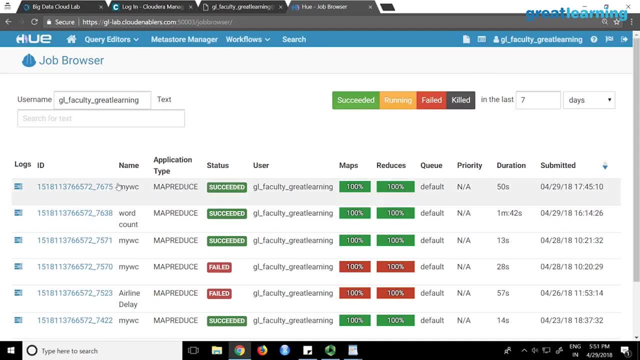 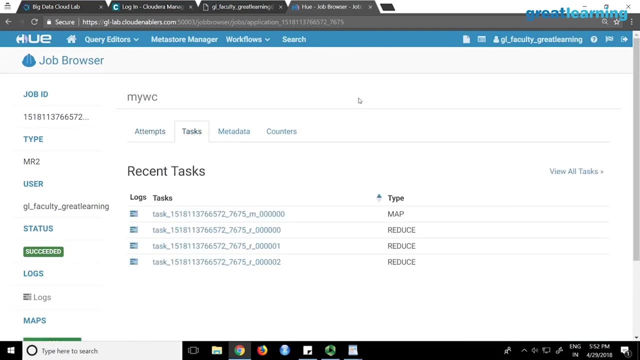 browser will just show you all the jobs ran. so this is my word count: map reduce ran by gl faculty. right, it says map 100 reduce 100. everything was fine. if you click on this guy, yeah, it will say that attempts right one. if you go to task, it will show you how many mappers how many. 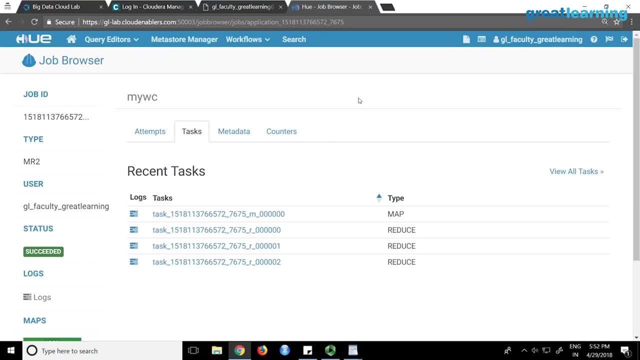 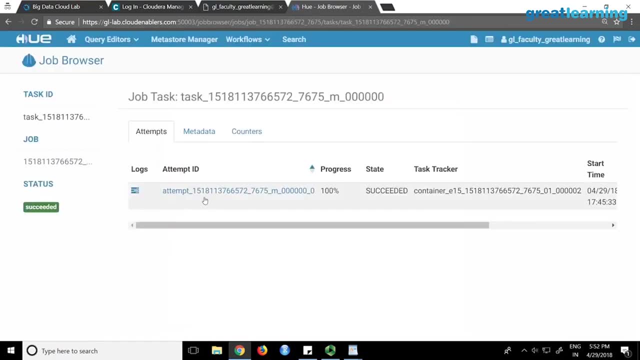 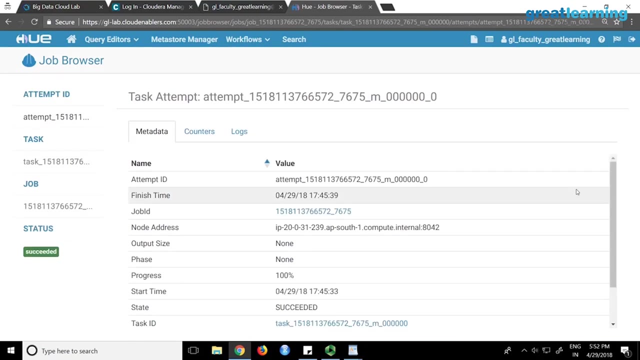 reducers ran. so one map was ran, three reducers were ran. now if i go to one of this mapper- let's say this mapper- if i click on this guy- i clicked on the mapper, okay, it says an attempt. if i click on this attempt, i'll get the details where the mapper ran. so the mapper actually ran on this. 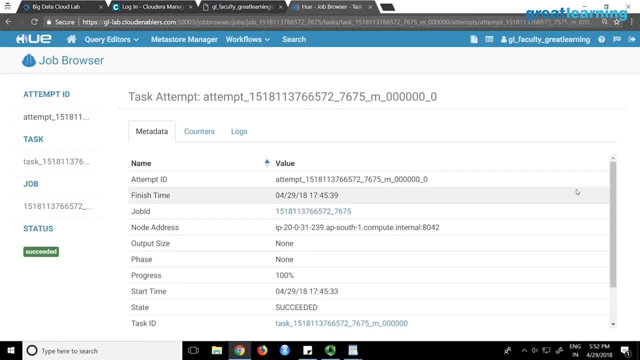 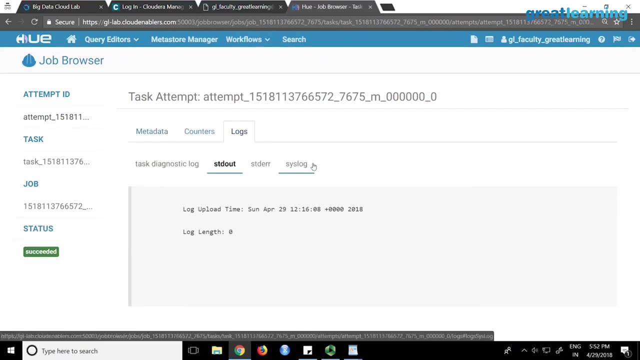 machine 20 0, 31 239. this is where the mapper ran right and it says progress 100 succeeded. you know all the details. logs are available here in the mapper. so if you go to the logs you can see the logs. it says std out, stdr syslog. all the logs are available. job browser is actually part of. 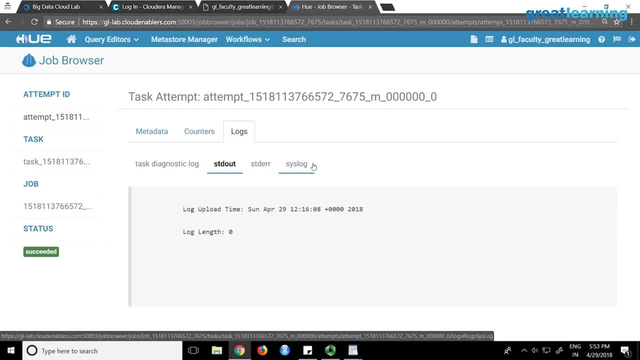 hadoop only. okay, and hue will just put it in a very nice ui and give it to you so you can track the jobs. so from here you can see how many mappers ran, reducers ran, any errors were there? anything crashed, everything command line. you have to look at yarn logs actually and you don't have access. 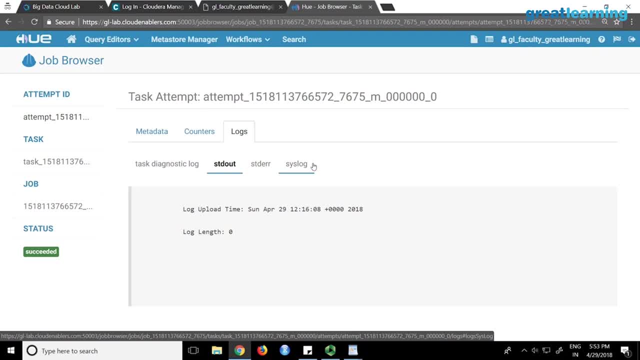 actually that's what you can see normally. another thing, very important question: normally you will ever in your life run a map, produce job like this. you will not go and say, okay, yarn, yarn, jar and run what you do. you will schedule it using uzi. you will go to your admin and say that i have a program to. 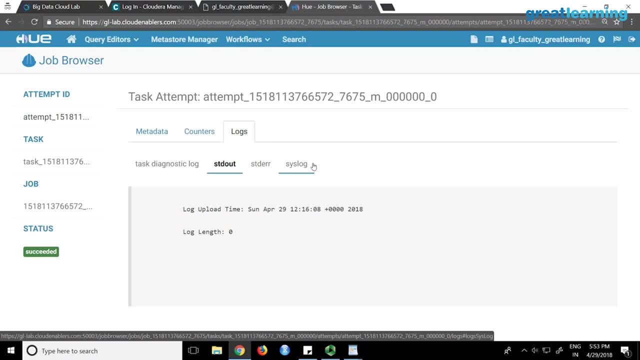 run. he will say: i will give you uzi and in uzi. so if you are submitting the code to uzi, you don't need driver. very important point, please make a note. you don't need to write the driver because driver will be with uzi. in uzi you can set. you know what is the text? input all these things. you 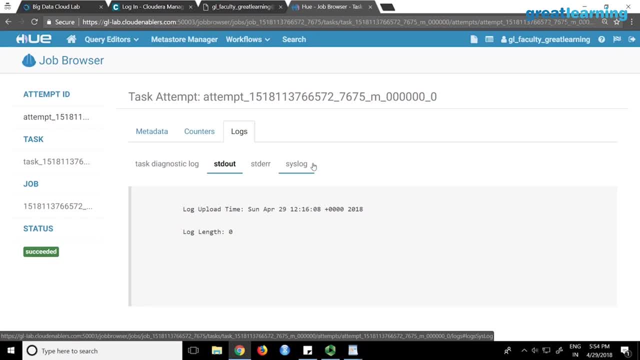 can set in uzi as an xml. in uzi, you simply provide the mapper code and you will get the code and you mapper class, reducer class. that's it. it will run it for you. in uzi. what you do is that there is a file called a workflowxml. in that xml file you will define all the driver property- same thing. 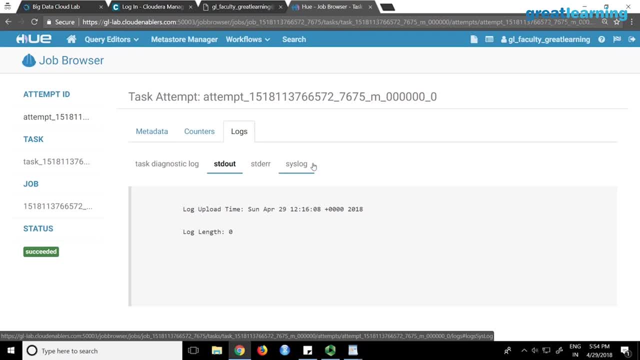 you wrote here like: what is the input format, output format, everything. you will write there and in uzi you will say: this is my mapper, this is my reducer code. you will submit the jar file and then you can schedule it. you can say: every day, 11 o'clock, you run it, will run it for you and that's. 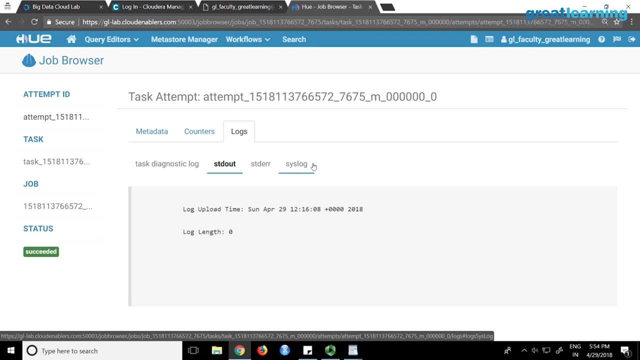 what you won't directly run from command line in a production network. nobody will give you access. also, don't worry now, if you are a java guy, you can also do unit testing in map reduce. the framework is called mr unit. you could have heard about j unit. it's an extension of j unit. it's called mr unit. 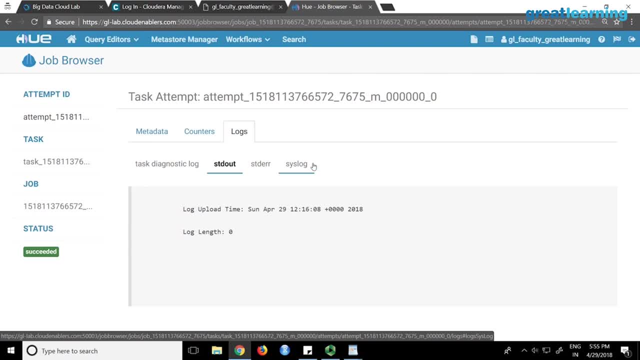 mr unit map, reduce unit. you can run unit testing so all the regular testing things can be done. there is mr unit for unit testing and then you have integration testing and you know black box testing, all these things testing. there is a separate team for all these things. i'm not from. 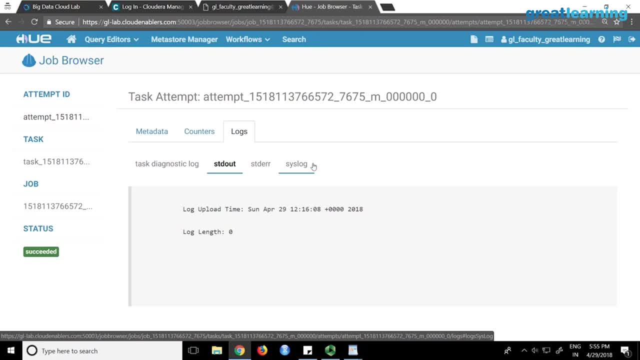 testing background, but you can run it for all these things. i'm not from testing background, but it there is a team actually who does so. you have a test cluster which is exact replica of your production cluster. otherwise, how do you do this? right, you created everything. you packaged the jar. 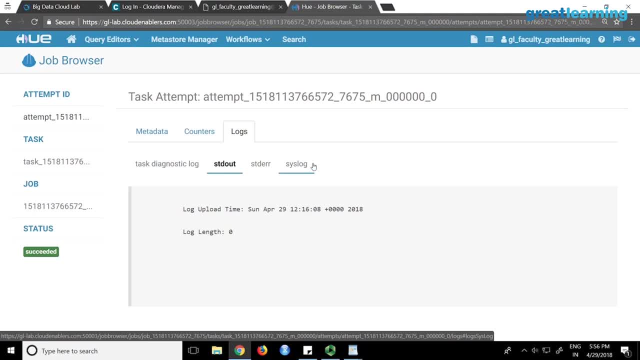 you ran, the entire cluster crashed. so then you can't have such situation. so you have to debug and test it completely in a testing cluster. then only you submit it in the production cluster. so once you submit in the production cluster, no error should come. error can come, resource is: 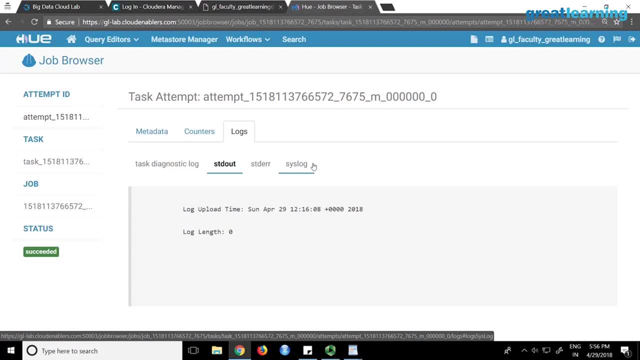 not available like that in the code and all, no error is accepted because you will need to do a lot of work to do that. so you will very rarely get chance to again resubmit. lot of people will be submitting jobs actually in most of the companies. i am saying that cluster is always. 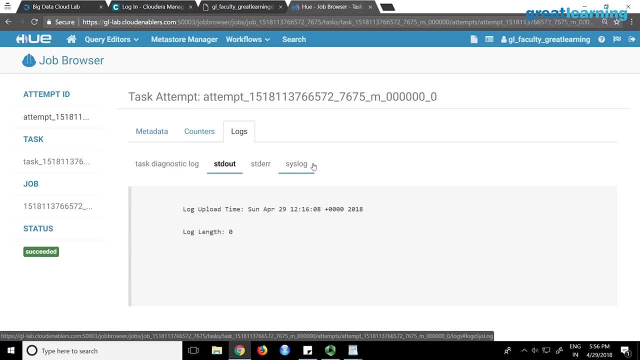 busy, lot of jobs will be running, spark this, that, so you don't have time to again, again test and run in a production cluster, right, but it will be already written. it's not like every time you write it. so these are all business use cases, right? say, for example, uh, when i was training people in 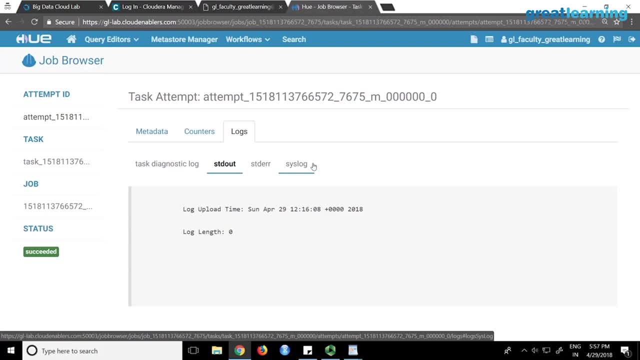 the flipkart. okay, flipkart used to have a map reduce program and they would have the logs from their website where people browse. okay, and then there was a map reduce program which will read these log files. it creates some key value pair and then it will output like how many people search for white items or something. so this will run as a batch job. 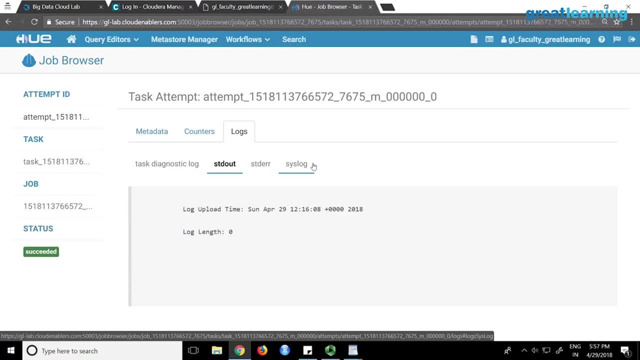 because they will collect three days worth data. third day, 12 o'clock, this program will run. so once you write a program forever, it runs. it is not like every time you're writing a new program for the business use case. you write a program that keeps on running whenever you want. 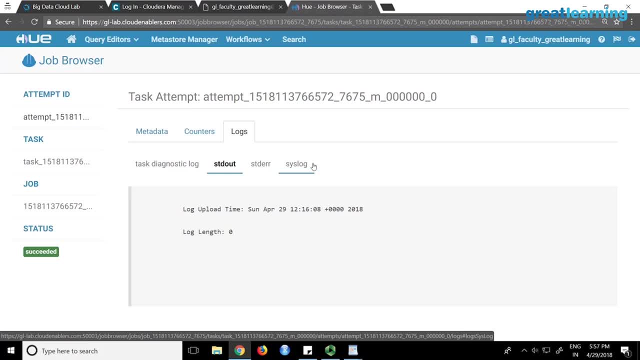 if you are having things like splunk and all, it can read. okay. if you are using bi tools- i'm not 100 sure- like this tableau and all, i think it has to be in a tabular format. you are learning tableau, i think right, tabular have not worked. splunk i have worked. splunk can read from any textile and 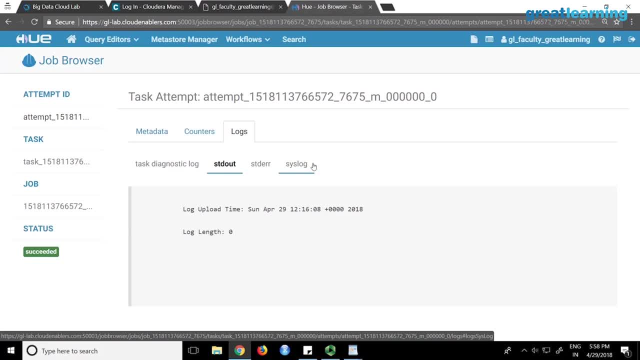 visualize whatever you give it's possible plan can work with any type of data, even from hdfs. so there is something called hunk, hunk, hadoop on splunk, a splunk on hadoop. sorry, that's called hunk we have. okay, you can google actually hunk app we used to install, so hadoop plus splunk is called. 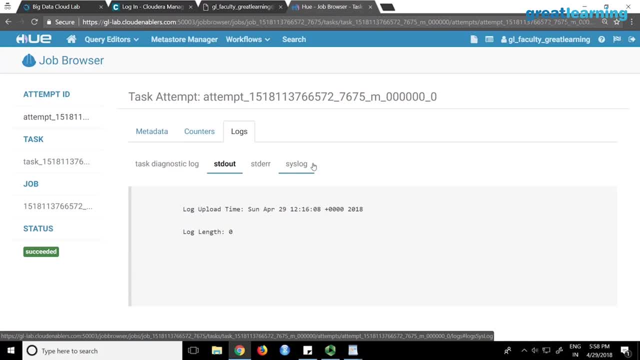 hunk. so there is an integration between splunk and hadoop. it can easily read and write to hadoop. so, uh, monitoring this job will. uh, this job browser will help you to monitor. right now the job run really fast if it was a end uh forever running job. one ways you can track from here, another way there. 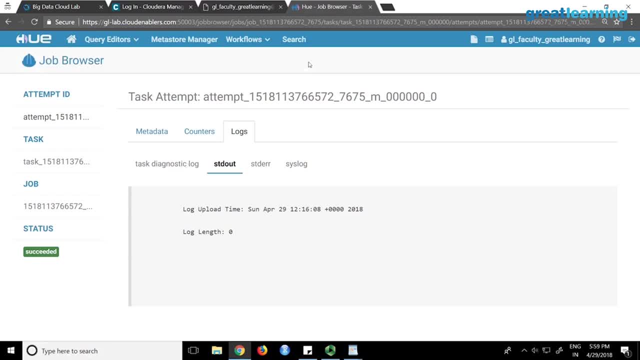 is a resource manager ui but i will try to fetch the ui. i don't have it right now with me. the manager ui i will show you from there. it will show running jobs how much percentage it is complete mapper: 33 percentage, 40 percent. you can figure out. there is some time it is going to take. 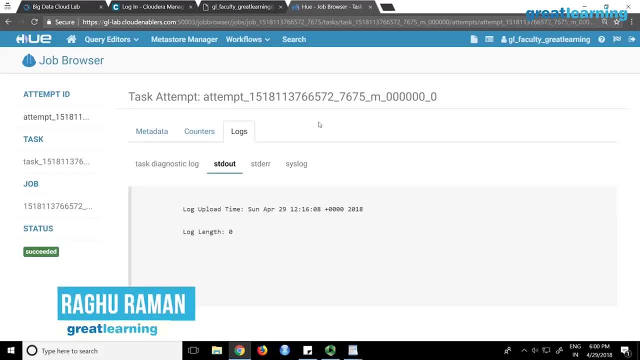 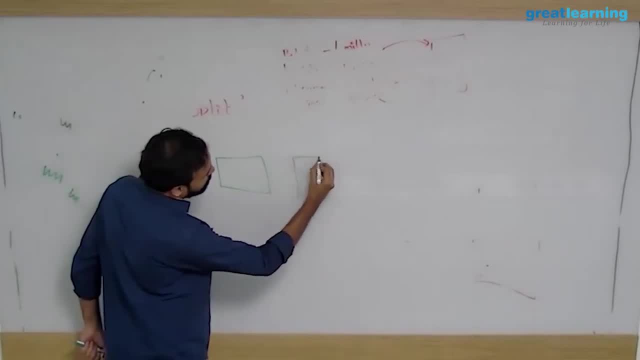 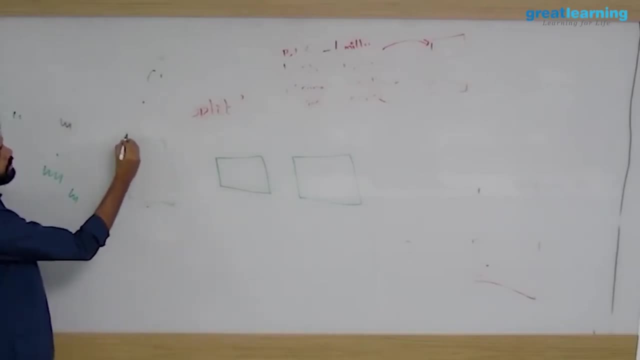 so i need to talk a little bit about yarn, okay, because otherwise i will not be doing justice. see, the idea is very simple, right? if you have two data nodes? okay, and we talked about a master, right, there is somebody called name node. i told you that this is the master for. 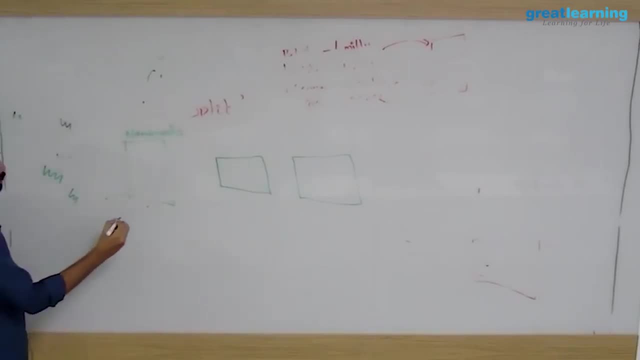 hdfs. this guy is looking at where is your block and all. there is also one more guy called resource manager. he is also a master. this guy is part of yarn. so when now we ran the program, the program will hit this guy. the jar file you created will hit this guy, resource manager. 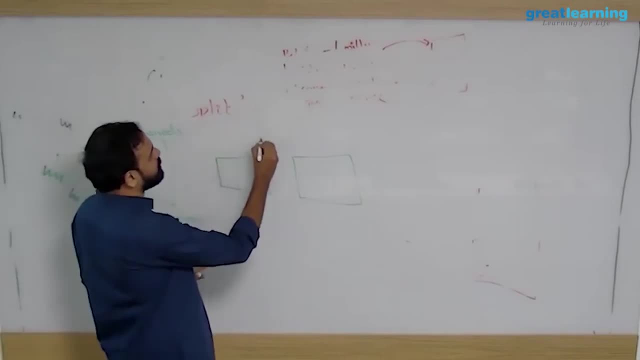 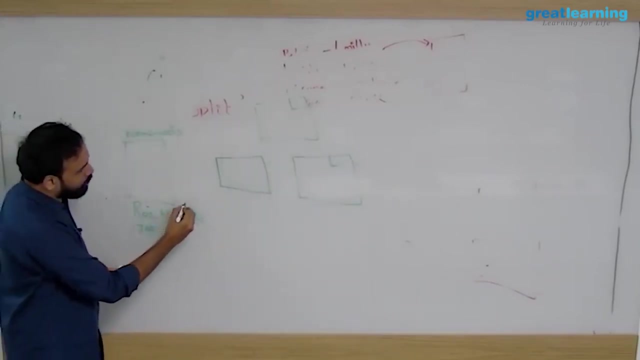 and what this guy will do. let's say, our data is in three machine machines. okay, data is here, data is here. this guy will contact one of the other machine. okay, this is a slave machine. okay, and this machine will launch a process called app master. it's called application master. it is launched during the program. it will not be there. 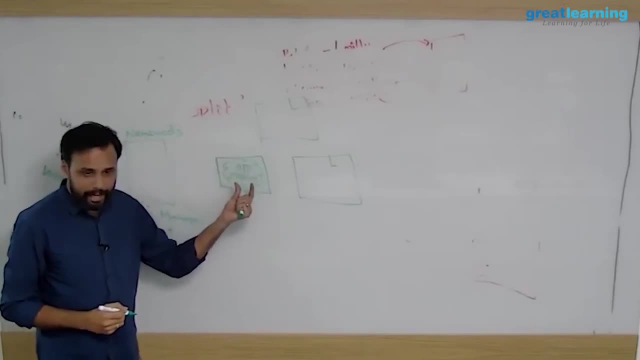 once this guy is launched, this guy will decide how to run your program. so, ideally, when this guy is launched, he will look at the. just because this is not the straight line which we like to see, because if it is not there, then we have come to current process. 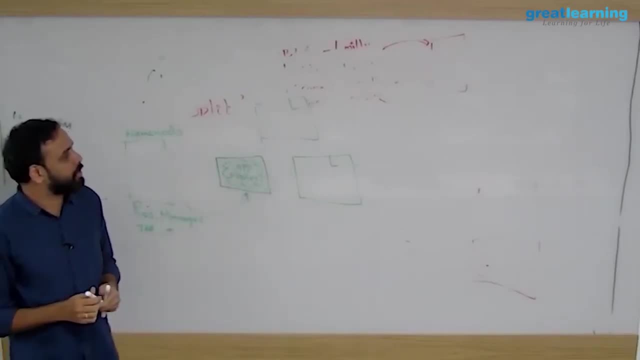 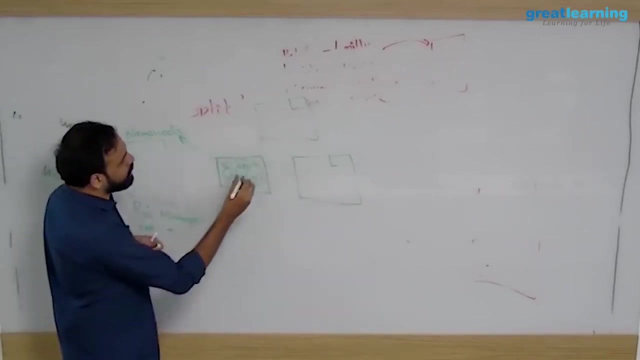 will look at the data you want to analyze. so we have said we have said that the data booktxt, some text file, it is available here and here. this guy will talk to your name node and understand where is the data. so now the data is here and here, right? so this guy will then talk to these. 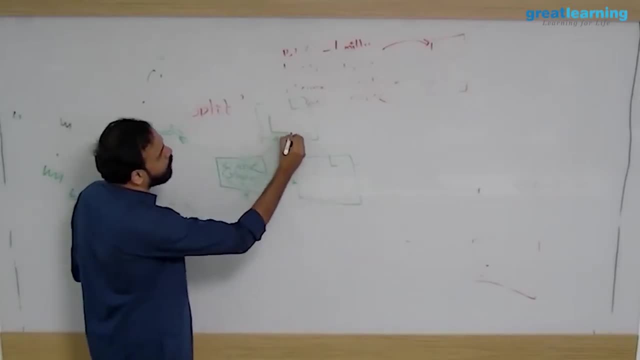 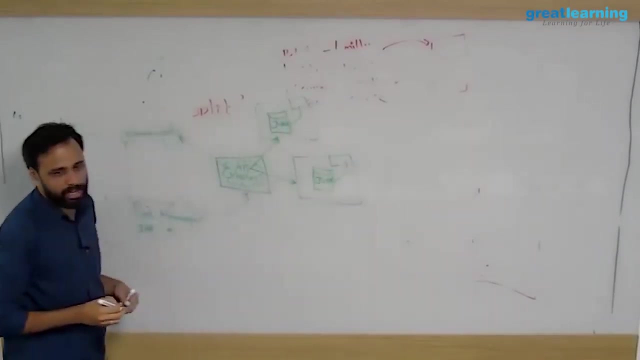 two machines, okay, and ask them to launch one one jvm, this guy will launch one one jvm and then the block will be copied here and that is how processing happens, because if you want to run any processing, you need resources. resources should be the ram and processor, and all they are dynamically. 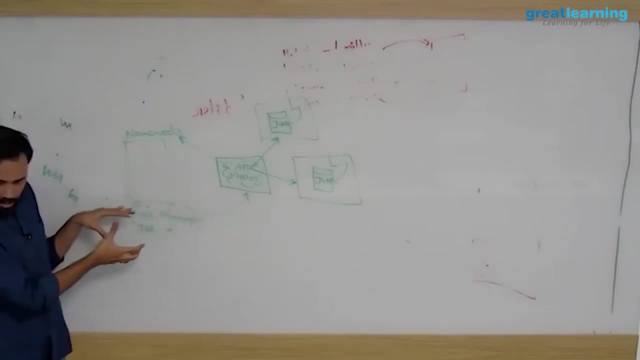 allocated by yarn. this is all yarn framework. so the master will pick your program. it will ask one machine to dynamically launch this app. master. this will start. this will talk to your name node and understand where is your data and will contact these two machines and say that you know what you. 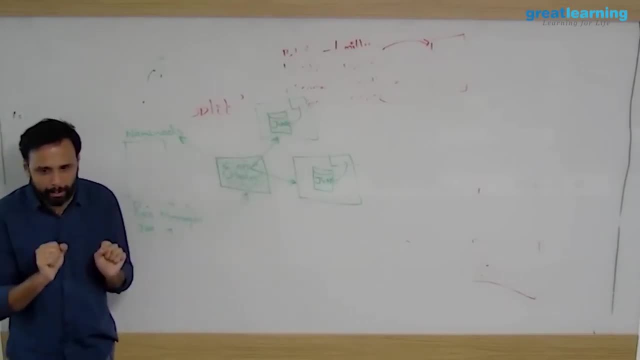 have one. one block will first give you the mapper. i have the mapper ready with the entire map. reduce with this guy, it knows where is a mapper reducer. it will say that my mapper is ready. launch two jvms. i'll give you the mapper. these two machines will launch to two jvms. your blocks are loaded here. input split. 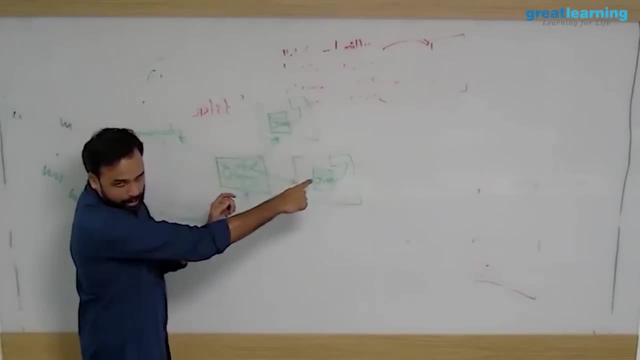 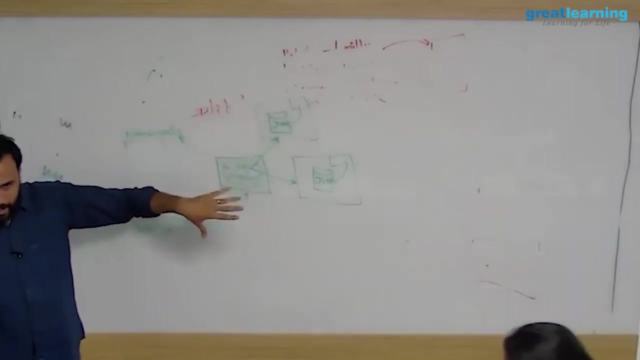 everything happens. first it will push mapper mapper. mapper is over. let me push reducer. probably reducer is only here, there, and your output is collected. so, and once the entire code is done, jvms are deleted, atmosphere is deleted, everything back to normal. so this is your yarn framework. actually, i mean, how so this resource manager has a ui? 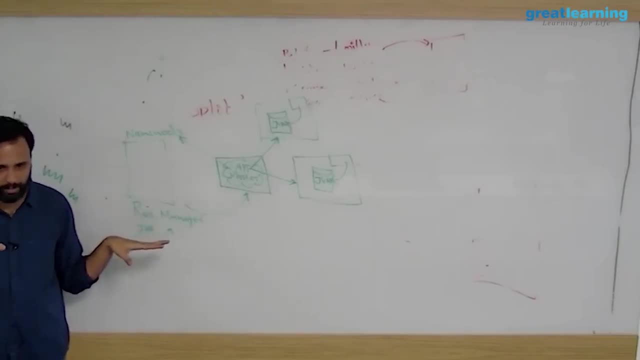 using that you can see how many applications are running in your cluster right and resource manager can accept any type of application, not only my produce, spark these. any framework you write and give your yarn will accept and run it for you. so if you submit the jar, it goes to resource manager. this is a server where two masters are running. one master is named. 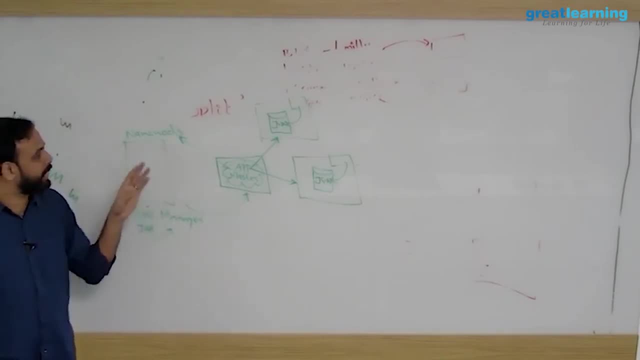 node. he handles only storage. he does, he has no idea about processing. resource manager handles only processing, he has no idea about storage. so normally in a hadoop cluster you will have a master machine where- uh- resource manager name node- all the master demons will be running master processes. 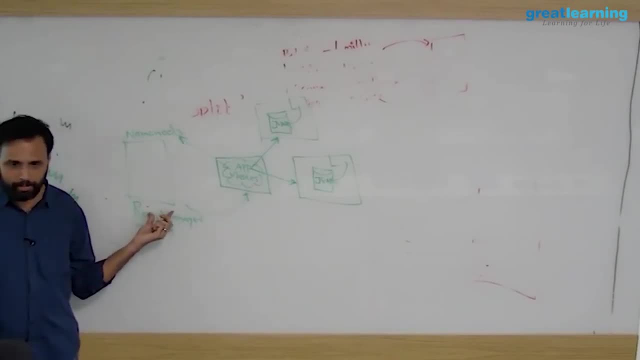 will be running. so if i submit my jar, this guy will pick it up right. and then this guy will contact one of the node, any random node, and ask it to launch this process called application master. now, this is delegation of job, because this guy cannot run your code. so it says: app master, you run. 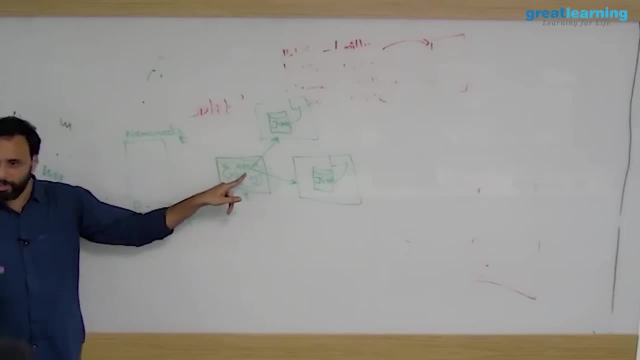 it. now it is the responsibility of this guy to figure out where is the data and ask these machines to launch containers and give the code and ask them to run. even in a spark, it runs the same way. spark also runs the same way. in spark you have something called executor. these are called. 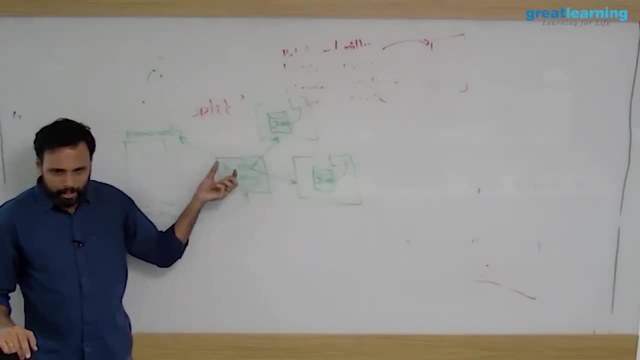 executors and spark and spark driver will be running here. it will push all your logic to these executors, right? so the mapper code will first push to both the machines, they will process it, and then the reducer code will push to whichever machines. but your yarn decides. so now the question is: what if 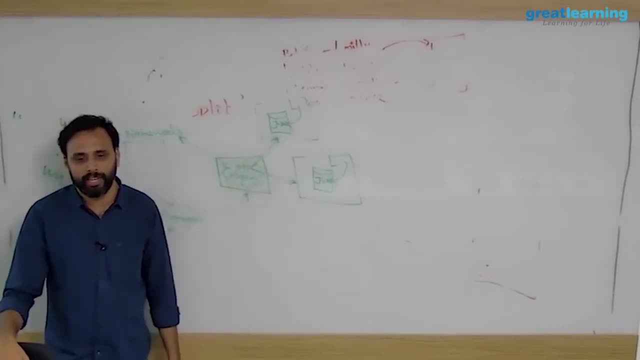 this machine says i don't have resource to launch a container, no problem, it can be. but now the situation is what if this machine says i cannot launch a container, i am already busy, i am already running lot of programs. i don't have resources to launch a container. this will be already identified. 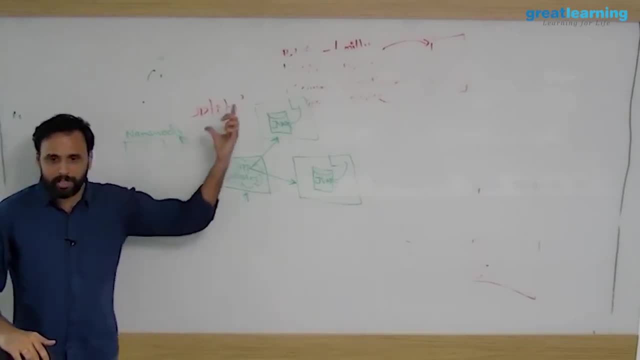 okay, because the solution is already there. resource manager tracks all the resources. it knows who is busy, who is not busy, so it will tell the app master. you know what i know? your block is here. don't go to that guy. he will not give you a container. go to the replica, so resources are dynamically tracked. actually, right, and once the 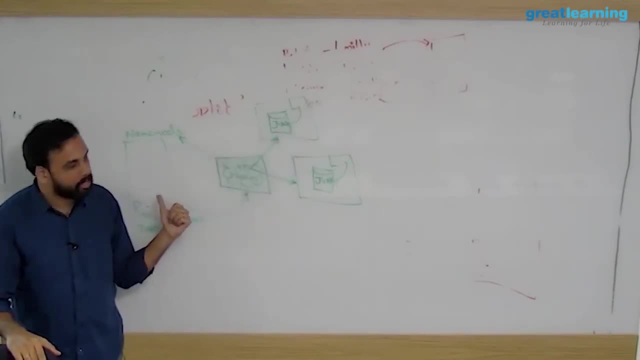 mapper runs in a jvm. your resource manager will say that don't kill the jvm because the reducer also need to run on this machine. probably you can use the same jvm, right, why should you kill the jvm? this jvm will be killed because once the mapper is over here, this guy has nothing to do. it will kill him. 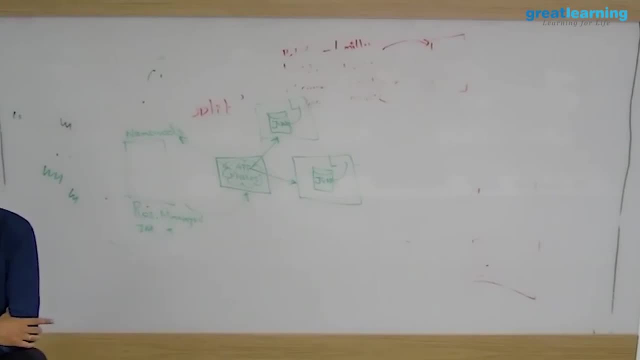 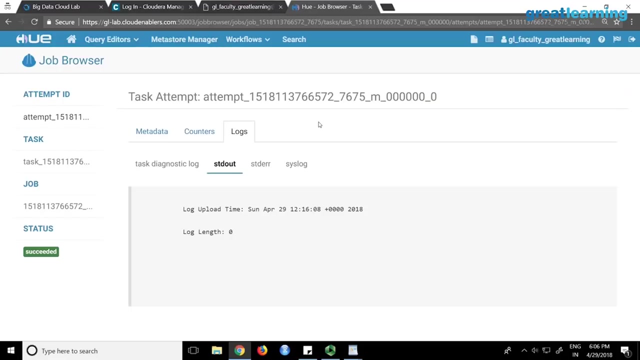 so this dynamic resource management is done by yarn. it's very, very important in hadoop. actually, all these guys- resource manager, app, master these containers together. that framework is called yarn, your processing framework, resource management framework, our resource manager. this is the master guy. he will be controlling all this because if you submit 100 jobs, 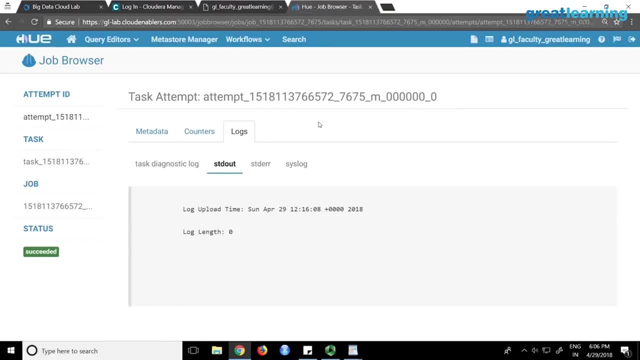 right. this guy cannot run 100 jobs. he will launch 100 app masters. it is like your ceo: you have to work and give back everything to the project. what happens if a project comes right? you are getting a project in your company. who will get the project? probably the ceo will get. 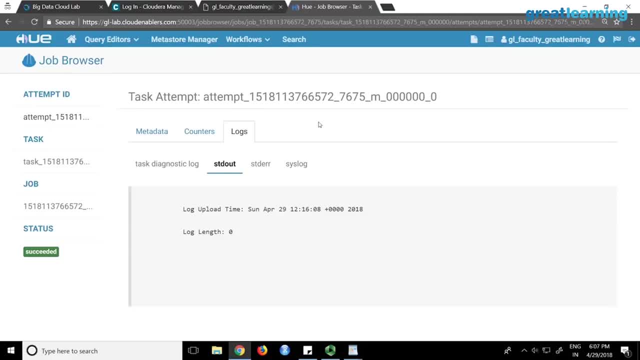 the project right? just taking an example. okay, so the ceo gets the project and will the ceo actually write the code? what will happen? he will contact a manager. that manager is this machine. will the manager write the code? manager will contact another machine and ask an actual coding guide to start working. 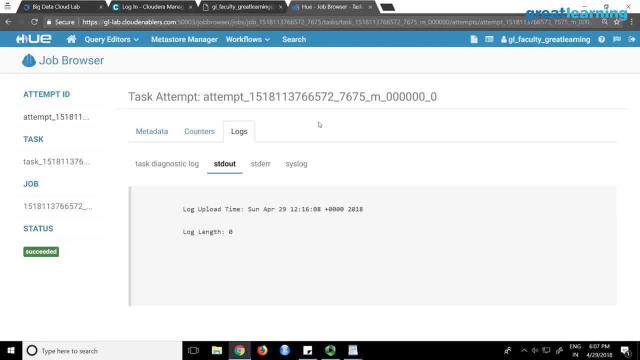 So the manager is simply passing instructions. This is your level 1, phase 1 of the project, phase 2 of the project. do this, do this. So this guy, this app master, is like a manager. His job is to ensure the program goes to everybody and everybody runs. 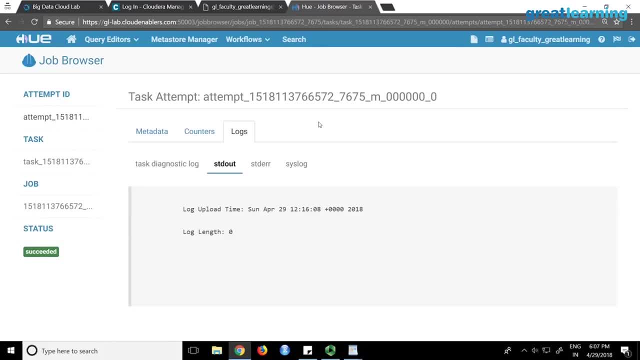 And if anybody dies during the work, meaning if that JVM crashes, that machine goes down, it will tell the resource manager that one guy has died during the work. what should we do If there is error? get another guy? very simple, right. 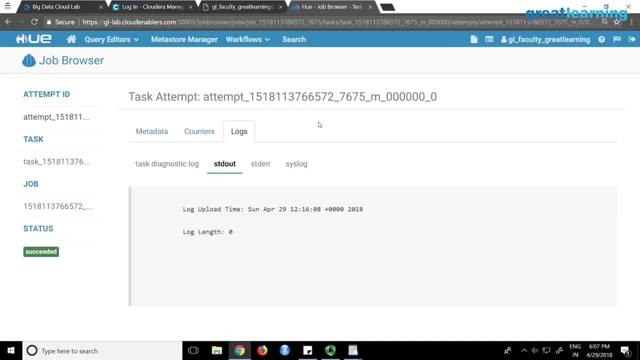 You have a replica block, it will start on another piece of machine. very simple. Finally, you saw the output right. That will be read and collected by this app master. This is the guy. so actually it is not the app master. within the app master: your MapReduce. 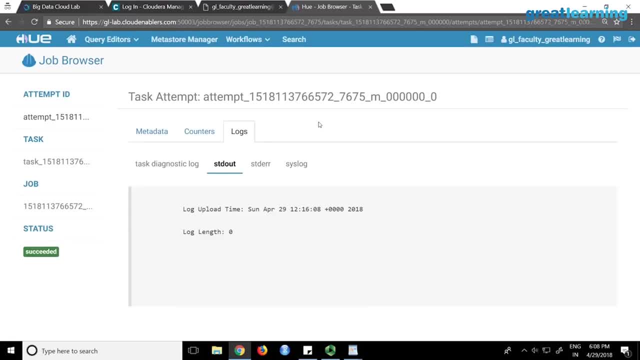 driver is running. In the driver you have set, which is the set mapper, set reducer classes, right. So the app master will pick up first the mapper class and send it to these guys and say: complete the mapper phase. Once the mapper phase is complete, 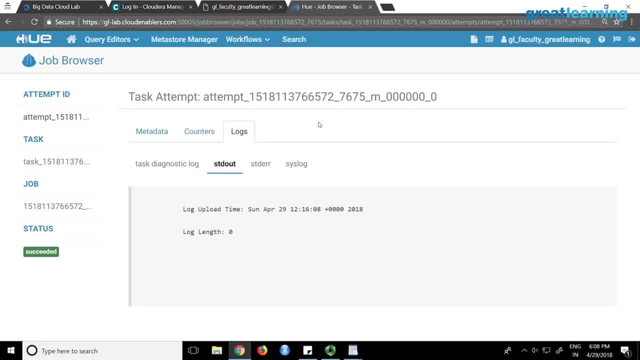 Shuffle will happen automatically. Then it will say: I am sending you the reducer code. run this code. So the business logic will be there with app master. it will not run it, it will just push it to the workers, like your manager. 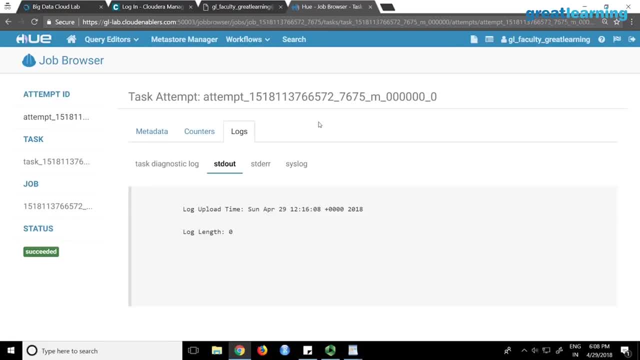 He will say that this is what needs to be done. I will not do it. you have to do it and give me the output. and all of this is highly available. Anything crashes, it will rectify. For example, app master can crash. the machine can crash. it will be notified to resource. 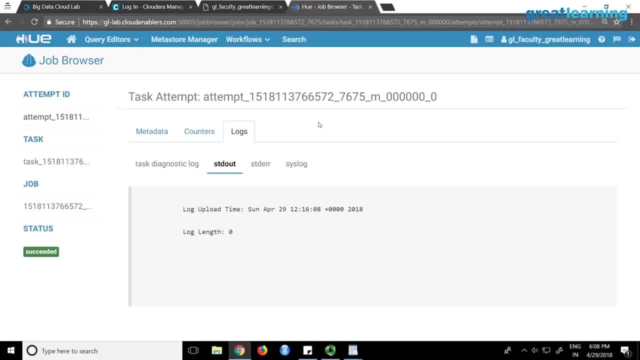 manager. he will launch another app, master Right. All of these are check pointed. these progress. So resource manager knows still what this guy has done the job. The manager can quit from the company right During a project. Does that mean the project will get hold? 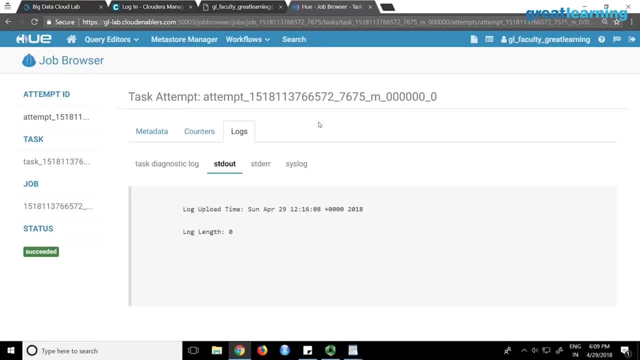 No, another manager will come. he will start from where this guy left. No, I am saying this guy crashes app master. The intermediate data is pushed in hard disk also, so you will not lose any data or anything. in this example, App master's status will be communicated with resource manager. 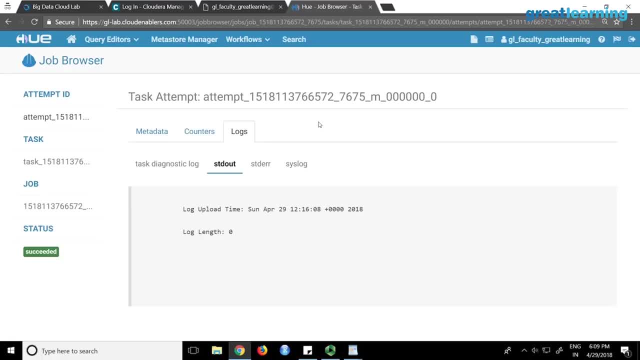 It is in constant touch with resource manager. Mapper's local output is in local file system. Mapper output is in local file system. So there is something called job information. It is a bit complicated. That is why I do not want to talk much about it. 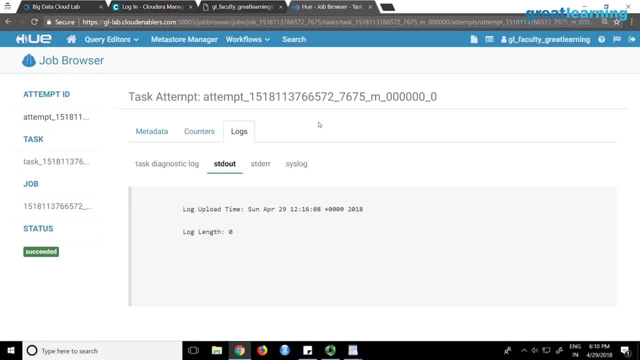 There is something called Job Information and Job Stats, like what is happening in the system, how much the mapper is completed, how much the reducer is completed. So these are your job statistics That will be constantly communicated with your resource manager, And the resource manager knows this application is running. 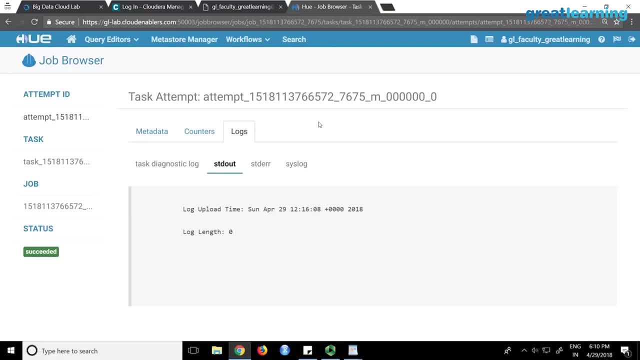 It is the, Even though the job is app master has nothing to do with the job. your project is happening, the coders are coding. does? 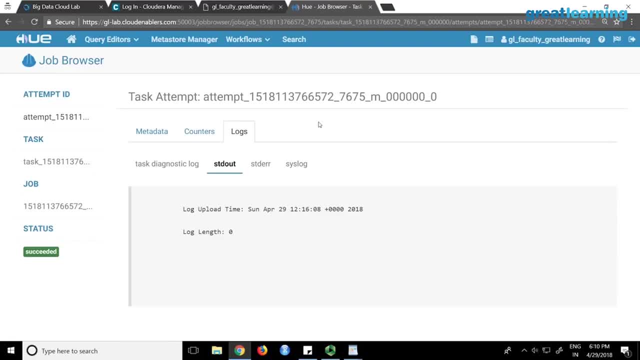 manager has anything to do with it. he is just controlling. so if the manager resigns today, tomorrow, if somebody comes, what you do, the ceo will already know the status because he could have been in reporting. he will say that from here you start like that, a new app master will be. 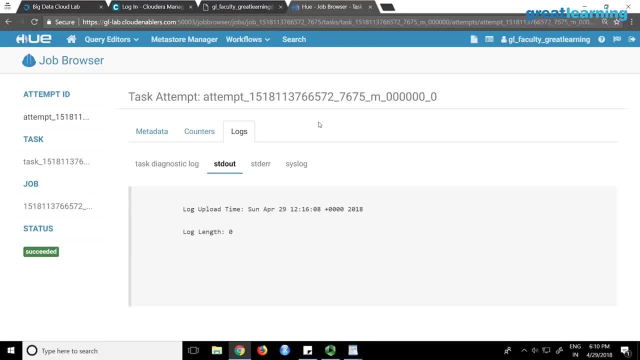 launched, relaunched. okay, that day will continue from where this guy has lived. so job information can be periodically saved- what is the status of your job and all- and he can simply query- right? he can simply query the containers and understand what is happening, right? so this is all highly 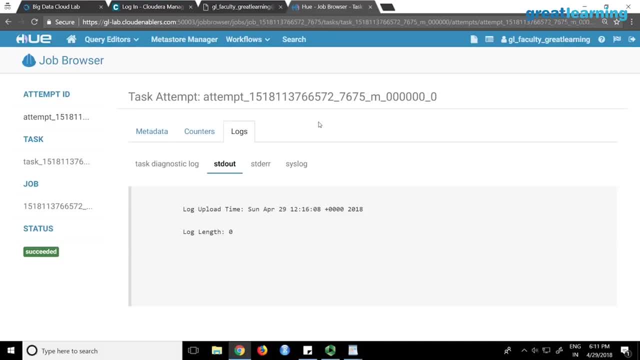 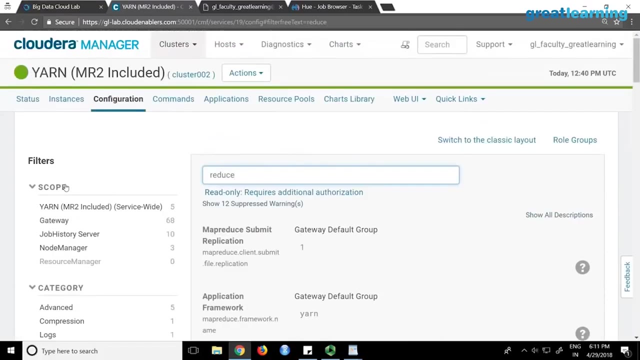 available. whatever is this job execution resource manager can be too highly available. so, resource manager, we can see. right, there is no direct access to this guy. i was checking the cloud manager. so if you go to the cloud manager, go to yarn. this is yarn, right, if i? 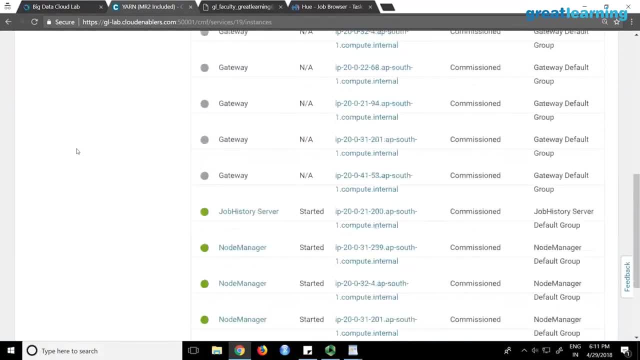 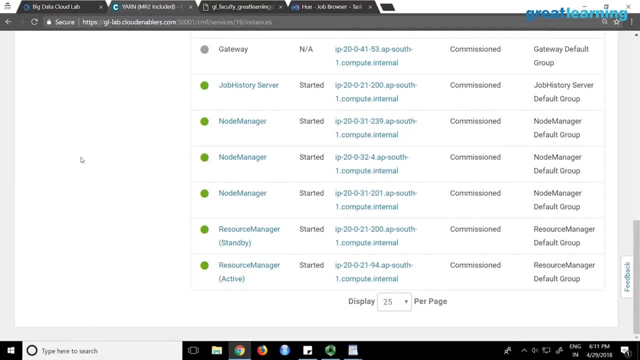 go to instances in yarn. um, can you see this? what is this active and how many resource managers? two, right, so you have a ui for resource manager but it is blocked. for us only active resource manager is running. standby is like high availability: if the active fails, other guy will take over. like you have a what you say, precedent and what what you have. 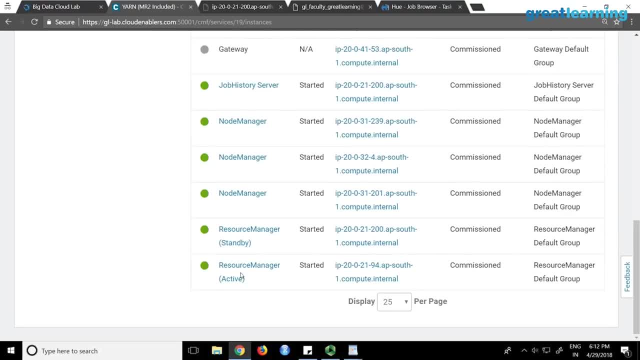 vice president: right. only one guy can be there. if president is not available, the other guy will take over. like that: for high availability we configure two, because there is a chance arm will go down some reason. right for that, like: if you are having around 300, 400 nodes, okay, then i can set up. 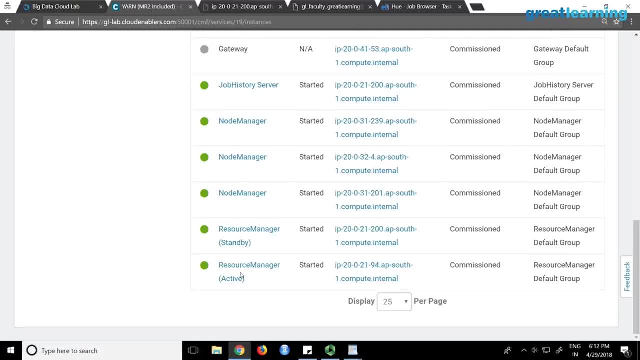 a master box where name node will be running, resource manager will be running. but if the cluster is very big, right, the reason is that name node will require a lot of ram to store the meta data and access on top of that resource manager also requires. so we will build them in separate. 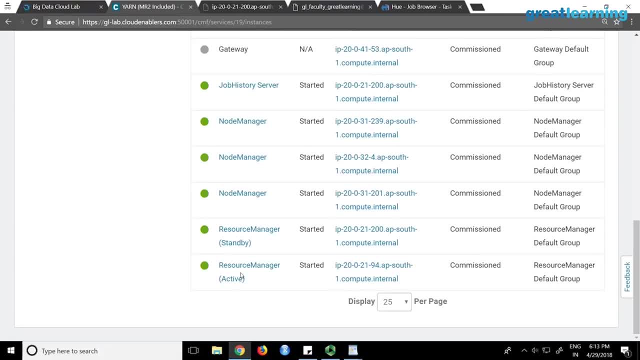 machines, not one machine can be one machine or two machines. you can do that. so i will tell you this. i don't know whether i'm supposed to tell like you can. you can get these quick start vms. probably you're aware of it, right, some of you might be aware of it. you can go to clouderacom. 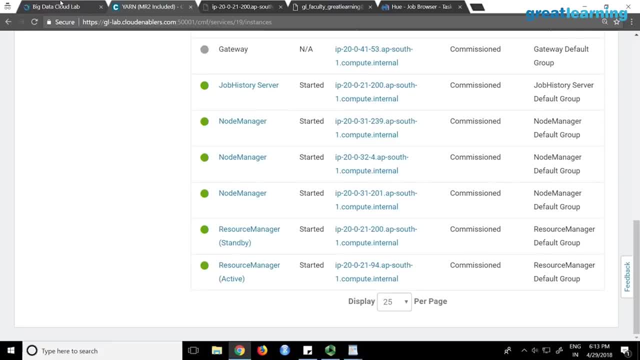 they will give you a vm for free. download it. install it. only drawback is you need 16 gb ram laptop. start that vm, it will have everything. so data security: it is a big question because it all depends on your company. only, like when we were working with icica bank, some of their data was. 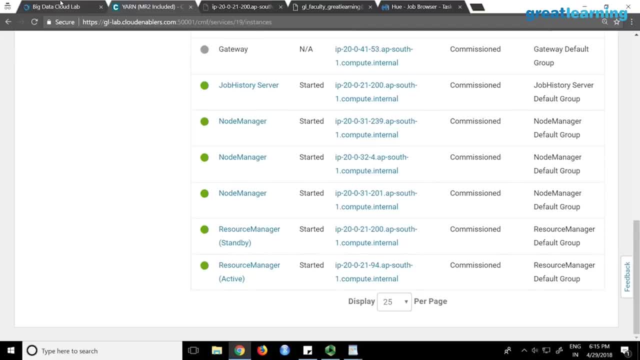 so secure. so they said: uh, you know we will not keep it on hadoop. some transactional data was there. some was very sensitive data. so they said we will manage it ourselves. they had their own data warehouse or something. if they allow us, hadoop has lot of security if you're storing the 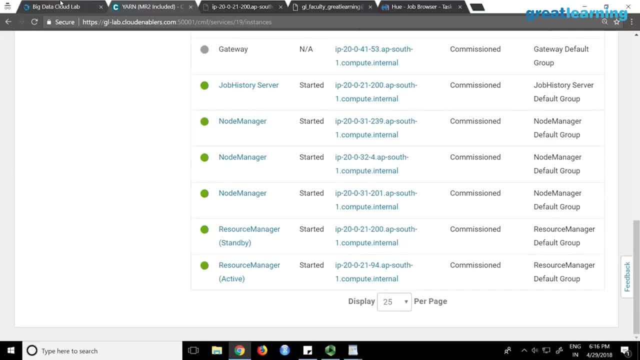 data on hadoop. it is secure. actually, it's a common security platform. we have something called kerberos and then there is something called sentry. these are the tools which will manage security. it's not company wise, for example. it is a service, right? so if, if, uh, you know, apple says that, 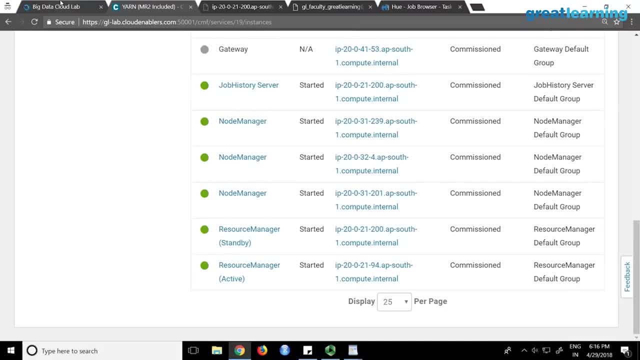 their mobile phone is secure. it is for everybody, not for a company. right common security they have like that you can secure. all the data can be secured. correct yarn is designed in that way. yarn can handle any type of workload. also, you need support, for example if you have written a python. 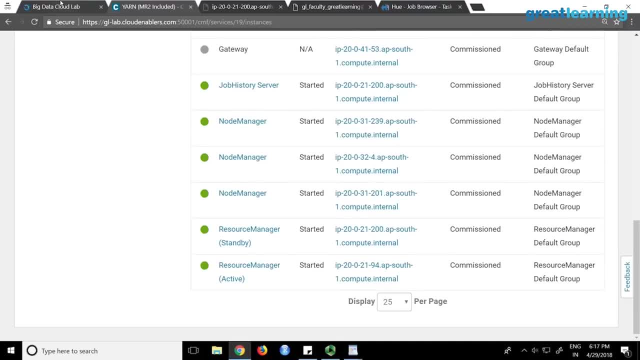 using python. python has to be installed in all data nodes, otherwise nothing will work. a scala program and same jvm can be used. scala uses jdk, only so, but python. if i'm running, if python is not installed, my yarn will say that i don't know what you're talking about. so python. 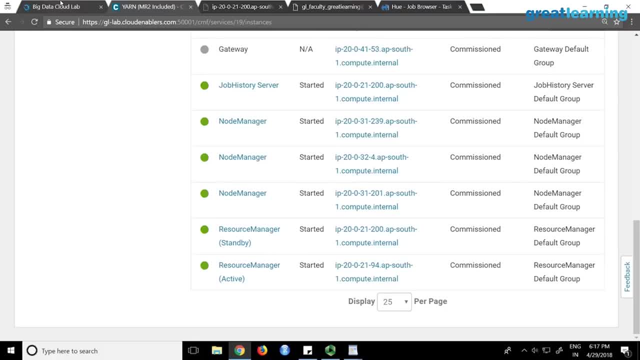 has to be installed, so these binaries need to be there wherever you have support, depending on what program you want to run. so jar is nothing, but inside you have class files only, right. so jar is not passed as it is. jar is what packaged? class information only, so it will fetch these. 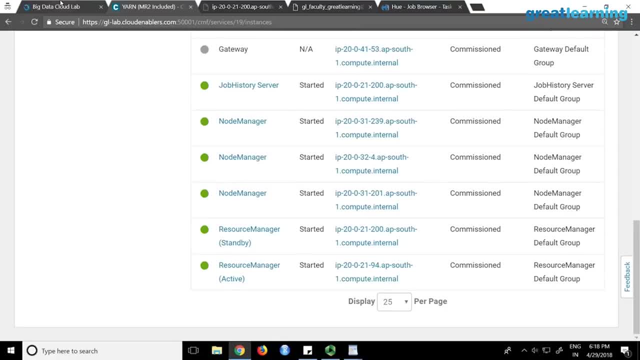 individual classes, your mapper class, reducer class. yeah, so, uh, when your program map reduce actually runs, okay, the jar file will be read initially from your, from local file system. your jar is there, then, uh it, before actually the map produce program runs, this object will be initialized. new configuration object. it should know. so now next question is that: how do you know? 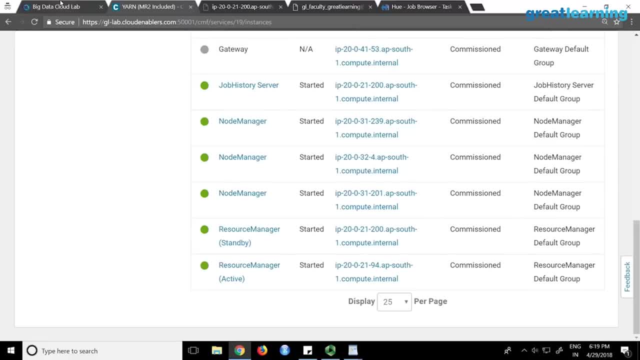 where is the resource manager? right, you don't know, the program doesn't know the program doesn't know where is the resource manager or anything in a hadoop cluster. so, using this configuration object only, it is reading the cluster configuration. whichever hadoop cluster, you are submitting the program and then it finds out the resource manager and 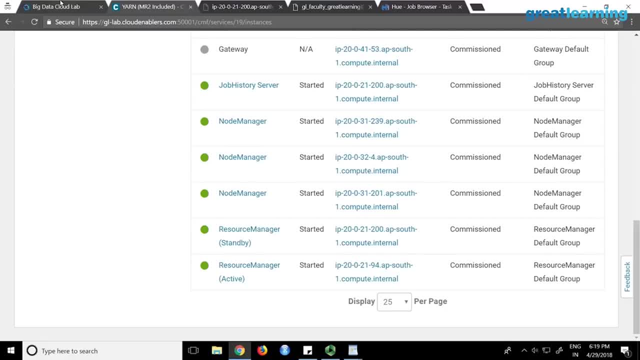 goes to the resource manager. once it reaches the resource manager to delegate to an app master where the class files will be identified and it will start running individual mapper class and reduce the class. once app master receives your code it will read the driver and delegate with the resource manager. so i can say that i want 10 reducers in in my 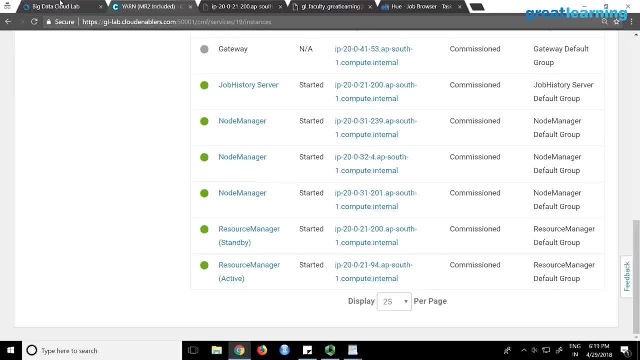 code where i will write it in the driver. so, before it runs, the app master has to get 10 containers right. it will talk to the resource manager and say that this guy has written he needs 10 reducers. please allocate. i'm going to run and the resource manager will say that i'll give it to you. you run. 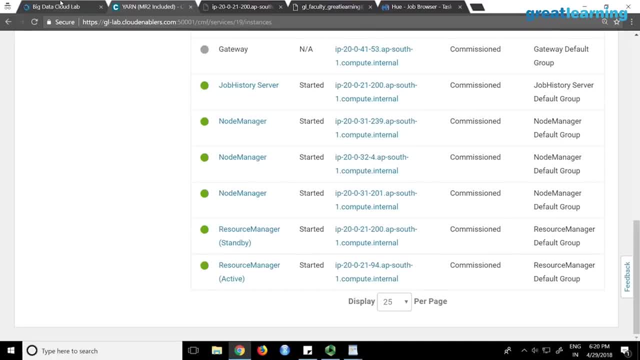 because the driver is running only on the app master, so app master will read your driver configuration. so this is more valid in spark because in spark, in the driver, you can say how many containers you need, what is their ram, what is their core, everything. all this will be read by this guy and this guy will tell, go to the yarn and say that you know. 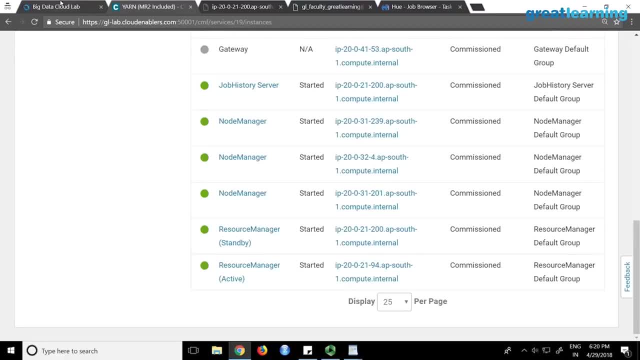 this guy is asking for these many containers, can i give it? once this guy say yes, then only the program runs. so you cannot say that i want 100 containers, thousand containers. probably those many resources are not there in the cluster. so either your program will wait in a queue or it. 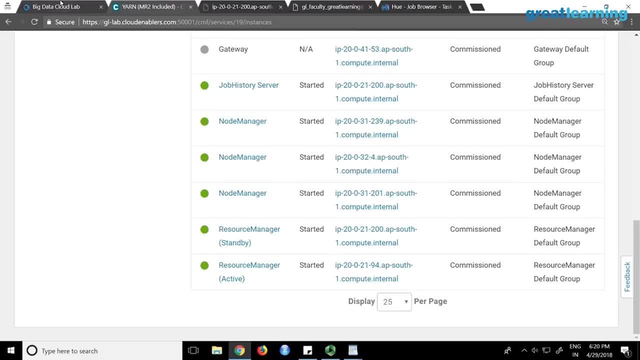 will get lesser containers where it will execute very slow. that is also possible, right? so this will run in the cluster. driver actually runs there. resource manager will say that it will know total resources in the cluster. right. app master will say that i need these many containers. so 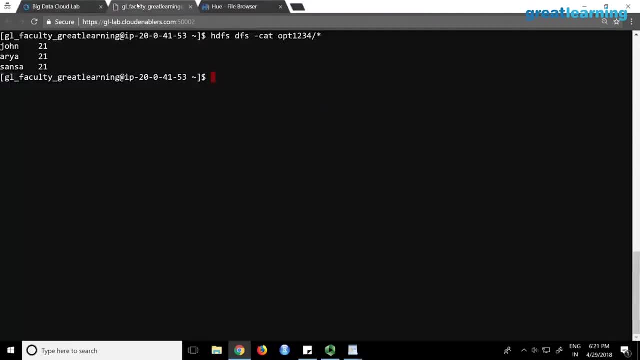 this guy knows whether i should give it or not, right, yeah? so one more thing i wanted to tell you was that if you look at the output, right, see, i'm doing an ls of opt 1234. yeah, so you have three files, right, but how do you get the output in a single file? many times that's a concern, because you may be. 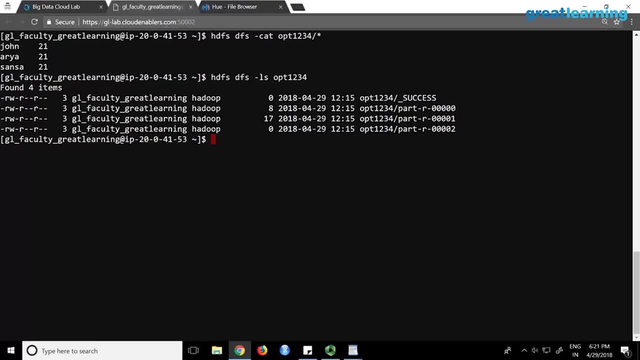 running with 20 reducers. 20 reducers will produce 20 files. i don't want 20 output, i want one output right to do that. you can simply do this. that will simply indicates your program ran successfully. that success means it ran successfully. if it failed, there are other error codes right, one fail. 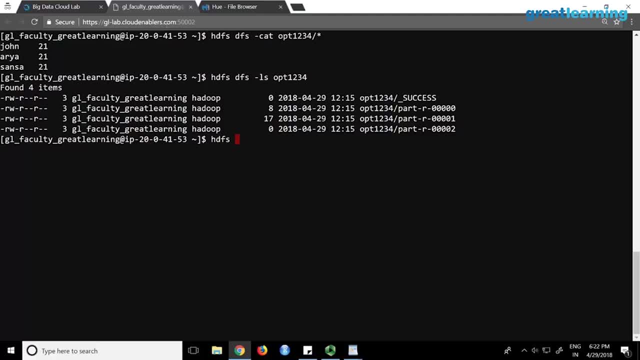 with error code one, two, it will show there. so by looking at that you can see what happened with the program. so you can say: hdfs dfs- hyphen- get merge, okay. and you can say opt1234- slash star. let's say result dot txt. run this command, all of you. hdfs dfs- hyphen- get merge. the final, the output folder. 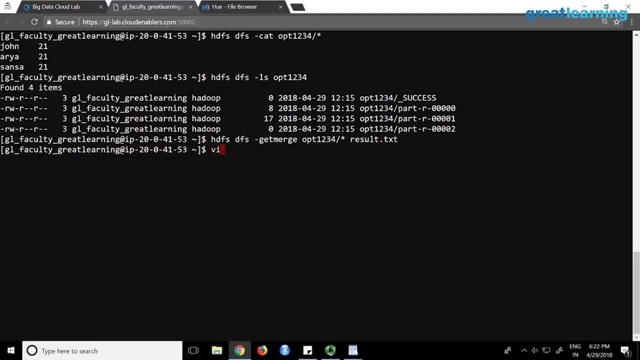 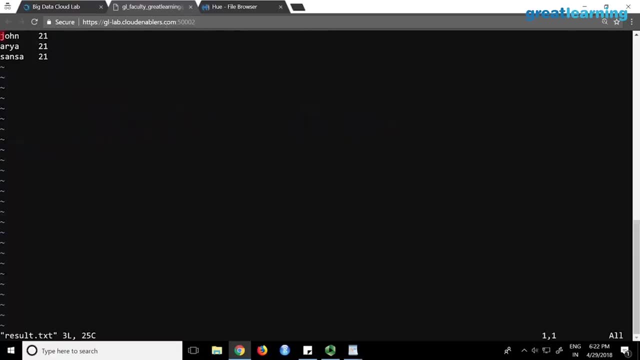 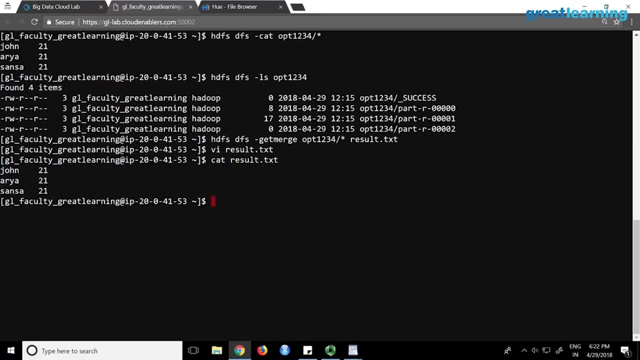 slash star the result: dot txt. now if i do a vi- result: dot txt, i will have the output. or i can say: cat result dot txt. so you are down. you are combining or merging all the output files into a single text file and downloading to linux. are you able to? 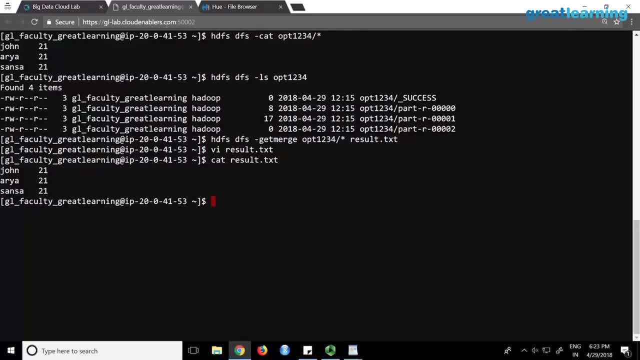 understand what i'm doing. the get merge command will merge all the files from hadoop and download as a text file to your linux file system. then you have to upload it to your linux file system again. i don't know whether there is a command directly merges there. get merge will get it. 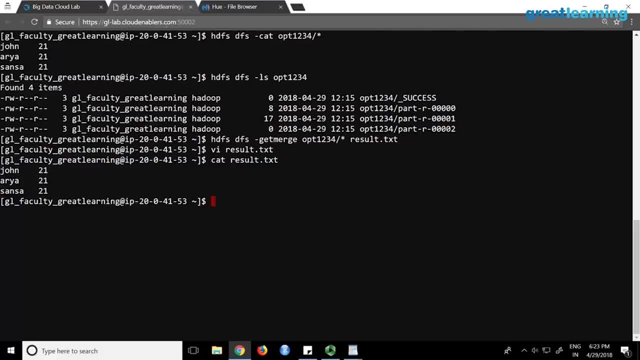 then probably you can upload it there if you want. ah, if it is too big, you can't do a get merge directly because the size also has to be considered correct. we will, so ideally this get merge is not everywhere used. okay, this is just to show you that we can merge normally. we will keep. 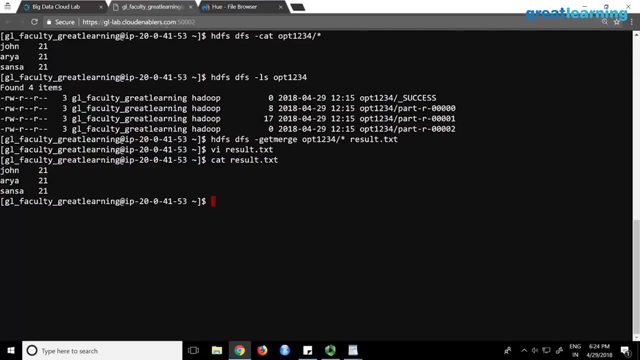 it as part file, then the problem is you have to write another java program to combine the outputs. if you want map reduce program, right, huh, so that is another problem with map reduce right. so anything you write again you have to say that, okay, this command will do that. if you want, you can. 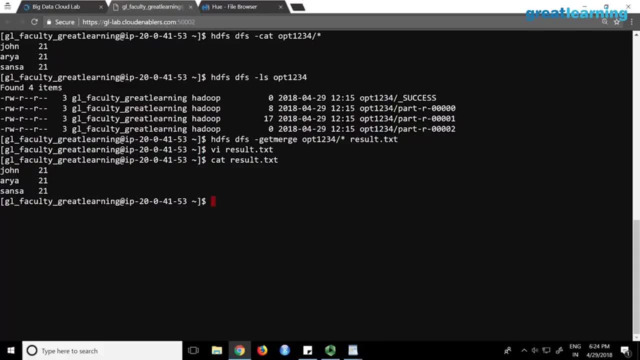 manually download and you can say: get and get the file and merge it. if you have a very big box, and download and merge it, ah, so you don't have to run the map reduce everywhere. see, you have a very big box, you download the files and merge it yourself. normal java program. you can write these: 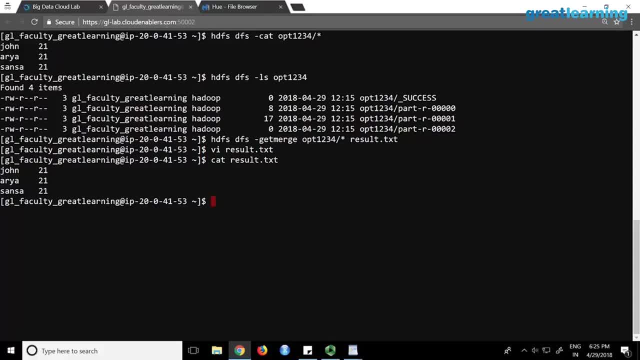 are normal text files. probably your gateway node is very small. okay, you can download to other machines also. right, it should not be always the gateway node, right, you know, you have got all the right. i can get it. or i can get it to amazon s3 or somewhere and then say: merge it from there.